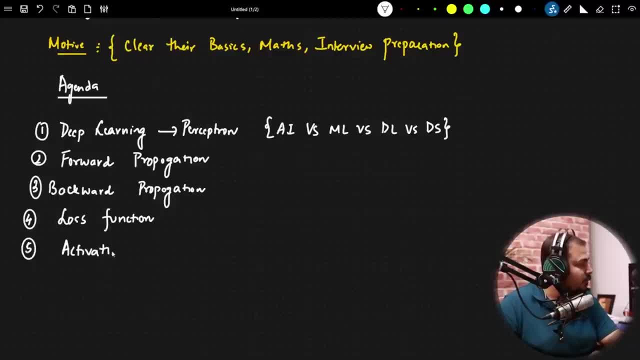 Fifth one is something called as activation functions- Okay. Sixth one that we are going to basically see is something called as optimizers- Okay, So we are trying to cover all these things. If you are in the thousand feet height, right? What is exactly deep learning? 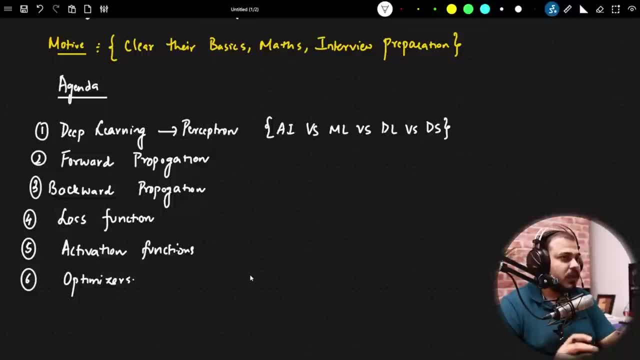 Why are these terms coming up? You know, all those things we'll try to discuss tomorrow. We are: Yeah, Projects will also be covered. on the second or the third day We'll try to cover projects and we will be learning in such a way. 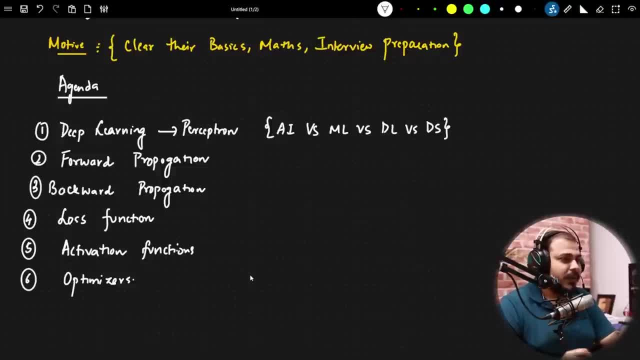 That we understand the maths, We understand it properly, We we do the implementation and at the end of the day, it will be helpful for the interview preparation. So, yes, I hope everybody is ready. The energy is high, So hit like we will be starting the session right. prerequisite: some idea about machine learning. 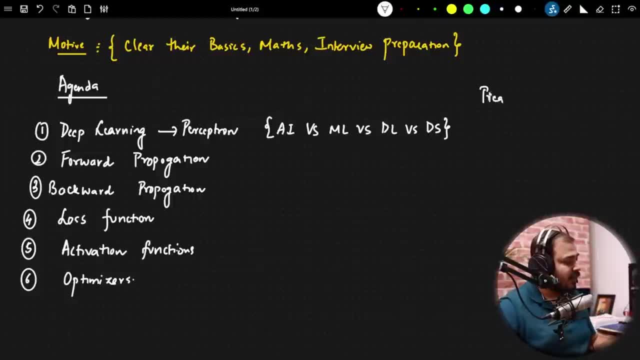 So your prerequisite is that you need to know Python programming language prerequisite. You need to know number one, Python, some idea about at least one algorithm in machine learning. And third, is that some idea about stats, which I have already taken in the previous session. 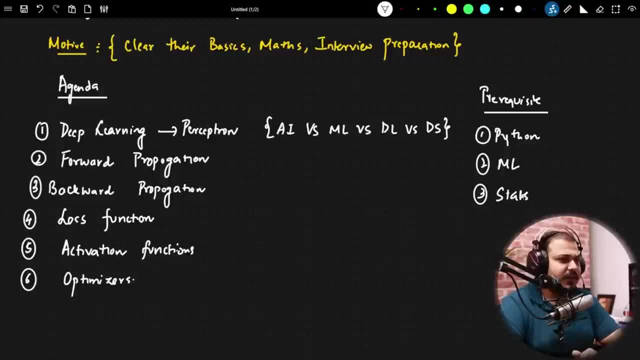 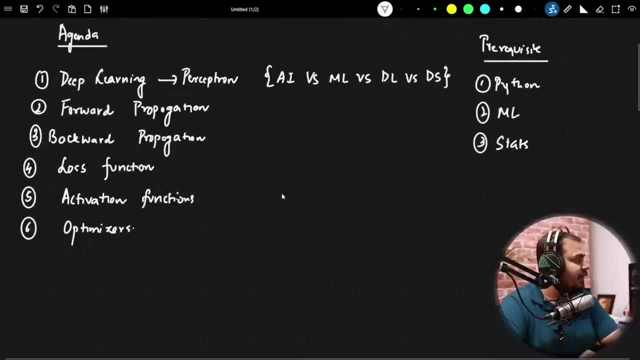 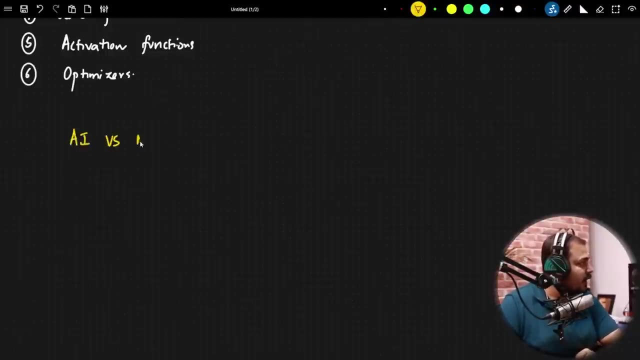 OK, So we will try to cover all of this. Yes, If linear regression also. you know that is more than sufficient to start with. OK, So let's go ahead and let's start the first thing, The first topic of this session. we are going to cover something called as AI versus ML versus 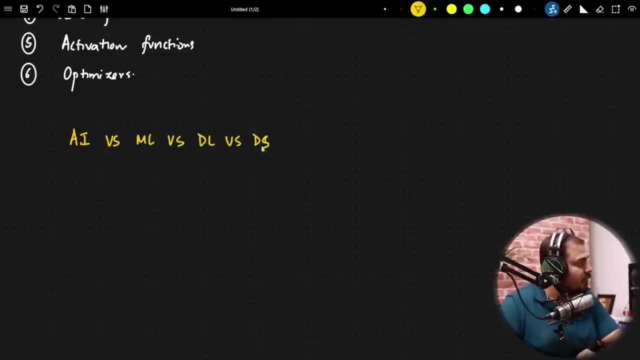 DL- DL versus data science- right, And what is the importance of DL? We will be trying to know- and deep learning- This is this will be our main focus of this session, where we will be understanding about deep learning. OK, So this is what we are basically going to cover up. 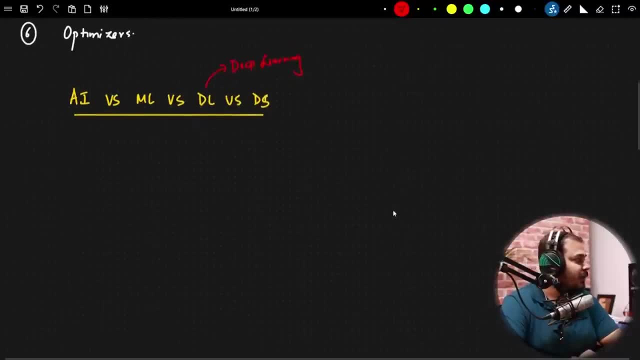 OK, So perfect, Let's go ahead and let's start. OK, Let's consider this entire universe. Let's consider there is a universe which is called as AI. OK, So Suppose if I say this is my, this is the universe of AI. 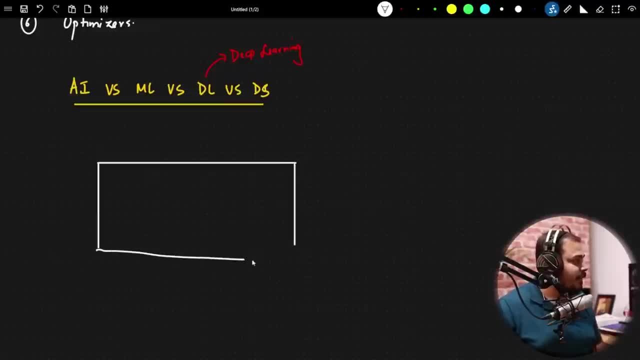 This is a separate universe. Let's say, consider it AI, And I hope everybody knows the full form of AI, that is, artificial intelligence. So here we try to create an application. So AI is a kind of application which can do its own task. 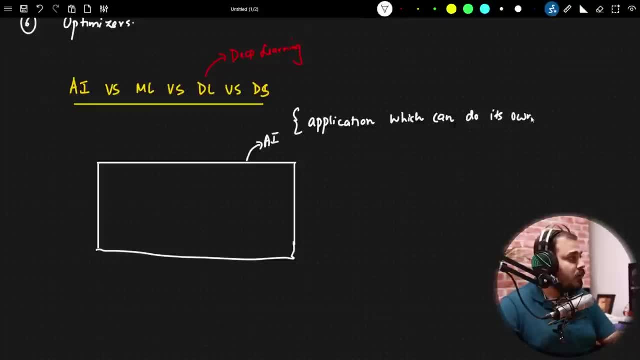 It can do its own task without any human intervention, Without any human intervention. OK, So this is what is exactly AI? OK, Without any human intervention. So human intervention basically means that the human do not have to tell the application what to do, just with the behavior of the user, of the person, that who is using this application. 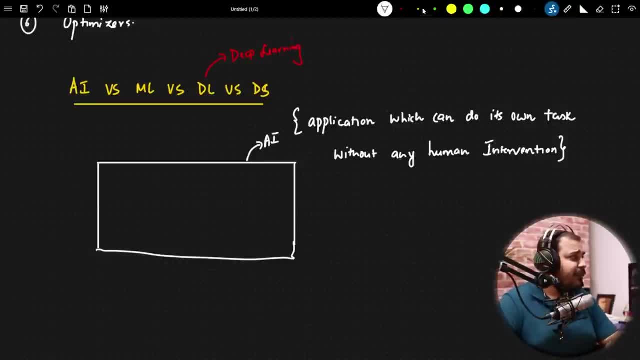 It can automatically take its own decision. Best example that I would like to consider. Number one: I hope everybody has seen Netflix app. It provides you automatic recommendation. Second is self-driving cars: Autopilot cars, self-driving cars- I think you have a brief idea about it. 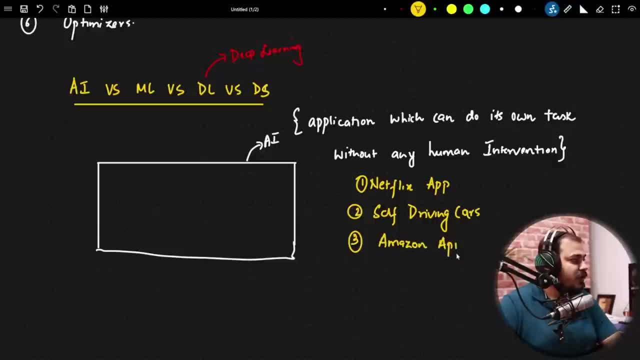 Third, let's say Amazon application. So I am his own application which, wherever you do the shopping, Right Automatic recommendations are there. In see, if i talk about ai application, it is just like an ai module integrated with some kind of integrated with the software that is already existing, like netflix app is obviously used for. 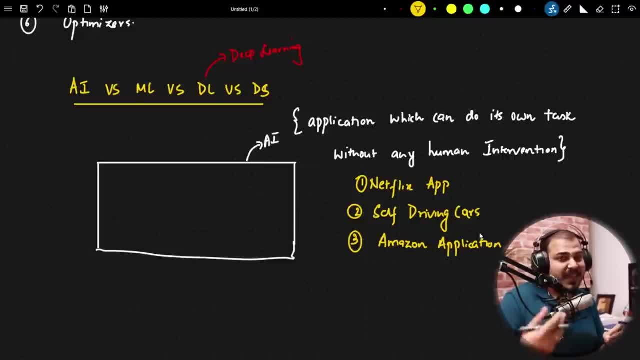 seeing movies. okay, but to make the experience better, what we do is that we include an ai module which gives you recommendation based on your behavior, right? so all these things we actually cover, uh, in this specific thing, at the end of the day, whether you are working as a computer, 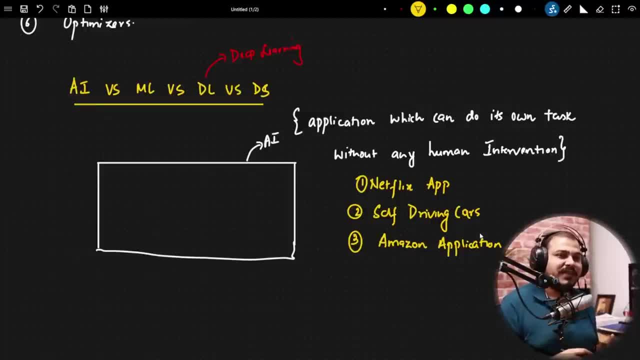 vision developer. you are working as a data scientist, you are working as a deep learning developer. at the end of the day, you know, you are actually creating an ai application. that is the most important thing to understand. okay, uh, yes, a very good example. uh, probably you have seen sofia. 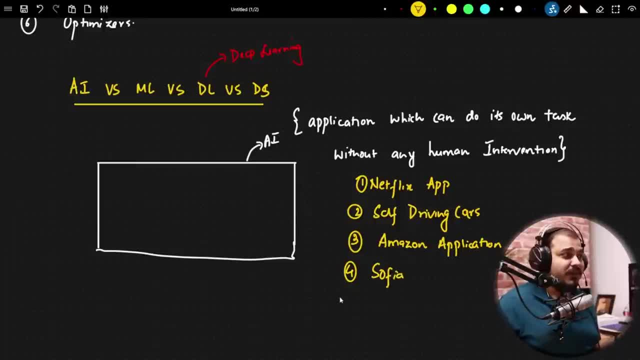 you have seen chatbots, right? uh, chatbots is one of the tasks we which we specifically do, right, so chatbot is also one of the tasks, uh, one of the ai application, in short, uh, you can basically consider, and i hope everybody knows recently, uh, elon musk, you know his bot tutor by twitter. 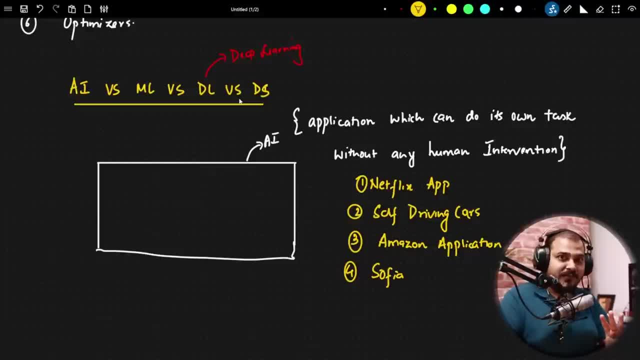 for 44.2 billion dollars and three main reasons. what he has actually given is that, uh, one of the most important reason, uh, that is definitely helpful for all the people who are learning ai, you know. so, uh, he wants to make the machine learning algorithm that is basically used to. 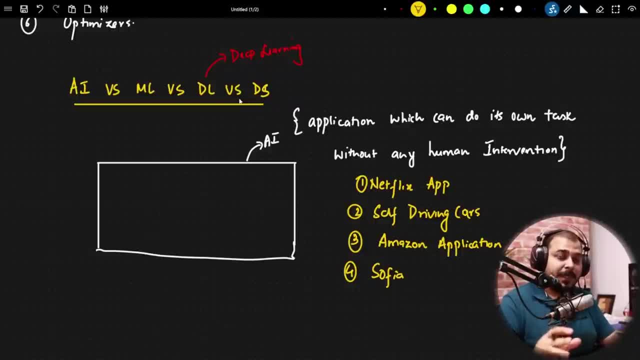 recommend the content as an open source. okay, now, if this is coming as an open source, trust me it will be quite amazing, because then you'll be able to get the idea. yes, a kind of recommendation idea we already have, but if that entire machine learning algorithm is made as an open source, you will definitely be able. 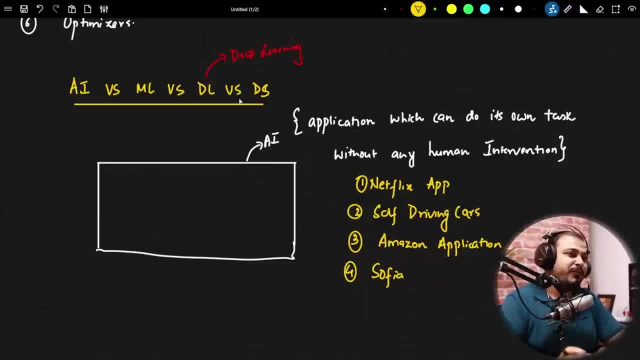 to understand. how does youtube recommendation work or instagram recommendation works and different kind of recommendation actually work? okay, so, uh, this is what actually comes in the form of ai. so here, ai is a machine learning algorithm and it's a machine learning algorithm. so it's a machine learning algorithm and it's a machine learning algorithm. so ai is nothing but. 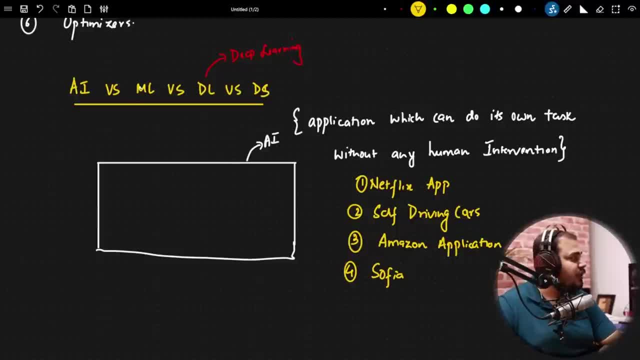 artificial intelligence. now let's go to the next one, which is called as machine learning. so machine learning is a subset of ai. so suppose, if i probably draw a kind of circle over here, and this circle is quite big, suppose let's say i am drawing a circle again. it is a little bit big, it's okay. let's say: 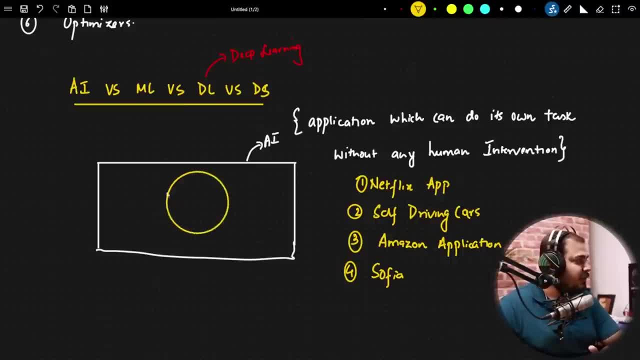 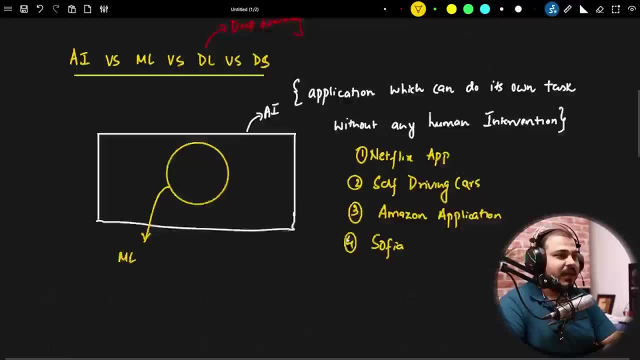 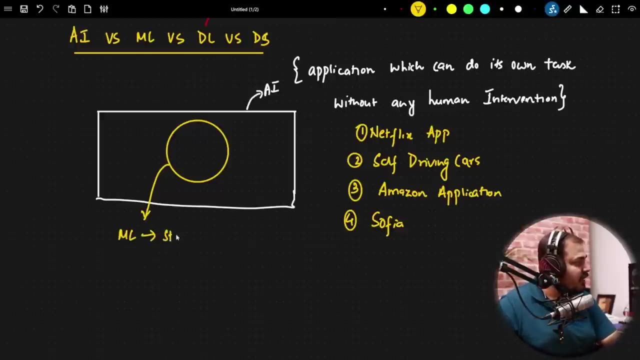 this is machine learning. okay, now, in this machine learning, what happens? is that, suppose, if i consider: this is machine learning, okay, so in machine learning, what exactly is machine learning? and uh, what do we do in machine learning? okay, so machine learning basically provides you stats tool: stats tool to analyze the data. to analyze the data, visualize the data. 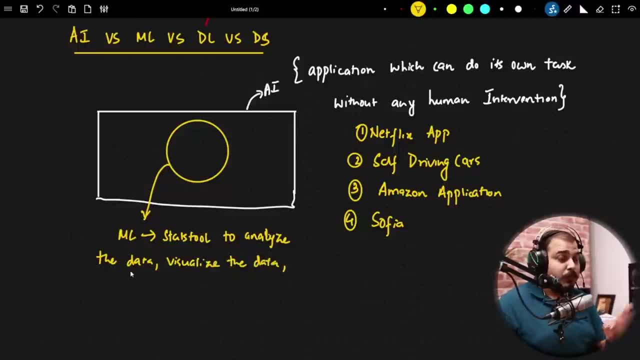 visualize the data and to do most of the machine learning tasks like predictions, predictions for for casting and many more things right, and similarly, in unsupervised, we do clustering, forecasting and many more things right. so this is what a machine learning is all about. they provide you. 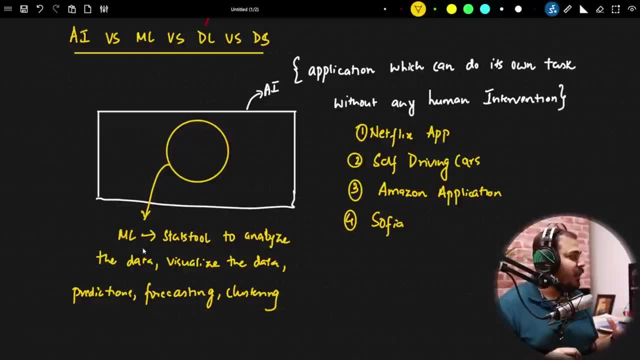 stats tool, you know, to analyze the data, visualize the data, predictions doing, forecasting and clustering. you know, yeah, power bay is also kind of tool which will actually help you to analyze the data, and all right. so internally it also uses the machine learning application, machine learning algorithms over here. 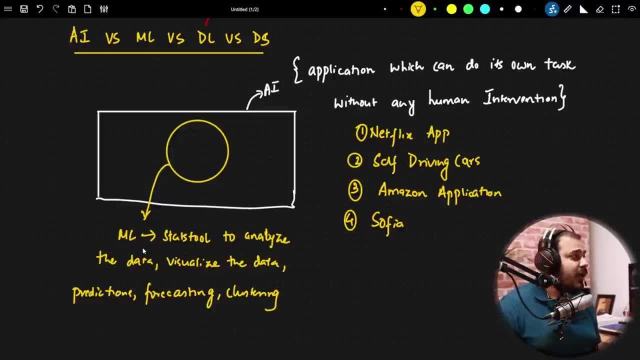 were there. it uses visualization tools integrated into it, but at the end of the day again, it is a kind of an ai application itself, right? so here i hope everybody has got an idea about what exactly machine learning is all about, you know. so it provides you stats tool if you really want to. 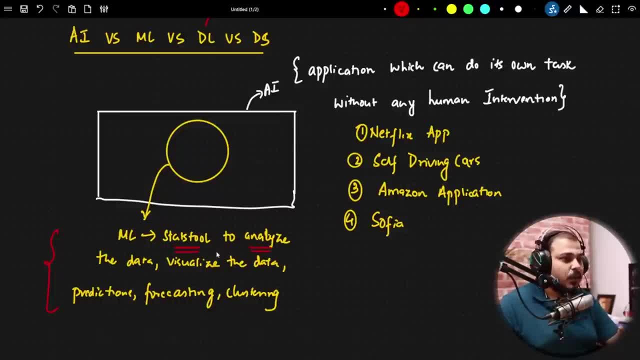 make any person understand, you have to basically say in this particular way that it provides stats tool to analyze the data, visualize the data, predictions, doing forecasting and clustering, and all right. so, anyhow, we basically say machine learning, ml is a subset of ai. okay, ml is a subset. 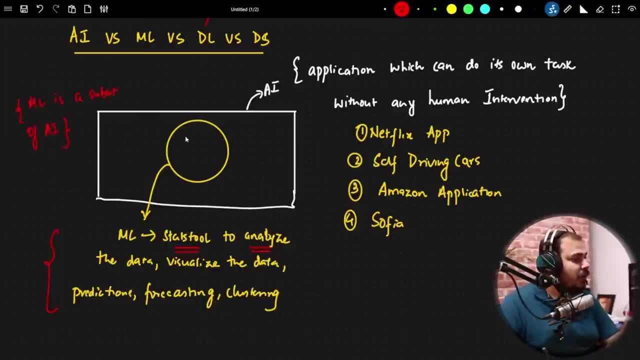 of ai perfect, so i hope everybody has understood till here. uh, i hope you're getting that better definition what you are basically learning in these things right now. coming to this now, it's not like you know machine learning. whenever we talk about you know there are different different. 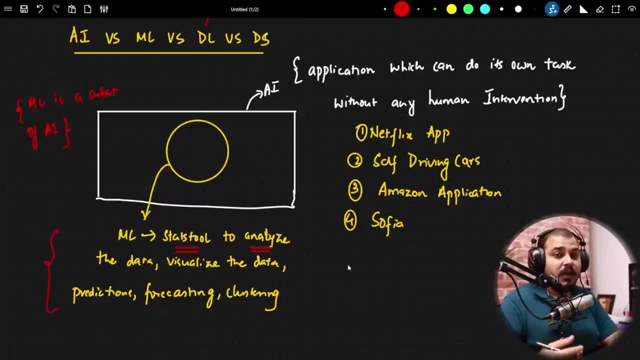 components also that comes like nlp- natural language processing. uh, you know there are different different components also that comes like nlp natural language processing. over there it will be an integrated part of it. suppose, if you use tools like a programming language, like python, we use stats, you know, to understand different different things. but here 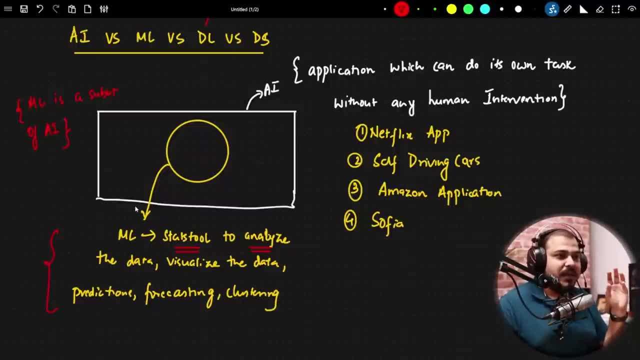 i'm trying to cover the major chunk, you know, which will basically help you to understand all these things. now, coming to the next one, which is called as deep learning. now, deep learning, super, super important, okay, and this is what our entire five session is all about, you know. so, another subset. 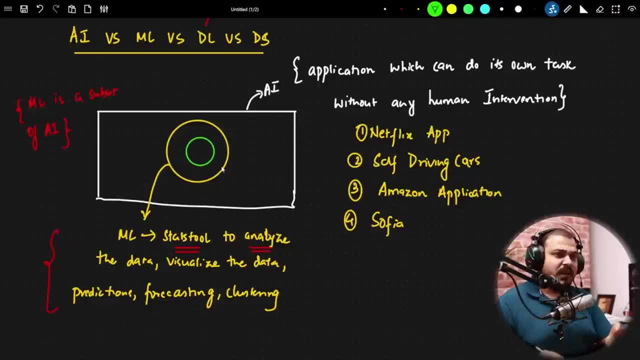 of machine learning. we basically say it as deep learning. okay, deep learning is not becoming is is, it's not learning, it's not learning, it's not learning in the way it's being learned. so i don't, It's not like recently, only did not come up. you know deep learning. 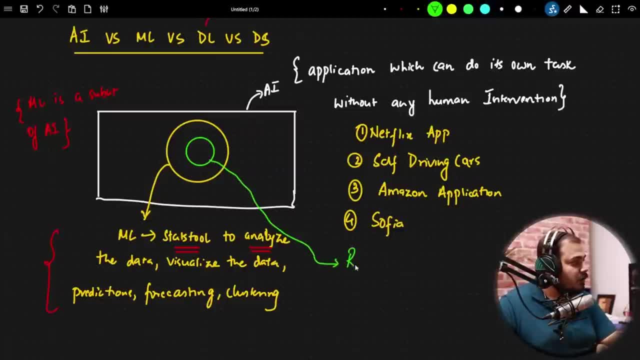 The researcher were- if I probably write it over here, the researchers were working from 1958.. Researchers were basically working from 1958. But right now it became really, really, really amazing because of the amount of data that is getting created and because of amazing GPU hardwares that we have. 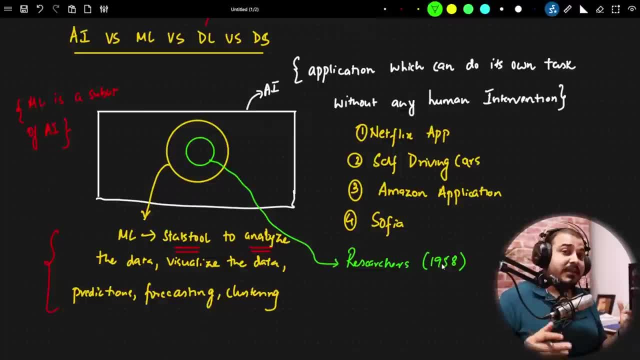 Thanks to NVIDIA because of the entire research that you are they are actually doing. you know, right now I'm also having RTX 3090 and probably, if you work with this GPU, trust me how amazing models you will be able to train right. 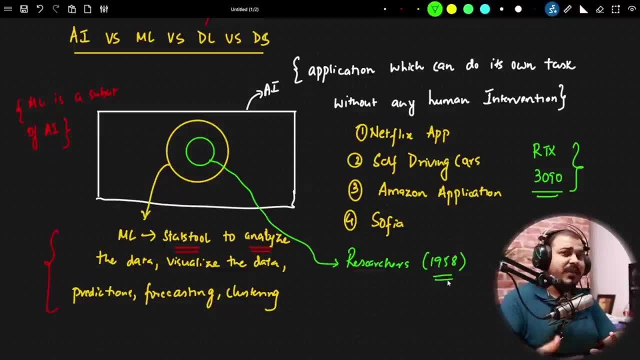 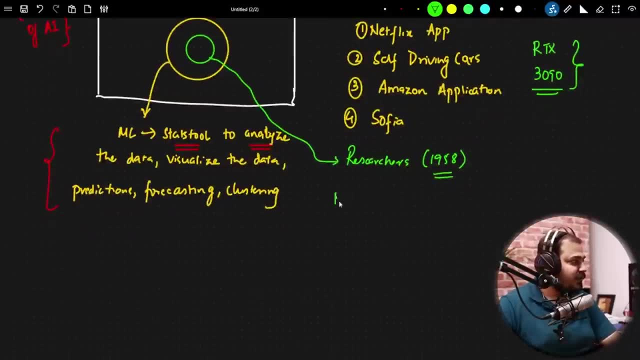 So, researchers, you know they started working in 1958 and first probably, if I talk about any kind of neural network right, They specifically was focusing on working on multi-layered neural network right, Multi-layered neural network And first neural network. 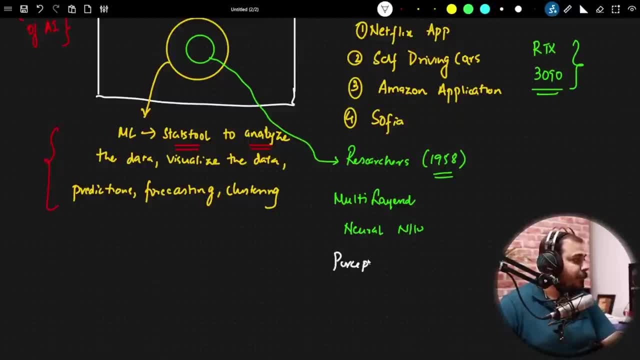 If I probably talk about is something called as perceptron. right, And today we will be discussing about perceptron in depth. We'll try to understand what exactly is perceptron, and all right, But the main aim of deep learning- main aim of deep learning, suppose, if I consider this. 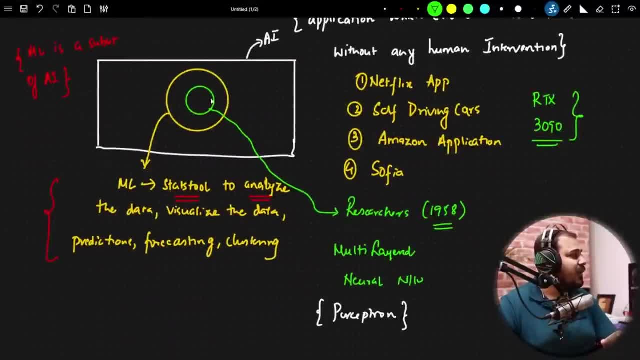 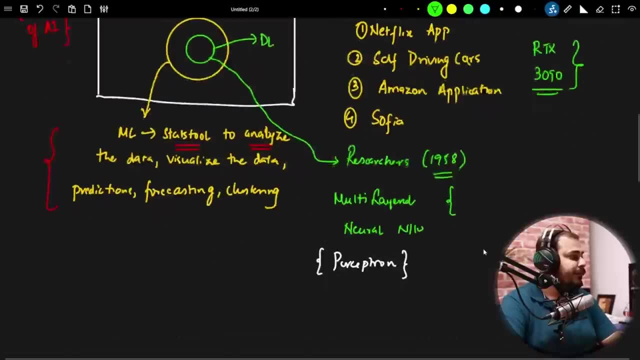 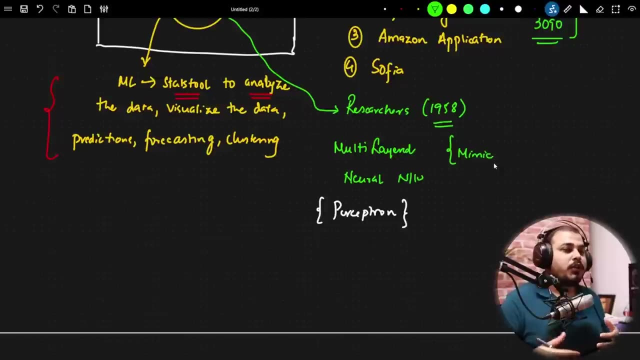 as deep learning. the main aim of deep learning is basically to mimic mimic human brain, okay. So this main aim is basically to basically to mimic. Mimic basically means like How we human being learn things right. We also want to make sure that the machine also learns in that particular way. 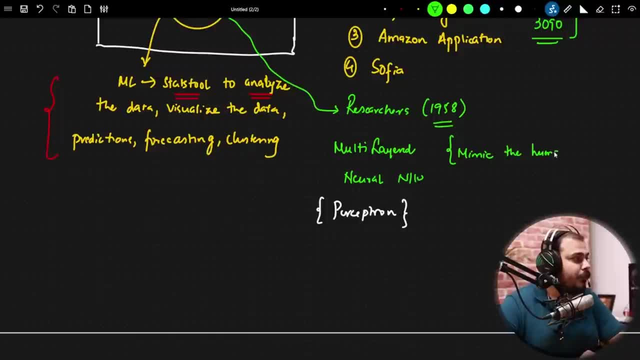 So here you can basically say: mimic the human brain, right? So mimicking the human brain is the most important thing in this specific thing, right? So here you're specifically mimicking the human brain and we are making sure that the machine learning algorithms also learn in that particular way, or any machine also learns in that specific 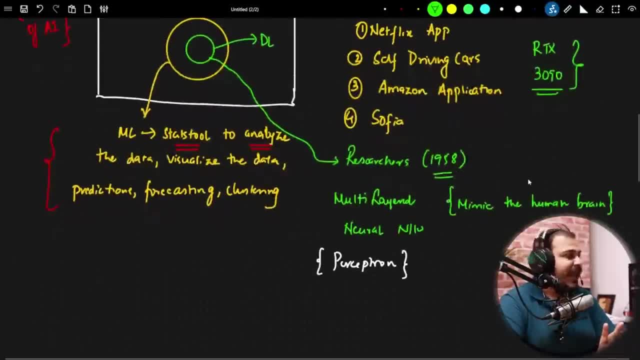 way right. So this is an idea about deep learning, And our entire focus will be on deep learning for this entire five days, where we'll be learning multiple things and all right. So what are things we will be specifically learning in deep learning? 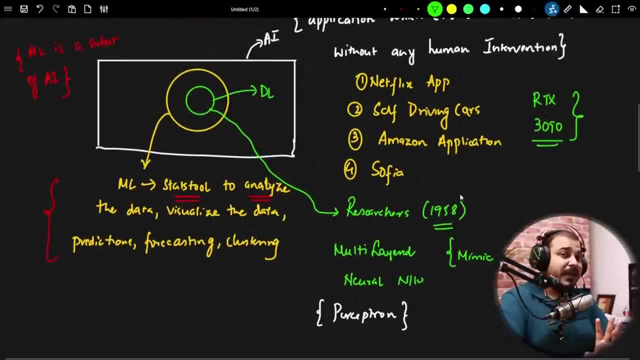 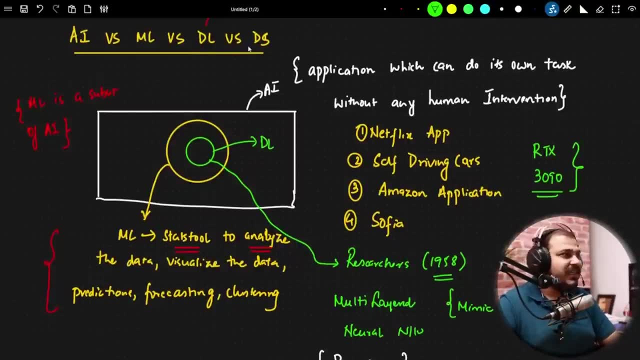 I'll just tell you in another five minutes, and by that you'll be able to get an entire idea about it. Now one very important thing: where does data science fall into this right? Where does DS, that is, data science- fall? 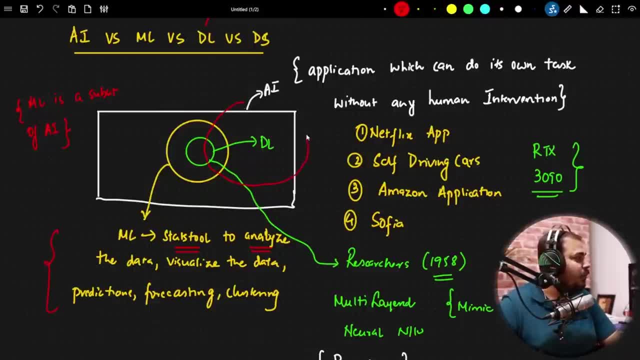 Suppose, if I say, data science can be the part of everything you know, so it can be the part of everything over here. right It, it can. It can basically like: if you are a data scientist, you probably have to work on machine. 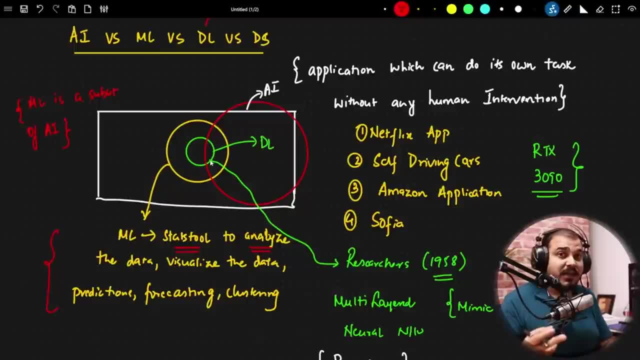 learning algorithms. You have to work. probably you may get a work to work as a data analyst, right, You may also work as a deep learning developer, But at the end of the day, the goal is to create an AI application. okay, 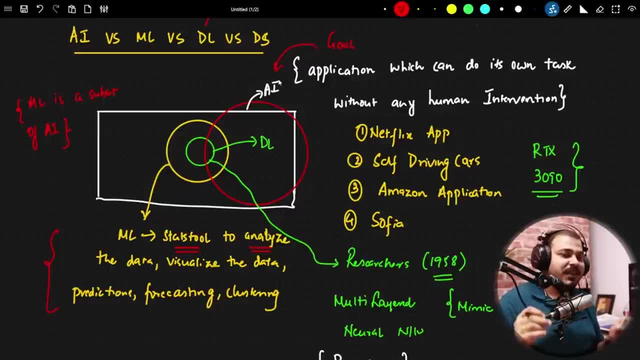 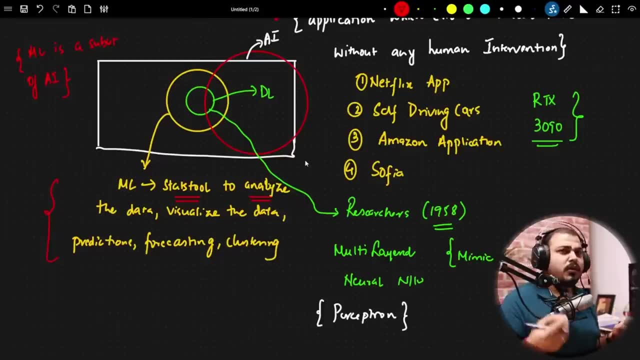 The goal, the last goal, the final goal is basically to create an AI application. So this was the first section. Quickly I wanted to cover it. So one very important Question that we usually get: where does computer vision come into existence? 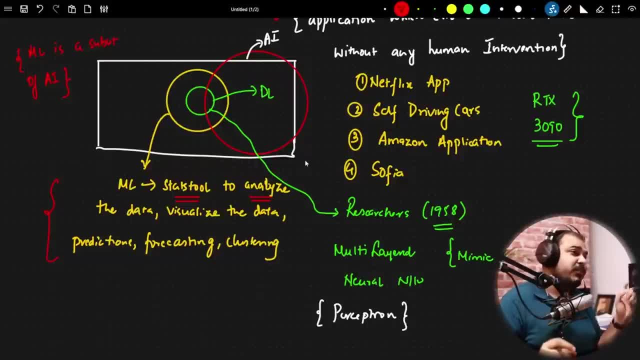 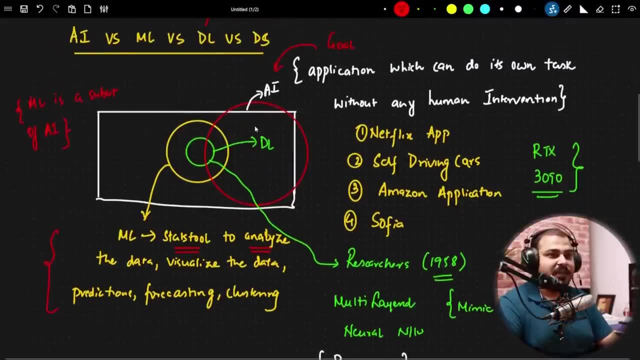 It can be a part of deep learning also. We can also use computer vision in machine learning also, and we can use all these things. But at the end of the day, we are basically creating an AI application. But here I really want to talk about the major chunk that we are basically discussing. that is popular. 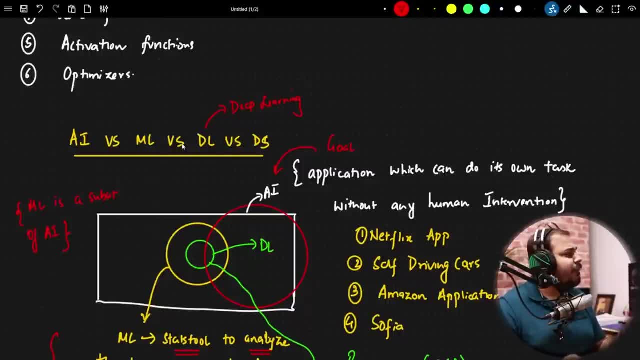 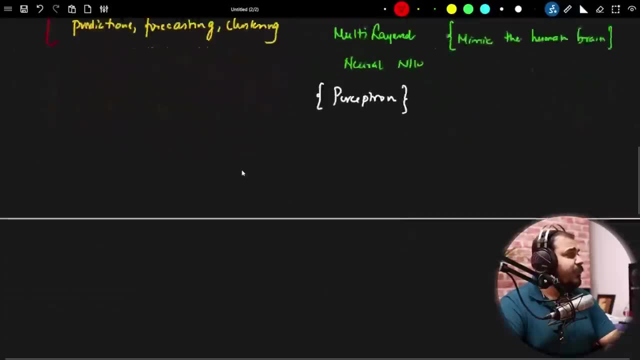 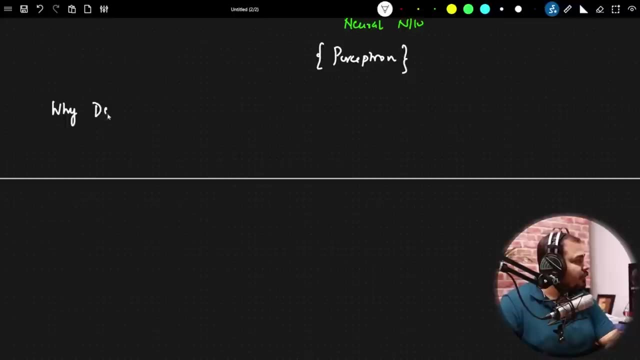 throughout the entire world. Whenever we people talk about AI, ML, DL or data science, we basically focus onto this right Now, perfect, Everybody's able to understand. Now we will ask a very common question. Okay, The common question will be that why deep learning is becoming so popular. 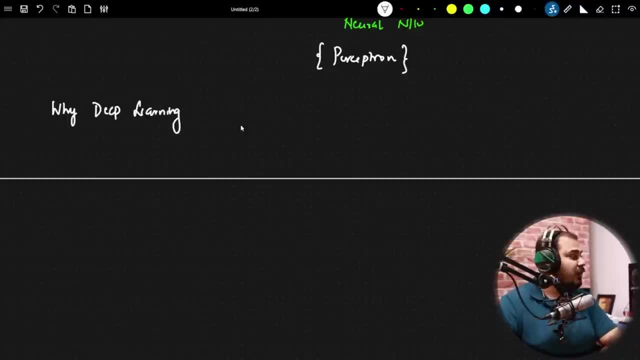 It is becoming so popular. It is even becoming popular more than machine learning. Why deep learning is becoming popular? Right, Why deep learning is becoming popular? Now, this is the question that we will try to answer: Why deep learning is becoming popular. 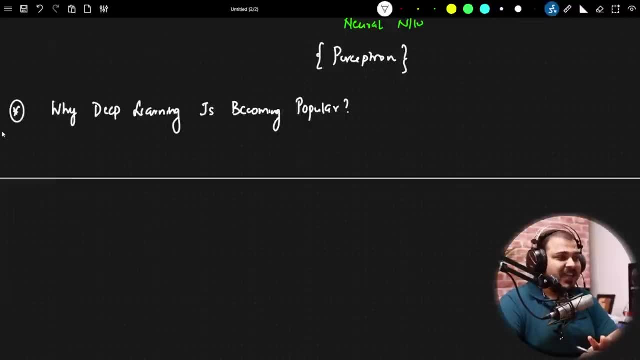 And, uh, you know, I hope everybody has basically, uh, already told some of the points and we had already discussed before. So the one major point, why deep learning is basically becoming popular. So here I'm just saying why, right? 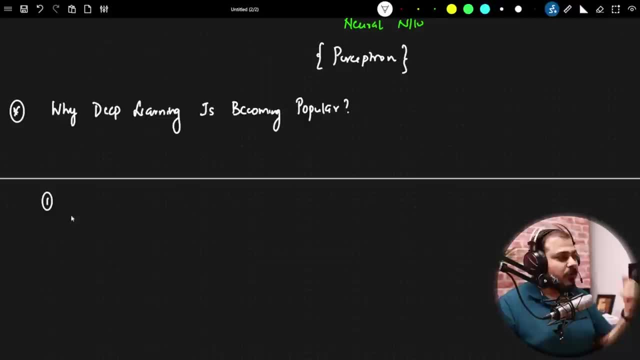 The first point, obviously right, Let's let's go back to 2005,. right, 2005,, which was the amazing social media network that actually came up before 2005.. Only Orkut was there in the market, right. 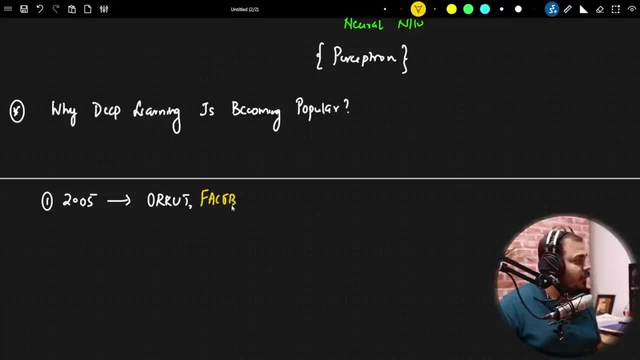 Then, later on, what happened? Facebook came. right now, Facebook is entirely based on web 2.0, what is web 2.0?? It is a kind of entire. the web application is developed in such a way that you'll be able to log in. 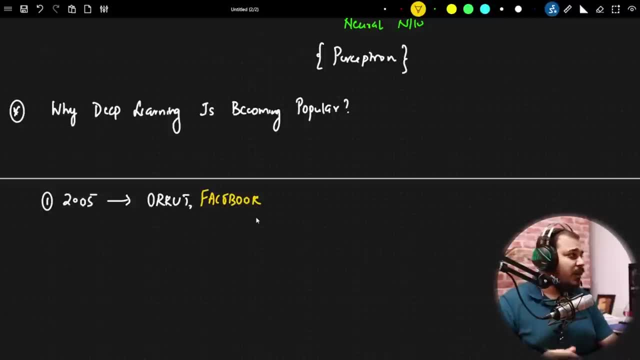 You'll be able to store your data. You'll be able to interact with other people. So this Facebook was a social media networking website, right? You could put images and all later on Instagram phase. uh, WhatsApp, LinkedIn, Twitter, right. 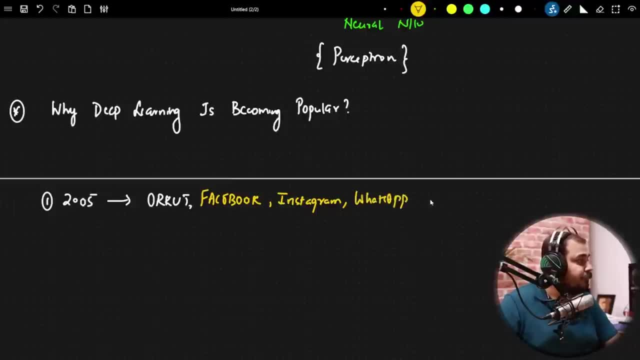 Instagram, uh, WhatsApp, right, Uh, LinkedIn, Twitter, right. This- all This, all Websites, it is all web application- had actually come right now. in this all web application, what was the main thing like? here you are interacting with people, you're posting something. because of this, the data started to get generated exponentially right. 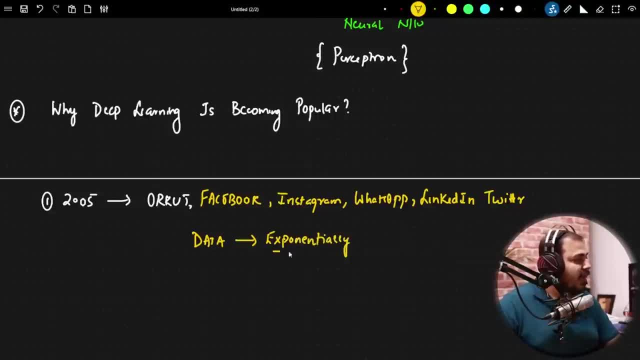 Exponentially huge amount of data was actually getting generated right. Exponentially, It was increasing. The size of the data was definitely increasing right. So at that point of time, when I talk about 2008, you know, 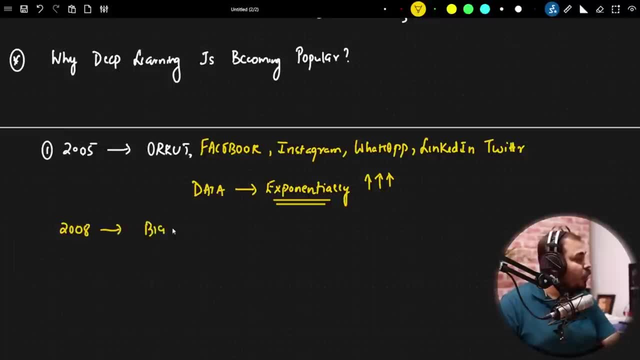 The concept of big data. you know, big data was wasn't very high in demand, you know, because they wanted to store that data efficiently. They wanted to store this data efficiently. So that is the reason why big data team basically- uh, big data engineering skill became very famous at that point of time. 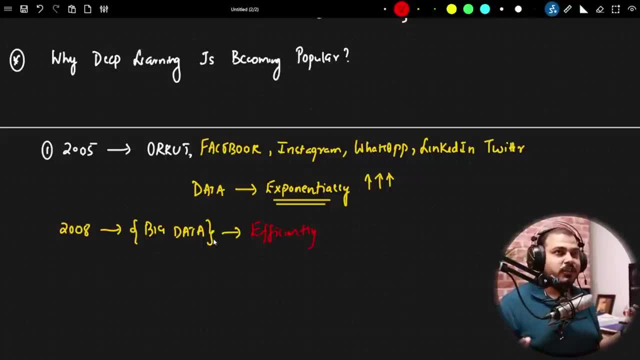 You know people were looking for, like when I was doing my engineering. you know, somewhere in 2010 and 11, there was huge opening of big data, and big data are the people which are who are actually storing this. Yeah, 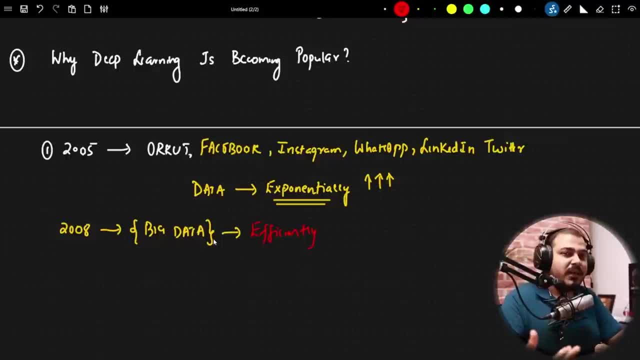 Yeah, Yeah, information efficiently, so that we can actually read that particular data and use it wherever we require, Right? So, uh, that is why big data becomes very, really, really, really popular. Now, as we went with time, you know, in, probably in 2013,, let's say, 2013,- 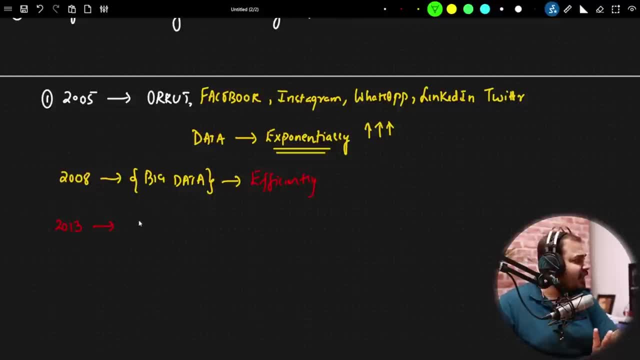 as we went in time, now what things were happening. Company had huge amount of data, right. So company had. company had huge, huge amount of data, right, Huge amount of data. Now, if company has huge amount of data, 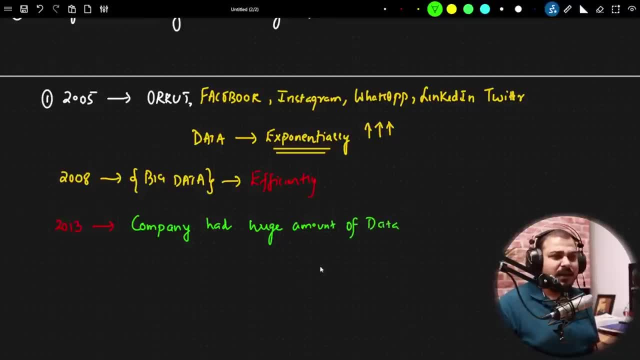 will they just store and keep it? Will they just store and keep it Right? The answer is no. right The answer is no. They really want to use this data and basically bring a seamless experience into the products. right, They want to bring a seamless experience. 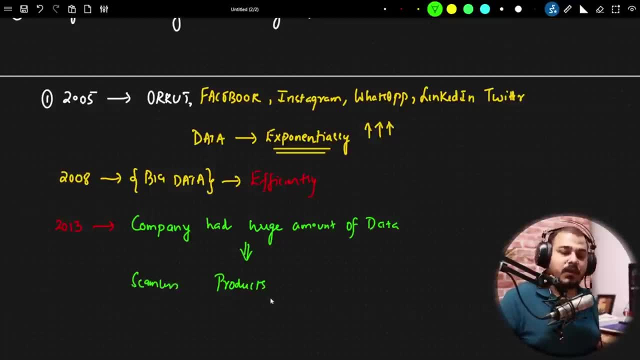 They want to make the product better and how that is basically possible. That is only possible when you utilize the data that is already available. So, because of that, what happened? Since we had a huge data data science, AI, I'll just write AI. 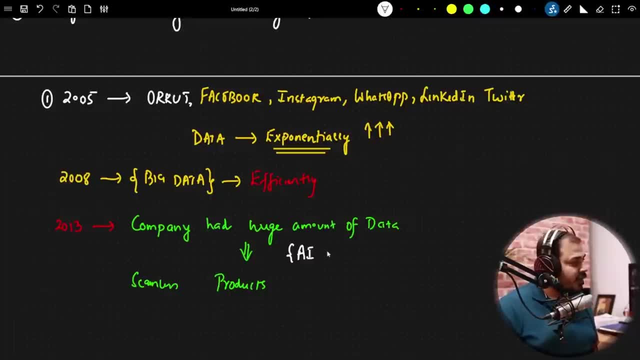 AI started becoming very, very popular. AI became popular. Do you know when did I start learning AI? It was in the year 2013 to 14, right. So at this point of time I made a successful career transition And at that point of time only, I started learning. 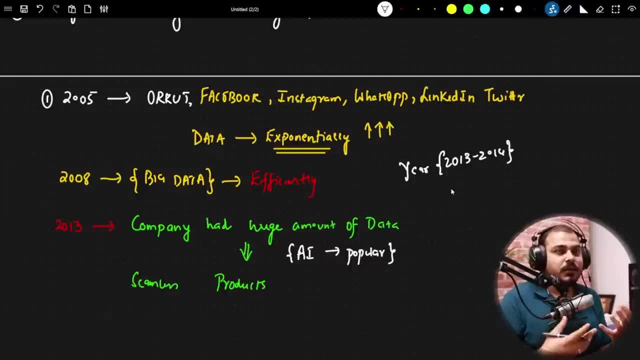 And I knew that In the future this really has a good, um you know, scope. in short, because data is getting generated from everywhere. Companies have peta, peta bites of data and every day it is going to increase And probably in the future it is going to increase again exponentially. 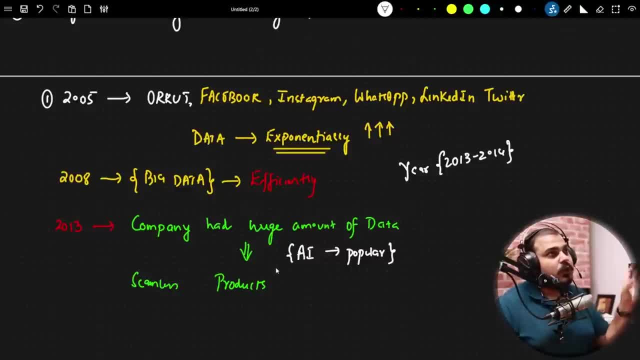 So definitely, you know, uh, in order to for the company to make the products better, they really want to utilize this specific data and make the product still much more better itself And best example- you can basically talk about Netflix, right. 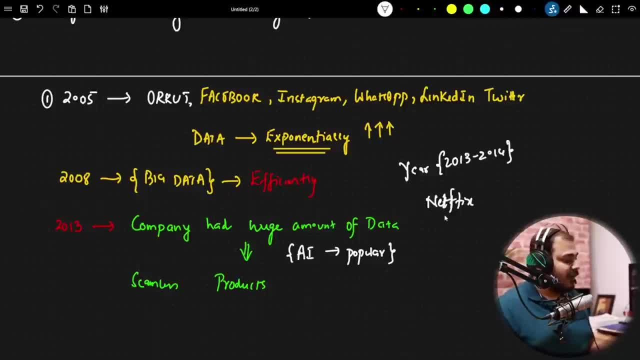 Netflix is using, uh, whatever data we have, basically, uh, using the app right While seeing movies, our profile information and all, and based on that, they are recommending things right. So that is why that is so important, right With respect to the data, right. 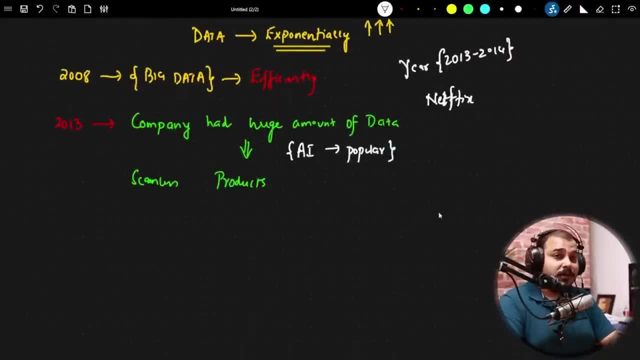 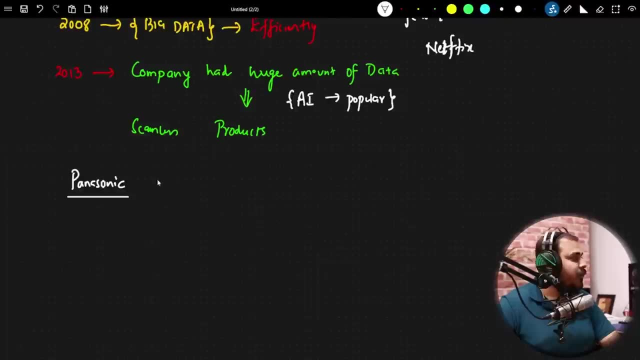 So data really has a amazing importance. altogether, Let's talk about my one of my company experience. that is, Panasonic. So what is Panasonic famous for? Panasonic has lot, of lot of products, right? And what are this kind of products? Let's say ACs, right? Uh, TVs, refrigerators. 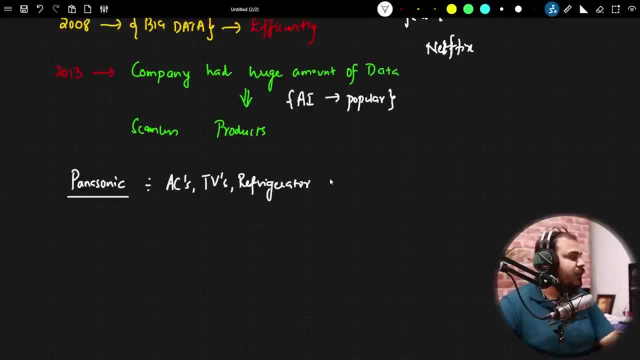 right And initially also this: all products right. They were definitely generating data. They were definitely generating data And when I joined Panasonic somewhere around two, three years back, you know, I got a chance to make this products quite smarter right. 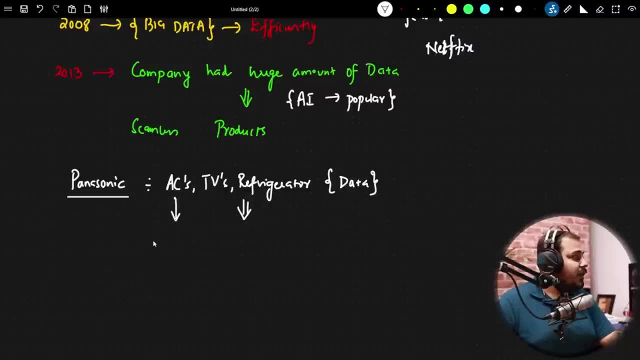 Suppose I was specifically working with ACS. What did I do? I? I I created a model, you know. I created a model which can reduce the electricity bill, which can reduce the electricity bill right, Because people, you know. 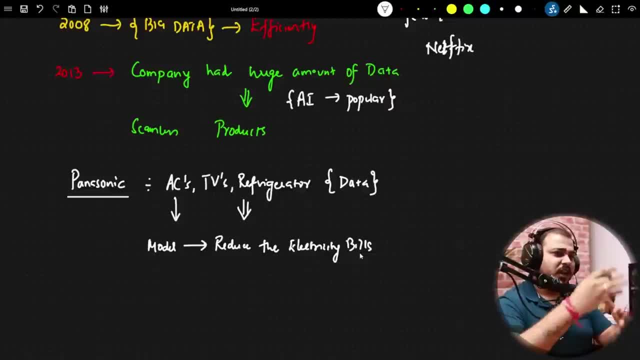 how they use the AC. they bump up some time in the higher temperature, They they come down directly to some lower temperature, and all based on the outside temperature. What if I showed them a model that, okay, use this kind of profile and based on the outside temperature? 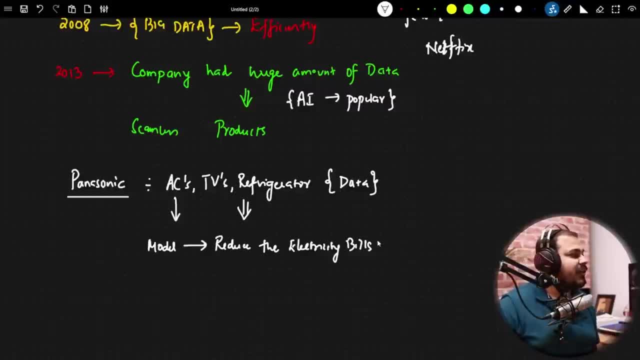 you will be able to efficiently handle the ACS and probably your electricity bill may get reduced right. So this is one example. Now, because of this, what happens is that they actually provide some seamless experience to the client, And definitely when you come up with this kind of model. 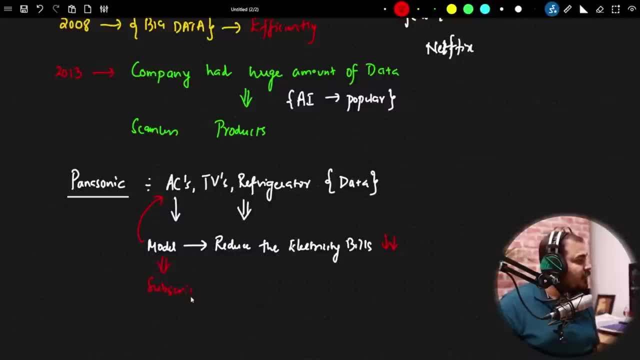 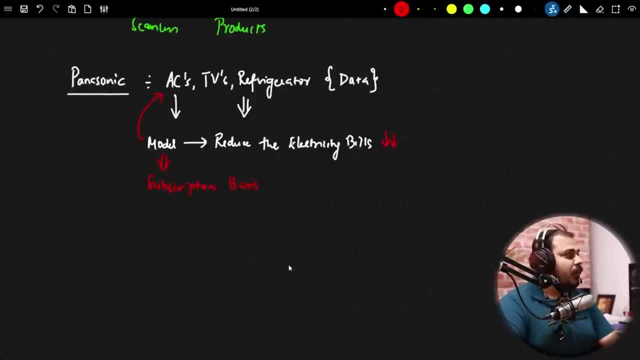 this can also be sold in subscription basis- right Subscription basis. So through this, at the end of the day, since they are bringing seamless experience in the product, so what will happen is that the company will generate revenues. They will generate revenues, They will be able to make better decisions. 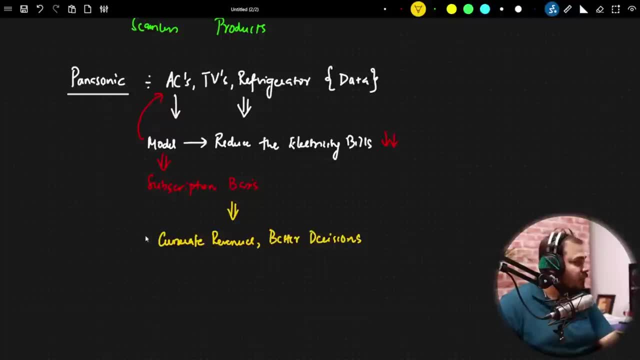 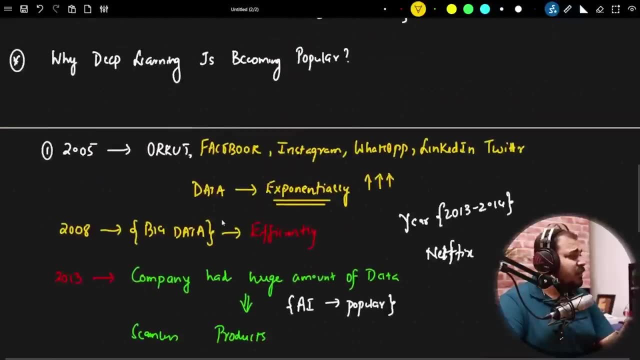 Right, They will be able to make better decisions. Perfect, So I hope you are able to understand the importance of the data, And this is, with respect to the first point, right. All these things that I explained why deep learning is becoming popular, because 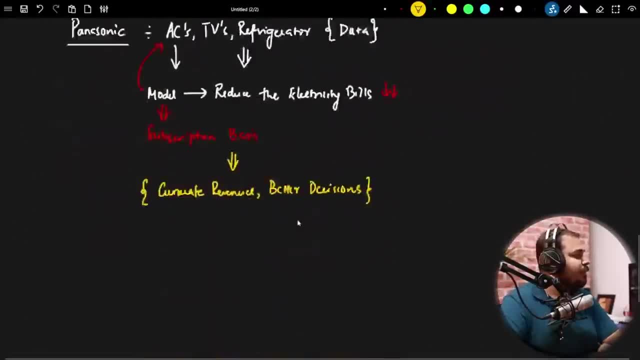 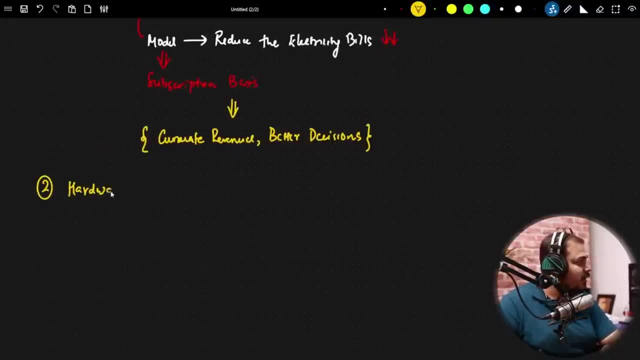 now you have a huge amount of data. Now let's go to the second point, right? Second point which is super, again very important, right, And that is hardware advancement, right, Hardware advancement. I hope everybody knows about NVIDIA, right? 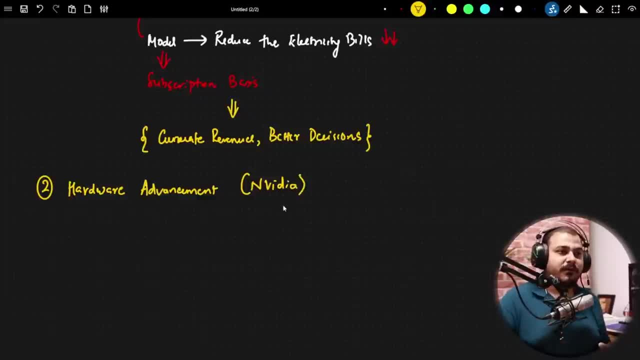 I hope everybody knows about NVIDIA. What is so special about NVIDIA? They come up with this amazing GPUs, right. What is GPUs? Graphic processing units- Right. And you know that in deep learning, whenever you create a multilayer neural network, 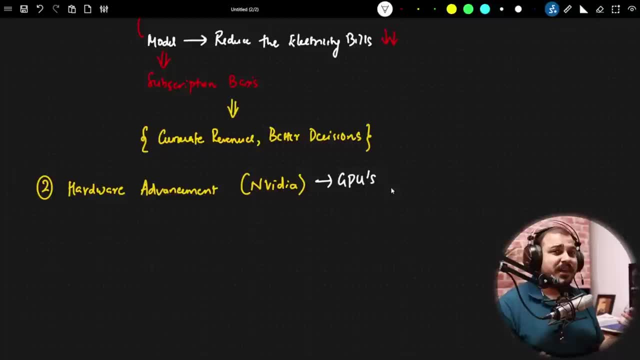 many parameters are actually created right, And when many parameters are actually created, you have to probably do the training in the power in, in in epochs right, Multiple epochs Right, And when you create multiple epochs, and probably for that a lot of times will be basically taking place right. so 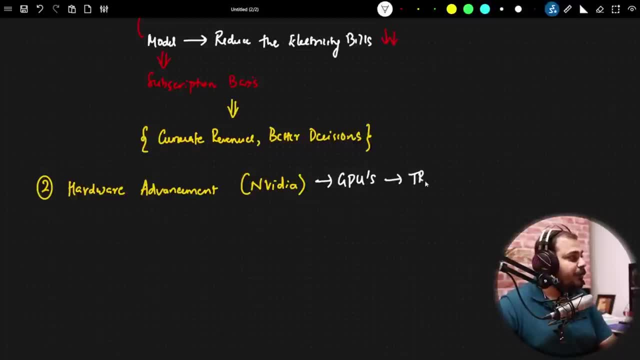 GPUs actually helps you to train your model very faster and right now the GPUs are training the models and specifically right training the models. it will be very, very handy. you know now recently like if I talk about GPUs, this GPUs cost is really reducing day by day, and that is all because of the technological 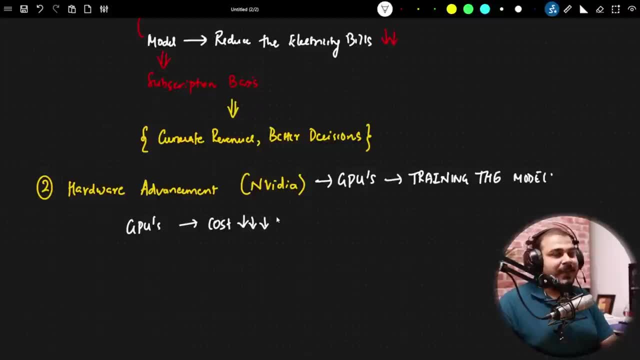 advancement. you know the before GPUs like, let's say, let's say, let's say an example of RTX Titan. okay, so this was one GPU which I had on the first instance and Nvidia had actually gifted me this, but today I am actually using RTX 3090, which is more efficient than Titan, RTX, right? so all this GPUs, people. 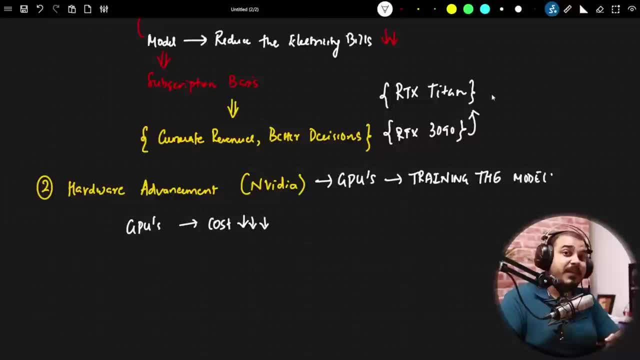 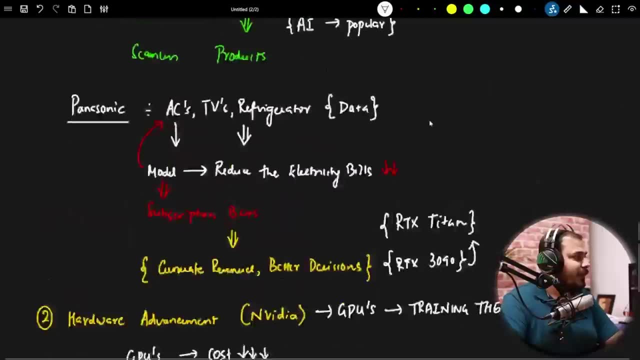 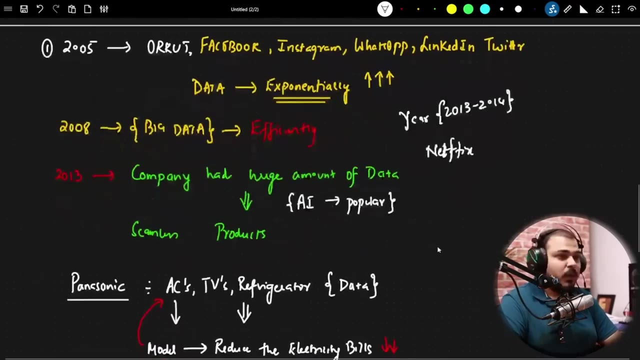 are actually using. Nvidia is doing more, better jobs. they're coming up with their own library so that we can basically train our deep learning models in an efficient way. right, so I hope the another interview question: everybody is clear about why deep learning is becoming very popular, right? okay, now let's talk about the next. 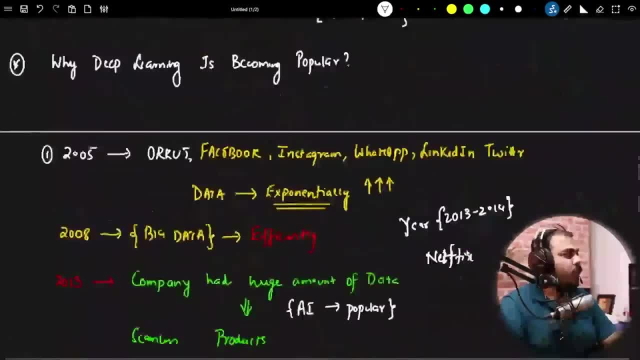 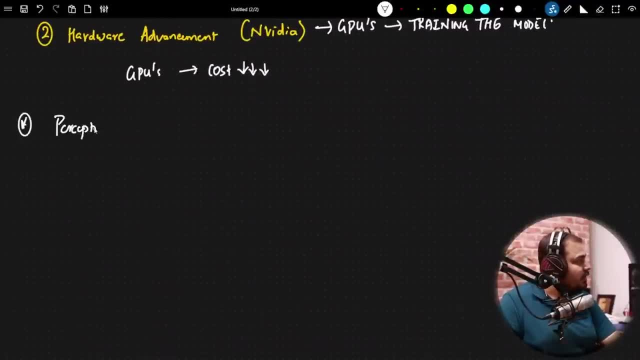 thing. let's talk about the first thing, which is called as perceptron now. now let's go to the next point, which is called as perceptron, and this is where I will first of all discuss about single layer, multi-layered neuron, single layer neural network and 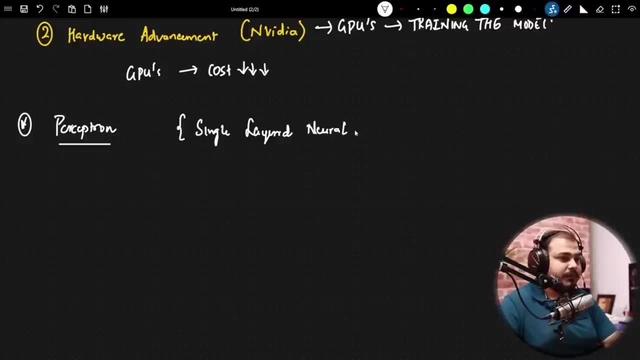 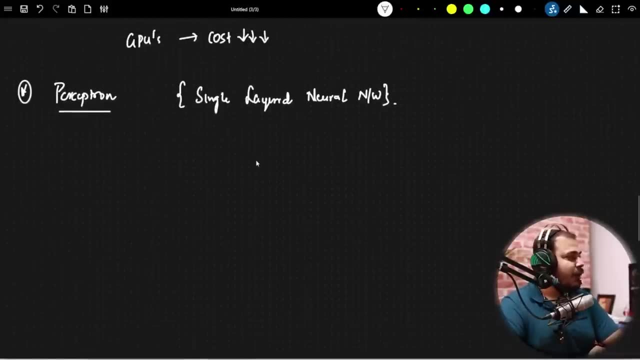 we will probably discuss about multi-layered neural network right now, single layer neural network. now, what happens basically in the single layer neural network? I'll just take an example of perceptron. okay, very simple. now if I consider: okay, what is the basic structure of this multi-layered or? 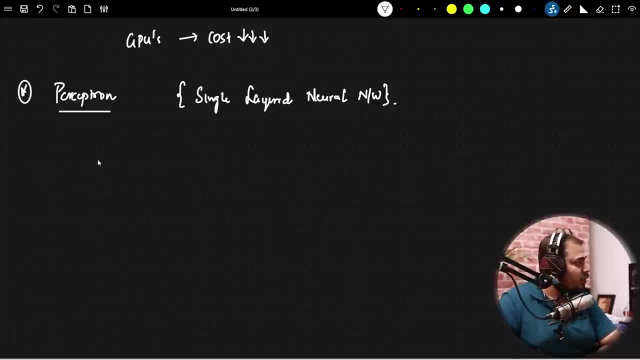 single layer neural network or this perceptron. let's say, now suppose I will be drawing some circles. the circles are not some food item, okay, so I'm just trying to draw the circles. let's say, I'll draw one more circle over here and I'll draw one more circle over here. okay, now this yeah. 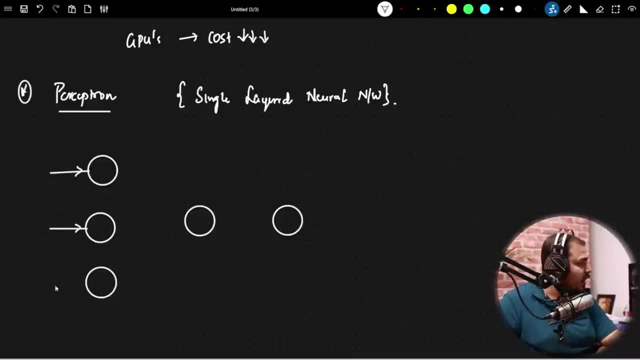 I'll also be covering NLP, so don't worry. so this are my input. okay. so this, we basically say it has input layers. okay, this, since I'm creating a single layer neural network. so this becomes my hidden layer one. so this becomes my hidden layer one, okay. and finally, this becomes my output. 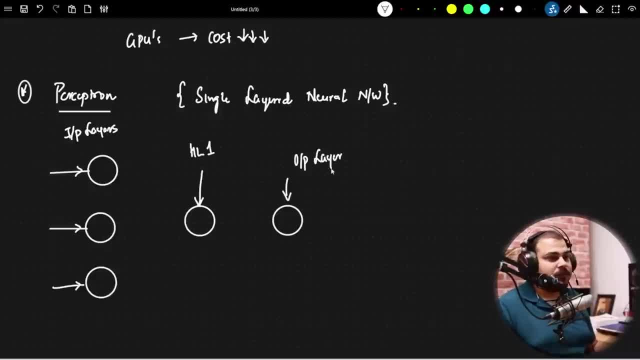 layer. okay, this becomes my output layer. now, always remember, and let's, let's do one thing: let's connect this every dots. okay, let's connect this debris dots, and I will try to show you with respect to a good example, with respect to our brain, okay, so, finally, I get my output over here. 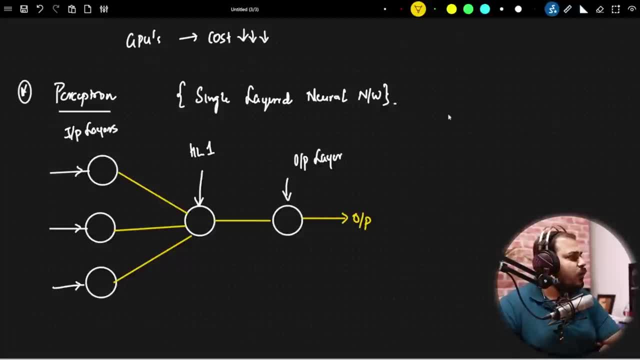 okay, now let's let's take one very good example. okay, let's say I have a data set which shows whether the student has passed or not. okay, suppose the student studies for play and this will basically be my pass- sleep and this will be my play. sorry, pass or fail, pass or fail. 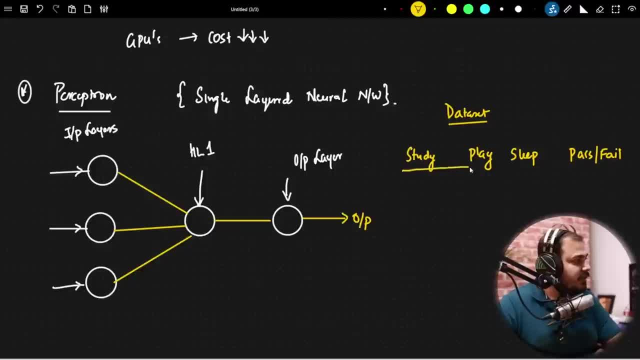 okay, let's say that I have this specific data set. okay, let's say, in one of the student has a record which is called as he basically studies for seven hours, he plays for three hours, he sleeps for seven hours, so probably, if he's studying for this many hours, I can say that the person will pass. and since this is a 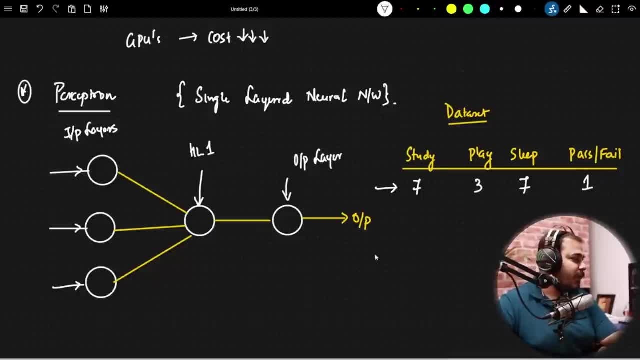 binary classification, I am just going to make it as one. okay, then let's say: second record is that if the student study for two hours, he plays for five hours, he sleep for eight hours, most of the chance is that the student will fail. okay, the third record, if I consider: 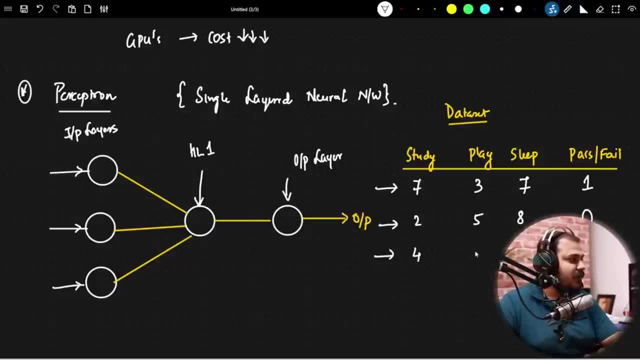 suppose let's say, the student studies for four hours, he plays for three hours, he sleeps for seven hours. I'm going to make it as pass. okay, let's say like this: I have so many records available with me. okay, now with respect to this neural network, how will I basically use this beta data set to train this binary? 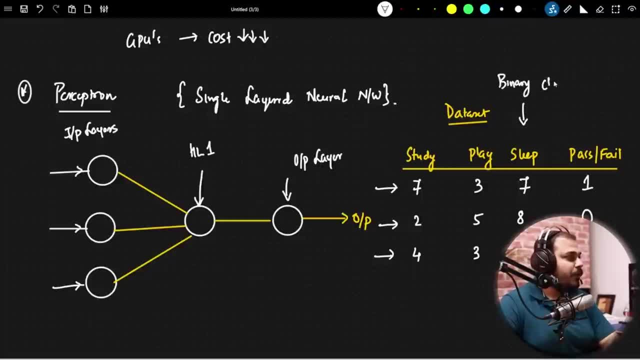 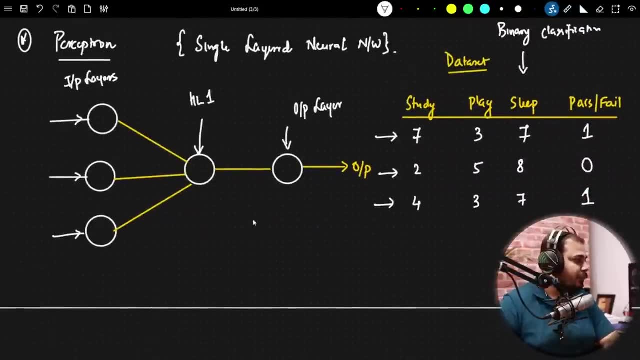 classification. okay now let's say, I have this data set and I'm going to train this binary classification because this is a binary classification problem. okay, binary classification, let's see this. okay. so I hope everybody is able to see this binary classification problem now. always understand: this is my input layer. okay, now, in this input layer. 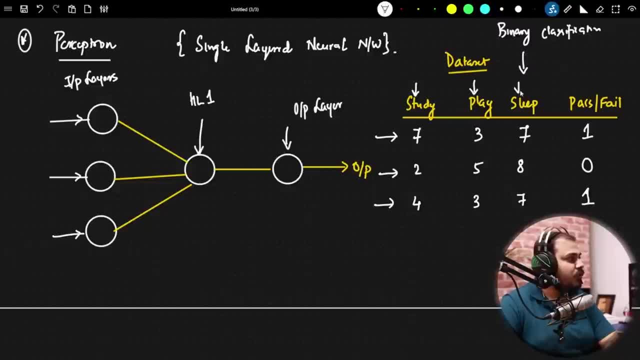 this inputs will get passed. okay, this inputs record by record, it will get passed. so the first input is nothing but study: okay, I can basically say: it has X one. then the second input is basically play. I can basically say X 2. and this third input is nothing but sleep. I can. 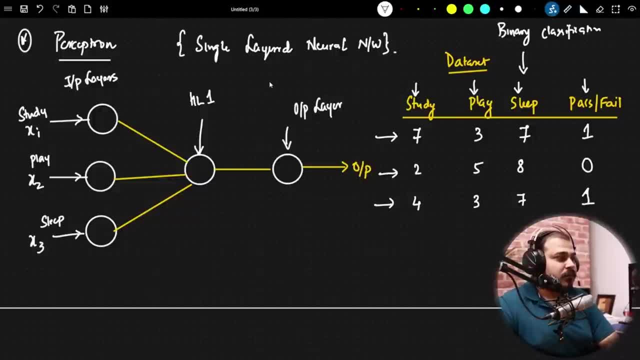 basically say X 3. okay, here you can basically see that. okay, fine, X 1, X 2, X 3 is my inputs. okay, inputs, I will be passing this records. okay, I will be passing this records. okay, so here what I'm doing: every record will get passed. 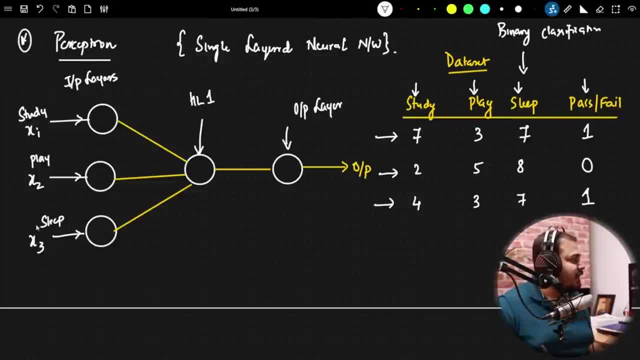 at one time- suppose in the first instance I pass 7, 3, 7, right, because that is what is my first record- basically say, okay, now, let's say I have my eyes right and my brain is there. now what is this input? now I am able to see this monitor, I am able to see the camera right, so this 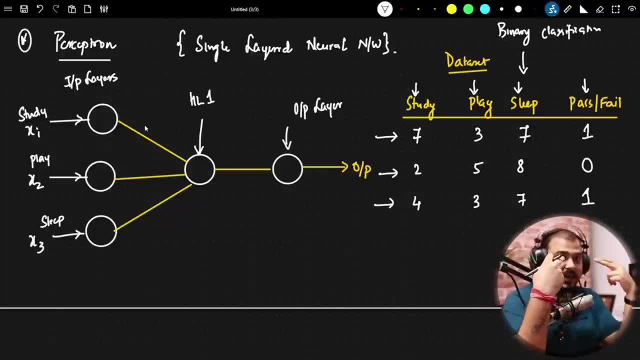 signal that is basically passing, that is an input. right now, when I see this, right, when I'm, when I'm seeing this, I am able to determine: okay, this is a camera and I'm seeing to the camera. right, I'm seeing definitely to the camera and seeing you all right, so just say hi to me. right, I'm seeing to you, I'm seeing. 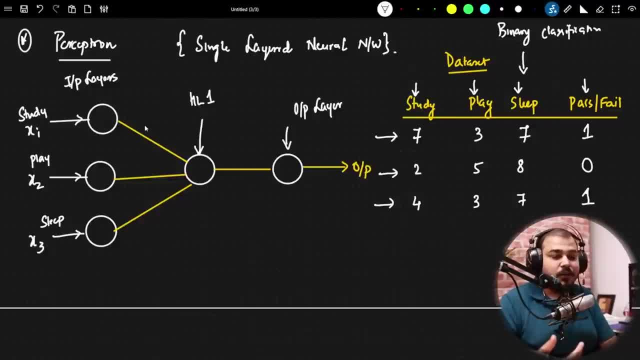 you all through this virtual weeks world, right, and definitely many people are able also to see me. if i close this camera, then obviously i'll not. you'll not be able to see me or i'll not be able to see you, but when i see this, 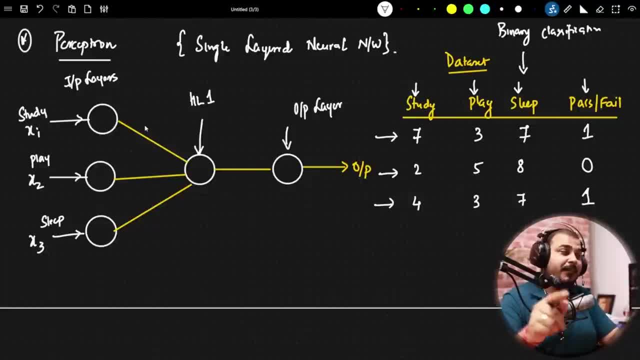 camera i'm able to determine: okay, this is the camera. and for seeing to the camera, i have to see over here how this is happening. this input is passing through my eyes, this neural network, the signal goes to the neural network and this is my hidden layer. this is my hidden layer: neurons. 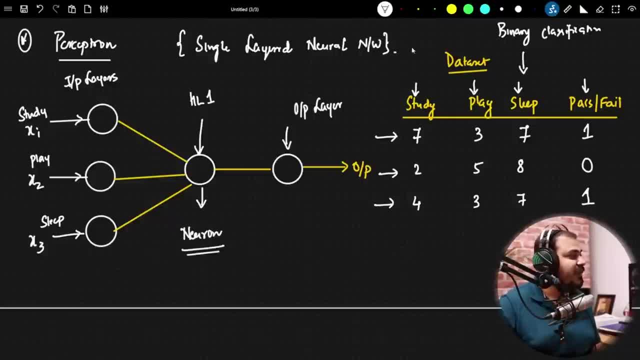 so here i specifically talk about neurons. so this: we basically say that, okay, this hidden layer has one neuron. and what is this neuron? neuron, biological neuron, everybody is familiar with that. right, neuron does some kind of signal processing. right, it does some kind of signal processing. now, since i'm seeing this camera obviously through the input layer, so my eyes- 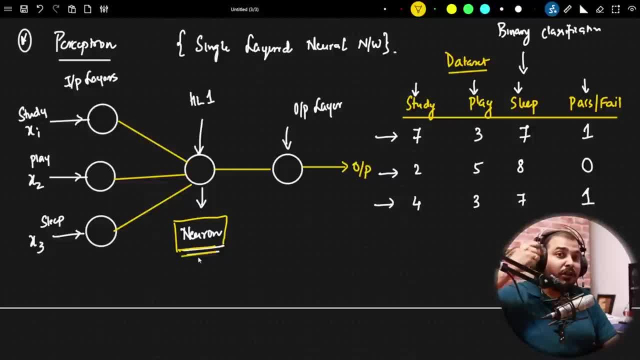 becomes my input layer when it goes to the next neurons. those neurons pre-process that data. and then, finally, it comes to my output layer and then it goes to the next neurons. those neurons pre-process that data layer. output layer is nothing, but it is my brain somewhere in the back-end side. 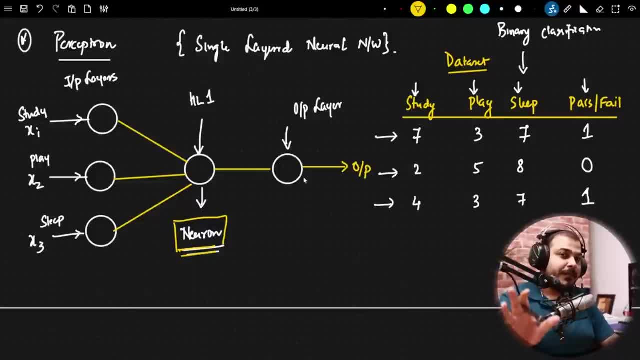 which is responsible for seeing or visualizing the camera. right? so this, let's consider, this- is my another neuron, this is my output neuron, which will basically be able to predict what this is, whether it is a camera, whether it is a television, whether it is a mobile phone or whatever. it is right. so this is. 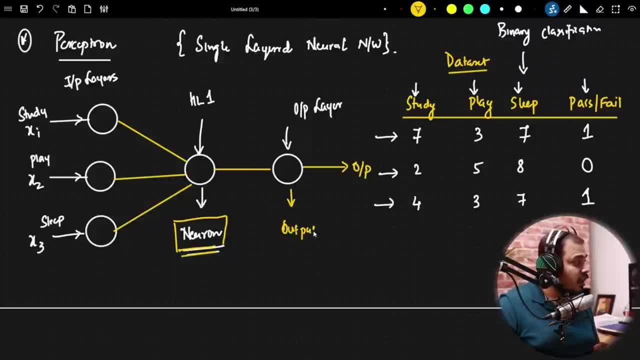 what is the importance of this? so this specifically is called as output neuron. okay, and this is responsible for planning your final output, how it looks like. but let's consider a baby. when a baby is born, right? if he sees the camera for the first time, will he be able to predict that this is a camera? the answer: 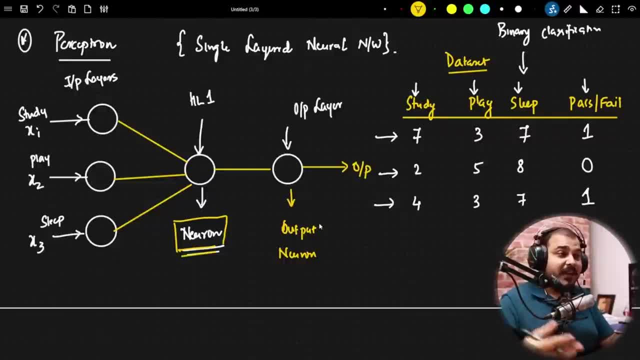 is no right. obviously he needs to train, right, we need to tell him that, okay, this is a camera, this is food, this is your bed, this is this, this is milk, like that. right, we have to tell him. we have to continuously train him. then, after a couple of months, right? 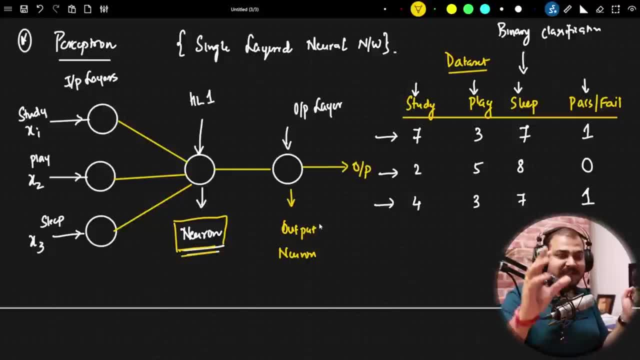 after a couple of months he'll be able to understand. as soon as he sees a bottle of milk, he will start crying right. that usually happens with my son, so I, my son is somewhere on seven months now. he understands what is a mobile phone. he understands well how does this milk look like, you know, in a bottle. so all those 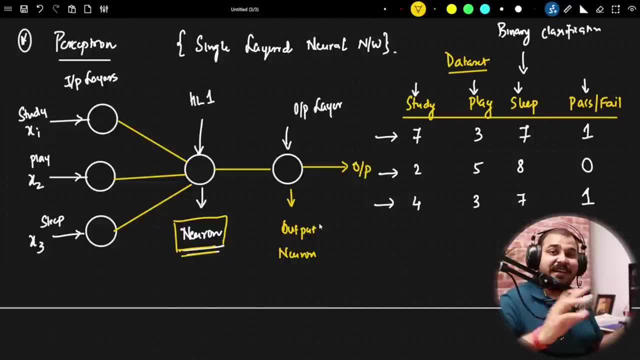 things is basically be able to understand because, from the day one is getting trained right, he's getting trained on that specific thing. so whenever we create a neural network from scratch, right, always we need to train them right. we need to train them based on the outputs. this is the output, right? this is what is the output we have to train based. 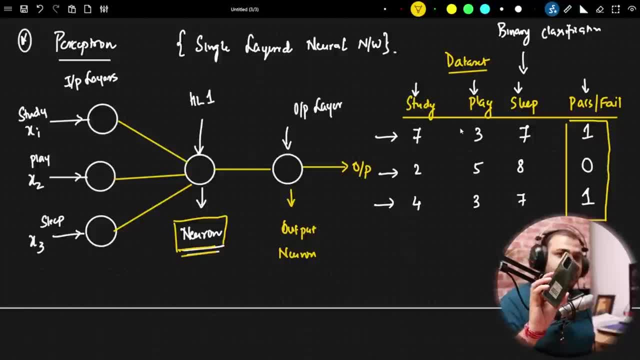 on this input data. suppose, if I show the mobile phone, it should be able to predict: okay, this is a mobile phone, right, we have to train them, right? suppose if there is a camera and if I see the camera, I have to train that. okay, this is the camera itself, right? so the training process is something different. 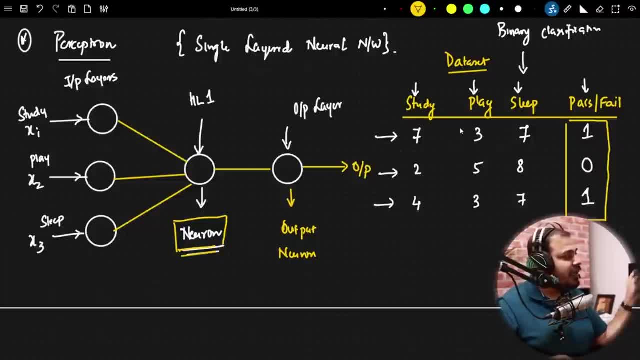 right, but I hope everybody is able to understand what does the hidden layer one look like and what is output layer. and like this we may have any number of hidden layers, because the signal passes through various neurons, one neuron to the other neuron, and each and every neurons will be having a different. 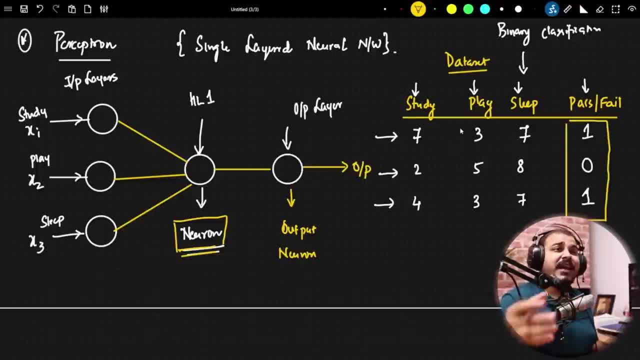 different hidden layer. in the hidden layer one I may have five to ten neurons. in the next layer I may have hundred neurons. right, and each and every neuron will be processing those signals that is given from the input layer. so is this clear till here everybody? so recently my, my child also said: Papa right and 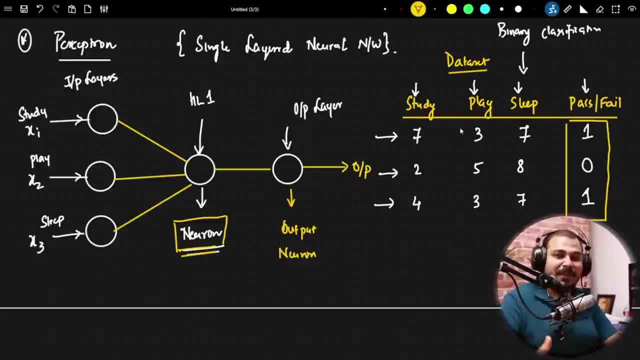 so I have to train him for six months and to tell him daily: Papa, Papa, Papa, Papa. then, finally, was able to talk about it, right? so that is the most happiest part. I have trained a original human neural network, so that's, that's amazing, right? so that is the reason why I'm able to explain you with so much of 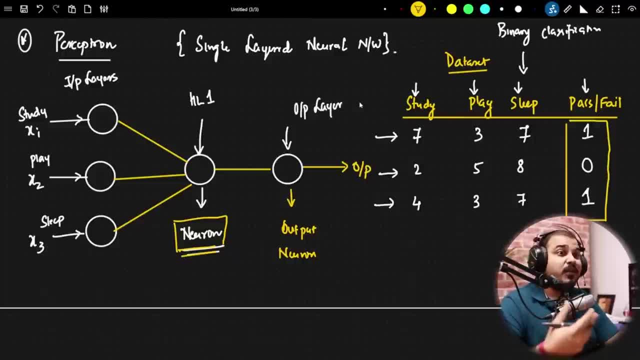 intense analysis right now, we understand what kind of processing will happen in the next section. okay, fine, I have understood. this is my input layer, this is my hidden layer, this is my output, but what is the processing that actually happens? right, What is the processing? What is this line for when the signal is getting passed? 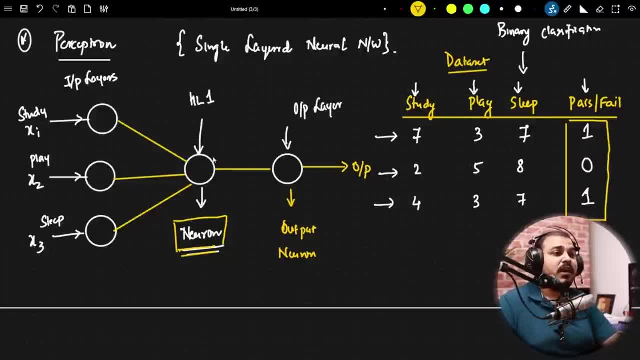 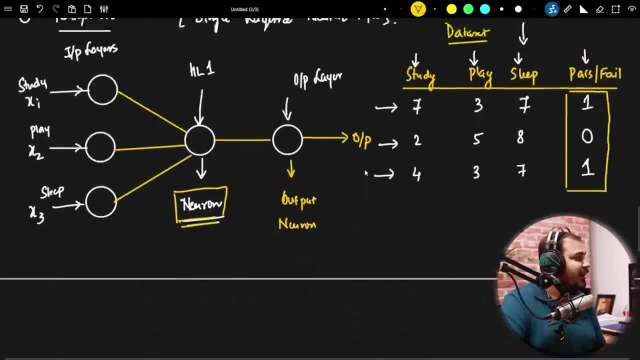 from here to here. What is the thing that will happen inside this neuron that we can basically see? Okay, So, uh, I hope everybody's clear till here. Let's go to the next step And uh, I'll, I'll still not again, uh, create all these things. So I will just do a little bit of smart work. 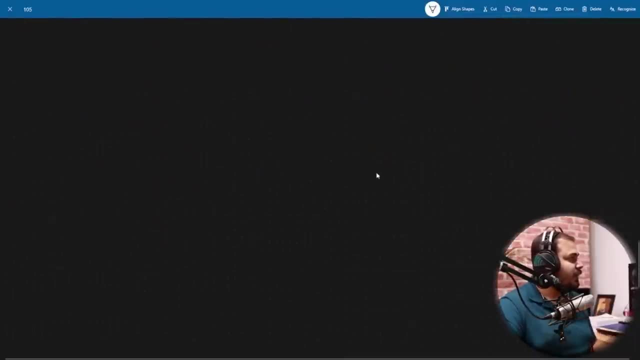 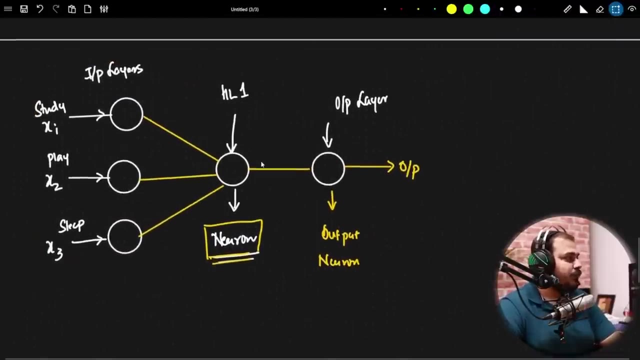 and I'll copy the same thing. copy it and I will paste it over here. Amazing, right. So this I love this editor, you know now? uh, let's go. Okay, I've already shown my data set. My data set. 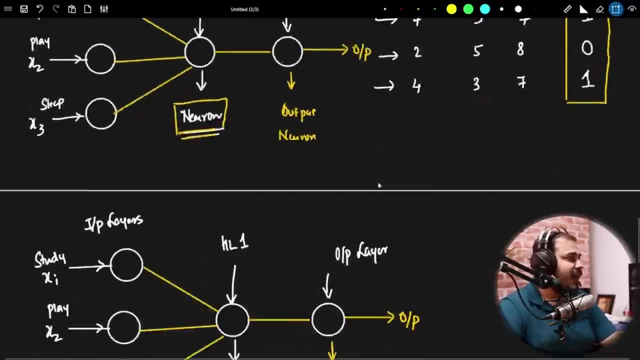 looks like this: Okay, Uh, 7, 3, 7, 1 like this. So input will definitely go. What happens when the input from the input layer it goes to the hidden layer one? No, it is not necessary. You. 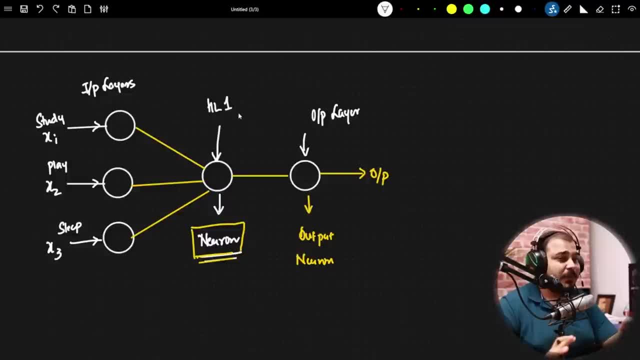 need to have hidden layer one only. Okay, You can have many hidden layers. I'm just talking about perceptron. This is one example. Okay, Now let's say what happens in this layer, What happens in between, as soon as the input goes to the hidden layer one. 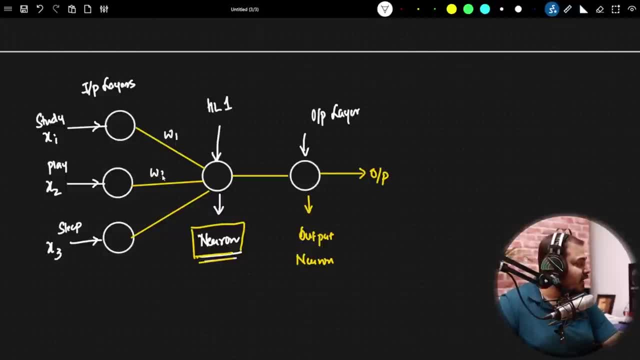 So here we assign weights. Let's say, these are my weights. Okay, Now what is the importance of this particular weight? We will try to understand. but before that, what do we do with this weights? We'll try to understand. Okay, Let me create it. Uh, once again, for you all, I can take this much. 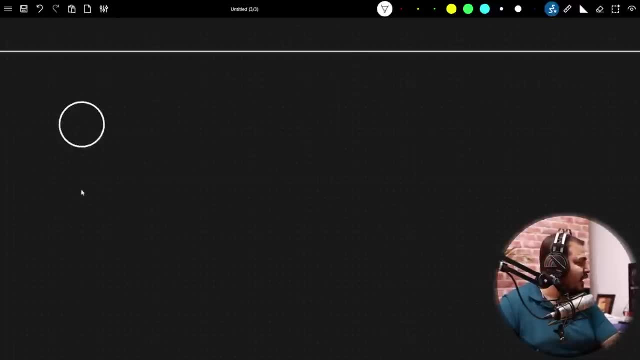 pain. Come on. So this is my input layer: input one, input two, input three. All right, And let's say, in my hidden layer, this time I take it Two neurons. So one, two neurons. let's say I can have any number of neurons. Okay, I'll talk about. 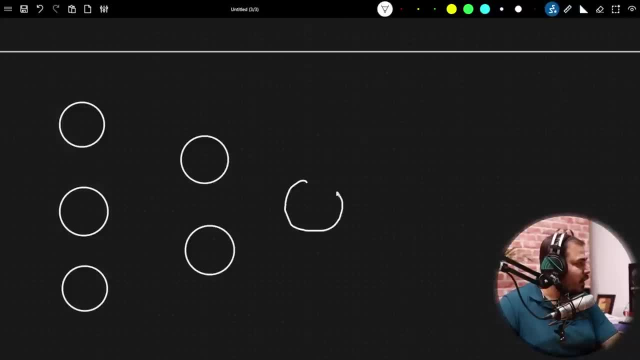 how the weights is decided, and all don't worry. Okay, And finally, this is my output lab. Let's connect this quickly. Uh, so this is my I: one input one, input two, input three, and this is getting connected over here, here. here, Remember, every neurons will get connected, right, Every. 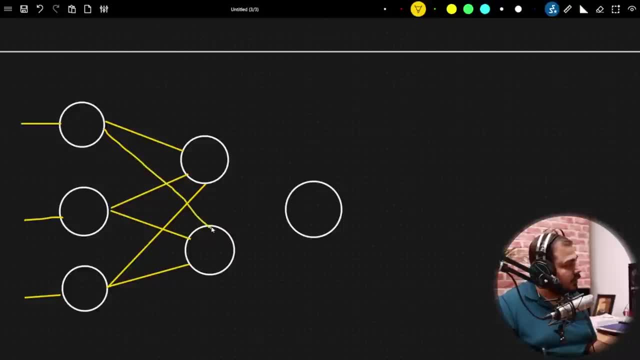 neuron has to get connected, you know. Then only it will be working, because it is just like a brain cells, right, Every signal will get passed. Okay, Let's talk about it. So this is my X one, This is my X two, This is my X three. Now, 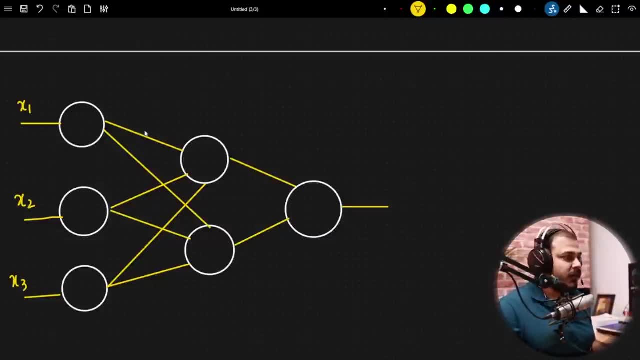 what happens, what happens inside this? Let's let's talk about it Like: uh, what exactly happens in this? So here I will be assigning different, different weights. Okay, I will be assigning different, different weights. So let me just make this diagram a little bit more simpler, So that 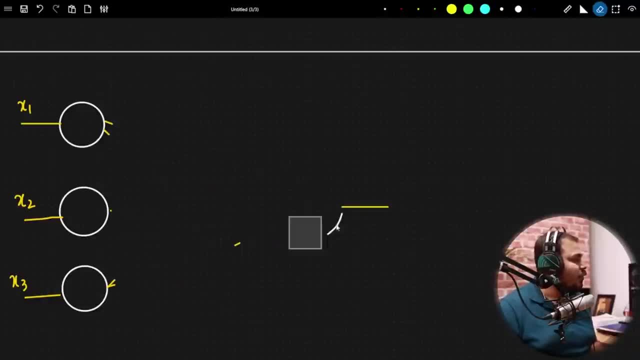 again, you should not get confused, because if we are able to understand one right, Then definitely you will be able to understand all the other things. Okay, So what I'm going to do? I'm just going to take one neuron, or I'll make this neuron. 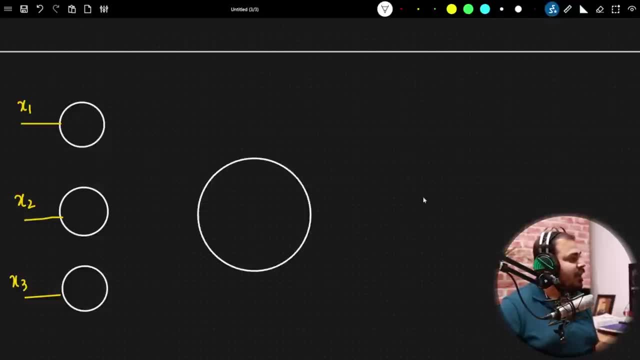 size bigger, so that two operations can fit in this. And finally my output. Okay, So this will get connected over here, This will get connected over here, and this will get connected over here, And this will get connected over here And finally, this is my output. So this is my. 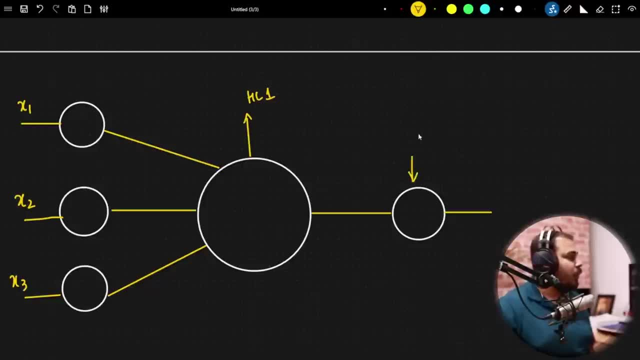 hidden layer one. This is my output layer. Okay, So I hope everybody now here. I've already told you we will assign different weights. I'll talk about the importance of weights. Now, inside this, there will be two operations that will be happening. The first operation will be that. 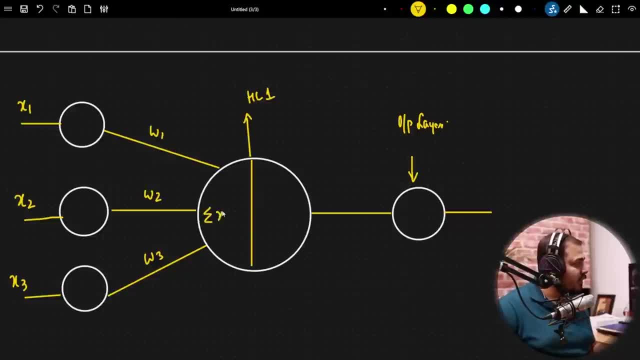 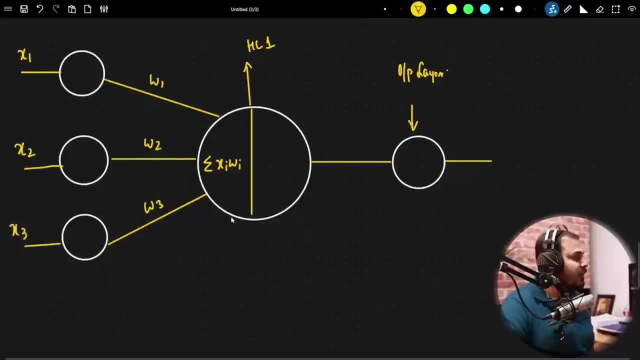 we just have to do the summation of X of I and W of I. Okay, So what we are doing? summation of x of i, w of i. This basically means what? if I write the equation, what is summation of X of i, w of i? it is nothing but x one w one plus x two w two plus x three w three. 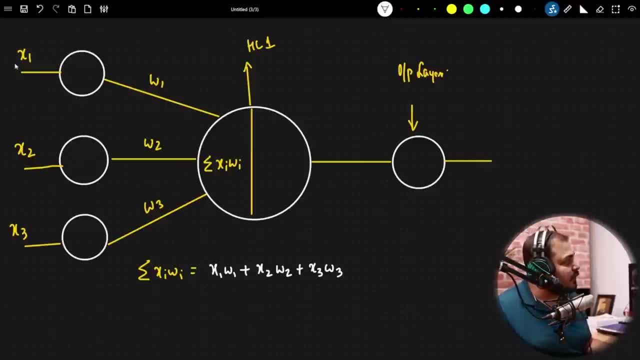 plus Okay. So here what we are actually doing, we are just multiplying x one w one plus x two and w two and x three and w three. Right, I can also write this as w, w transpose x. okay, And I hope everybody remembers this thing right, It is similar to: 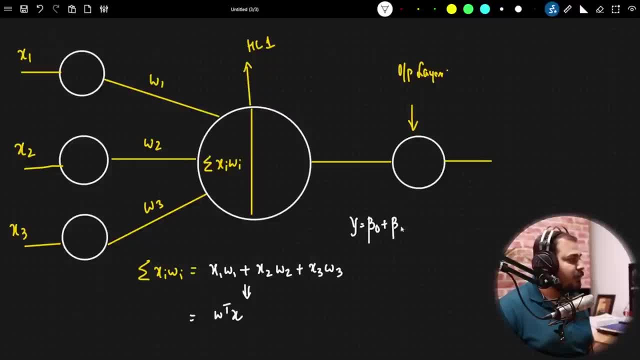 our equation of the linear regression, like beta 0 plus beta 1 multiplied by x right. We can also write this as: beta transpose x right: Same linear regression. If you remember, in linear regression we also use y is equal to mx plus c. Different, different equations, right, So same thing. 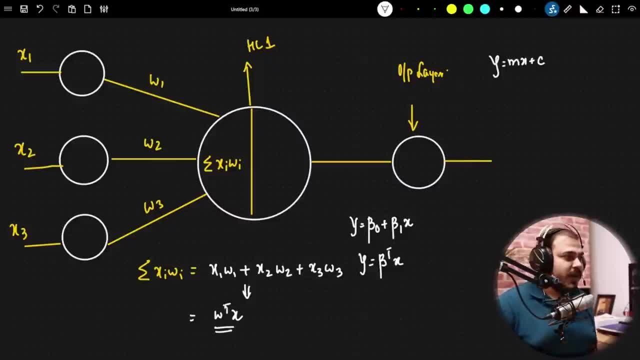 right. So this is nothing, but w transpose x. okay. So w transpose x is nothing, but it is the summation of x1, it is a summation of inputs multiplied by the weights. okay, Input multiplied by the weights. So this is the first step, This is the first step in the signal, okay. 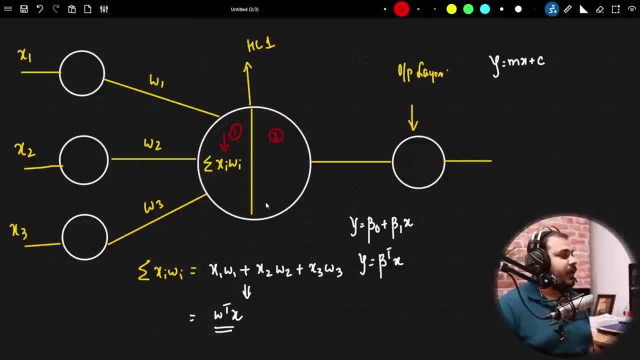 This is basically the first step. Now what about the second step? In the second step, we pass this equation to an activation function. We pass this to an activation function. okay, So we pass this to an activation function. okay, Now let me first of all okay, before going to the second step. 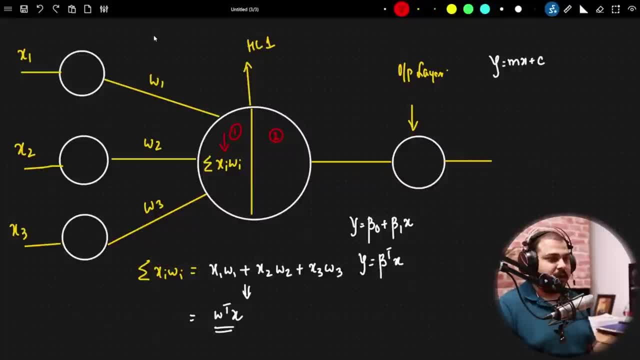 let us understand. what is the importance of this weights? okay, Now tell me, guys, suppose if I put my hot, if I put a hot object in my right hand, then will I not move my right hand away? It is a very common question, see. 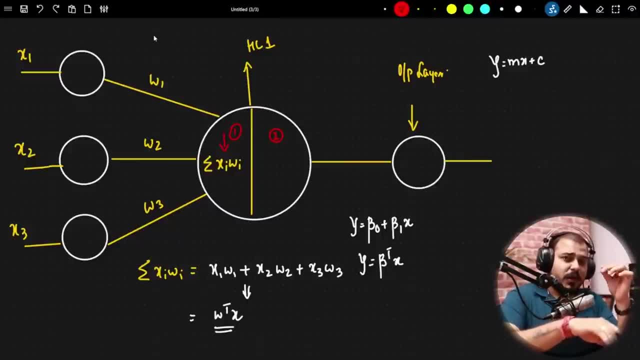 Very simple question. What I am doing is that I will put a hot object into my right hand and then obviously, it is sure that I will be removing my right hand. okay, I will be removing my right hand Now, when I remove the right hand. the reason why I am removing the right hand. 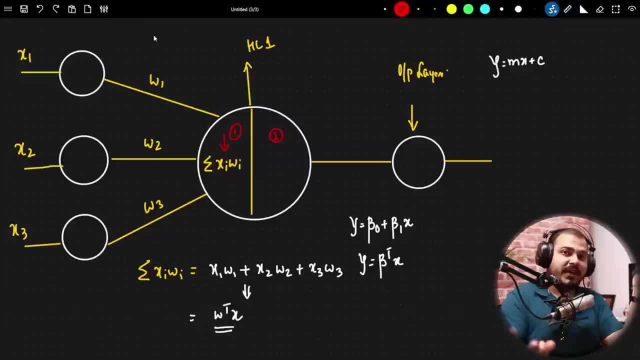 because the neurons that are passing from here, those are getting activated right, Those are getting activated right. If I am putting a hot object over here, the neurons will definitely pass the signal to the brain. I am saying that something hot object is placed and I am going to move it, So these weights will. 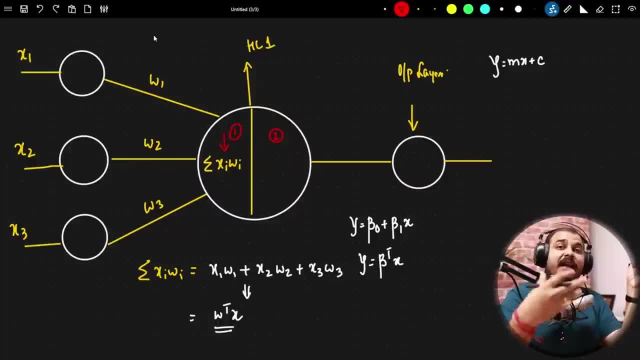 actually help your neurons to act, whether it should be activated or what level it should be activated. Let us say, if I am putting the hot object into my hand, I am not moving my left hand. That basically means my neurons are signaling the weights over here and it is making sure that all 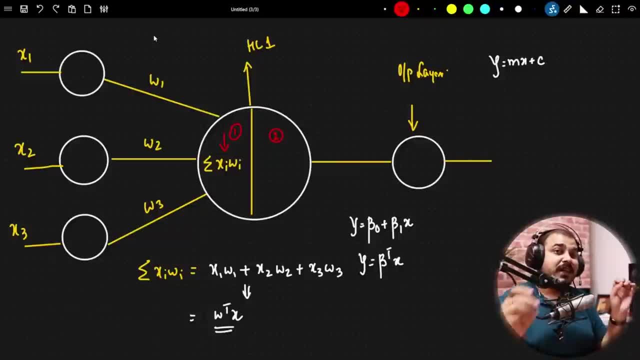 these neurons get activated till it passes the signal. So this is the importance of weights During the training of the neuron network. also, we will be taking care that which weights should have what value, so that the neuron should be activated till that level or not. okay, Very, very simple. This is the 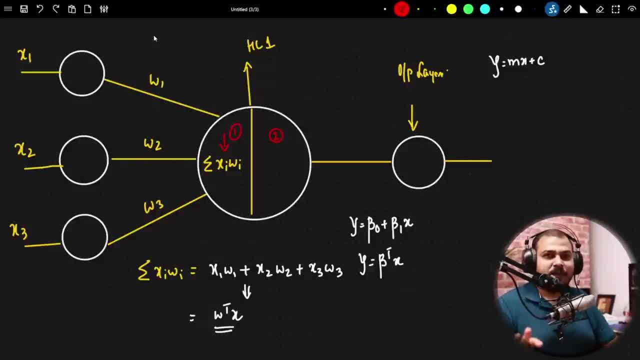 most easiest way to understand about weights. okay, So weights basically says that how much the neuron should get activated or deactivated. That's it, Very simple if you really want to understand as a person who really want to clear the job interview as quick as possible, okay. 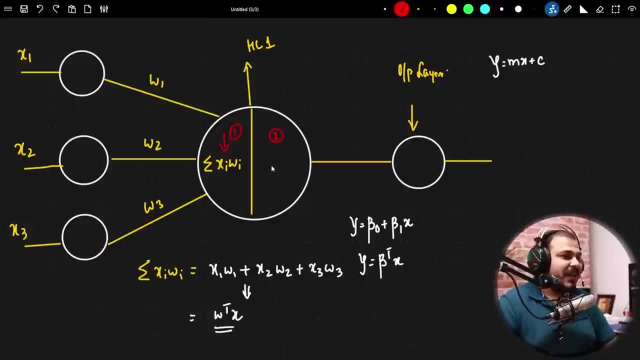 Now, I hope everybody has understood this. okay. Now, what if see these weights also? initially, we initialise it as zero. Okay, We initialise it as zero. right, Let's say that I have initialised it to zero. It is not necessary that we always. 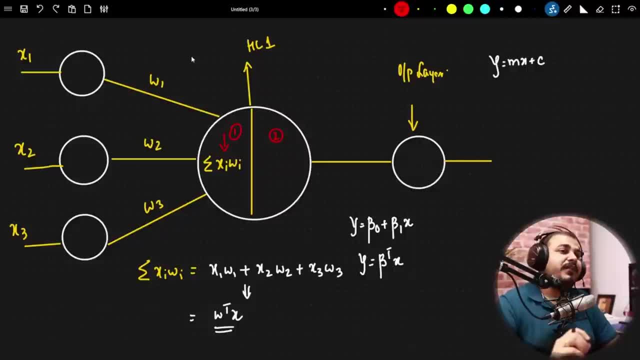 initialise to zero. but let us say I have initialised to zero. Now, if I have initialised to zero, what will happen? X1 multiplied by zero will be zero. X2 multiplied by zero will be zero. X3 multiplied by W3 will also be zero. Okay, Now what about X3 multiplied by W3?? Now I have you. have you need to? 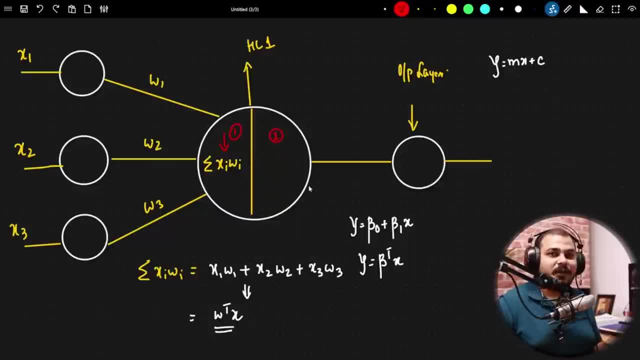 actually measure what this bar is. one dimensional means essentially the cycle of speed, and I am already Okay. now, when all this value is zero, we are just passing zero right. So for that, for that to overcome, so that the weight should not be zero. 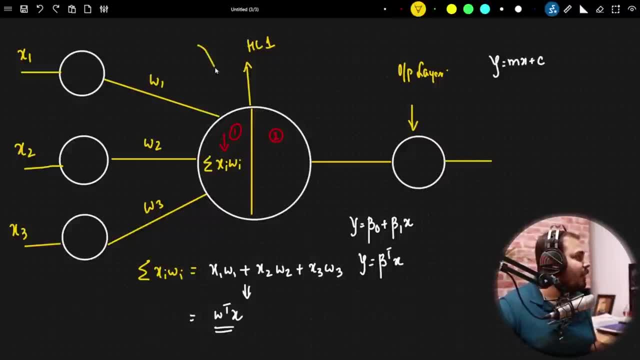 we add another parameter, one more parameter which is called as bias. Okay, so I hope everybody's understood. why do we add a bias? And I hope you have seen this term right. This is a constant term. We basically say it as a constant. 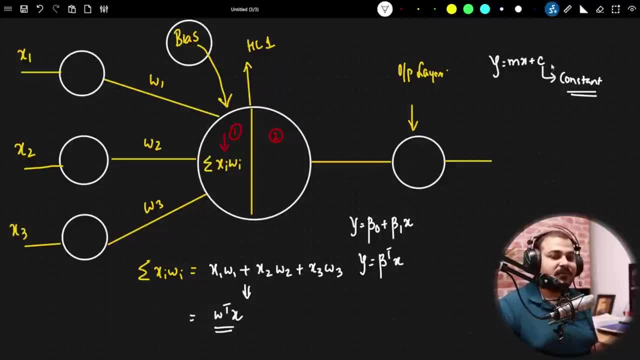 We basically say that it is an intercept right. Intercept right. We say C as intercept right. So that is the reason why in that equation also you'll find an intercept. In this also you have a bias such that by mistake 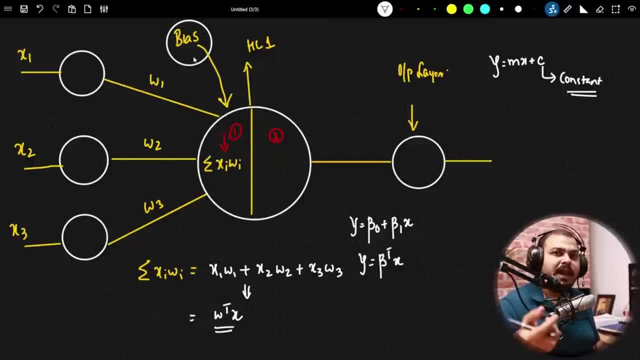 if you probably initialize all the weights as zero, bias will have some value, so that some value it will not be equal to zero. So we can continue that particular training. Later on we can update the weights right Now. what happens in the second step? 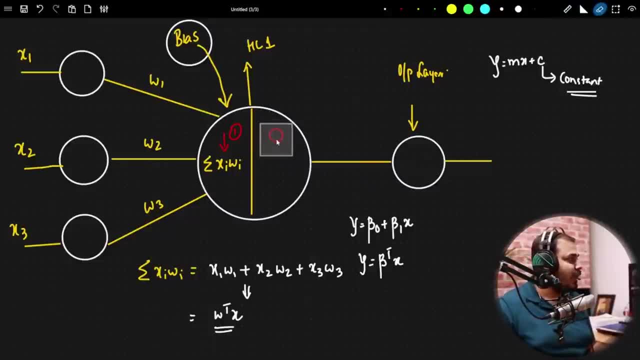 Let's understand, okay, What happens in the second step. Okay, so, in the second step, let's say that this entire equation, this entire equation that I have written, that is, summation of x of i, w of i, is given by y. 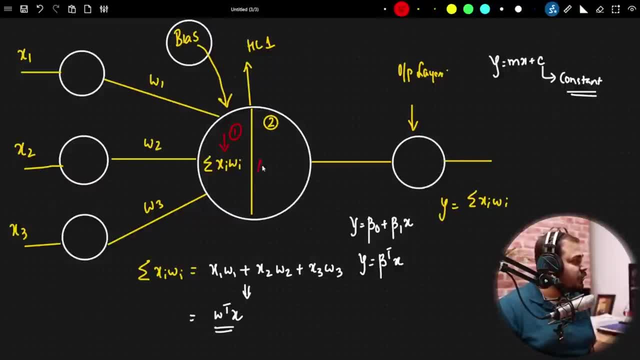 Okay, then we pass an activation function. an activation function on top of y. Okay, an activation function on top of y. Okay now, yeah, Bias will be required in Every hidden layer. okay, Every, every hidden layer, it will be required. 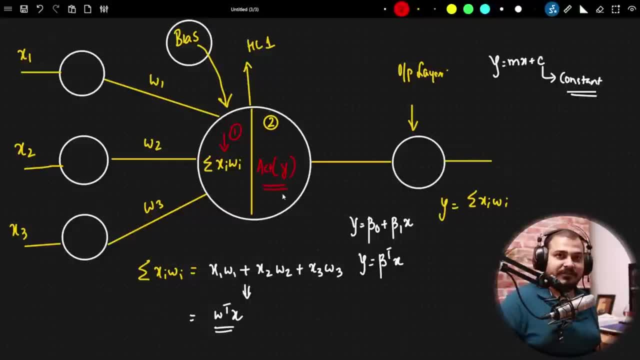 One bias will basically be required. Now, what is this activation function? Let's say, let's say again: I put a hot object in my hand, I'm moving the hand. right, I'm moving the hand. So this basically shows that, whether the neuron should be activated or deactivated, right? 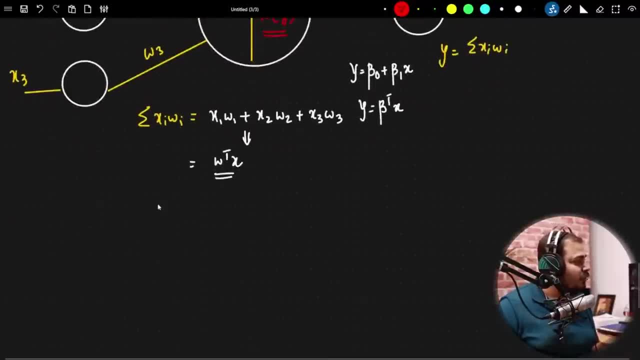 So one of the activation function, one example of the activation function which I'm going to basically take is something called a sigmoid activation function. Now, the sigmoid activation function, what it does is that I will talk about the equation. it is one e to the power of minus y. let's say okay. 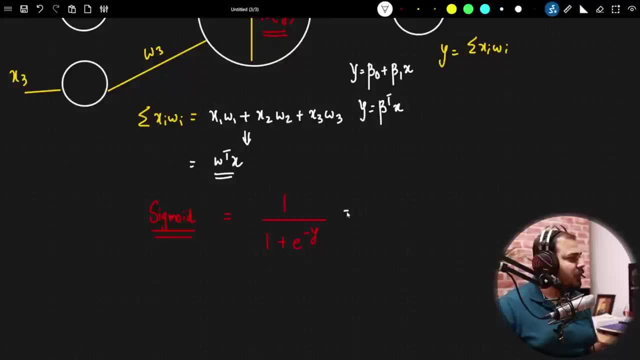 Now we will discuss about ReLU and all on the other in the upcoming classes. but let's say one example of this. This is that sigmoid activation function. we basically use it for binary classification. let's say binary classification, okay. 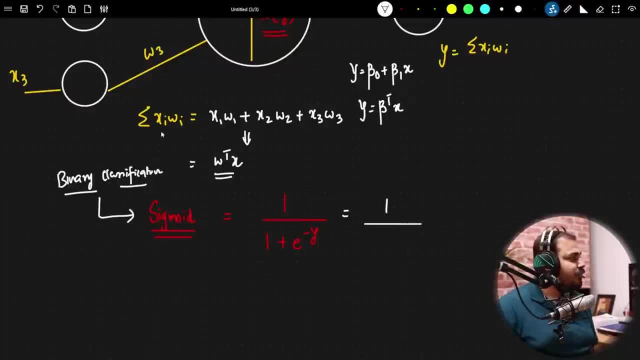 Now, if I replace y now y, is what This one right One plus e to the power of minus, This summation of x of y, w of y right Plus bias. Sorry, I have to add bias also on top of it. okay. 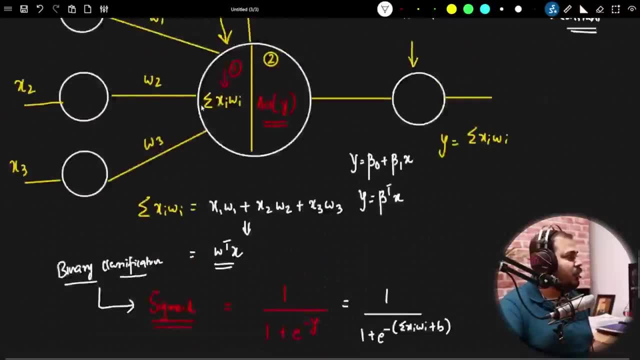 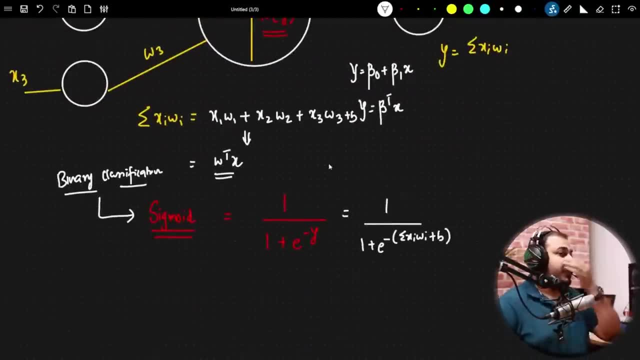 I have to add bias also on top of it, because this bias is also getting added right Over here now. this entire thing will become summation of x of y, w of y plus bias. okay, B, okay. Now the output of this equation is either 0 or 1.. 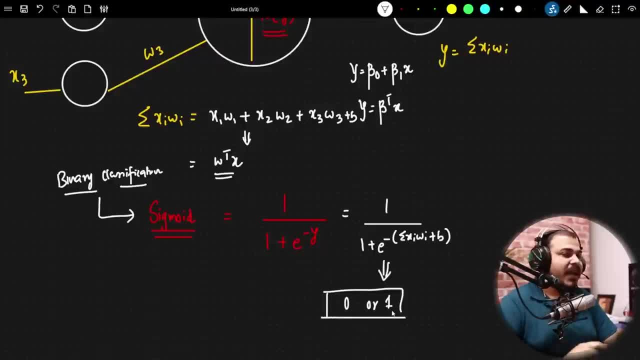 That is what sigmoid activation Function does about. Sigmoid activation function always gives the output as 0 or 1.. It is not like it always gives 0 or 1,. it can give you values between 0 to 1.. We write a condition: if it is greater than 0.5, we basically take it as 1,. greater than or equal to 0.5, we take it as 1, and if it is less than 0.5, we take it as 0,. okay, 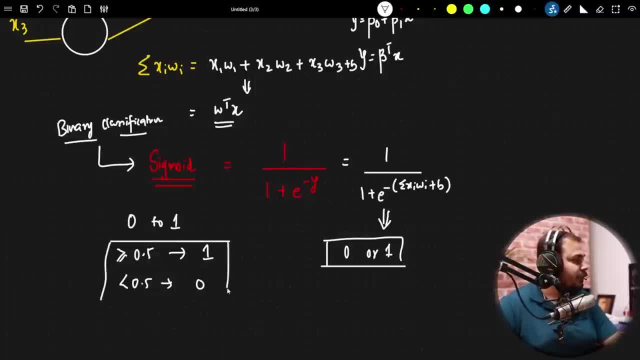 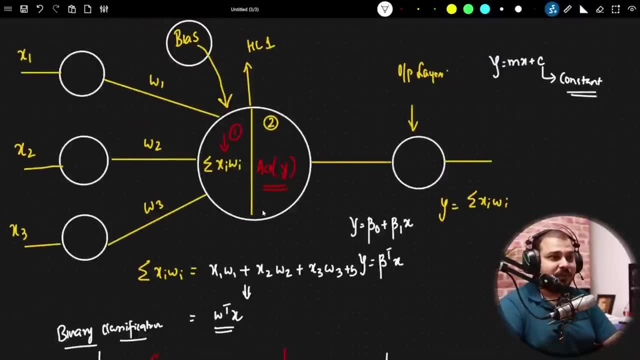 So these two conditions usually applies in sigmoid activation function. But the main reason of the sigmoid activation function is this: It is to basically say that, whether this neuron is activated or not, okay, So I hope everybody is able to understand, And this usually happens in every neuron, okay, 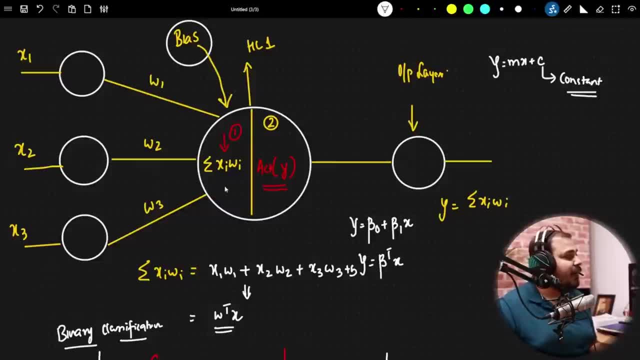 First thing, summation of the weights and the inputs, along with the bias. So here I am going to write plus bias, and then this will be an activation function of y. okay, On top of it, we take this entire thing and we put up an activation function. okay. 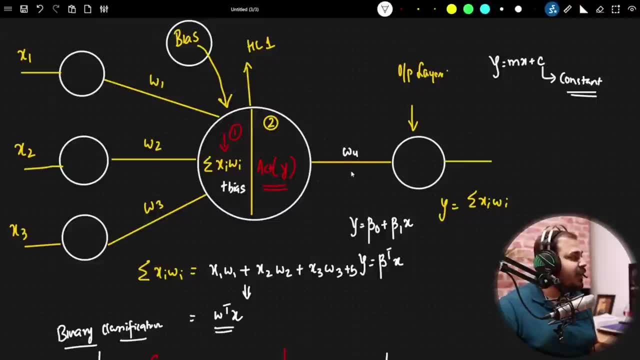 So this is what happens, and then, when we go to the next layer, another weight will get initialized over. here Again, two steps will appear, Basically happen. That will be the summation of this output, whatever output I am getting over here. 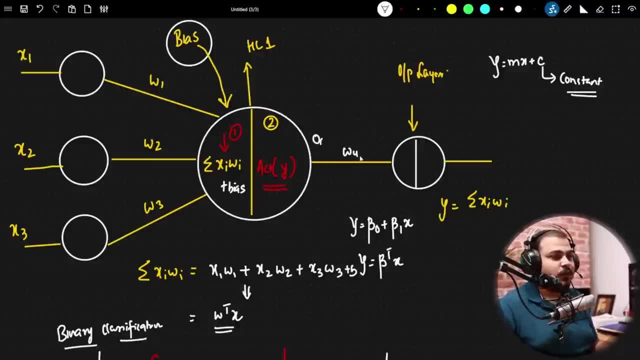 Let's say O1, okay, O1, and this will get multiplied to W4.. Again, what will happen Over here? the next activation function will get applied and, finally, I will be able to get 0 or 1.. Now, this is with respect to binary classification. 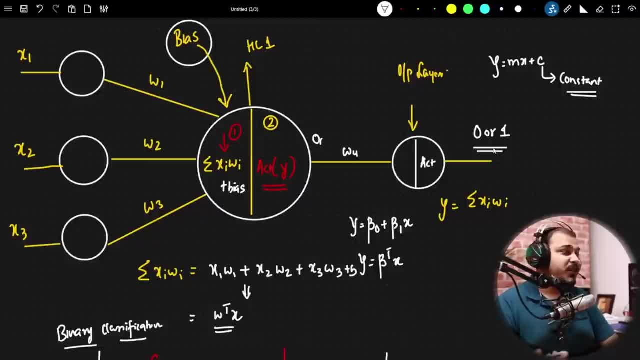 We use sigmoid activation function For linear regression, what all things we use. There is another activation function which is called as linear activation function. This also thing we will discuss Today. I just want to introduce Today. I just want to introduce you to some basic, basic topics, and that name should be always there. 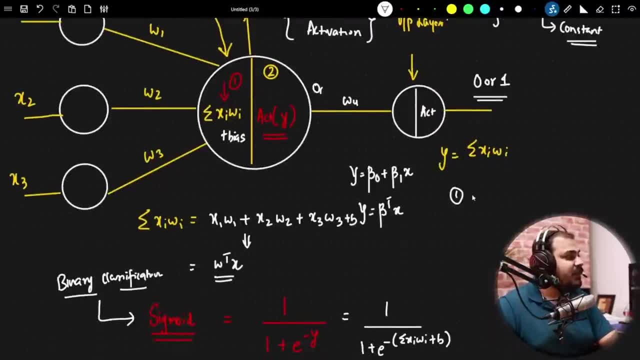 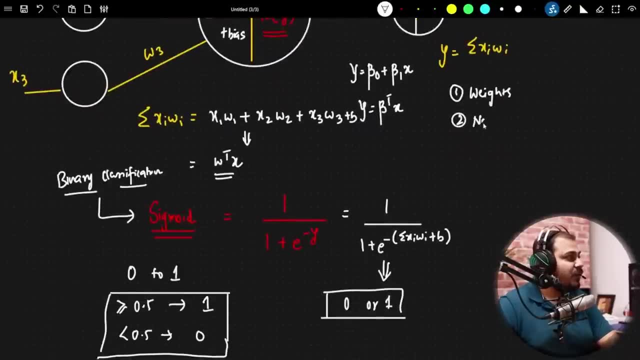 So what all things we have learnt till now? We have learnt topics like what is weights right? We have learnt topics like what is neurons- right? We have learnt about neurons. We have learnt about hidden layers. We have learnt about activation. 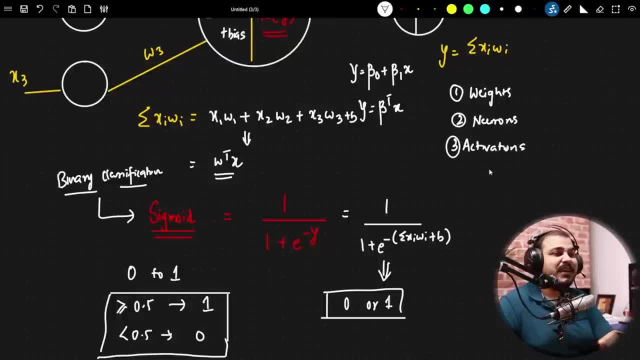 We have got an idea. We have got an idea about this terminology. What is activation functions, right. So all these things, slowly, slowly. now we are going to cover more and more topics, okay, But today I just want to show you what all topics are basically there. 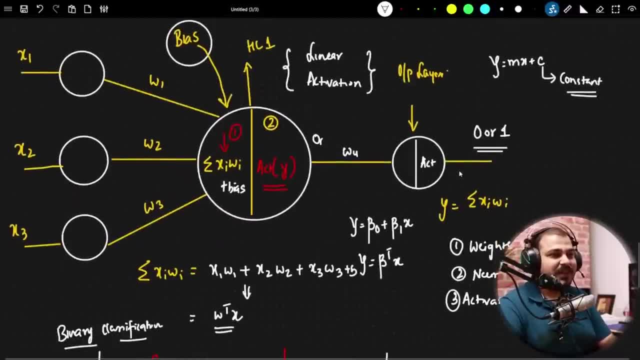 What all topics are basically there. okay, Everybody is able to understand, right? So I hope everybody was able to understand till here. Let's continue the next topic Now. I will give you an idea about forward propagation Now, whatever operation that we have done till here. 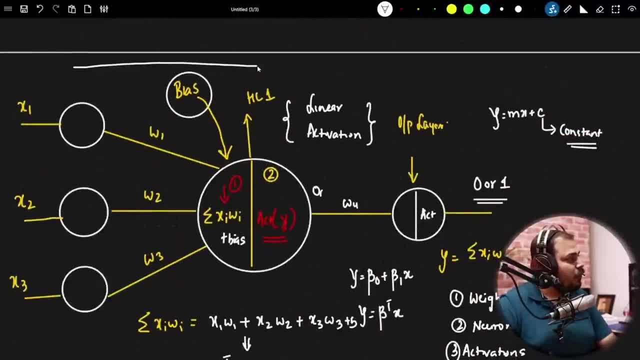 from here to here till the output right, What all functions. we did? We basically took the input multiplied by the weights, added a bias and activate right. We multiplied the inputs with the weights, added another bias and activate right. 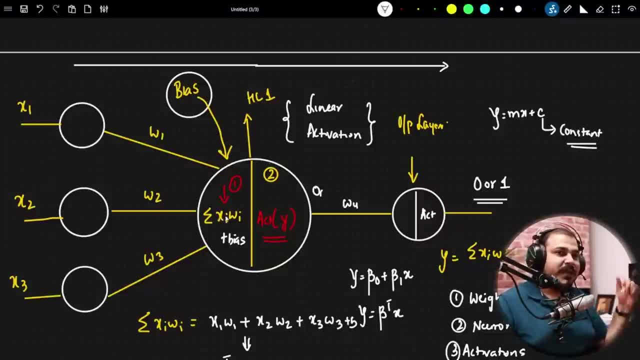 So this you can basically remember: We took an input, we multiplied with the weights, we added a bias and then we activated right. So this entire process till the end is called as forward propagation. So this is basically called as forward propagation. 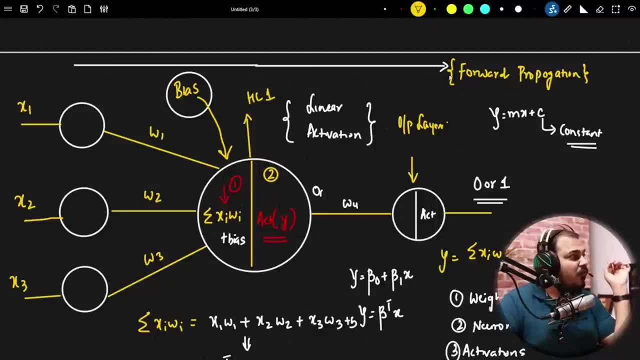 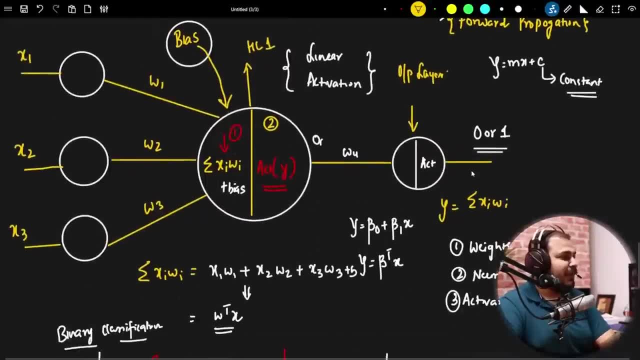 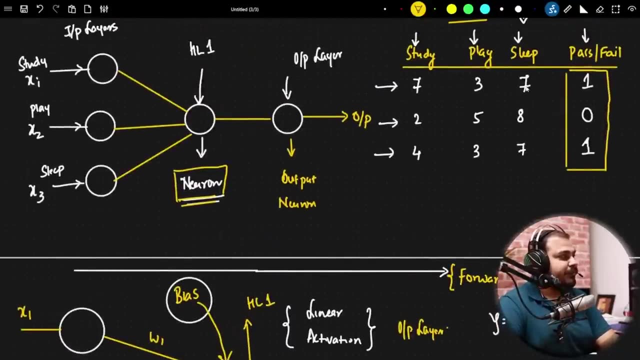 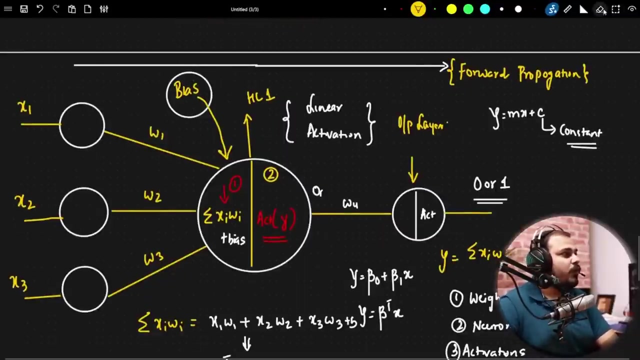 Okay, So this is basically called as forward propagation. Now let's discuss one very important thing. Okay, let's discuss one very important thing. Let's say, let's say, for this first input, okay, this first input, 737, I passed. I went inside this, I initialized a weight and let's say I got an output of. I got an output of, let's say, I got an output of 0.. 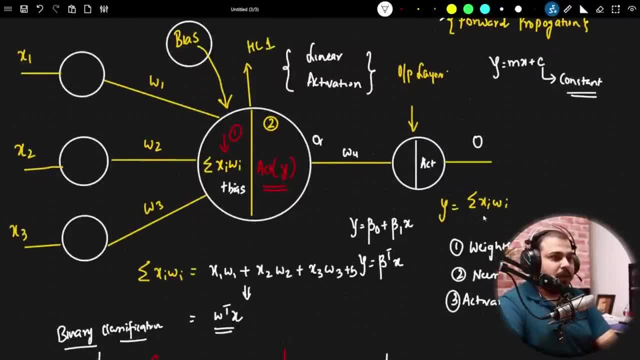 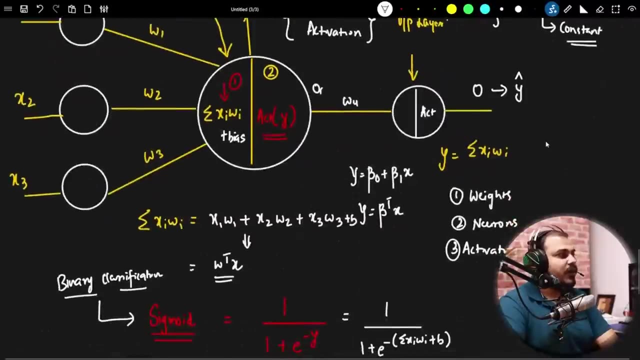 Okay, I got an output of 0.. Now, when I got an output of 0,. okay, when I got an output of 0, but this 0 will be my predicted value. y hat, This will be my predicted value. that is y hat. Okay, for the forward propagation. first, forward propagation. Then what is my y? Y is my truth value. So what is my truth value over here? My truth value is 1.. 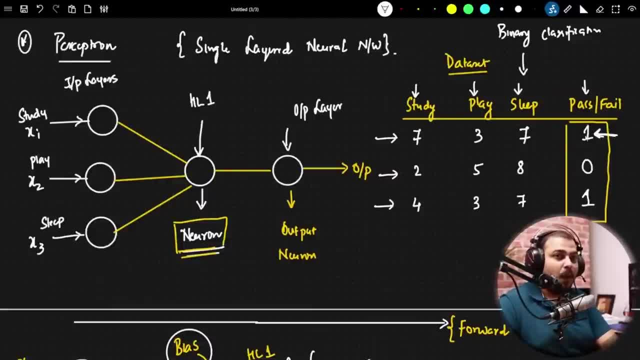 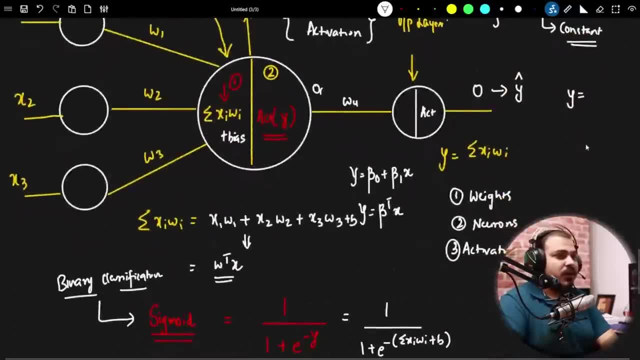 Right, My truth value is 1.. I hope everybody is able to understand what is my truth value here. Obviously, my truth value is 1.. So if I take this- 0 and 1, if I just subtract it- y minus y hat, obviously this is not the output that I want. I want 1 as my output, but I am getting 0 as my output, Right? So if I subtract y minus y hat, I'm actually going to get 1.. 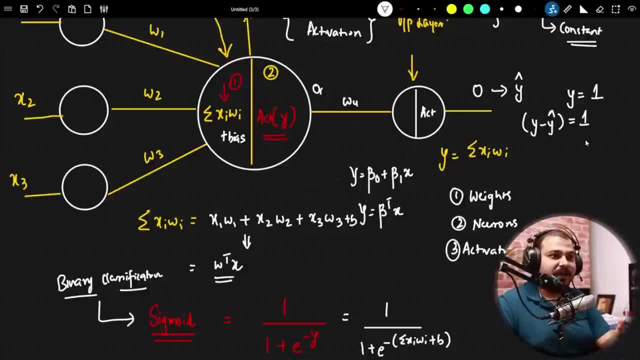 Right. So if I subtract y minus y hat, I'm actually going to get 1.. Yes or no? Yes, everybody is clear. See, y is nothing but 1.. y hat is 0.. 1 minus 0 is 1.. Right, 1 minus 0 is 1.. Yes or no? Okay Now, since my difference is 1, and I know my output is completely wrong- that I'm getting Right, So what I have? to make sure that this difference should be very near to 0. Okay. 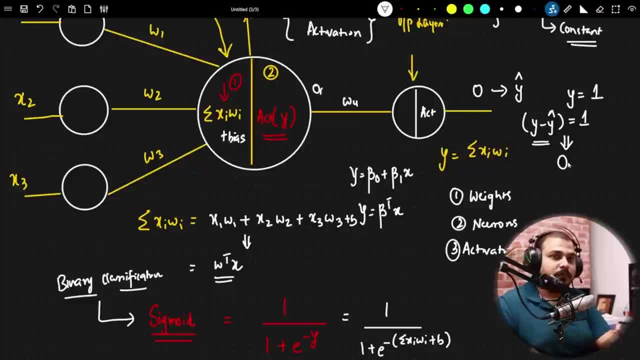 This difference should be very near to 0.. So what can I do for that? And what is this y minus y hat? There is a very important term which is called as loss function. So what is loss function? Loss function, they are different kind of loss function. Okay, They are different kind of loss function, which I'll be discussing, But here I'm more focused to tell you about terminologies. 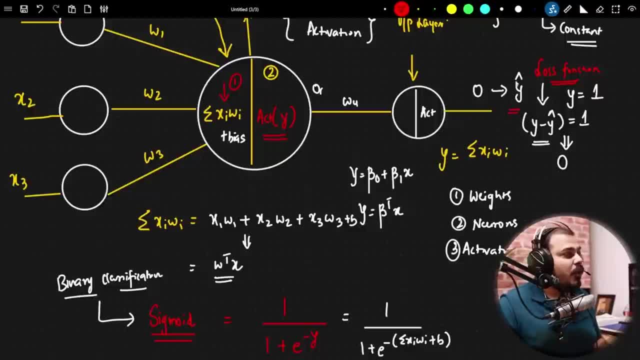 So loss function will basically find out the difference between your predicted values And your real value, And always the main aim should be that we should try to minimize the difference. Everybody clear We should try to minimize the difference. The difference should be very much near to 0. Then only this y hat and y will be matching Right. So this is basically called as loss function. Okay, This is basically called as loss function. 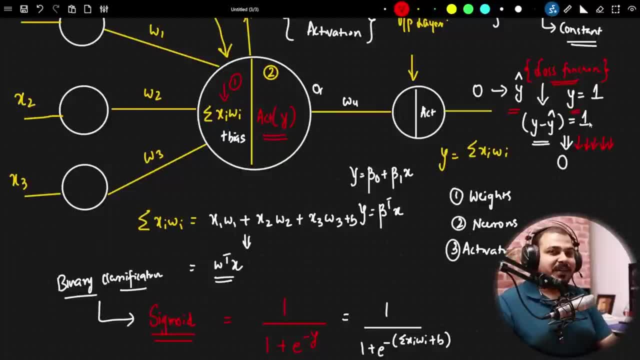 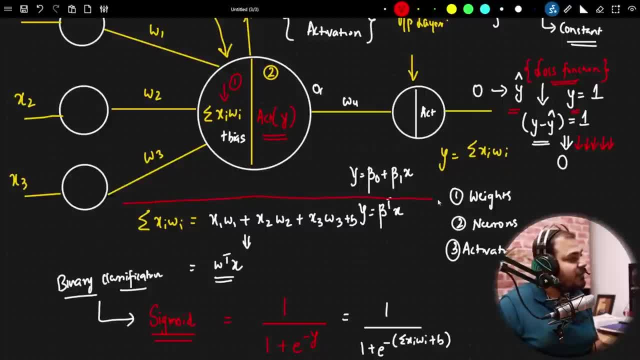 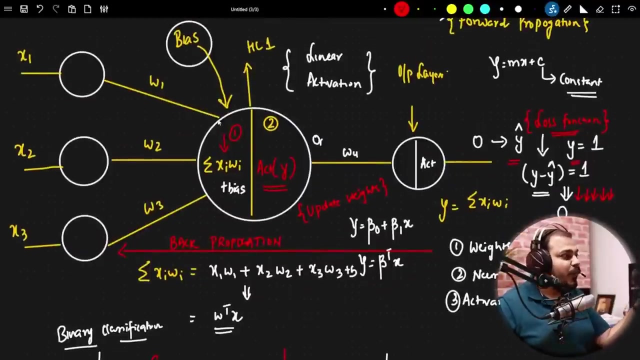 a very important thing, which is called as back propagation. And what is the aim of the back propagation? The main aim of the back propagation is to update weights, Because only when I update these weights, only while we are updating these weights, then only we will be able to get this. 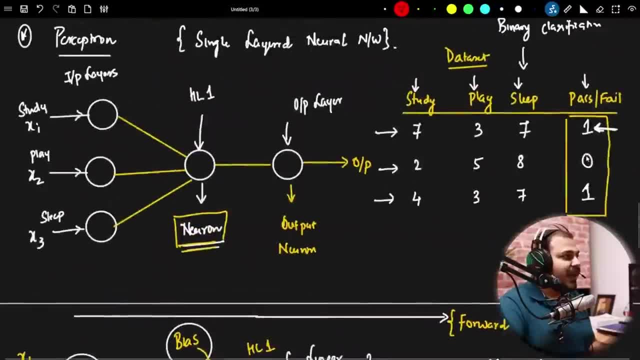 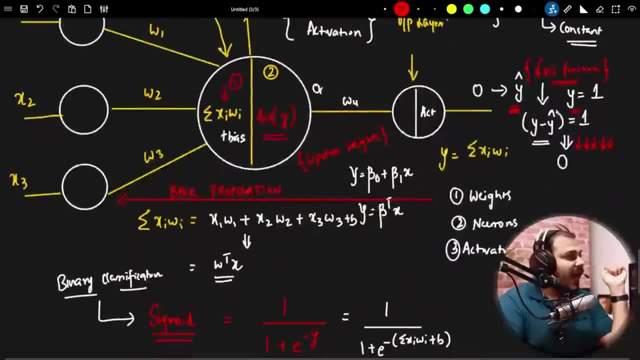 predicted output matched to our real output. What is my real output over here? I am training a supervised machine. I am training a supervised machine. I am training a supervised machine Learning, a deep learning problem statement. My output should be one, but I am actually getting. 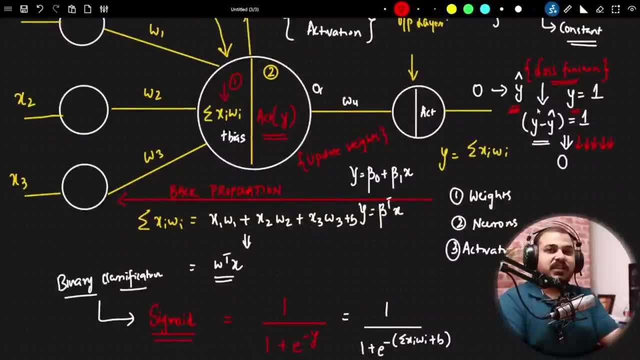 zero Right. So to reduce this difference, what we have to do is that we have to update these weights, Right, We have to update these weights, And this updation process will basically happen because of back propagation. And how is this basically happening? How back propagation is. 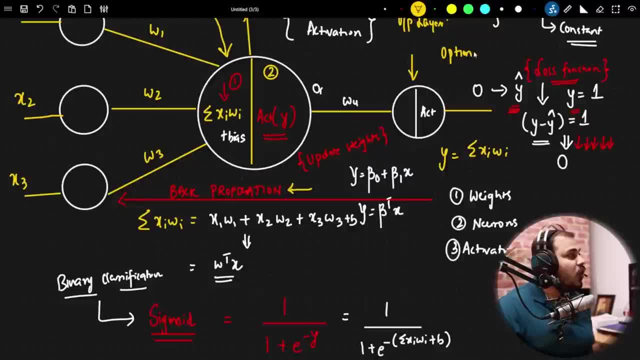 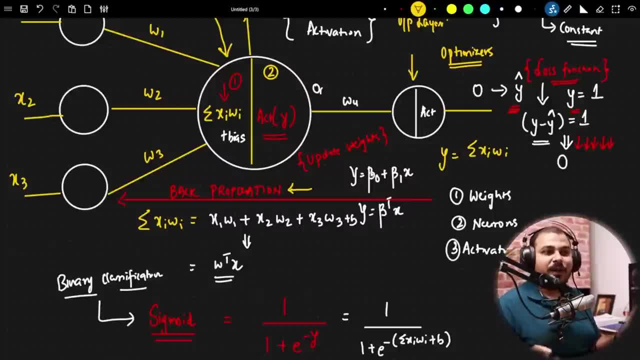 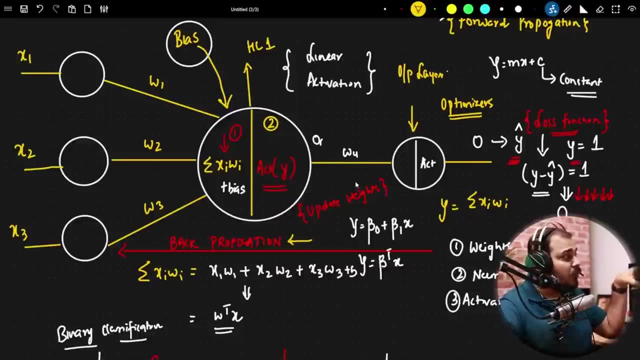 propagating. So, guys, are you able to understand or not Understand the process? Don't worry about what is happening inside, That I will definitely cover, The maths part I will definitely cover. But understand how the training happens. This is the training process. Training process includes: 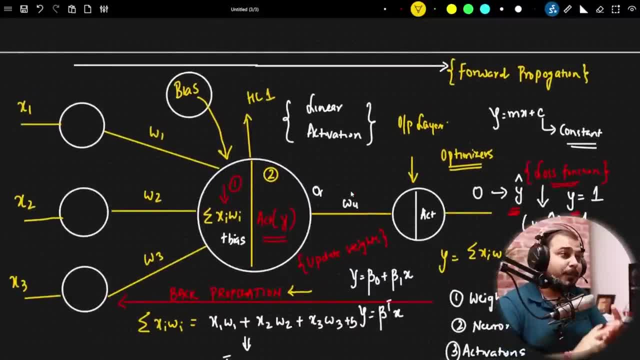 weights. It includes forward propagation. It includes back propagation. It includes back propagation. It includes bias. It includes this operation that is happening inside the neurons And then, when we get the output, we find out the loss function Right. And what is the difference? 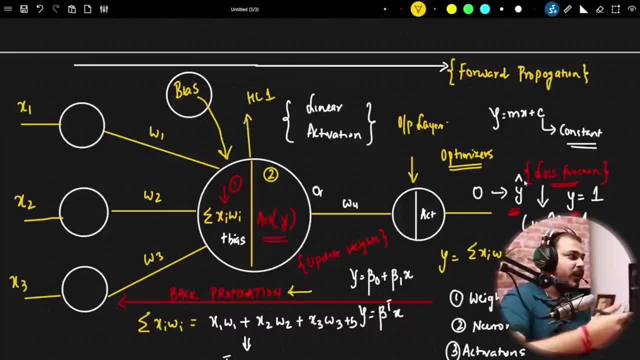 between the loss function. If the difference is high, then we back propagate it and we update the weights with the help of back propagation, And over there we use something called as optimizers. How many of you know simple linear regression? How many of you know simple linear regression? 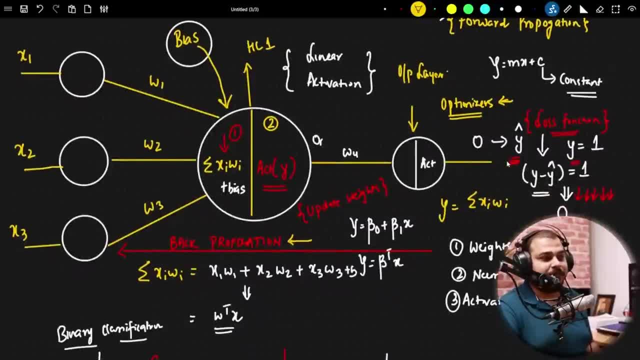 How many of you know simple linear regression? Tell me. Okay, How many of you know simple linear regression? Just tell me, In simple linear regression. have you heard of gradient descent? So one example of an optimizer is gradient descent. What is gradient descent doing over there? It is changing the correlation. So what is gradient descent doing over there? It is changing the correlation. 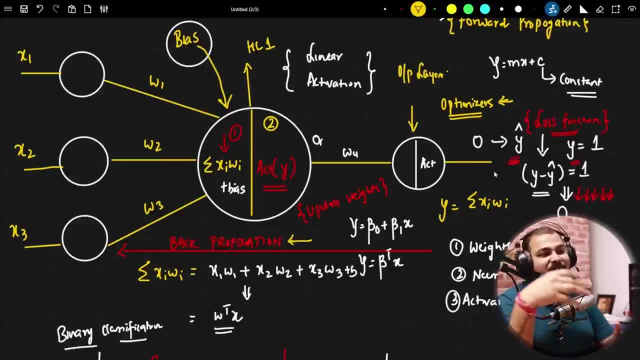 It is changing the correlation. So what is gradient descent doing over there? It is changing the correlation. It is a combination of both forward and backward propagation. In the backward propagation, weights will get updated, In the forward propagation weights multiplied by the inputs, Bias will get added and an activation function will. 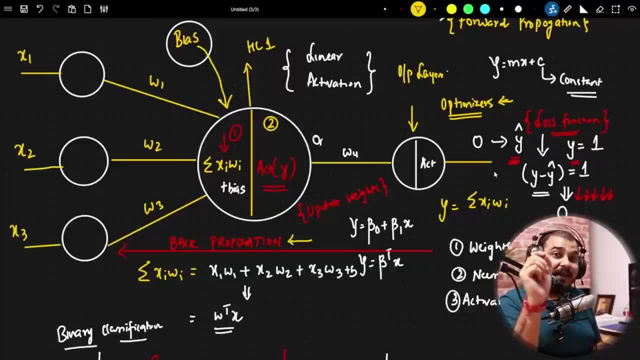 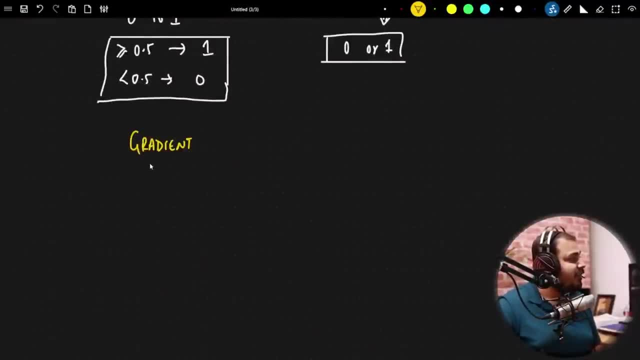 get added till, the output is basically coming. So in simple linear regression, I hope everybody has heard about gradient descent. What is gradient descent? What it does is that. I hope everybody has seen this curve. It is called gradient descent and it is created using 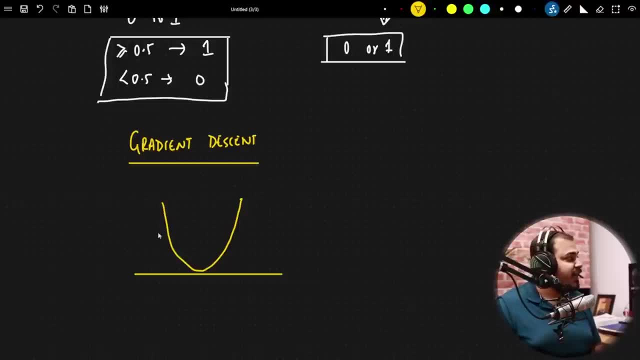 curve right- see, in this curve right gradient descent, will make sure that the coefficient- this is the coefficient right, this will be the coefficient, it will make sure that it will update this coefficient from here or here to basically come to the global minima and this global minima. 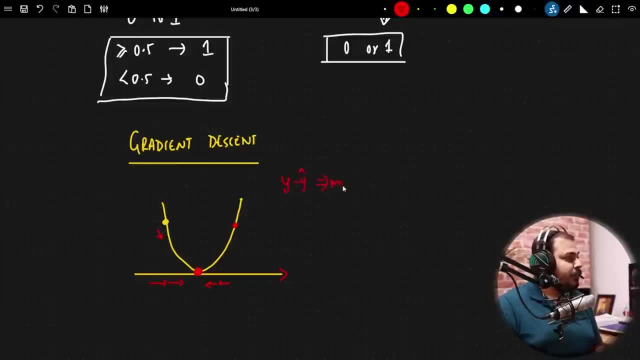 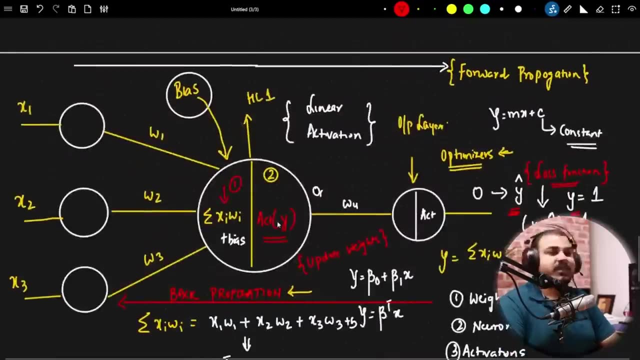 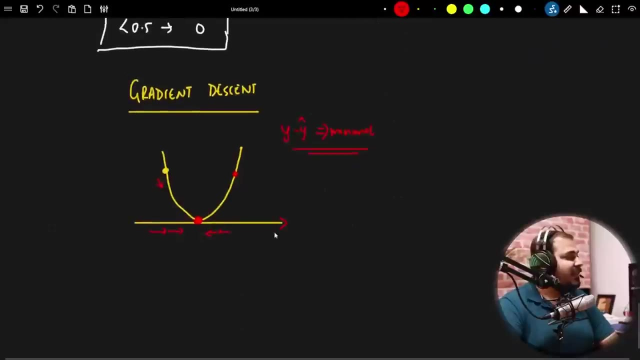 the difference of y and y hat will be minimal, and the same thing is basically happening in this thing also. so that is the reason when i explained about machine learning. whether you have seen or not, i have explained this specific thing and this gradient descent is a kind of 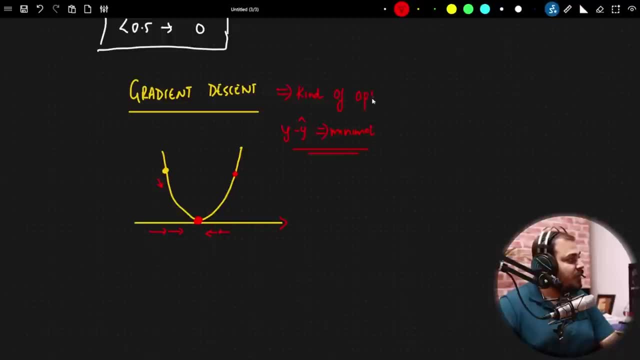 optimizer. this is a kind of optimizers. so, in short, let's start the story, whatever things we have learned from today. so, story conclusions, i'll say so. first step: what is this? first step? we have learned about input layer. now, from the input where it goes to the second step, the second step, weights will get added. 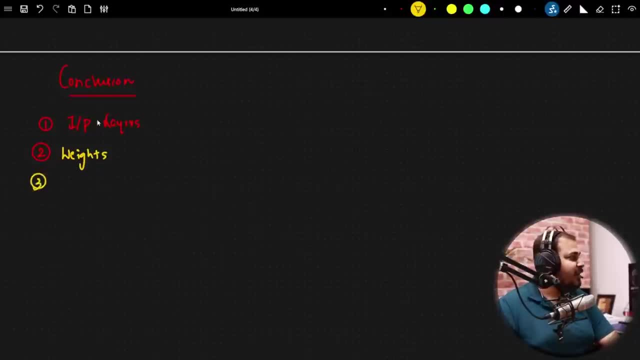 right. the third step: after the weights, the input and the weights will get added, and then it will get added along with the bias. and then what is the fourth step? an activation function will get applied. activation function will get applied till the last layer. this entire process in the 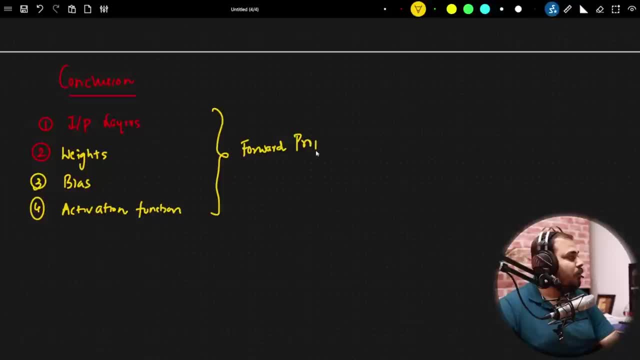 forward propagation. forward propagation right and in the backward propagation. what will happen? fifth step: in the backward propagation. first we calculate the loss function. loss function is nothing but the difference between y, hat and y. let's say- let's take this one example- the different types of loss function. we have to minimize this. 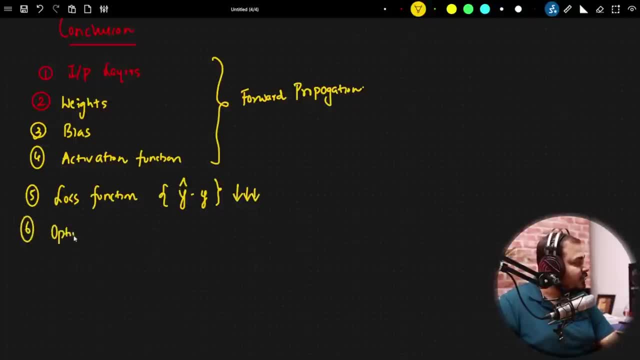 value. how do we minimize? we use optimizers. optimizes what it does: it updates the weight, updates the weight and this is the way to do it. so we have to minimize this value and we have to reduce the entire process. of what? backward propagation? backward propagation, and if this step is 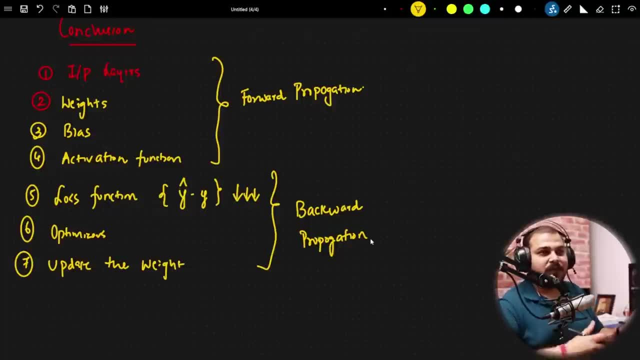 happening. one like one feeder, proper one backward. if you are doing it thousand times, our neural network will get trained, just like a baby gets twained. that's it, that's it. that's that's how important ticket, how easy it is you from putting fairly much coverage. hell yeah, deixar. 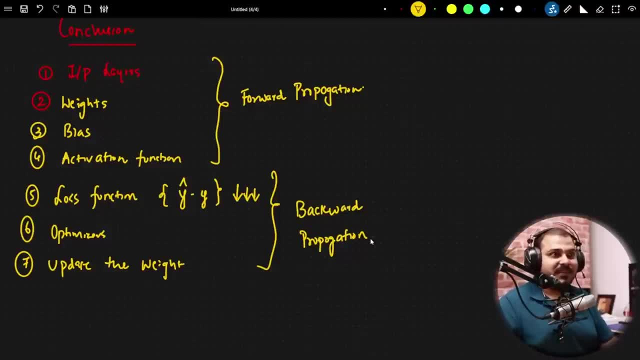 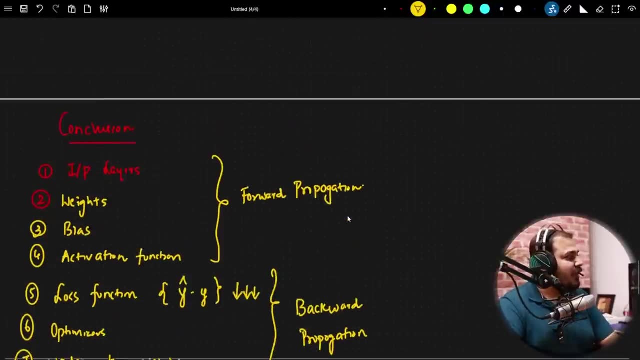 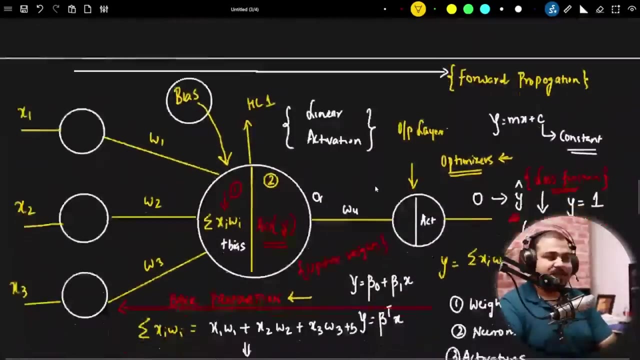 you are able to basically see it with examples, right? You are able to understand this right. So it is just the combination of forward and backward propagation, And here you will be able to get some amazing outputs like this. let it be image classification, object detection. 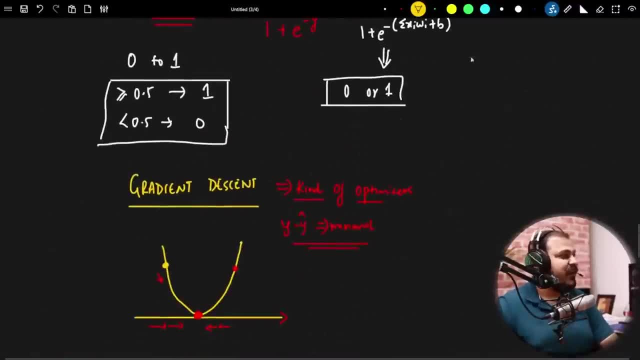 Now what all things in deep learning will be there? Very much important. One thing: you'll learn about ANN. You'll learn about CNN. You'll learn about RNN. Everything works on forward propagation and backward propagation. You'll learn about object detection. 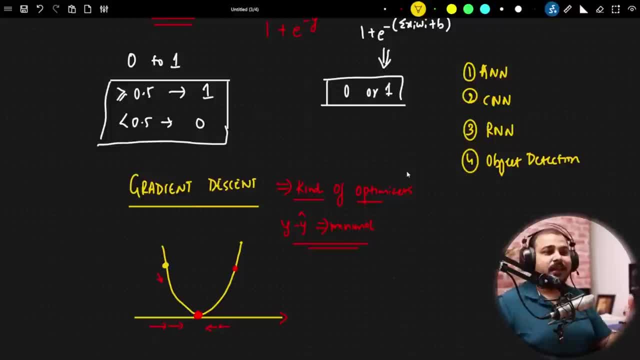 Object detection. Everything works on forward and backward propagation with different optimizers, right, And we don't have to even do 1,000 times Within 10 times. also, if the neural network is able to train, it is able to train right. 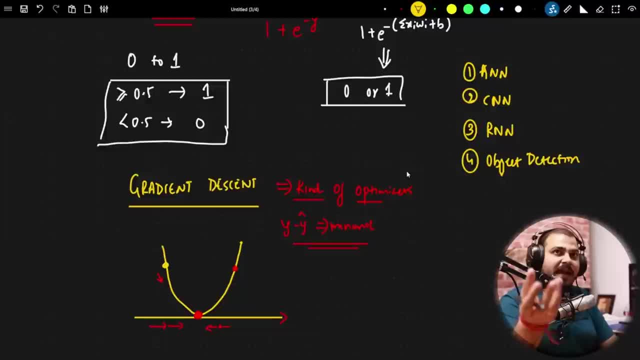 Okay, let's take one example. I've shown you a new kind of species. Let's say, I've shown you a new kind of flower. Suppose you don't know the flower name. Okay, today I will train you. okay, this flower is black rose. let's say: 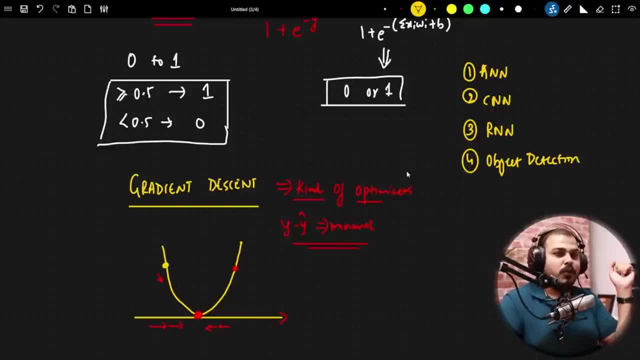 Okay, so you'll just remember. okay, he told black rose. Tomorrow I may show you again that particular flower that you may again not be able to remember. If tomorrow, as I say you that, okay, this is black rose, then second day, okay, you'll get more confident. 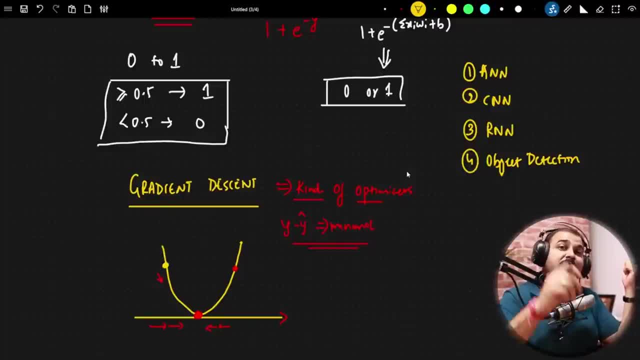 On the third or a fourth day, whenever I show you that particular flower, you will be saying that: okay, this is black rose. On the third or a fourth day, whenever I show you that particular flower, you will be saying that: okay, this is black rose. 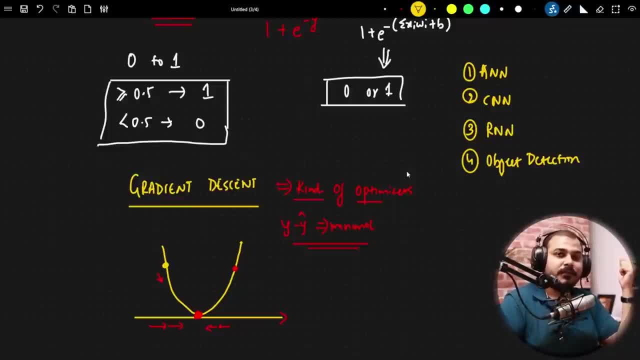 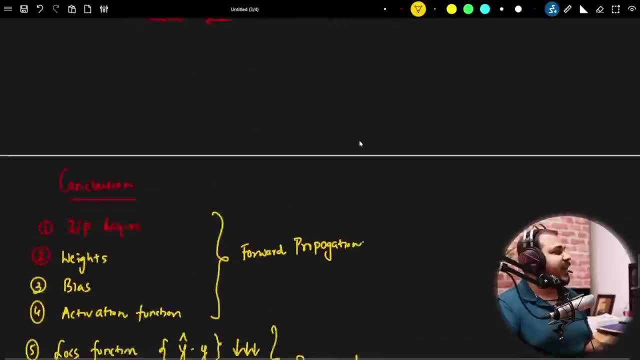 it is a black rose, and that is how we train a neural network, like we train a human being. now let's understand. how does a multi-layer neural network look? that was a single layer neural network, right. a multi-layer neural network will have a lot of inputs. let's say i have inputs over. 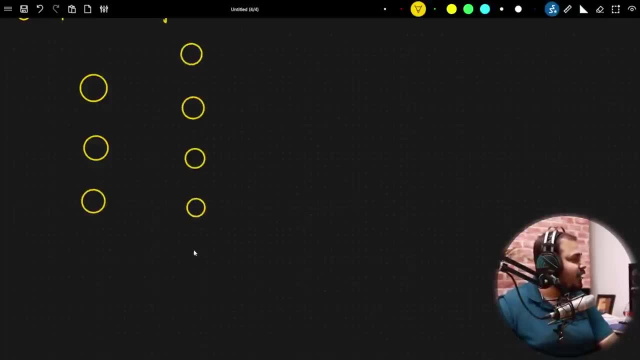 here in the hidden layer i will be having so many different, different neurons. right over here again i may have any number of neurons, not limited to anything, and here in the output layer also i may have multi-class classification problem. okay, and this all will be combined together. let's say i'm 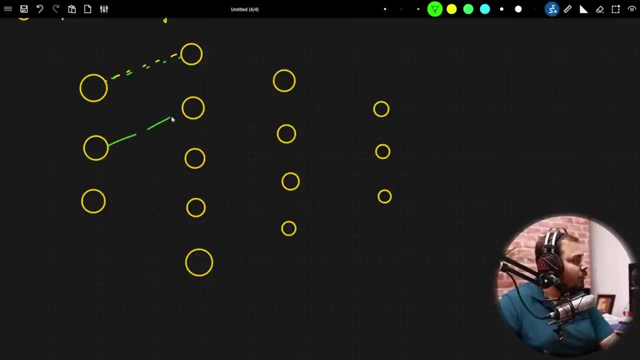 going to use green dots. this all will be combined together. right, this all will be combined together and this is nothing but a multi-layer neural network and it is going to basically just do the same process, whatever i've taught you in the single layer. nothing different in every. 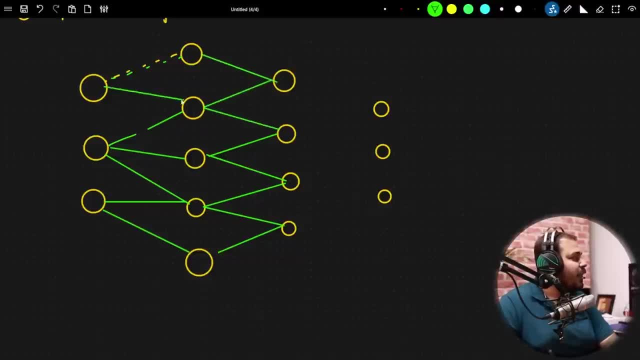 layer bias will get added. everything is almost same. everything. nothing. i'm not hidden anything, any concept with you now. everything will get connected and everything will there. just for case of multi-classification, a different types of activation function may get used. a different kind of loss function may get used. that's it okay. so this exactly is called as a multi-layered. 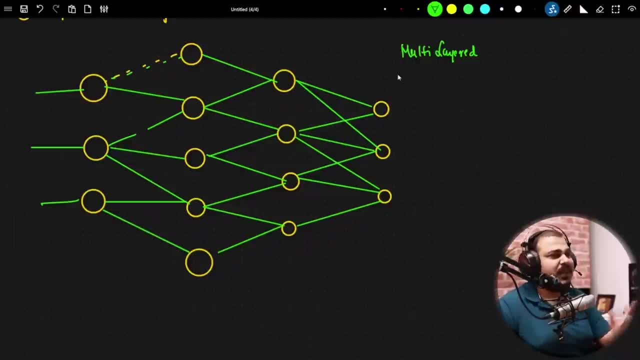 neural network. it will not be only two hidden layers, any number of hidden layer, so multi-layered neural network. and finally, this is my output. okay, so this is my output layer. this is my hidden layer two. this is my hidden layer one. this is my input layer. that's it. and just imagine one hour we have. 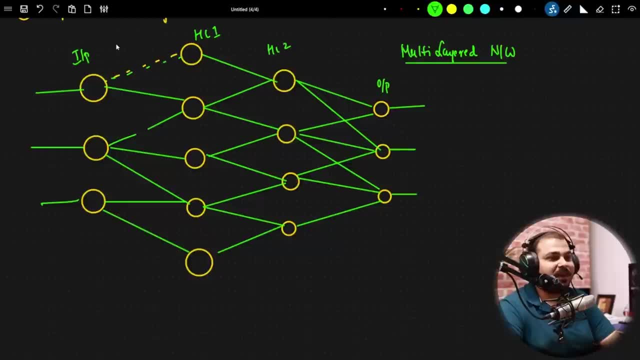 covered so many things. if you know this much for the interview also, then also you'll be able to crack the job with some practical implementation, because they will not go inside that. how, how, uh, mathematical equation will be there in optimized, and all that just for our learning interest. we learn those things. 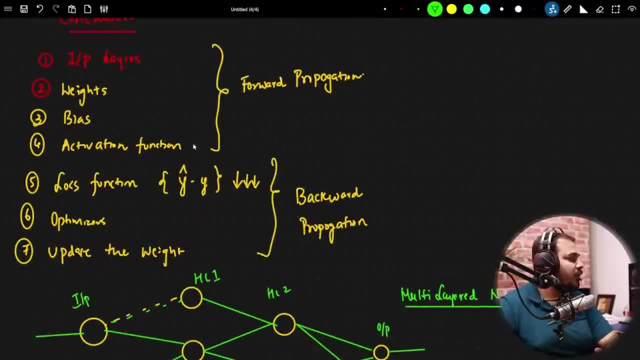 now. what we will do is that tomorrow, uh, we will understand about in-depth activation functions. what are the different types of activation function will also be understanding loss function tomorrow. i'll try to cover this too. how to updates the weight and optimizers will be covered in day three and in day two we'll try to cover this two: how to updates the weight and. 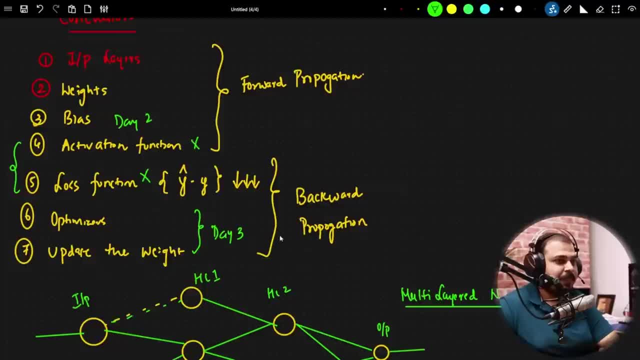 optimizers. we'll be covered in day three and in day two we'll try to cover this. two techniques we'll. in day three, we'll also see practical examples. okay, and those practical examples will be super important because by that you will be able to learn ann anyhow that you want. 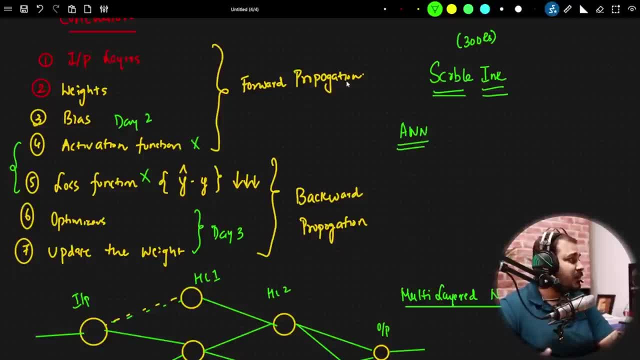 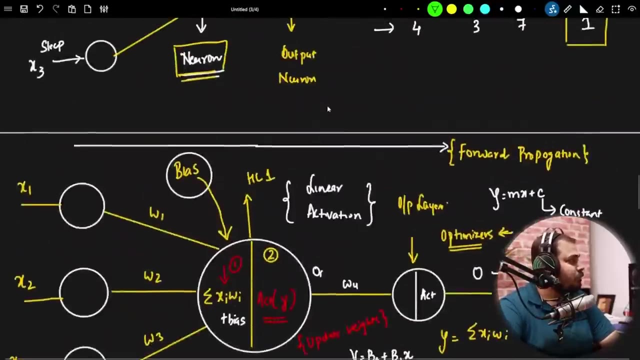 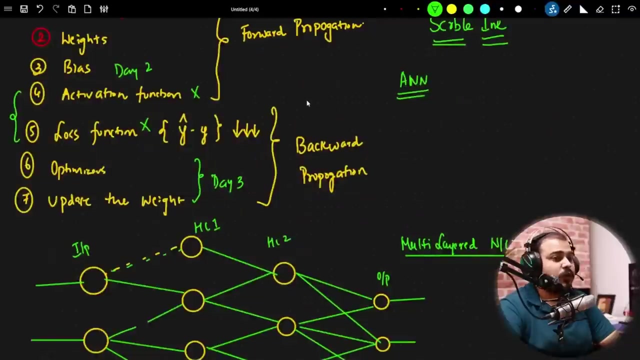 okay. so why there is a need of neural network? it is basically to mimic the human brain, how our human brain basically gets trained. we also want to train our neural network like that. okay, our machine learning applications or any applications like that, okay, okay, perfect, uh, now, uh. okay, there is also one concept in uh: back propagation. you know there. 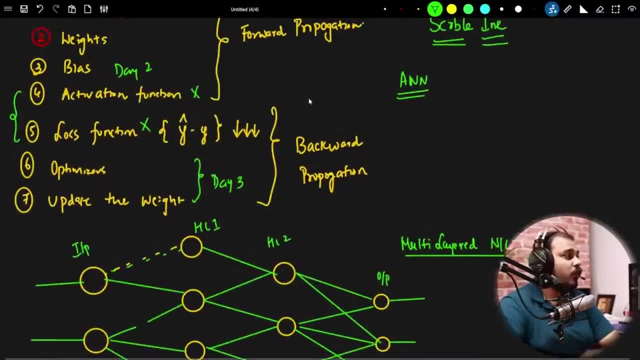 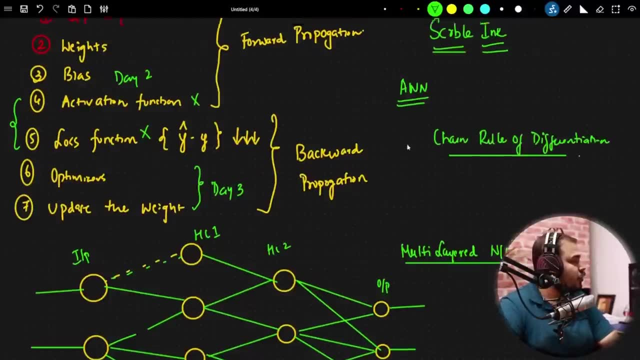 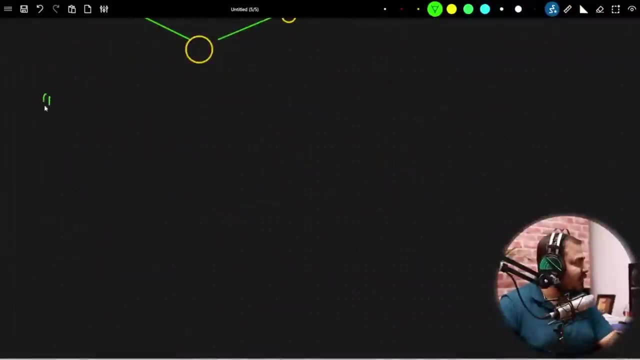 is something called as uh, derivative or chain rule of differentiation. so that thing also. tomorrow i'll cover chain rule of differentiation. so i hope you have understood this video. see what are things we are going to learn. first of all, we are going to learn ann. okay, already we have started this. perceptron is a concept of ann. 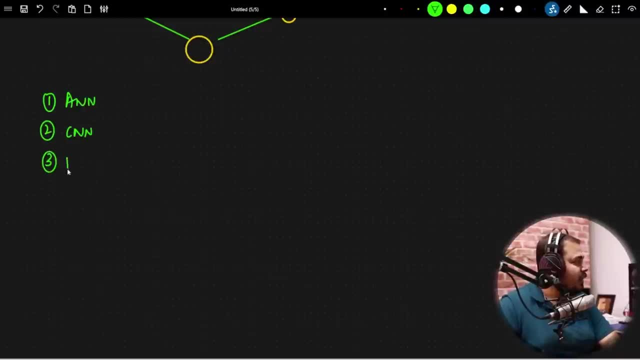 then we'll go with cnn, then we'll go with rnn and then probably we will try to close some example of object detection. but i need another seven days to complete nlp. okay, nlp introduction will be done over here. okay, but nlp completely in depth, i will take another seven days to 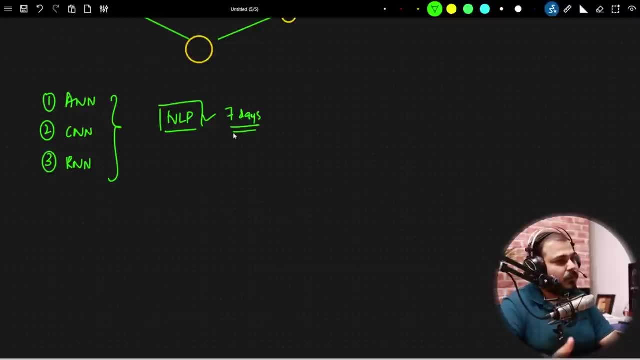 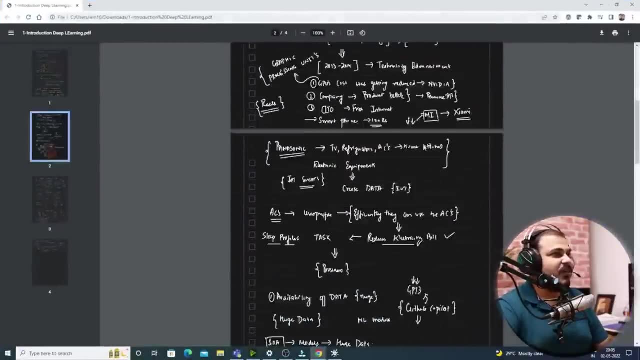 complete it okay, so that we will plan it probably in this month or in next month. okay, see, this is one of the session that i had taken- the deep learning- and this is how the material looks like. so that's it from my side, and, yes, keep on rocking, keep on learning, i will. 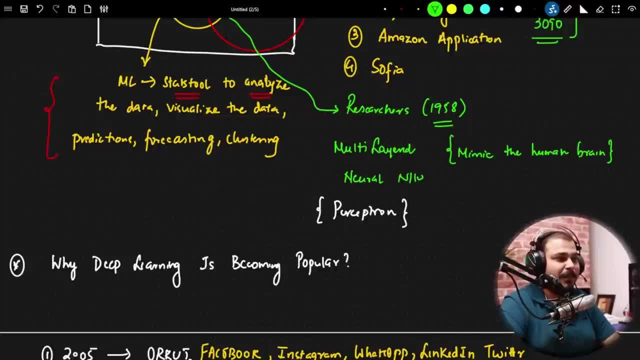 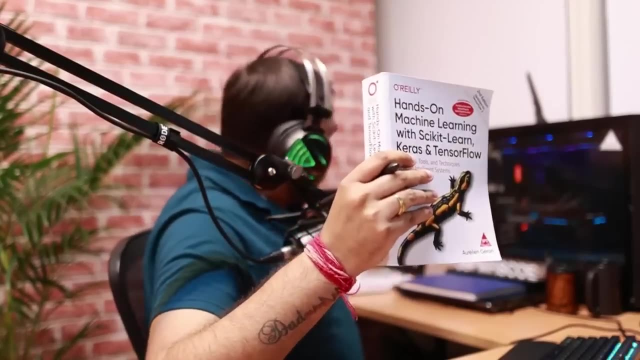 see you all in the next session. have a great day. thank you, vandal, bye, bye. okay, and yes, about the books. i do refer this book. uh, let me show you the book that i refer. this is the book that i refer. okay, apart from this, i also have one more book. so these two books. 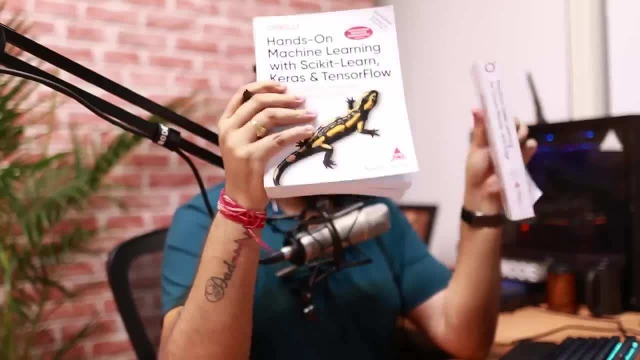 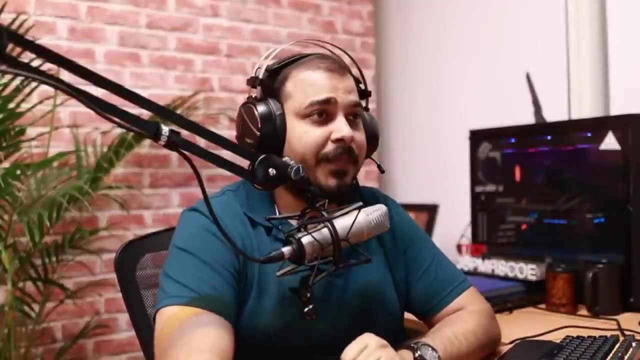 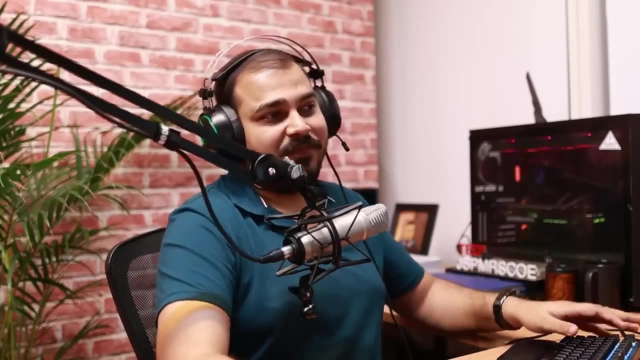 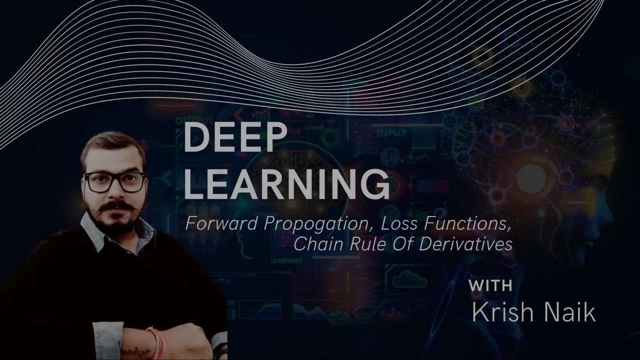 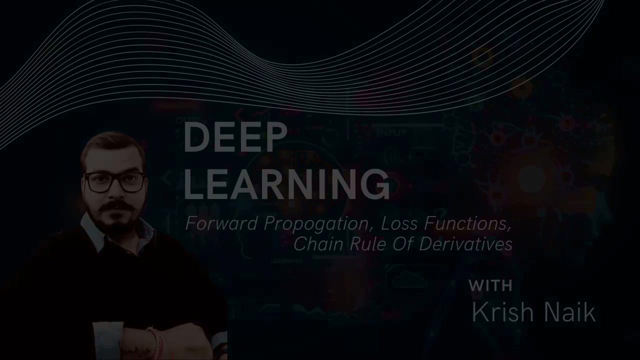 i usually refer. okay, so i've already completed anyhow these two books and probably we will be covering many books as such. okay, this is the plan and, yeah, please make sure that you share it everywhere. okay, thank you everyone. have a great day. thank you, bye, bye, so let's continue. 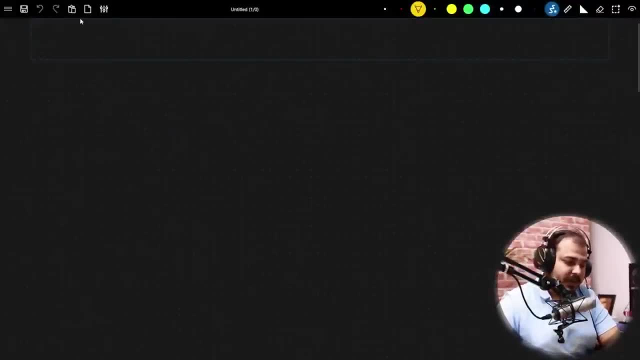 So let's continue, So, let's continue. Uh, So today is the day two. I've cleared the screen and let me write. today is the day two of deep learning session. So, deep learning, and what is the agenda that we are going to cover today? 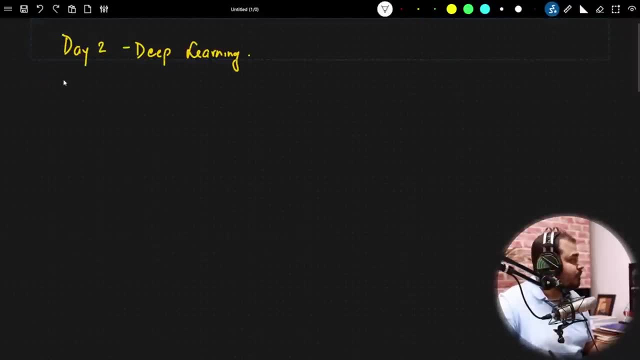 Number one, the agenda. we'll go again. we'll get an idea about forward propagation. Then we will understand. before understanding the loss functions, we will first of all understand chain rule of derivatives. We'll understand this and then we'll also be getting an idea about many things as such. 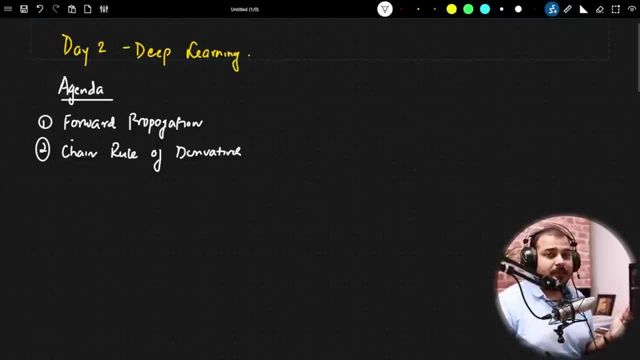 about chain rule of derivatives or differentiation, which is a very important topic. Then, after completing chain rule of derivatives, we are going to understand a very important problem, which is called as vanishing gradient problem. Okay, so we are going to understand about vanishing gradient problem. 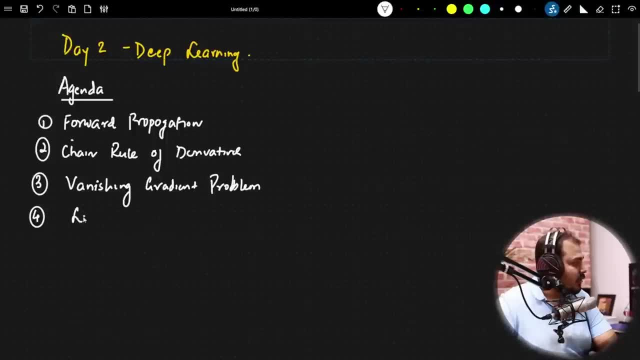 The fourth thing that we are going to understand is basically about loss functions. What are the different types of loss functions? So in this session, we are going to cover all these things, okay, And we are going to cover in an efficient manner wherein I will probably write each. 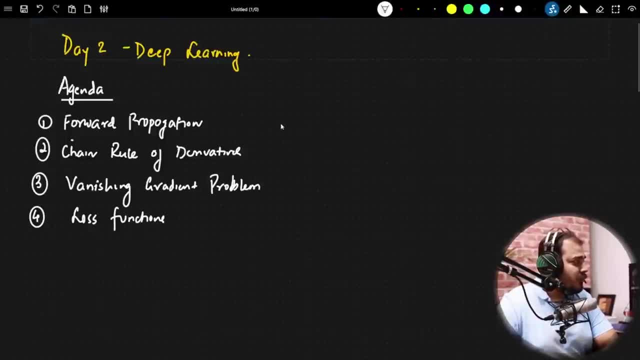 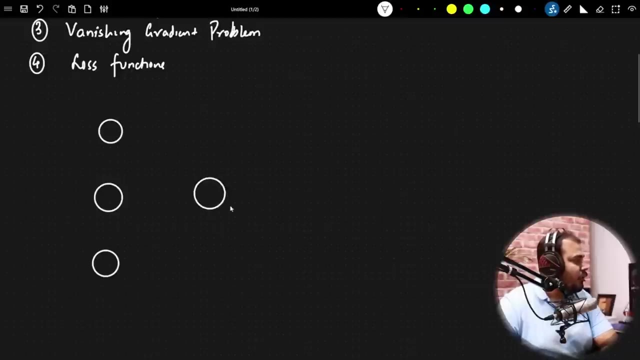 and everything in front of you, and we'll try to complete this in two hours of time, Okay, So let's go ahead, and let's first of all again go back to the basics, or whatever we think we learned yesterday. So suppose this is my neural network with three inputs, and I have one neuron in the 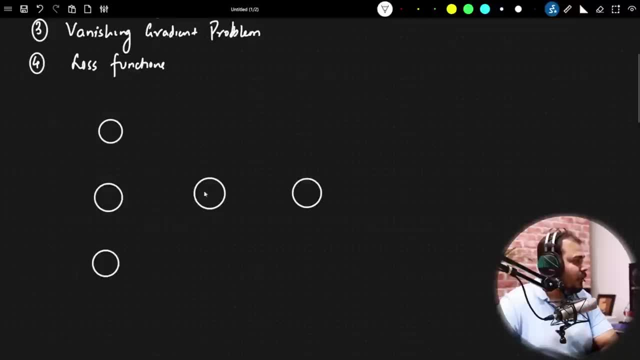 hidden layer and finally, one neuron in the output layer. right, So this becomes my input X1,, X2, X3,. let's say This is my X1, X2, X3. And this in further will get connected to our output. 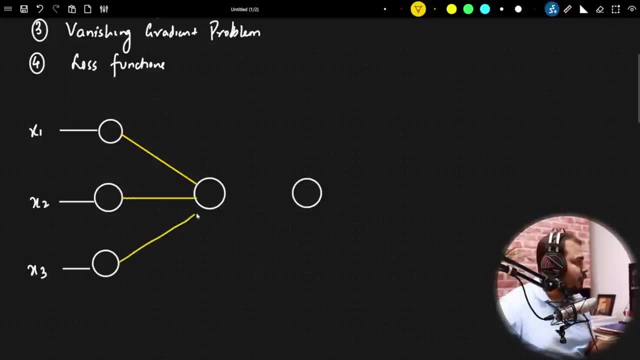 And this in further will get connected to our hidden neuron. okay, And finally, this goes to my output layer. Okay, so this is my hidden layer one, Hidden layer one, And this is my output layer. Just to add one more thing: we have something called as bias. 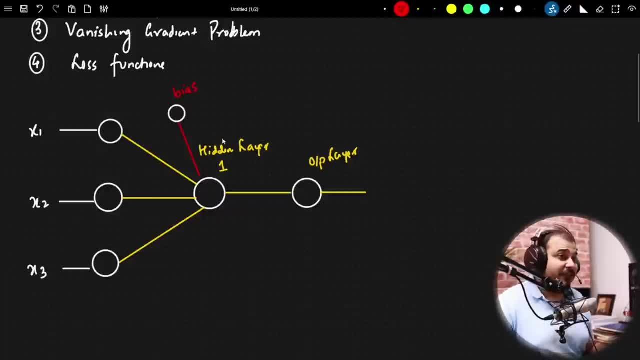 Bias also gets added, and bias also gets added in each and every hidden layer. so, and then what we do? we get basically y hat, and then we define our loss function. my loss will nothing be, it will be the difference between y and y hat, and our main aim is to reduce this loss value. so what we do: 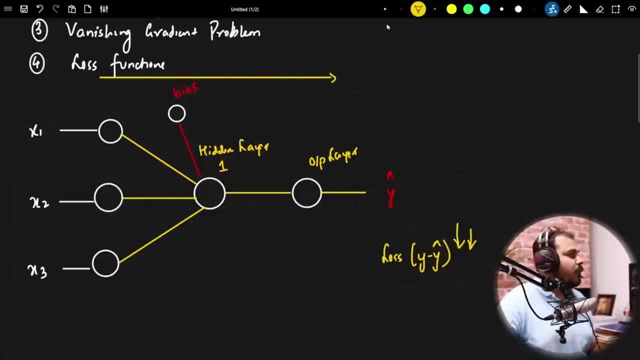 first step is basically the forward propagation. in the forward propagation, we assign different weights. these weights are assigned randomly and there are various ways to assign the weights, which we will be having a look onto it, okay, and then, finally, i go to w4, which is another weight. 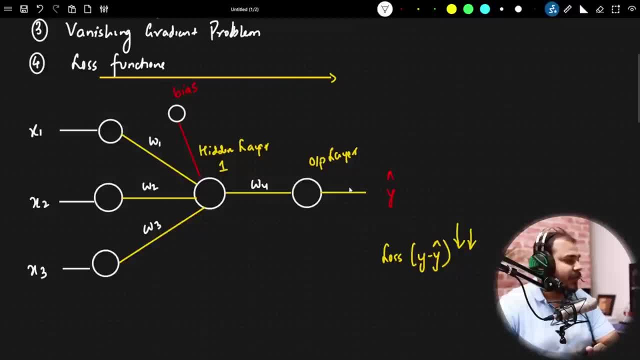 over here. whatever output is basically coming from here, it will go over here and finally it will go to the output layer. this inputs are basically your data points, which i have already discussed yesterday. okay, and over here, two things basically happen in every neuron. first i will say: 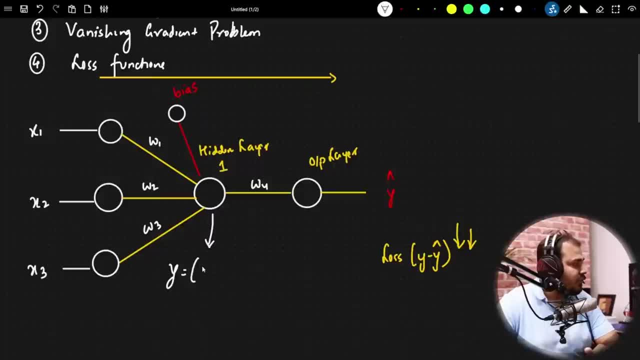 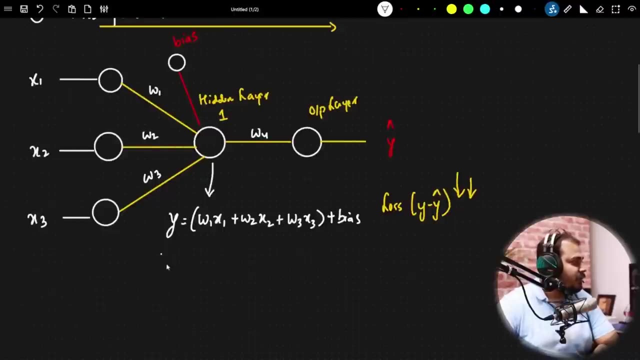 y is equal to, it is nothing but summation of w1, x1 plus w2, x2 plus w3, x3, and then a bias gets added over here, and after that we have something called as an activation function will get applied on top of it, which i will specifically write as z. 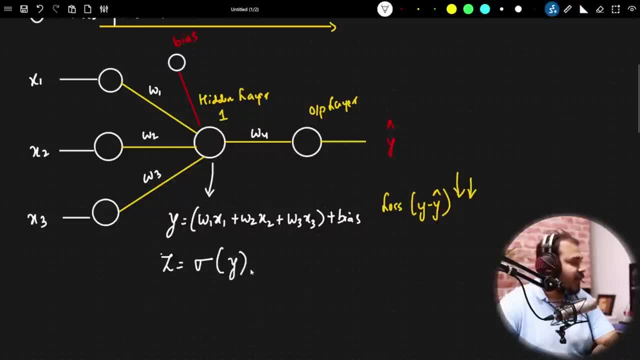 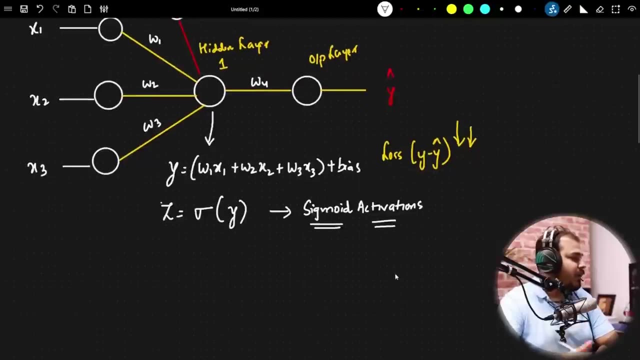 so let's come consider. this is the symbol that i'm using as an activation function. one activation function that we have already seen is something called as sigmoid activation function. we will also see different kinds of activation functions today. okay, sigmoid activation function. main aim is that we try to convert this y value. 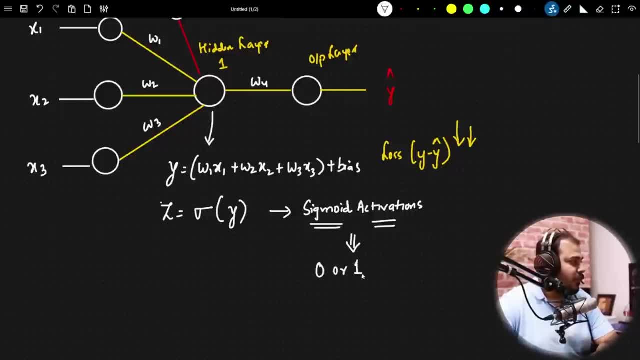 as 0 or 1. okay, so whenever it is greater than or 0.5, we get it as 1, if it is less than 0.5, we get it as 0. so till yesterday, we had discussed all these things. uh, this y can also be given by: 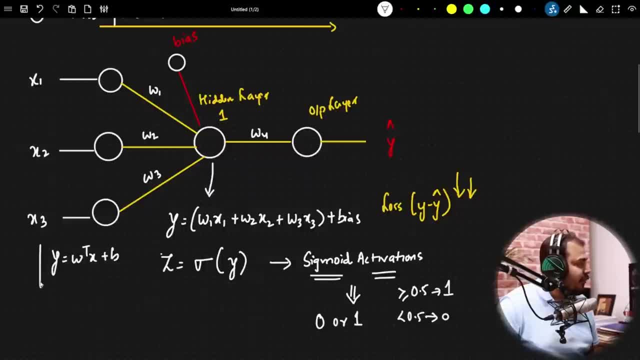 another symbol, which is nothing but w. transpose x plus b, okay, and this is nothing but a- linear in short. but because of the activation function, we basically get non-linear properties. okay, we are able to solve non-linear problems. so till here, we have basically discussed. okay, all the resource link will be given in the description. perfect, now, uh, let's go ahead and. 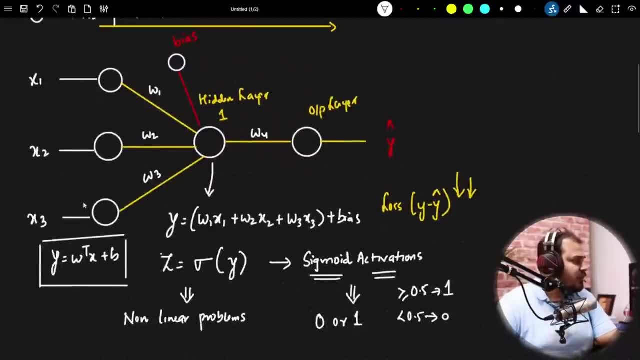 let's try to understand. i hope everybody has understood. this specific thing usually happens in the forward propagation right. so this is what happens in the power forward propagation in every layer, right in every layer. the forward propagation basically happens right now, once i get my output, that is, y hat, and then we calculate. 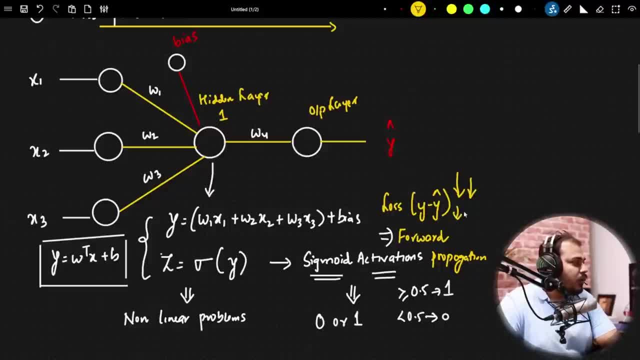 our loss function. now, what will happen in order to reduce the loss function? how will we be able to reduce the loss function? okay, that is what, uh, we are going to understand now in in order to reduce the loss, we really need to update this weights, right? we really? 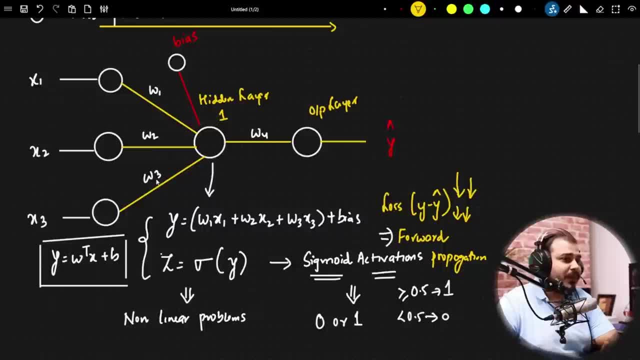 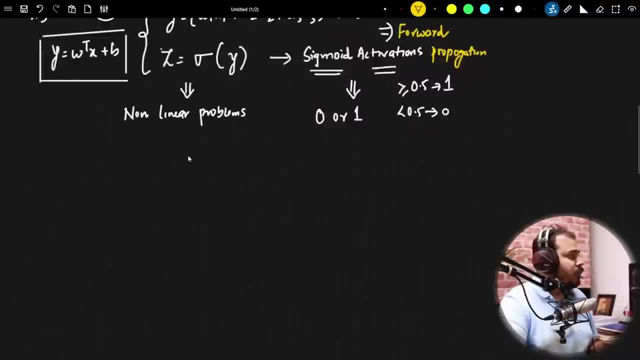 need to update this way and this updation of the weights usually happen in the back propagation. okay, and how the weights are getting updated. that is what we are going to see. so let's go to the back propagation. second step, which we are specifically going to discuss about back propagation here, in this back 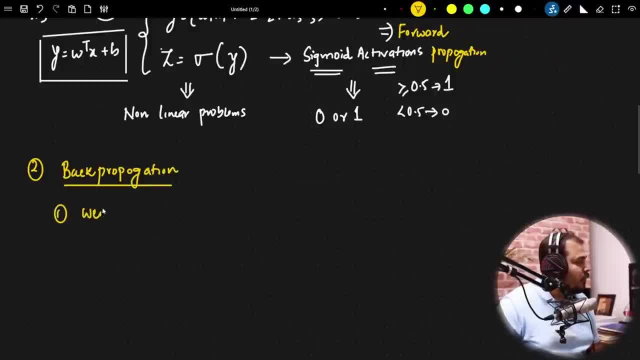 propagation. we will see two things. one is weight updation formula, weight updation formula. the second thing that we are probably going to see, uh in the weight updation formula, is that: uh, what is the chain rule of differentiation? chain rule of differentiation. so this is what we are. 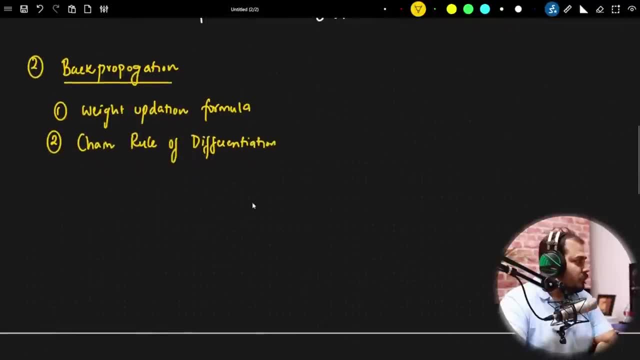 going to cover this, both the topics we will be covering now. let's let me again define this. entire things now over here. let's say i have three inputs and one hidden neuron and one output neuron. right, this all will be interconnected right now over here. this is my input, this is my weights: w1, w2, w3. 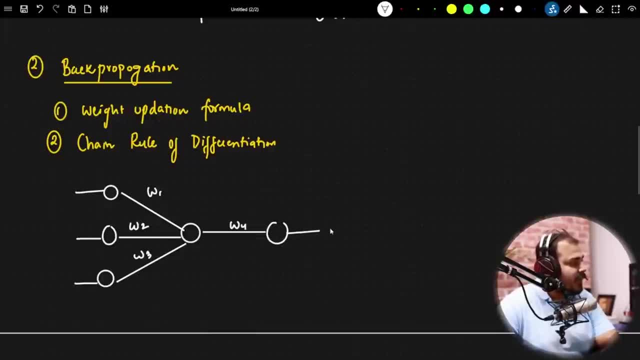 let's say this weight is w4 and finally i get my output. this output is nothing but my y hat. right, then i calculate in my loss y minus y hat and my. in order to reduce this loss, what we do we do, we have to update this weight. so the weight updation formula, and that is where optimizers 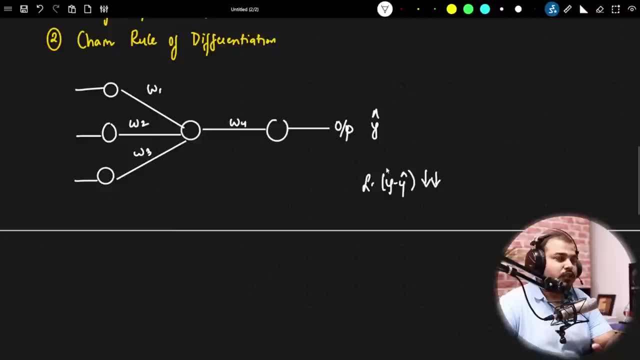 will also come. okay, optimizers will be very much useful when we are actually doing chain rule of differentiation. now suppose i want to update this weight w4, how this weights gets updated. forward propagation: i hope everybody is clear right now. in the backward propagation the main aim is that we have to update this weight. so here i'm just going to write backward propagation. 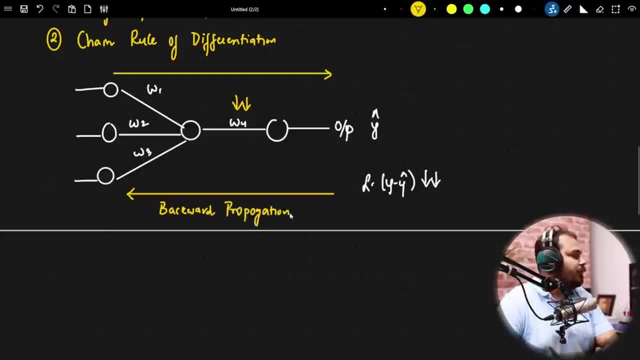 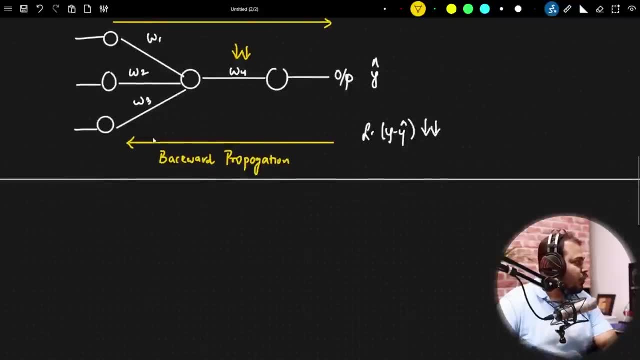 okay, now in the backward propagation we need to update weights w4, w1, w2, w3. now how this weight updation will happen. so here i'm going to write the weight updation formula. weight updation formula. the weight updation formula is very, very simple. i will write a generic formula. i'll say w new: 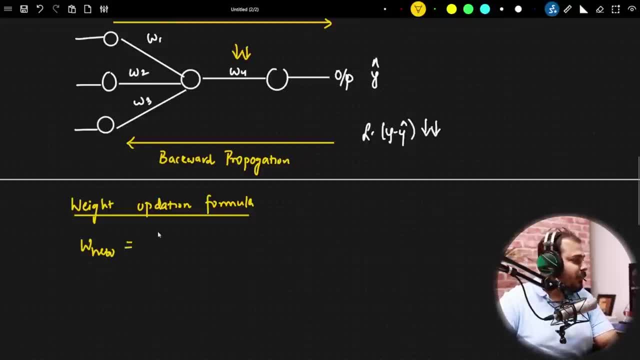 w new basically means the weight that is getting updated. there's nothing but w old. the weight that's wold basically means the previous weight, because in the forward propagation this weight will have a different value and when we do the back propagation we need to update this. so previous. 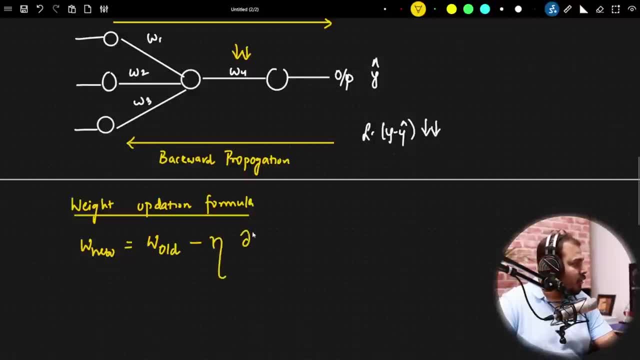 weight, whatever it was, minus learning rate, derivative of loss with respect to derivative of wold. so i will be discussing about each and every parameters over here. this parameter that you see is nothing, but it is a learning rate. i'll talk about the importance of learning rate. 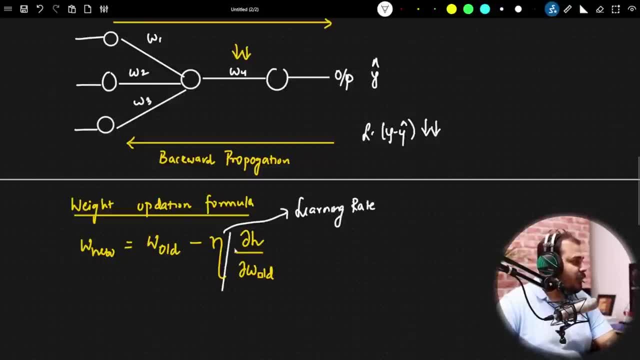 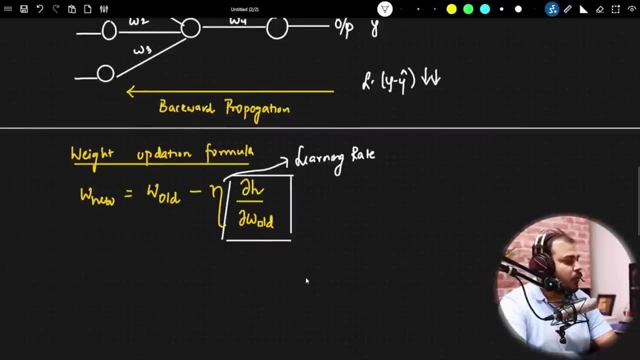 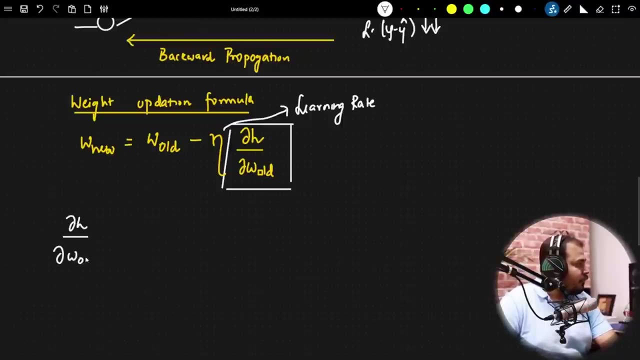 just in some time. but the first important thing that we really need to understand is this value. okay, so what is this derivative of loss with respect to derivative of wold? okay, so this derivative of loss with respect to derivative of wold is nothing, but it is basically calculating. 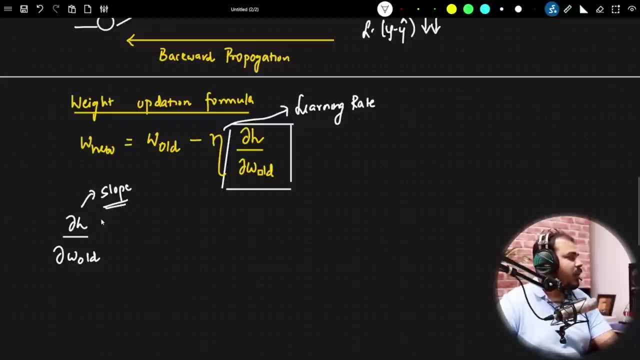 the slope. okay, we are basically trying to calculate the slope. now, when we are calculating this slope, i hope everybody has learned linear regression right. in linear regression also, what we do, we update, we update the weights or coefficient, right. so i hope everybody have learned in the simple linear 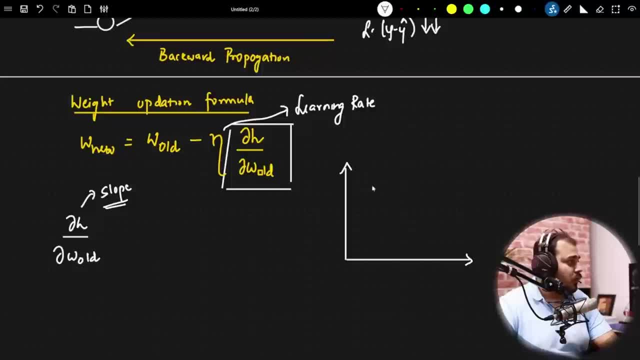 regression. i've also made live sessions on machine learning also for the same. now, in this case, what happens is that we basically get this kind of curve, and this is basically called as gradient descent. this gradient descent is nothing, but it is the graph with respect to weight. 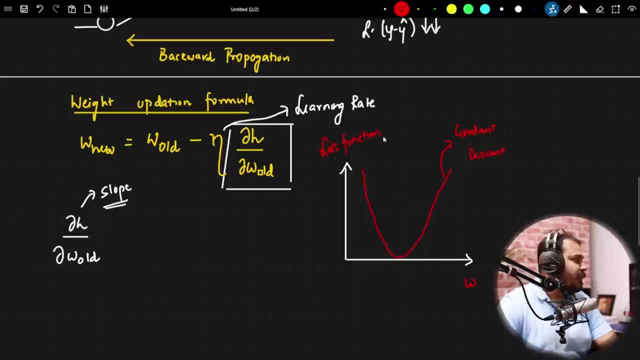 and the loss function. okay, weights and the loss function. now in this graph, this point that you probably see. this point is basically called as global minima. this point is basically called as global minima. when we are training and updating the weights, we definitely have to come to this. 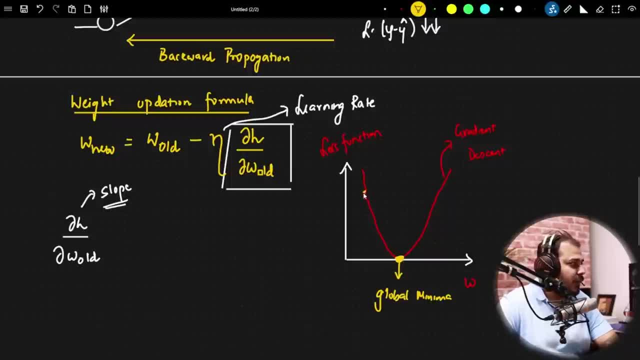 particular point. okay, anyhow, it may be at this point, or it may be at this point, but anyhow, we to come into this particular point now, why this formula will definitely work. that is what we are going to understand first of all. okay, suppose let's say that i have one point over here initially. 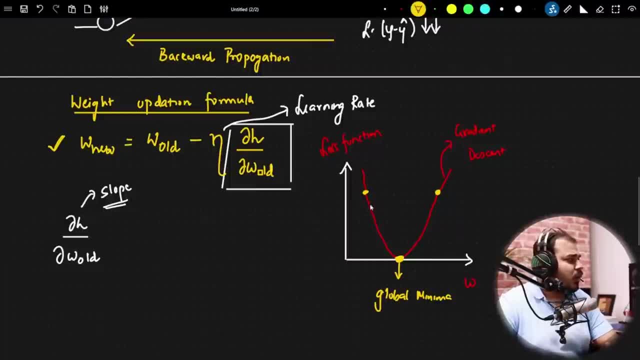 let's say, with respect to w, any weights, the previous weights, i got a loss function which is coming at this point. okay, here i've. i've actually drawn a 2d diagram, but this usually looks like a 3d curve. okay, 3d curve. just imagine that, uh, there is a mountain and we have inverted. 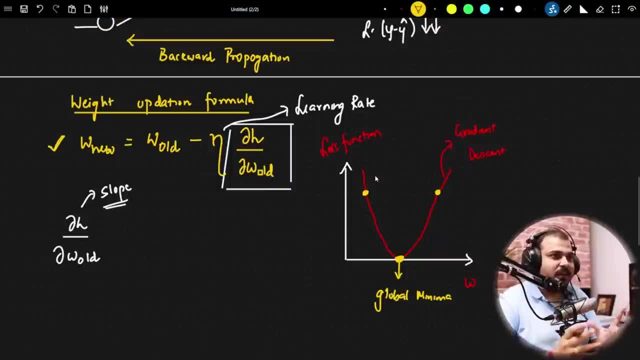 that mountain right. so in that way this will be like a 3d curve, okay, and our main aim is basically to come to this specific point. okay, now, during this 3d curve, let's say that first point comes over here now, when we apply this derivative of loss with respect to this weight, at this specific 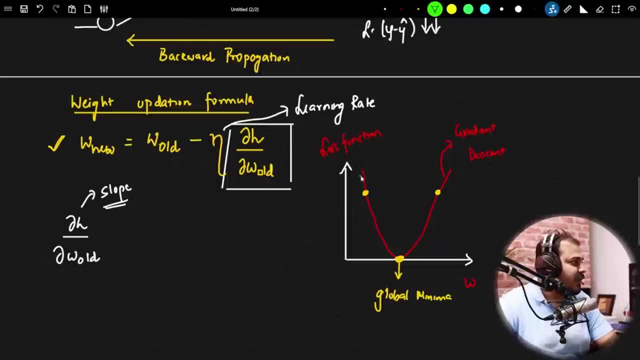 point. in short, what we are actually doing is that we are basically creating a tangent line and then, basically, Based on this tangent line, we basically find out the slope, Slope. we actually find out like this: Now, this is basically my loss function. 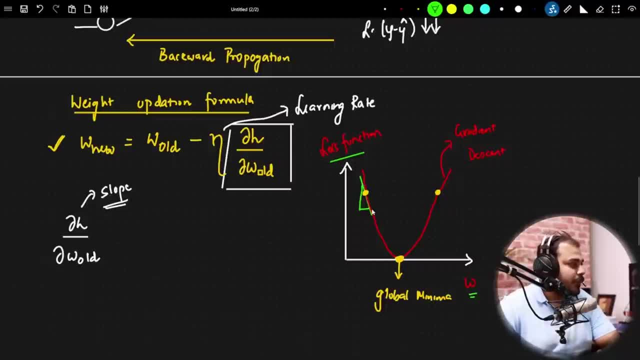 This is my weights. okay, Now, when we try to find out the slope, now, the first thing we need to understand whether this is a positive slope or negative slope. And how do you determine this? Obviously, through calculation. we will definitely get it as a positive or negative slope. 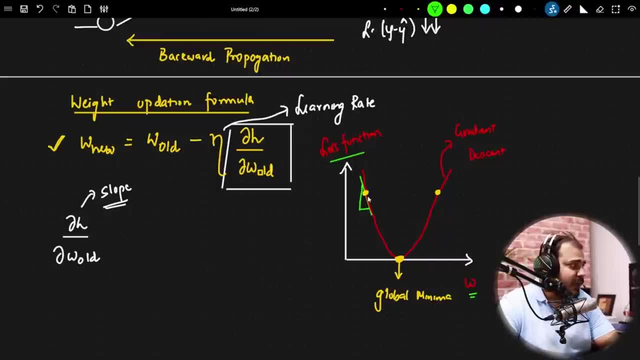 But one very important thing that you should definitely be knowing is that whenever the right side of the line, see whenever this right side of the line is pointing downwards, okay, Whenever this right side of the line is pointing downwards, then we should basically understand that. 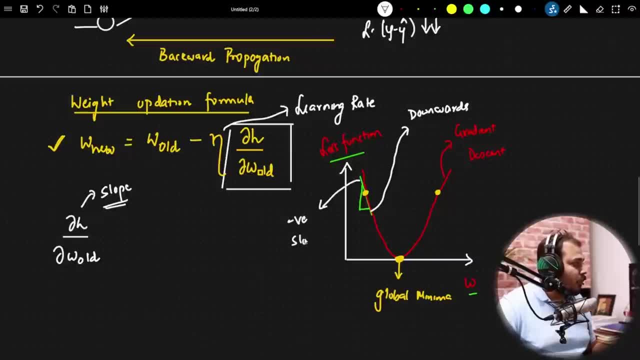 this is a negative slope. Okay, negative slope. Now, when it is a negative slope, suppose, if I go and point this weights over here, right, this is my weights Now. my main target should be that I should be increasing this weight. 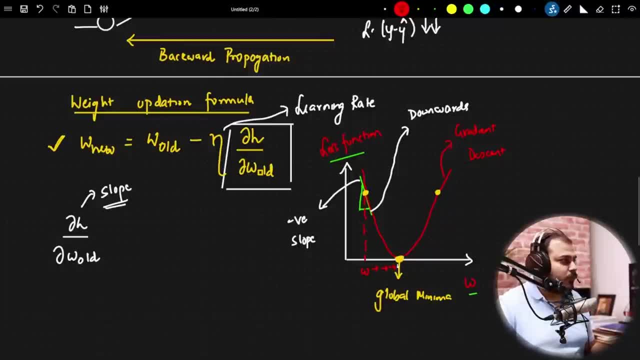 so that I move to this global minima. okay, I should be moving to this global minima Now. in order to do this, I have to increase the weight And in this particular option, weight updation formula, either I can increase or decrease the weight. okay. 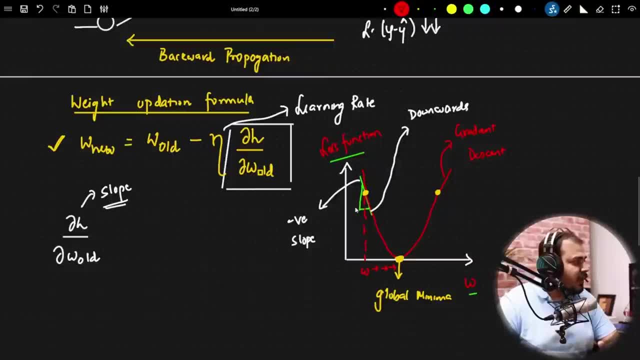 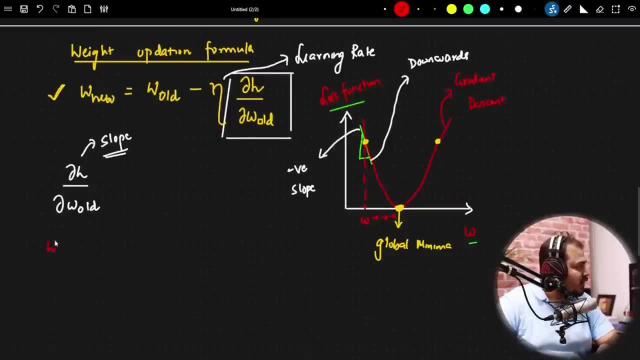 I can either increase or decrease the weight, So suppose in this particular case I get a negative slope. Negative slope basically means some negative value. So my weight updation formula will now become- see what it will become- W. 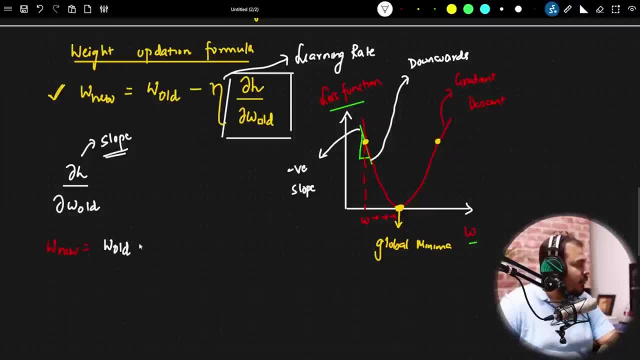 W new is equal to W old, minus learning rate of some negative value in the case of negative slope. And in case of negative slope, you have already seen that I have to increase my weights. I have to increase this weights to come over here, right? 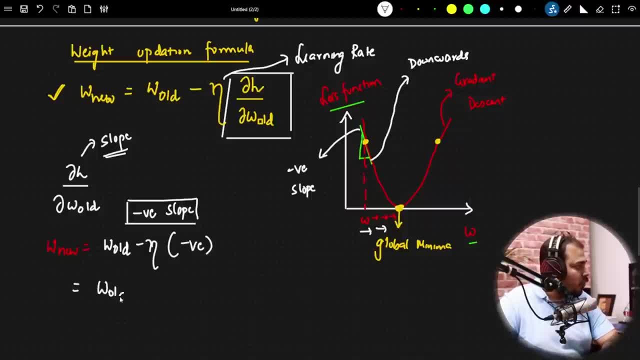 That is what I am actually looking at Now. what will happen W old negative into negative will be a positive value, right? This positive value will be multiplied by learning rate, multiplied by some positive value. So here you know that, at the end of the day, 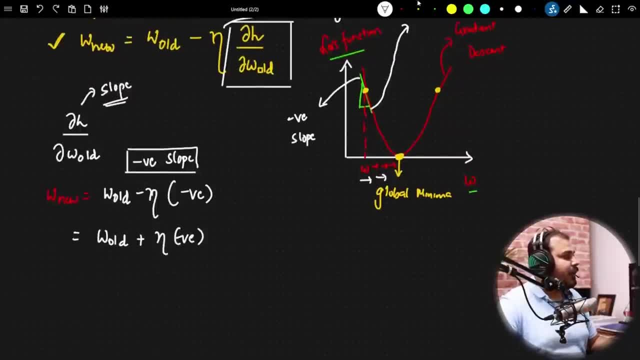 what will happen? My W new. let me write it down over here: My W new. so this will be a positive value, right? My W new will be always greater than W old, because I am adding the previous weights in this particular case. 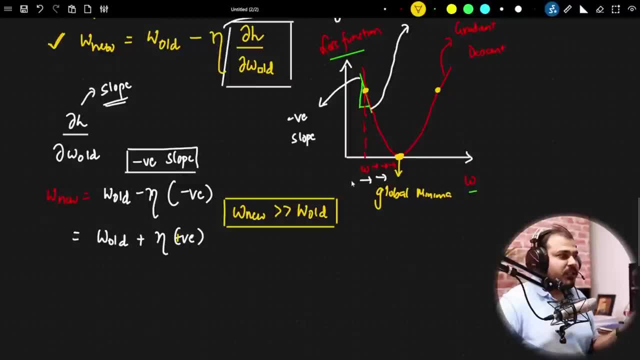 So whenever we have a negative slope by this specific equation, it will definitely work, because we are trying to increase the weights and that is the reason why W new, when we are applying over here a negative slope, then it will become minus into minus. 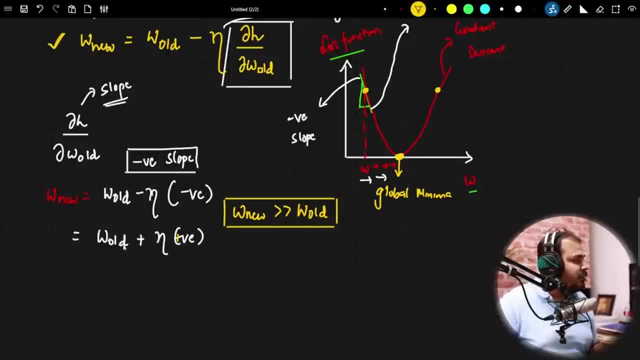 which will be nothing but positive. And when I probably add up this value, my W new will definitely be greater than W old. Okay, So definitely with the help of a negative slope, I am able to increase the weights, which is basically what I want over here. 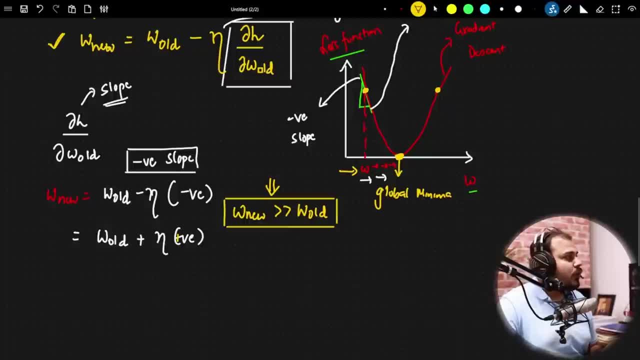 Let's say, in the case of this slope, suppose in this point I go and draw a, I draw I, I go and draw up a slope like this. Now, in this particular case, what will be my slope? This will basically be a positive slope. 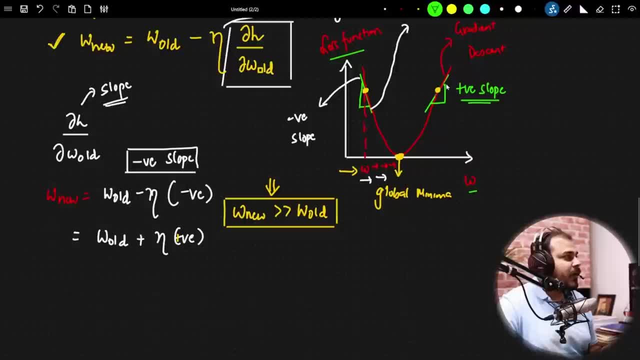 How I'm saying because just see the right side, right hand side of the line, It is pointing upwards. Here it was pointing downwards And if you do the calculation also of this particular slope, it will be a positive slope. Now, in this particular case, 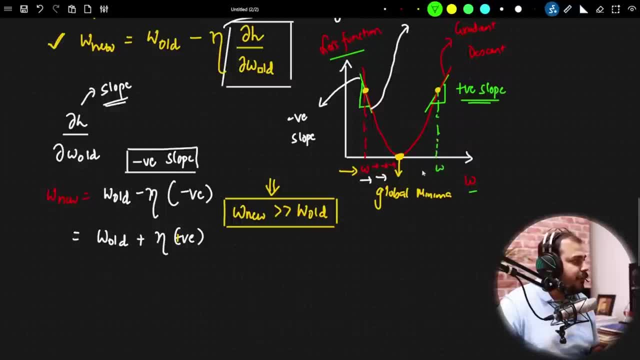 if I go and probably plot this W over here, I, in order to come over here, I have to decrease this weight. I have to decrease this weight. Okay, Now what will happen? The again formula see in this particular case. 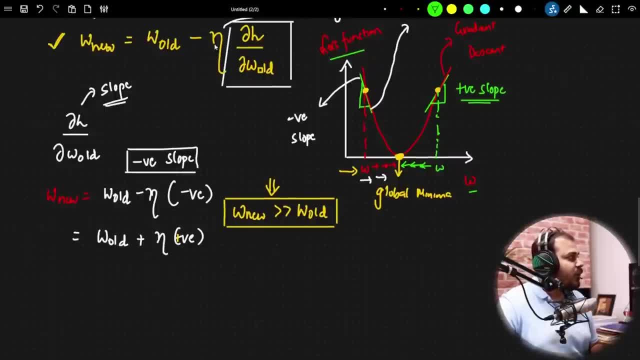 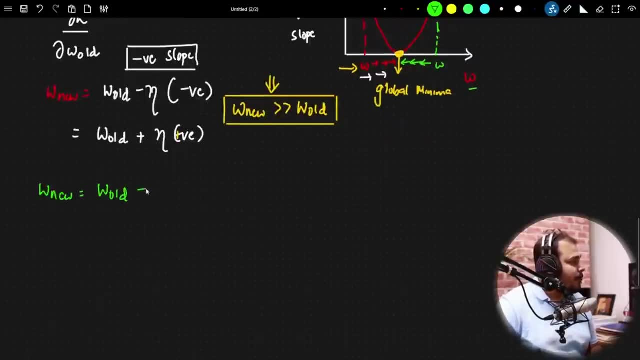 I'm getting a positive slope. Okay, If I put this positive slope in this equation, what will happen Now? my W new will be W old, minus learning rate of some positive value, Right Of some positive value, And when I probably subtract this with a positive value. 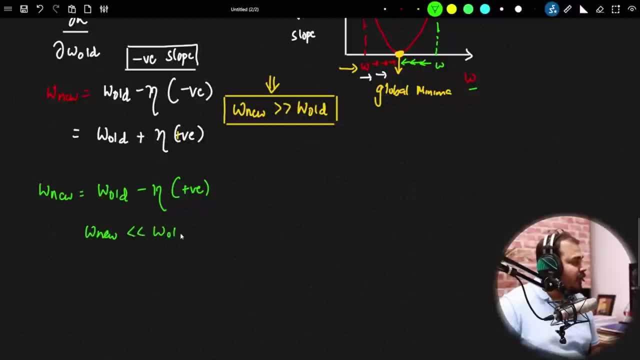 what will happen? W new will begin it less than W old. right. This is what we. it is proved. So what was our main aim? with respect to weights, I should be able to increase or decrease the weights, And that is what I'm able to do it over here. 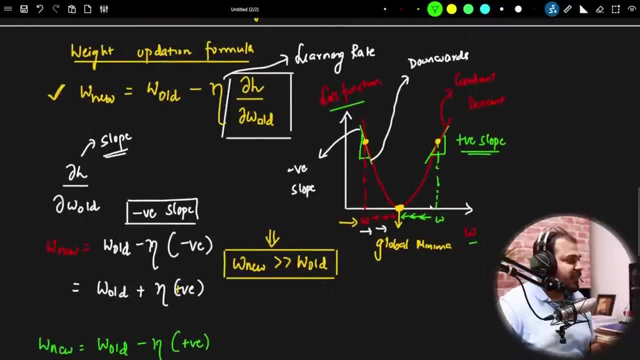 Right, So through this, through this, uh, this is basically a gradient descent, Uh, and this is basically happening from the loss function. I will discuss about all the loss functions, just going forward. but just understand that in linear regression also. 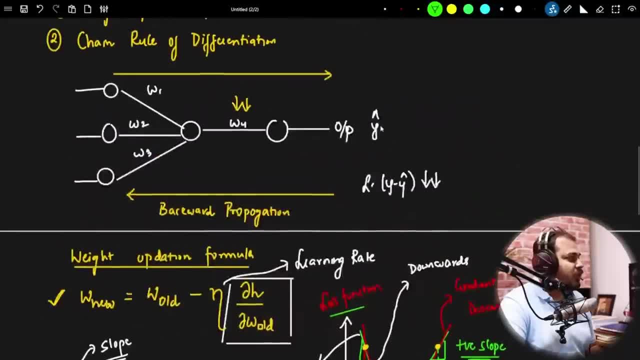 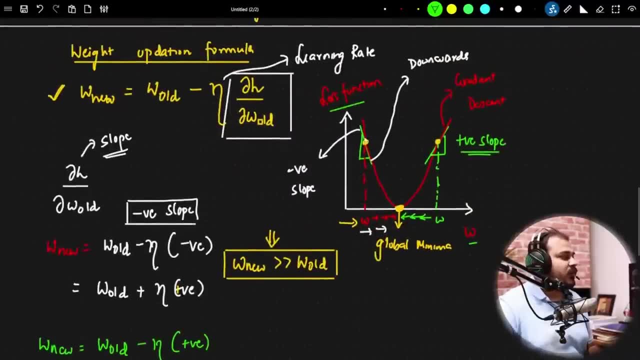 whenever I plotted by using this loss function, which I have actually used over here, that is, Y minus Y hat whole square. at that point of time you'll be able to see if I plot with respect to weights and loss function, I'll be getting this gradient descent and for back propagation. 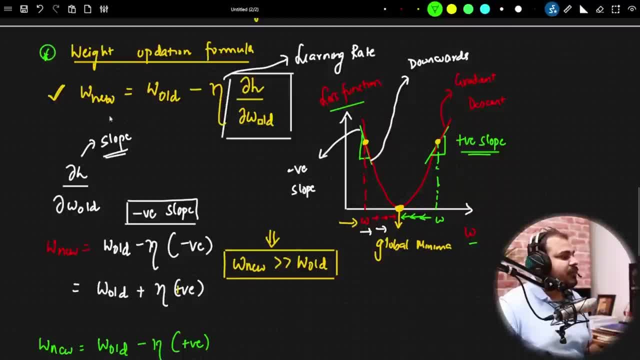 how I'm updating the formula. This is the updation formula, whereas W new is equal to W old, minus learning rate of DL, uh derivative of loss with respect to derivative of W old. But now, what is the importance of this learning rate? 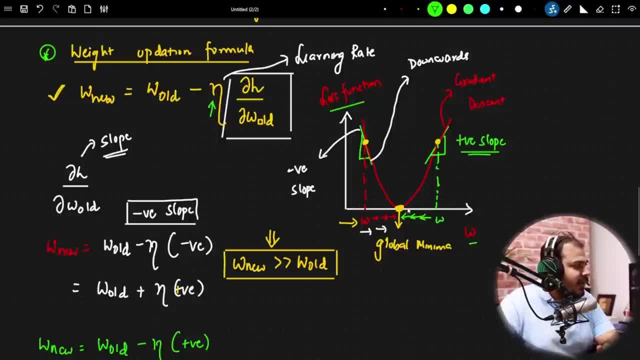 We need to understand Now. see, guys, I need to come to this global mini now. my main aim is basically to come to this global minima and in order to come, I can take larger step also, I can take smaller step also. 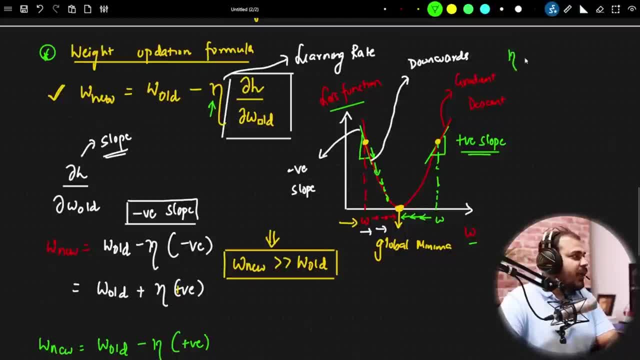 right. It is always a good practice that our learning rate should be a small number. If it is a small number, we will be slowly converging into the global minimum. Okay, We will be slowly converging into the global minima, If I probably take a larger number. 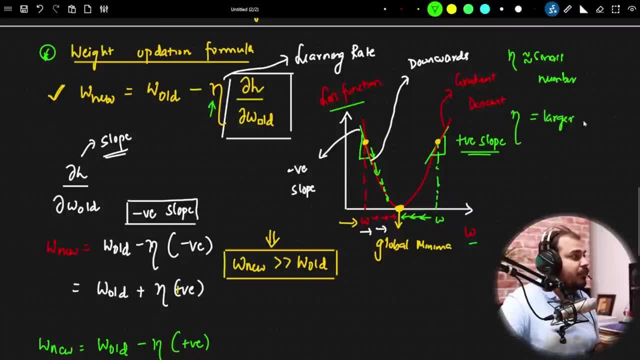 what happens if my learning rate is a larger number? then it may be a problem sometime because my my, this point, which points, will be jumping here and there And it it may be a situation that it may never come to the global minima. 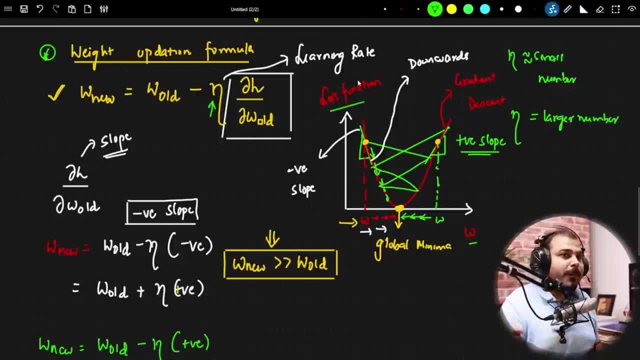 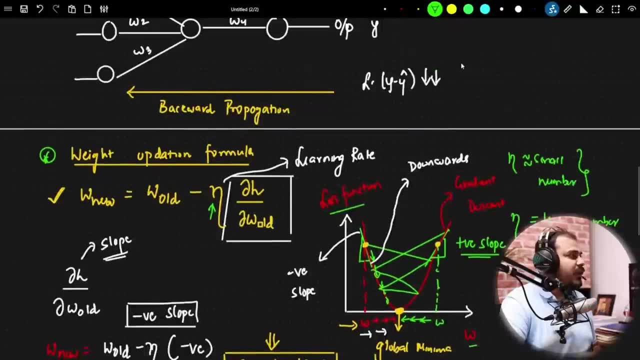 It will be jumping here and there, So it is always a good practice that you take a learning rate as a smaller number. The learning rate that I usually take, or any probably researchers usually take, is somewhere around 0.01, or you can also take 0.01,. 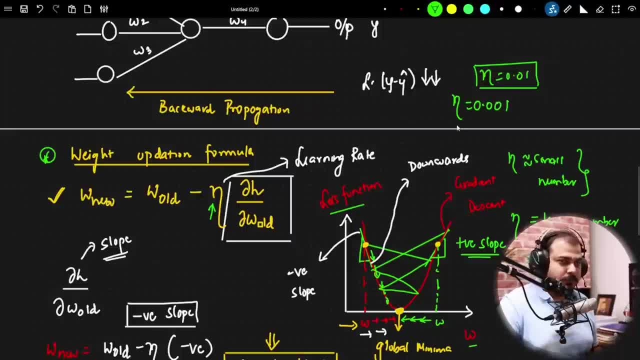 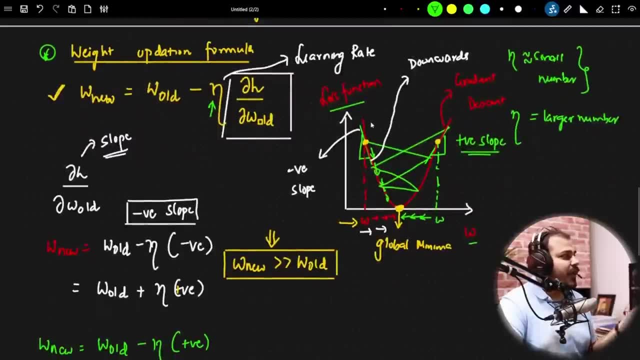 right, And this I will try to show you in the practical also. Okay, So our main aim should be that we should slowly converge. Otherwise it may be a situation where I may never reach the global minima, or not. So I hope you are able to understand till here. 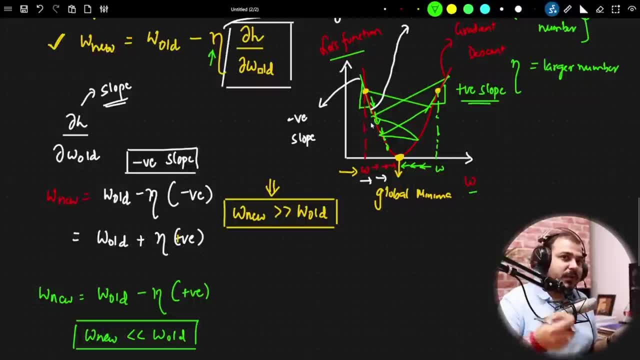 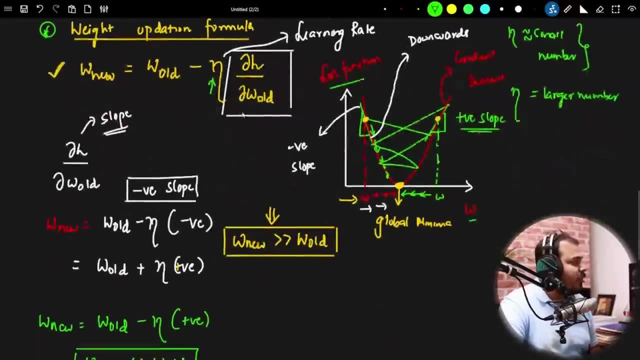 Uh, please do hit like if you're able to understand and please do comments. comment down some good messages If I can see whether you're following or not. Okay, So till here. I hope everybody's able to understand. with respect to the weight updation formula, 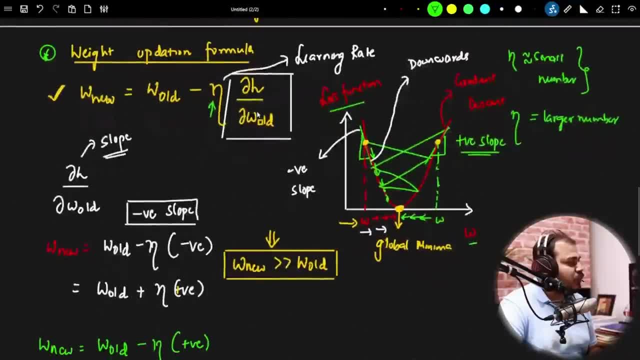 Perfect, Okay, Now after the weight updation. now you have understood this. weight updation basically happens in this specific way and you are able to clearly see that, how the weight updation usually happens and what all things we are able to do with this. 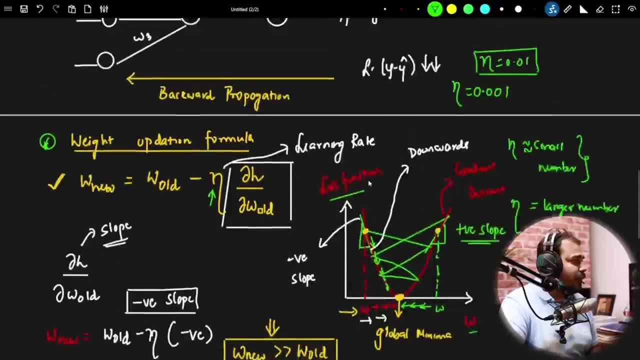 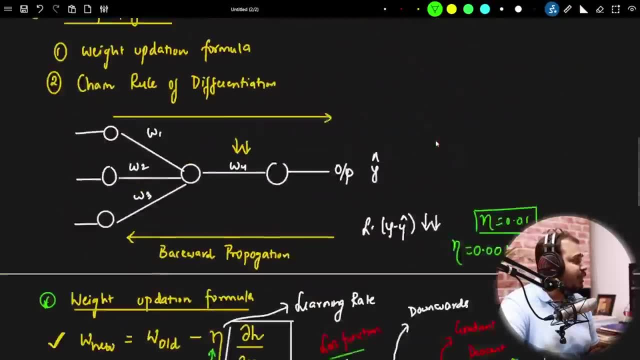 And this is how, in the back propagation, we basically do it. Now let's take one very simple example and let's see the entire chain: rule of differentiation. Now second point over here. I told you about first point. in back propagation, First thing that happens is weight updation formula. 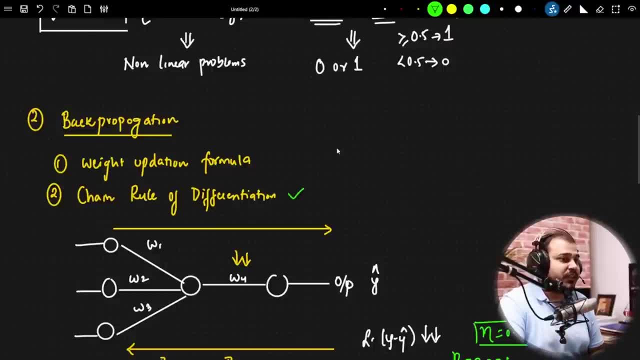 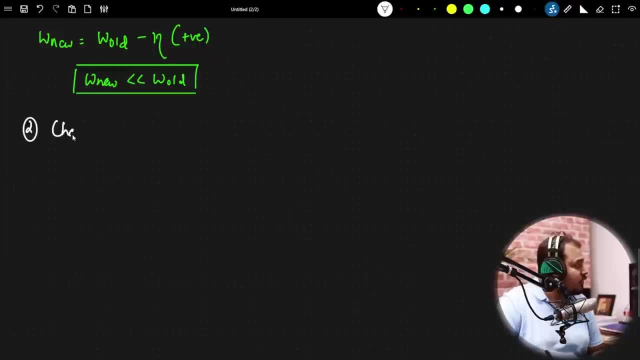 The second thing that basically happens is something called as chain rule of differentiation. Okay, Now, let's go to the second point. Now, in the second point, I basically see something called as chain rule of differentiation. Okay, Now, in the chain rule of differentiation, 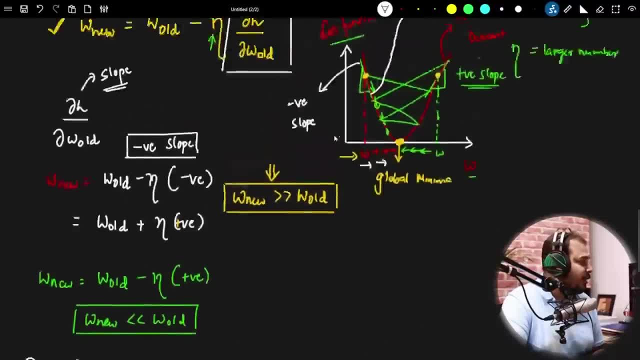 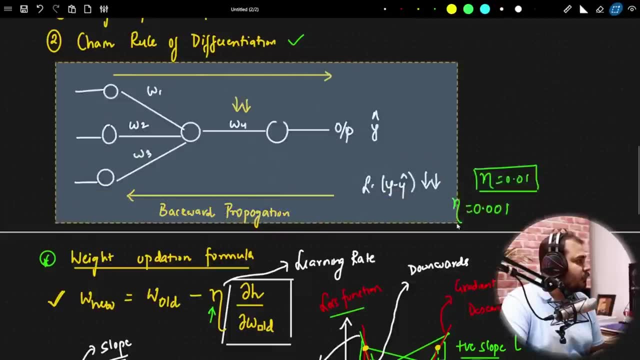 what happens and what is this chain rule of differentiation? We'll try to understand. Okay, Everybody has understood this, So I'm just going to copy this entire thing, Okay, And probably just paste it over there so that I don't have to rework it. 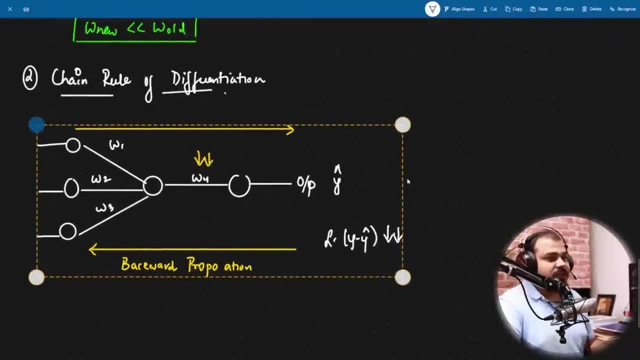 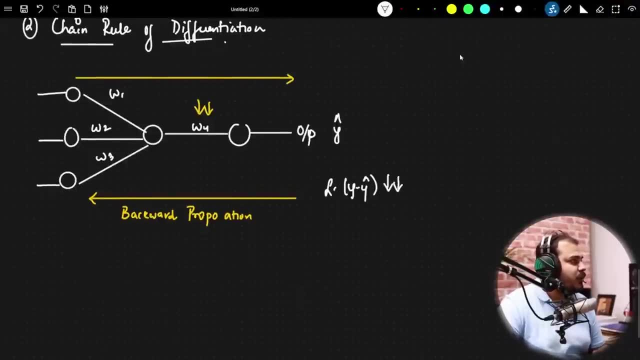 Okay, Now let's take the same diagram. Okay, Now you have understood what happens in the forward propagation and you have also understood the weight updation formula. Let me write the weight updation formula. It is nothing but W old, sorry. 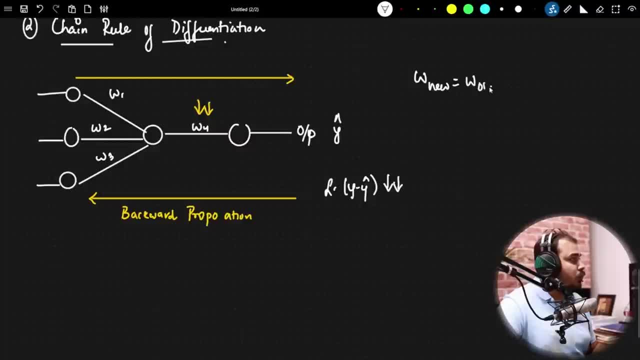 W new is equal to W old, minus learning rate, multiplied by derivative of loss with respect to derivative of W old. Okay, So this is the formula Perfect. Everybody has understood, I guess. Now our main thing is that how this derivative of loss with respect to derivative of W old happens. 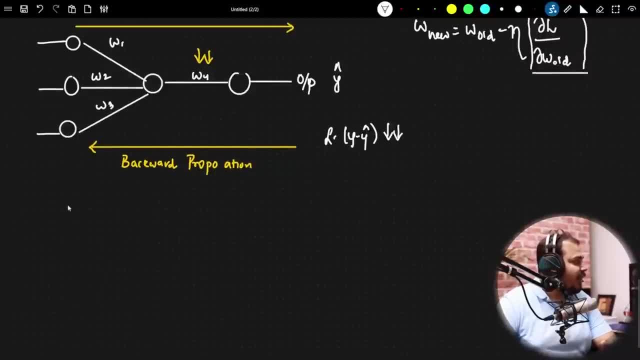 We need to understand. Okay, Let's say I want to find out the derivative of loss with respect to derivative of W4, W4 old. Okay, I want to find out this. So how W4 will get updated? Okay, How. 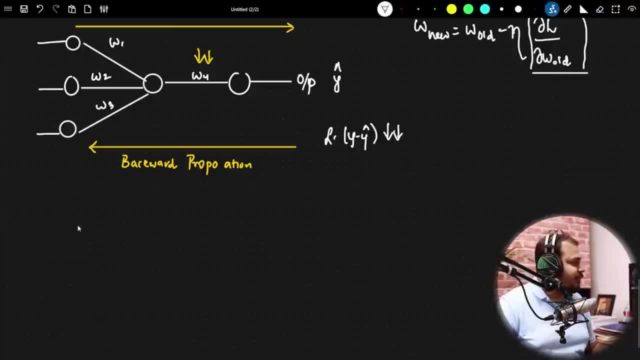 how W4 will get updated. So what I can write is that I can basically say: W4 new is equal to W4 old, minus learning rate of derivative of loss with respect to derivative of W4 old. Okay, So this is the formula for W4.. 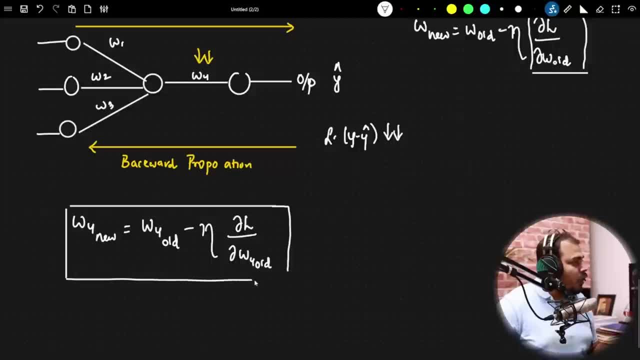 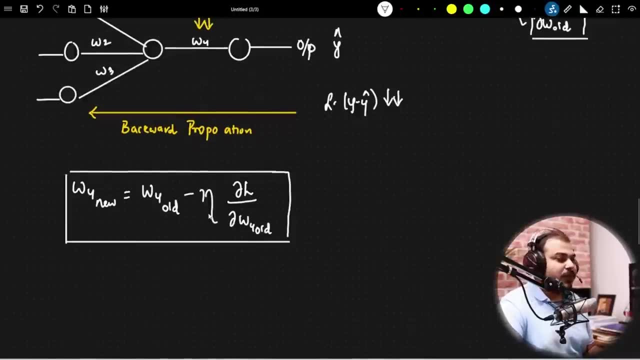 Whenever we try to update W4, right, All the other values, we can easily get it. Okay, We can basically easily get it. All the values like W4 old, we'll be able to get it. Learning rate is initializing initially. 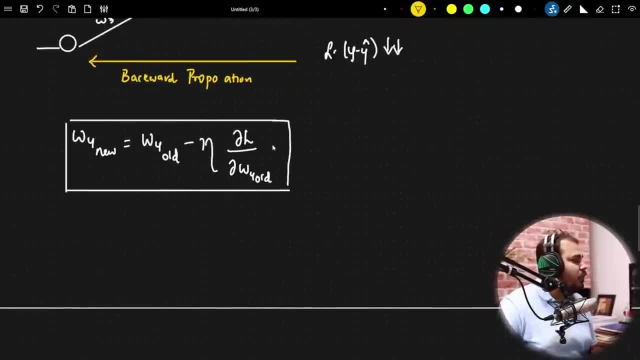 but. but the question lies: how do I find this value, that is, derivative of loss with respect to derivative of W old. Now derivative of loss with respect to derivative of W4 old. here I will specifically use something called as chain rule of derivative. 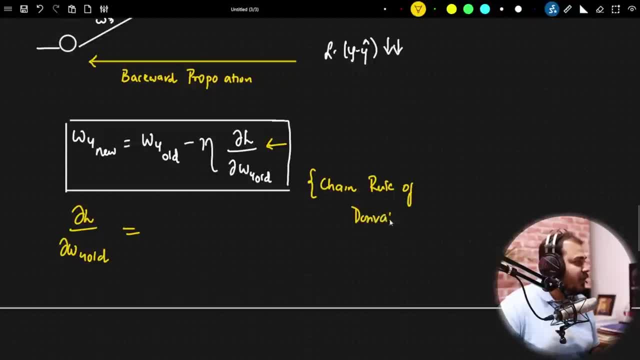 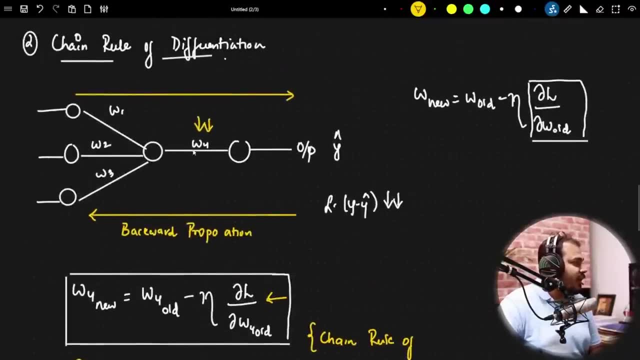 Now, what is the chain rule of derivative? in order to find out, Let's, let's understand. Okay Now, chain rule of derivative is basically say: since this is my loss, right, Let me write it down over here. Let's say: 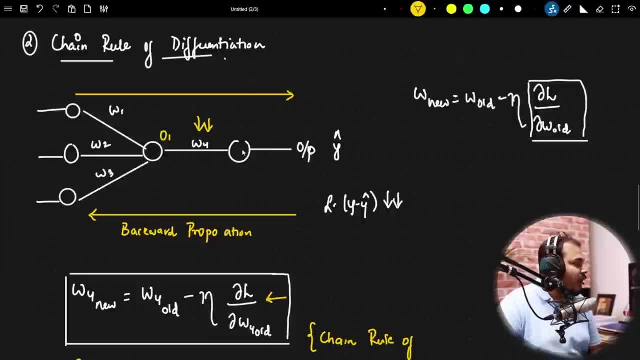 the output of this neuron is basically O1. The output of this neuron is basically O2.. What is this output? This, multiplied by the weights, is basically my output after applying an activation function. This inputs multiplied this X1,, X2,. 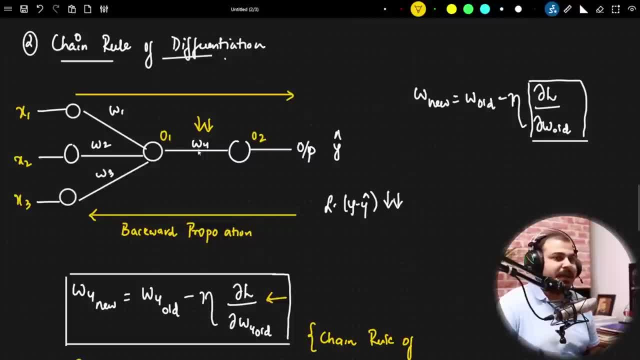 X3 multiplied by this added a bias and then activation function, I'll be getting an output as O1.. I hope that everybody's clear about- because I've already covered it Now- how to basically update this W4? W4 with the help of chain rule. 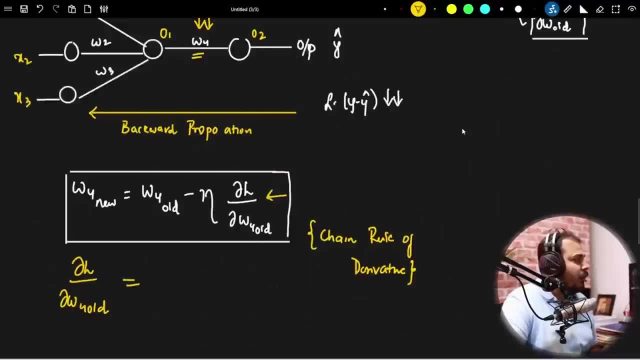 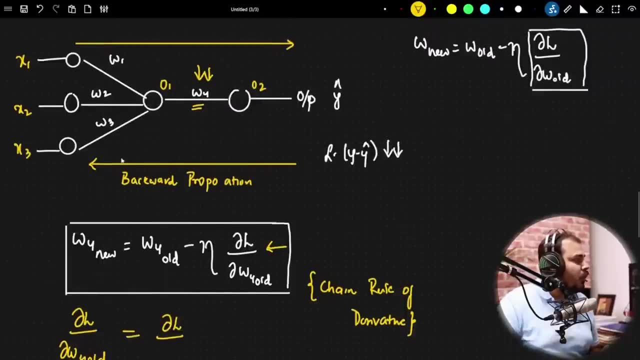 Okay, I'll write down the equation over here. Okay, Now, in order to, in order to find out this, what I will write, I will say that derivative of loss. Now, loss is dependent on what? it is dependent on the O2 value. 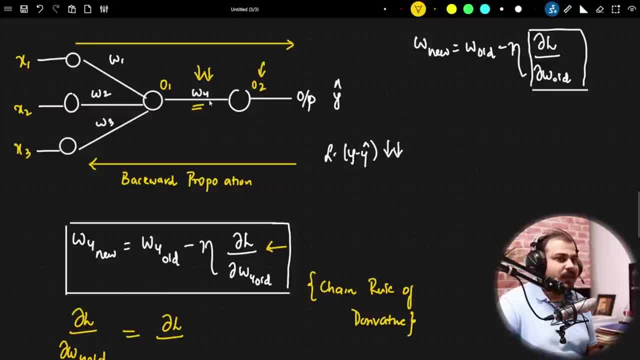 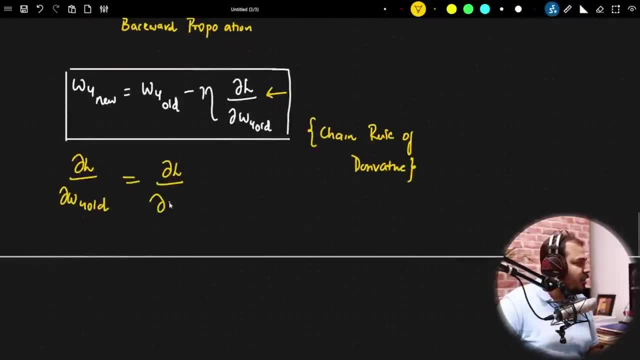 First of all, Okay, It is dependent on O2, because I need to update W4.. So, first of all, this loss is dependent on O2.. So I can basically write derivative of loss with respect to derivative of O2.. And then, according to the chain rule, 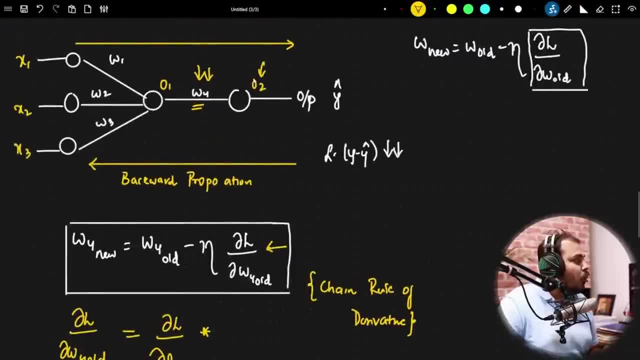 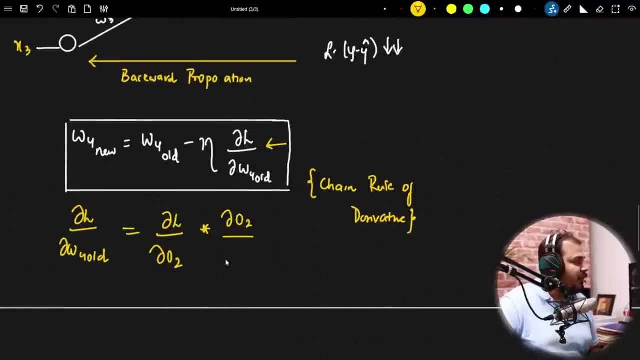 the next step that we will be going on, where in O2 is now dependent on W4. So what I will write in further step is that derivative of O2 divided by derivative of W4. Now here, if I sub, if I just cross this two. 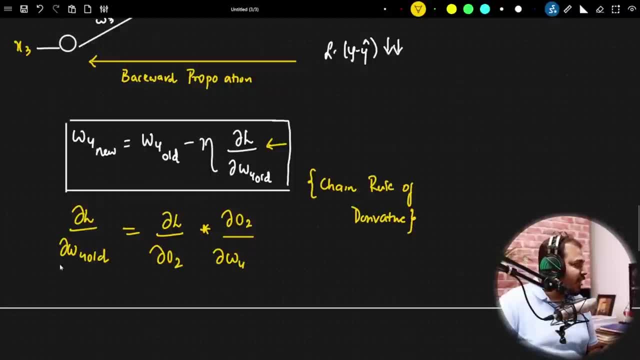 okay, if I cross this two, then what will happen? I will be getting this only right. This will be my W4 old If I cross this two, because this also can be removed, right, And this is what what chain rule of derivative basically means. 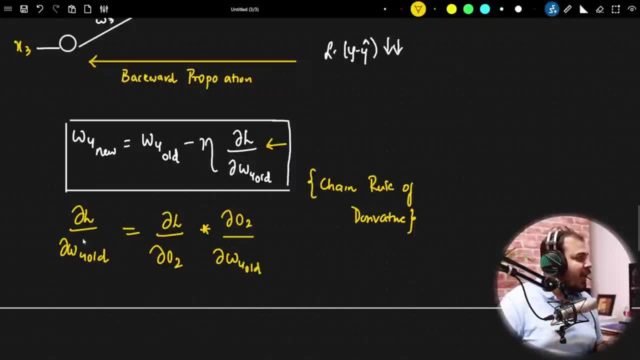 There will be a chain that will be formed in order to calculate this derivative of loss, right? So this is one example of the chain rule to update W4.. And what exactly is happening over here? We are basically trying to calculate the slope with respect to this particular derivative. 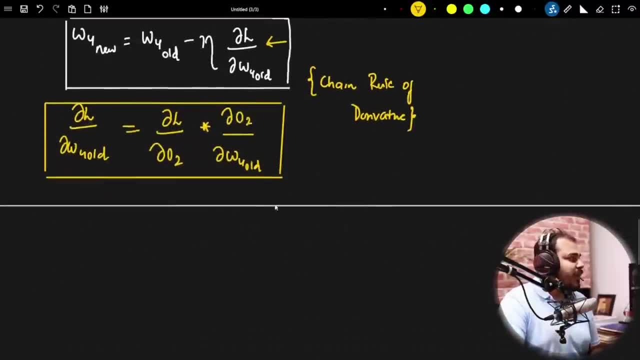 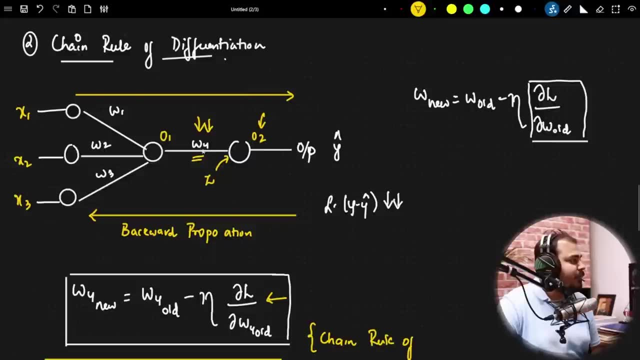 and we'll be able to get the answer. Okay, Let me add one more step. What is O2?? Let's say, this is my Z input. Okay, Z input is nothing but O1, multiplied by W4, and then we add a bias, and then we add an activation function. 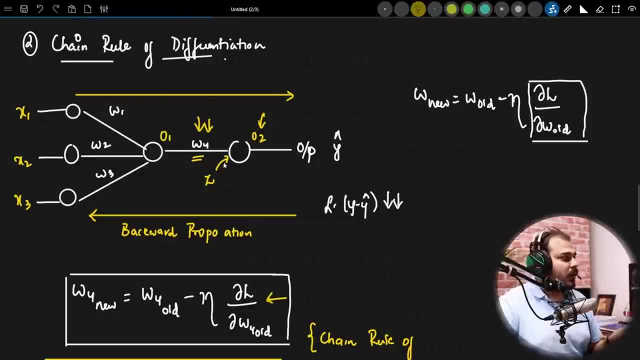 right, We add a bias and then we add activation function, right. So what is this Z? If I write what is this Z? Z is nothing, but it is an activation function applied to O1, W4 plus bias. I hope everybody's correct with this particular thing. 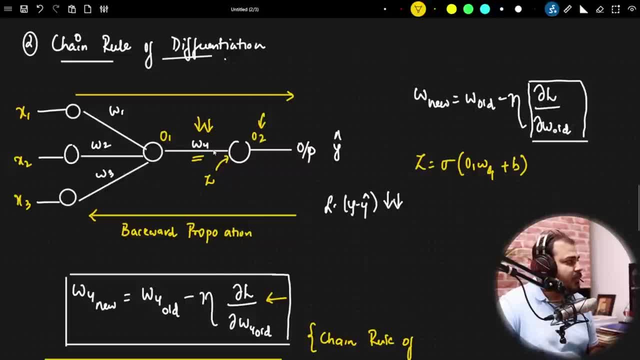 right, I hope everybody's able to understand over here. right: O1 multiplied by W4 plus bias, because here also bias will get added right, Here also bias will get added. Here also bias will get added right, Another bias. 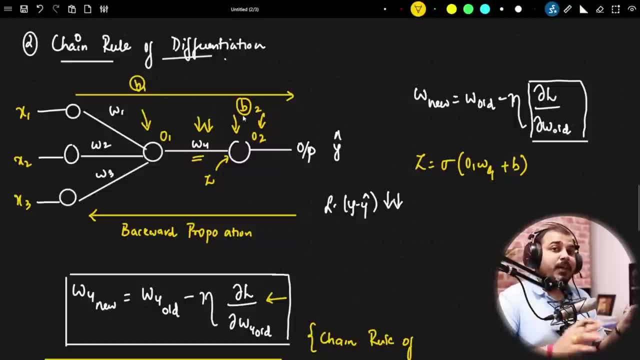 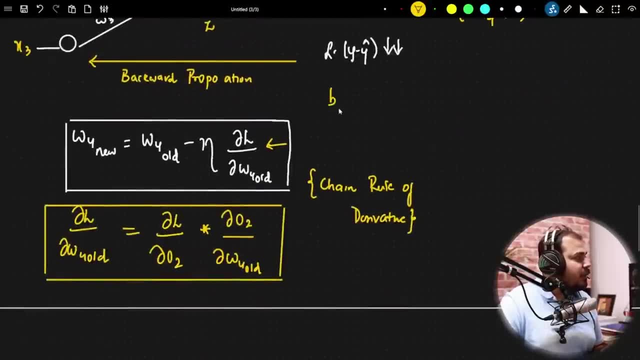 So this will be B1,, this will be B2. And bias will also have the same updation formula, like how weights are actually having. Okay, So if I probably write the bias activation function, it will be nothing but B2. old is equal to. 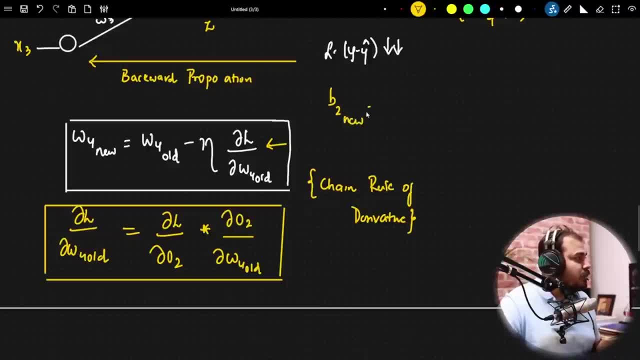 sorry, B2 new, It should be. B2 new is equal to B2 old minus learning rate of derivative of loss with respect to derivative of B2 old right. So this is the bias activation function. Sorry, not bias activation. This is a bias updation formula. 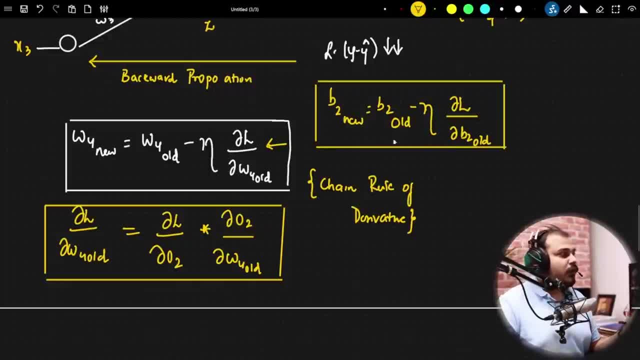 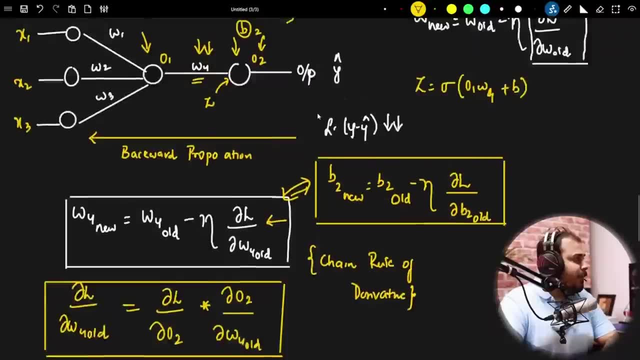 right Bias updation formula And it is similar. These two are almost similar. For bias also, it will happen. For weights also, it will happen. Okay, So I hope everybody's able to understand till here, right Now. what is our next step? 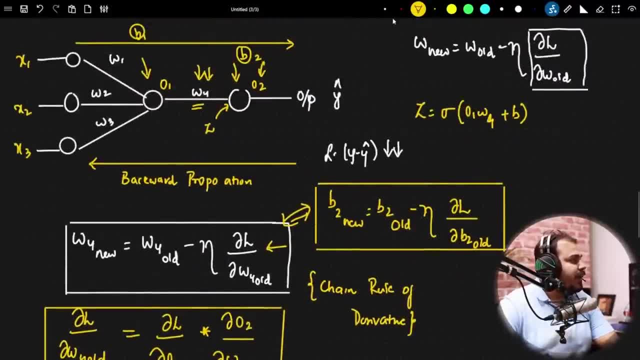 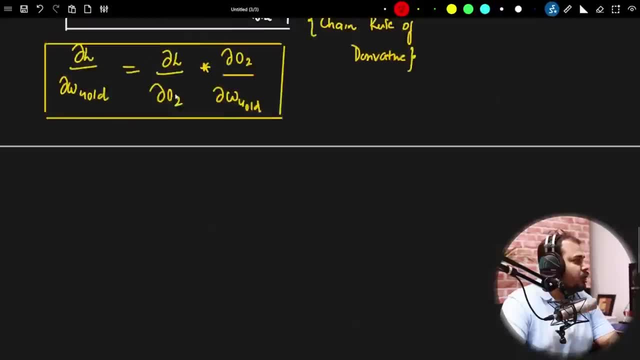 Okay. The next step is that let's say, I want to update this. This particular value of this weights W1.. So how I will go ahead, Let's see. Okay, So I will write derivative of derivative of let me. 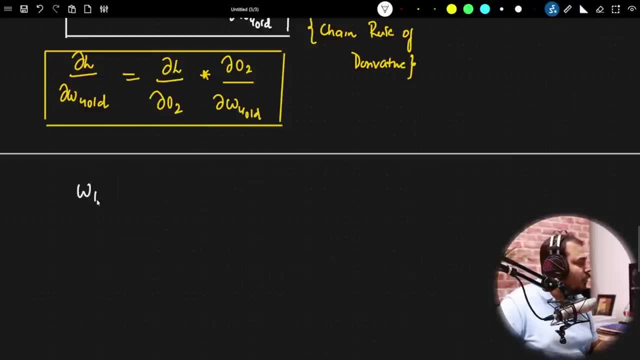 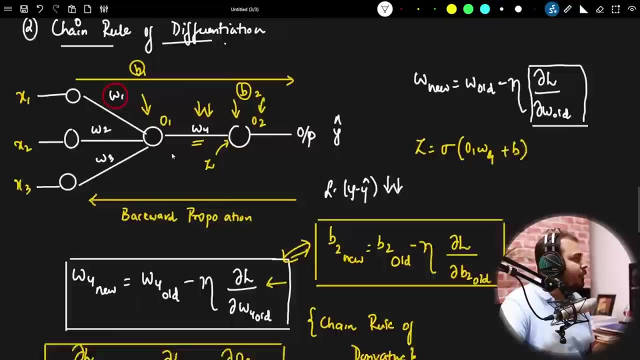 let me write it down So how it will be. I will basically write: W1 new is equal to W1 old, minus learning rate of derivative of loss with respect to derivative of W1 old right. This is the formula for updating W1.. 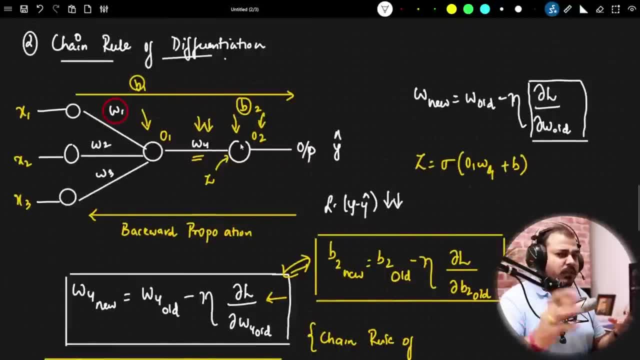 Yes For updating W1.. This is the formula. Now just try it from your side. No, just pause the video and try it from your side. that how will my chain rule work in this particular case? How will my chain rule work in this particular case when I am basically trying to find out the derivative of loss with respect to W1?? 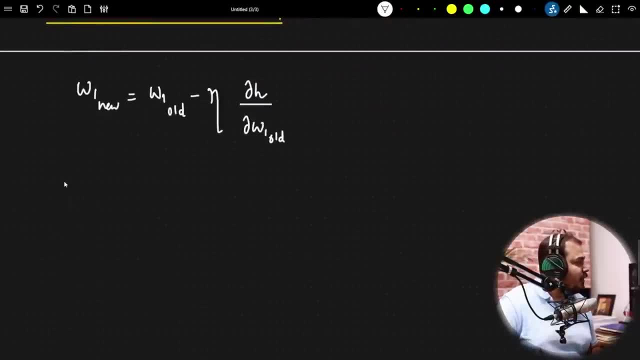 So here I'm just going to take this up. Okay, I'm basically going to take this derivative of loss with respect to derivative of W1 old. Now how I'm going to basically write this chain rule, Because for this, only this, is my main concern. 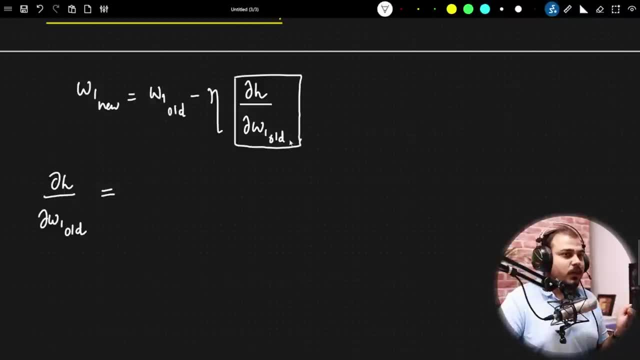 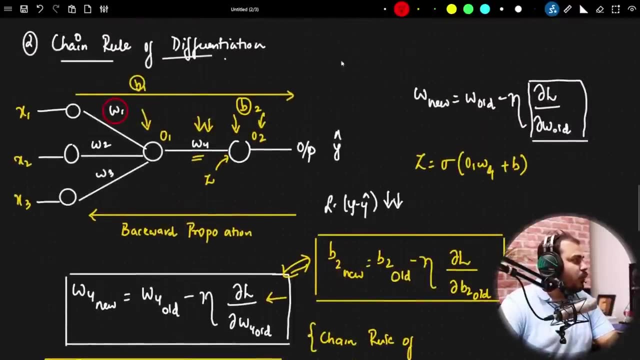 right, This is how I have to apply the chain rule in this particular equation. Okay, So how will I go ahead Now? let's go Okay Now. first step: you know that loss is dependent on O2.. O2 is dependent on O1 and O1 is dependent on W1. 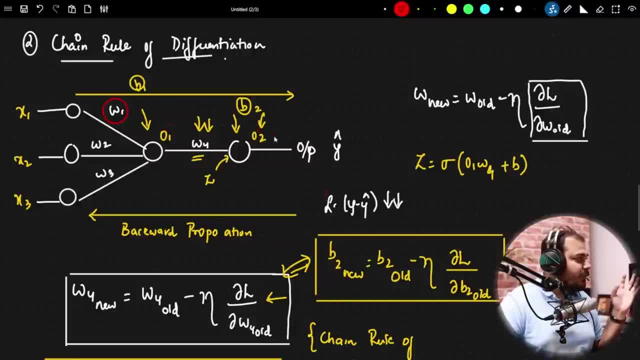 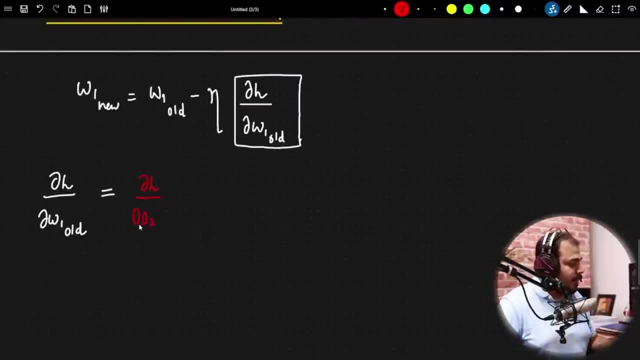 Okay, Now see, see the chain rule. Loss is first of all dependent on O2.. So what I will write? I will basically write derivative of loss. with respect to derivative of loss, Okay, With respect to derivative of O2.. Okay. 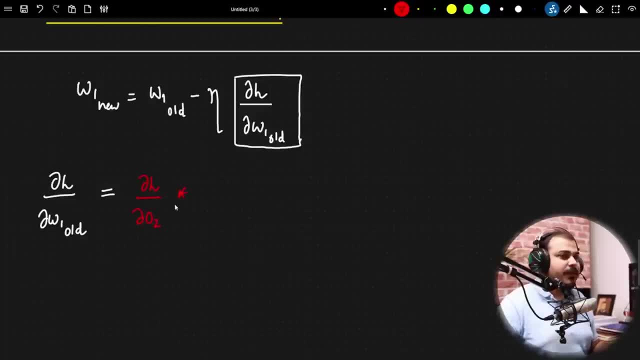 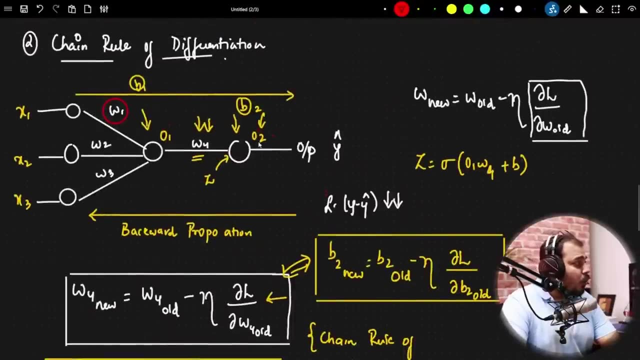 First step, derivative of O2.. Then I will multiply it over here. Okay, Derivative of loss with respect to derivative of O2.. Now O2 is dependent on O1. You can see over here, right, Because O1 output is this one. 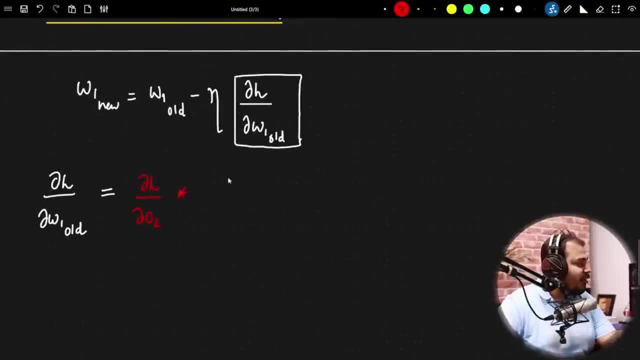 O2 output is this one. So in the next step, what I will write is that I will basically say: derivative of O2 divided by derivative of O1.. Right, So this step is also very much clear. Okay, And the next step. 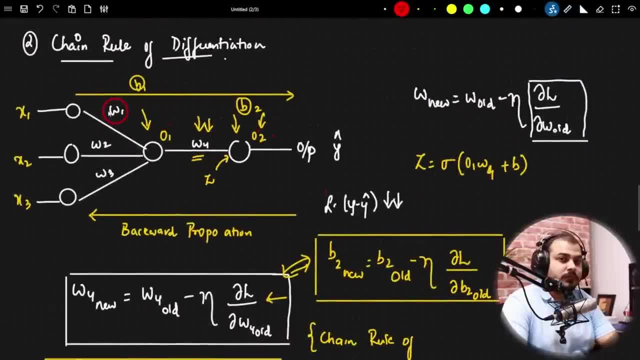 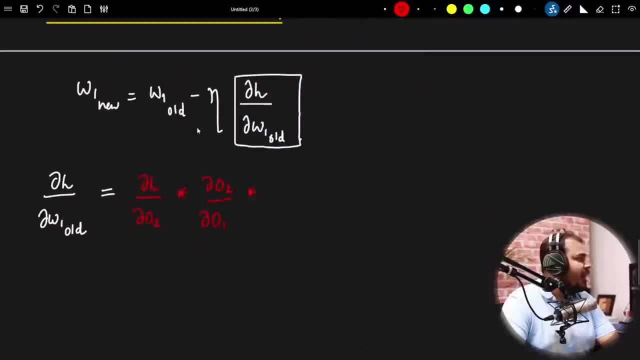 what we are basically doing. O1 is now dependent on W1.. You can see over here O1, this O1 is dependent on W1.. Right, So now I will go ahead and write the next step. That is derivative of O1 divided by derivative of W1. 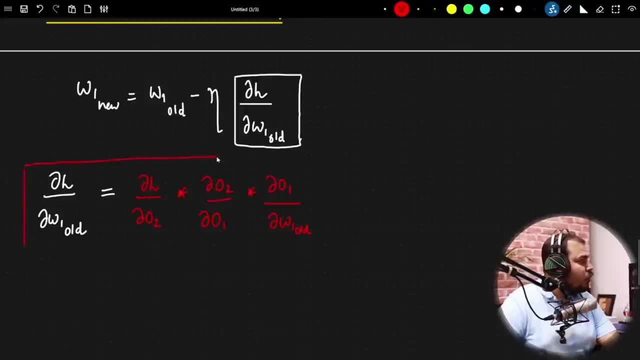 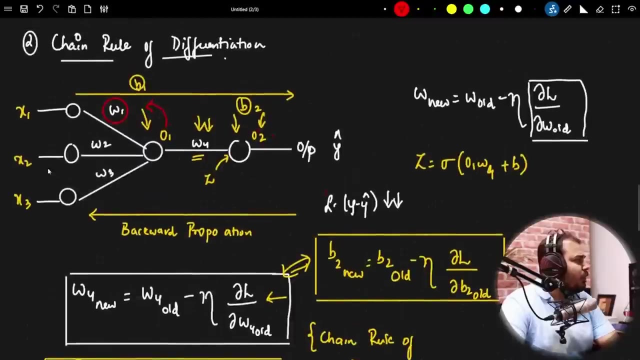 Right, So this becomes my new chain rule of differentiation. to update W1.. Right, To update W1.. This becomes my different chain rule of differentiation. Right, So I hope everybody is able to understand. Now just try it out with respect to W2.. 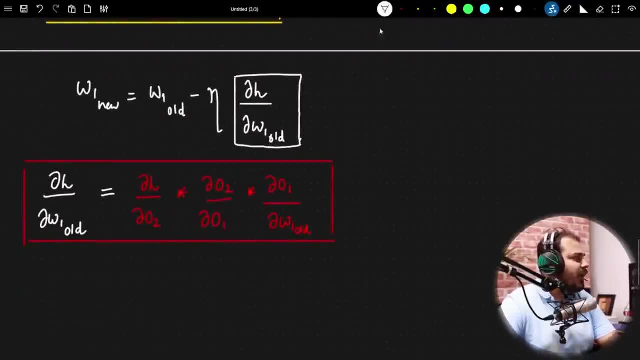 With respect to W2, what will be my updation formula? So again, I will go and write over here: W2 new is equal to W2 old, minus learning rate of derivative of loss with respect to derivative of W2 old. Okay, 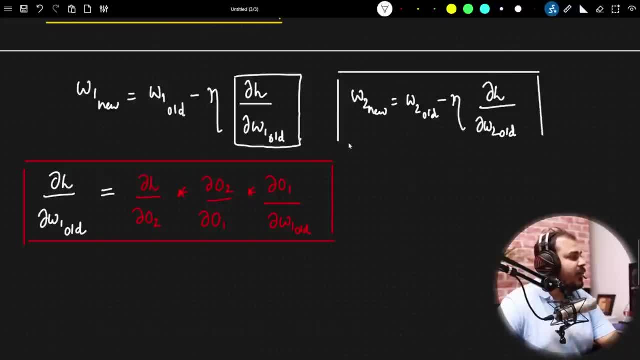 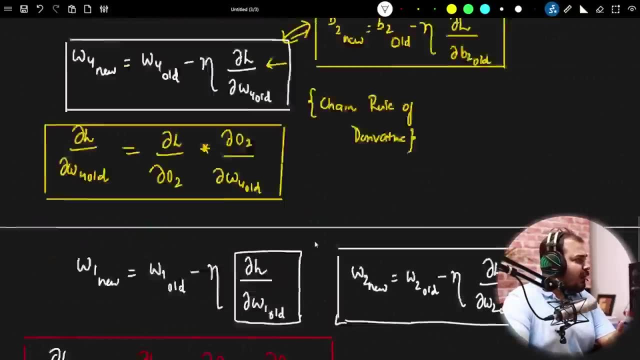 So this is my another formula. Now, how do I write Derivative of loss with respect to derivative of W2, old, Okay? How do I write: Okay, See, don't worry about W4.. You may be thinking: where is W4?? 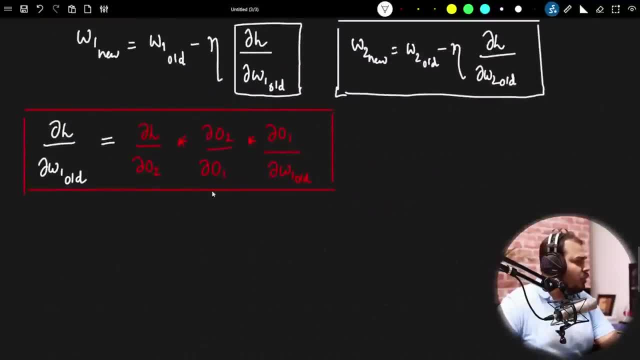 W4 can still be divided. See this same thing. this derivative of O2 to derivative of O21 can also be done with chain rule, like this: Derivative of W4 multiplied by derivative of W4 by derivative of O1.. Yes, 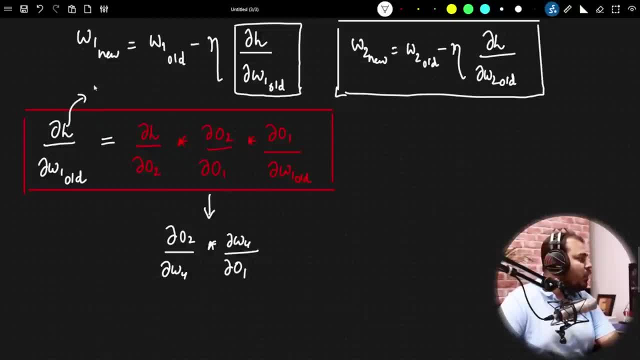 So I hope everybody is able to understand this: L is nothing but loss right. Loss is dependent on that right. So like this, you can still more divide it. since we are learning chain rule of differentiation, It can be expanded to any manner you want. 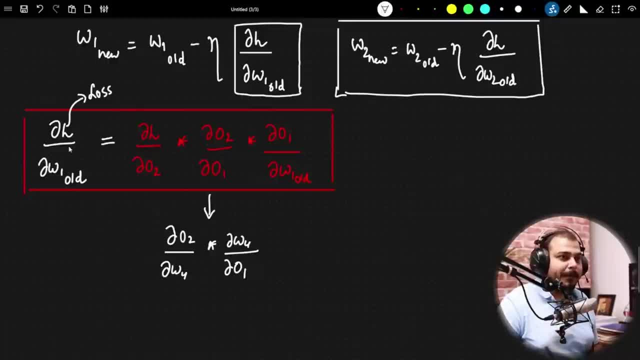 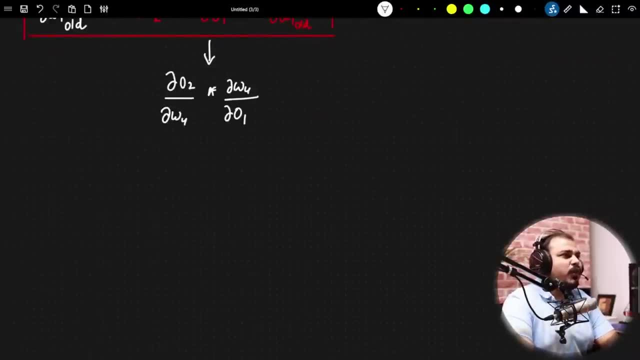 but at the end of the day you will be getting this specific thing only Right Now. let's see one more example. Let's say I create a separate neural network. This neural network looks a little bit cubism. Okay, Let's say in the first in I just have one input layer. 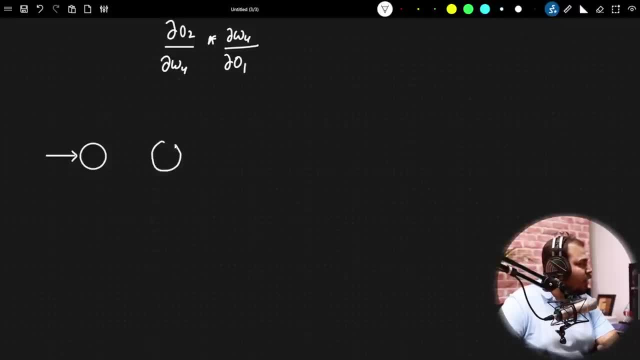 one input neuron. Okay, Then I have one hidden neuron. Okay, Then in the next hidden layer I have two hidden neuron and in the third, in the final output, I have one hidden one neuron in the output layer. So when I combine this, 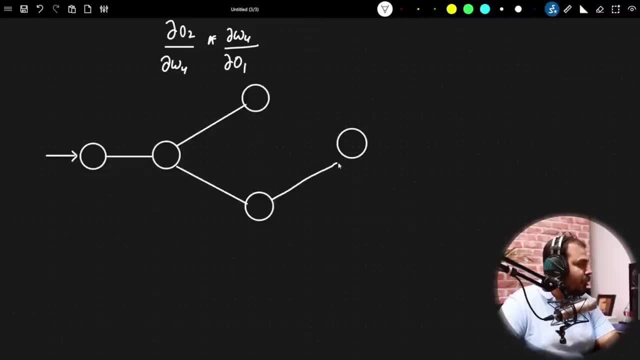 this becomes at this shape: Okay. This becomes at this shape: Okay. And finally I get my output. Okay, Now let's say, this is my X1.. Okay, This is my W1.. This is my W2.. This is my W3.. 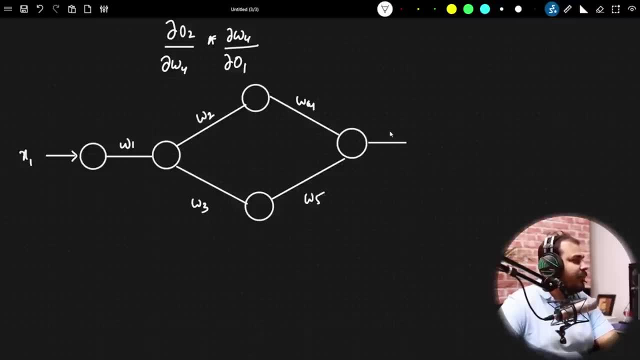 This is my W4.. This is my W5.. And finally, this is my output of this. So let's say I'll also write the output. This output is nothing but O11.. This output is nothing but O21.. This output is nothing but O22.. 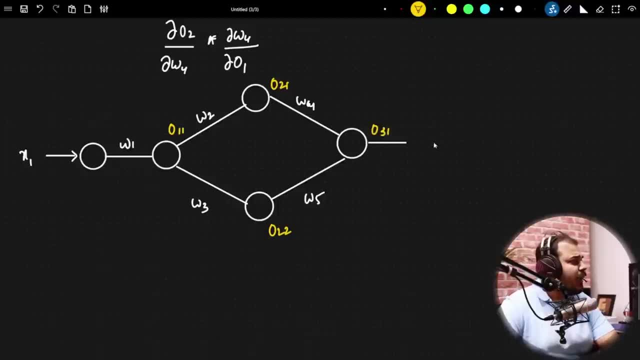 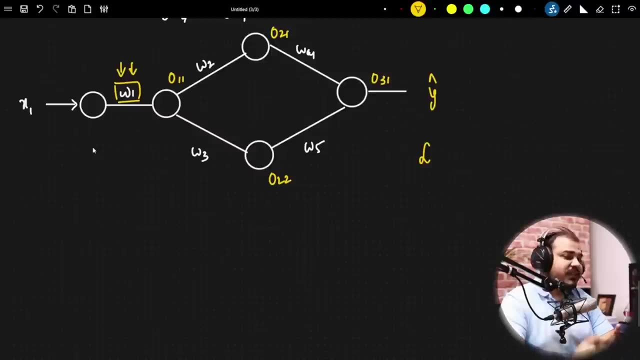 And this output is nothing but O31.. And then what happens? I get Y hat, And then, finally, I get my loss. Okay, So let me just show you. First of all, you try- I would suggest you try it by yourself- and then come to a conclusion. 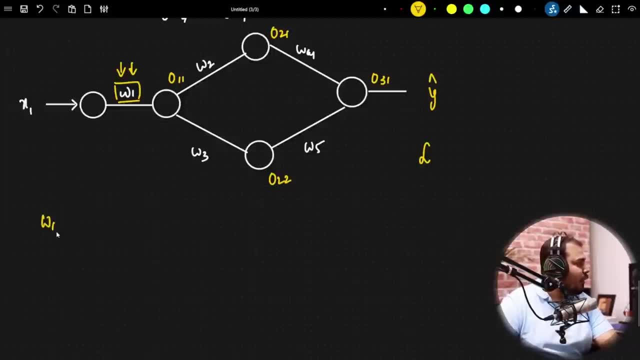 Okay, So over here I can basically write: W1 old is equal to sorry, it should be new. Again, I'm writing old, So W1 new is equal to W1 old minus learning. rate of derivative of loss with respect to. 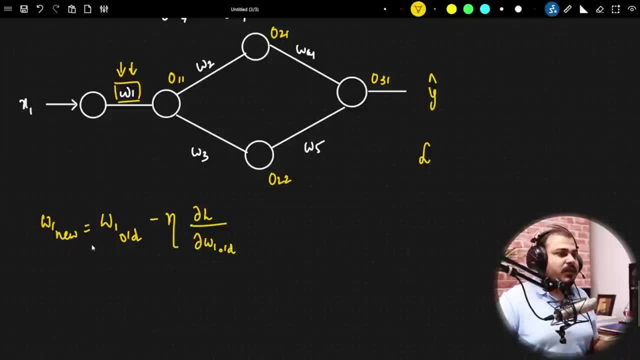 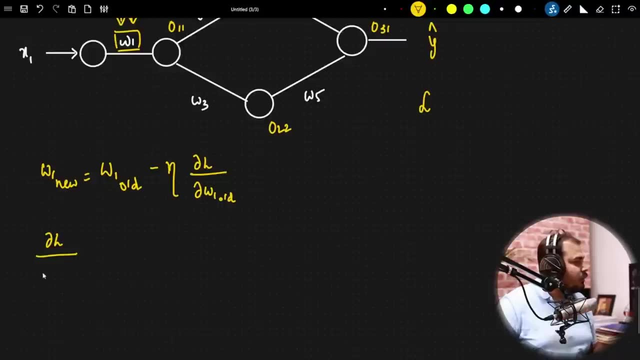 derivative of W1 old. This is the weight updation formula. This everybody knows it. Okay, But if we go to the next step, how do we calculate derivative of loss With respect to derivative of W1 old? Now just understand the chain rule. 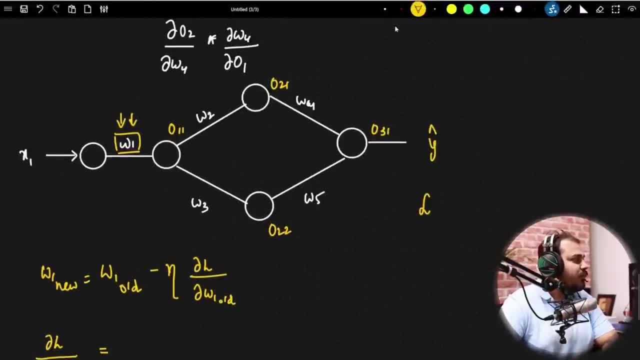 There are two routes that you can basically see over here. The first route goes in this way: Loss is dependent on O31.. O31 is dependent on O21.. O21 is dependent on O11 and O11 is dependent on W1.. 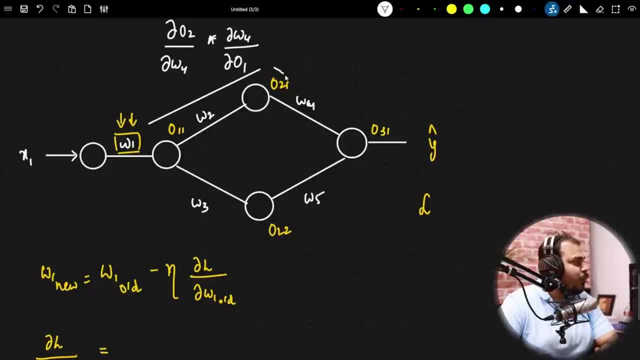 This is one route, So this is basically my one route which I can actually go, And the other route is something this one. I have one more route that is basically dependent on this in order to get this, In order to update W1, because this all dependency is also there. 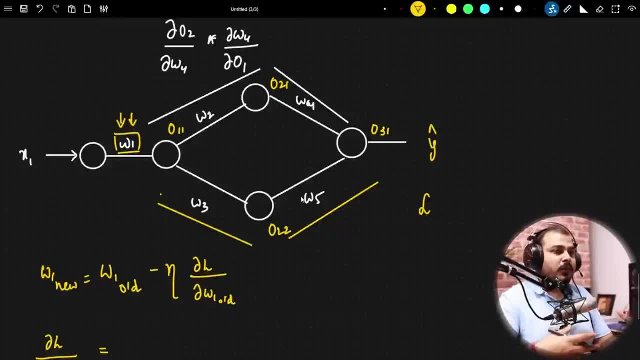 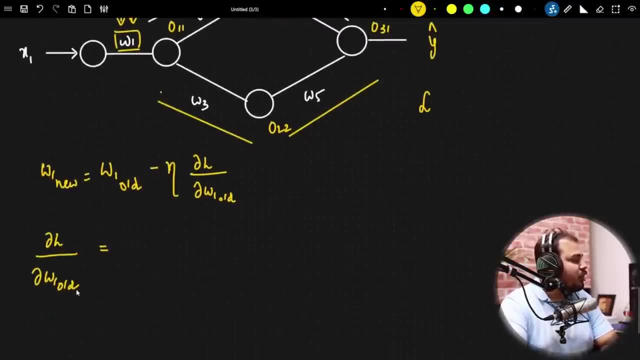 So how do I go ahead? How do I combine these two things? Okay, How do I combine these two things. Okay. So let's go and update this Now. how do I write derivative of loss with respect to derivative of W1 old? 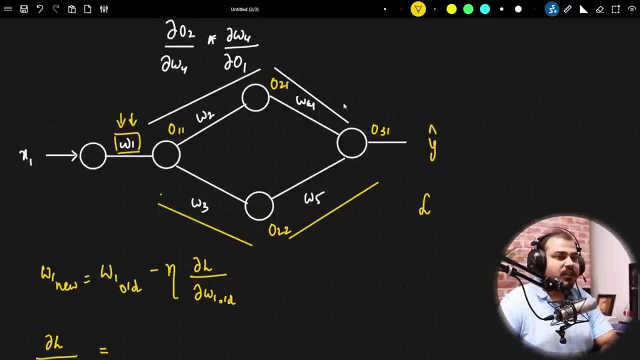 First I will take this path and find out the chain rule of differentiation, And then I will be adding this path. So when I combine both of them, it is just like an OR operation. Okay, So let's go ahead. So first of all, 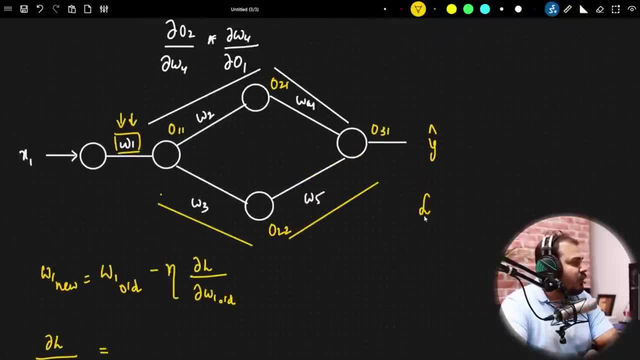 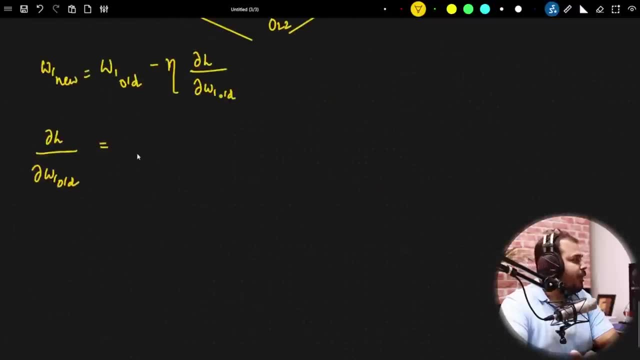 let's go on the topmost path. So here derivative of loss is dependent on O31.. O31 is dependent on O21.. O21 is dependent on O11.. O11 is dependent on W1.. Okay, So here I can basically write derivative of loss. 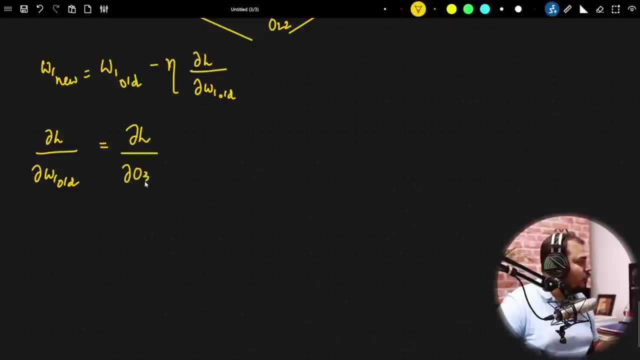 Derivative of loss with respect to derivative of O31.. Then multiplied by derivative of O31 divided by derivative of O21. Then multiplied by derivative of O21 divided by O21, is dependent on O11.. Right O11 and then again multiplied by derivative of O11 divided by derivative of W1- old. 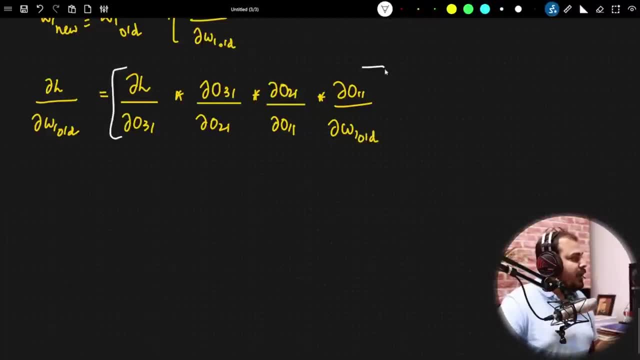 So this is one. This is the first path. Right Now, in the second path, I will be adding one more, That is the lower path. Right, The lower path will be what Over here. Lower path is again derivative of loss dependent on O31.. 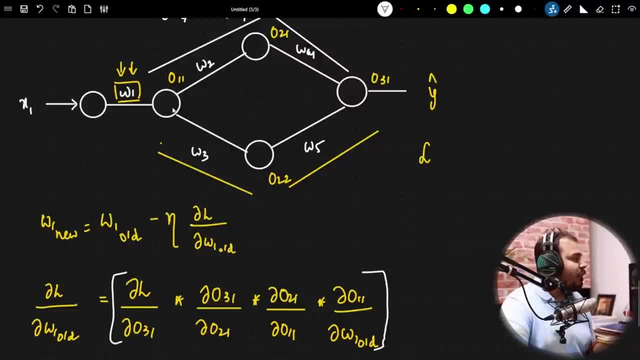 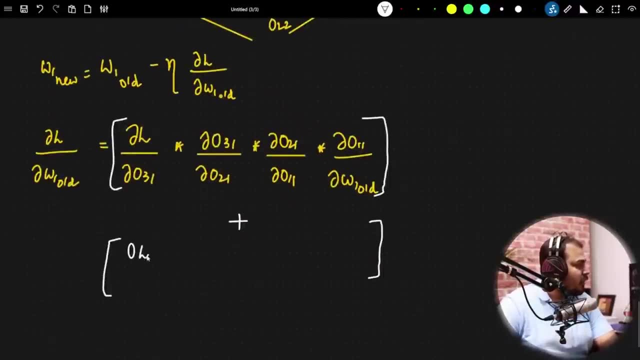 O31 is dependent on O22.. O22 is dependent on O11.. O11 is dependent on O21.. O11 is dependent on W1.. Very simple Right. So here I will basically write: derivative of loss. Derivative of loss is dependent on O31 plus. 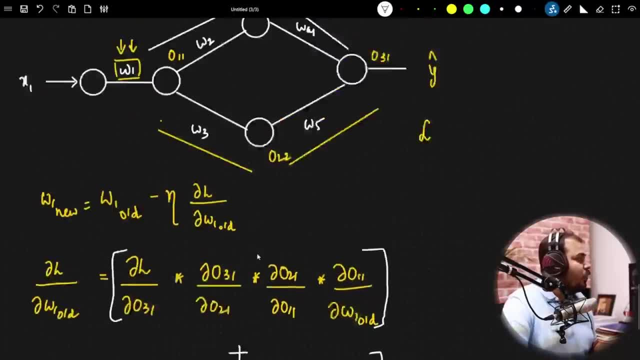 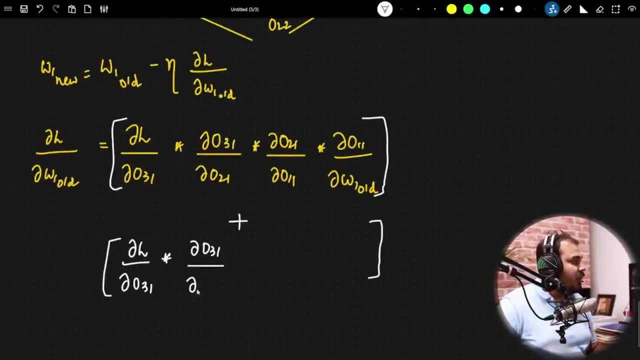 Sorry, multiplied. Since we are doing chain rule, then O31 is dependent on O22.. So now I will change this. Derivative of O31 is dependent on derivative of O22.. Then again we'll try to multiply this. derivative of O22 is dependent on O11. 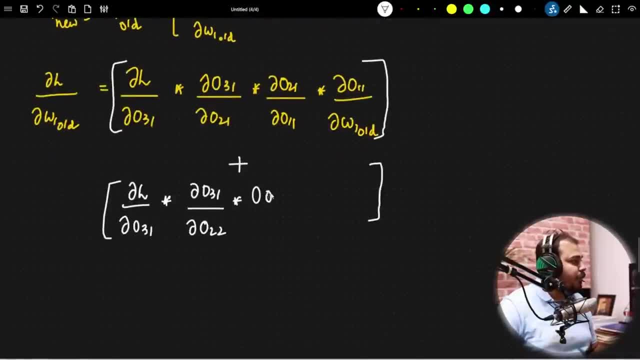 Then again, we'll try to multiply this. derivative of O22 is dependent on O11.. Right, So, derivative of O22.. Derivative of O22 is dependent on derivative of O11.. And finally, derivative of O11 is dependent on derivative of W1.. 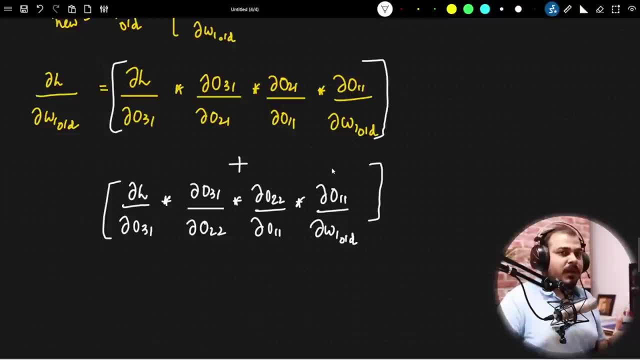 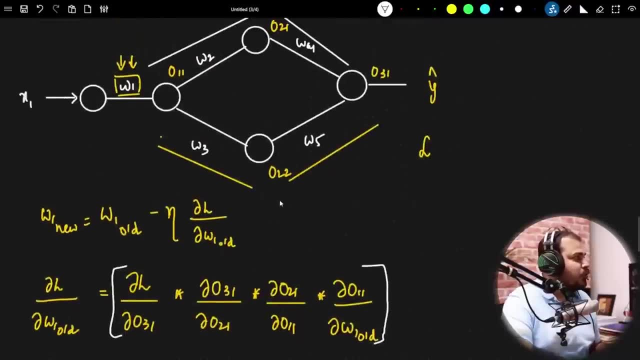 Hold Right. So we have to add this both up, and then we will be able to get the solution for the weight updation formula in the backward propagation. So this usually happens in the backward propagation. So this usually happens in the backward propagation. 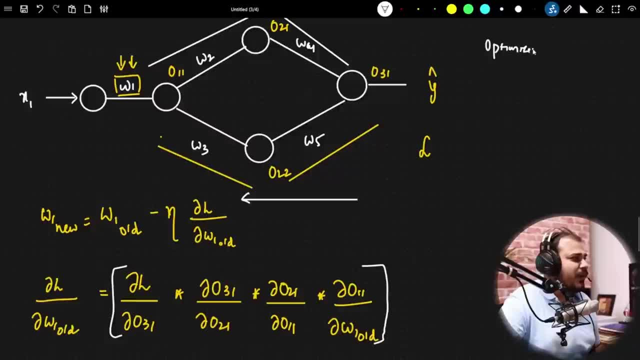 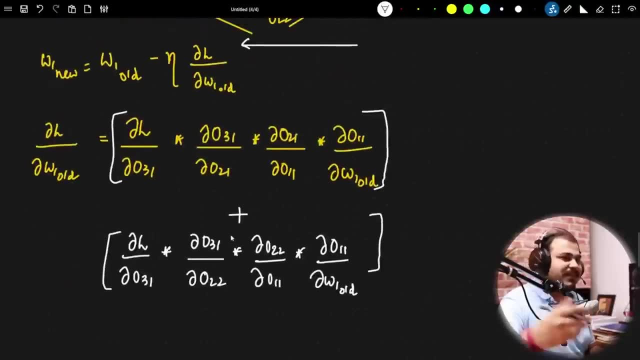 Who does this task? There is something called as optimizers. We'll discuss about this in depth, But I really wanted to make you understand about what exactly is chain rule of differentiation And this is what exactly chain rule of differentiation is Right. So we basically call this as chain rule of derivatives. 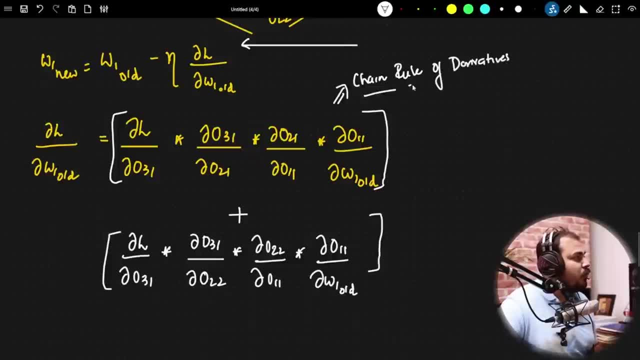 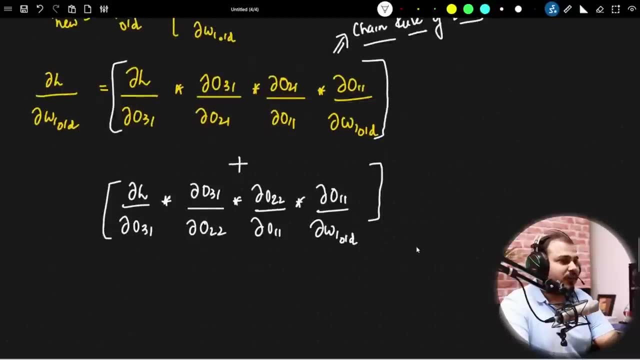 Right Chain rule of derivatives. Now we'll go to the next topic. Okay, So I hope everybody has understood about the chain rule of differentiation. Okay, So the next topic that we are probably going to discuss about is something called as vanishing gradient problem. Okay, So, vanishing gradient problem is a major, major problem. It's a major, major problem which we will try to see to it. Okay, So the next topic that I'm going to cover is something called as vanishing gradient problem. 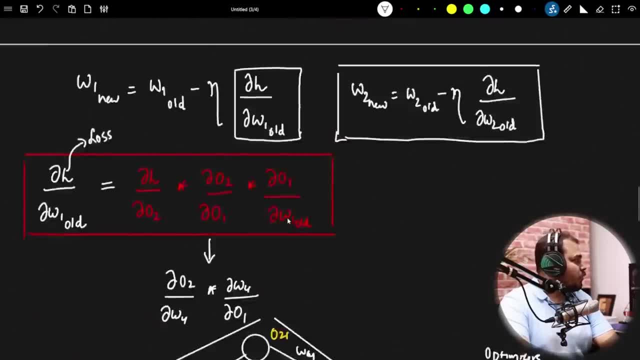 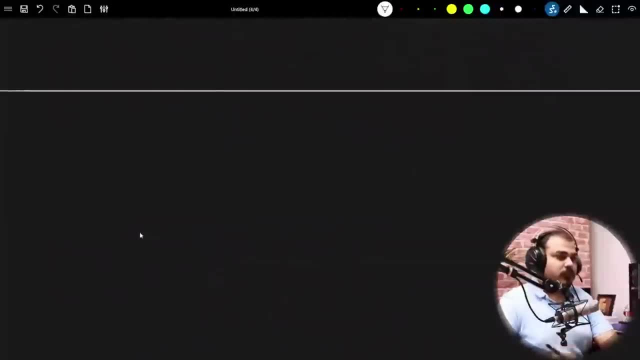 Okay, So let me see which. this is basically third. Okay, Third, coming to the vanishing gradient problem. Okay, So number three is basically called as vanishing gradient problem. Okay, Now, what happens in a vanishing gradient problem? Okay, Now one very, very important thing that you really need to understand. Okay, What exactly is vanishing gradient? A super important interview question. Okay, Super, super important interview question. 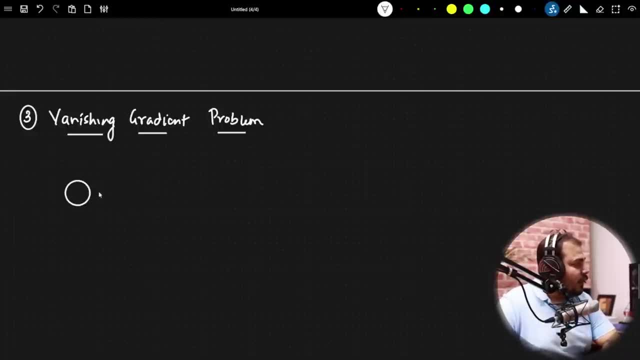 Now, let's say I have a very deep neural network like this Very deep neural network which looks like this: Okay, So this is a very deep neural network. Okay, Suppose I say: this is my x1.. My, this is my weights. 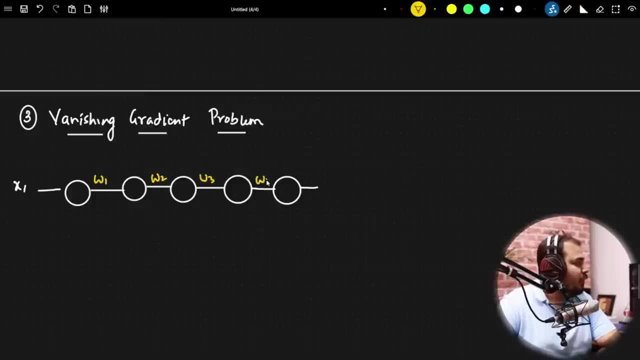 W1.. This is my weights: W2.. W3.. W4.. And finally I get my output, Which is my y hat And the loss function. Now I'm first time writing a loss function formula Which is basically called as mean squared error. So mean squared error formula is 1 by 2 y minus y hat, whole squared. 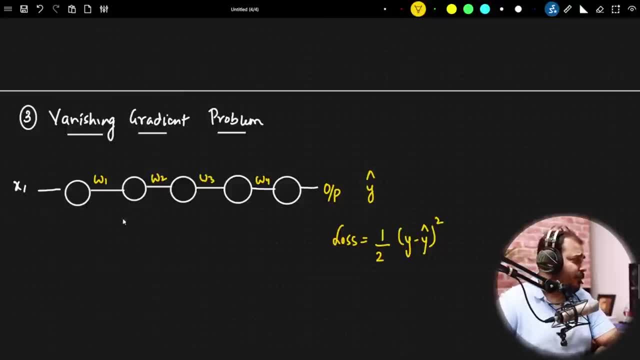 Okay, We'll discuss about this. What exactly is mean squared error and all? I hope everybody knows which activation function initially we are discussing about. We are discussing about sigmoid activation function, Sigmoid activation function. Now there are some properties of sigmoid activation function. Sigmoid activation functions gives you value with respect to 0 or 1.. 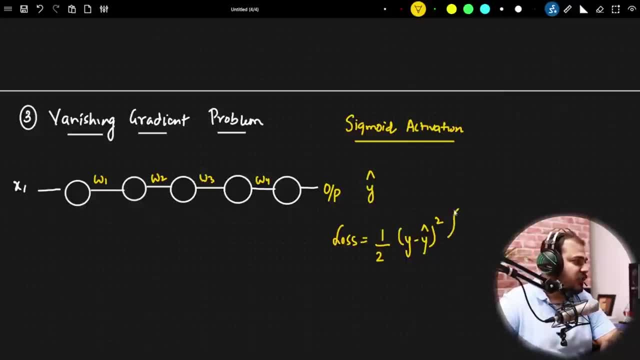 Okay, It gives you value with 0 and 1.. What is this loss function? This loss function is MSC Mean squared error. We'll discuss about this, Okay, Just in some time. We'll discuss in completely depth. We'll understand every maths. I'll not leave out any, even a single maths in this, Okay. 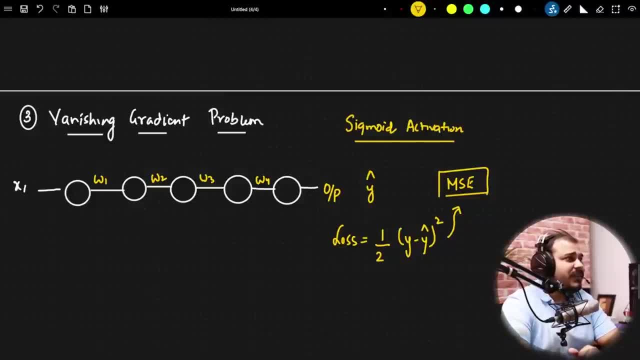 Now, Let's, let's, let's consider this neural network. So I have this specific neural network. Now, in this neural network, we need to understand two important things, Okay, Which which is super important for any interview, Okay, So over here, as you know, we will be basically adding bias 1.. Here, bias 2.. 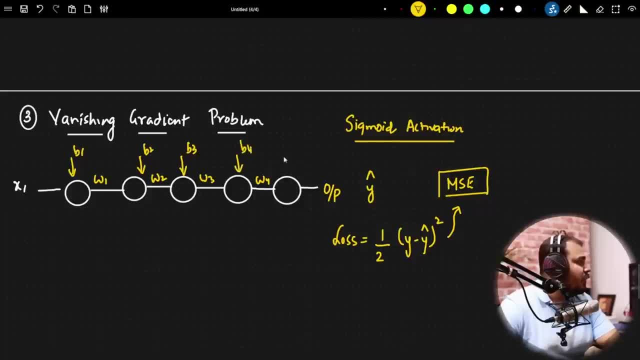 Here bias. 3.. Right Here bias, 4. Here bias, 5.. So bias will be getting added in every hidden layer which I have already discussed. Right, Let's say that the output, the output for this layer, is nothing but 0 to 1.. For this it is 0, 3, 1.. 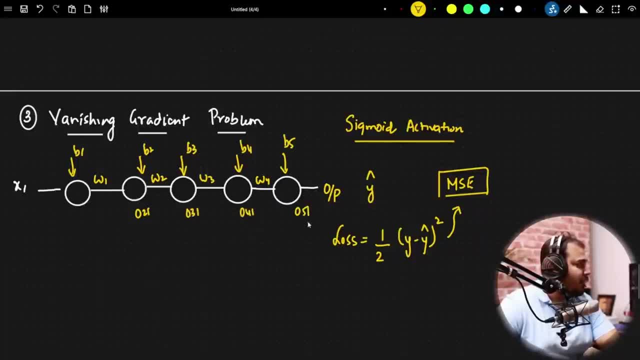 For 0, 4, 1.. And this is basically my 0 5, 1.. Let's say I have this many outputs Right Now, tell me, in order to update W 1.. How will I write the formula Or my? 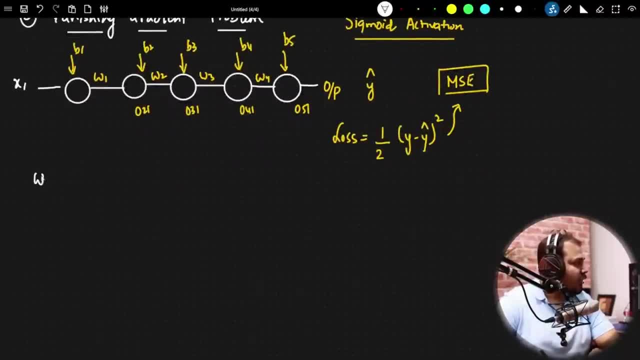 Weight updation formula That also we have discussed again. I'm revising it clearly to you: W 1 new is equal to W 1 old, minus learning rate of derivative of loss with respect to derivative of W 1 new. Okay, This is the formula. I hope everybody knows this. I have written it 10 times now. Okay, 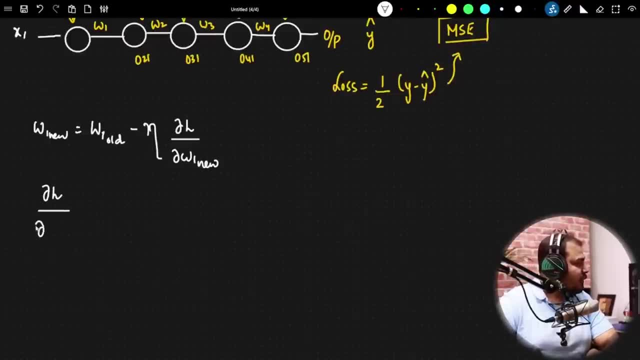 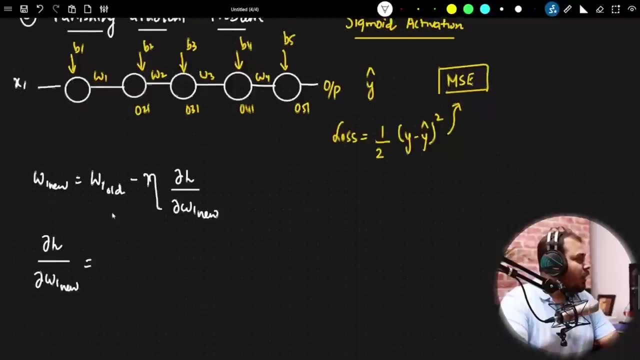 Now let's go to the next step. If I write derivative of loss with respect to derivative of derivative of W 1 new, then how will I write the chain rule? The chain rule will be very simple, So I will write derivative of loss with respect to derivative of 0- 5- 1.. 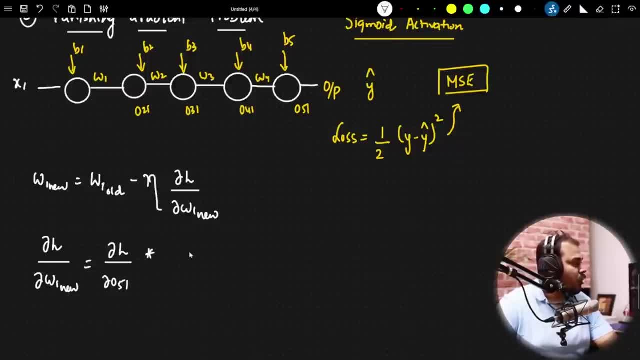 Okay, Multiplied by 0, 5, 1 is now dependent on 0 4, 1.. So I will write derivative of loss: Derivative of loss with respect to derivative of 0 4- 1.. Then I will go ahead. Sorry, This will be derivative of 0 5- 1.. 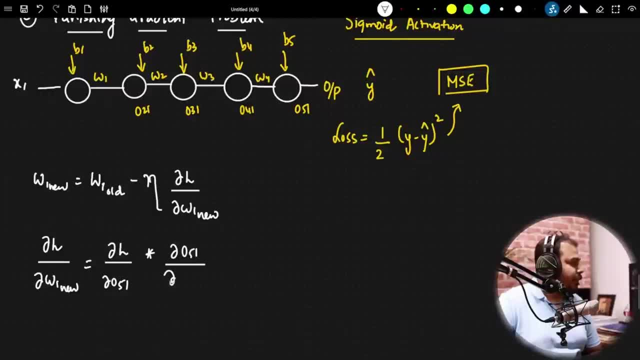 Derivative of 0, 5- 1 divided by derivative of 0, 4- 1.. So the derivative of loss with respect to derivative of 0, 4- 1 will be 0, 4- 1.. So here will be 0, 4- 1 multiplied by derivative of 0, 4- 1, divided by derivative of 0, 3- 1.. 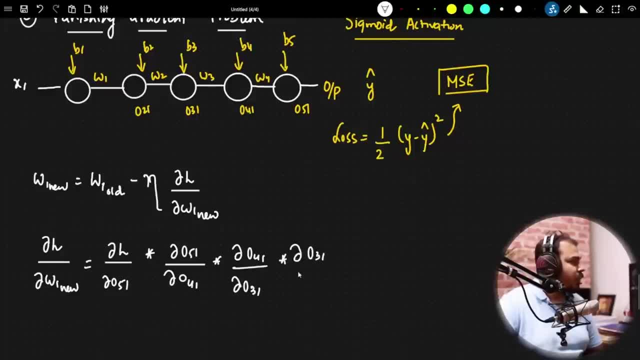 And then the derivative of 0- 3- 1 divided by derivative of 0- 2- 1.. Okay, Multiplied by derivative of 0- 2- 1 divided by derivative of W- 1.. OK, So I hope everybody is getting clear with this. 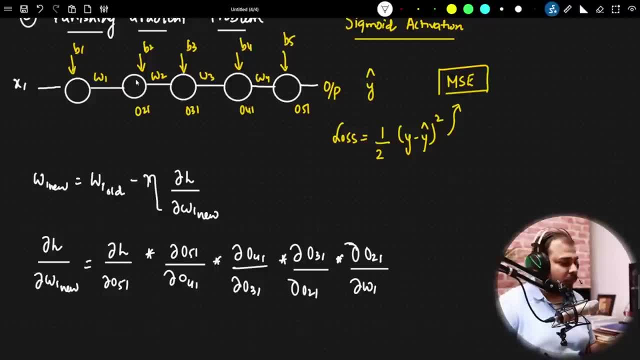 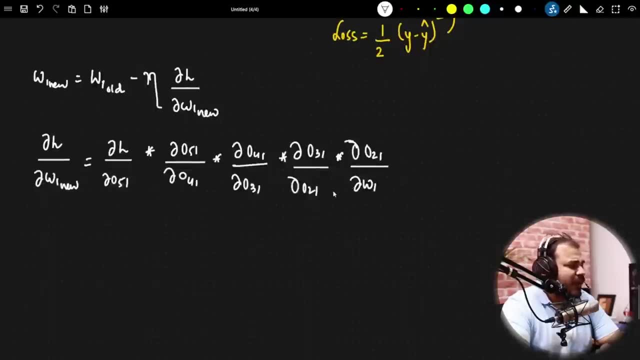 So this will be my chain rule to in order to update W 1 new w1. okay, very much clear. now what will be my next step in this, what, what i have to actually do? now see one thing, very important thing: the kind of activation function we use in each and every layer. 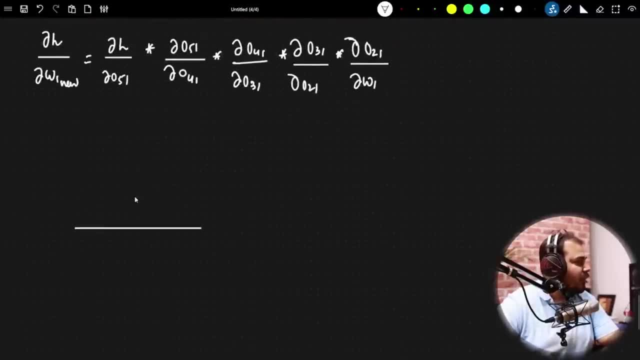 we use an activation function which is called as sigmoid activation function, and i hope everybody knows how what a sigmoid activation function formula is. it is nothing but 1 plus e to the power of minus x. okay, so this is the sigmoid activation formula and we know our output is. 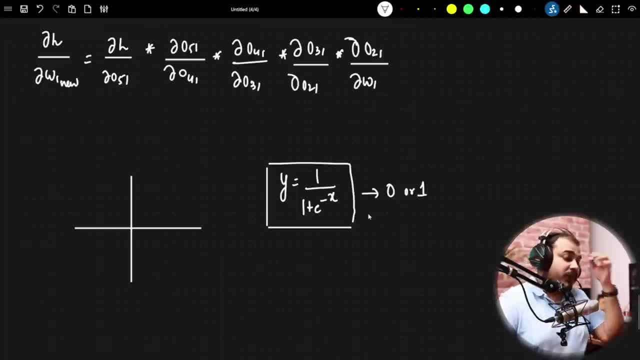 either 0 or 1. okay, 0 or 1, where i specifically say: if it is greater than 0.5, then it is going to be 1, if it is less than 0.5, it is going to be 0. now, let's, let's draw this okay. 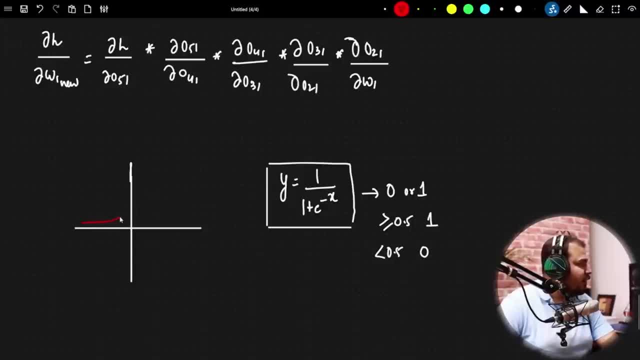 now my sigmoid activation function curve looks something like this: okay, it looks something like this: okay, my value will be between 0 to 1. let's say this is my uh, this is my uh. if i probably say y is equal to w, transpose x plus b: this is my y. okay, this is 0.5. okay, and with. 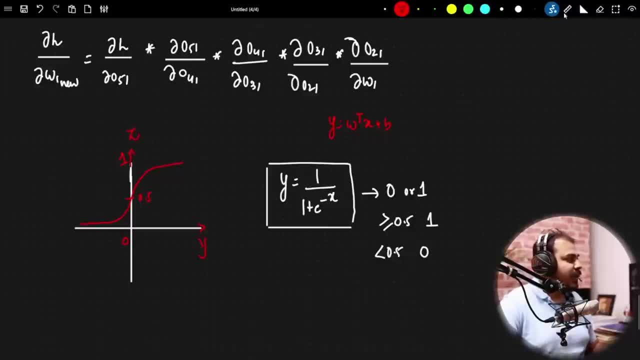 respect to this. this is my uh z value. okay, z i can consider as my up after applying an activation function like this. okay, so it will be. z is equal to okay. this is my z now over here. you know that this will be all your negative values. this will be your positive values. right, this is fine, okay. 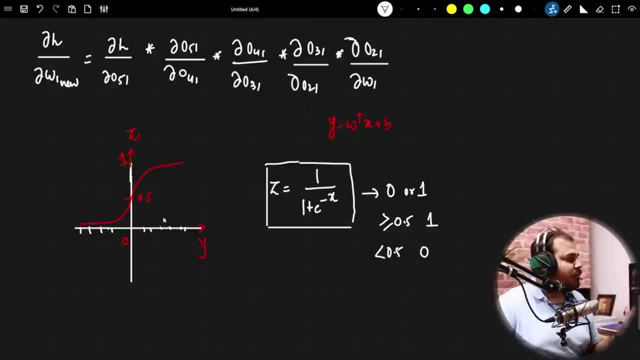 i hope we know about this. one important property of the sigmoid activation function is that it is the derivative of this sigmoid activation function. whenever we try to find out, whenever we try to find out the derivative of sigmoid, it will be ranging between 0 to 0.25. so my derivative curve will be: 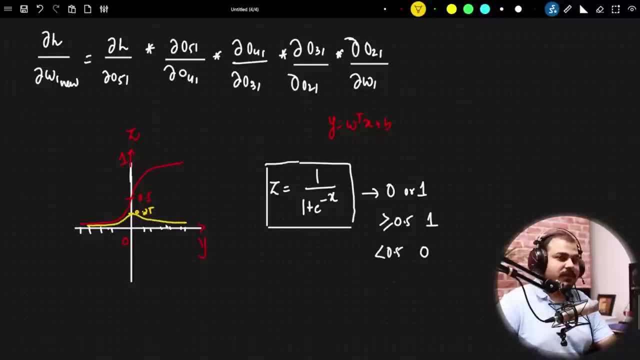 looking like this. okay, it will be looking like this. my derivative curve will be looking like this and it will always be ranging between 0 to 0.25. remember: this yellow line is nothing but derivative. whenever i find out the derivative of this equation, it will always be ranging. 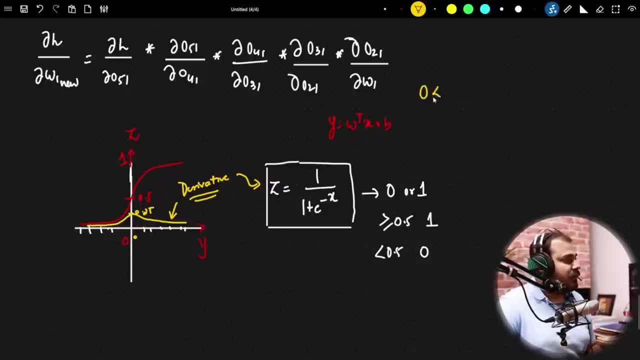 between 0 to 0.25. so if i write 0 is less than or equal to sigmoid of sigmoid of y, okay, is always being ranging between 0 to 0.25. this is basically my derivative condition. okay, so i'm going to basically write it as derivative condition. okay, now, because of this, because of this, okay, because. 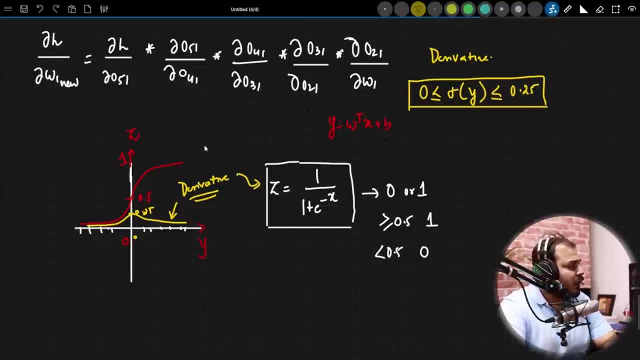 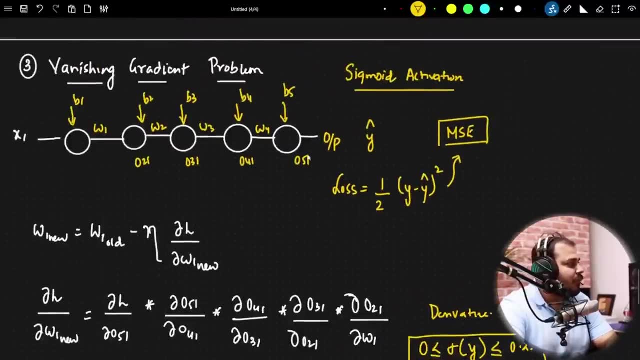 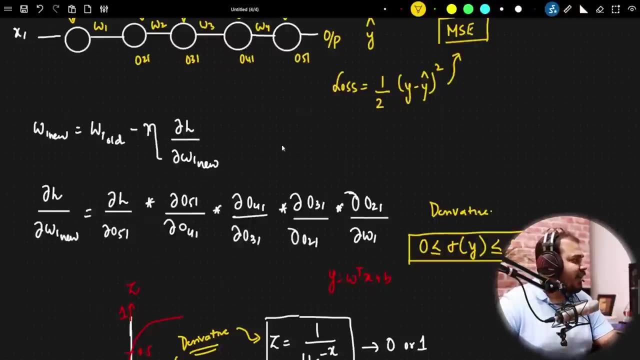 of this, what will happen? just understand over here, if i talk about these derivatives, since i'm taking 041 031 021, 051, can you tell me that in each and every value, sigmoid is getting used? because if i probably take, let's say if i, if i, if i probably take, what is 051? 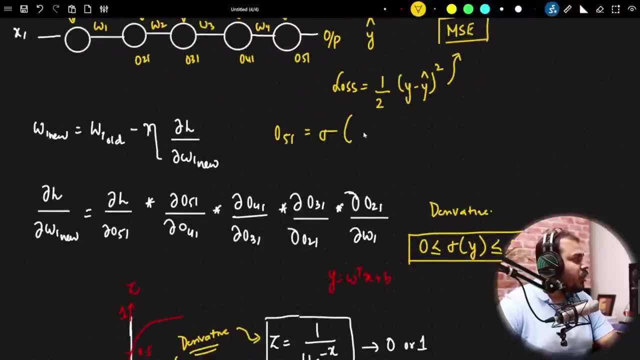 051 is nothing. but we apply an activation function on top of 041 multiplied by w4 and add a bias, so on top of it we apply an activation function. right. so everywhere we are using the same function. so everywhere we are using the same function. so everywhere we are using the same function. 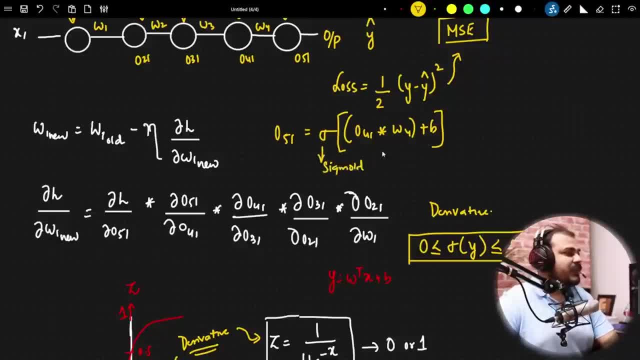 the sigmoid activation function right now, since we are using the sigmoid activation function everywhere in the back propagation. when i'm finding the derivative, tell me the value will always be ranging between 0 to 0.25. right, it will always be ranging between 0 to 0.25. yes, so in the backward. 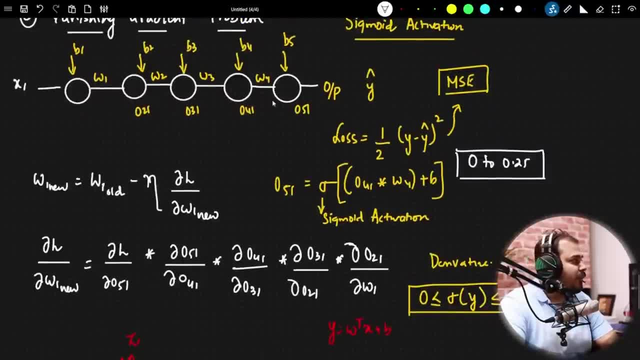 propagation, when i'm finding the derivative with respect to 051, with respect to anything, or 041. everywhere sigmoid activation function is getting used and because of the sigmoid activation function, we have understood that the derivative of sigmoid activation function always ranges between 0 to 0.25.. 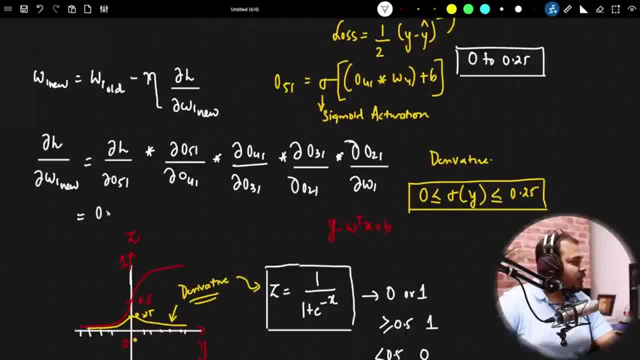 Now what will happen? Now see, in this particular case, let's say for this my derivative, I got it as 0.25.. Let's take as an example. Let's take as an example because anyhow, my values will be ranging between 0 to 0.25 and 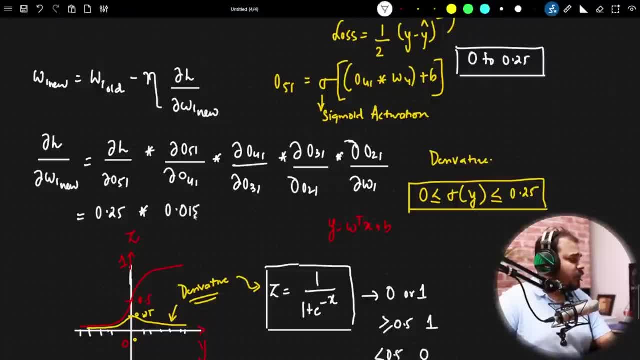 it will be like that that I keep on updating these values and this value will keep on decreasing somewhere. It will keep on decreasing like, let's say, 0.10, then 0.05,, then 0.02, then like this: 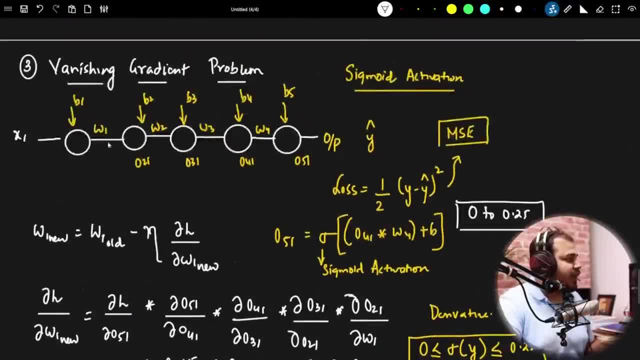 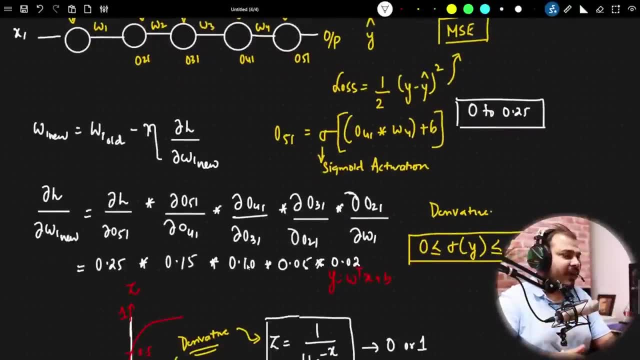 it will keep on decreasing because, as we are going to this chain rule, as we are going to calculate the derivative, always we are trying to get this particular value and it is always going to get reduced till we go to the end of the chain. 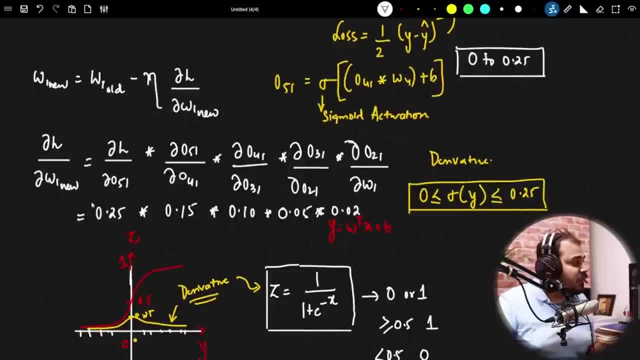 Now one very important thing: what will happen because of this? Since we are multiplying with smaller values, don't you think we will be able to get a very small value? okay, We will be getting a very small value. The answer is yes, we will definitely be getting a very small value. 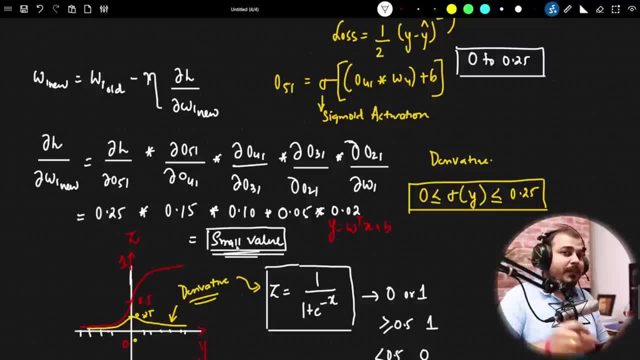 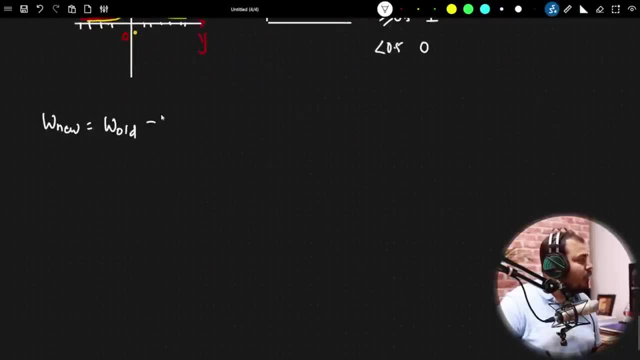 Now what happens if we get a very small value over here? What happens if we get a very small value? I will go and update my weight formula. no, So now it will be: W new is equal to W old, minus learning rate, which is again a small. 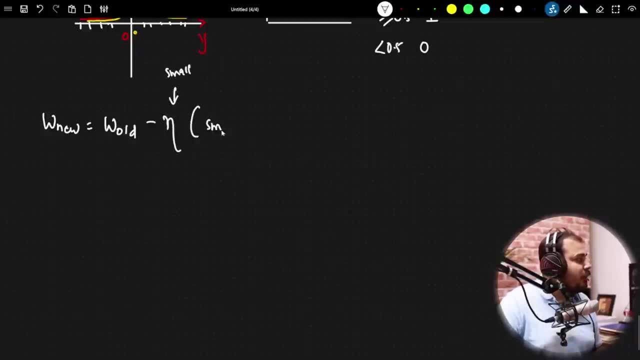 number, which is again a small number, multiplied by a small number. Now, when I multiply this small number, then what will happen? What will happen with this small number? This at one point of time, let's say at one point of time. suppose, if I say this, W new. 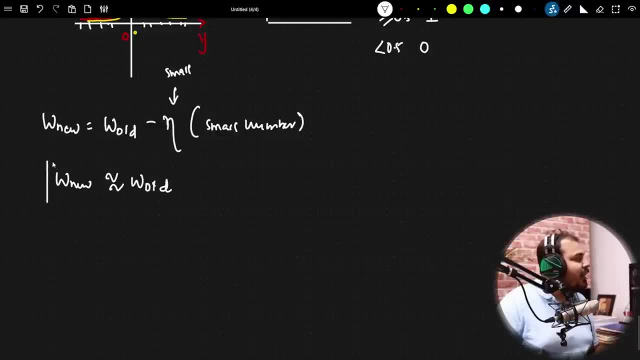 will be approximately equal to W old. It will hardly change. And if it is hardly changing, then what is basically happening? Weights are not getting updated And this situation where weights are not getting updated or it is just getting updated by a smaller value. 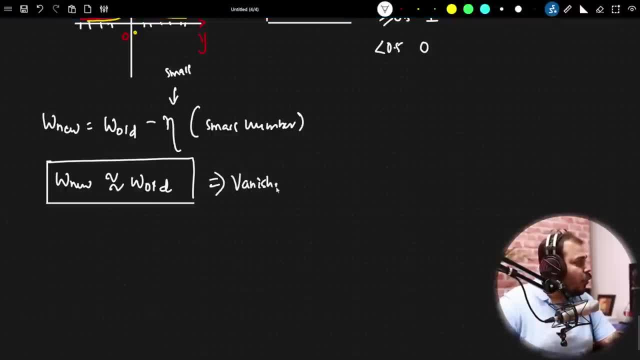 Okay, This problem is basically called as a vanishing gradient problem. This is called as a vanishing gradient problem. Now, how to solve this vanishing gradient problem? It is approximately equal right, My W new and W old are approximately equal. 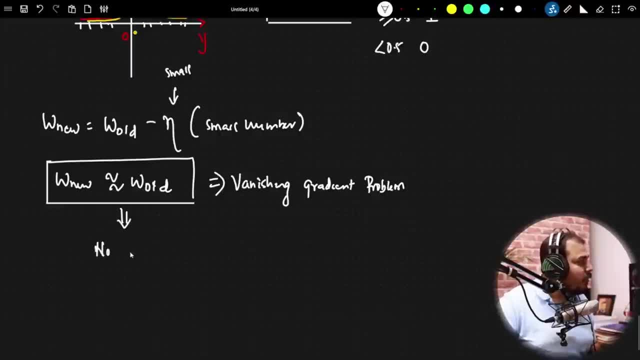 And that is the reason. over here, no change in the weights are happening, No change in weights, And this specifically thing is called as vanishing gradient problem. And how to basically solve this? Use another activation function. Use another activation function. That is the reason why we came up with another activation function. 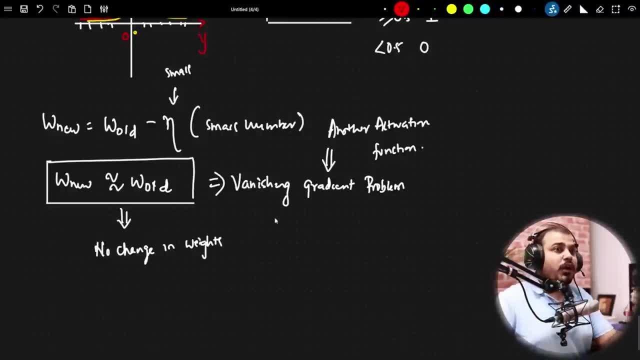 There are so many different kind of activation function. Now let me note down all the activation functions that we are going to learn after this. The first activation function I hope everybody knows about it is nothing but sigmoid. But the second activation function that we are going to learn is tanh. 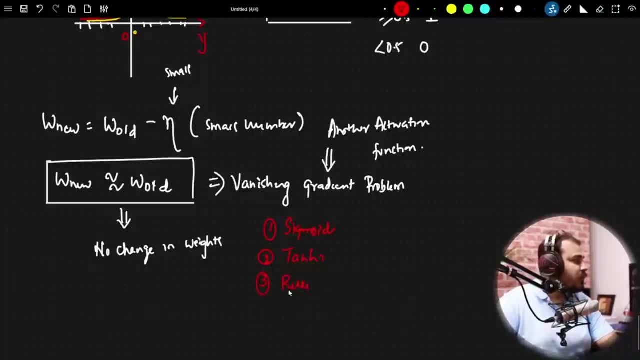 Okay, Which will discuss about. Third activation function which we are going to discuss about is ReLU. then, fourth activation function we'll discuss about is pre relu, like leaky relu- sorry, not pre relu, it is leaky relu, leaky relu. and similarly we will be. 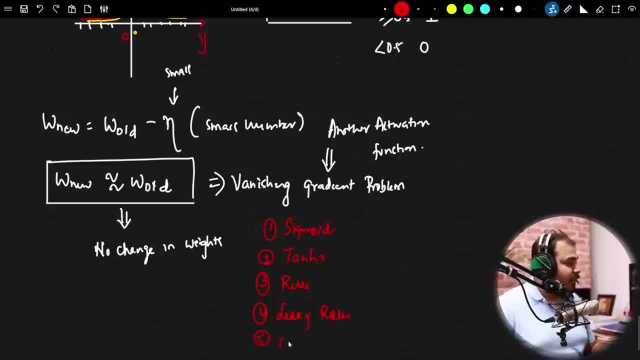 discussing about pre relu, pre relu and different, different activation functions. okay, so let's go ahead and let's try to see about the activation function and what is the best activation function we can actually use that we are going to see. okay, so I'm going to share my screen with you again, a proper screen. 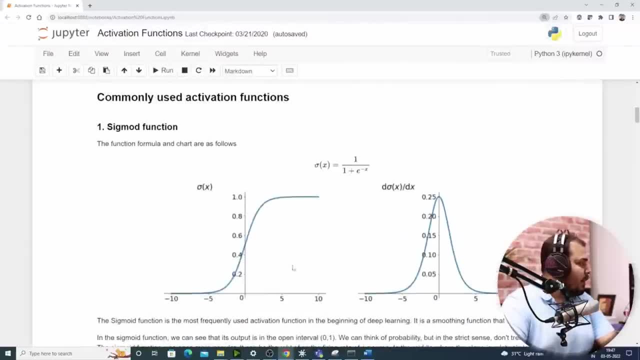 okay, so this is my sigmoid activation function. okay, so let me open another pen for you so that I can write on top of it. okay, but can I get a quick confirmation? you are able to understand everything? yes, you are able to understand everything, or not very much clearly. yeah, 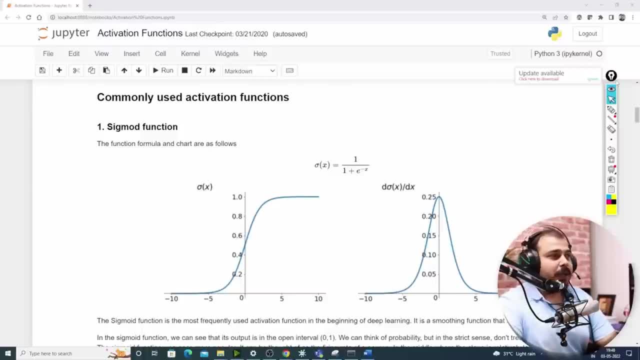 yes, okay now, if you are able to understand, as usual, as I always say, please hit like, and that will actually boost my energy. okay, and it will help me to teach you much better, okay, okay, now let's go ahead for discussing the first activation function, which is called a sigmoid. I've told you 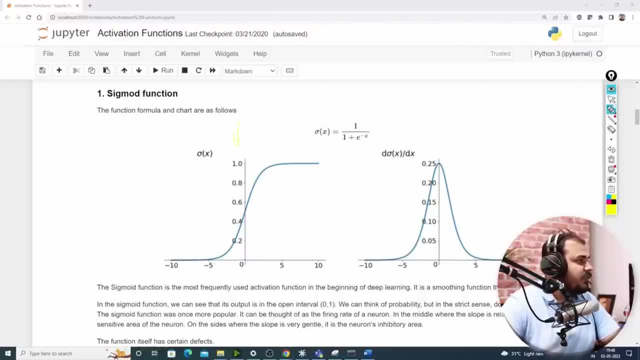 in the left hand side that you basically see. this is the functionality. this is the functionality of the activation function on the left hand side. this is basically the derivative. okay, this is basically the derivative whenever we are doing the back propagation. so in the activation function- sigma activation function- we have seen it will be. 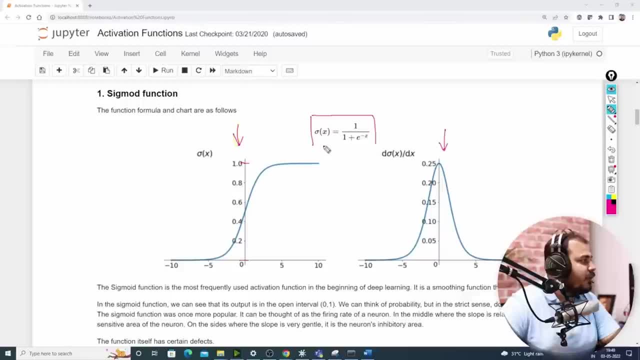 ranging between 0 to 1, and this is the formula which we have already seen. if i want to find out the derivative of sigma activation function, it will be ranging between 0 to 0.25, because of which vanishing gradient problem exists. vanishing gradient problem exists. this we have clearly. 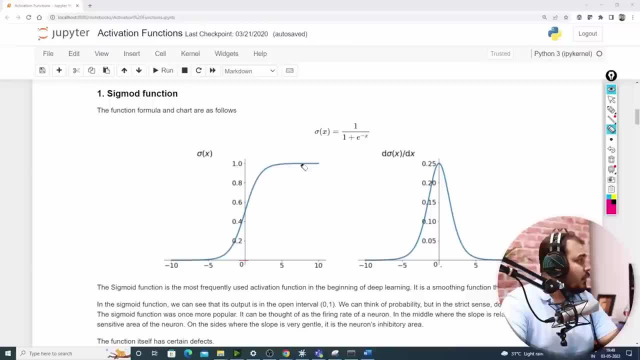 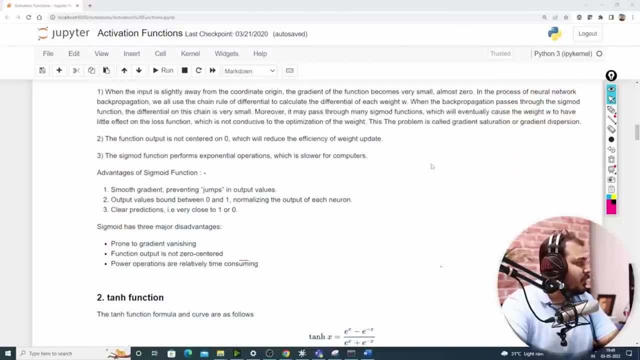 understood, okay, and this is a major issue over here. so there you can basically check out. okay, now let's understand some of the important properties of sigmoid activation function. okay, what all things are there and, based on that, what all disadvantage are there. we'll try to understand, okay. so now, first thing: advantages of sigmoid activation function. 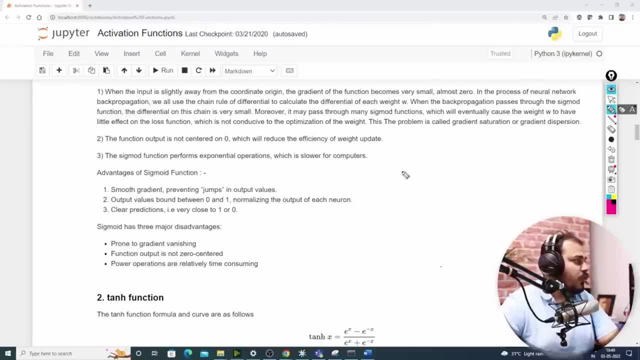 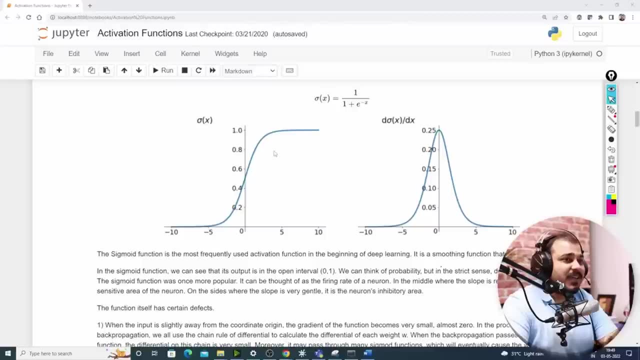 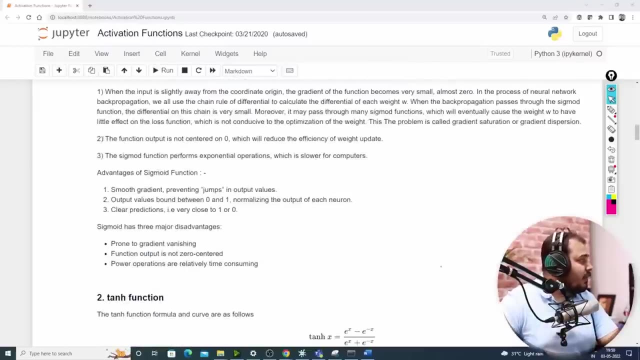 smooth gradient prevent jump in output value. so you know that here in the sigmoid activation function we have the smooth gradient right. so because of this, the convergence will be quickly done and will help us to work in a better way. okay, but always remember this point: the input, the 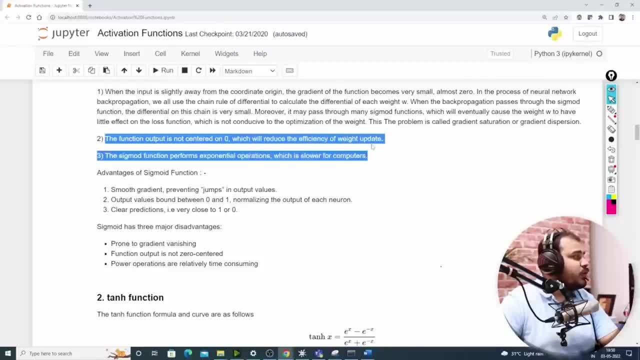 function output is not centered on 0, which will reduce the efficiency of the weight update. now, what is this? centered, not zero. now, see, guys, suppose, if i want to do a conversion function and i want to do a conversion function, and i want to do a conversion function and i want to do a conversion function, 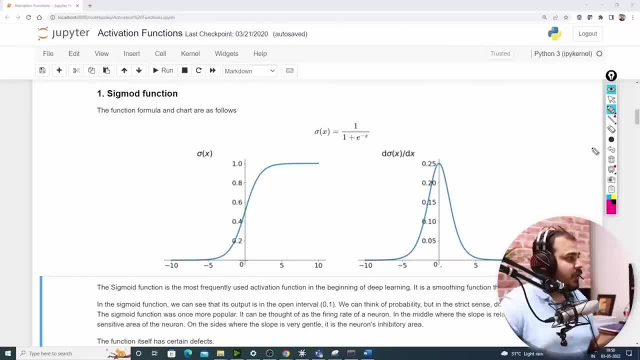 if i have a curve. if i have a curve, let's say, uh, if i have a curve which looks like this when i say it is centered to zero, suppose, if there is a curve that passes which, which passes like this, which passes through the mean, that is zero, which passes through the 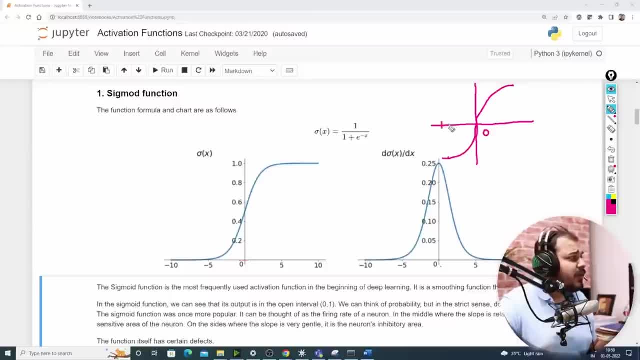 origin. okay, and over here you can see that there will be negative values. there will be positive values also, right during this particular scenario, we say this curve as zero centered curve, zero centered curve, okay. so whenever we have a zero centered curve, the weight updation becomes very much easy. okay, it? it efficiently updates the weight. okay, so in this, 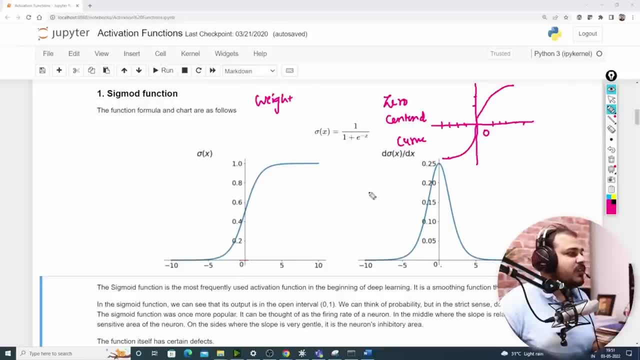 particular case, it is not passing through zero, so definitely, this is not zero centered. okay, that is the exact meaning of zero center, perfect. so if you have understood till here, i hope, uh, we'll go to the next step and we'll try to understand that. this advantage also in terms of the weight update. 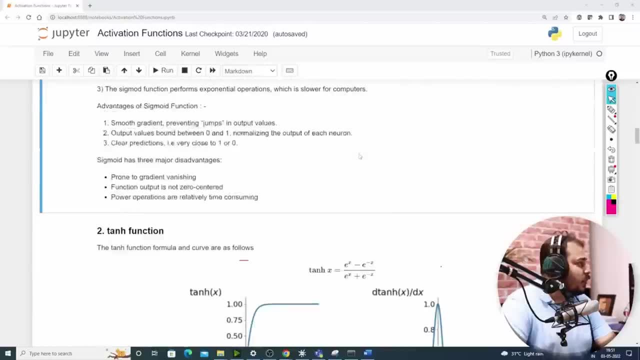 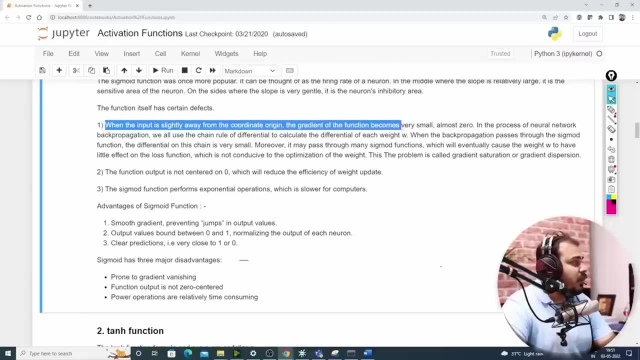 into this and i will be giving you this material so that you can read it through it. okay, now, when the input slightly, is slightly away from the coordinate origin, the gradient of the function becomes very small. that is almost zero. okay, this is what i talked, spoken about right in the back. 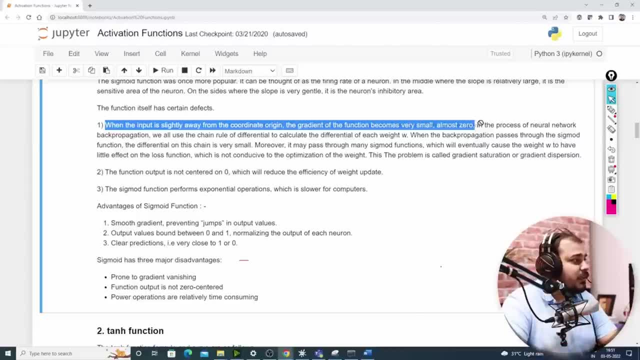 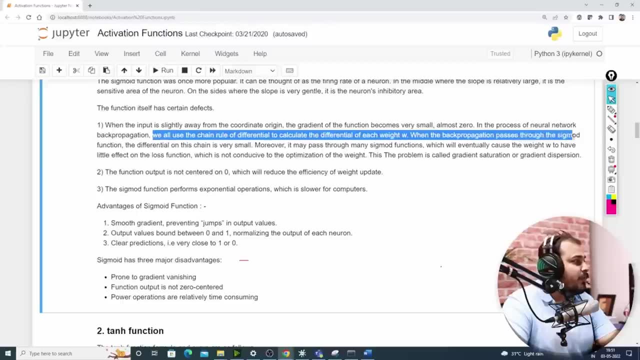 propagation, right back propagation. so here you can see, in the process of neural network back propagation we all use chain rule of differential to calculate the differential of each weight. when the back propagation passes through the sigmoid function the differential on the chain is very small and because of that vanishing gradient problem. 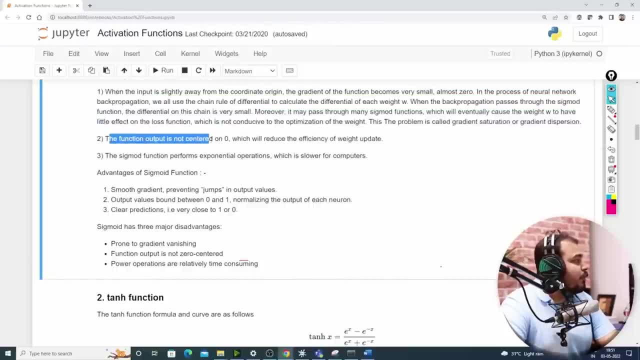 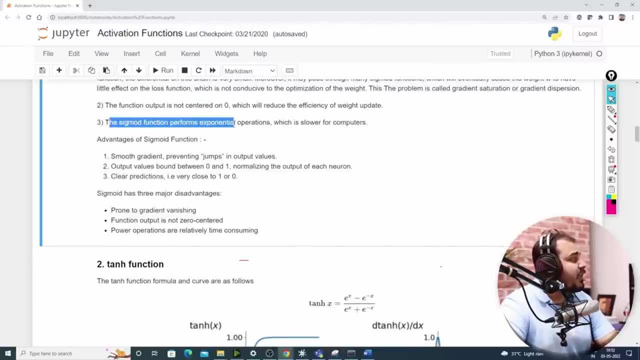 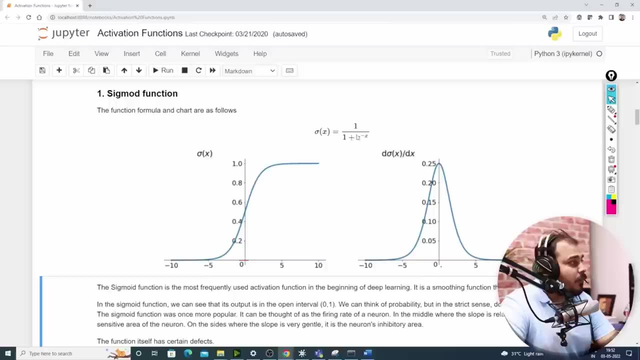 exists. okay, now the function output is not zero, centered on zero, which will reduce the efficiency of weight. update this also. i've actually told you. the sigmoid function performs exponentially operation, which is slower for computers. now, what is this exponential operation? this is the operation that is there. the formula for sigmoid is nothing but one plus one, uh, one divided by one plus e to 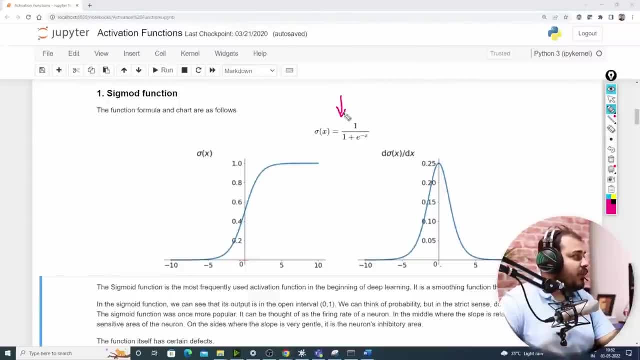 the power of minus x. this is exactly an exponential function and whenever we need to perform this operation, it takes time. the time complexity increases, since there is an exponential function. okay, so this is a major issue. some of the issues with respect to sigmoid activation function. okay, now let's go to. 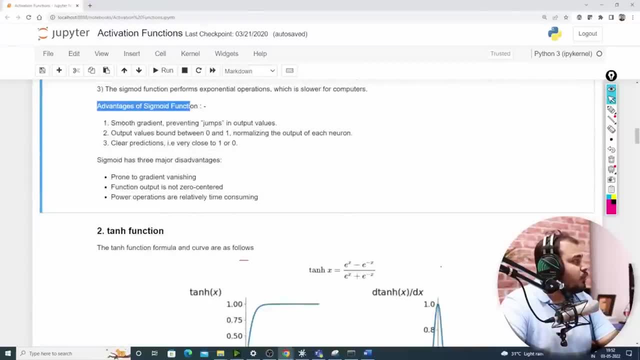 the next one, sigmoid. what are the advantages of sigmoid? smoother gradient, prevent jumping output values between zero and one, so normalizing the output of each neuron. clear prediction when a signal is very close to one or zero. this all our things. are there here. you see major three. 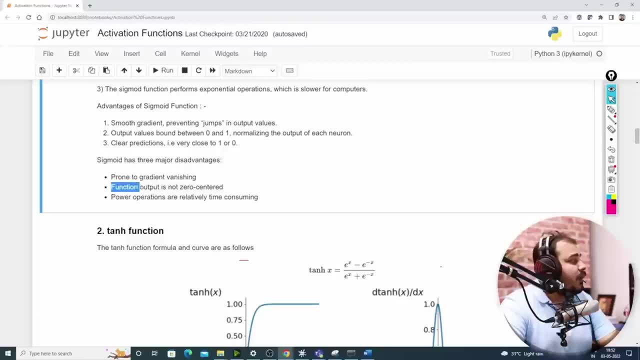 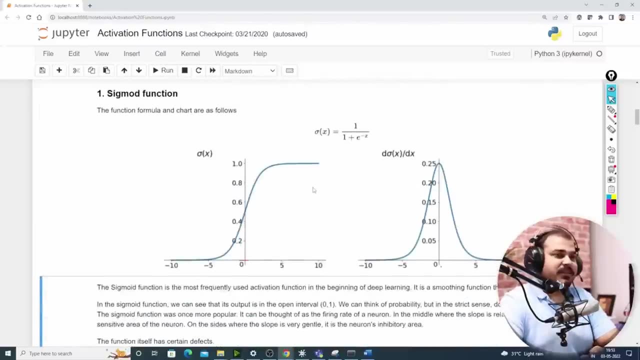 disadvantage. it is prone to gradient descent. uh sorry, gradient vanishing. function output is not zero. centered power operation are relatively time consuming. now, in order to prevent this, the researchers will not keep quiet because obviously, uh, if there is a vanishing gradient problem, we cannot create a deep neural network. right, we cannot do this. we cannot create a deep neural network. it. 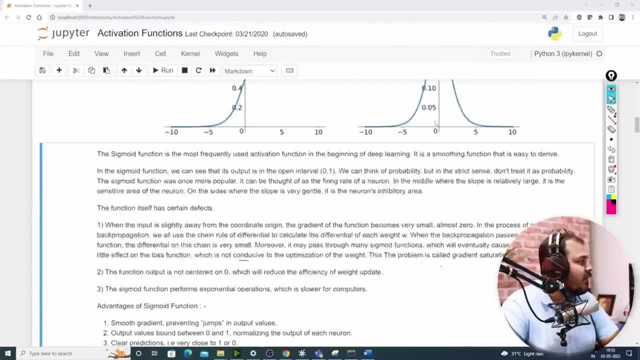 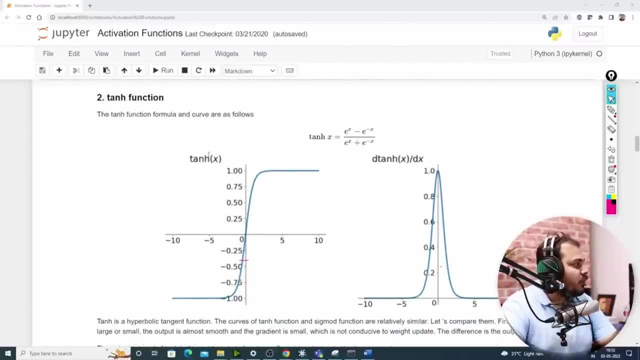 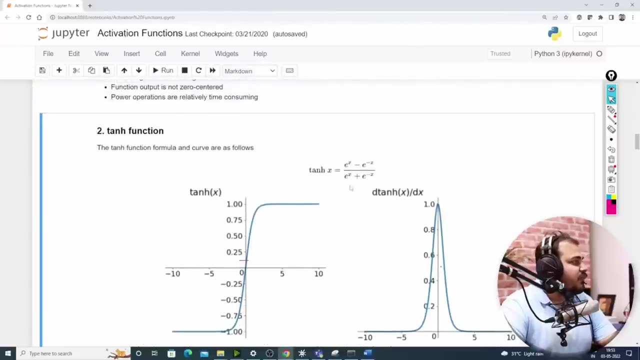 is very, very difficult. so what do we do in this particular case? so here i will go down now. now the second activation function that we usually use is something called as tan h. okay, tan h, uh. it is also called as hyperbolic tangent function. now, in hyperbolic tangent function, the formula looks: 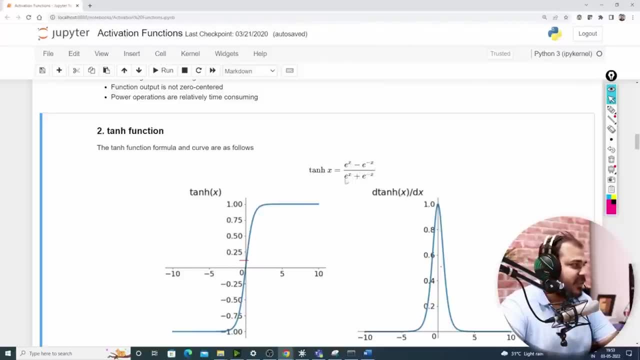 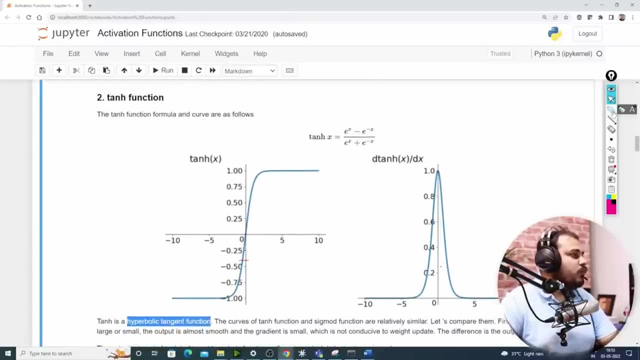 something like this: e to the power of x minus, e to the power of minus x, divided by e to the power of x plus, e to the power of minus x. now here you can see that my value, two main important- my value ranges between minus one to plus one in tan h function whenever i apply a tan h activation. 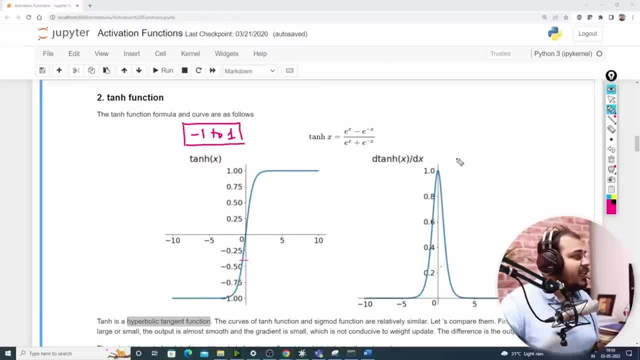 function, my value will be ranging between minus one to plus one and in the case of derivative, it will be ranging between zero to one right in the derivative side. yes, anytime we find out the derivative, it will be ranging between zero to one right. in the previous case, when we were using 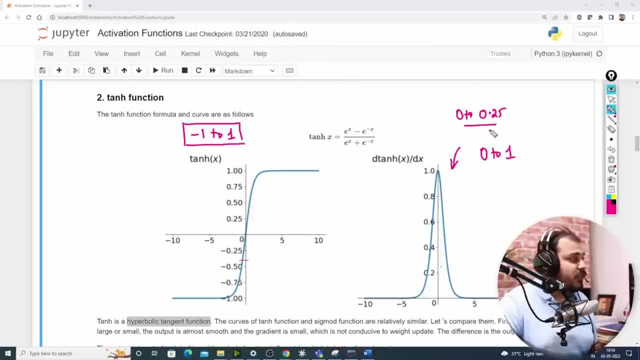 sigmoid. there it was ranging between zero to point to five right, which is pretty much better now because my value is basically ranging between zero to one right. does this prevent vanishing gradient problem? still, there will be a issue, right guys, if we go on constructing a deep neural network- deep, deep neural network- at one point of time there. 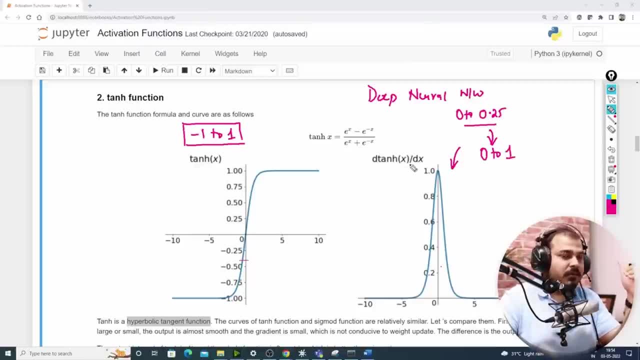 may be chances that vanishing gradient problem still exists right, so because of that we should also not use tan h function. but this was the second activation function that researcher came up with, because the first activation function still had that issue and this had issues of vanishing gradient. 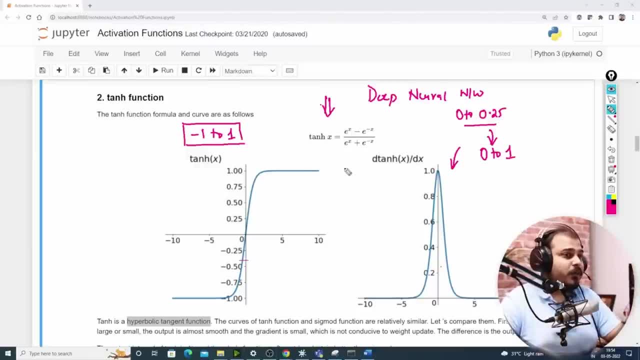 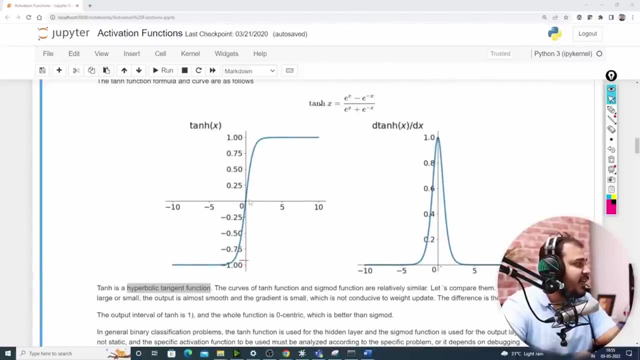 but after, uh, when we are actually constructing a very deep neural network. okay, so i hope everybody has understood this specific thing. okay, and please remember the formula, the derivative. whenever you try to find out the derivative of this curve, you'll always be getting the value between 0 to 1. okay, this is zero centric. see that zero centric problem is also solved over here. this: 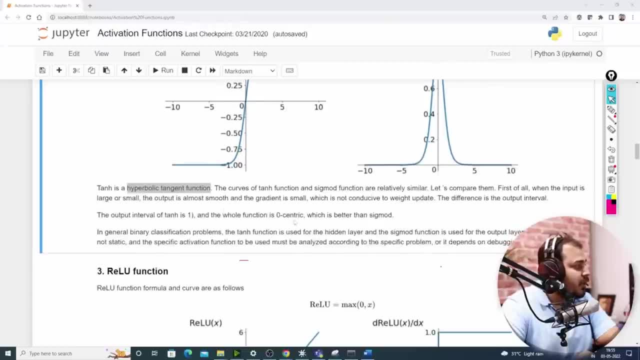 is also having zero centric, which is better than sigmoid. it is written over here: okay, so tan h is a hyperbolic tangent function. the curves of tan h function and sigmoid function are very relatively smaller. let's compare them. first of all, when the input is larger, the output is also smooth. the 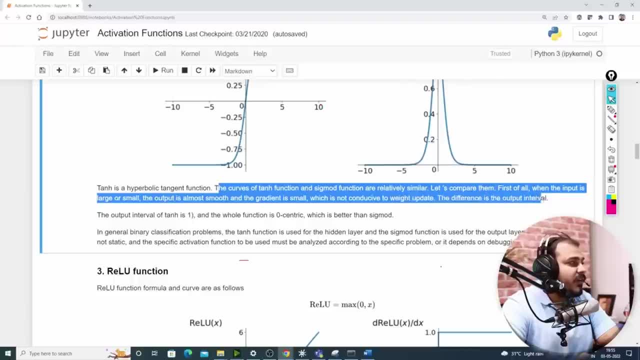 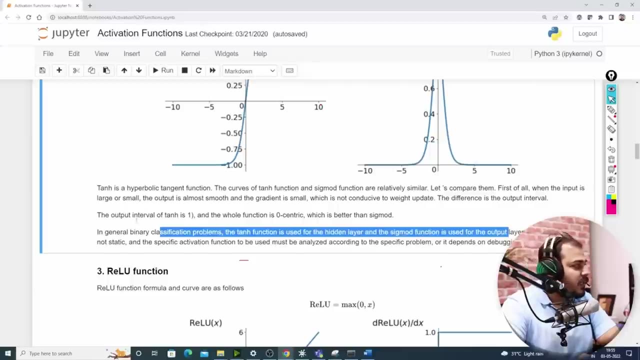 gradient is small, which is conducive to weight update. the difference is the output interval, uh, the whole zero centric, which is better than sigmoid. in binary classification problem we basically use tan, tan h functions for the hidden layer and sigmoid for the output layer. okay, so i hope everybody is able to understand. but still, i said that there will be chances of 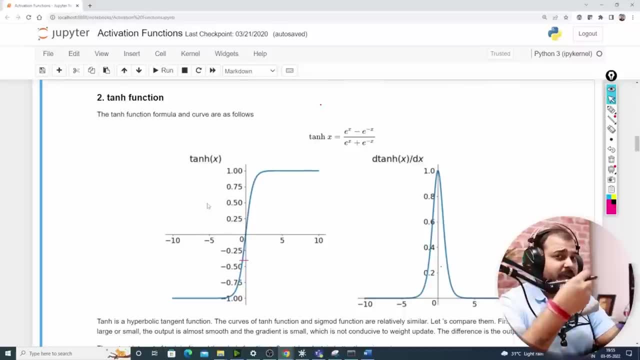 vanishing gradient problem. so now, what we do? what do we do? we cannot keep quiet. there will be another researcher who will be doing his PhD, so he has to come up with new equations and he has to come up with new research. and probably the next activation- 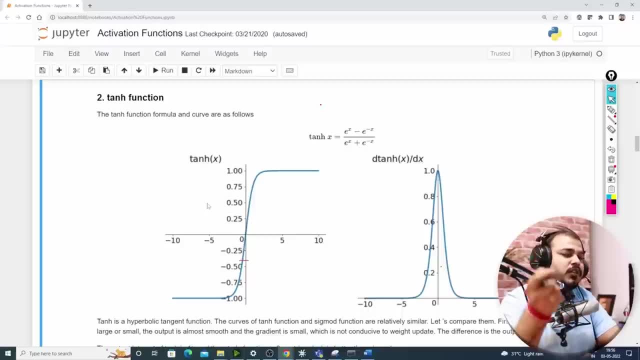 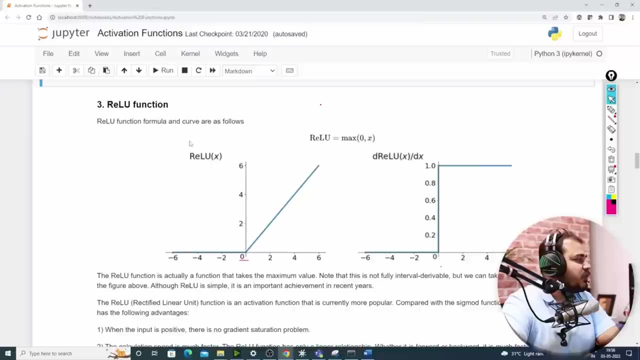 function is an amazing activation function and right now it is the most popular activation function which is being used by everyone without any knowledge. if that person does not have any knowledge also, then also he'll be using that activation function and that activation function is nothing but ReLU. okay, ReLU activation function or ReLU activation function for full form is rectified. 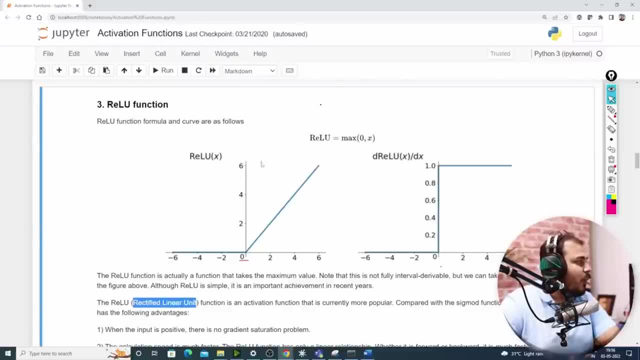 unit which you can see over here: rectified linear unit. over here the formula is nothing but max 0, x. either it will be 0 or whatever value the x is. if the x value is negative, then it will be 0. okay, whenever the x value is. 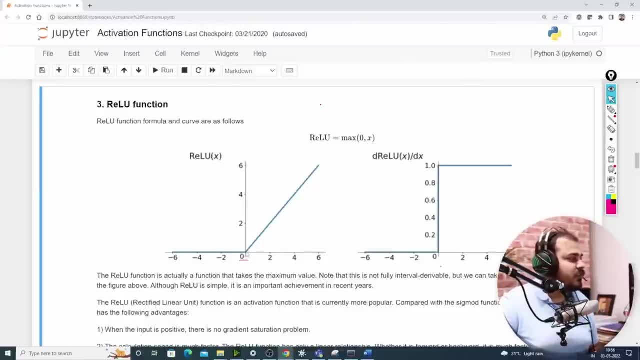 negative. whenever we apply this ReLU activation function on top of it, it becomes 0. whenever it is positive, it will come to that same positive value. suppose if the x value is 1, then I'm going to get 1. if the x value is 2, I'm. 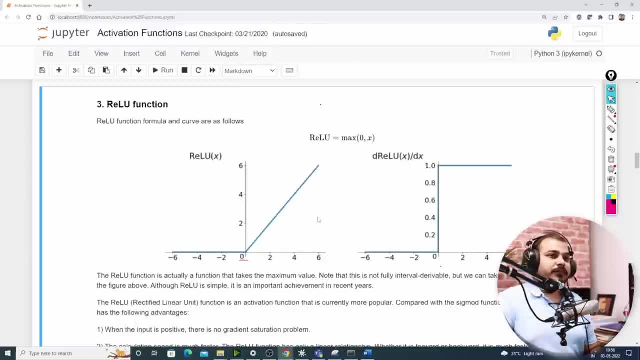 going to get 2. if the x value is 3, I'm going to get 3, right, so this is pretty much amazing. and whenever I try to find out the derivative of ReLU, the value is either 0 or 1. okay, 0 or 1. now this is again a. 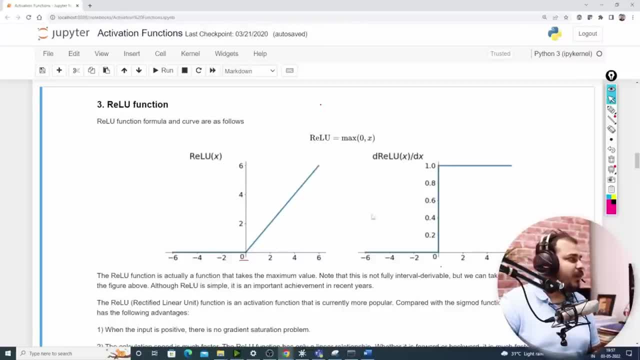 major concern, guys, because let's say, if one of the weights during the derivative right, when we are updating the weights, if it becomes 0, this neuron, the neurons that I have, right suppose let's say this is my hidden layer 1 neuron, this will become dead dead. 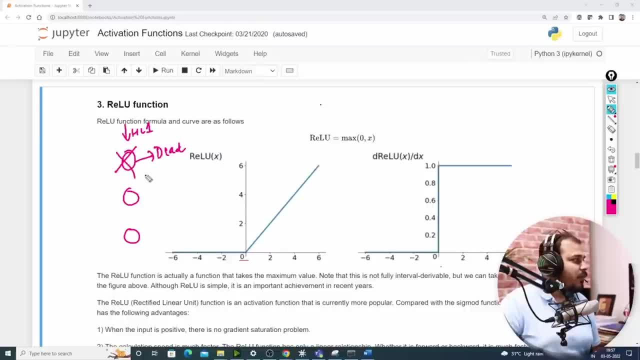 during the back propagation. right, in the forward propagation. also in the forward propagation is fine, it will not do anything. but in the back propagation also. when I am trying to find out a derivative, the value is either 0 or 1. right, the value is either 0 or 1. if it becomes 0 in the back propagation, that. 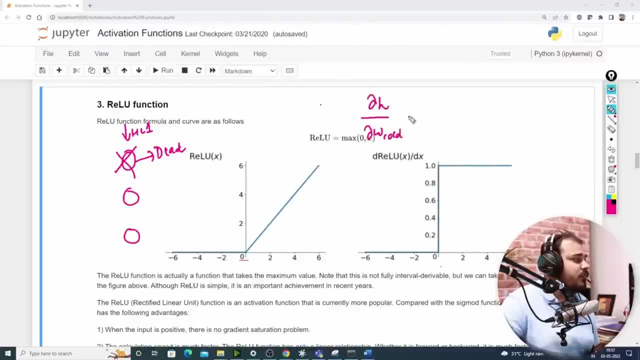 entire derivative chain rule right, this will become 0 right. when this is becoming 0, W new will be approximately equal to W old. right this will be approximately equal to 0. that basically means that neuron will be completely dead. this is one disadvantage of ReLU activation function other than. 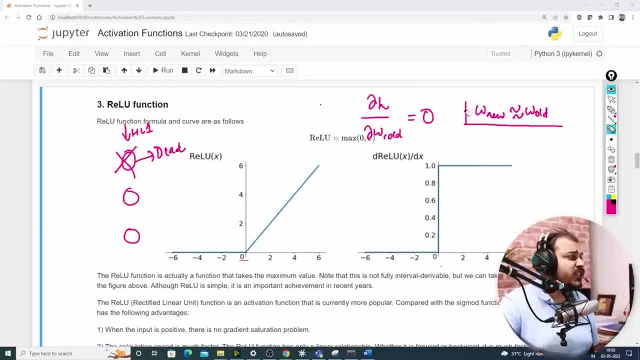 that this is solving or this is doing an exceptional, exceptional performance, because over here- just imagine the over here- you don't have any exponential operation. also, here you just have this simple operation, which is pretty much quicker than the previous one. okay, so here you don't have any, it is. 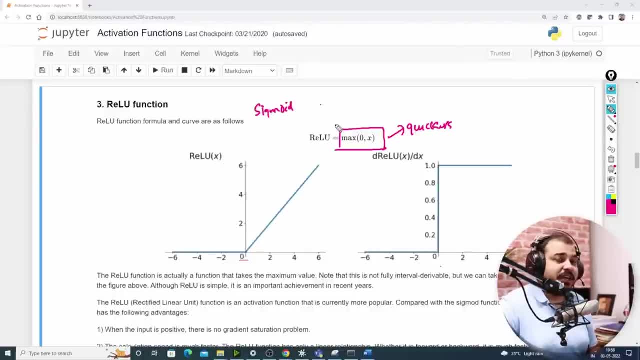 obviously a very simple operation which is pretty much quicker than the previous one. okay, so here you don't have any. it is obviously better than sigmoid. it is obviously solving the vanishing gradient problem. it is obviously solving the other problems that it had. it is also solving 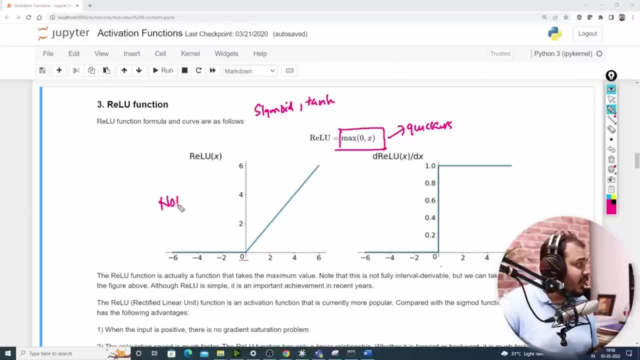 the tanh function problem. it is not zero centric. it is not zero centric over here, just see, it is just passing through zero, but we are not getting any negative values. it is not zero centric. this is only the one disadvantage that it has, other than that everything that it has it has better than sigmoid and tanh. 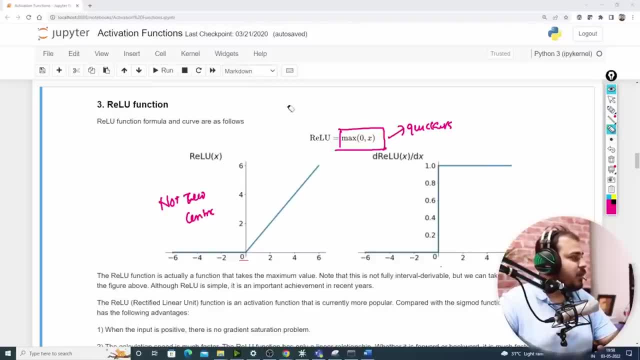 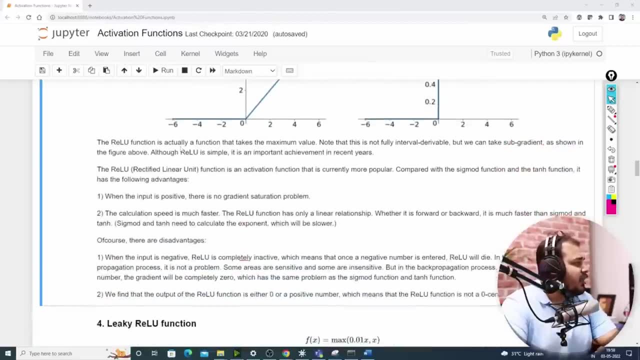 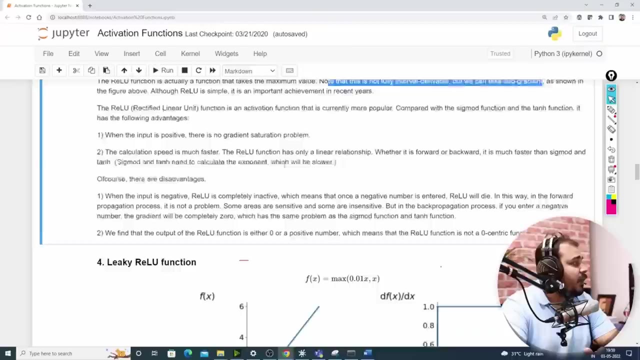 activation function. okay, so I hope you are able to understand this part also where we have specifically discussed about ReLU activation function. now let's read about it. a ReLU function is actually a function that takes the maximum value. note that this is not fully interval variable we have. we can take sub gradient. it is an activation function. 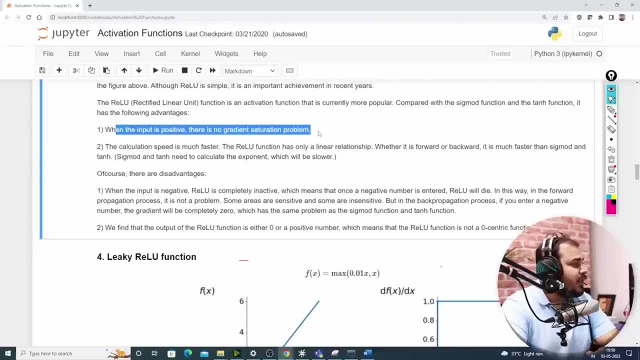 that is currently more popular. when the input is positive, there is no gradient saturation problem. the calculation speed is much more faster. the ReLU function has a linear relationship, whether it is forward or backward. it is much faster than sigmoid and tanh. okay, they are some disadvantage. when the input is negative, ReLU is completely inactive. 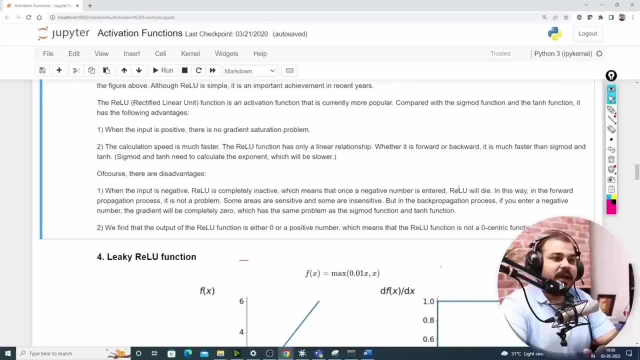 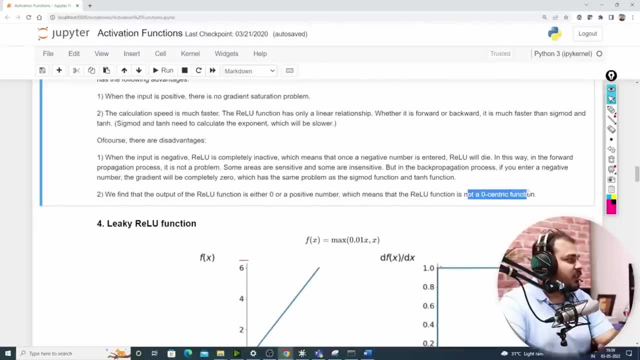 which means once a negative number is entered, ReLU will die. okay, ReLU will die okay. so, and it is also not zero centric. so you can. I will be giving you this entire materials in the description, probably after the session. you can check it out. okay, now, in order to solve this dead ReLU or dead neuron, okay, we have. 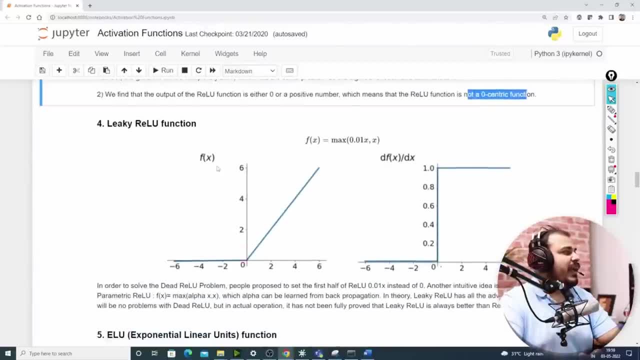 another activation function which we call it as leaky ReLU function. and this is a function which we call it as leaky ReLU function, and only one thing is basically getting changed, where they are not saying that it will be zero, but it will be point zero, one multiplied by that X value. so now my 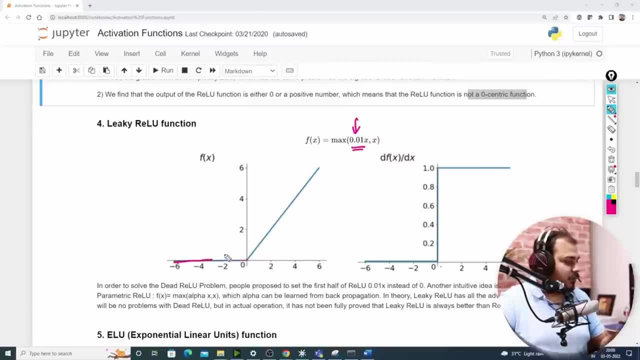 value will be little bit coming like this in leaky ReLU: see, in leaky ReLU, it will be something coming like this and it will be going like this now, in this particular case, I will be having some negative values. it will never be zero in. 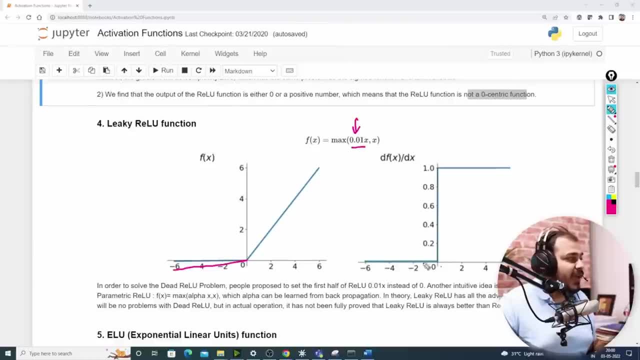 this particular case. also, whenever I am trying to find out a derivative, it will never be zero and it will be a small number over here, you can see, over here and over here. right? so this is important, right, this is specifically supported. so leaky ReLU function solves the dead neuron problem. dead neuron problem: that 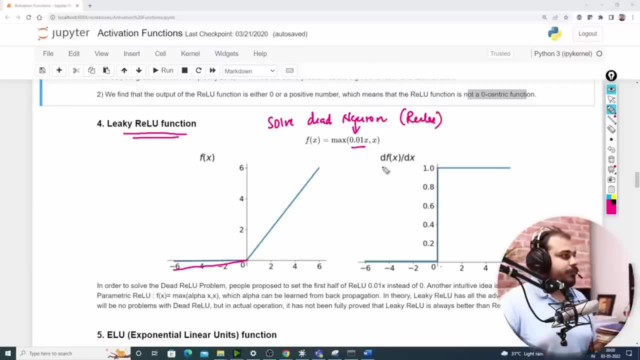 was basically happening in ReLU. okay, I hope everybody is able to understand very much, simply. okay, so remember this formula and then we will be able to understand this. perfect. so, and then I'll also tell you which which activation function you should use blindly, for what kind of scenario you have to use blindly everything I will. 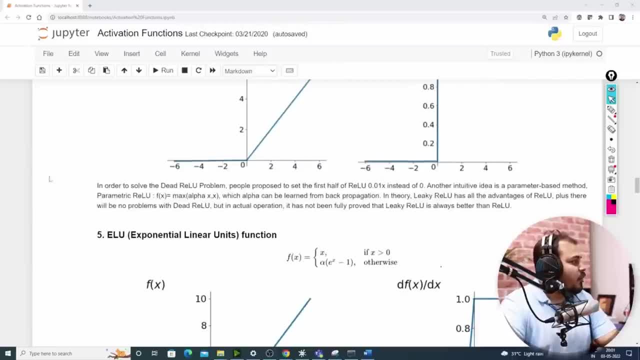 talk about it once I complete all this activation function. so, in order to solve the dead ReLU problem, people propose to set the first half of the ReLU as 0.01 X instead of 0. other intuitive idea is a parameter based method where we can also 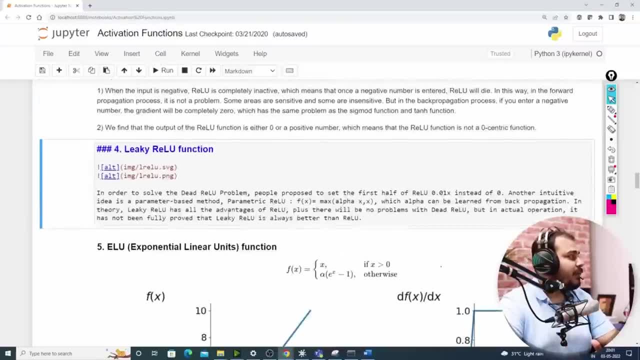 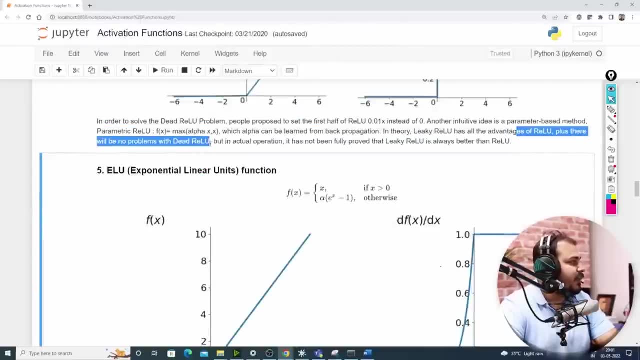 supply parameters, not only 0.01, but some other parameters also. okay, so here it is in theory leaky. ReLU has the advantages of ReLU, plus there will be no problem with dead ReLU. but actual operation it is not fully proved. they are also saying that it is not fully proved, but 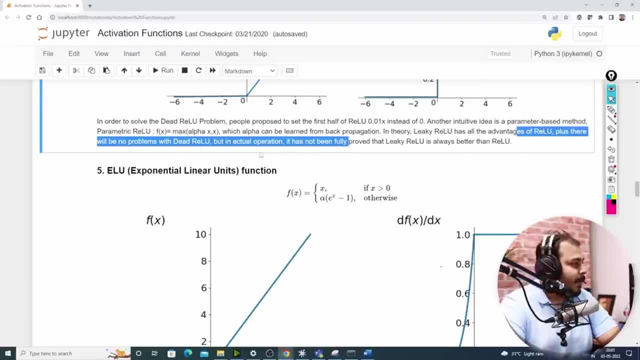 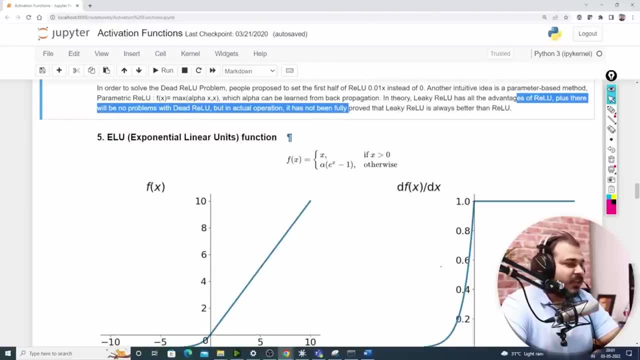 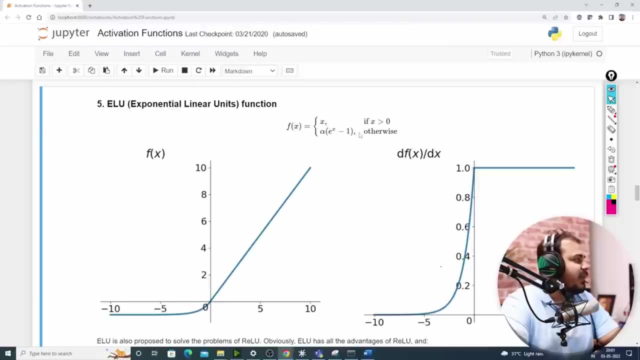 yes, people use that specific option also. okay, now let's go to the next step, which is called as exponential linear units. okay now, in exponential linear units, we have a different formula. whenever the x value is greater than zero, we have x, otherwise we apply this particular operation. 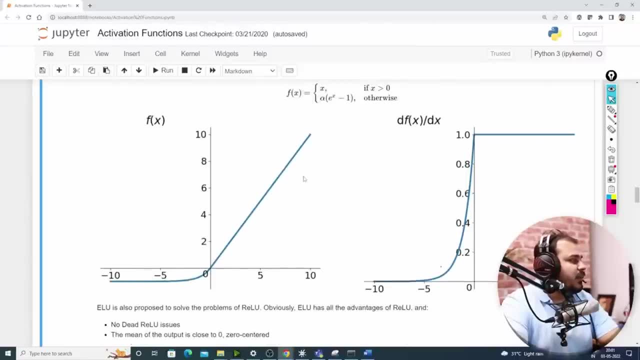 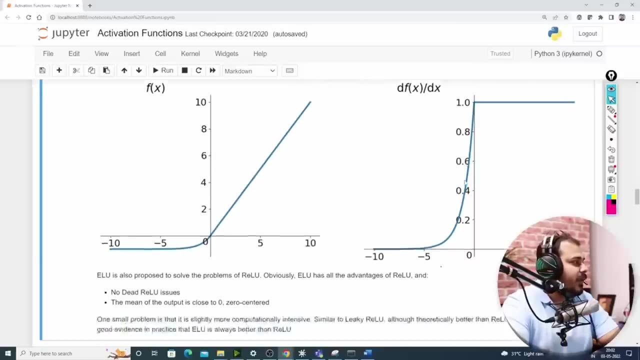 over there. so we will be getting this kind of curve, but always remember, in the derivative also, you can see we are also able to get this exponential curve and again the value will be ranging between zero to one. again, no dead relu issue. this means the output is close to zero, zero centered one. 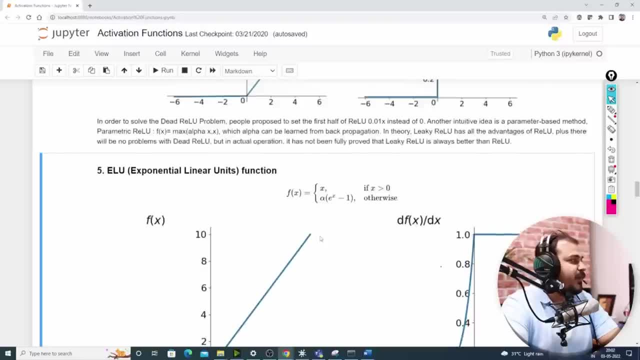 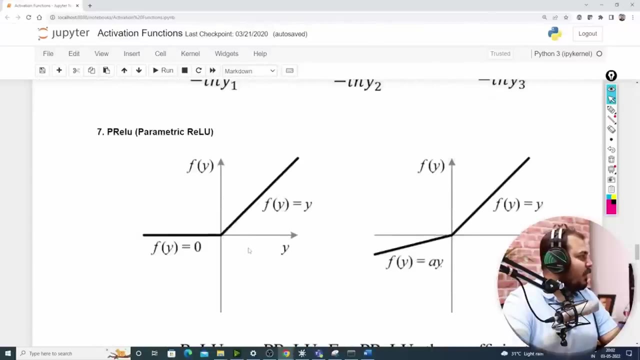 small problem that it is slightly more expensive, computationally expensive, because we are using exponential value. okay, only this. many things are there. they are small, minute, minute changes which people do use. softmax will discuss this in activation function. but let's see one more. there is also something called as pre relu. Pre Relu, just by 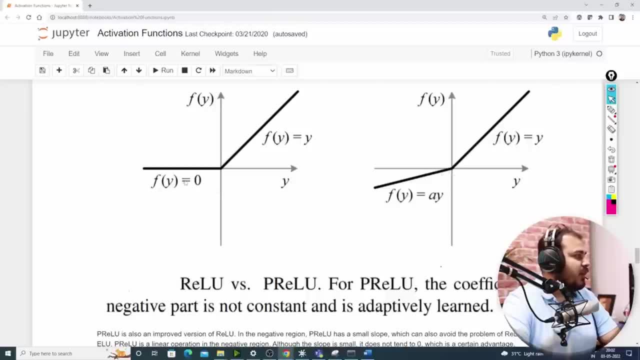 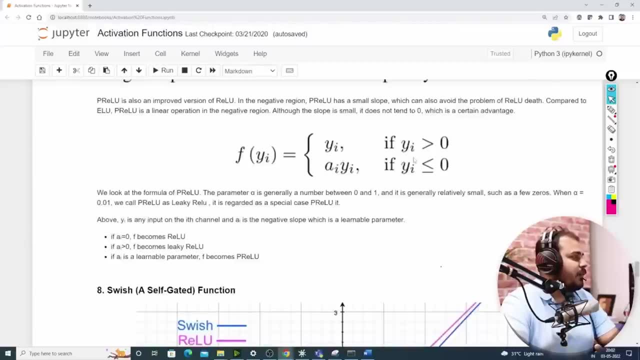 seeing the diagram, you will be able to understand what we are they're trying to do, okay. so instead of radically having this, we will be having in this way, okay, which solves the problem. okay? so here W is greater than zero. if it is less than, or is equal. 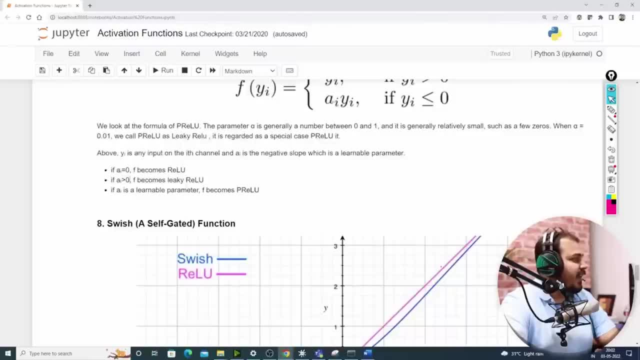 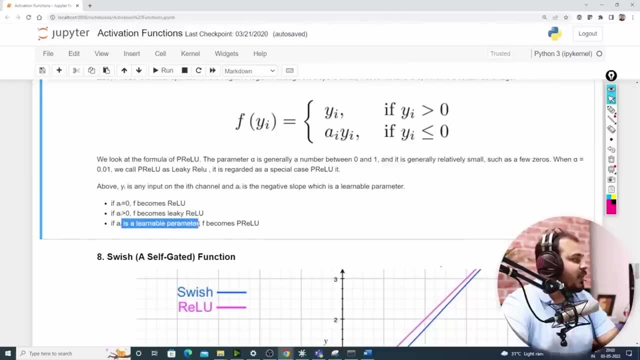 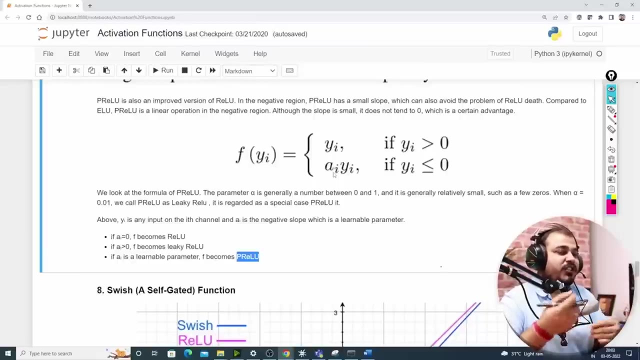 to zero. we are, we multiply a constant. okay, so if A is zero, it becomes relu. if A is greater than zero, it becomes leaky Relu if A is Ler. So in learnable parameters, this will keep on changing. okay, this will keep on changing. 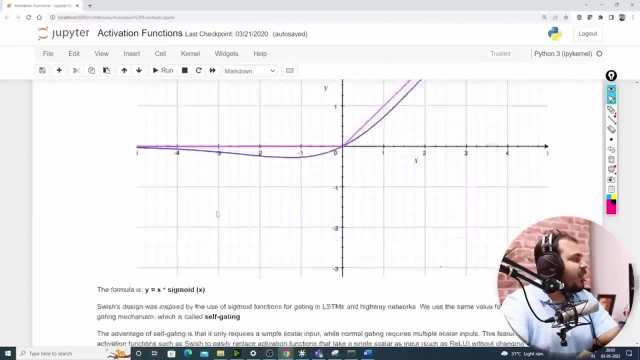 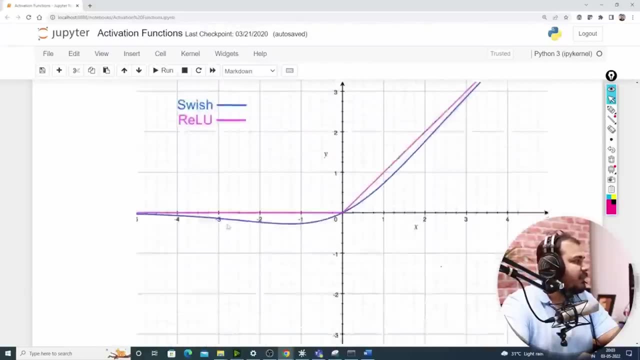 That is the only difference. And then there is also another activation function which is called a switch, a self-gated function. I think this is brought by Google itself. Another activation function over here shows switch and relu. In this particular case, we have this kind of curve. 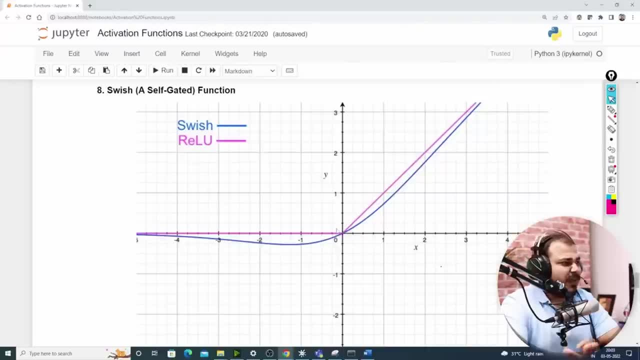 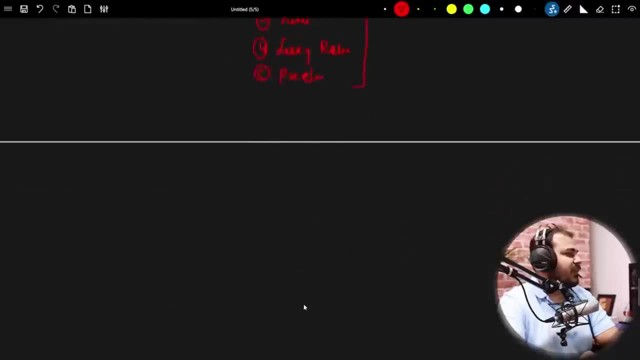 One problem is that we cannot find out a derivative of zero. okay, but you can use any kind of activation function. But, in short, if I go with respect to using any activation function, let's see how do we go ahead with it. okay, 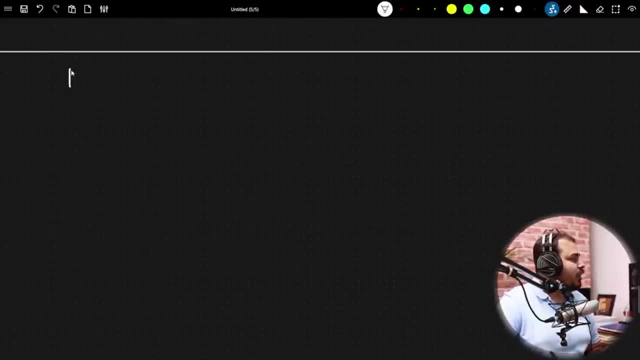 So what is the funda, or what is the technique to understand which activation function we should use, Technique, which activation function we should use. Which activation function we should use. okay, Which activation function we should use? Now, the technique should be very simple, okay. 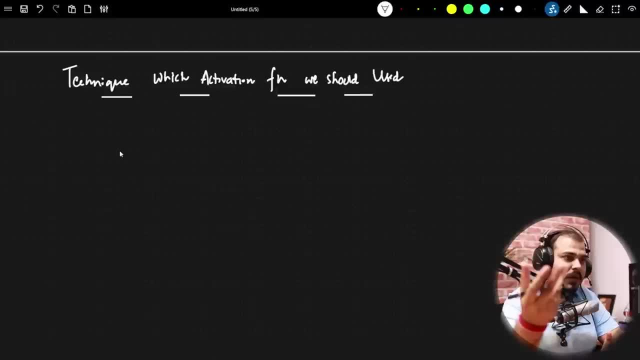 You know that you cannot use sigmoid activation function. okay, If you use sigmoid activation function, what will happen? Vanishing gradient problem will happen. right, It is very much clear. Vanishing gradient problem will be there. You cannot use tanh. 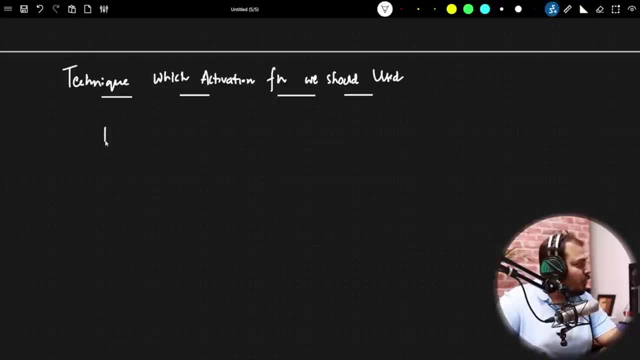 There is also vanishing gradient. So suppose you have binary classification. Suppose you have binary classification. Now, in binary classification the funda will be that suppose this is your neural network. okay, Let's say this is your neural network and this is your output. 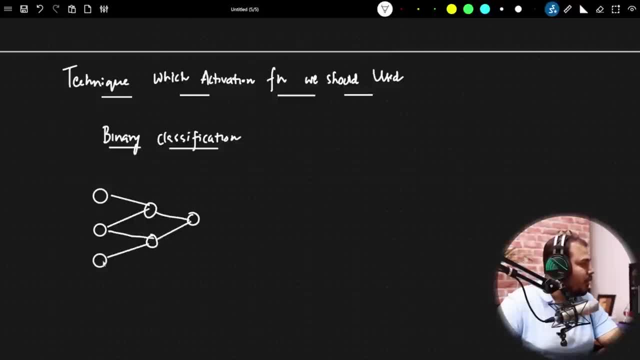 Let's say this is your entire neural network. okay, Now, in this particular case, always remember, in the hidden layer, try to use ReLU activation function. In the hidden layer, always use ReLU activation function. It is the most efficient activation function, okay. 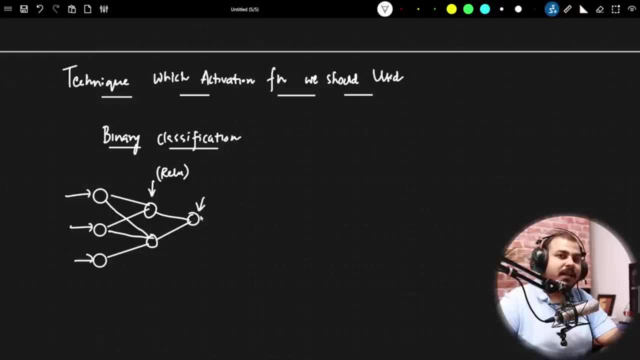 ReLU activation function In the output layer. if this is a binary classification problem, use sigmoid activation function. Sigmoid activation function. okay, This should be the funda. Let's say, with the help of ReLU, okay, With the help of ReLU. the convergence is not happening. 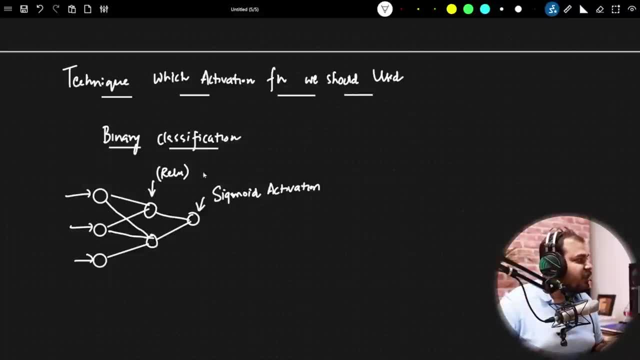 That activation function, the convergence is not happening. Then what will happen? You can change this ReLU. You can change this ReLU to something called as pre-ReLU or eLU, right, You can change this, But always remember, whenever you are doing a binary classification problem, your output. 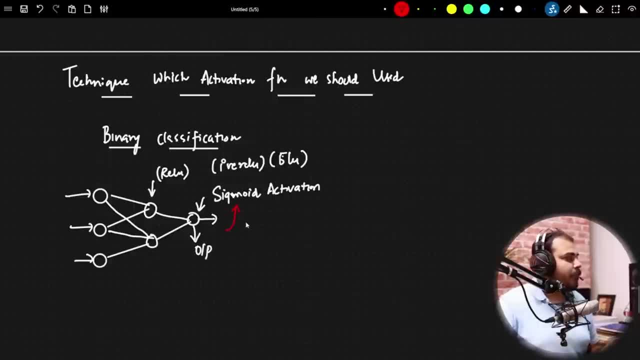 should have the sigmoid activation function only. okay, Sigmoid activation function. Now let's talk about multiclass classification problem. In multiclass classification problem, suppose this is my neurons and this is my hidden layer And this is my, let's say, two output are there? 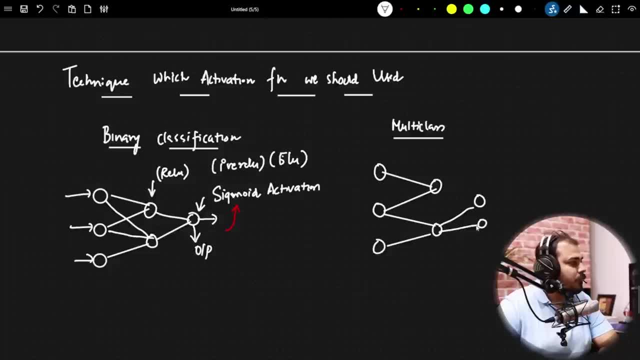 Now, in the case of multiclass classification problem. okay, In the case of multiclass classification problem, use another activation function which is called as softmax. I will discuss about softmax just in a while, when we are discussing about loss function. So softmax activation function can be used over here in the output layer. 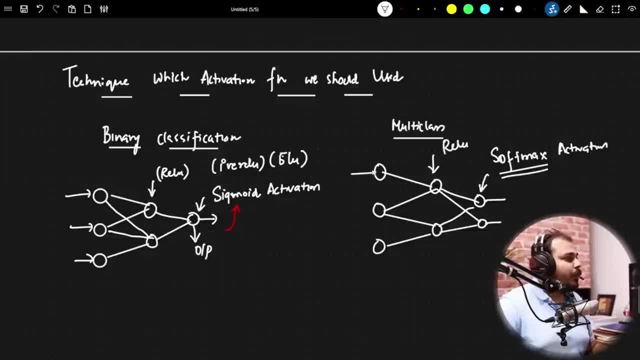 Over here again. you can use the combination of ReLU- Okay, ReLU or pre-ReLU or other kind of ReLU if the convergence is not happening. But by default always make sure that go with ReLU- okay, ReLU solves most of the problem, right. 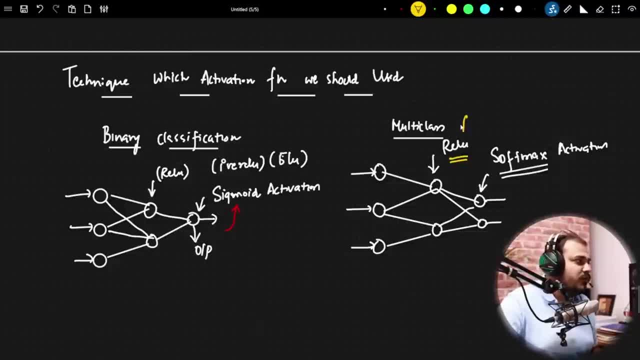 So that is the reason: in each and every hidden layer, in each and every neuron, use ReLU activation function. in hidden layers, In output layer for multiclass, use softmax activation function or sigmoid activation function. Now, in the case of regression, problem statement. 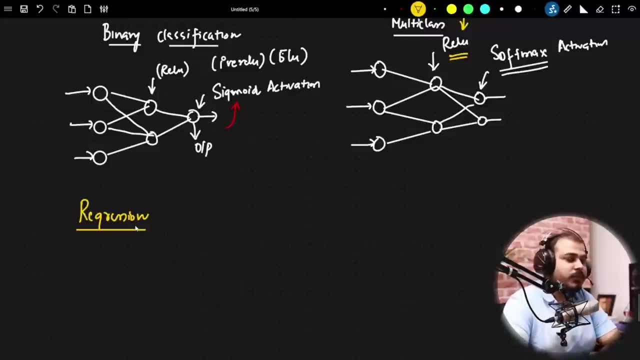 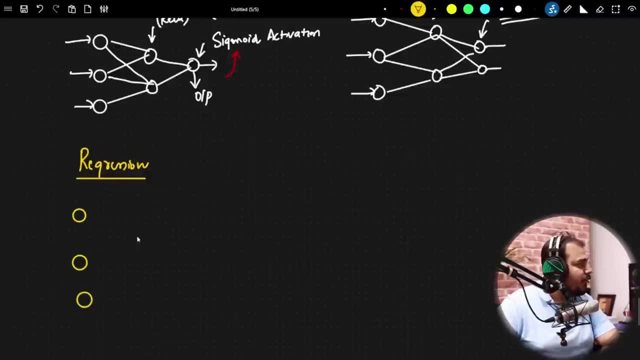 In the case of regression problem statement. what can you use in the case of regression problem statement? In regression problem statement again, the funda will be same. okay, Suppose this is the hidden layer and this is the output layer. Regression basically means you will be having a continuous value. 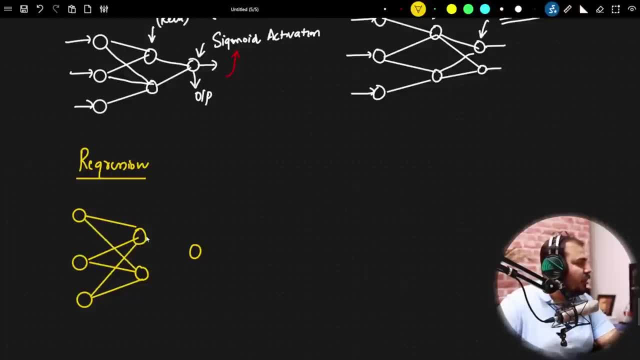 I hope everybody knows machine learning right, A basic of machine learning. Now, in regression case, always remember here in the hidden layer use ReLU or any variation of ReLU, But in the output layer use an activation function which is called as linear activation. 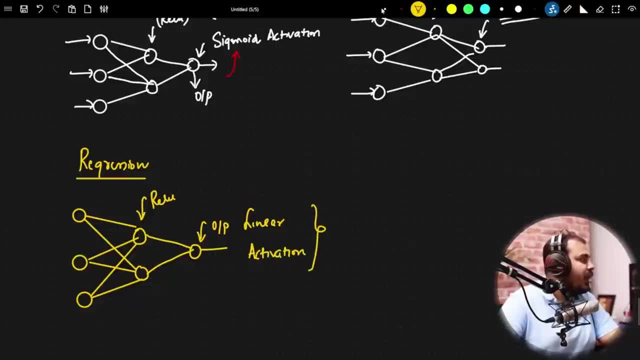 function, Okay, Linear activation function. So there is another kind of activation function which is called as linear activation function, And over here there will be also a separate loss function which I will be discussing about in just after we complete this activation function. 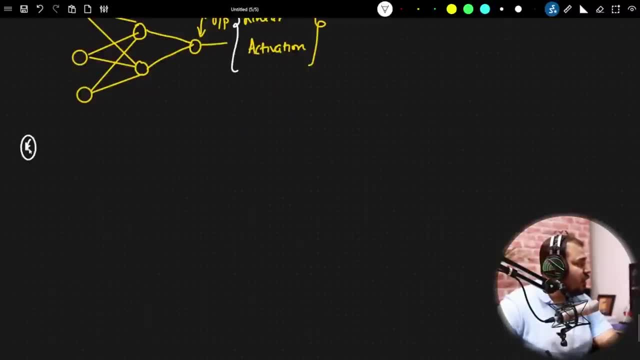 Okay, Now the next topic that I am actually going to discuss about is something called as activation, Activation function. So not sorry, not activation function, it is basically loss function. Now we are going to deep dive into loss functions, okay, So everybody is able to understand. see, I am not seeing anywhere. everything is in my 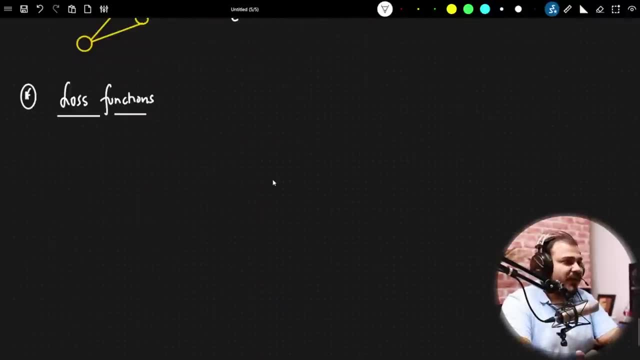 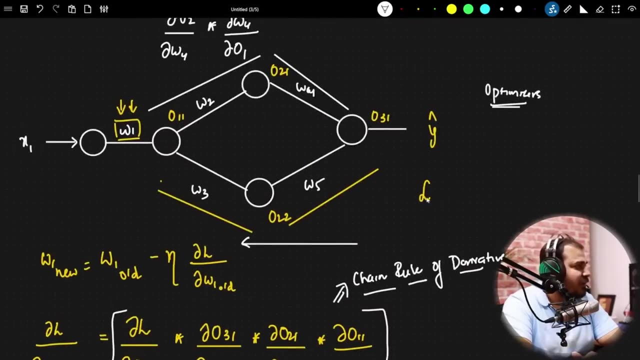 mind. I am able to teach you directly by writing things. Till now, we have seen neural networks like: where did loss actually come in this stage? right, I told you that we should always try to reduce this loss. right, Loss came over here everything. 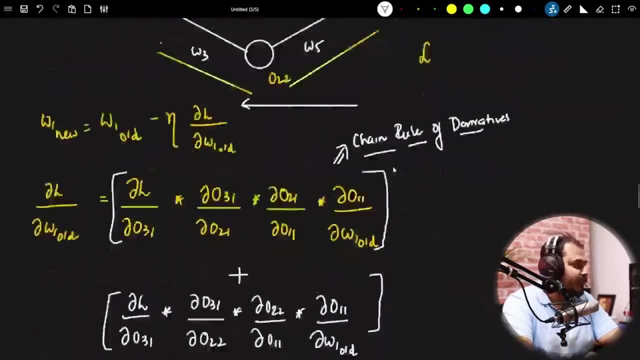 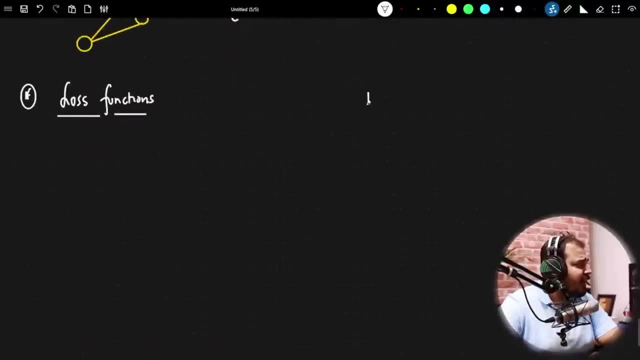 After the forward propagation, loss will be coming and we need to reduce the loss. But there are different types of loss function also that we really need to discuss. Okay, Let's say I have a data set. or let's talk about this: deep learning and deep learning. 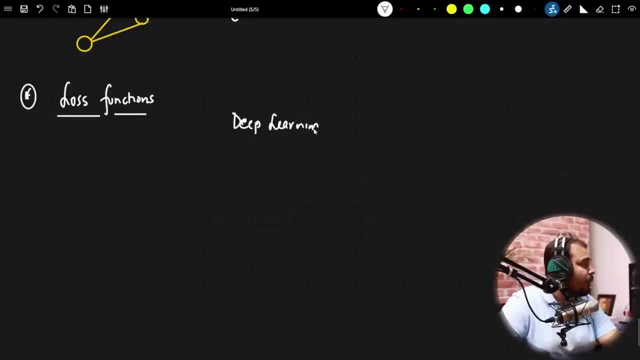 specifically with respect to artificial neural network, If I probably say A and N, right, We solve two different kind of problems. The first problem is something called as regression and the second problem that we basically solve is something called as classification. okay, Now, whenever we are trying to solve these two, basically regression or classification- 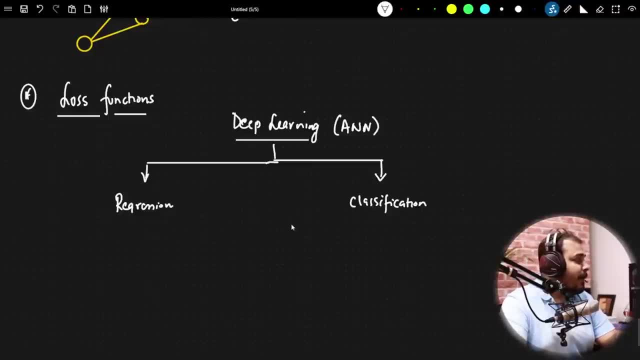 we basically learn these all things over here. okay, Now in regression, always understand the data set how it look like. let's say, I have a data set over here. Okay, It has values like years of experience. okay, degree, okay. 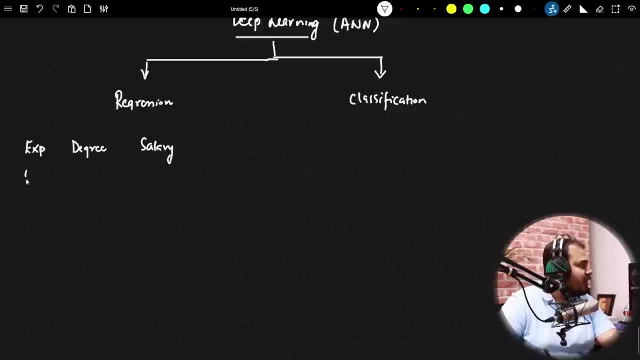 And the output feature is salary. Now, here, if I say the person is 10 years experience and he is having PhD, the salary will be quite high, right? So here you will be having a continuous value, right? So this continuous value is basically my output feature and this is basically a kind of regression. 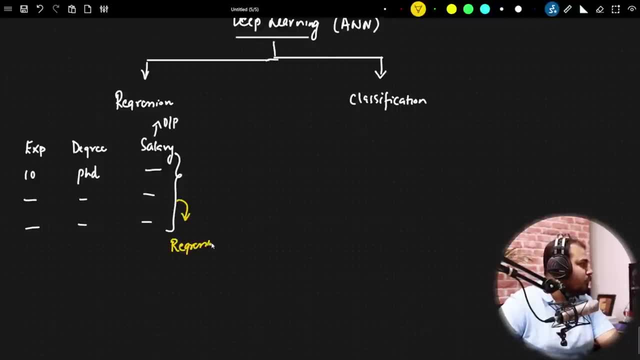 problem. This is basically a kind of regression problem. Okay, Very, very simple, Very, very clear. Okay, In the case of classification, how my data set will look like. If I probably see an example with respect to data set, let's say it will be like playing. 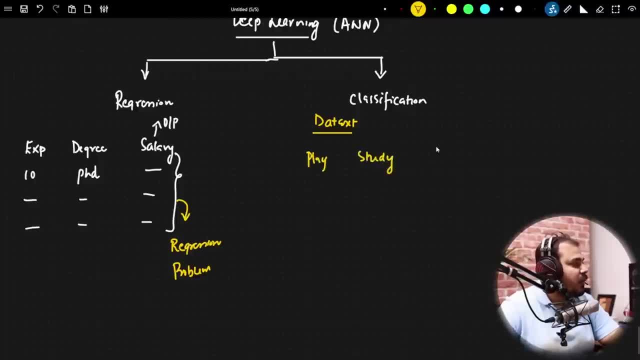 hours, study hours, and whether the person is able to pass or fail. Okay, Now this becomes a classification problem. It can be a binary classification. Okay, Let's say, if it is a multi classification, Suppose the person plays for 10 hours. 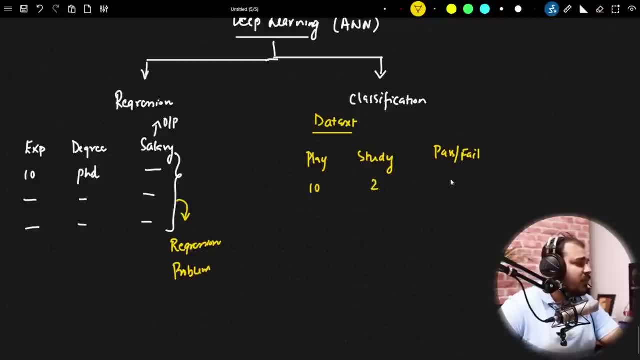 the person plays for 10 hours, he studies for two hours, then obviously the chance is that the person may fail right. if the person studies for plays for four hours and he studies for three hours, then also i think the person may fail right. let's say, the person is studying playing for five hours. 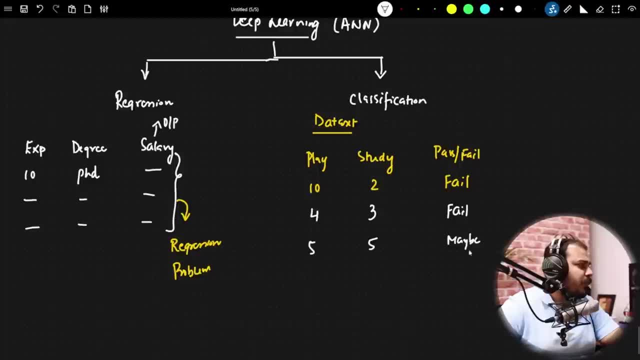 and he's studying for five hours, then maybe, maybe he may pass. and i may have another data set, like if the person is playing for two hours and if he's studying for seven hours, he may pass. so here, what is happening? here you have a multi-class classification problem. 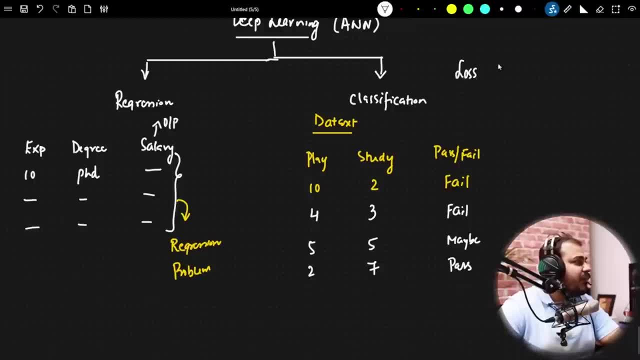 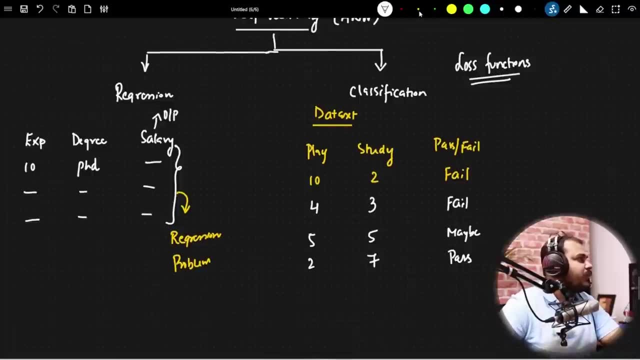 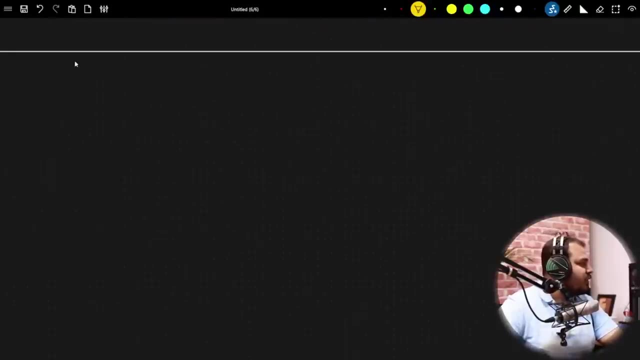 now, with respect to this kind of problems, you will have different, different loss function. okay, loss function. so the first loss function that i am going to discuss about is with respect to regression, and the second i will go ahead with discussing classification now. in regression, we discuss basically three different types. 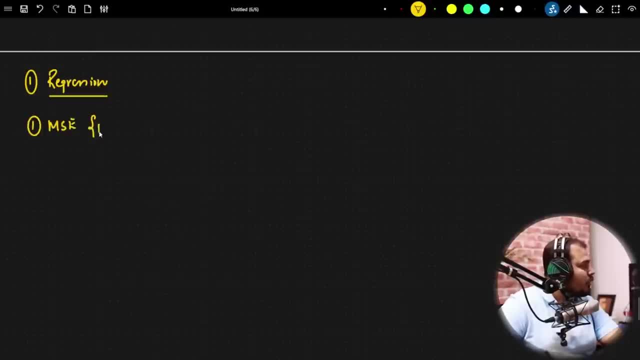 one is: mean squared error. i'm going to write it down: mean squared error, and this all will work for a continuous output feature, okay. second is: mean absolute error. mean absolute error. okay, mean absolute error. the third one that we are basically going to discuss about is something: 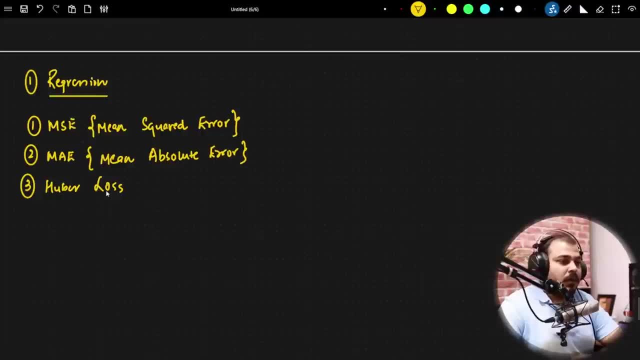 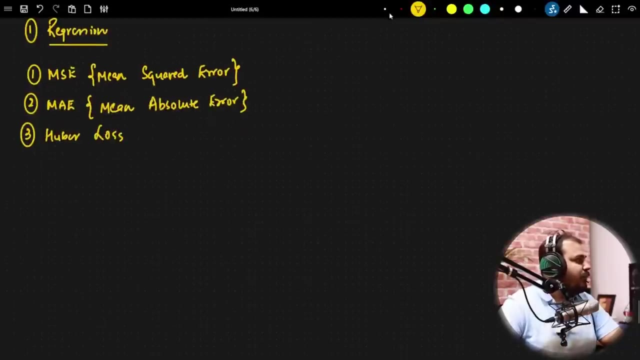 called as huber loss. okay, huber loss. so we are going to basically discuss this three main: first for regression, and then we will continue for classification. so let's go ahead and let's try to understand what exactly is mean squared error, and before that, i want to discuss about two different things. 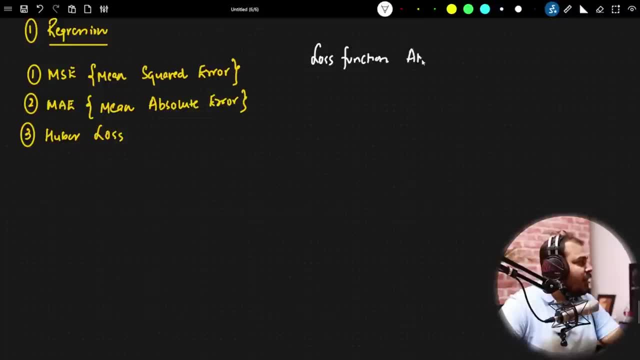 one is loss function and cost function. now i'm introducing a new term which is called as cost function. okay, let's say, guys, this is my input, right? i'm going to say that this is my input, right, this is my hidden layer and this is my output now, usually in forward propagation, let's say in my 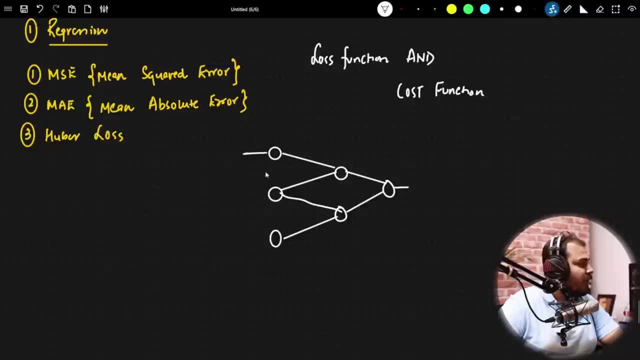 data set i have 100 records. let's say, in my data set i have 100 records. okay, in my data set i have 100 records, 100 records right now, during the forward propagation. what happens during the forward propagation? what happens? i pass one record, i calculate the y hat and then i pass the y hat and 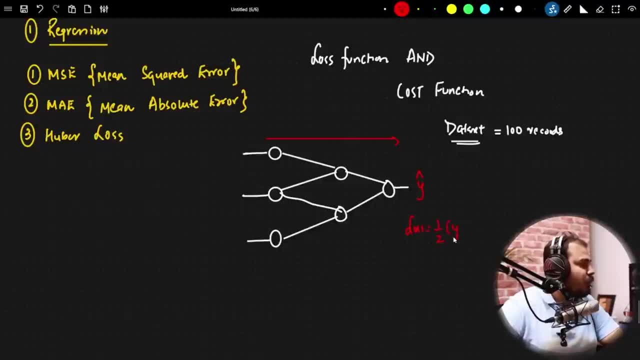 then i calculate the loss and the formula is very simple: y minus y hat whole square. okay, and then i basically do the backward propagation. this happens usually for every record. we are calculating the loss. but this is not an efficient scenario. suppose, if i have 100 records i can set up a. 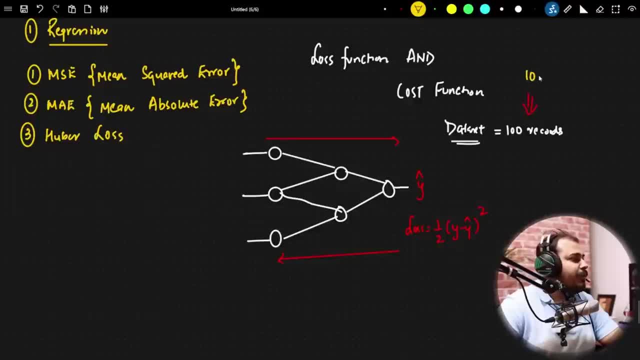 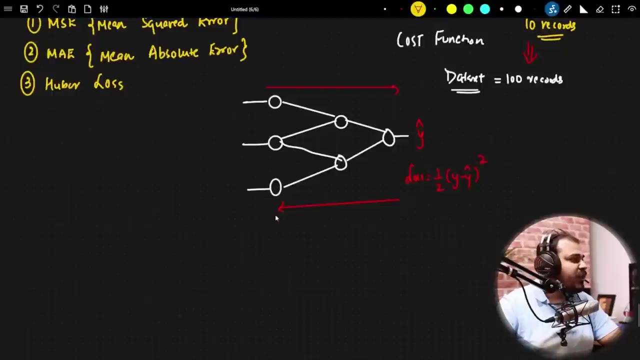 path size. i can basically say: at every forward propagation past 10 records and when you are passing the 10 records, then you calculate the loss for the 10 records. okay, whenever i pass catch at once, then the formula will be changing instead of loss i will. 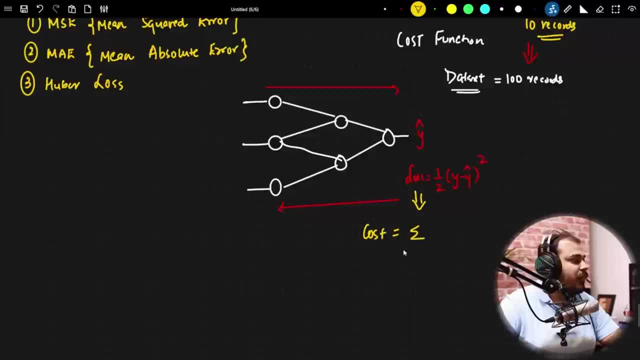 try to write this as cost function and this cost function will be: i is equal to 1 to n, which is my back size, and this formula will be: y minus y hat whole square and here i will be having 1 by 2, okay, so i hope everybody is able to understand what is the difference between loss and cost function. 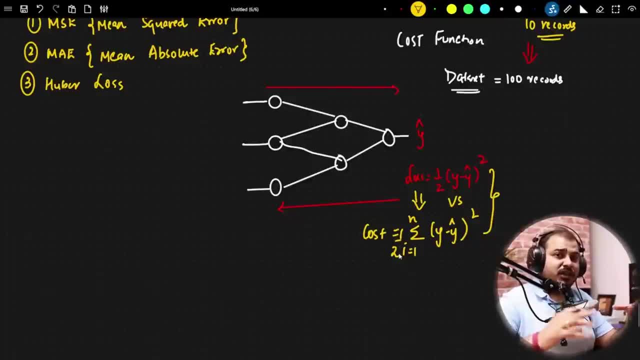 in loss function, i specifically provide one data point. in cost function, i specifically provide batch of data points. okay, so this is the basic difference. okay, in the forward and the backward propagation, in every propagation, in every epochs- we also say it as epochs- we pass a batch of records, not just a single record. okay, so till here, i hope everybody's. 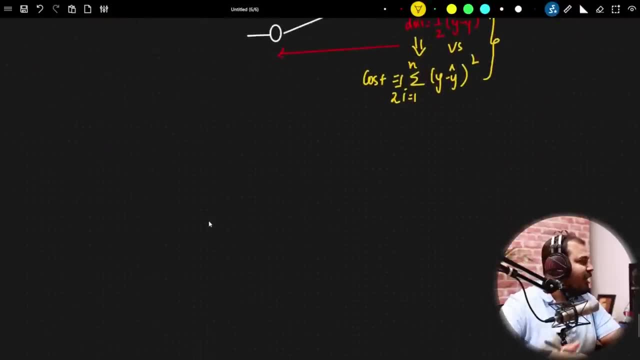 clear. now let's go ahead and like, let's try to understand. what is this mean squared error? so first one that we are going to understand is something called a mean squared error, and this is for regression. okay, we basically also write it as msc: now, mean squared error. 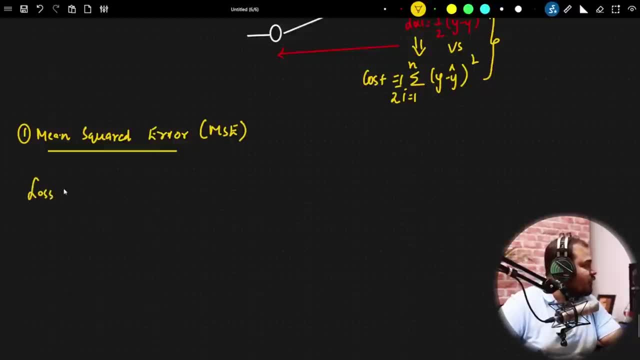 already. i have written the formula. if you go ahead with loss function, the formula is nothing but 1 by 2. y minus y hat whole square. if i probably go with respect to cost function, the formula is: summation of i is equal to 1 to n, 1 by 2. 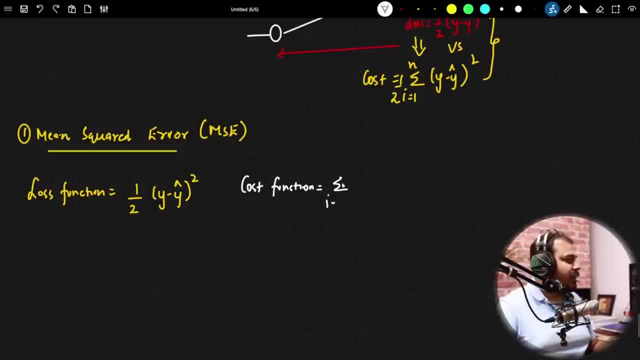 y minus, or let me write it like this little bit, like this, so it will be easy, it will be: 1 by 2. summation of i is equal to 1 to n. y minus y hat whole square. okay, so this, this i hope everybody is able to uh understand over here. okay, very easily, you are able to understand the loss function will. 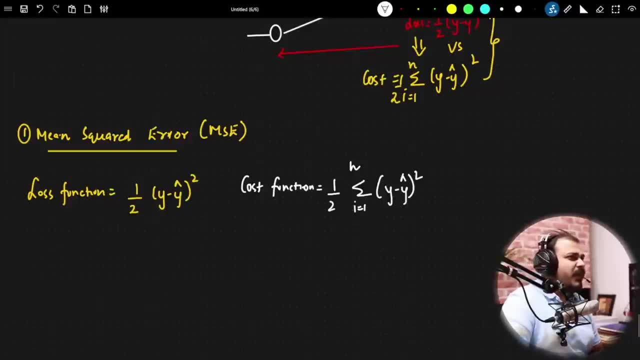 be written like this. the cost function will be written like this: okay, but we need to understand what exactly is this mean squared error, this formula that you are able to see. okay, this formula is basically called as quadratic equation- quadratic equation. now, what is so special about this quadratic equation? okay, so i hope everybody knows this formula: a minus b, whole square, so you. 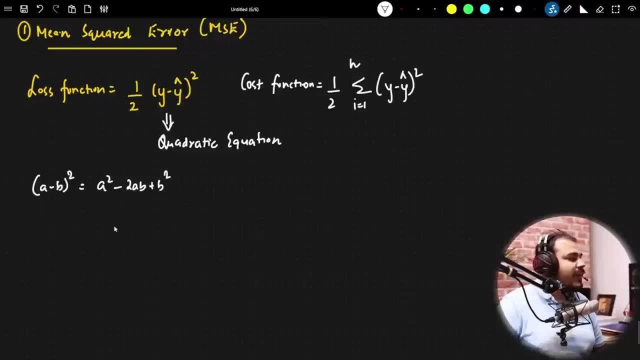 say a square minus 2, a b plus b square, this is also quadratic equation. if you probably want to see a generic definition of quadratic equation, it is nothing but a x squared plus b, x plus c. okay, and whenever you construct this quadratic equation, whenever you construct this quadratic equation, you will be able to see that we get a kind of curve. 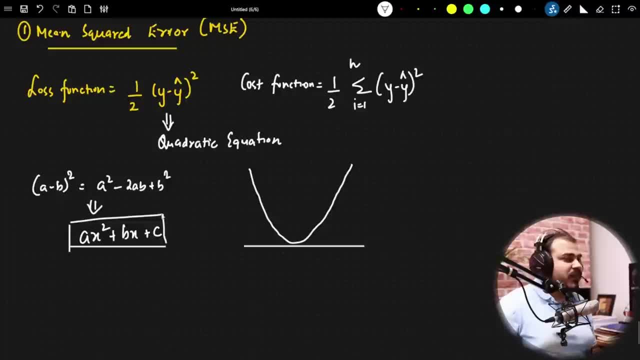 this kind of curve. okay, because this is the loss function and if you remember, this quadratic equation gives us something like this kind of gradient descent. okay, if you probably go and write plotting a quadratic equation- okay, quadratic equation, equation- at that point of time you will be getting this kind of curve. okay. now, what is this curve? 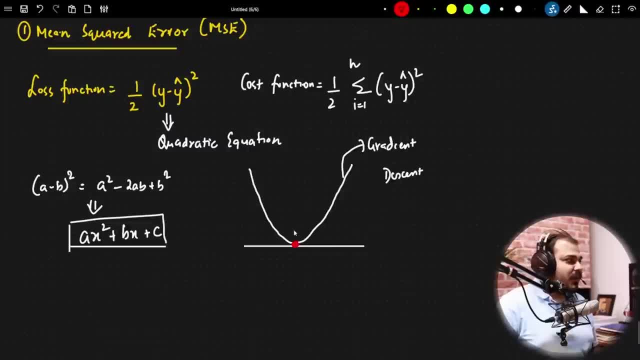 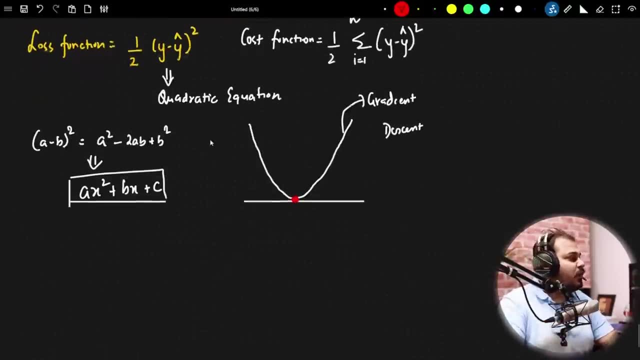 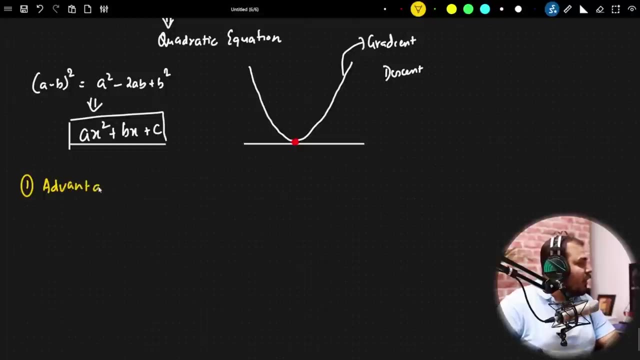 here you will be able to see. this is my one single point. okay, this curve, this quadratic equation, has lot of disadvantages, lot of advantages. okay, so let me note down some of the advantages. so first i will go ahead and note down the advantages of this quadratic equation or this curve. okay, 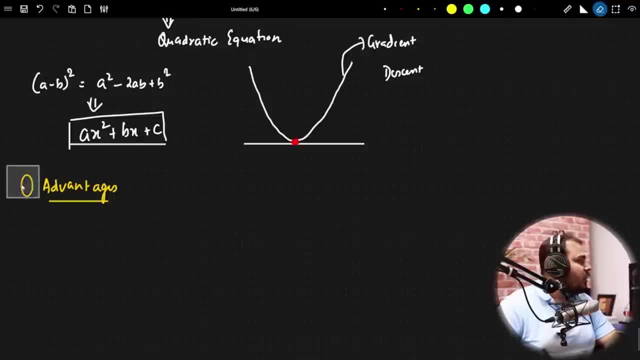 so i will just go and note down all the advantages. the first advantage, let's discuss about it. the first advantage, okay, the first advantage over here. whenever we have this kind of curve, that basically means it can be differentiable. so it is definitely differentiable that we have. 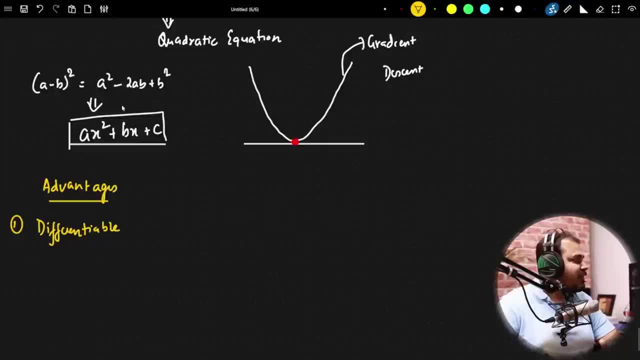 already seen, right? that is how weight updation formula basically happens. this curve is basically getting created by this quadratic equation only, right? so it is obviously differentiable. the second advantage is that it can be differentiated by this quadratic equation. the second thing that you can basically write: it has only one global or local minima. it has only 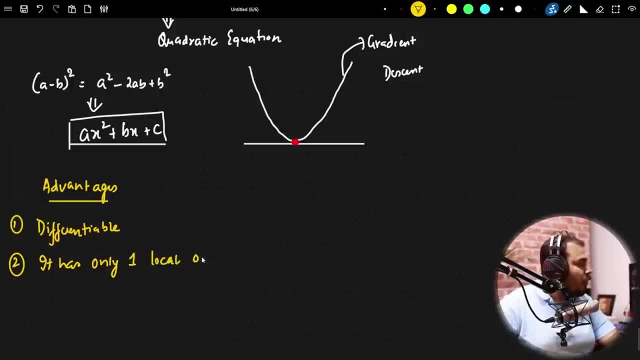 one local or global minima. it has only one, not more than one. okay, it has obviously just one local or global minima. the third point: you can basically write: it converges faster, it converges faster. so these are some of the advantages of this quadratic equation. 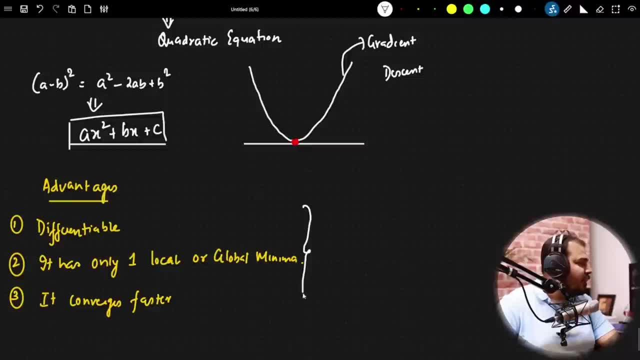 of the amazing advantages of using this. but, as we say, everything that comes up, it has pros, it has cons. so let's talk about the disadvantages. disadvantages, the first disadvantage that is there, and only disadvantage: it is not robust to outliers. big issue, big, big, big issue, and just 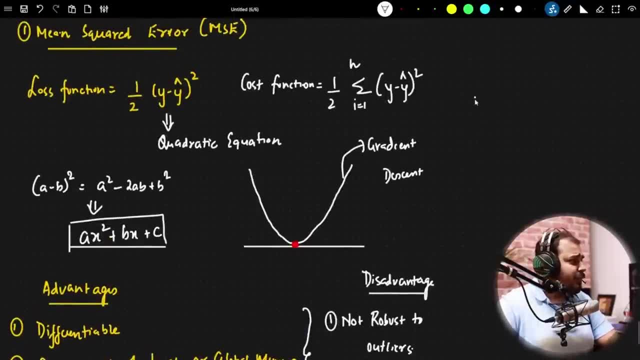 by seeing the formula you can actually understand. let's say i'm solving a linear regression problem. let's say i have a data points which looks like this: okay, let's say i have an outliers. let's say i have this outliers. if i remove this outliers, obviously you know that my linear regression line that will be getting created. it will get created. 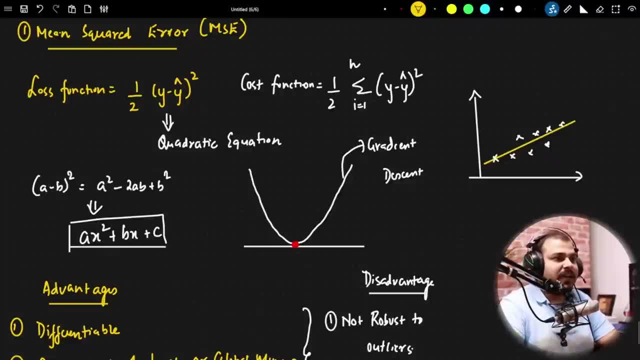 like this: okay, it will definitely get created like this, right, it will definitely get created like this over here. but now, if i have some outliers, what will happen? just see this. i'll remove this line. i'll remove this line. let's say, i'm having some outliers over. 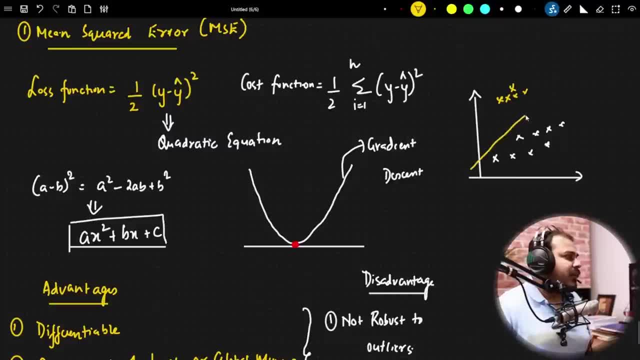 here, then my line, that new line that will get created, it will look like this now why this line changing is happening so much, why this line changes so much, the reason it changes so much: it is because i am penalizing the error. this is my error, right, and that error i'm squaring it. 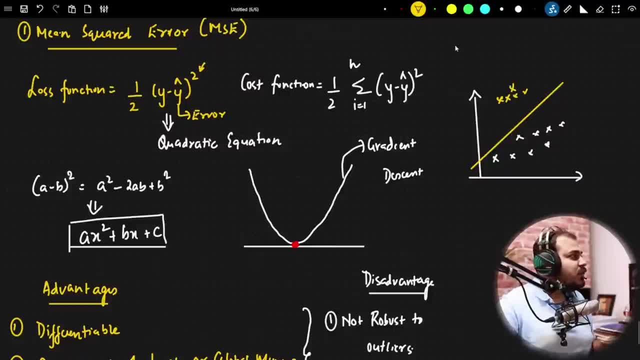 the reason it shifts so much? because we are penalizing the error. okay, we are penalizing the error if there are no outliers, that is fine, but if our errors are too much, then we are penalizing them, since we are squaring the error over here, and because of that, 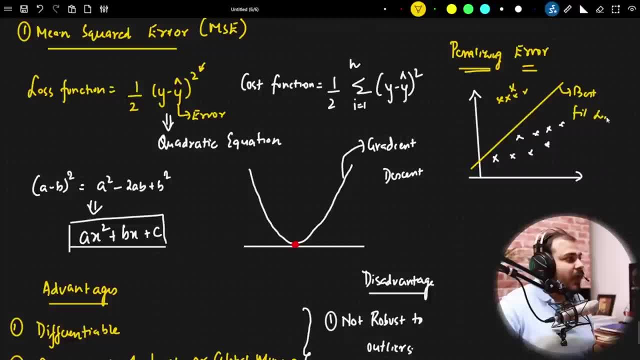 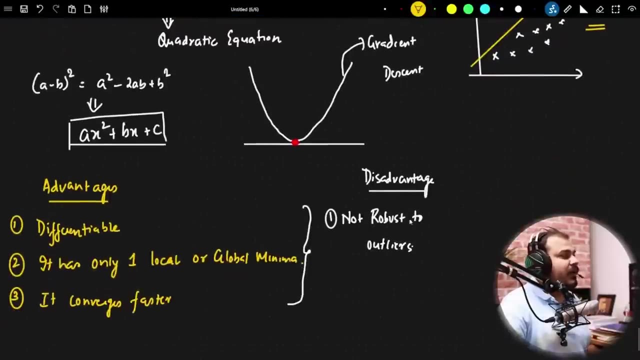 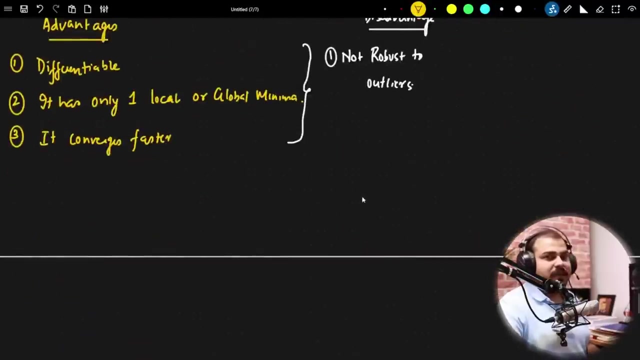 the best fit line which you basically have, will have a major, major shift. okay, we'll have a major shift. in short, right. so this is the only disadvantage with respect to the mean squared error: that it is not robust to outliers. okay, now, coming to the second one. obviously, if it is not, 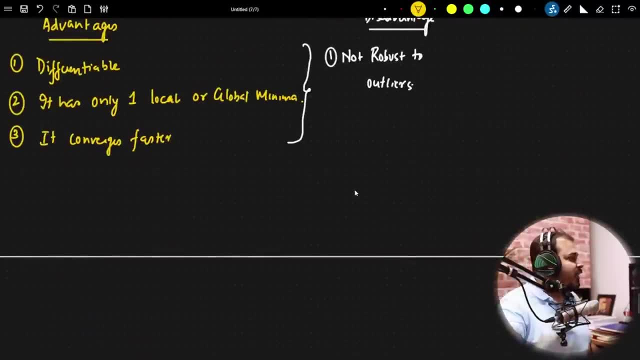 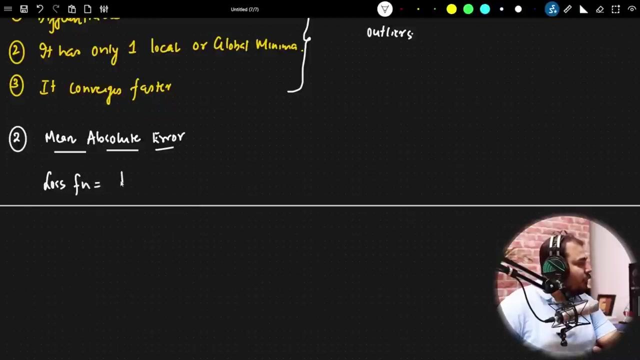 robust to outliers. again, researcher will not keep quiet, they'll come up with something. so, coming to the second one, which is called as mean absolute error: mean absolute error. now, what exactly is mean absolute error? i'll just write it down as formula. okay, so over here, my loss function formula will be 1 by 2: absolute of y minus y hat. our cost function will basically: 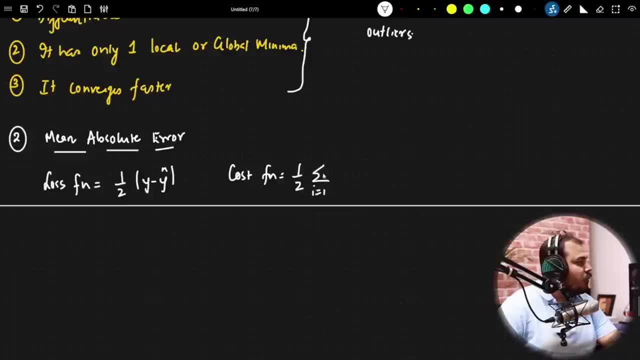 be 1 by 2, summation of i is equal to 1 to n, y minus y. hat right, this is how it will be now. we are not squaring it so definitely. the major advantage will be that it is it is. what is the major advantage? it is robust to outliers. 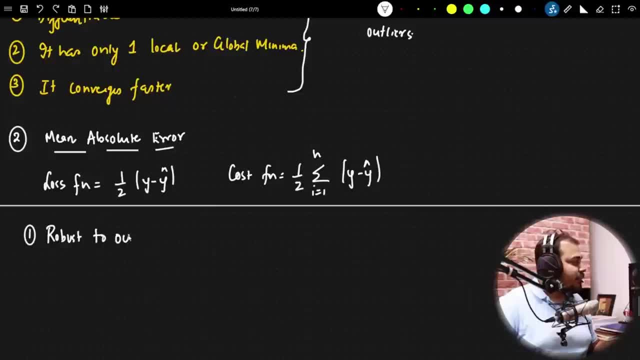 because now we are not penalizing, we are squaring it. sorry, we are not squaring it, so we are not penalizing for that specific error. we are taking the absolute value right. so this is the major advantage with respect to the mean absolute error. so that basically means, even though i have a kind 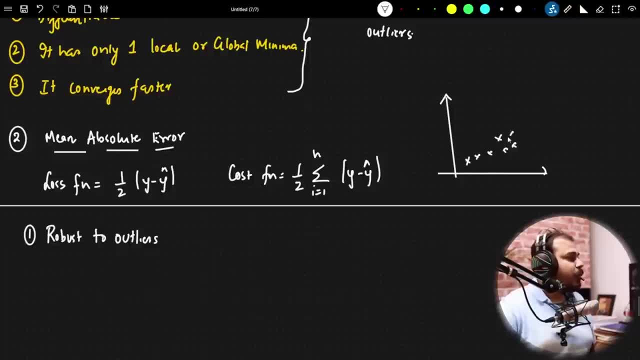 of outlier. let's say like this: suppose these are my points and suppose i want to have a cost function if i have some outliers, there will be a shift, but not a major shift. the shift may be this much initially. the line may be simple. then what you'll be? there'll be a, there'll be a minor shift, okay. 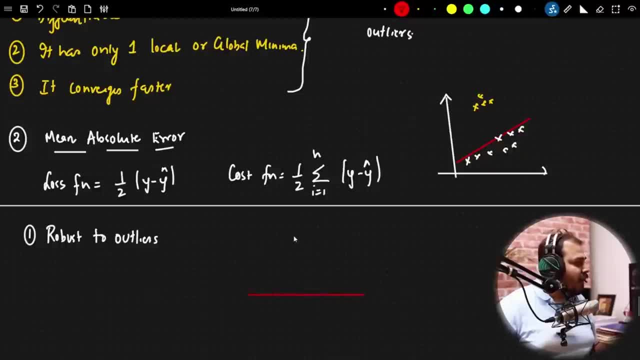 and how does this mean? absolute error curve. look like this curve will be looking something like this, like how we had for quadratic equation. the curve for mean absolute error will be like this and for this the derivative will not be simple. we have to basically take sub gradient, sub gradient. 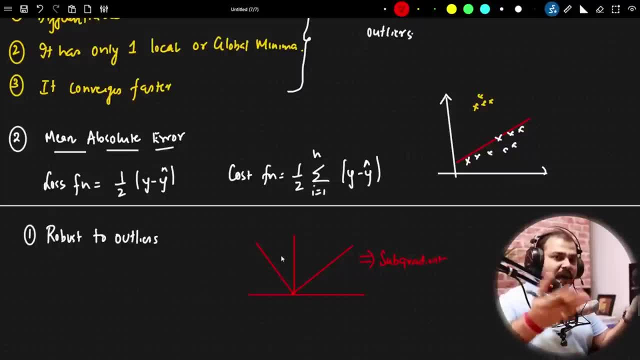 basically means we need to divide this line, separate, part by part, and basically calculate the slope. that is what it is, you know, because here we don't have any kind of curve, we have to take part by part, because this keeps on changing it. it can change from one part to the other part. 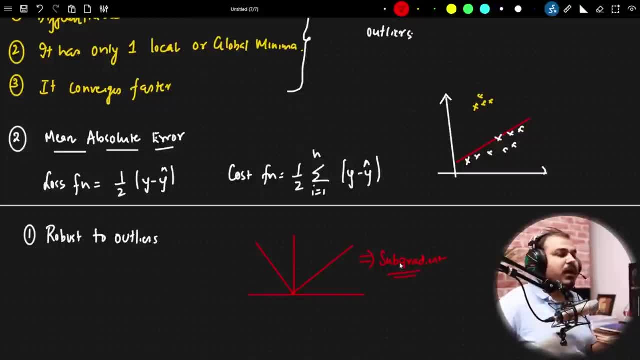 right. so here we have to basically take the sub gradient, to basically calculate or update the weights. not a major task, but it does take little bit time. it is time consuming, time constraint, is there? so timing, timing wise, obviously it is more than the previous one, that is mean squared error. okay, now coming to the third one. the third. 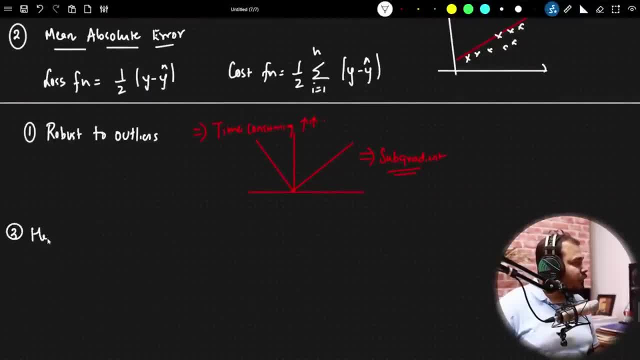 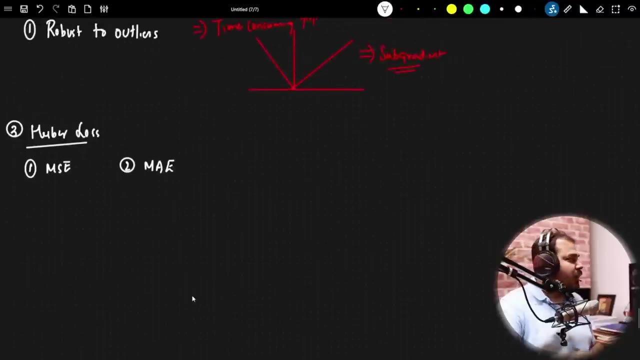 one for the linear regression is something called as huber loss. huber loss, in short, is the combination mean squared error, and it is the combination of mean absolute error. okay, Yes, Yes, No, No. mean squared error means absolute error. now, here the loss will look something like this: 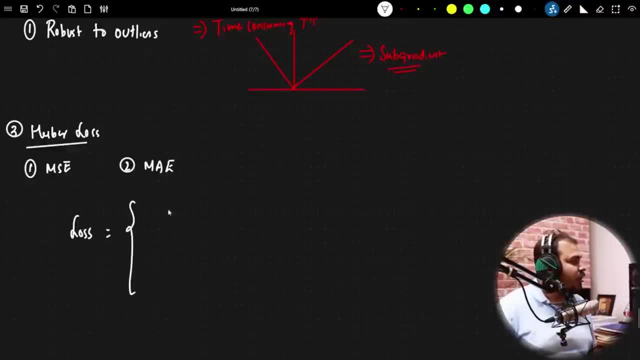 the loss or the cost function will look something like this: so here you can write 1 by 2, y minus y, hat whole square. and this is specifically this will be specifically when it will be used when the outliers are not there, right? so if i write a condition, if y minus. 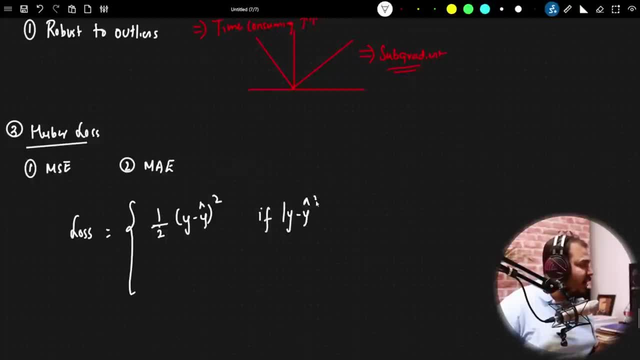 if y minus y hat is less than or equal to some hyper parameter which is basically given by this delta sign, so this will be some hyper parameter. okay, so i will basically write this as a hyper parameter if the difference is less than this value, if the error difference is less than this: 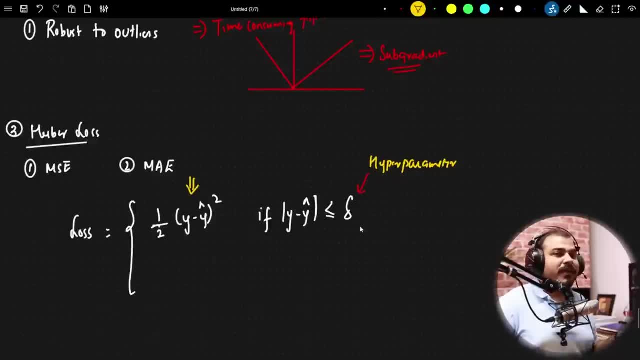 value, then probably i will go with this, because this will denote whether there is an outlier or not present in this. and if in the second case it will be something like y minus y hat whole square and this delta sign will be some hyper parameter. okay, so if i write, 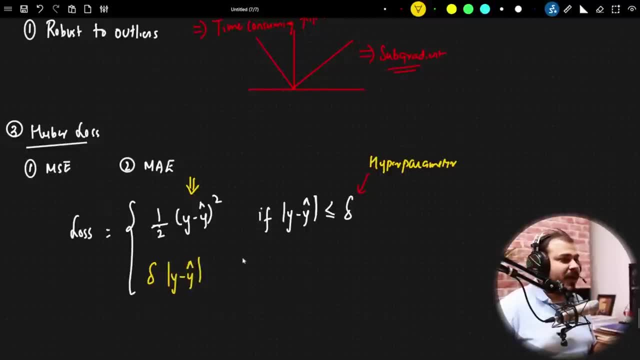 we will be taking care of y minus y, hat minus half by delta square, otherwise. so if there are outliers, we will specifically use this same hyper parameter and we'll use this equation to solve that. so two condition: one is basically when the when the outliers are not present, when the outliers 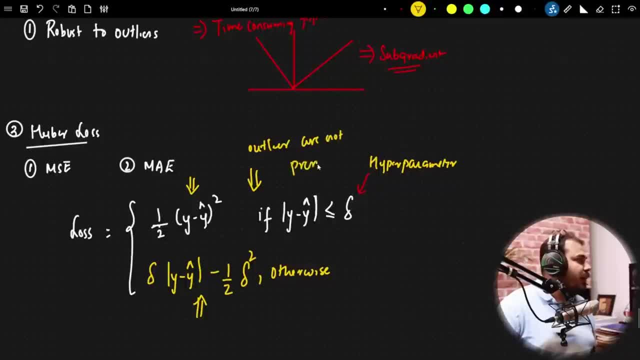 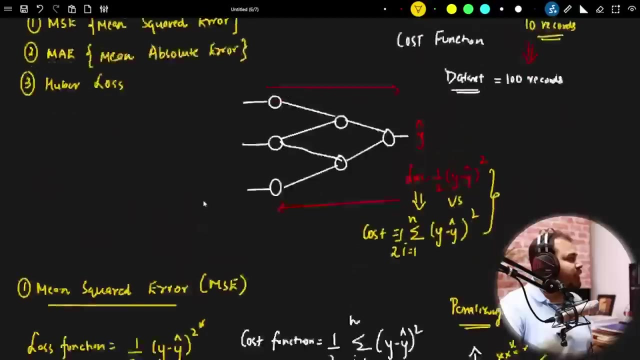 are not present are not present, and if the outliers are present, we can definitely use this one. and this is specifically a hyper parameter which can be found out when we are doing the coding. okay, so this is specifically to huber loss. so, till here, everybody is clear, because we have 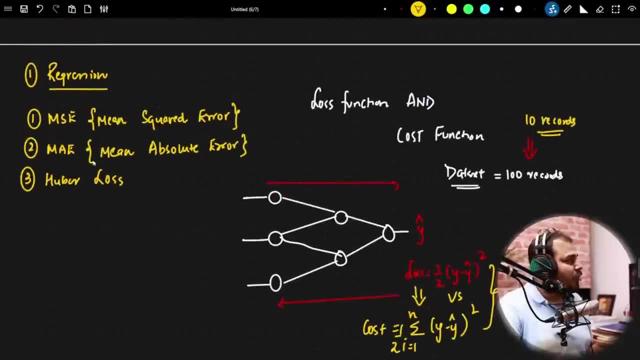 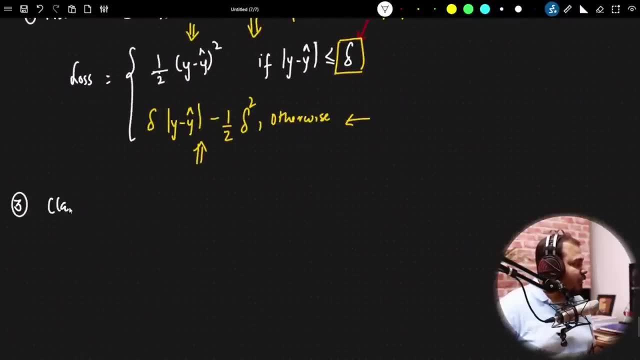 discussed, mean squared error, mean absolute error and huber loss for the regression. now we will go ahead and discuss about the classification one. so the next topic is: with respect to classification loss function, what are the different different classification loss function we will try to discuss now. in classification we specify the classification loss function and we will discuss. 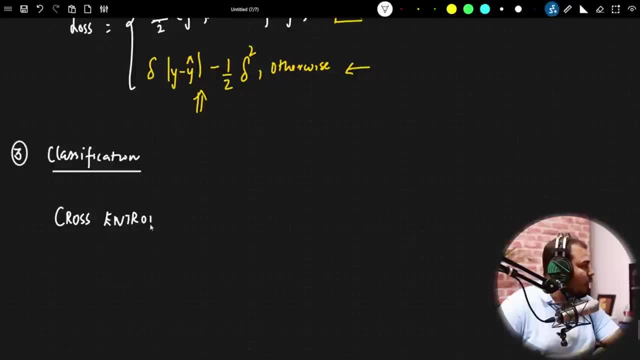 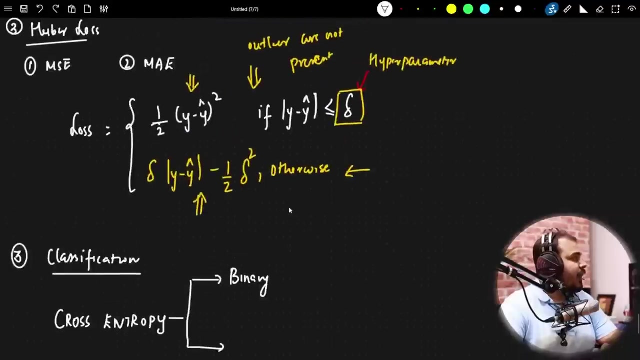 specifically use something called as cross entropy, cross entropy. this cross entropy- usually loss function, is for two types. one is for binary classification and the second one is for i'll write like this: there are two types of this. okay, uh, okay, sorry. for cost function, you can basically write: summation of i is equal to 1 to n. 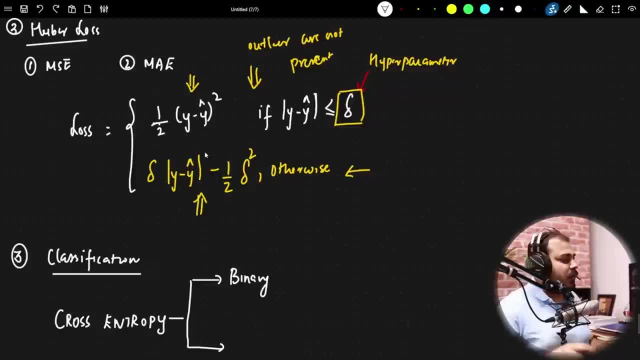 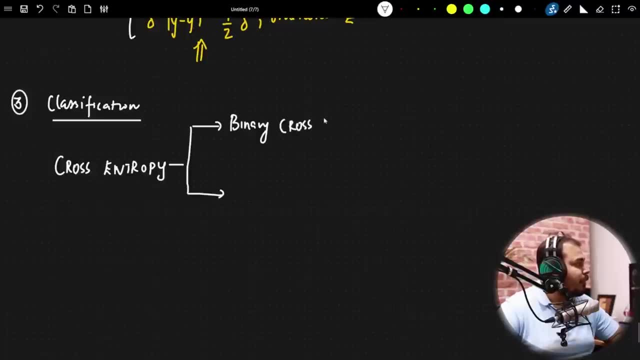 okay, i think that you can basically do. okay, it's. it's very simple. okay now, in classification: uh, i basically have a binary cross entropy and i have categorical cross entropy. okay, now, in binary entropy, we basically do it for binary classification. for the multi-class classification problem, we use categorical cross entropy. 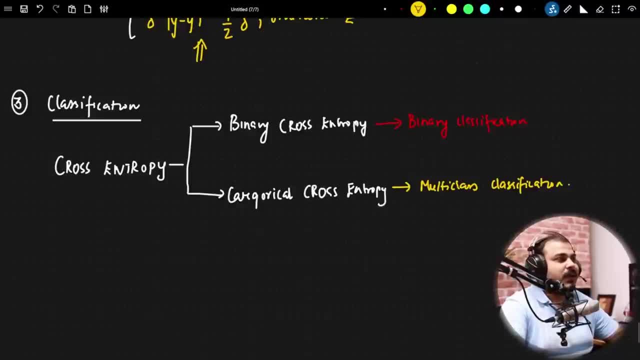 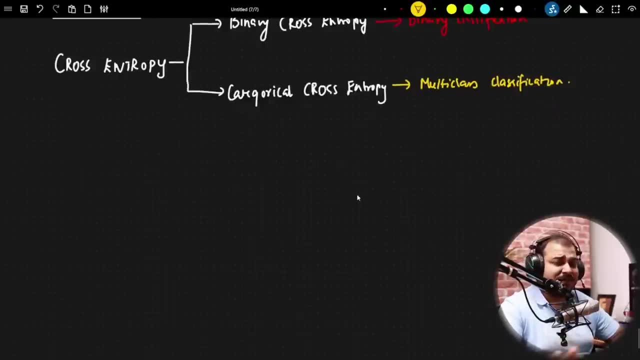 okay, so this is what we basically use for all these things and uh, uh, you know we will go ahead with the formula and i will try to see binary cross entropy. i hope everybody has learned that. learned about logistic regression. Just comment down whether you have learned. 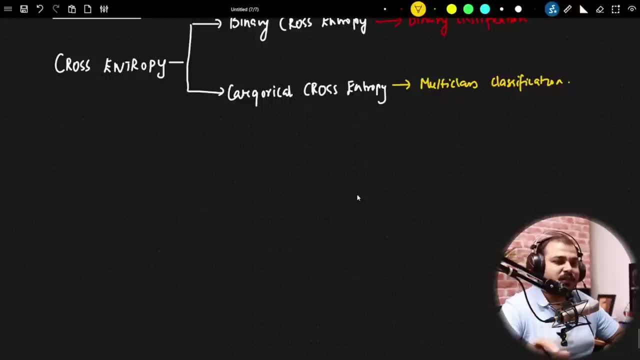 logistic regression or not, The logistic regression, whatever loss function is used, right, that log loss. Similarly, that is used for the binary cross entropy. So let me just write it down. So for first, binary cross entropy, okay, we actually use a loss function. 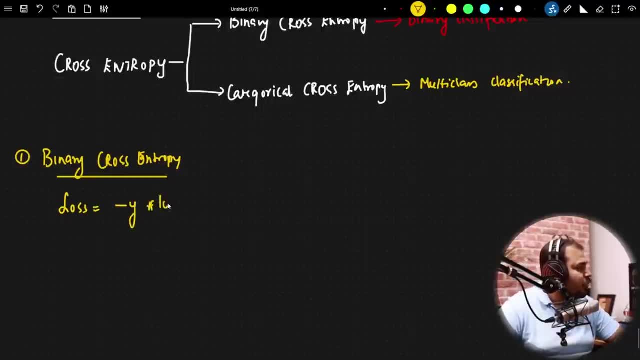 which will be a log loss function, which is given by minus y log of y hat minus one minus y multiplied by log of one minus y hat. Okay, This is the loss that is used in logistic regression also, Because logistic regression is a binary classification problem. 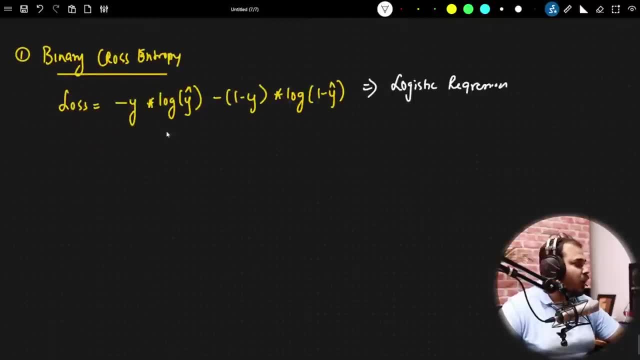 Okay, If I- and this is basically called as log loss, Okay, log loss. I can also write this in a different format. So my loss function. it will look something like this: now: Minus log one, minus y hat if y is equal to zero. 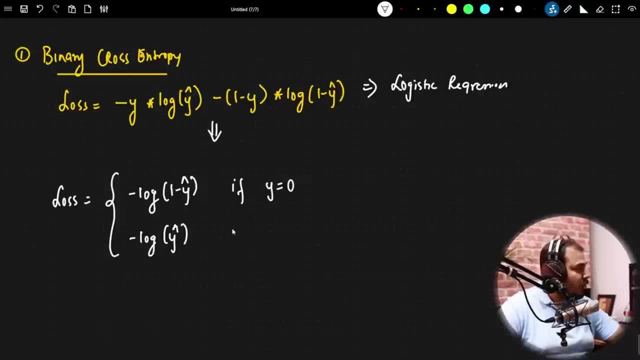 Minus log y hat. if y is equal to one, Okay, That basically means, whenever this y is zero, whenever this y is zero, right, whenever this y is zero, then what will happen? We, just, you can see, zero multiplied by this will be zero. 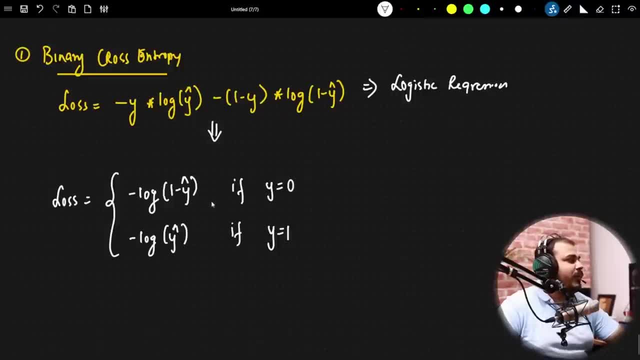 One minus zero is nothing. but so we have this minus log. one minus y hat. Okay, And then I have log of y hat. if y is equal to one, y is equal to one basically means this entire thing will become zero. So I'll be having minus log of y hat. 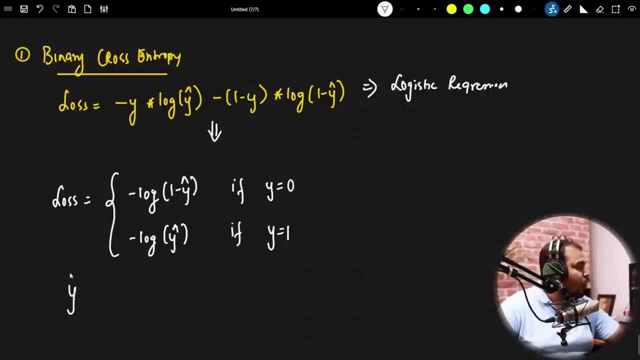 But the question arises- this is basically for the loss. How do we calculate y hat? The y hat calculation is very simple. right, We basically use the sigmoid activation function. Right Sigmoid activation function in the last layer. This is how we basically come up with y hat function. 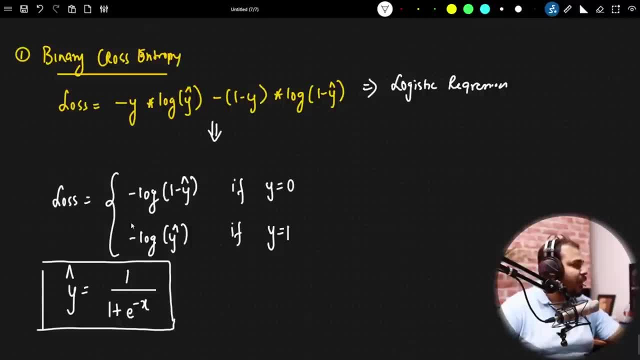 This is how we basically come up with y hat function, up with y hat for y, we definitely. then we apply this log loss on top of it and then we do the back propagation. everybody is clear with that. okay, and this is specifically for binary classification. 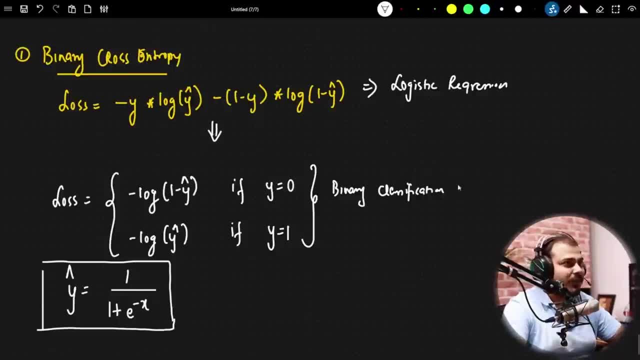 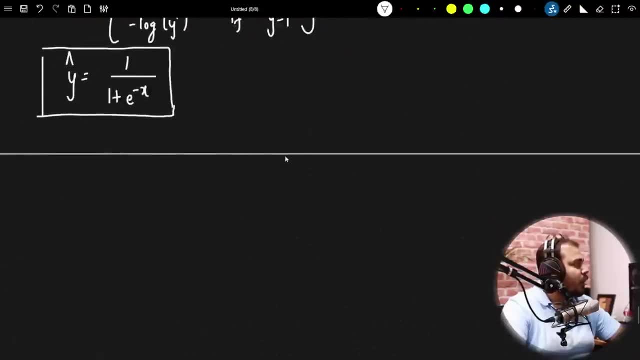 binary classification, and that is the power of binary cross entropy. okay, now the next thing that we are going to discuss about is coming to the next one. uh, let's discuss about this- categorical cross entropy. okay, so the second one is categorical cross entropy. a categorical cross entropy is nothing, but it is a multi-class classification problem. 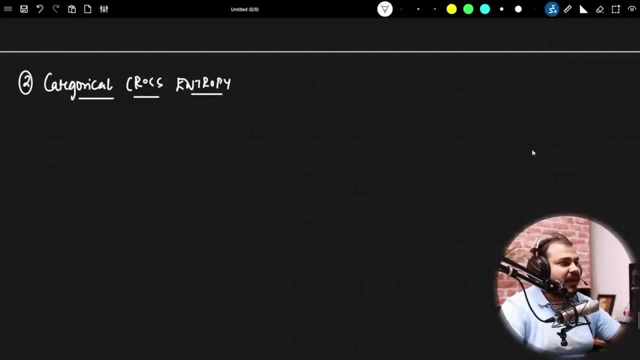 okay, multi-class classification problem. now, in the case of categorical cross entropy, what will happen? let's say i have some features, let's say i have a data set like f1, f2, f3 and i have output something. okay, let's say so, values: are there two, three, four, five, six, seven, eight, nine, ten, some value in the data set? and 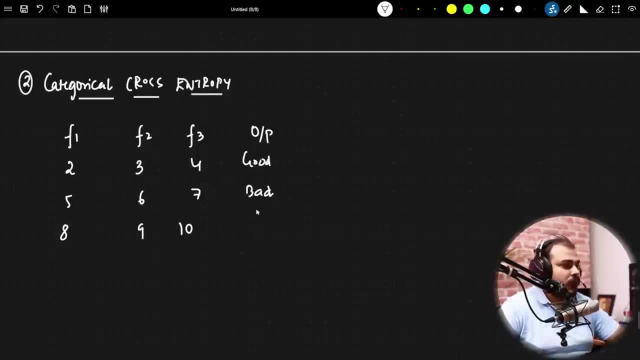 my output is good, bad, non neutral, let's say: okay, i have this specific output. now, the first thing in categorical cross entropy. what we do, whatever output- since this is a multi-class classification problem- right, multi-class classification problem- first of all, what we do is that we convert this into a one hot encoded format. one hot encoded format basically means what happens. 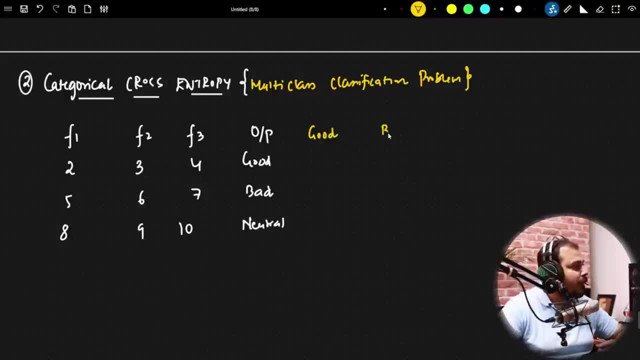 for this output. now i will be having columns like good, bad, neutral. this is the first step that we do. wherever the good value is, that becomes one and remaining all becomes zero. wherever bad is there, that will become one and remaining all will be zero. wherever neutral is. 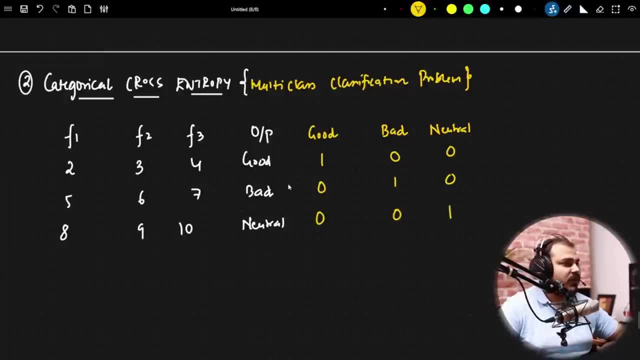 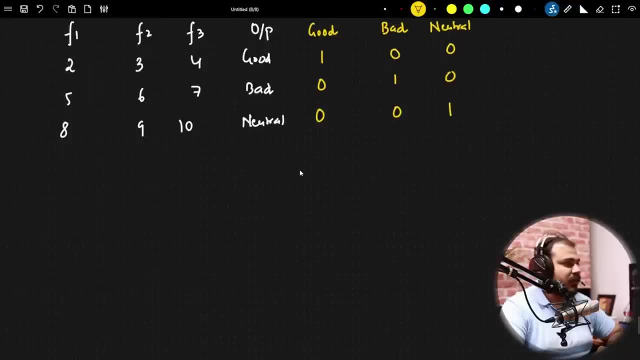 there, that will become one and remaining all will be zero. okay, so this is the first step. okay, and for what is the loss function? for categorical cross entropy, okay. for multi-class classification, we can write: loss is equal to x of i, comma y of i. okay, and here i'll make you understand the formula. 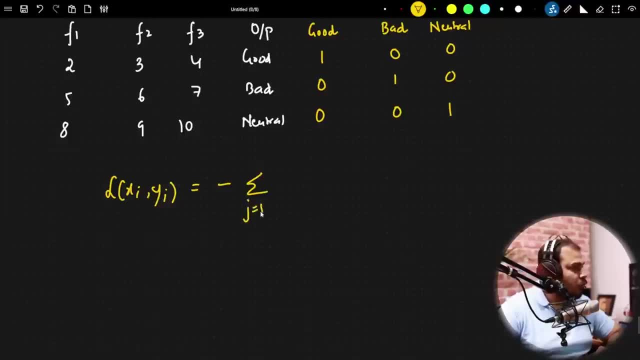 let me write down the formula: summation of j is equal to one to j is equal to one to c. c basically means number of categories. okay, y of i j multiplied by log to the base. e. y of i j hat. okay, and this is just the formula. okay for the loss function. now let me make you. 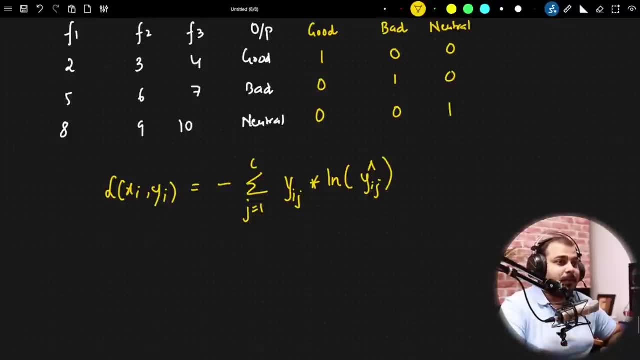 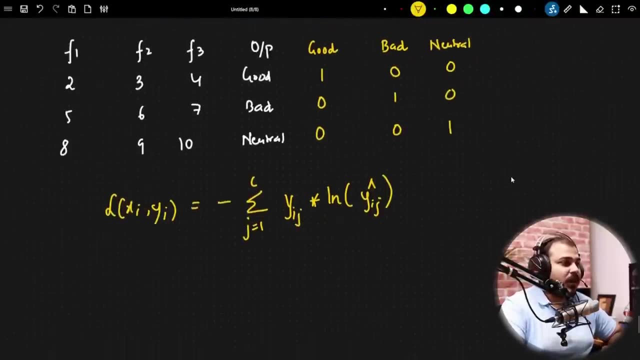 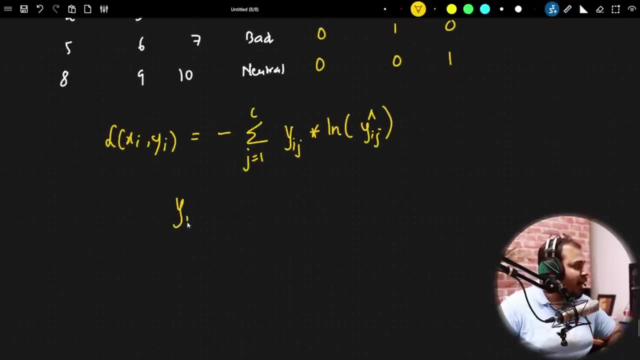 understand what this exactly loss function is basically saying okay, and what all things are, uh, basically coming out of this information, from this. everything right, we'll try to understand. so let's consider, let's consider whenever i write in this way, see, whenever i write y of i. 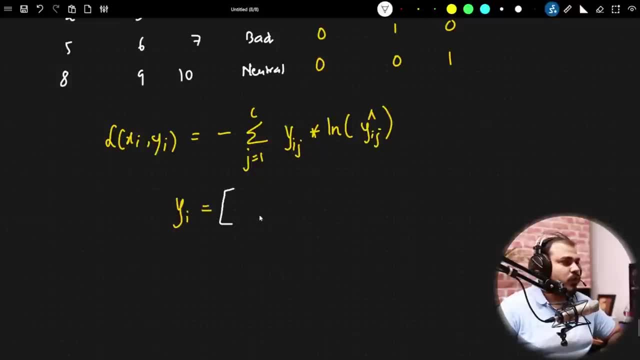 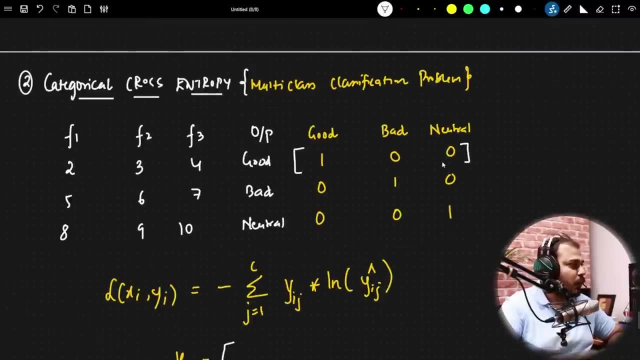 let's say i'm writing y of i. y of i for the first row, for the first row, first row, this row. let's say this is my first row, right? how do i denote it? how do i denote it? i may write, okay, y of i1. y of i1 is nothing but this first one for the first row. this is y of i1. 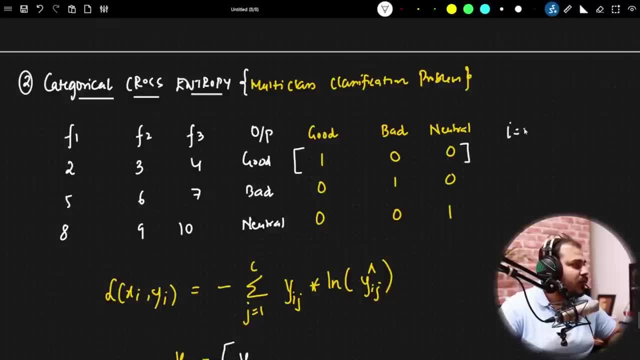 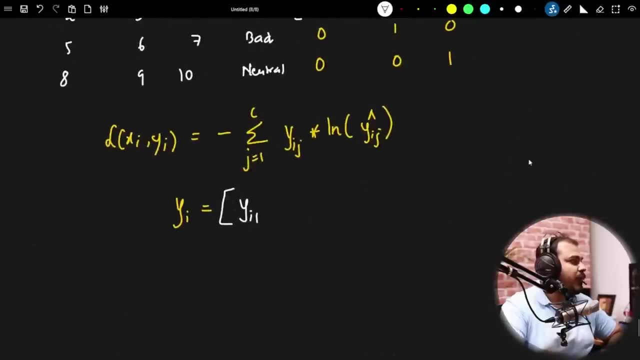 y of i2, y of i3. i is nothing but row. i is equal to row. j is nothing but column. okay, i will just talk about it. okay, i is equal to row and j is equal to top. so if i write y of i1 comma, y of i2, 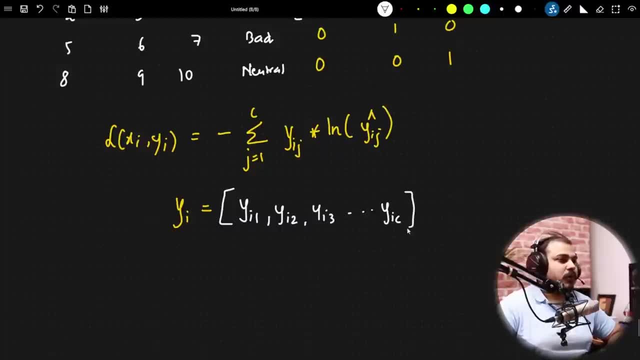 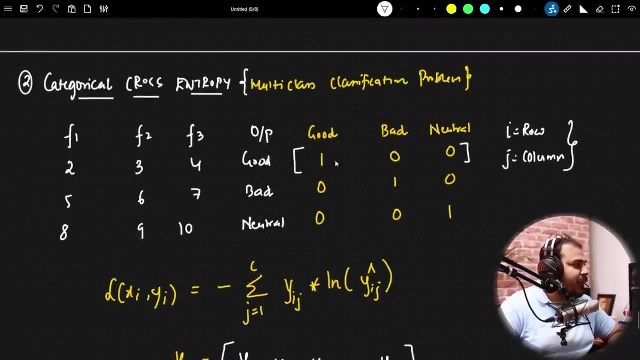 i3. last will be going to y of ic. okay, ic basically means number of categories. okay, now, if i write with respect to y of ij, then two things will be coming. see one if the element, if the element is in class, what does this basically mean? over here, if good is present, then this will become one. 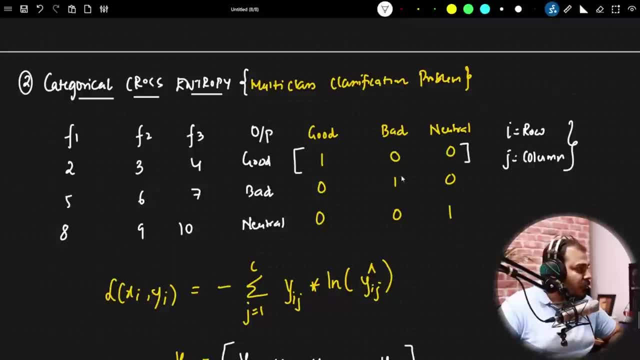 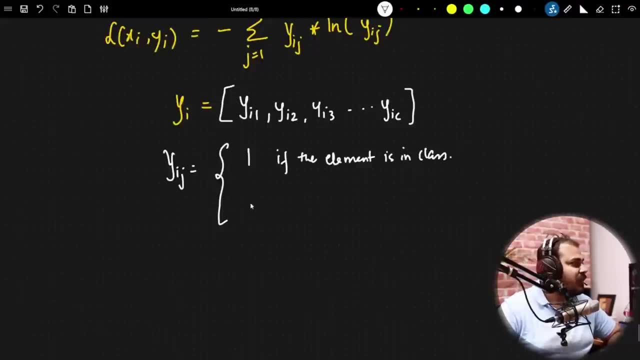 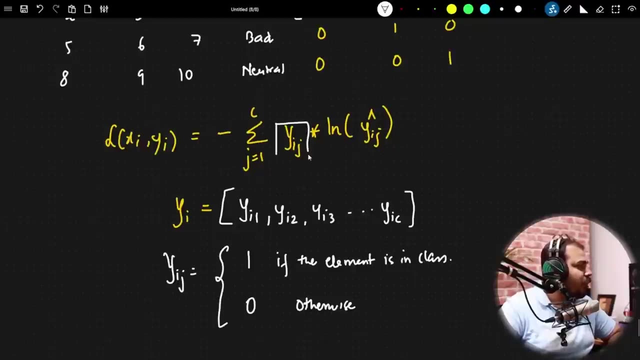 remaining all will become zero. okay, if, if bad is in the way, this will only become one, remaining all will be zero. so here we are basically writing one if the element is in class zero. otherwise, this is how we calculate this y, hat, y of ij, this y of ij. we basically find out in this way. so here is what i am getting: my y of ij. but how do i? 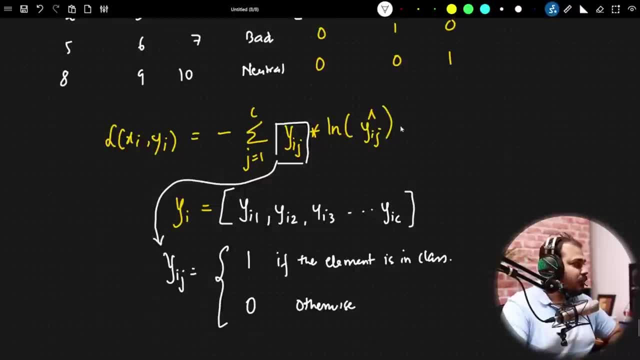 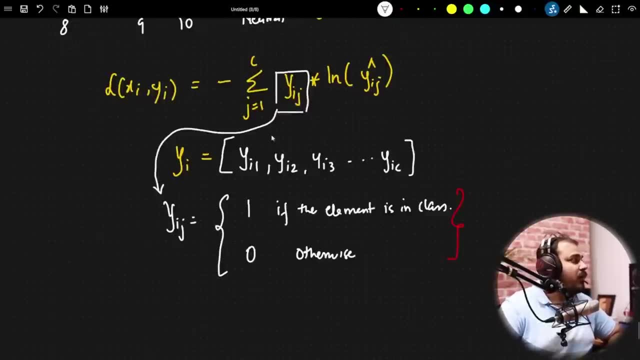 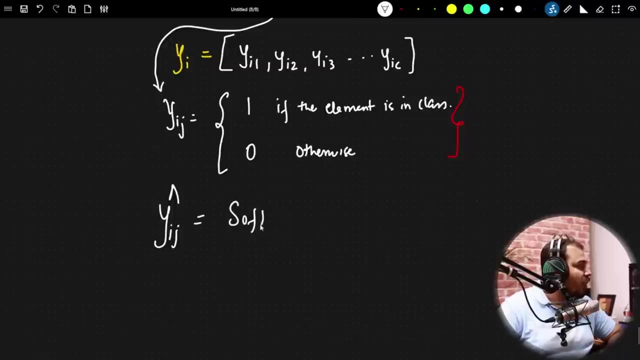 get my y of i ij hat. now we have calculated this right. we got this y of i j, we are able to find it out. but what about y of ij? now, y of ij is basically thought through another activation function, which is called as softmax activation function. this softmax activation function, i told you it is applied in the output. 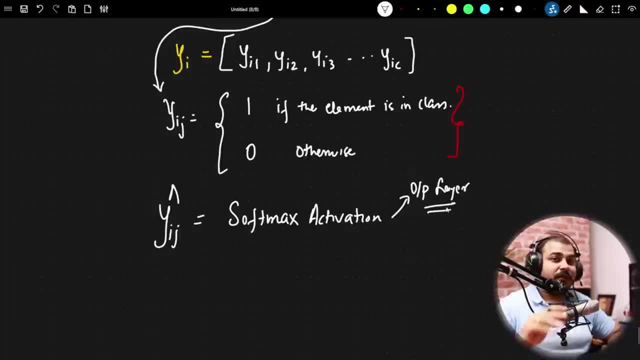 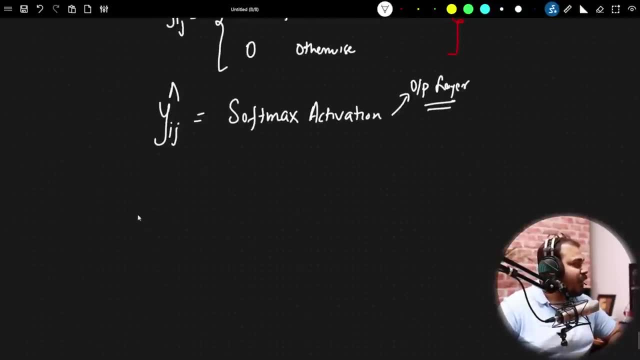 layer for multiple classification problem, right, everybody remembers that. and what is the formula of this? what is the formula of this? the formula is very simple. it is nothing. but we basically say: softmax of any z value is nothing, but e of z of i, summation of j is equal to 1 to k, e of z j. i will. i will explain this thing also. 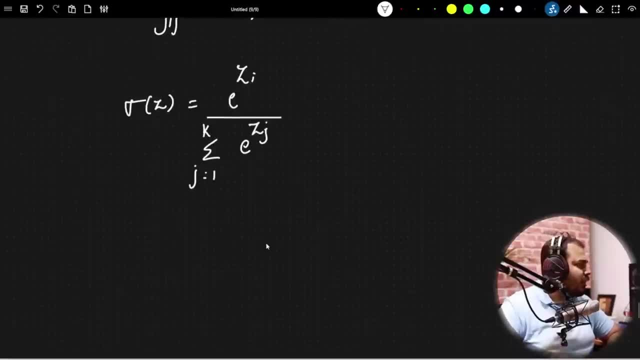 i will explain this thing also. let's say i have a neural network. i have a neural network which has two hidden layers, sorry, two output layer. this is my output one, this is my output two. let's say before i have three hidden neuron. okay, in this layer i had three hidden neuron. so this will 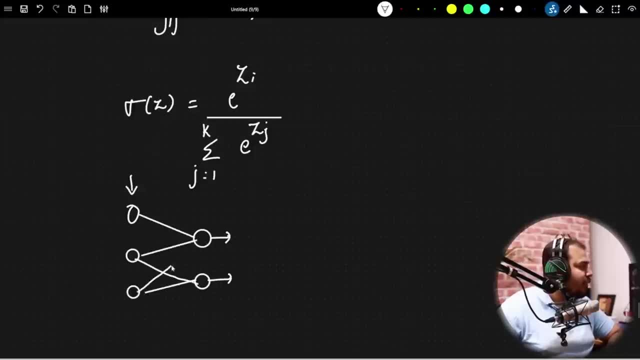 all get connected. Right, this will all get connected. Yes, now, over here, you know, weights will get assigned. right here, weights will get assigned. Let's say, the values that I'm actually getting after multiplying through the weights are something like this. Let's say: I'm getting over here 10, 20, 30, something like this, or 40, right, 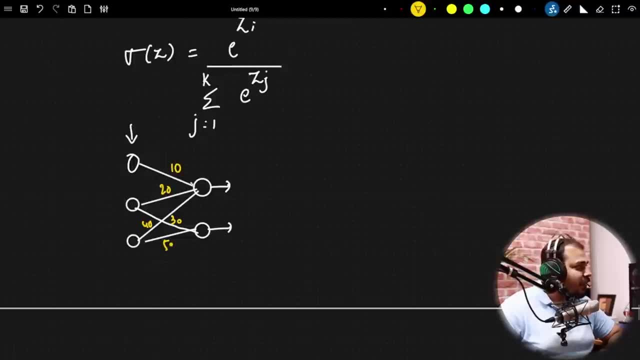 Let's say I'm getting like this and this is 50. now, in order to find out the output over here, What I will do is that I will apply this softmax activation function. Now this will be what suppose I want to calculate for this, For this particular thing. So E of J of I, let's say E of J of I, if I want to calculate for this. 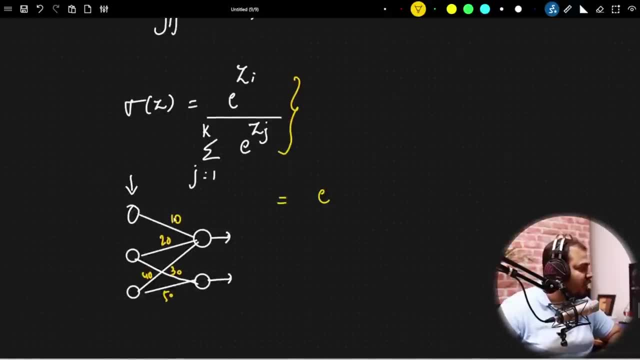 Let's say it will be E of J of I. let's say for this first thing, for this, how much? what will be my probability? So I'll write E of E to the power of 10 divided by e, to the power of 10 plus 20 plus 30 plus 40 plus 50. 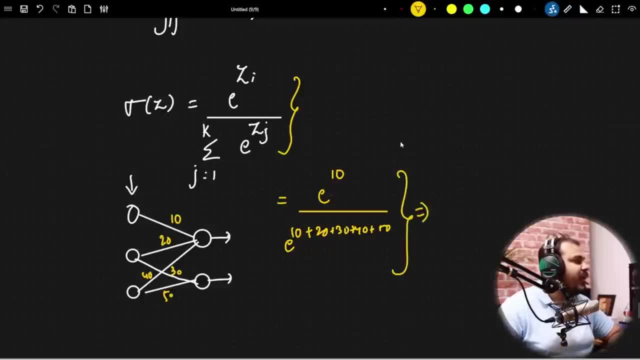 Right, and whenever I try to find out this, this I will be getting in the form of probability Like 0.4, 0.5, 0.6, but always remember both this probability summation will be equal to 1, Whichever will be the higher probability that class output will be coming up. 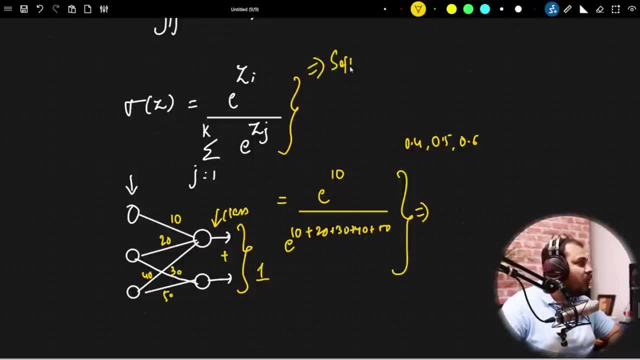 Right, and this activation function is called as softmax activation function. This is basically applied in every output layer, every every output layer. Okay, for a multi-class classification problem. Right, So I hope everybody is able to understand. Okay, now I want you all to understand this: for multi classification problem. 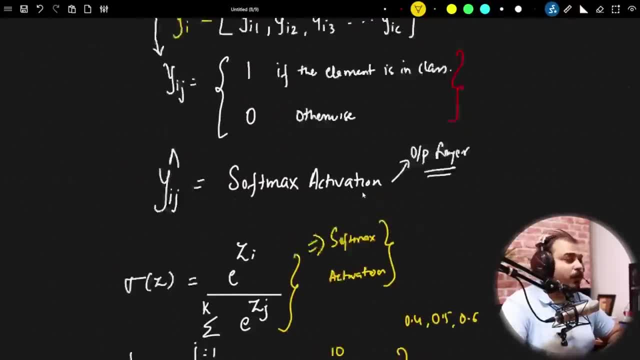 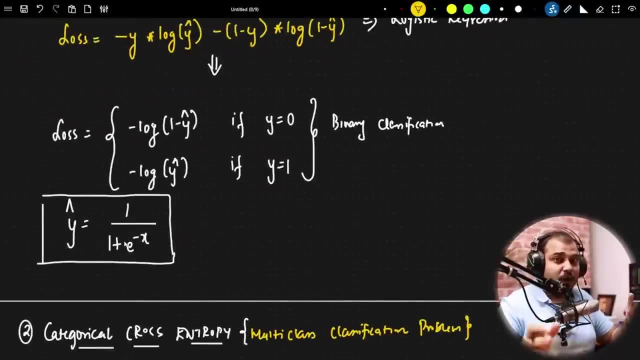 How we are basically under applying softmax activation in the output layer for binary classification problem. We are applying sigmoid activation function. This is the thinking you should basically be knowing, because tomorrow if I'm coding and Showing you how things are basically there- Okay, how things are basically working, you can basically understand. Okay, if it is a binary classification problem. 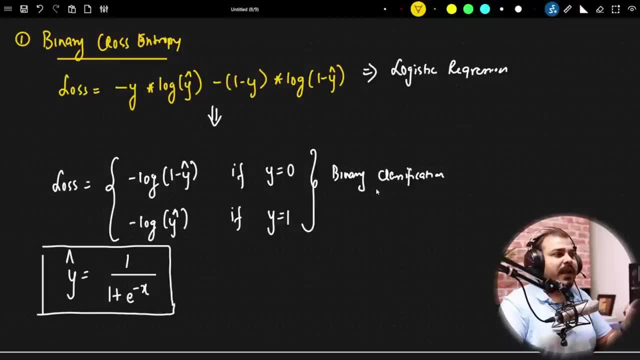 I'll basically be using a ReLU activation function And then in the output layer I'll be using a sigmoid activation function. Suppose it is a multi-class classification problem. in the middle layers I'll be using ReLU. in the outside, in the output layer, I'll basically be using a softmax activation function. 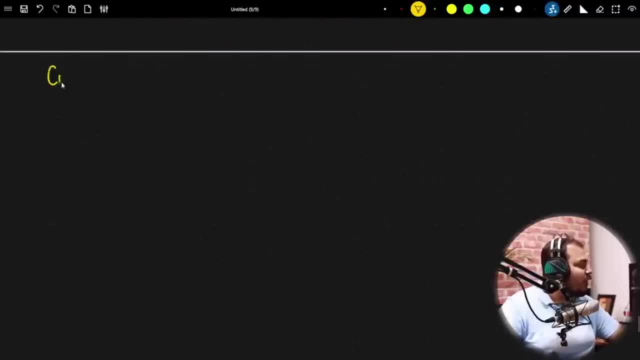 So again, let me repeat the conclusions out of all these sessions, of all this today's session: What all things we learnt. Let's say what, what are things we learnt? Okay, just tell me the answer. Okay, suppose I Use ReLU in middle layer and a softmax in the output layer. 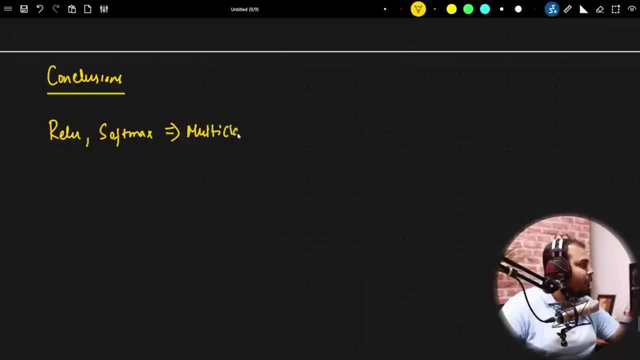 This becomes a multi-class classification problem, right. Multi-class classification problem. I can also use pre ReLU. I can also use this. if I use ReLU and sigmoid, Then this becomes a binary classification problem. right and loss function, what it will be used over here. 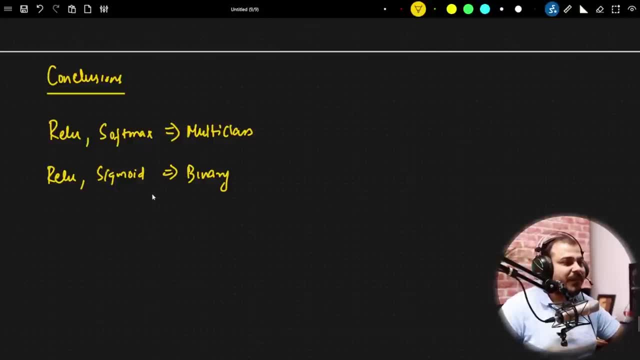 Obviously, you know that sigmoid activation function will be used over there, right ReLU in the hidden layer, right in the hidden layer. Similarly, this is for binary classification, for linear regression. What do we do? We apply a little bit change right in linear regression. We will definitely use ReLU. 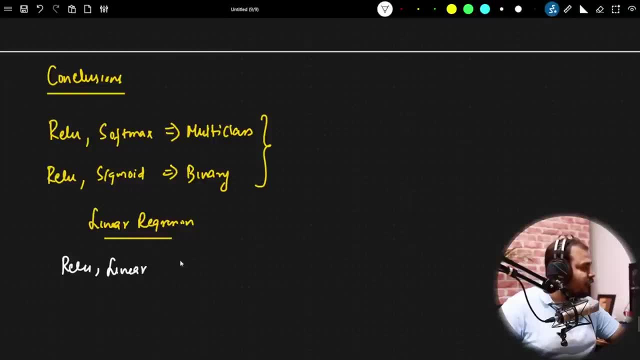 but in the output layer we have now linear activation function. and What is the loss that I apply over here? It will be MSE or MAE, right, or it may be Huber loss Right over here. what I apply for multi-class, it will be categorical cross entropy loss function. 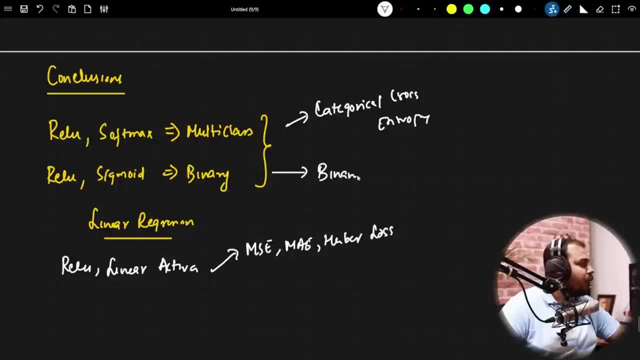 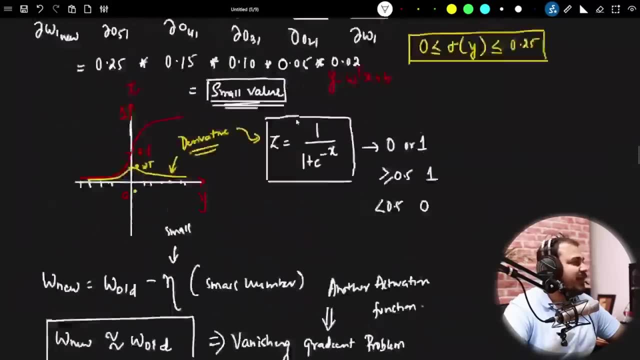 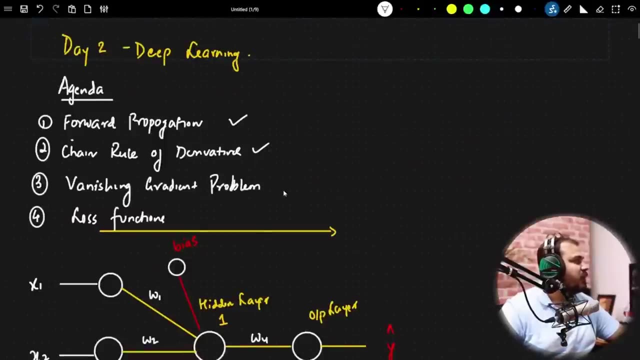 Right, and for this it will be binary cross entropy Loss function. Today we are ending this session now. What are things we learned? so many things we learned right. we completed activation function. we completed everything right. So what all things we learned? we finished forward propagation chain. rule of derivative vanishing gradient loss function. 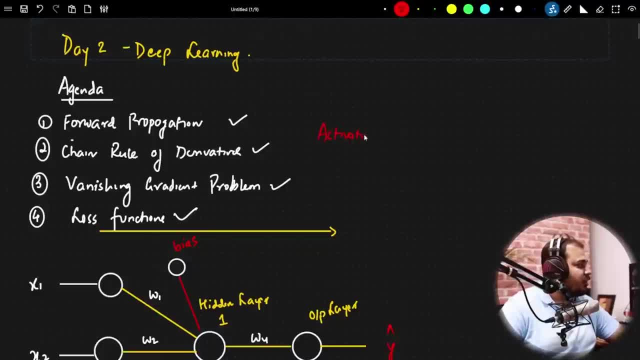 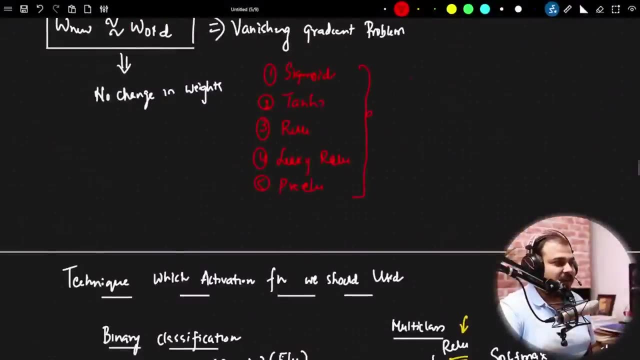 And then we also understood activation functions right. So all this things is basically completed right, and these are all interview questions. guys, They will definitely ask you all this kind of interview question. So how would you like to rate out of 10?? You can definitely rate me and if you like my session, definitely like it. 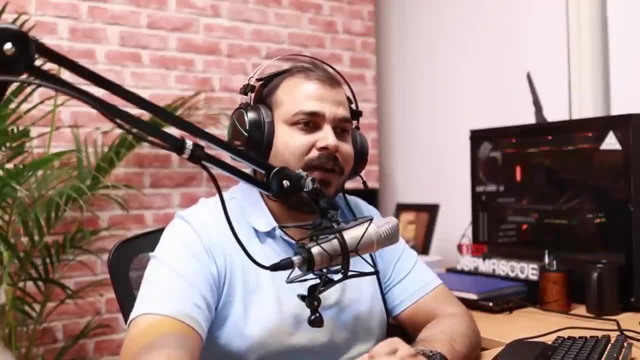 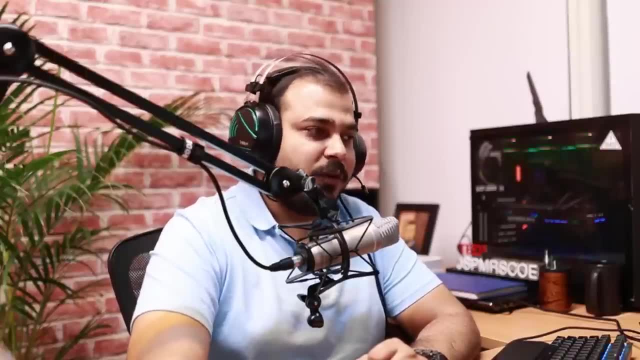 So tomorrow we are going to discuss about optimizers, and once we complete optimizers, We can see some examples of how to implement an ANN, and probably we'll come to try to complete it tomorrow itself. Okay, So, thank you guys, Have a great day, Keep on rocking, keep on learning. 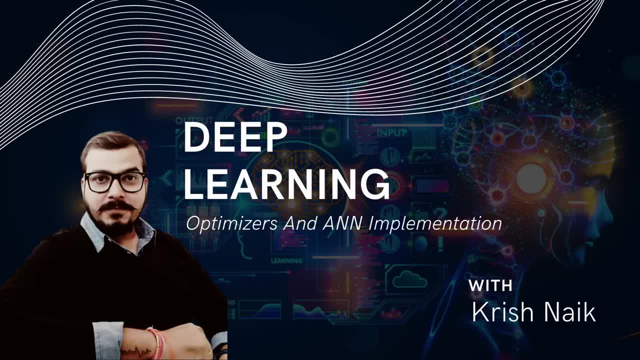 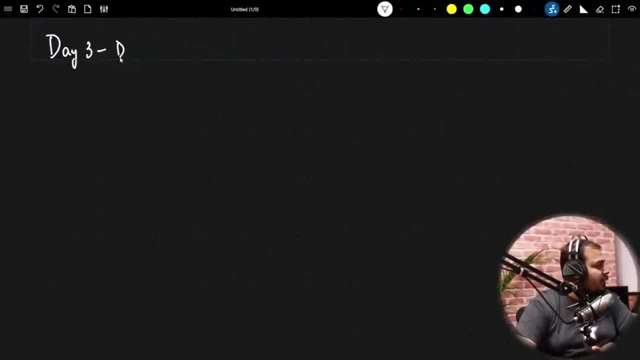 So day 3, Deep learning session. We are going to discuss about this today. Okay, day 3, deep learning. what are topics, agenda, what all things we are going to cover? Okay, the first thing is very much important, which is called as optimizers. right, 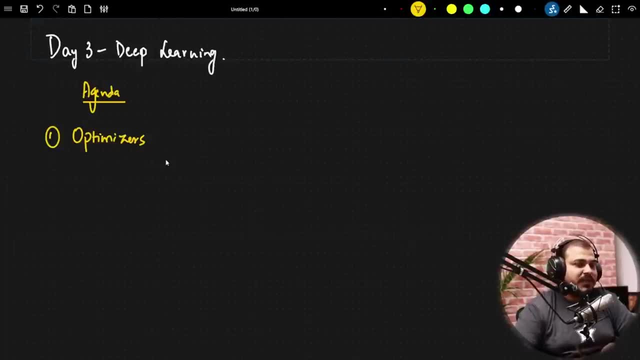 Optimizers are very much important In the back propagation to understand how the weights are getting updated and there are different, different types of optimization. Now, what all different types we will be learning today. So obviously we have covered gradient descent. Okay, You'll understand gradient descent. then we have something called as SGD, which is called as stochastic gradient descent. 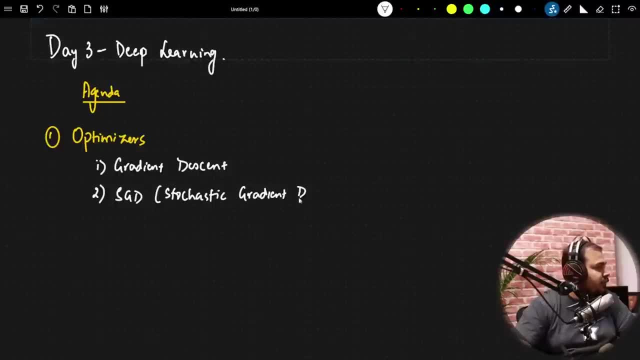 Stochastic Gradient descent. Third thing that we are going to cover is the gradient descent. Fourth topic that we are basically going to cover is something called as mini batch SGD- stochastic gradient descent. fourth topic that we are basically going to cover: SGD with momentum. Okay, so that part we are going to covering in the third or after this. in this we will basically be covering SGD with momentum. 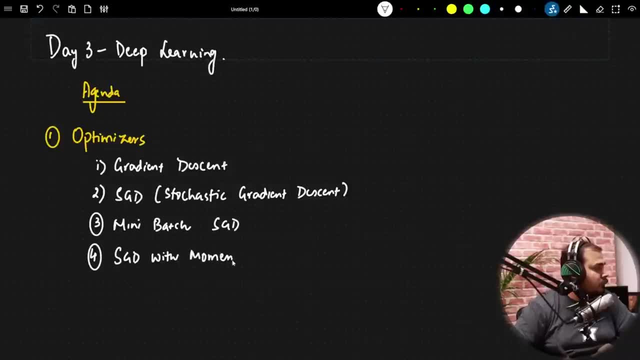 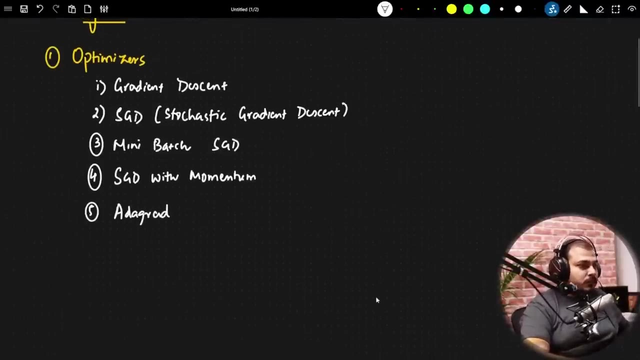 Then we have something called as Stochastic gradient descent, Stochastic gradient descent, Stochastic gradient descent At a Grad, So At a Grad adaptive gradient. We're going to cover this, okay. And The sixth one that we are going to basically cover is something called as RMS prop. 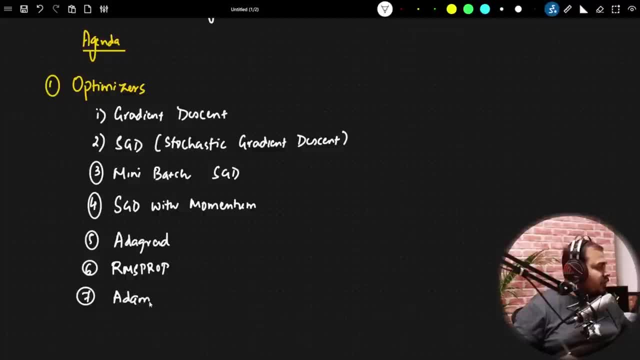 And finally, we will try to see ODM optimizer, which is currently the best optimizer which is going on in the market. many people uses this right along with this. So we are also going to cover what is what is batch, what is epochs, what is iterations. we are definitely 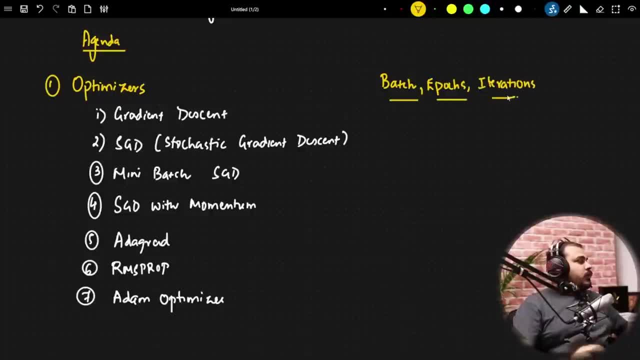 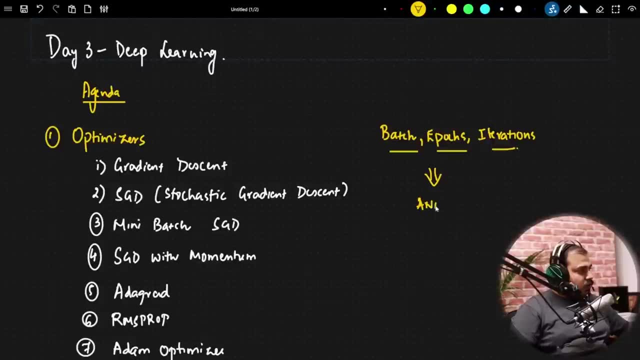 going to cover all these things. okay, so this is the agenda of this session. let's see whether we will be able to cover this and then, after this, we, if we get time, we will also be solving an ANN practical problem. and if you don't get time, don't worry. tomorrow we are going to cover the ANN and probably the CNN. 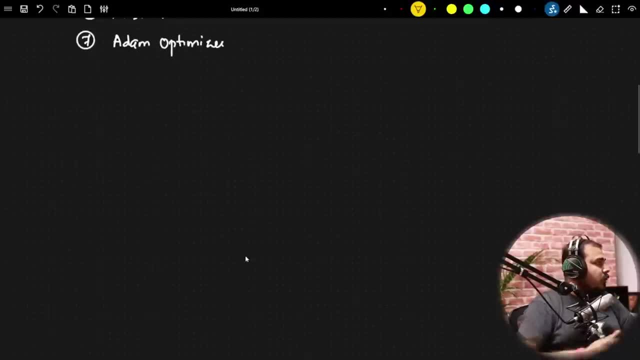 part. okay, till then I will start this one. so first optimizer: obviously we have seen about something called as gradient descent. okay, and gradient descent, we know what is the main: weight updation formula in the back propagation. weight updation formula and the back propagation, that is nothing but. 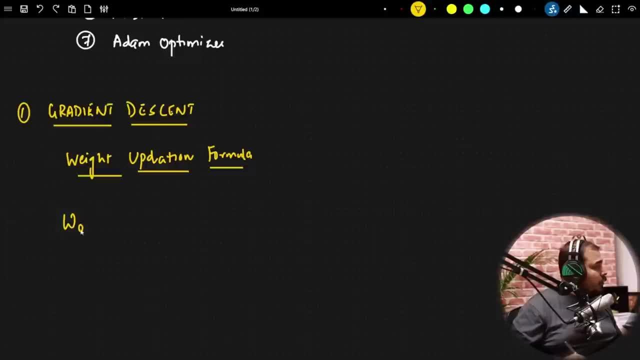 so what that means is that the gradient descent- it should have been something like weight old- sorry, weight new- is equal to weight old minus learning rate of derivative or loss with respect to derivative of W old. okay, so this is the first equation. I hope everybody knows about this because since we are discussing it from yesterday. so everybody should be well known with this specific thing and whenever we talk about gradient descent, we know that what we told you about gradient descent has something to do with matlab and ES. cabf are importantxter, and know that you have the possibility that if you are跑ing yüzden prison for every cell generation, this element can be something like a question. 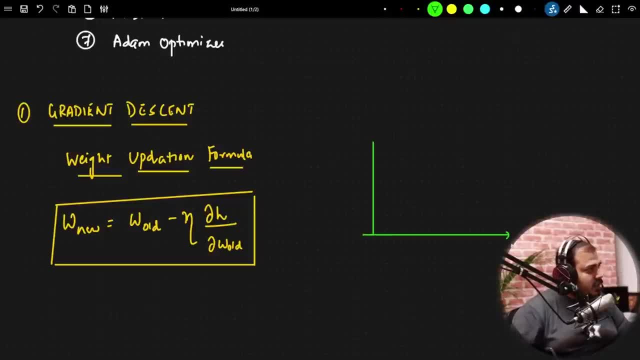 what we specifically have. we have in our X and Y axis. with respect to W, we will basically try to see the loss or cost function and we know that what happens? we get this kind of gradient descent right and this point. that is basically this. this is my global minima right and we have also understood what is the 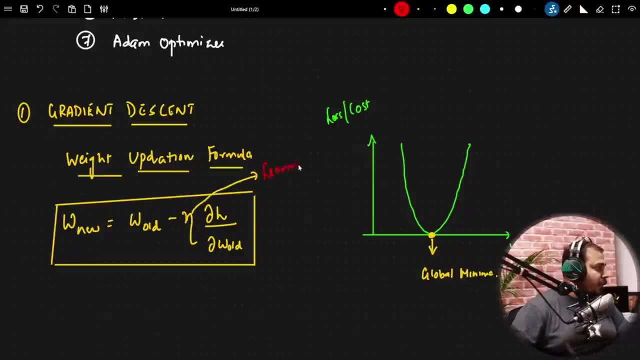 importance of this specific learning rate, this specific learning rate. that also we have understood. okay, and whenever we have any kind of points over here, what happens is that either we can increase the weight or decrease the weight, but our main aim is basically to come to the global minima. now let's go. 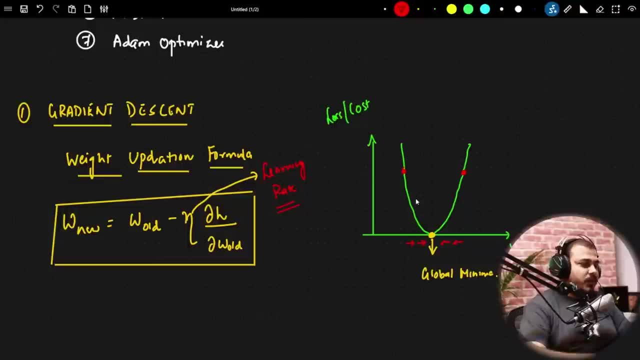 ahead and take one step ahead and try to understand different things. okay, now let's let's say: I have already told you that you have to take a step ahead and try to understand different things. okay, now let's let's say: I have already told you that. 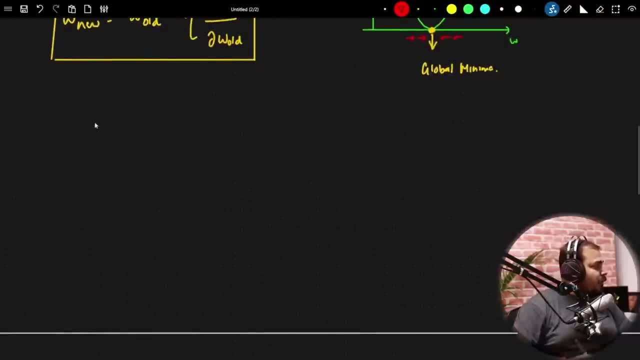 the difference between loss and cost function right now what part we are specifically discussing. let's say, I have my input feature. this is my hidden layer and this is my output layer. so if I'm connecting this, all dots- okay, if I'm connecting this all dots, this becomes my hidden layer, this becomes my. 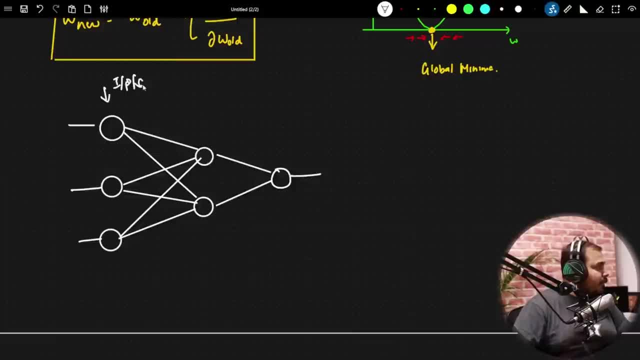 input layer. so this is my input layer, this is my hidden layer one and this is my output layer. you can have any number of layers, that is not a problem. so in forward propagation, what we do, we multiply it by the input weights and then we apply an activation function and 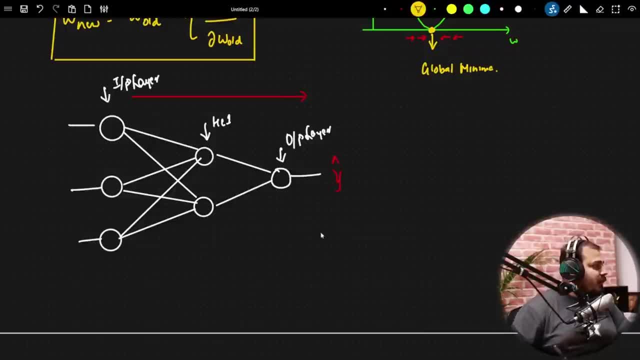 finally over here, I get y-hat and then we go ahead and define our loss function. one of the loss function is nothing but mean squared error, so I can basically write 1 by 2n. okay, yesterday, when I was discussing about the in the previous 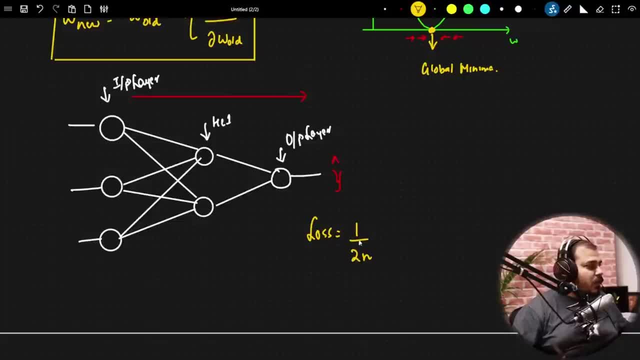 session when I was discussing about the loss function. at that point of time, you know, I used to write 1 by 2, okay, but I missed that n part, okay. so please do make sure that you write n. then i is equal to 1 to n. y minus y-hat whole. 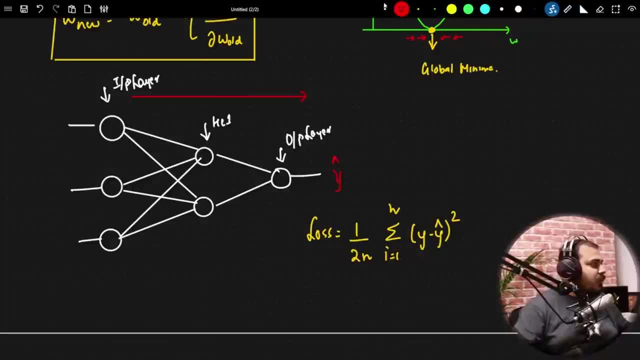 square. so if you talk about this, this is basically called as mean squared error. okay, so this is nothing, but it is a mean squared error. okay, this is the loss function that is basically getting applied. okay, then, in the backward propagation, our main aim is that we should basically update all this weight. 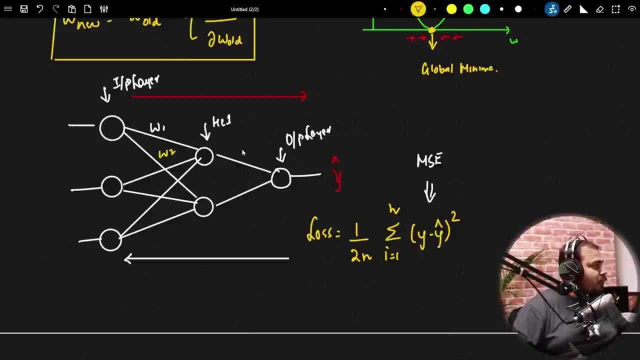 so 1, 1, w1, whatever weights you are basically having over here- w2, w3, w4- we need to update this weights for updating this weights. to minimize this loss function, we use optimizers. now, one example of the optimizers that we specifically use is: 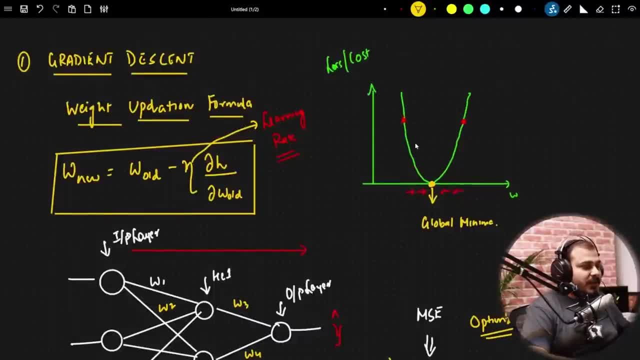 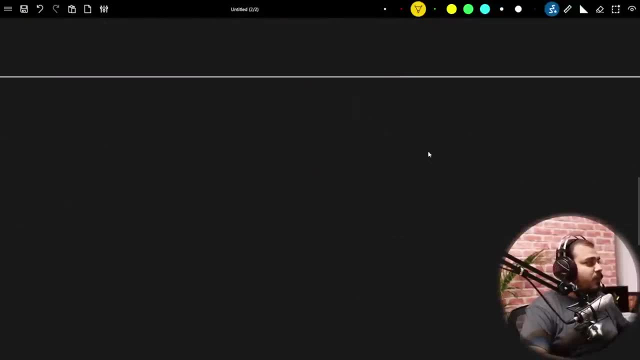 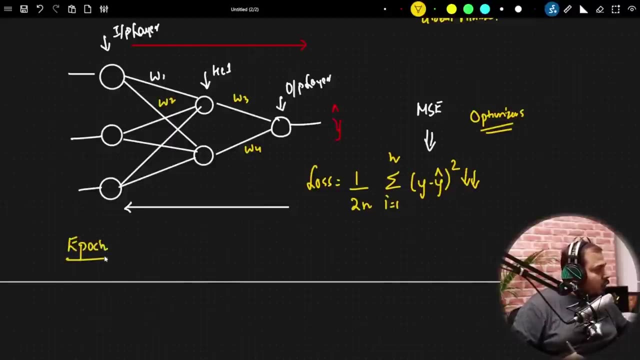 this is called as this gradient descent optimizer. now, in gradient descent optimizers, you know, what we do is that we pass, and first of all, before that, let's understand what is epoch. okay, so you need to get an idea about epoch now. what exactly is epoch? epoch? okay, i can call this as. 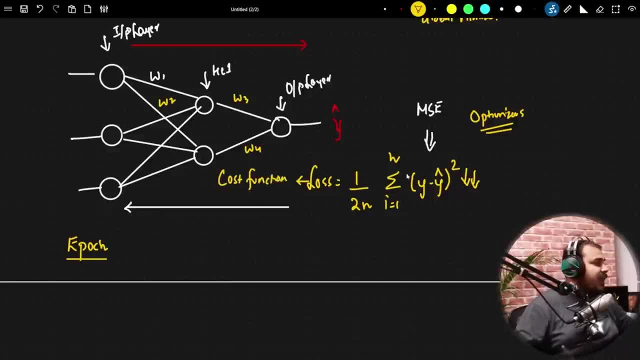 cost function. okay, this has cost function, but since i'm passing n data points, now what does epoch mean? epoch basically means, whenever i do one forward propagation and one backward propagation, this combines and says that, okay, we have basically passed one epoch. okay, one epoch. so if i have, let's say, if i have, million records, million records in my data set, okay, if i. 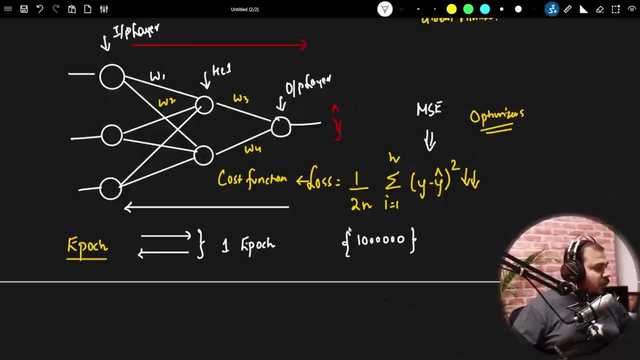 specifically have million records in my data set. now, if in the forward propagation at a time i'm actually, you know, getting, i'm giving million records at a time, i'm giving million records after giving, i'm getting y hat and i'm finding out the loss, okay, loss, i'll not say loss, but at least i'll say cost function. 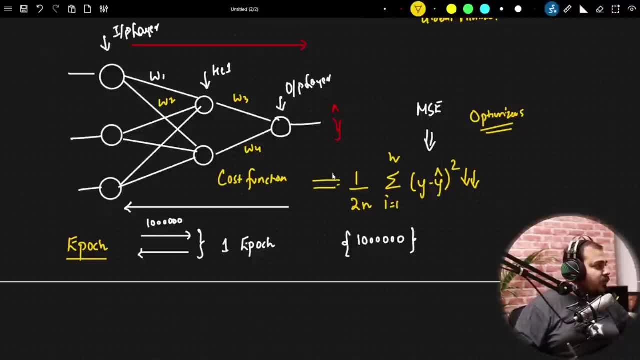 let me remove this. okay, suppose if i'm trying to find out cost function now, when i'm finding out cost function, the formula becomes something like this: right now, that basically means i to the one, that is, summation of i is equal to one to million. okay, so million. 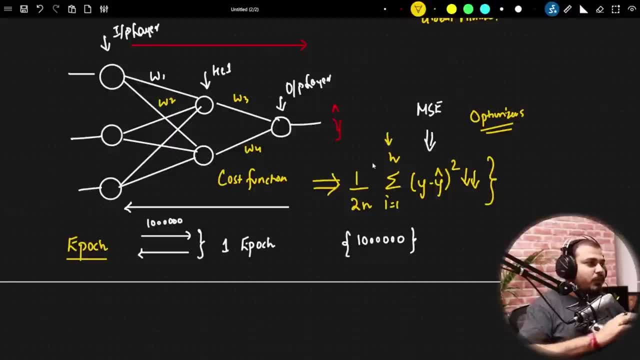 this n will basically be million. okay, so in basically what we are doing in the forward propagation, we are doing million different calculation of different inputs and weights, because they are million data points and at a, at a batch, we are taking million data points and we so in the backward propagation. then what will happen? all the weights will get updated and this 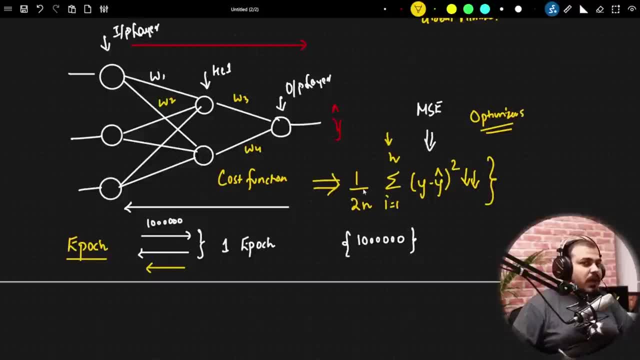 all weights will get verified and at some point this is just a mask and this is just a nutzen and will be getting updated based on this loss. now understand what is the disadvantage with respect to gradient descents if, when we are passing million records, just imagine million records. so the first disadvantage that I would like 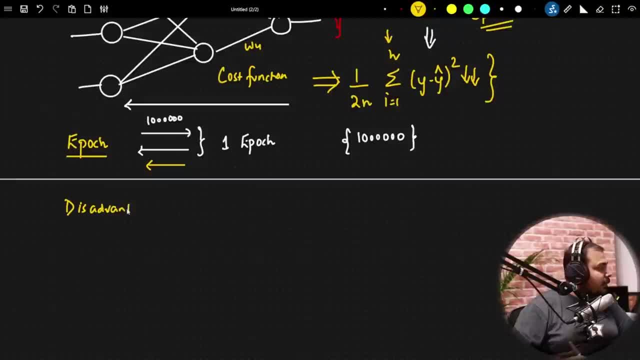 to talk about is basically is basically that if you are passing million records, definitely you require a huge RAM to load that records. right so resource extensive task it is. so the task is very resource expensive. you require huge RAM to accommodate million records in every epoch right so huge. it is like huge RAM. 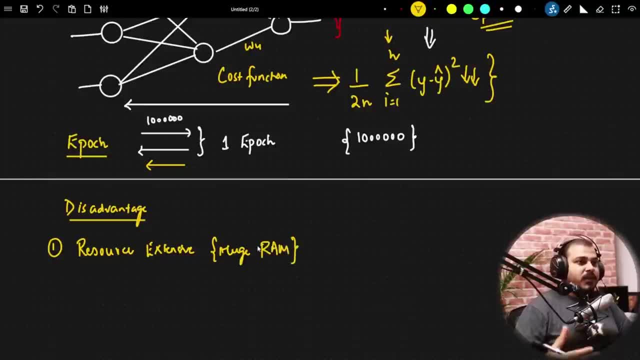 size at least you will require. again, for parallel processing, you also may be requiring GPUs, because million records processing is basically happening. right, it is obviously fast, we will be able to reach to global media, but just to run this we really need to have a big system, right? so this is the major, major disadvantage. try to understand why I'm. 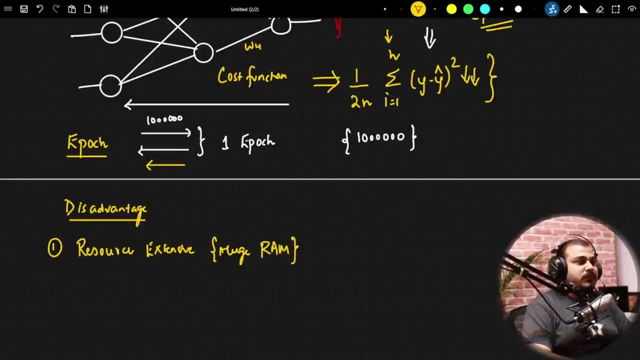 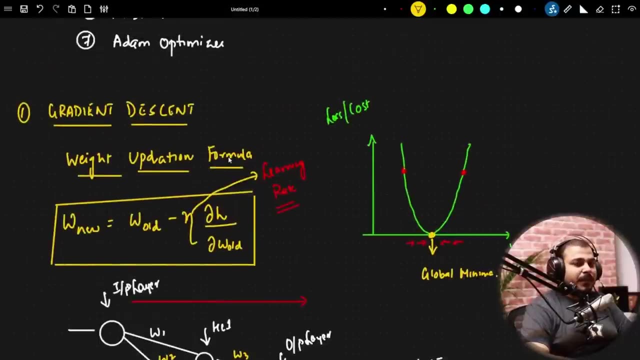 saying major disadvantage right over here. you can clearly understand that I cannot like, if I am using million records at every epoch, right, how much resources I will be requiring, right? so this is a major disadvantage with respect to gradient descent. okay, so what do we do? can we tweak this optimizer? 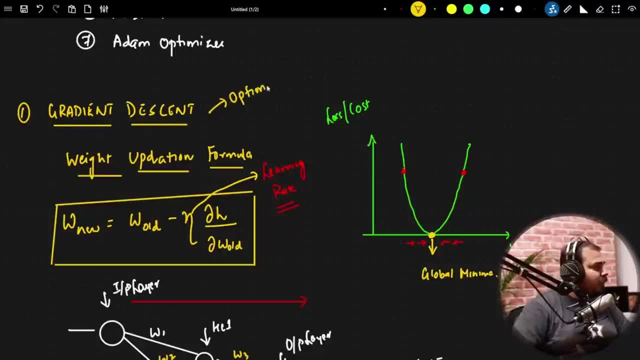 this is an optimizer. this gradient descent is a major, major disadvantage. this gradient descent is basically my optimizer. can I use some other optimizer which can make sure that with little bit number of resources also I'll be able to work nicely? okay, so for that, the second part that we 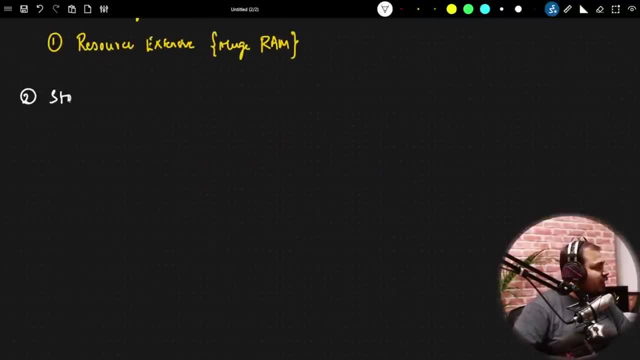 specifically discuss about is something called as stochastic gradient descent, stochastic, stochastic gradient descent and stochastic gradient descent. what we do, let's say that, okay, fine, we have million records, we have million records. that' fine, we have million records, we have million records. let's find millions of. 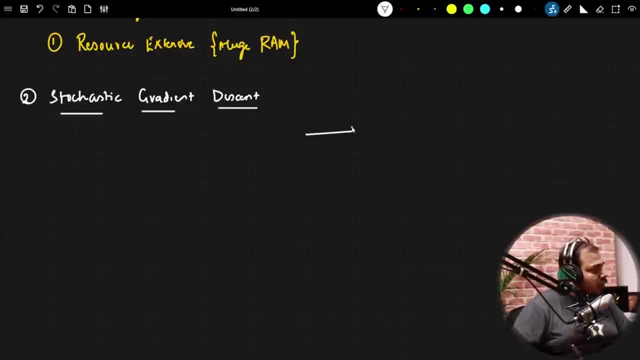 tests. let's say that, okay, fine, we have million records. we have millions of million records in every epoch, which is a combination of forward and backward propagation. let's say, in the epoch one, I just pass one record, that's it. I pass one record, I calculate the y-hat and then I calculate the loss, and then I. 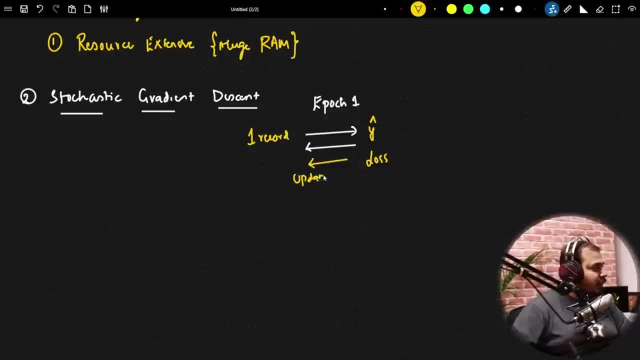 update the weights right. this step is basically updating the weights. now, if I have 1 million records and in every epoch, in every epoch- like, let's say, in side this epoch- I am passing only one record, still there are so many that still there are millions of records that is left. so when I pass one record in the 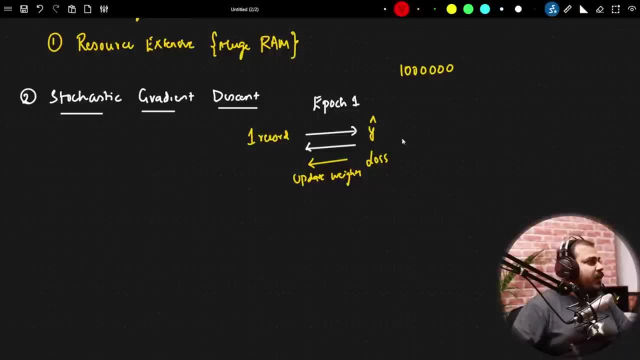 forward propagation. in the backward propagation I update the weight. this will basically called as iteration 1. now we are dividing this inside the epoch based on the data points we are dividing it, so this will now become iteration 1. now in the iteration 2 we will pass the second data point for doing the forward. 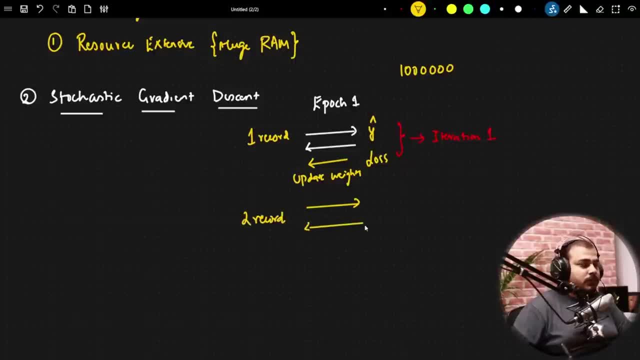 and the backward propagation. so now, here I will pass the second record and this will be my iteration 2, right? so like this, how many number of iteration I will have? how many number of iteration? just just a normal guess, since there are million records, okay, since there are million records, it will be going till. 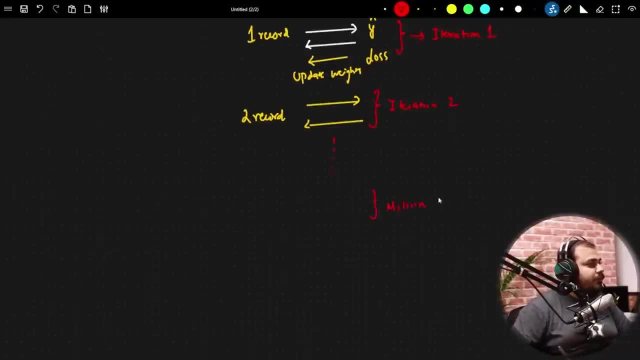 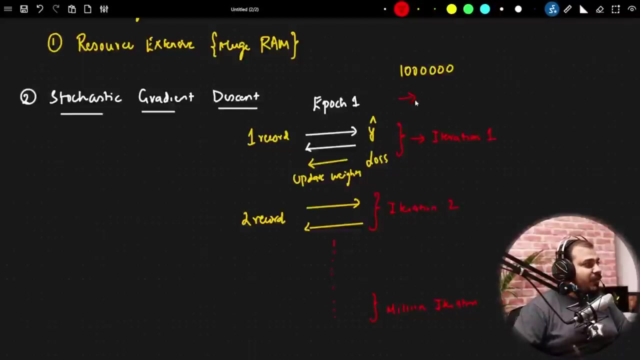 million iteration right, million iteration, million iteration if we just pass one, one record. so in every epoch we have to pass through million iteration. if you are just providing one record at a time and like this, we usually run for many number of epochs. when we are training this deep learning model, right, when we are training at least, we run with hundred. 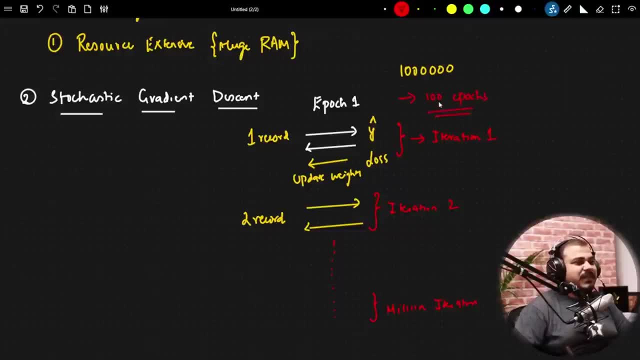 epochs. I'll be talking about this early stopping and all, but just let's say we are running it for hundred million, hundred epochs. so in every epoch, million iteration. just imagine for hundred epochs how many millions iteration will become simple, it is hundred million iterations right in this, in this step, in. 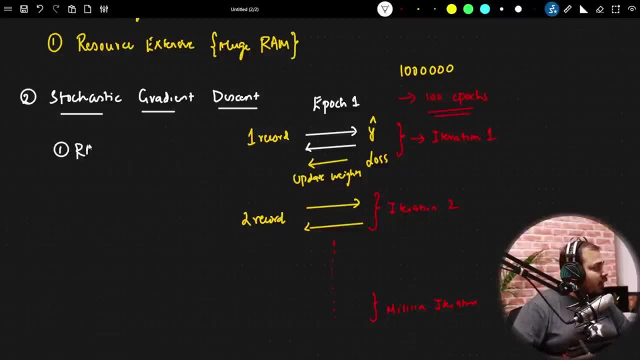 stochastic gradient. addition, you are making sure that you are not just passing one record at a time. I will not require that much RAM. no, I don't require that much RAM because I'm just passing one record at a time. but what is the major disadvantage? major disadvantage is that the convergence 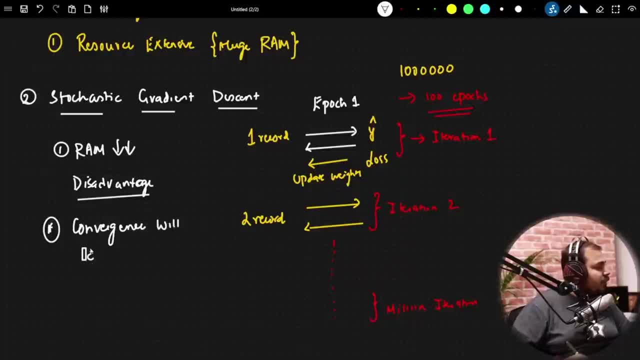 that is basically happening will be very slow. the convergence will be very slow, will be very, very slow. I hope everybody agrees with this. the convergence will be very, very slow. one record, then again back propagation, then again weights are have updating, you know. so the convergence will be very, very slow. this is the major disadvantage. 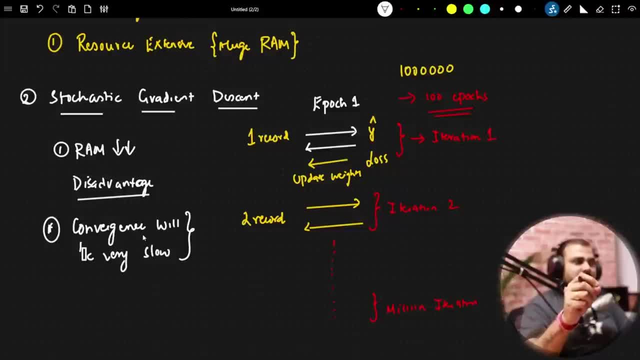 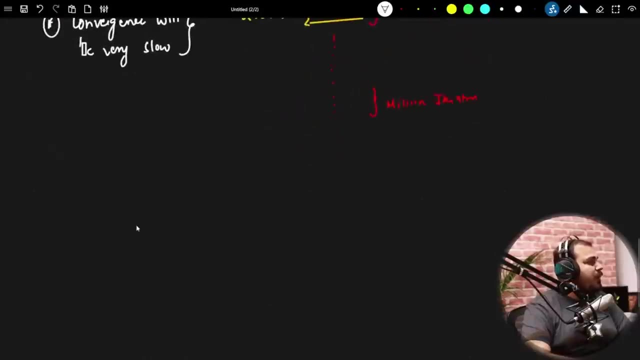 with stochastic gradient descent. okay, so now researcher will not keep quite. okay, it's one has come up with this, he has written PhD, is given, he's got a PhD. now he has written a research paper. there is some problems in this. now how do we fix this? then we go with the next optimizer, the third optimizer that we specifically. 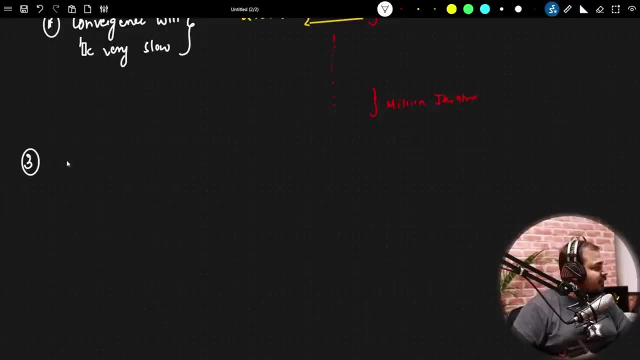 have. that optimizer is basically called as that size. let me take the full name over here: mini batch SGD. mini batch stochastic gradient descent. now, what is this mini batch stochastic gradient descent? let's, let's understand it in a better way. okay, let's, let's try to understand. okay here, what more problem? 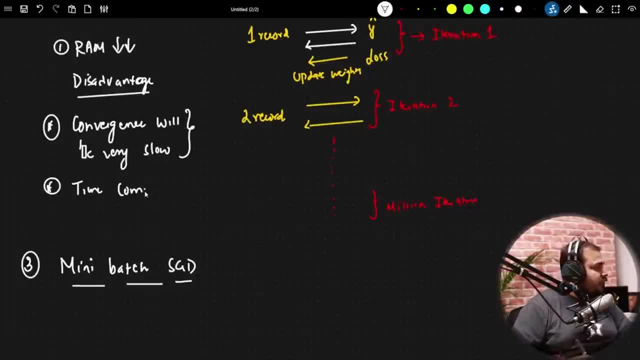 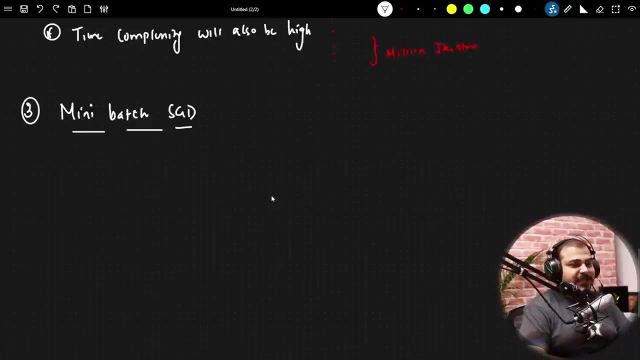 the current time complexity will also be very high. time complexity will also be also be high, obviously, dissolving the record resource constant, but time complexity will still be okay. now, what happens in mini batch SGD, let's understand. okay, nine mini batch SGD and mini batch SGD instead. now see, suppose, if I have one million records now instead of just. 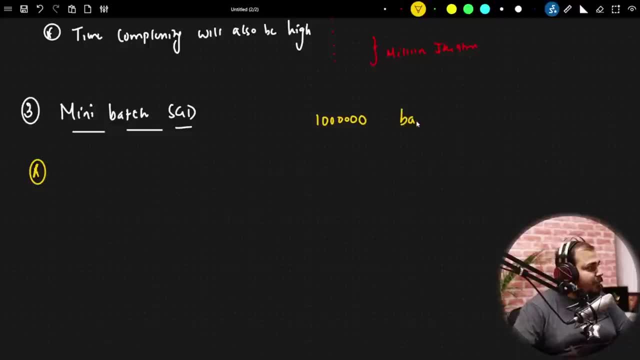 giving one record at a time. what I will do. I set up a batch size. let's say my batch size is now thousand. now, if my batch size is thousand, that basically means in every epoch that i do forward and backward propagation. let's say this is epoch one. i give thousand records, obviously because in every batch size i give means, in every. 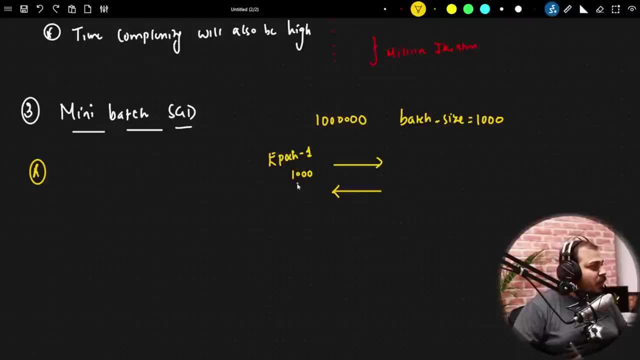 epoch i give, or inside every epoch i give, thousand records. let's say i'm giving thousand records over here in the forward propagation and backward propagation. okay, then total number of this will be my iteration one. right, this will be my iteration one. okay, so how many number of iteration will i? 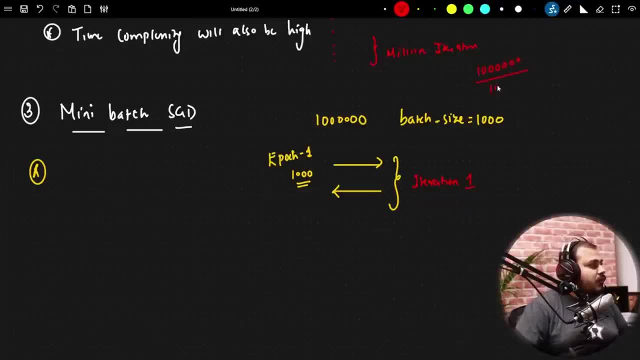 have to do: just divide million by thousand, then this will get cut, this will get cut, this will get cut. so that basically means now in the second iteration i'll give another thousand. so in iteration two i'll give another thousand records, data points. so like this: now i will be able to reduce this number of iteration to just thousand. 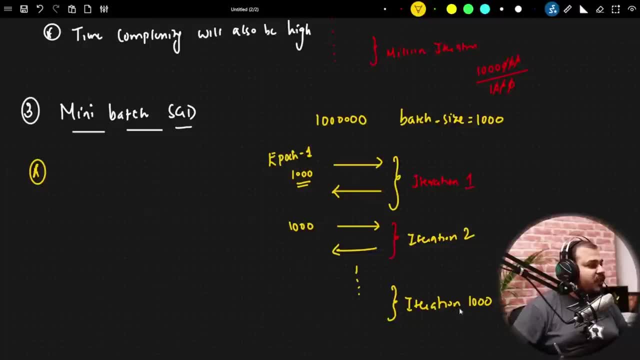 i will be able to basically just do till the number of iteration, that is, thousand, and with respect to all these things, my data points will get covered. now this looks a better approach. because why? because here now it is not that much resource intensive. we have removed this resource. 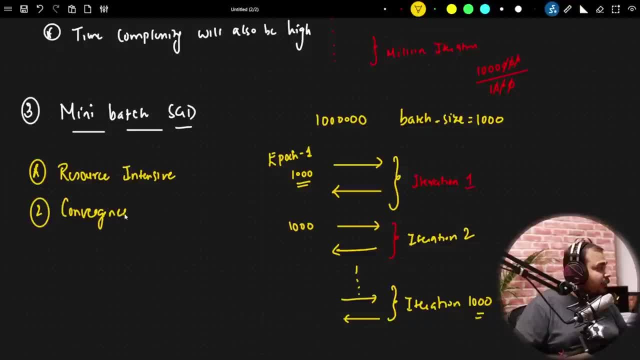 intensive. the second point is that convergence will be better when compared to the will be better and time complexity will also improve. time complexity will improve. i hope everybody agrees with this three point, and this is what we are able to do with the help of mini batches, gd. 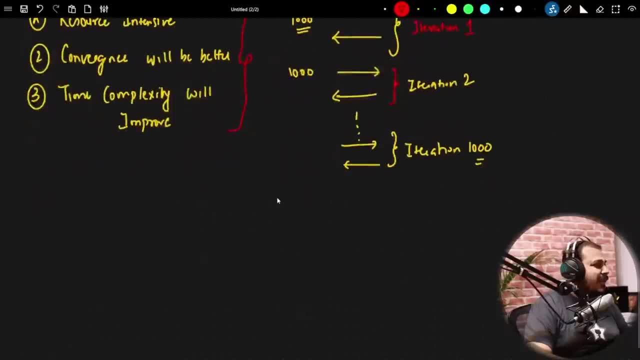 okay, now let me just show you through diagrammatically. okay, how will my gradient descent look like? so suppose this is my gradient descent. let's say this one. okay, my aim is to basically come to this global minima, global minima. okay, my main aim is basically to come to this global enema with the, with the help. 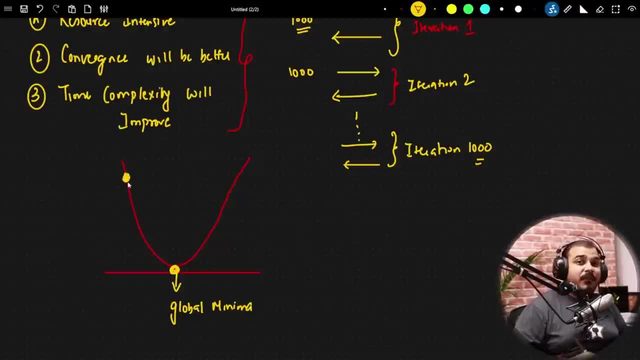 of. let's say, my first data point is over here. okay, with the help of gradient descent. first, we'll understand gradient descent. with the help of gradient descent, since we are passing millions record at one time, the convergence will happen like this: okay, the convergence will happen like this with gradient descent, but there are problems. what are the problems with gradient? 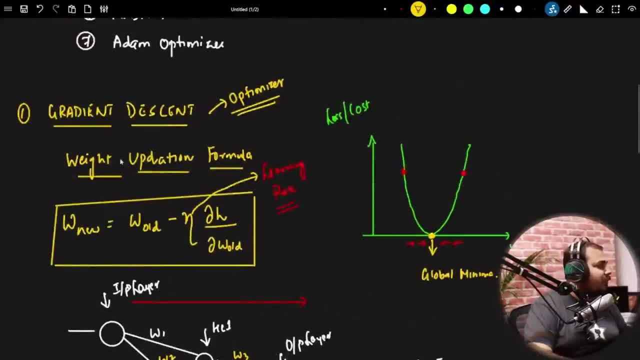 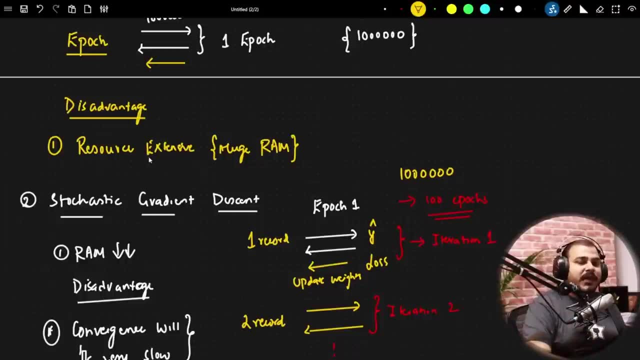 descent. we have written over here. right, we have written over here. the problem is that it will be resource extensive. we don't have a high ram to upload all the millions of record at one time. if we have a huge machine, this will work. you know the convergence will go down like this. that is fine. 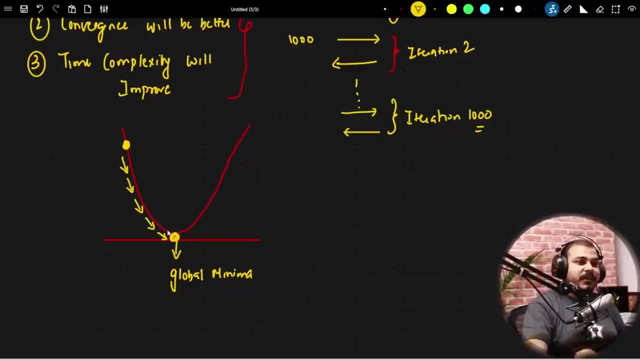 if we use stochastic gradient descent. if we use stochastic gradient descent. now, here we are giving record by record right, just one data point. so how my record will go with respect to one data point. let's say it will go like this: it will jump. like this it will jump. 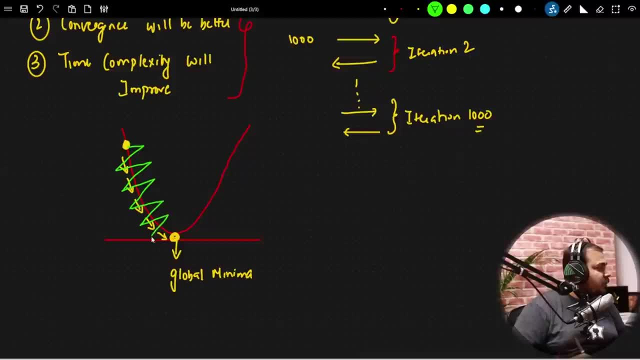 like this. this is with respect to stochastic gradient descent. the green one is basically with respect to stochastic gradient descent. the yellow one is basically my gradient descent, the stochastic gradient descent. why it will have so much zigzag? because it is only taking a single data point and it is updating the weights. so, because of this, so because of this, what will? 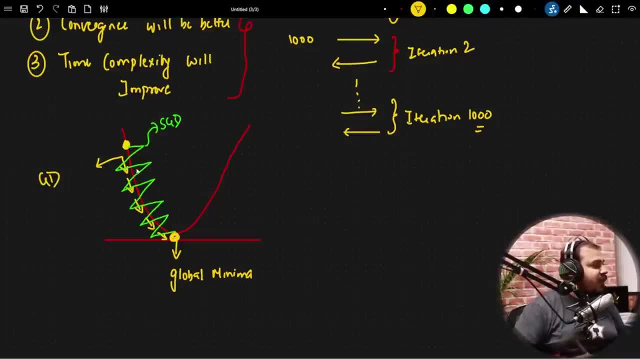 happen so many different different uh iterations, or so many different different ways. the movement will happen and this will basically happen because of sgd. now, with mini batch sgd, what will happen? this: this zigzag movement will be less. it will move like this. this zigzag movement will be less. it will move like this and we will be able to reach the global. 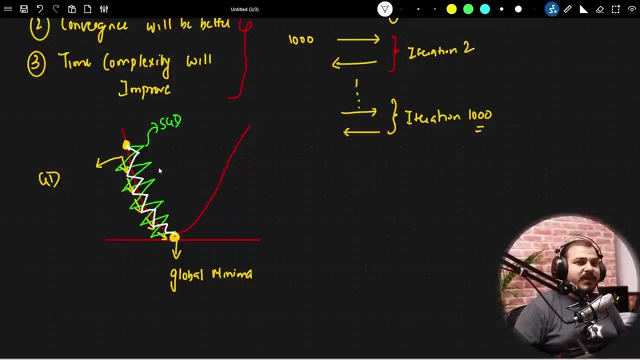 minimum, but still this zigzag movement is there and this zigzag movement is basically called as noise. this is called as noise which is having the highest noise. obviously, sgd is having the highest noise. gradient descent is having the least noise. and if i talk about mini batch sgd, which is this: 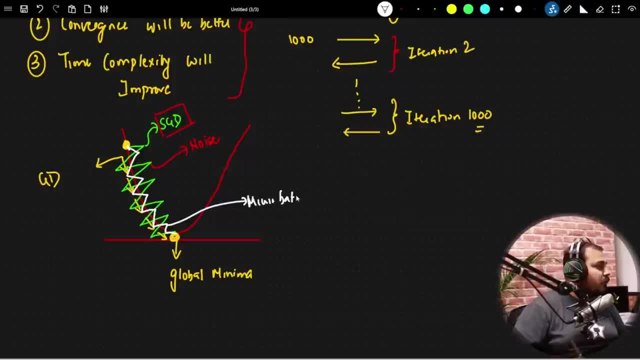 white line mini batch sgd, sgd. this has very minimal noise but it has noise right. the highest noise is basically with sgd. if we have noise, then it will definitely take time to basically come to the global minimum. let's let's consider: i want to climb a mountain. suppose this is my mountain. okay, 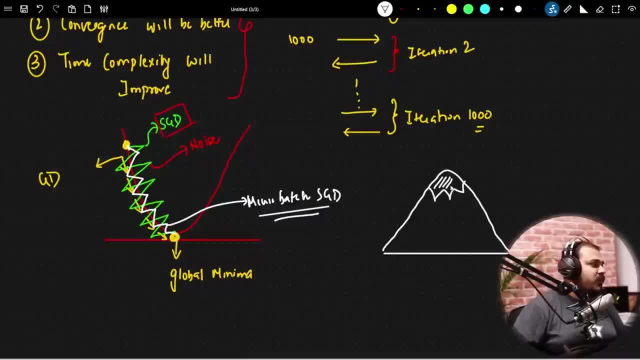 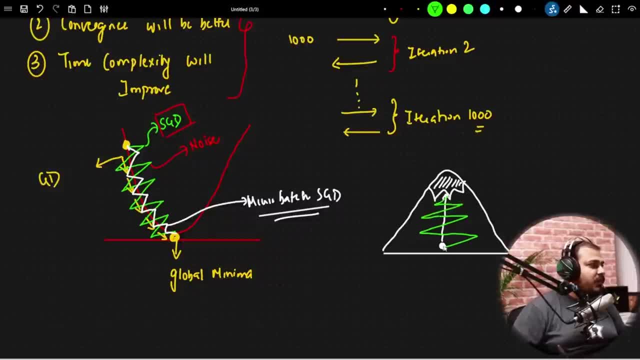 it will take time to reach to the peak. and what if the person just iterates or moves in this direction in this way, like this zigzag movement, then he will be able to reach better than this particular green person. right, it is that we have to reach this point. this point over here is global minima. 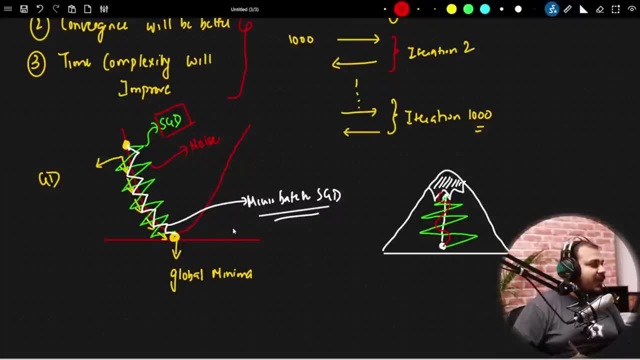 okay. so i hope everybody is able to understand. okay, and you have understood that over here, mini batch sgd gives us less noise, but there is definitely noise. now, one very important thing: still there is noise. how do we remove the noise? how do we remove the noise? this is the next question: how, how do we go ahead and remove the? 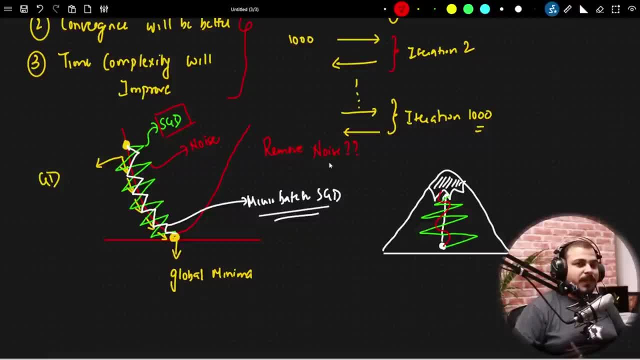 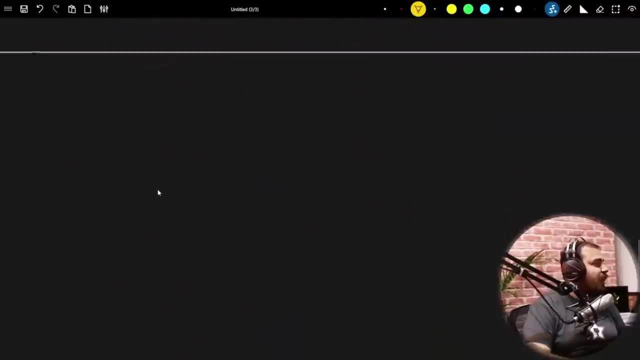 noise. now, in order to remove the noise, we use a concept which is called as momentum. we'll discuss about this momentum in completely depth. so, because of this, we have our next optimizer, which is called as, which is called as sgd with momentum. obviously, this sgd, we are talking about mini bash sgd, okay, mini batch sgd with momentum. 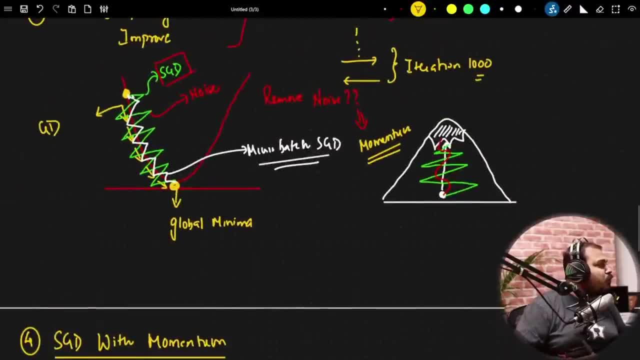 now, what this momentum will do is that it will smoothen this journey. it will smoothen this journey. it will make it smoother. it will make it smoother and reduce the noise and try to come to the global minima. okay, it will just smoother. how it will smoothen, i'll just talk about it. there is a separate maths. 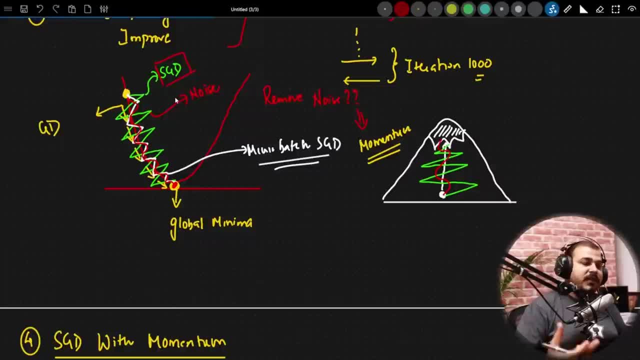 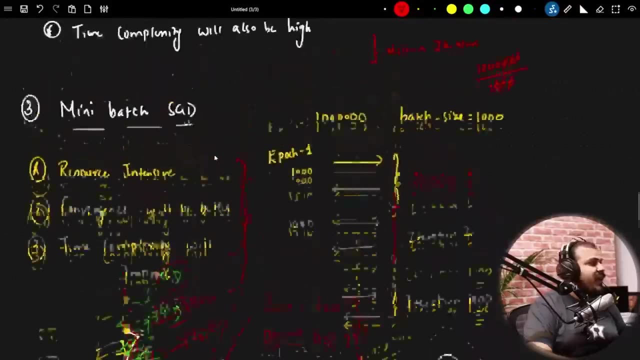 for that which is called as moving average, and with the help of this exponential moving average, we will be able to smoothen this journey and it will be able to reach the global minima efficiently. so quickly. let's understand. i hope everybody is able to understand. if you are able to understand. 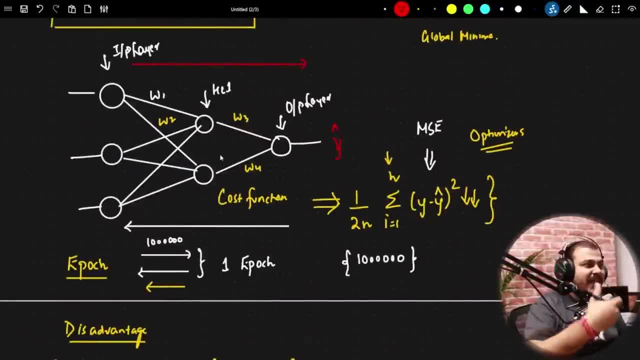 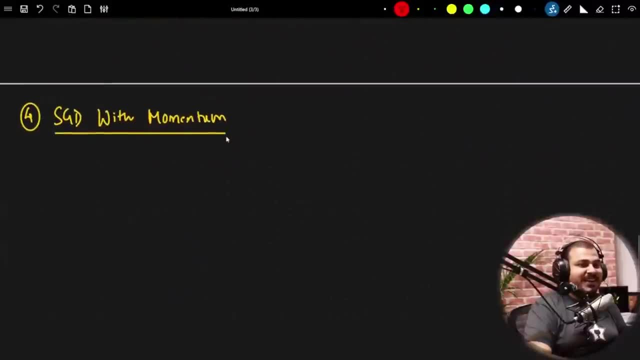 please give a like, say some symbol, say thumbs up, so that i'll be able to get an energy that you are able to understand with respect to whatever i'm teaching, and i hope my handwriting is perfectly fine and i hope i write a book one day, because i love writing these things, you know, and i'm, i'm. 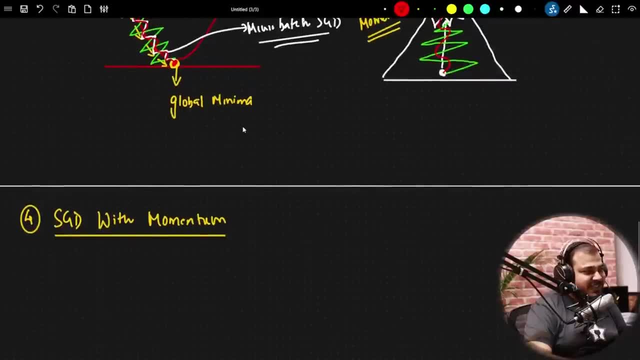 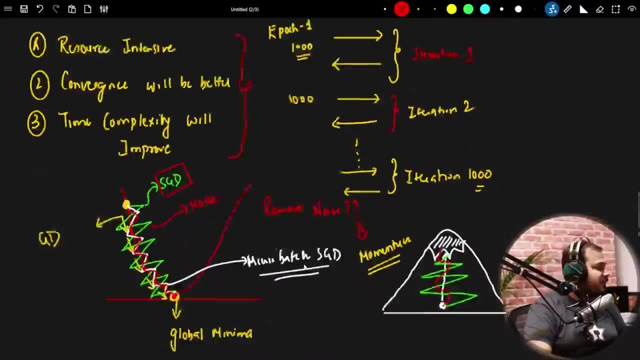 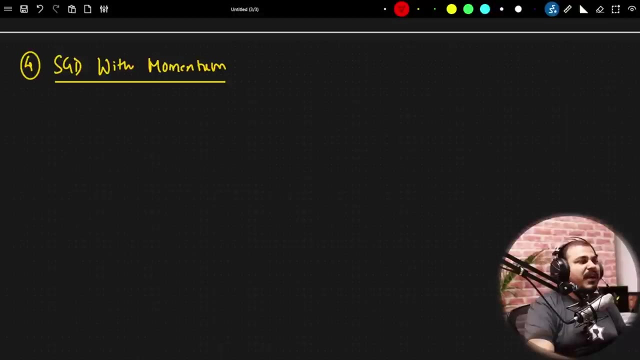 having fun writing this, so i don't create any ppts. so just let me know whether you are able to enjoy the video. you are able to understand things or not. right, just let me know. okay, perfect now. with respect to sgd, with momentum, how do we make sure that we are able to smoothen? 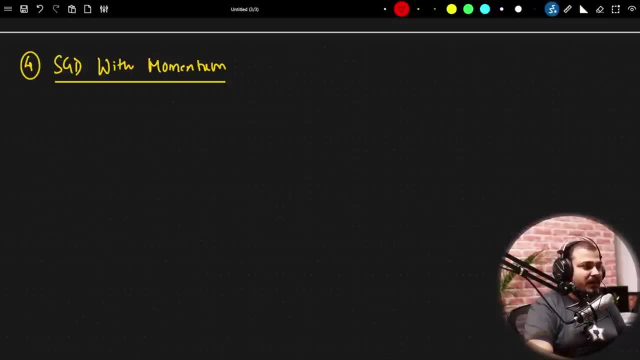 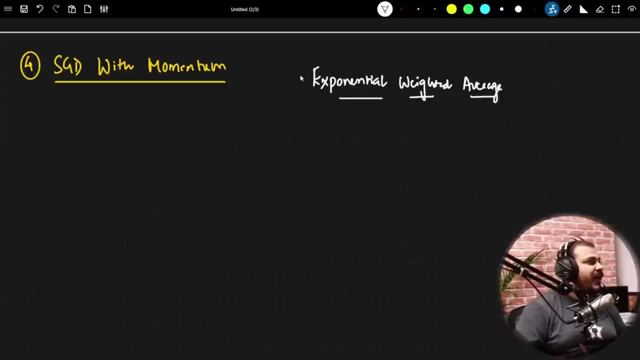 focusing on this exponential weighted average. so what is this concept? and this concept is also used in time series. some of the models, like arima model, arma model. we specifically use these things. i hope everybody have heard about this. uh, arima model, arma model and all okay. 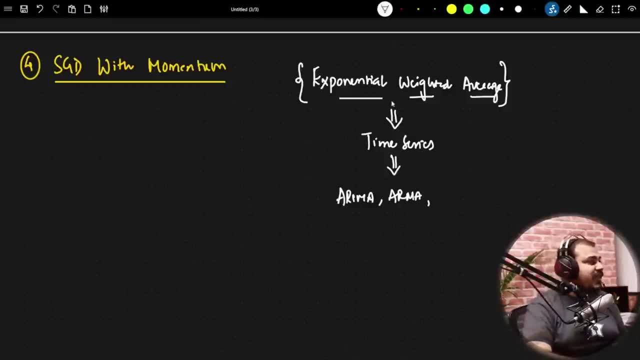 so let's understand what exactly is this exponential moving average? i hope everybody knows the weight updation formula, so weight updation i'll again write over here w new is equal to w old minus learning. rate of derivative of loss with respect to derivative of the blue world. 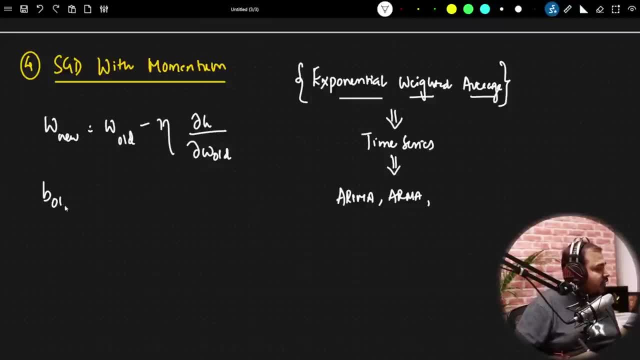 and similarly, bias bias old is equal sorry, bias new is equal to value of weight. Н is equal to w old minus learning rate of loss with respect to derivative of w old. and similarly, bias bias old is equal to sorry. bias new is equal to bias old minus learning rate of derivative of loss with respect to derivative of. 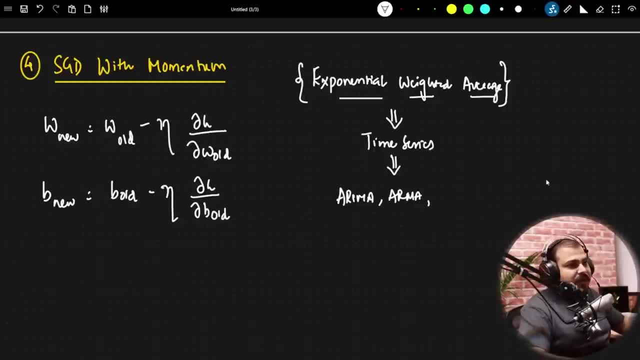 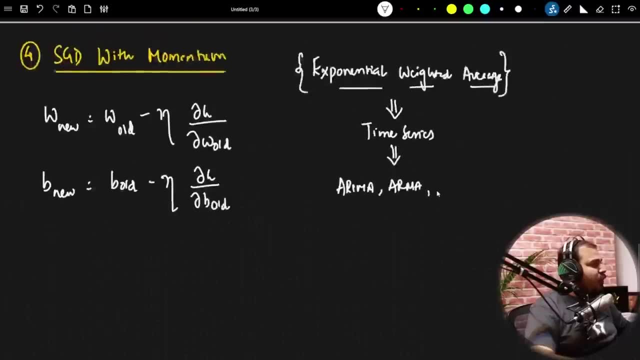 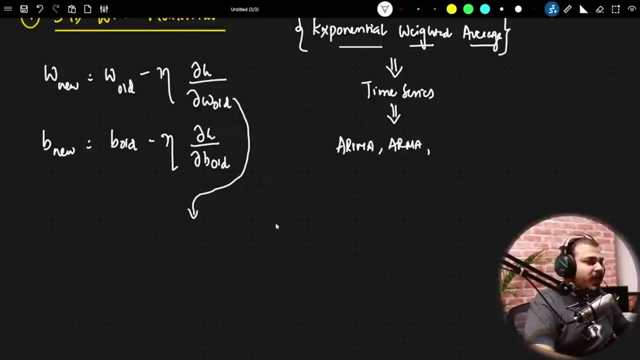 bias, old right, this two formula. everybody knows it, since i have written many number of times okay, and it should be very much clear to you. now let me do one thing, let me change this equation little bit, okay, and let it me. let me write it in a new format, okay, and probably this format will. 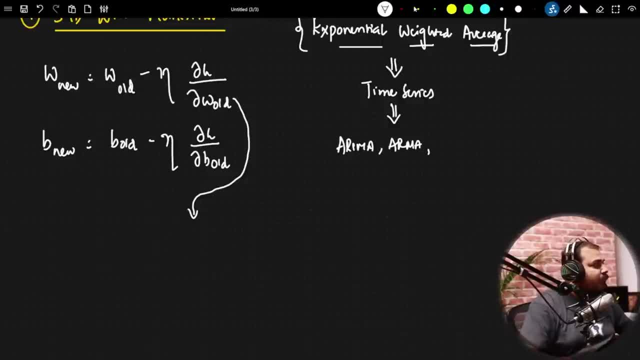 make sense, since we are doing exponential weighted average. so over here i'm basically going to write wt plus one, or let me write wt is equal to. instead of writing new, i'll write wt. and here i'll write wt minus one, minus learning. rate of derivative of loss with respect to. 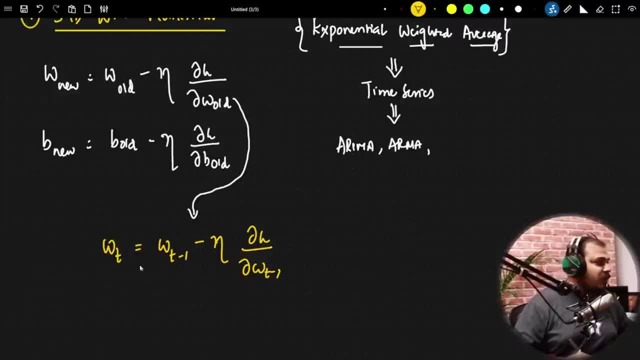 derivative of wt minus one. so this is also the same thing, because t basically means current time, t minus one basically means new, previous time. right, similarly over here, w new basically means the current weight, updated weights and w old is the older weight. okay, so i will just try to change this in this particular way. the reason why i'm doing this, i'll 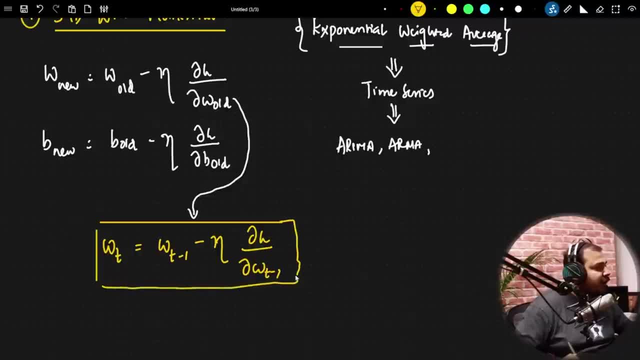 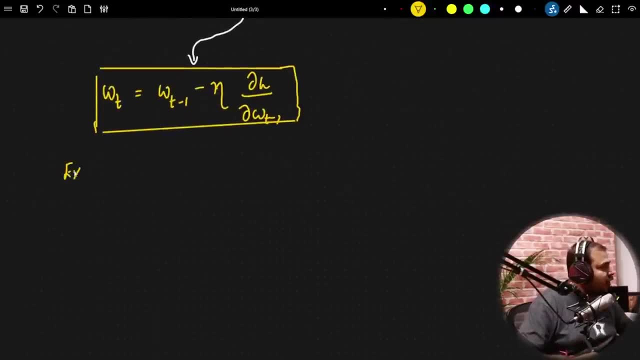 just let you know, because we really need to understand. what is this exponential weighted average? okay, now let's go ahead and understand about the exponential weighted average. now, in order to understand about exponential weighted average, i'll take a very simple example. i will take a very simple example. okay, so what does this exponential weighted average say? 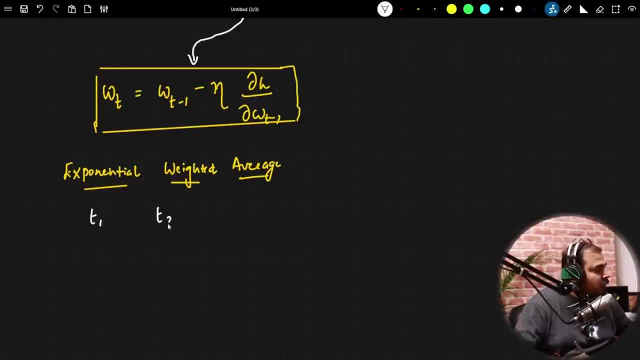 that. let's say, i have data set for time t1, t2, i have some values. let's say, i have some values. okay, for time t1, t2, t4, like this, till tn. okay, for time t1, the value is a1. for time t2, the value is a2. 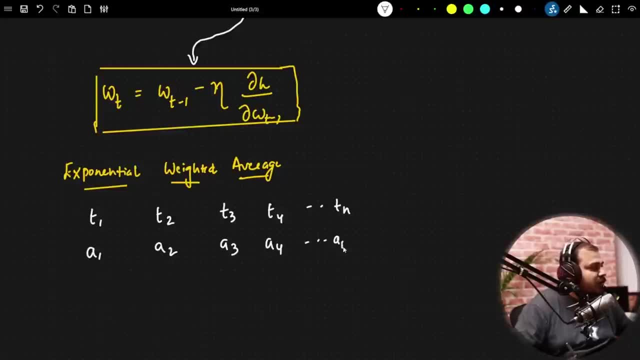 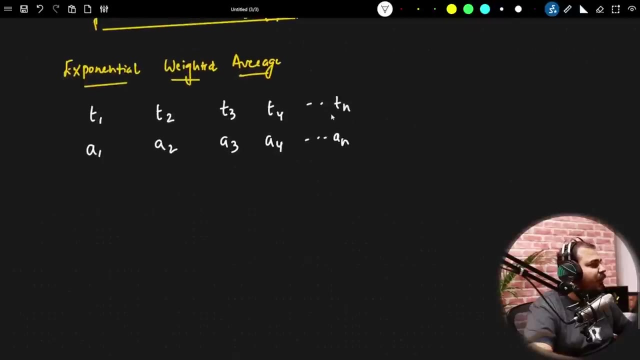 the time t3, the value is a3, this is a4 and like this, it is an. okay, so let's say: i have this all time over here, okay, and uh, well, i've just recently written the values over here and you'll be able to see it. uh, now the next step. what does this exponential weighted average say? okay, let's say: 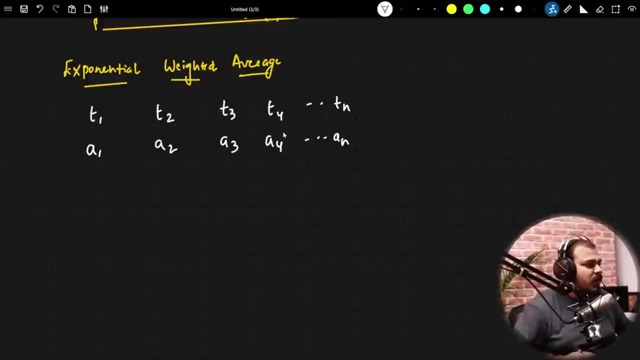 okay, and we'll try to understand. everything will make sense. okay, now here i will basically write: let's say i'm saying that the value of t1 at time t1 is basically a1. okay, and suppose, if i go ahead and try to say the value of time t2 and i have to make sure that i perform an exponential weighted, 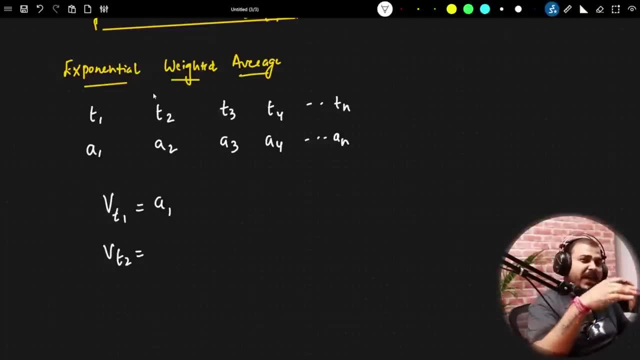 average on t1 and t2. i want to, i want to create a weighted average between this two time series data. let's see because, why? why this is very important because, with this help, i can also do forecasting. okay, forecasting now, in order to do the forecasting, i should also be dependent on the previous. 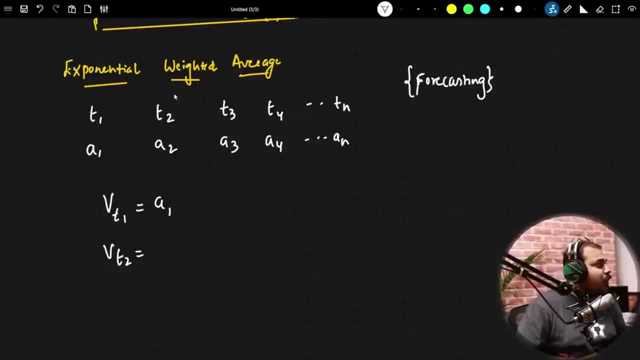 timestamp values like a1. okay, now, if i really want to apply the exponential weighted average, i will be considering this too and i will assign a weight. now, how i can assign a weight here, i'll be saying beta will, which will be my weight. weight values i will say multiplied by vt1 plus. 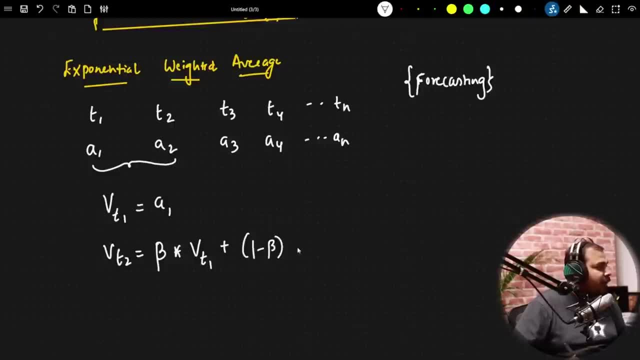 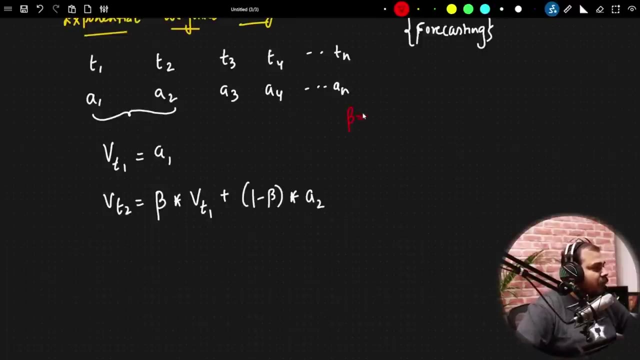 1 minus beta, multiplied by what is the value in a2? it is basic, sorry. what is the value in t2? it will basically be a2. now here what we are doing. i'll just make you understand. let's say, my beta. beta value is basically a hyper parameter. this is a hyper parameter which will actually help. 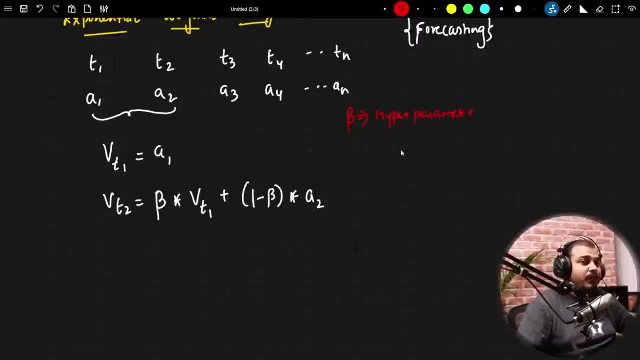 us to perform um, this weighted moving average, or weighted exponential moving average. this beta tells us on which value we should focus more. okay, on which value we should focus more, whether we should give importance to the current timestamp value or whether we should give the importance to the previous timestamp value. suppose, if i say, my beta value is ranging between 0 to 1. 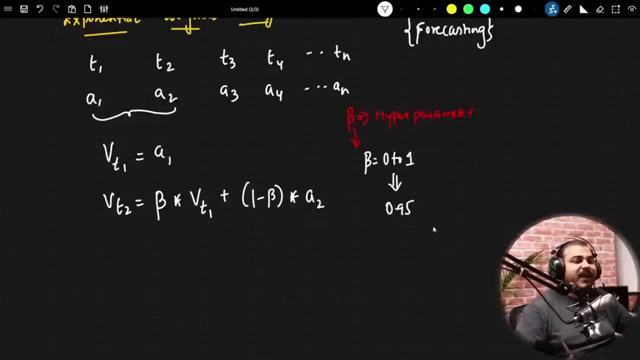 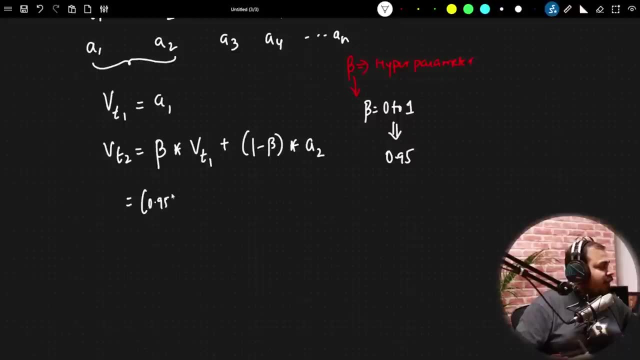 it usually ranges between 0 to 1. let's say, for the current instance, my beta value is 0.95. then what i will do? i will basically write 0.95 multiplied by vt1, plus 0.05 multiplied by a2. now, in this particular case, since i have assigned 0.95 as my beta value, 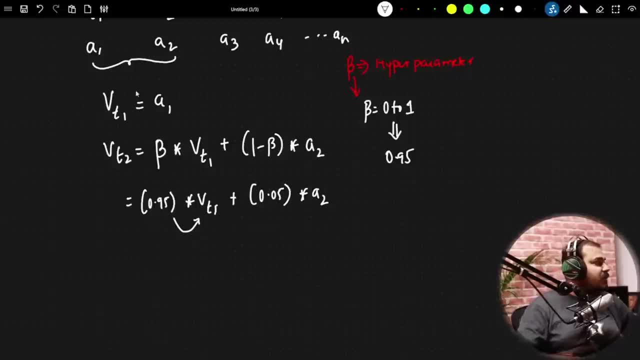 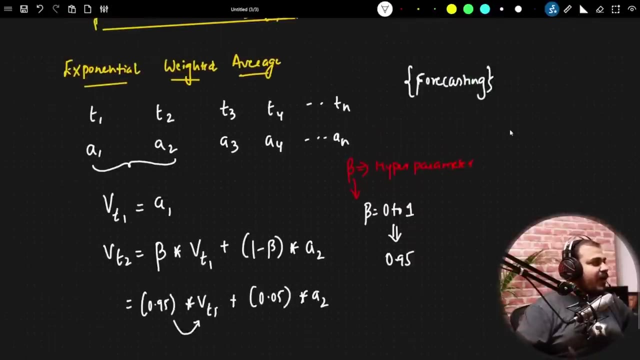 i am giving more importance to my vt1 value, that is my previous timestamp value, because if i replace vt1 i am going to get a1, and to the current timestamp value i am giving less importance. so let's say, if i plot this, if i plot this right, a1 and a2. okay, a1 is here, a2 is here. 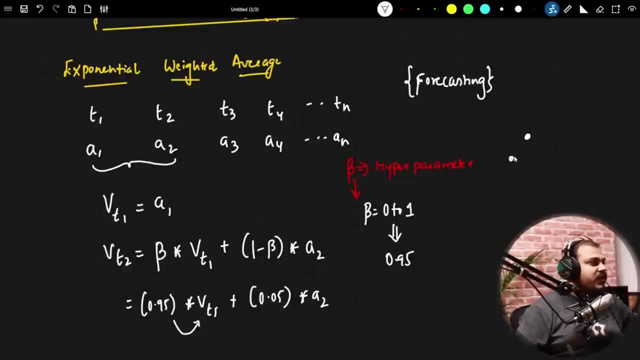 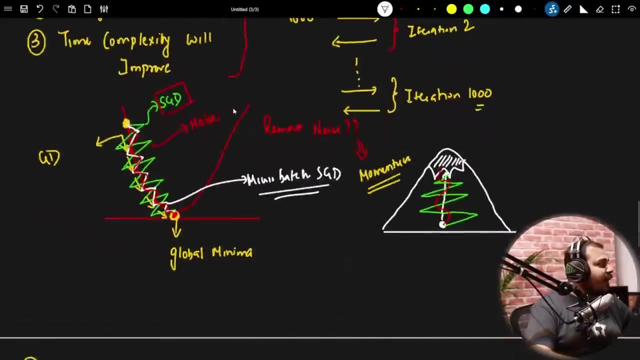 let's say now, if i smoothen this, if i smoothen this right, my smoothening will happen, my, my, my smoothing will basically happen and more control will be given to the previous point instead of the current point. okay, and that is how this smoothing process will go ahead, right? 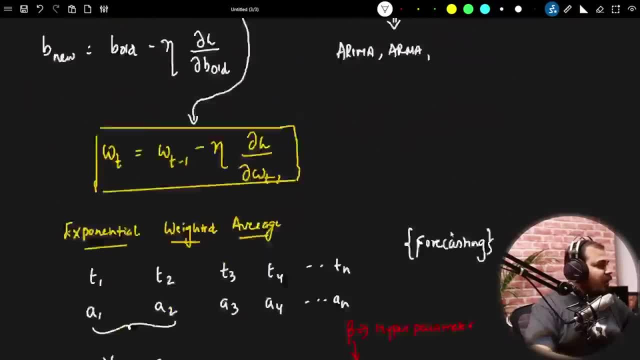 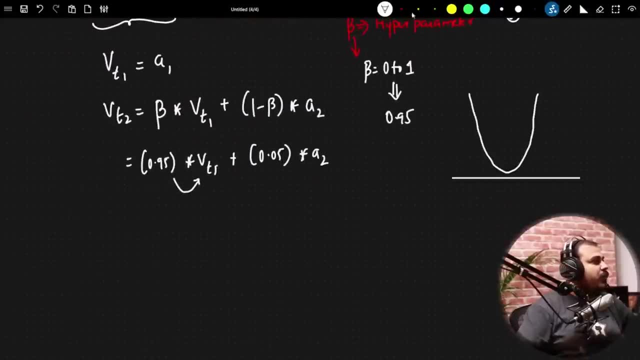 because we want to smoothen it. we want to smoothen it. so here, if i draw a new diagram for you what we are trying to do, suppose this is my gradient descent. okay, so initially let's say my point was here. okay, my point was here. the a1, the t1 point was here. 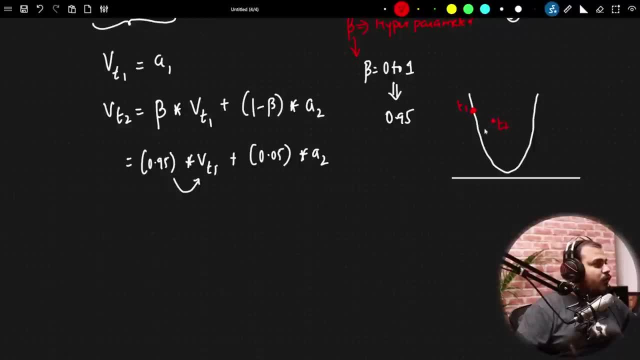 the t2 point. let's say it is here, t2 point is over here. now, if i assign beta onto this, instead of going in this direction, it will now go in something in this direction: okay, like this, and then we will get control, then t4 will get control, like this, and then finally it will. 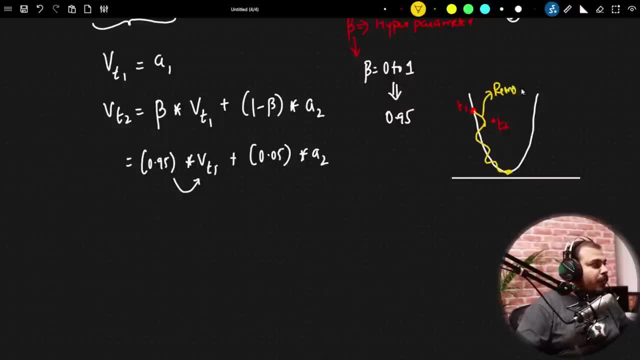 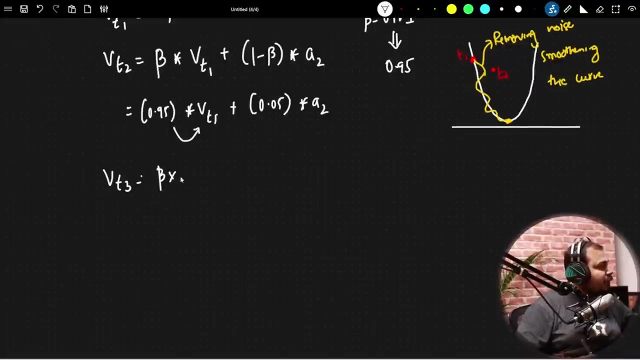 release the global minimum. so here we are removing the noise, removing the noise and is smoothening the curve. we are smoothening the curve, right, we are smoothing. so i said, beta is basically a hyper parameter. okay, now, similarly, if i say what is vt3, then if i write vt3, then this will basically become: 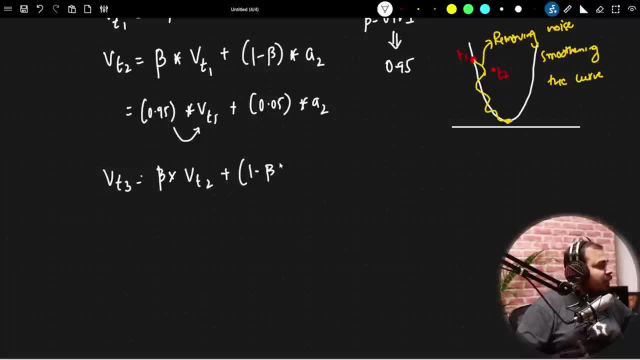 beta multiplied by vt3. right, so this is vt2 plus one minus beta multiplied by a3, because vt3- the value at time 3- is a3, and this vt2 will get replaced by this entire value, right? so, like this, for every timestamp we can assign a hyper parameter with beta so that this smoothing process will actually happen. okay, 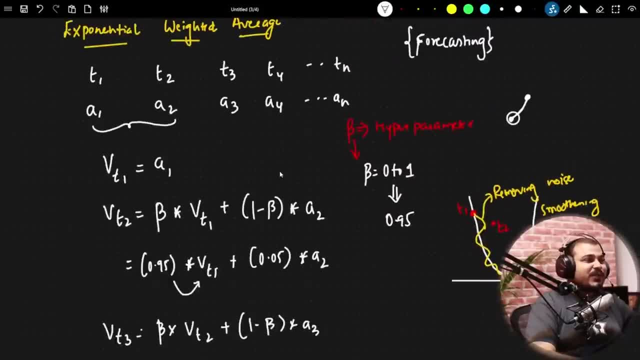 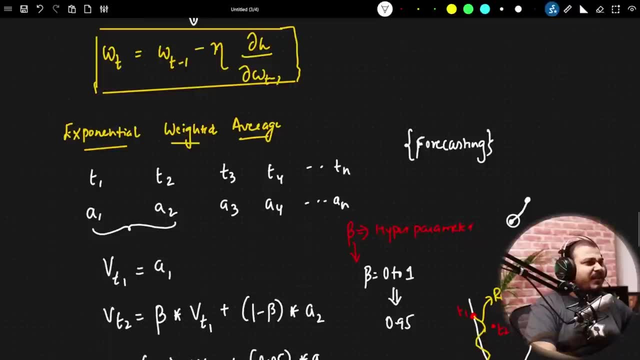 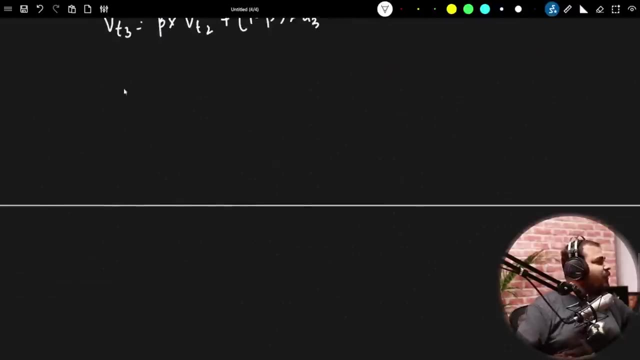 so where do i apply this? where do i apply this? now the question rises: where do i apply this weighted exponential weighted average? right, and it's very simple: where do we apply it? just a random guess. we basically apply this in the derivative of laws with respect to derivative of weights. now what i will do is that i will just go ahead and write. 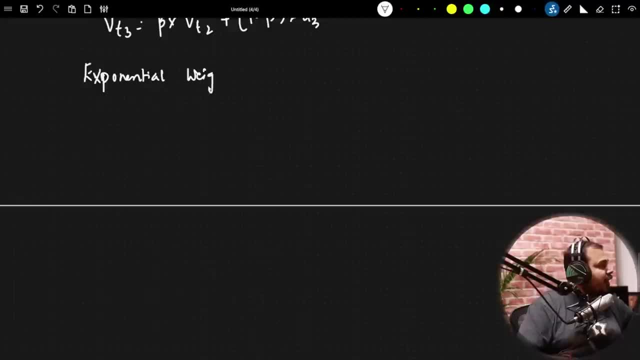 exponential weighted average is nothing. but here i'm just going to take this and now i'll write a equation. new equation: wt minus 1 minus learning rate. instead of writing derivative of loss with respect to derivative of wt t minus 1, i will just write vdw. now what is this vdw? let me write it down. vdw basically means: 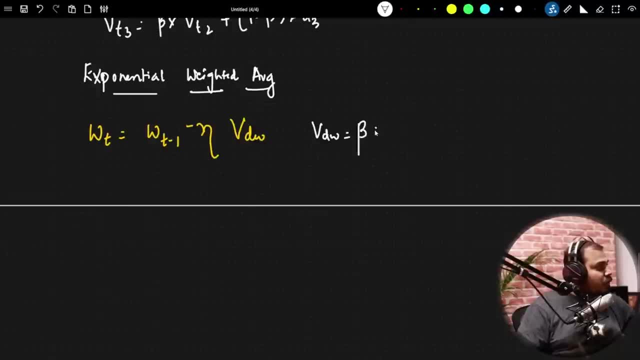 it will be. the weighted average with respect to vdw is nothing but value of the derivative. okay, beta multiplied by vdw, t minus 1 plus 1, minus beta multiplied by derivative of loss with respect to derivative of wt minus 1. that's it, and here we are bringing this exponential curve. 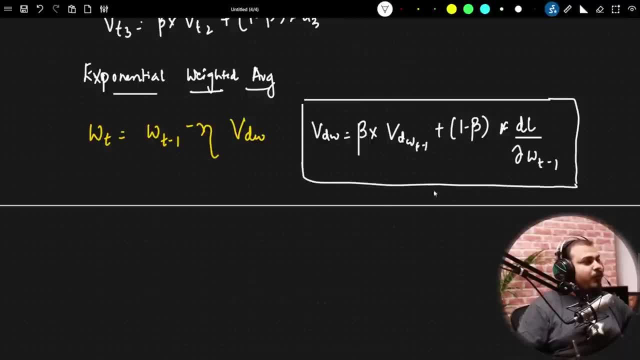 initially. now, since we bring this, we definitely know that what is going to happen over here, the smoothening of the curve, will basically happen, okay, with the help of this. vdw basically means- and this will be t right vdw- the value of the derivative of time t is nothing but beta. 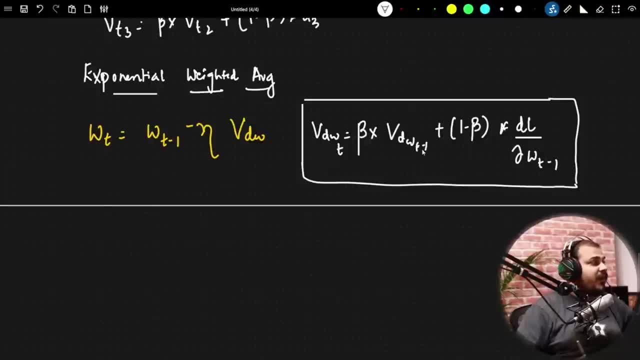 multiplied by vdw t minus 1 minus beta. multiplied by vdw t minus 1 minus beta. multiplied by vdw, the previous value of derivative by time: t minus 1 plus 1 minus beta. multiplied by derivative of loss with respect to derivative of wt minus 1. okay, so i hope you are getting an idea how we are. 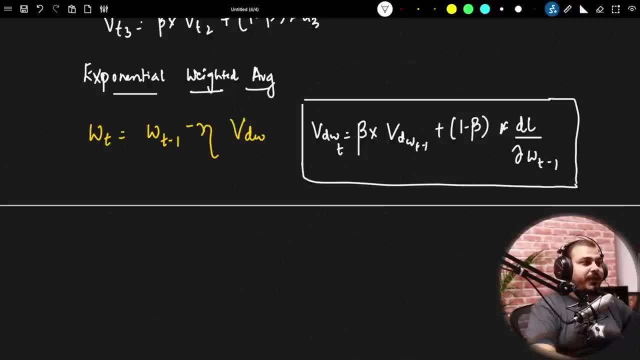 able to smoothen the curve in an efficient way. okay, and this is basically my exponential moving average. okay, and now, if i probably draw my curve, what all problems we are solving? suppose, if this is my gradient descent, i will basically start from here and i will be getting a smooth inversion to reach the global minima. and here 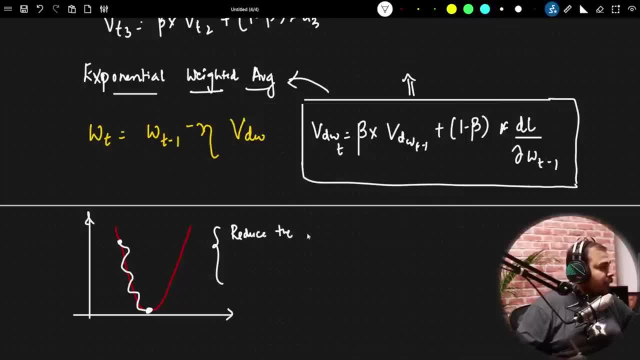 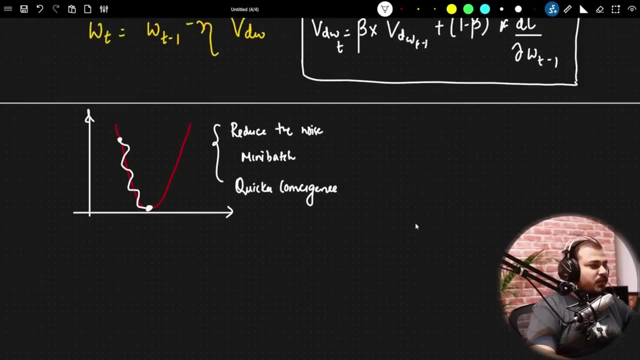 what all problems we are fixing. we are reducing the noise. we are reducing the noise. uh, this will also be working for mini batch and it will also be having a quicker convergence. so nice stories, right, guys? this is all say. the best way to learn something is just like. 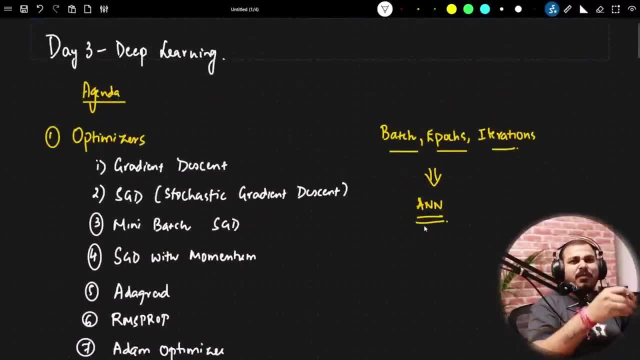 remember the story, how things goes: there are some problem. because of that problem, something else will come and this will keep on coming. today, if you really wanted to do a phd, find the loopholes in the previous things that are there, create a new one in front of you and that is done, okay. 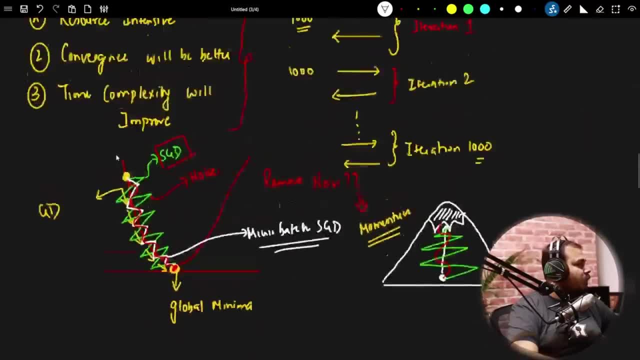 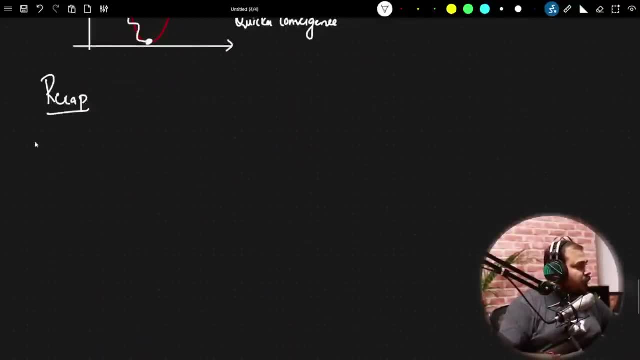 so just a quick recap. just a quick recap everyone, okay- what all things we are doing. so i hope you guys have a good day, have learnt. First thing, we learnt about something called as gradient descent. What did we do in gradient descent? You understood the problem. We cannot send millions of record. 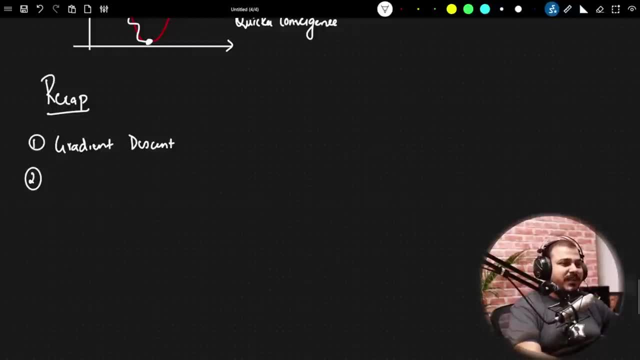 So I have to definitely go with gradient. I cannot go with gradient descent itself. So there is some problems, Obviously, millions of record, resource intensive, everything you know In interview also, they may ask you this, They may say you that, if there is so 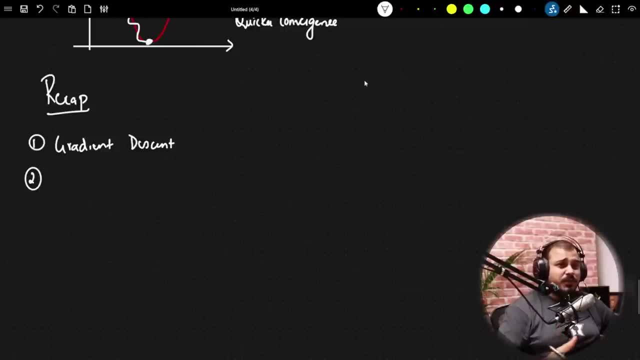 much of noise in probably my gradient descent. what do you think I should do, You say? I will just say that try to bring that smoothening factor in your optimizer. That's it Right, So easily. They will not ask you the equations, The reason I am telling you the equations. 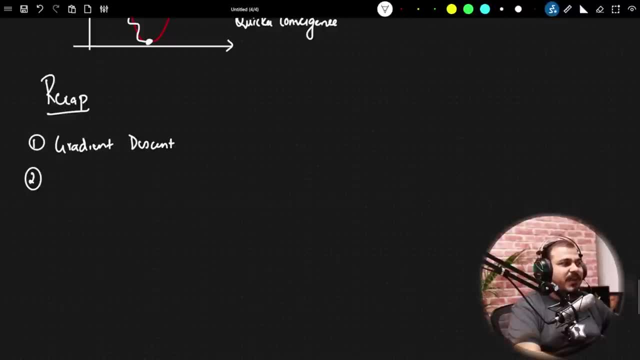 because you should be able to understand, Because, at the end of the day, if I am teaching, everybody should be able to understand. That is my main aim. Okay, Then, after gradient descent, what did we learn? We learnt about stochastic gradient descent. 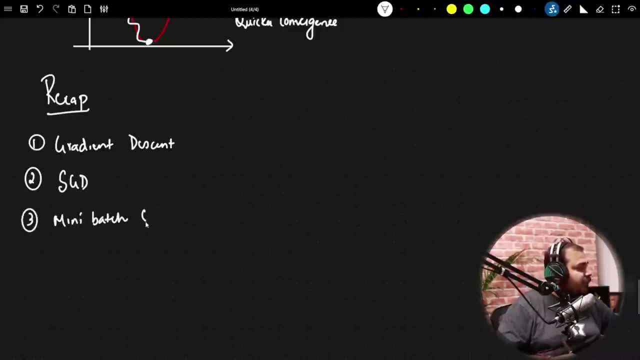 Then the third one is something called as mini batch SGD, Right, The fourth one that we actually focused on: Okay, This is basically SGD with momentum. Okay, Now, the fourth one that we are basically going to discuss is something called as Adagrad. Okay, So here I am specifically going to write Adagrad. Now in Adagrad, this: 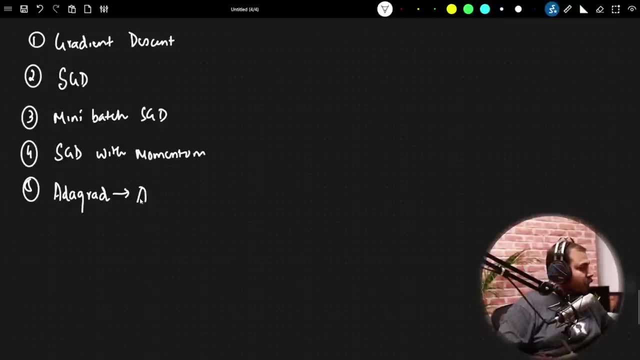 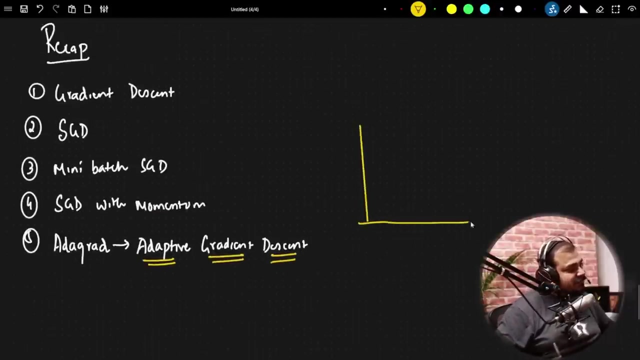 is basically Adagrad. Okay, Okay, Okay, This is the adaptive gradient descent. Okay, Now, what is this adaptive gradient descent? Let's discuss about this. Okay, And to discuss about this, let me again draw the gradient descent curve. Okay, So till now, whatever weight updation formula we have seen, right? 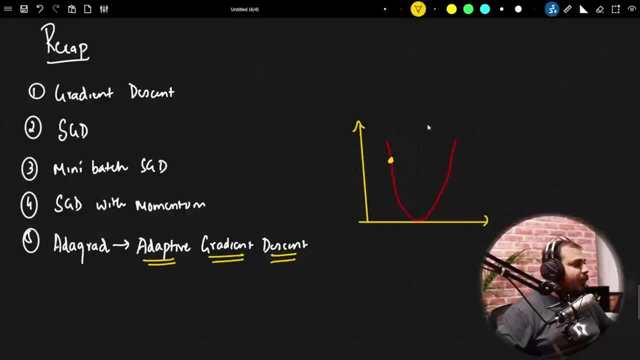 What is the thing over there? there, in the weight updation, there is one important parameter which is called as learning rate. now, this learning rate, you know, helps us to converge, or it helps us to maintain the speed of the convergence. right, but understand one thing okay: when we move, 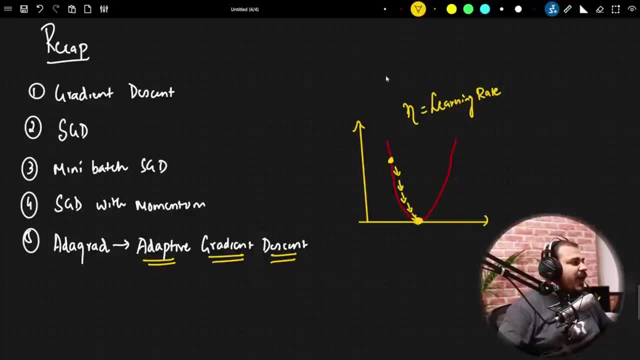 towards the global minima. don't you think? and this is right now fixed, right fixed in every algorithm, in every optimizers, this is right now fixed. can we change the learning rate in such a way that, let's say, my data point is somewhere here? initially, my learning rate should be high and as we go towards 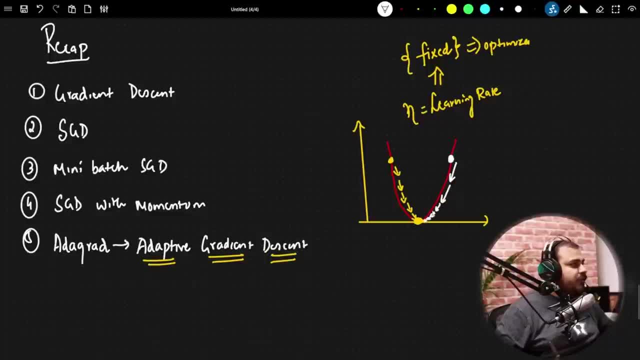 the global minima, though learning rate should decrease. so can we do this? because researchers will not keep quiet. they have to do the PhD right, so they will come up with something else right, and we have to learn those things. and again, I salute all the researchers. it is not a joke. they have created all these amazing things. you just go and see. 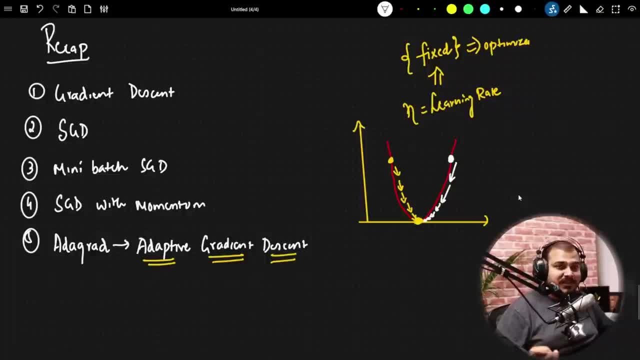 the research paper that they have written. you know, sometime you'll not even understand the equations. that's smart, they are okay. so over here, I have to make sure this, this adaptive- adaptive is the word right. my learning rate is fixed, but I want to make sure that I also change my learning rate value and 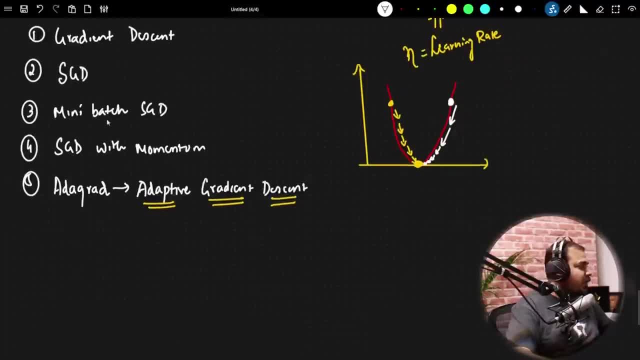 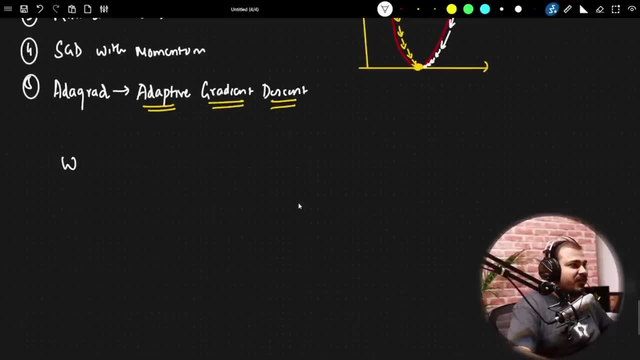 taste the on this right equation that way, because I am actually trying to make during a strategy. now, how can I do that? that is what we are going to discuss now. right now, you gradient descent? okay, in adaptive gradient descent, we replace this learning rate with something else. okay, if I really want to make right now the 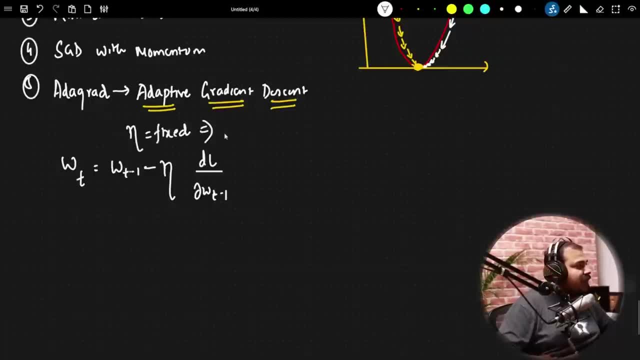 previous state is that this learning rate is fixed. I want to make this instead of fix. I want to make this adaptive adaptive. I have to make this changes as we approach the global minima. so what I will do is that I will replace this entire value with something else. now, what will I replace it with? I will 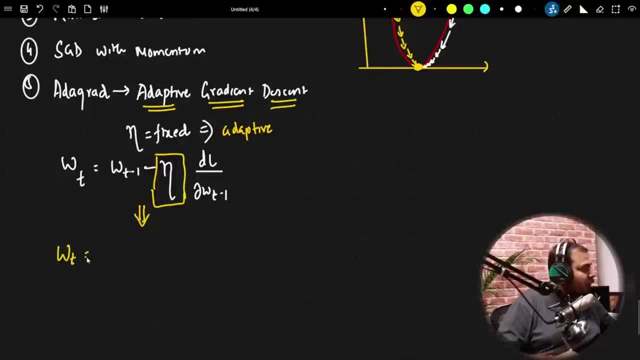 replace it with completely like this: see W of T, W. root of T minus 1. instead of lighting running rate, I will write eta. this is a kind of symbol which is called as eta. instead of this, I'm going to write this and remaining all will be. 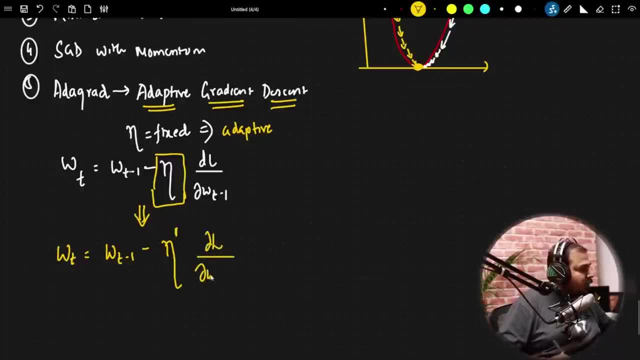 same remaining, all will be same. derivative of loss with respect to derivative of W T minus 1. okay now, let me just encircle this quickly. okay now, what is this? what is this value? this value, this value is basically- I'll write it as: n of eta is equal to learning rate divided by- and here I'm. 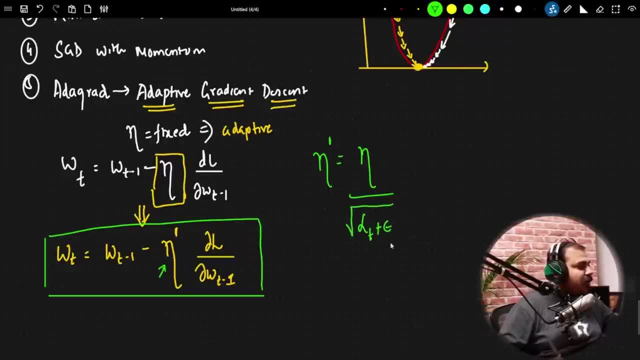 going to write a formula which is called as alpha T plus epsilon. okay, now I'll explain each and every parameter that is basically getting used. okay, each and every parameter that is basically getting used. we'll try to understand. okay now the first thing: why this epsilon is there. epsilon is actually there and this: 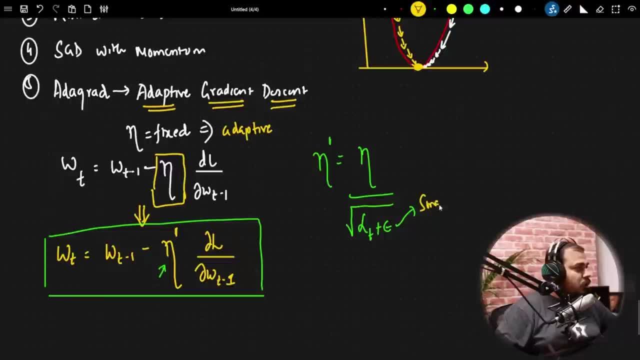 will basically be a small number, because, to avoid divide by zero condition, if alpha of T is 0, then this divided by this 0 is basically infinity. so in order to avoid this, we are actually adding this small number which is called as epsilon, so that this do not numerator- sorry denominator- never becomes 0, okay, 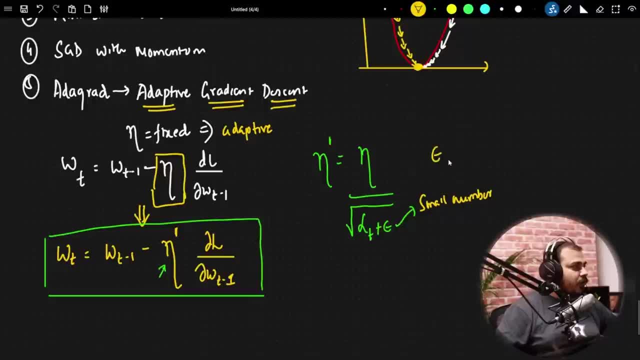 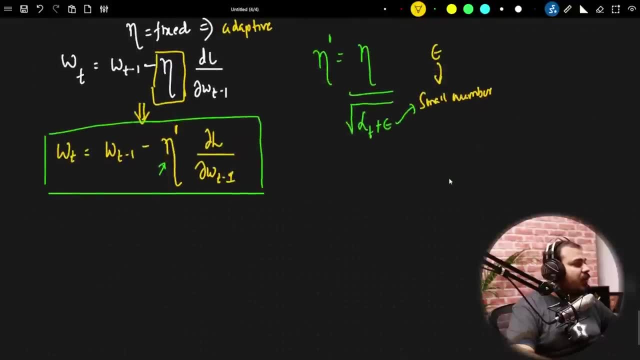 this is the first step, so I hope everybody understood about epsilon okay. so this is a small number. now the next thing is that: what is this alpha of T? now here, what I will be doing is that alpha of T. I will write a new equation. I'll say: summation of I is equal to 1 to T. T basically means current time stamp. 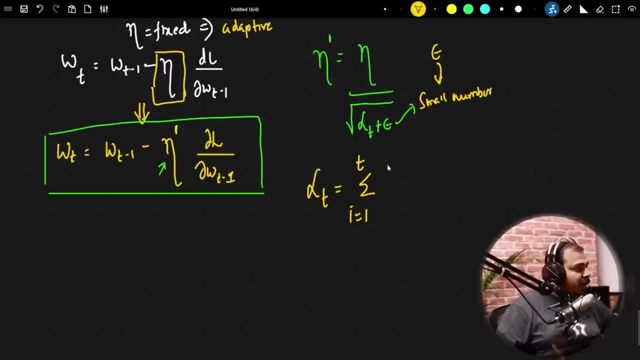 okay, current time stamp of that specific weight, and this will be divided: derivative of loss with respect to derivative of W T, whole square. okay, with respect to this time stamp, I'm doing the summation of all the previous weights also, and I'm also doing squaring. okay, now, when we bring this equation, what will happen? okay, my main. 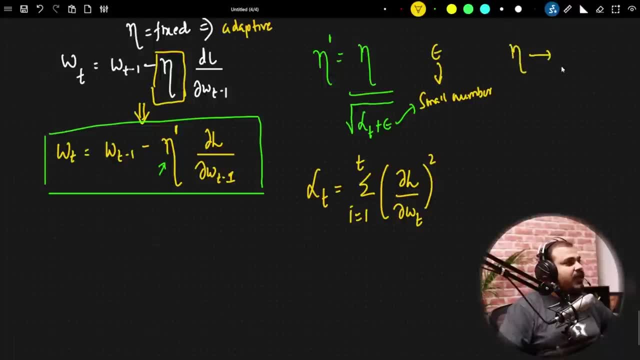 aim is that my learning rate, after it has started to train, you know we should keep on decreasing it as we reach the global minimum. right, we need to decrease it, right, we need to decrease it. now. focus on the numerator that is alpha of T. don't you think this alpha of T? whatever formula I have used? 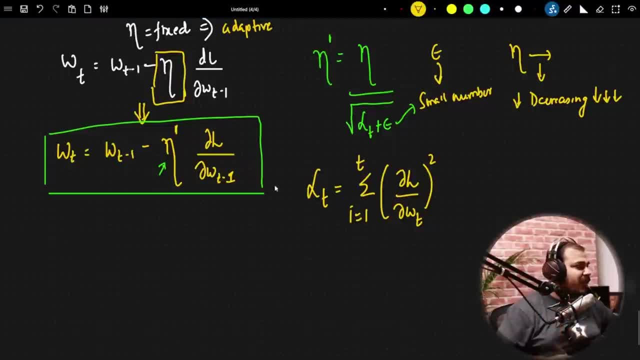 you know, as we go with respect to different different T value, right, with different different time stamp value, don't you feel? let's say, in T is equal to 1. if my learning rate is 0.01, at T is equal to 2, this may also get reduced. 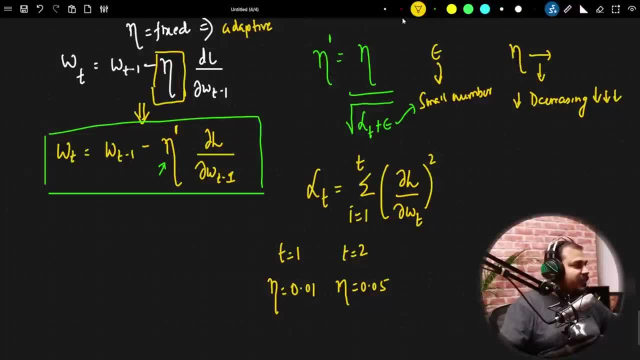 why it will get reduced. I'll talk about it. let's, let's. let's write it down. okay, I'm writing it down over here. and similarly, at T is equal to 3, this will get reduced to 0.002. let's say: okay, let's, let's. let's say: 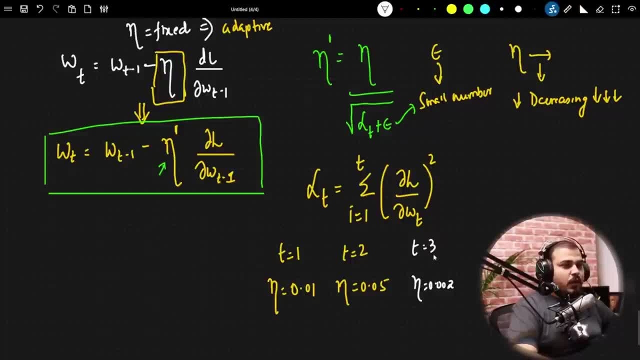 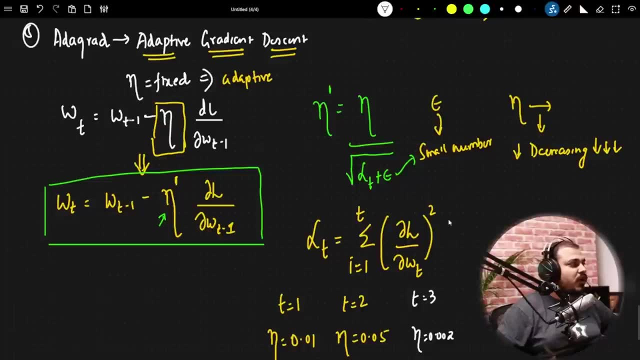 I'll prove it why this value will go down. over here you will be able to see that this derivative of loss with respect to derivative WT, as the time stamp goes on, this value will keep on increasing because we are doing the summation right, we are doing the summation and this value is getting. 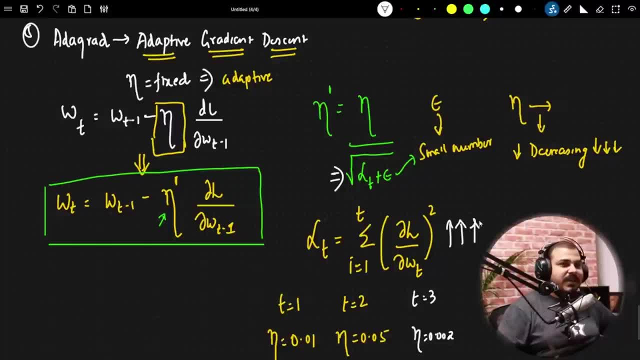 divided over here, right, since the value is increasing at every time, stamp this value we are going to insert over here and obviously, because of this, this entire equation, don't you think it will increase because we are dividing this with this? I hope everybody is agreeing with this, right. so whenever we divide this value, 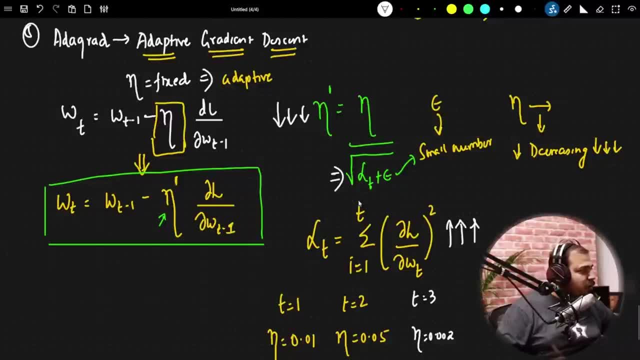 continuously, because, with respect to every time stamp, this value is going to increase, because alpha of T is nothing but the summation of I is equal to 1 to T, derivative of loss with respect to derivative of W T. okay, yeah, it should be 0.05. okay, so because of that, you will be seeing that. 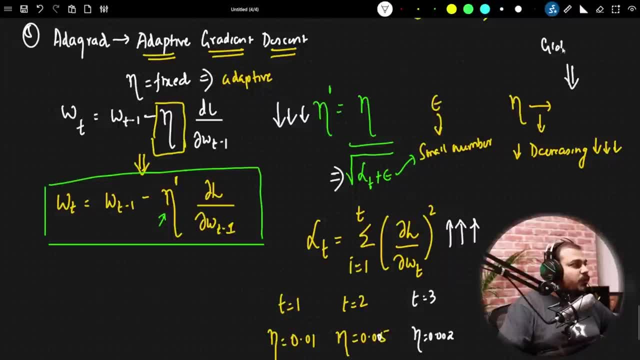 as we reach near the global minima. as we reach near the global minima, this value will keep on decreasing right and through that specific way, we are bringing adaptiveness in the learning rate, and this time the learning rate will never be fixed, since it will be decreasing. 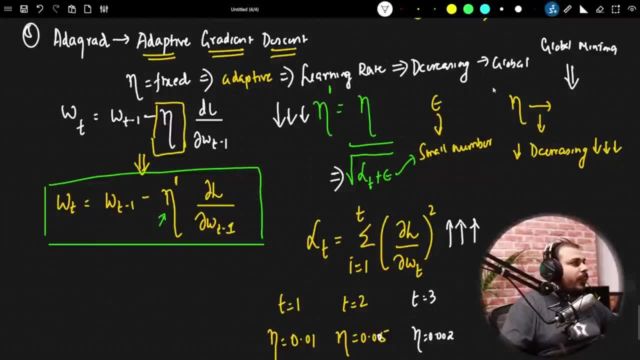 as we move towards the global minimum. okay, so this is the only change that is basically coming on the learning rate. okay, this is very super important to understand. timestamp basically means the weights at that particular timestamp, like w new, w old right. so w new basically means wt. 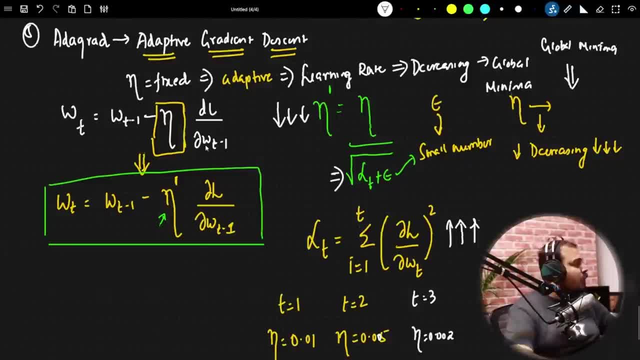 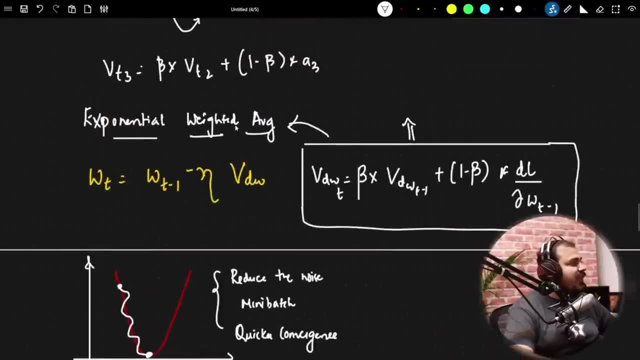 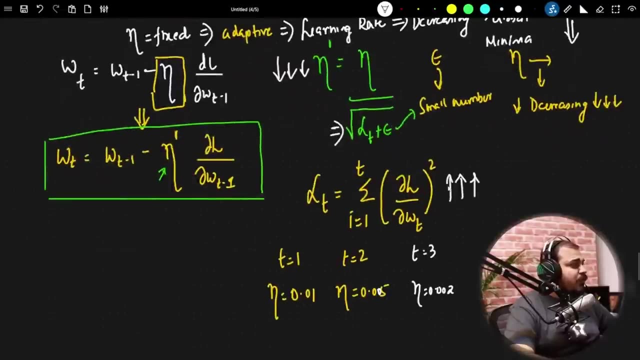 w old basically means wt minus one. now we will go to the next step. still over here, you see that we forgot to add this smoothening thing, the exponential weighted average. right, exponential weighted average is also not there. for learning rate also. you see the value. you know if this is. 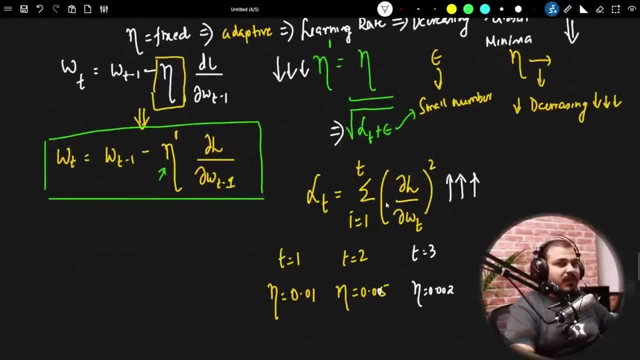 increasing by a very small amount of time, then it is increasing by a very small amount of time. a very huge number, because this will increase in a deep neural network term, will be increasing by a huge number. okay, so because of this, the learning rate change that may happen will also. 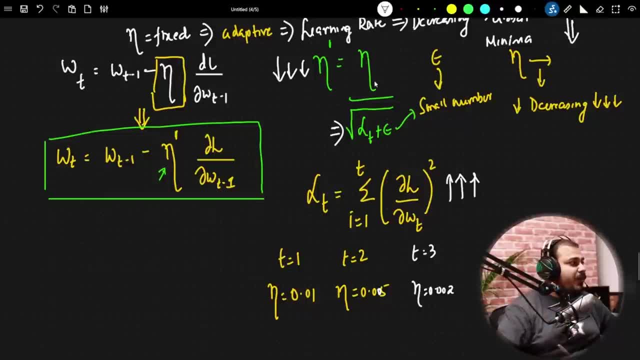 become negligible at some times. so how do we prevent that? this should not be a huge change. see, understand always something right when we are dividing by this right, there may be situation that alpha t can become a huge number, huge number also right in a deep neural network. we keep on adding things. we keep on adding derivative of loss with respect to 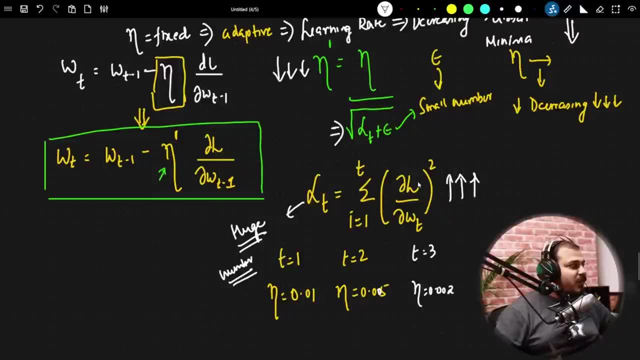 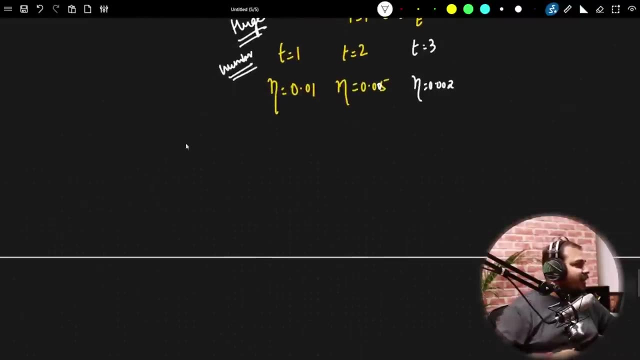 derivative of wt right with respect to timestamp. now, because of this, what happens? this n theta right? it will. there will be a negligible change, right? so in order to prevent this, we are going to go and understand the next uh optimizer, which is called as added delta. so here we are going. 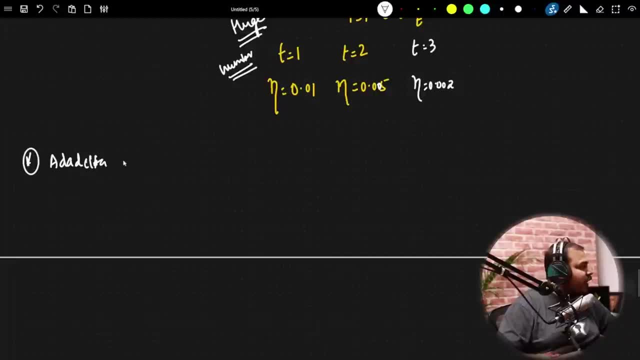 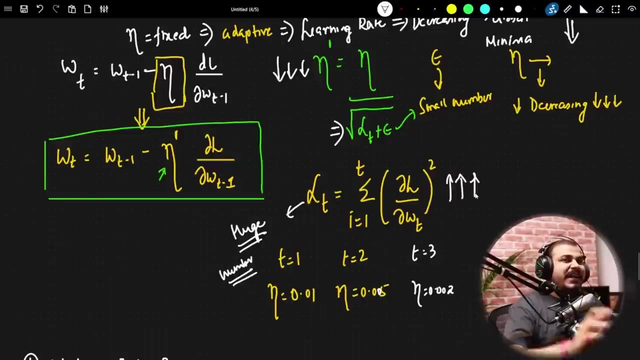 to discuss about added delta and rms prop. almost both both these optimizers has similar functionality. i hope you understood that. what is the problem over here? the problem is that if we keep on updating this, this value will keep on getting higher as iteration will happen, as more and more weights will get updated, and when i am 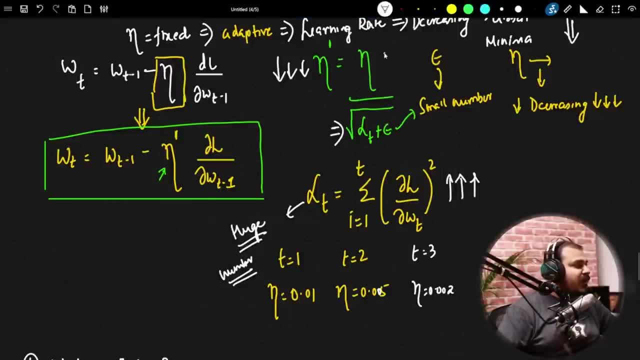 trying to place it over here and when i am dividing with this learning rate, which is already a small number. if the learning rate is 0.01, this will already be a smaller number, small number, right, and this n of n, theta of i, this when i am replacing over here, suppose, if this is a very small number. 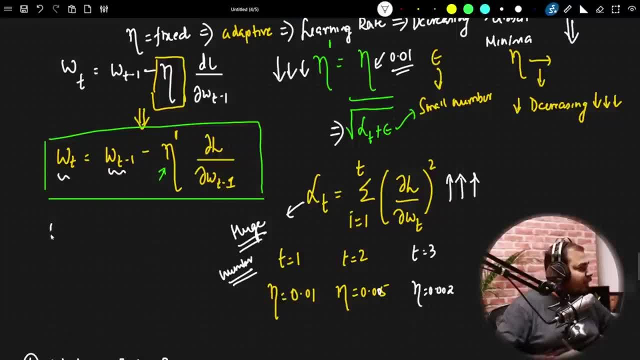 hardly. the previous weights and the current weights will change. this will approximately be equal to same wt will approximately be equal to wt minus one because of that. so we also have to make sure that this alpha of t does not reach is a very huge value. so how do we do this? how do we make sure that this alpha of t? 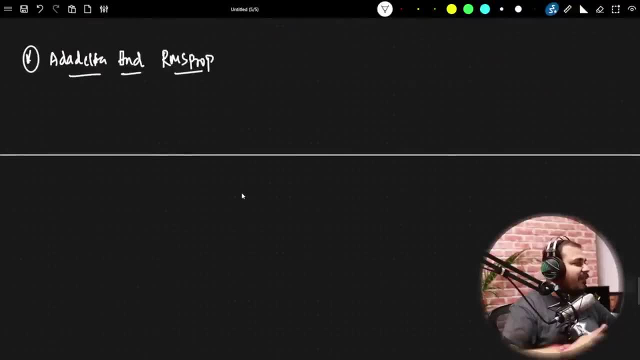 is never so big. now, in this particular case, i will again take this iti value and, instead of writing alpha of t, i will divide by another number which is called as hdw plus epsilon. i hope everybody understood what is the importance of epsilon, but let's. 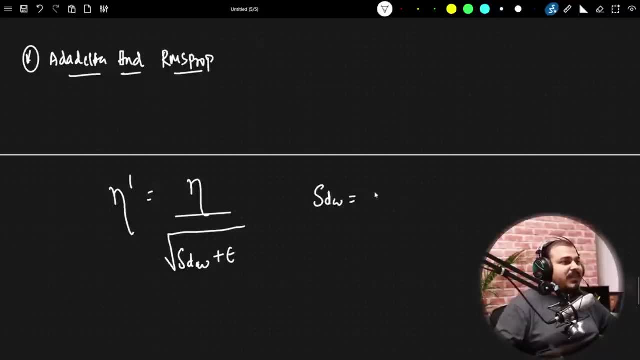 understand what hdw becomes now. hdw is nothing, but here we are going to apply exponential weighted average again so that we control this value. okay, so here we are going to basically apply exponential weighted average. how do i apply exponential weighted average? initially, let's say that we will initialize hdw as zero. okay, then, with respect to t, let's say this is t minus one. 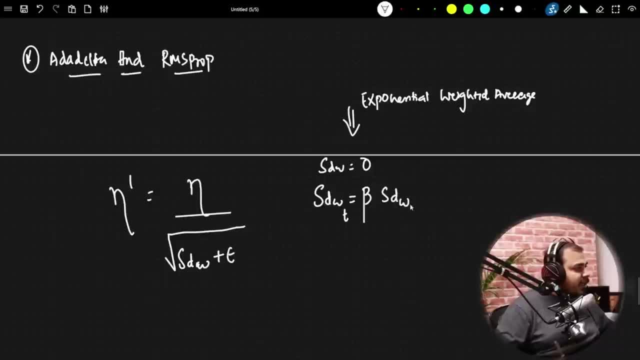 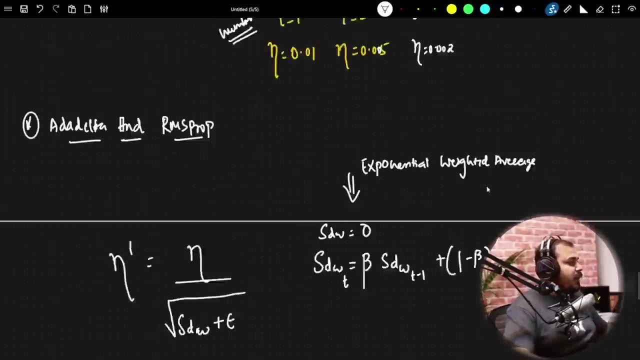 now, with respect to t, i will say that beta multiplied by hdw, t minus one plus one minus beta multiplied by derivative of loss, derivative of loss with respect to derivative of w, also square. we understood right. see what is the thing over here? we know that alpha t formula is: 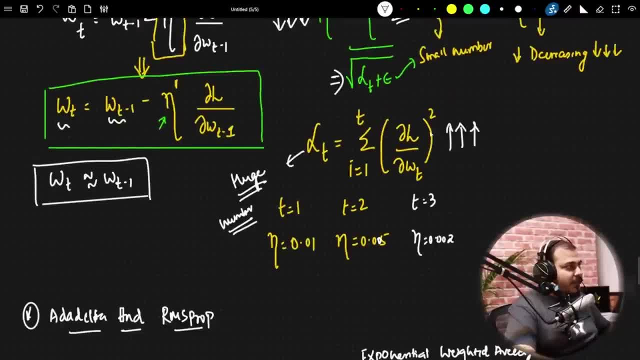 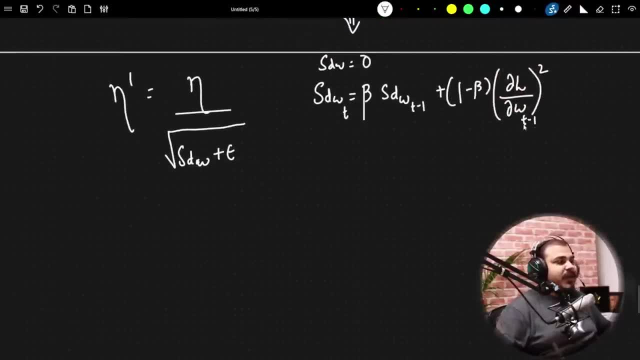 derivative of loss with respect to derivative of wt, whole square right, and we are also making sure that we keep it over here. and this will also be t minus one right we are. we are making sure that we keep it over here, but now it is controlled because of this exponential weighted average. 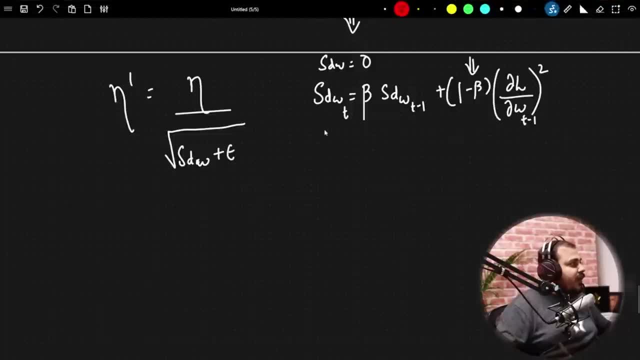 now suppose if my beta value- let's say my beta value- is 0.95, then what hdw t will happen? this will be 0.95 multiplied by hdw t minus one plus 0.05, with derivative of loss. with respect to derivative. 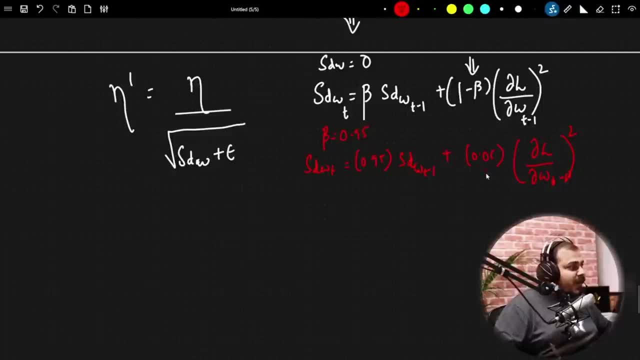 of wt minus one whole square. now we are controlling this with this parameter. now this will never increase or bump up by a very large value. it is, it will go. it is going to definitely increase by a smaller value. i hope everybody is able to understand, right? so now we are. 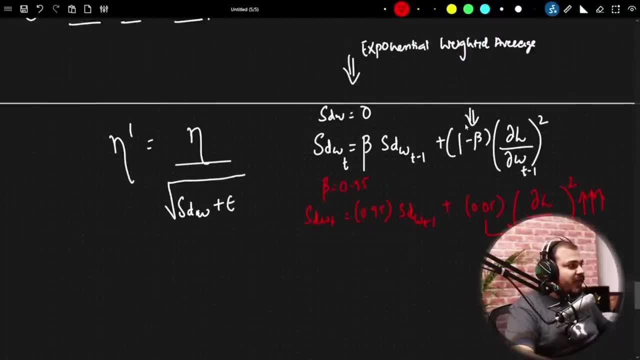 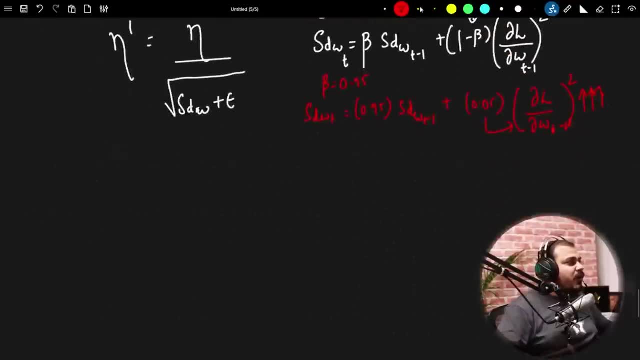 getting this idea what i am trying to say here. the problem was that we were not able to control this increase, but here we are definitely being able to control because of this beta value. right, one minus beta value, and this will be the current value. with respect to the previous value, whatever, 0 will assigned. 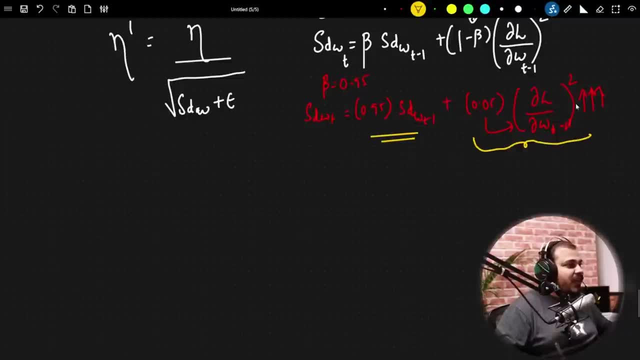 but we are making sure that this will always be in the controlled state. now, when this will be in the controlled state, obviously there will be a slow decreasing on edge h of theta in the next four hour period. opening current date: aus c of theta is up, so i will have to. 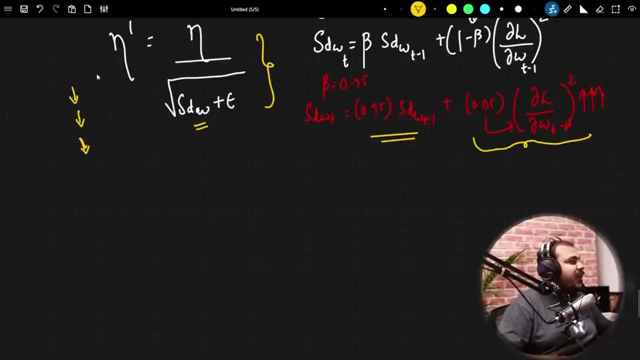 make sure that we have the current value of the previous value and we have this one whose value is 0, which means that we are able to control and improve about press. this will definitely make much easier in this column here, where i hope everybody will of this learning rate value also. 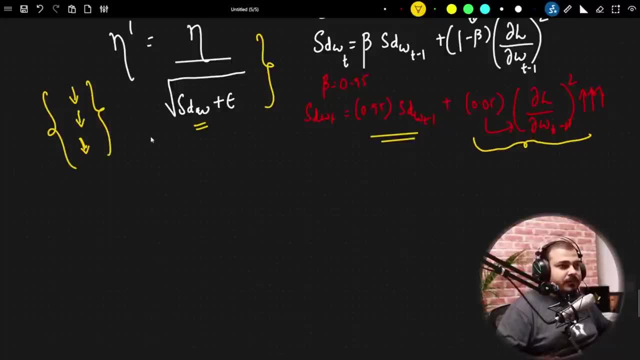 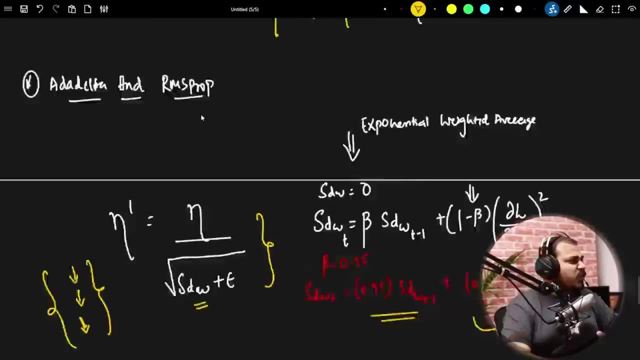 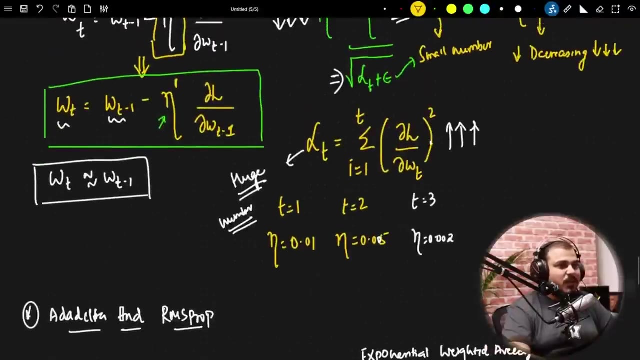 and we will be able to reach the global minimum. right? Are you understanding these things or not? guys, Just tell me. okay, It's just like a story. Now we have brought exponential weighted average into picture, right? Why? Because we really want to control this, okay, 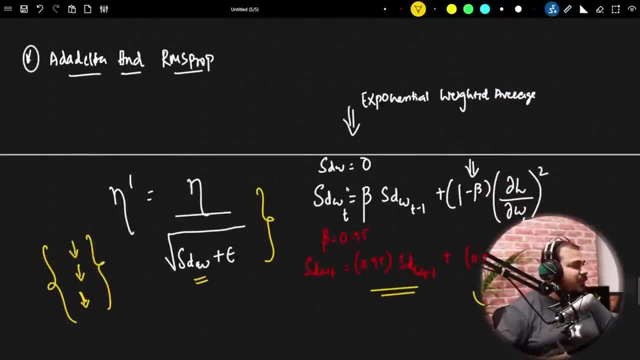 So HDW is a new term that I'm actually using. This HDW is nothing, but initially, at time t minus one, or time t, it will be zero. When we go to the next timestamp, we'll take the zero. we'll apply over here. 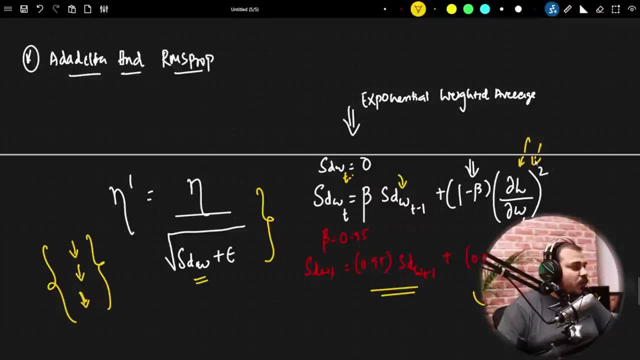 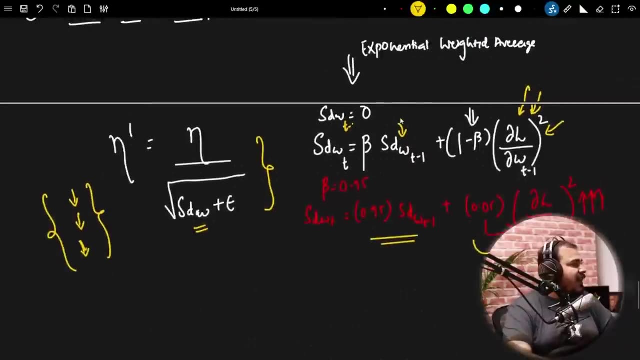 but we really need to control this value control. You have to control this value, how it increases, okay, And that is what we are doing with the help of exponential weighted average, okay, So I hope everybody's able to understand Now. finally see, everything is added. 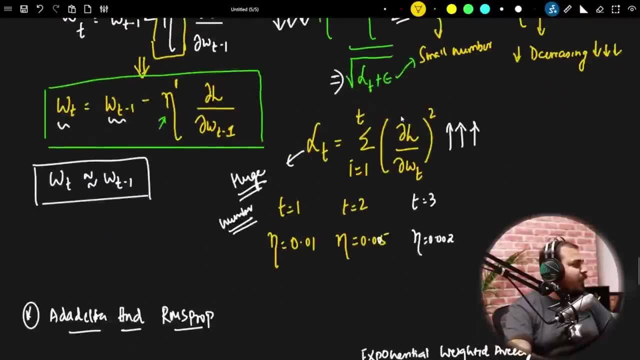 but still we again give, because here also my equation will look like this: See my weight updation formula still has this derivative of loss with respect to derivative of Wt minus one right, And whenever I have this, smoothening will not happen. 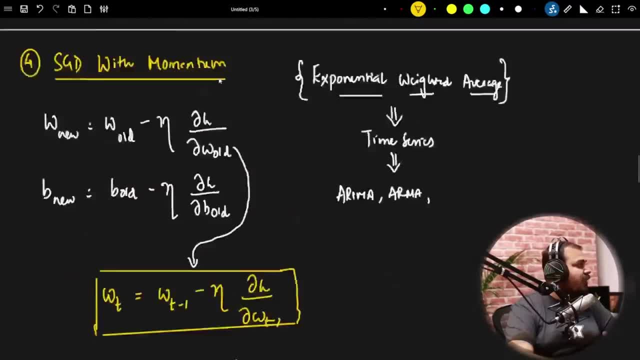 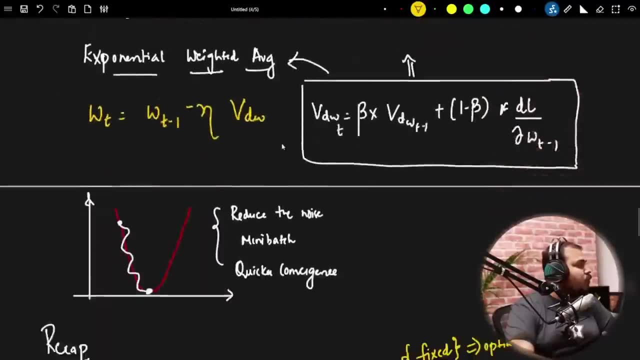 See smoothening. what is the equation? If I talk about smoothening here, I'm just saying that if I want to bring SGD with momentum over here, you can see that my smoothening equation will have VdW. but here what I'm using. 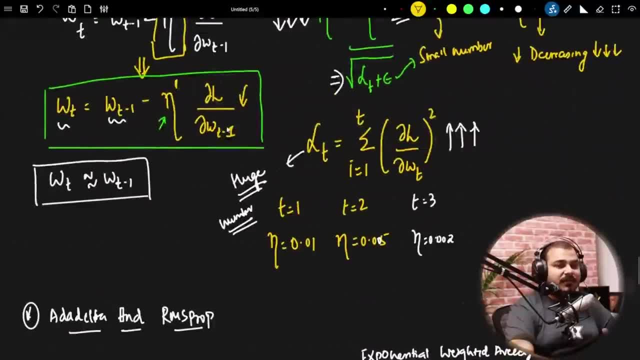 I'm using derivative of loss with respect to derivative of Wt minus one. Still I have removed basically the researchers in adaptive gradient descent and in Adelta and RMS prob. they are not doing the smoothening. still The smoothening is missing, right. 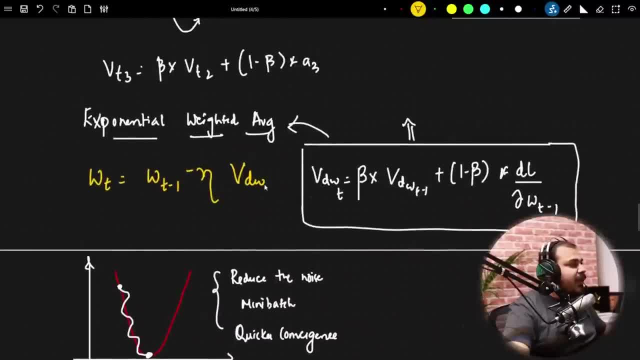 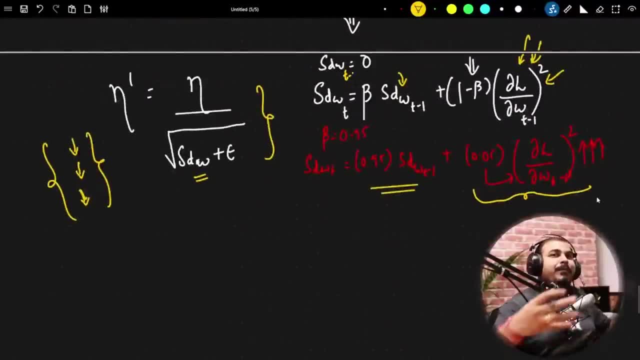 Because see in SGD momentum, what was the equation? that we saw VdW. Now this VdW and this HDW should be combined together. If we combine together, then it solves both the problem. okay, I'm going to again write this out quickly for you all. 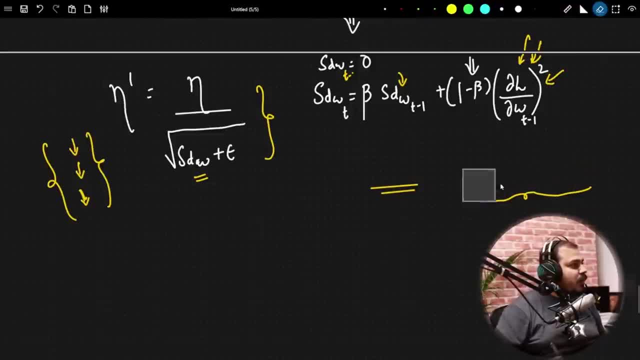 Let me rub it okay. Let me rub it quickly, okay, So what will happen if I apply a beta value of 0.95?? So my HDWt for the current timestamp will be 0.95 multiplied by HDWt minus one plus 0.05. 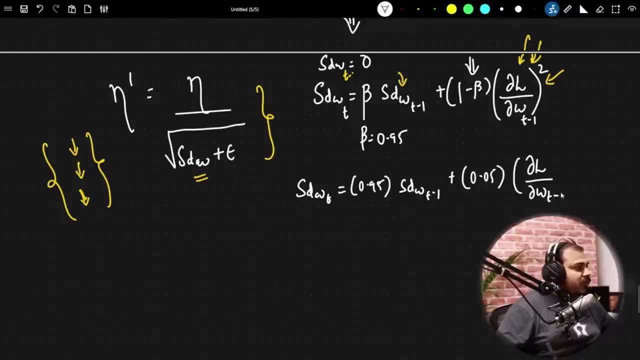 multiplied by derivative of loss with respect to derivative of T minus one whole square. Now we are controlling this. Let's increase with this right Now. we bought this HDW concept over here, but we left the momentum. The researcher left the smoothening momentum right over here. 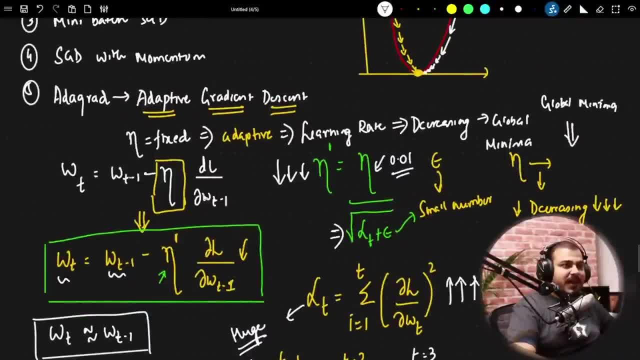 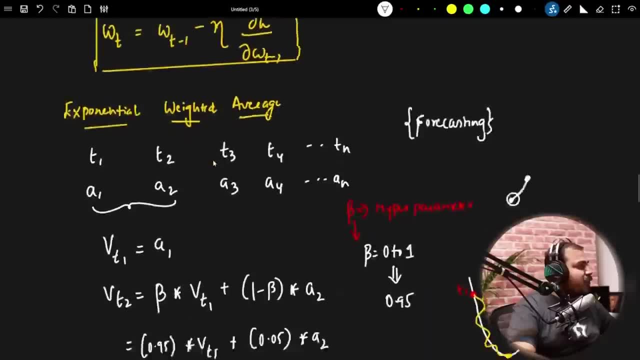 See, know where the smoothening momentum is present, right, So where that is, that is basically present over here In this SGD momentum we discussed right In SGD with momentum we brought this factor, That is, exponential weighted average. 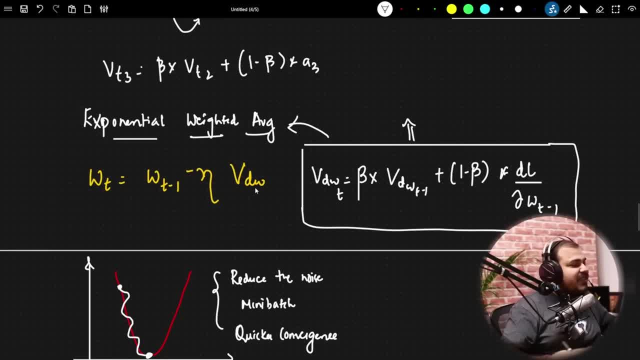 Now the next one that we are going to discuss. we are going to combine this exponential right, We are going to combine this exponential weighted average. We are going to combine this exponential weighted average average, and then we are also making sure that we have this adaptive learning rate. 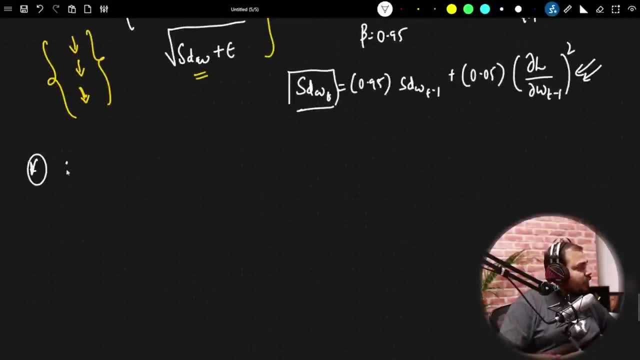 and when we combine both of them, we are going to get something called as atom optimizer. so in atom optimizer, what we do, we combine momentum along with the rms prop intuition that we have understood. what is the intuition that we understood over here? we made sure that here we have adaptive learning rate. adaptive learning rate when we combine both of this. 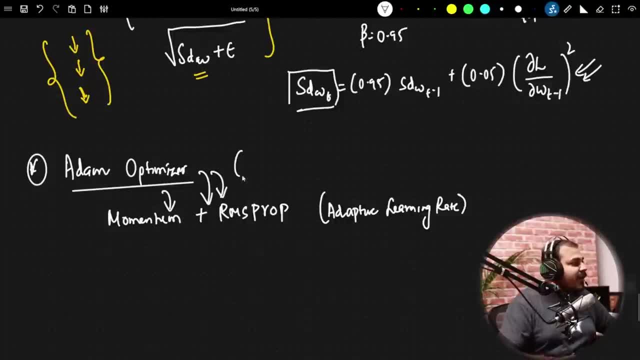 it becomes atom optimizer. right now, this is the best optimizer. yes, there are different different variants of this optimize optimizer, like adam max. there is different, different one, right, but right now, everybody is using the atom optimizer. okay, every everybody. most of the people are basically using atom optimizers and this is the best optimizer. right now, everybody is using the. 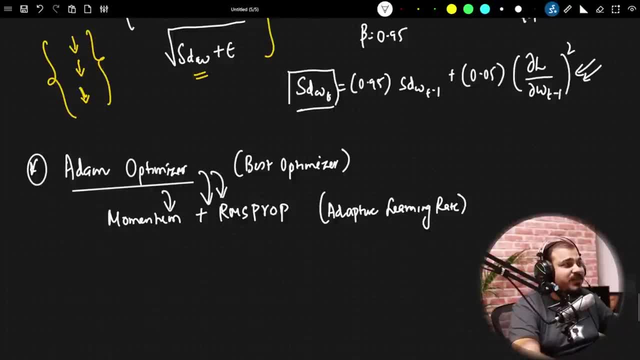 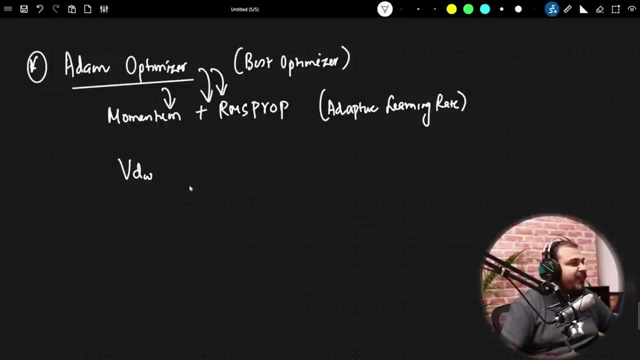 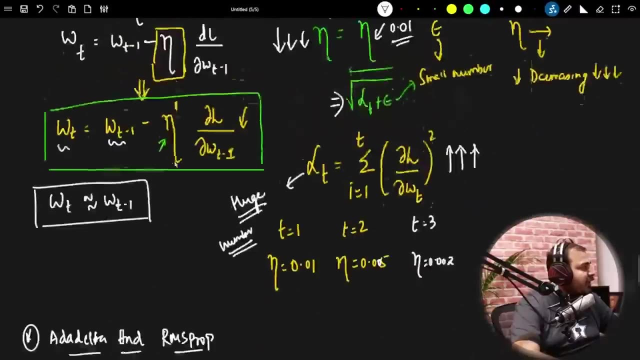 right now currently the best optimizer, which also researchers basically say. so here we are going to combine both this concept. now what will happen is that i will be having vdw and i will be having hdw and along with this, whatever i explained right, it also gets applied to bias, because bias will 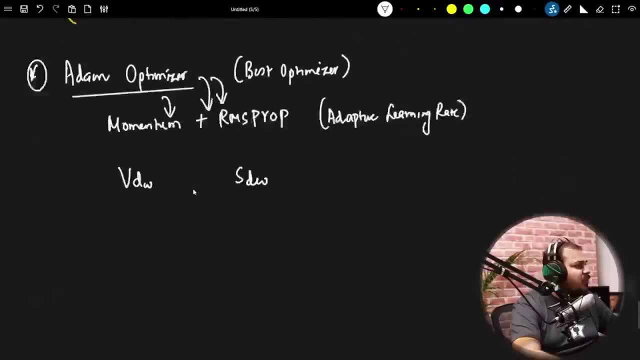 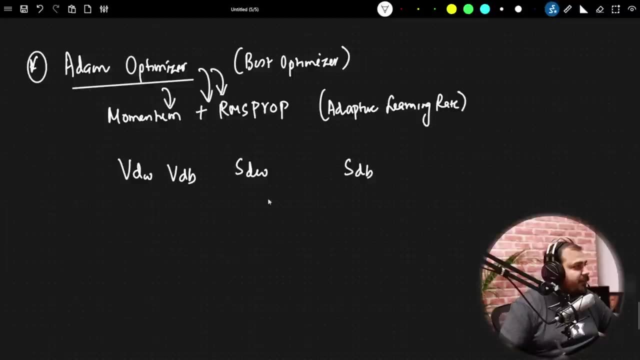 also get updated right. so same formula will get applied. so for bias also, instead of writing vdw, i will write now vdb. then here i will say hdb. initially this: all values will be zero. now, how, my, how? my equation will look like my weight updation equation will look like wt, wt minus one, mine, uh minus eta. and then here i will be having 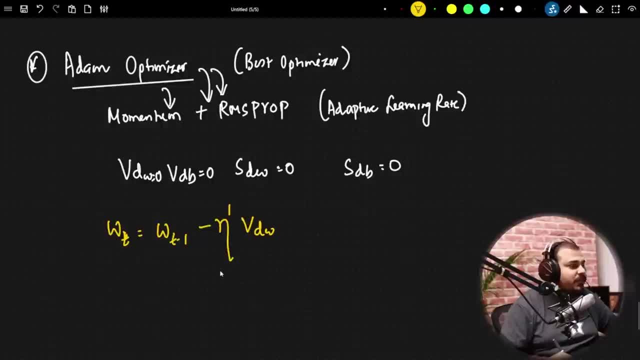 vdw. okay, this is for the weight updation formula, for bias updation formula. what will happen? bt? bt minus one, minus eta? here i will be having bdb, eta. everybody knows what is eta: learning rate divided by root of sdw plus epsilon. right, everybody knows this. what is vdw? vdw also everybody knows vdw is nothing but beta. 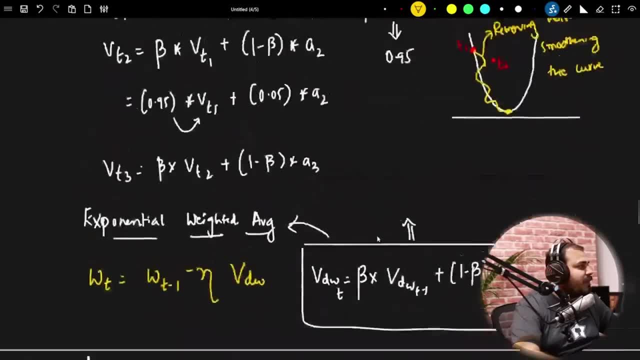 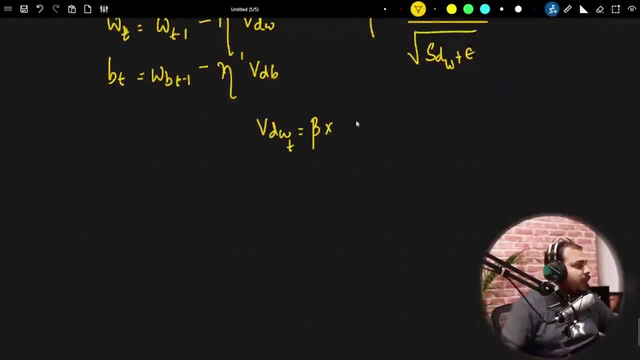 multiplied by. see the formula, what i have actually written over here: beta multiplied by wt, bdw t minus one, so multiplied by bdw t minus one. so this is what we are going to do here: we are going to write vdw t minus one multiplied by one, minus beta multiplied by derivative of loss with respect to. 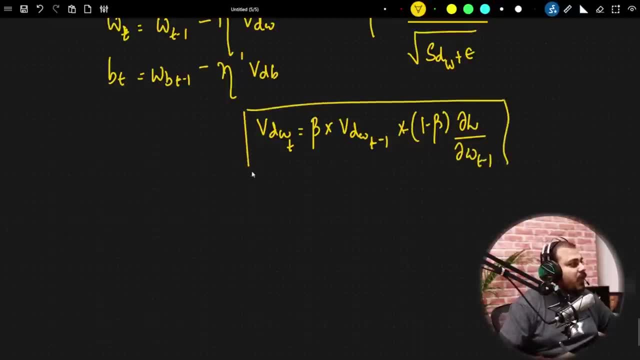 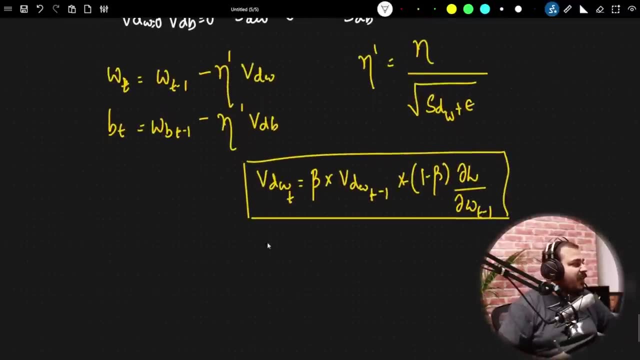 derivative of wt minus one. that's it. i am just combining this, both equation and whatever things. we have learnt it. we are just combining it over here in front of you itself, and this will also become what will be vd bt. this is nothing: beta multiplied by vd bt minus one multiplied by. 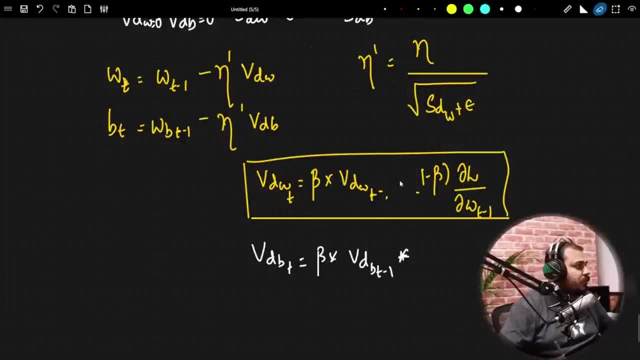 sorry, this will be addition, just a second. this will be one minus beta plus and this will also be plus one minus beta derivative of loss with respect to derivative of bt minus one. that's it now i have made you too much super smart. you know learning eta, what it becomes. you know the. 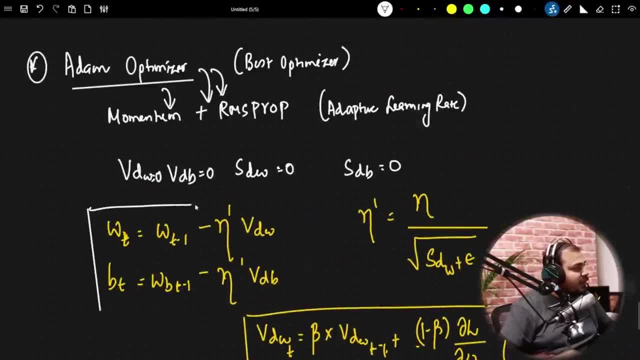 You know this. you combine this and this is your new weight updation formula for Adam optimizer. this will make sure that what all factors will get covered, what all factors. it is solving the problem of smoothening. It is forming following the problem of smoothing. It is making sure that the learning rate becomes adaptive. 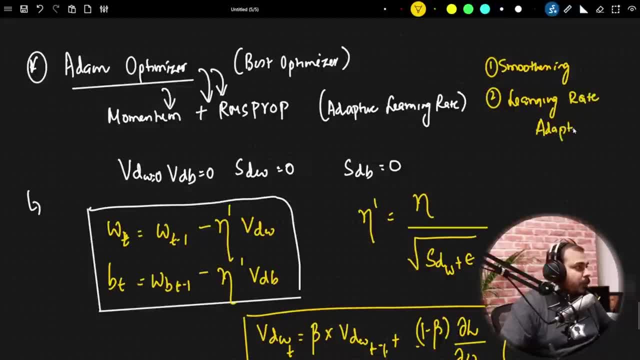 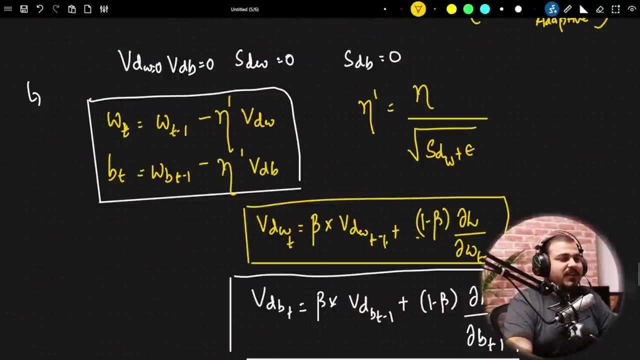 learning rate becomes adaptive and- And this is the story that we wanted to achieve- if you find some flaws also, you start writing a research paper, right, And there are different variants- Adam, max and Adam- and all right. So we'll keep the session today till this much. tomorrow We'll start the ANN practical. So thank you, one doll. 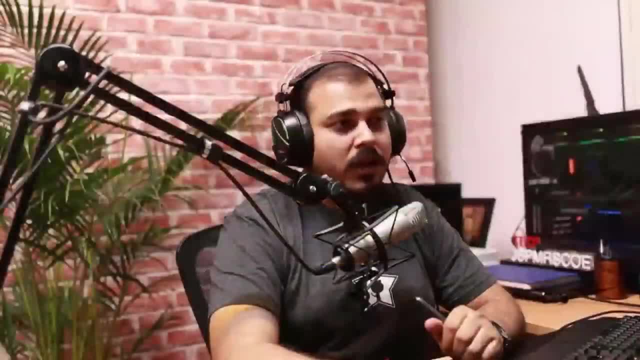 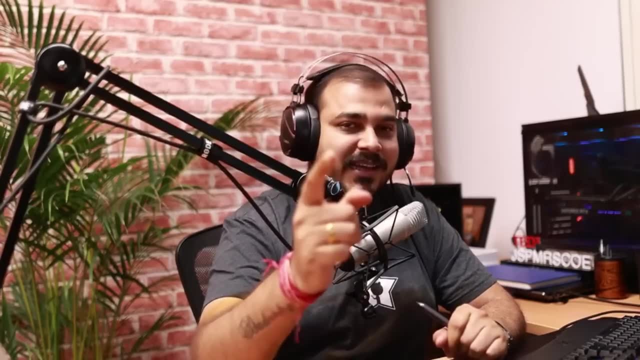 This was it for my side. Have a great day ahead. Keep on rocking, keep on learning, Never give up. always try to help others. That is it from my side. I Will see you all in the next session where we'll discuss about ANN and CNN. Have a great day. 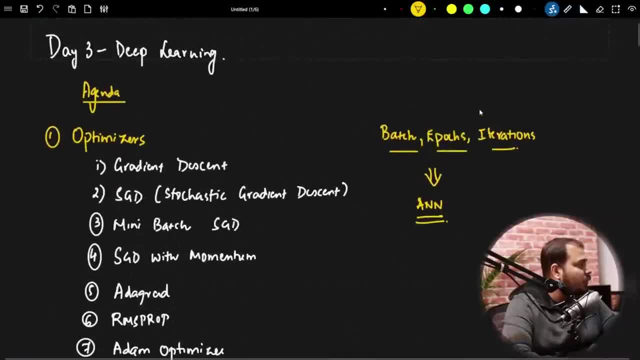 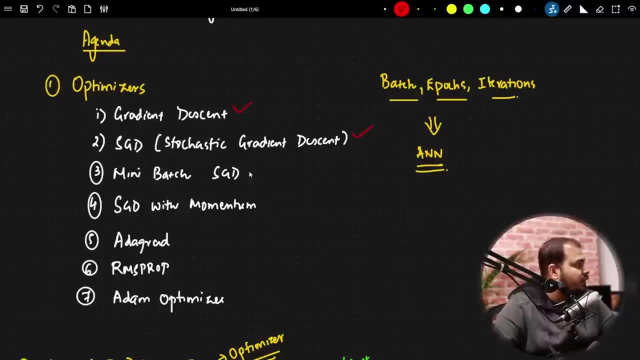 And in the previous session we have actually discussed about Optimizes. we have actually completed gradient descent, stochastic gradient descent, mini batch HDD STD with momentum adagraphic RMS prop and Adam optimizes right, we understood the entire maths for this. you know whatever maths was actually required. 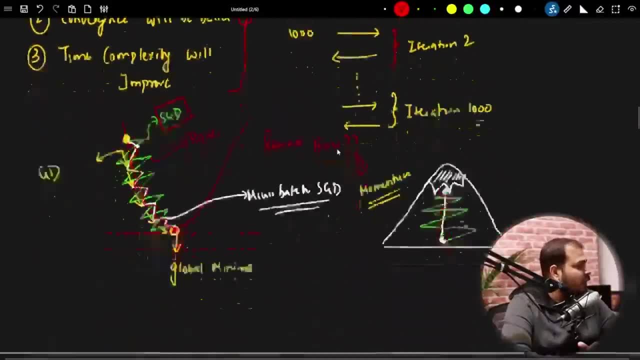 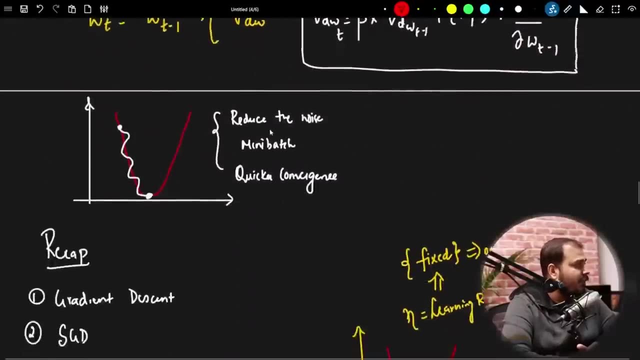 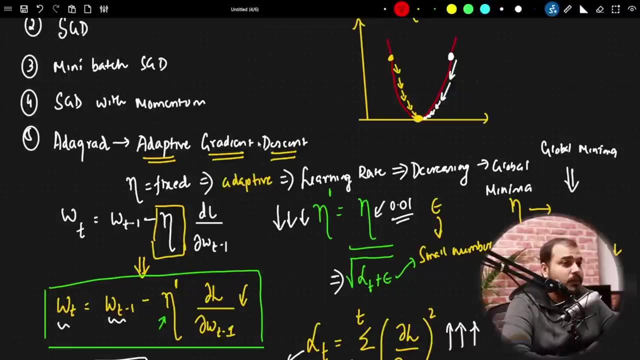 What is the difference? how the weight updation will basically happen. you know, and as you do with momentum, everything we actually can were Covered. we also understood about exponential weighted average. Then we understood about what is adaptive gradient descent. that basically means how we are actually being able to change. 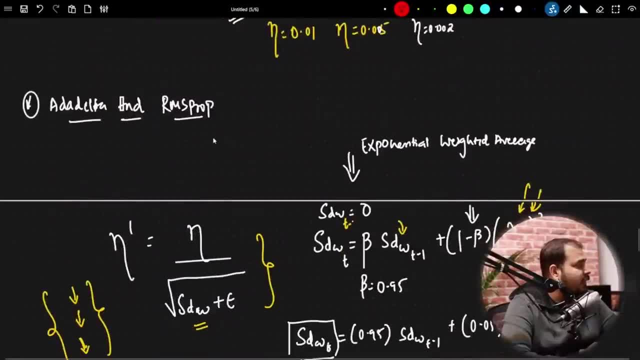 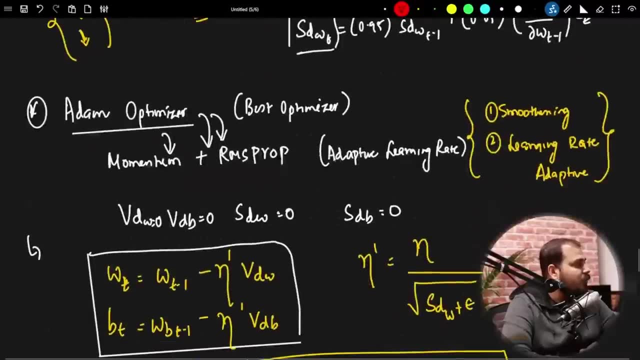 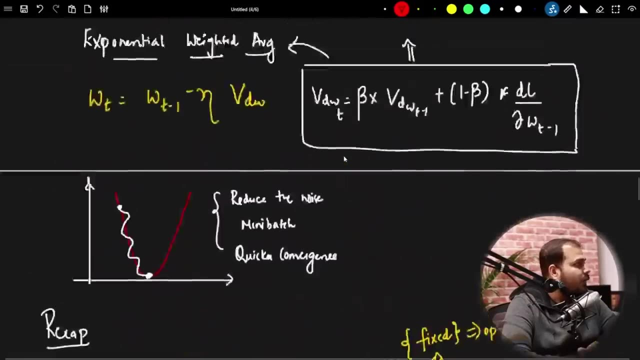 the learning rate. and Then we had this: Add a delta and RMS prop. then we had Adam optimizer and finally we saw how smoothening, How we were using adaptive learning rate along with exponential weighted average to basically go ahead with right. So let's talk about the agenda. 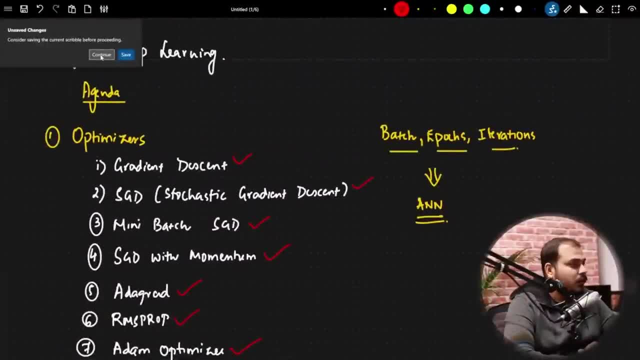 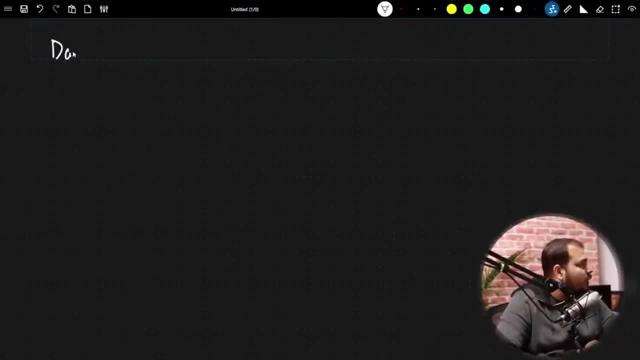 I'm just going to clear this quickly. Okay, so this is the day four. so day four or deep learning, Okay. Okay, now, in the day four or deep learning, what all things we are basically going to cover? Number one: we will be starting with a and n. 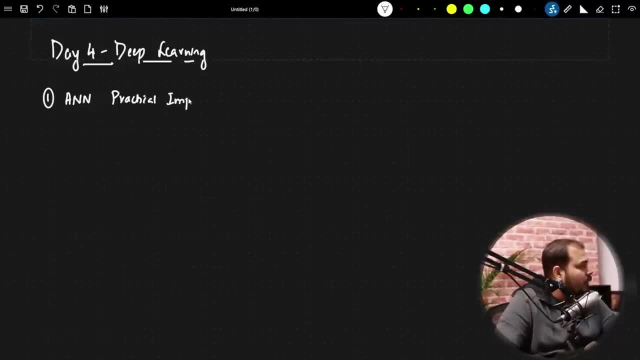 practical implementation. A and n- practical implementation. The data set is basically given in the pinned comment. okay, pinned comment. please check it out. You'll be able to see the data set. download it And just let me know whether you have downloaded or not. Okay, pinned comment. You can see right there. Google Drive link is given. Okay, 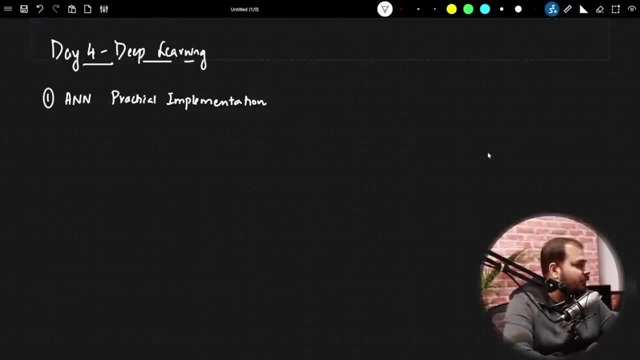 Check out the pinned comment guys. Okay for the data set. Okay, So we have completed a and n practical implementation. and the second one that we are basically going to understand is: what is early stopping? What is early stopping? What is early stopping? third thing we are going to understand about: 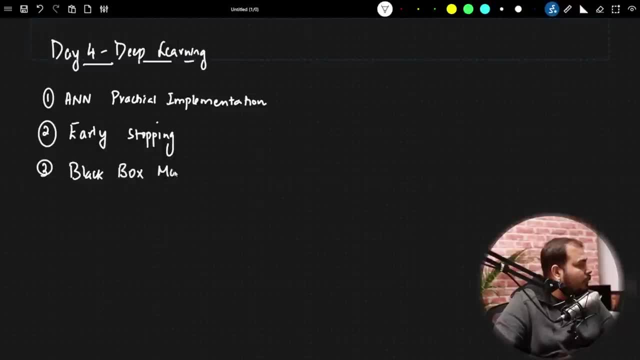 black box models Versus White box model. okay, and then, After we complete this, We are now going to understand about, You know, after black box model and The white box model, We are also going to understand about one important topic of CNN, so cnn introduction. we will try to cover it, you know. so let's see all these things, we will try. 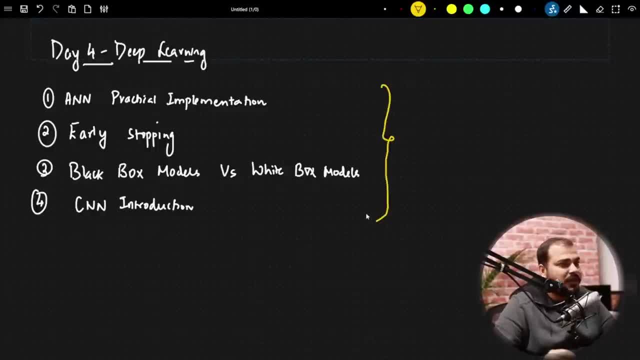 to cover it in today's session. okay, practical session will usually take a little bit more time because i really want to cover in-depth practical a and n, practical implementation, early stopping, which is a very important concept because many people say that how many epochs we should? basically 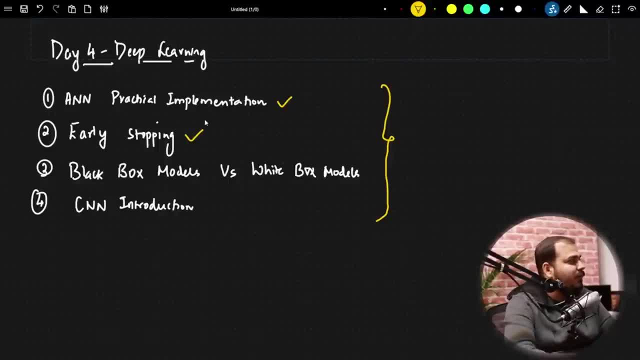 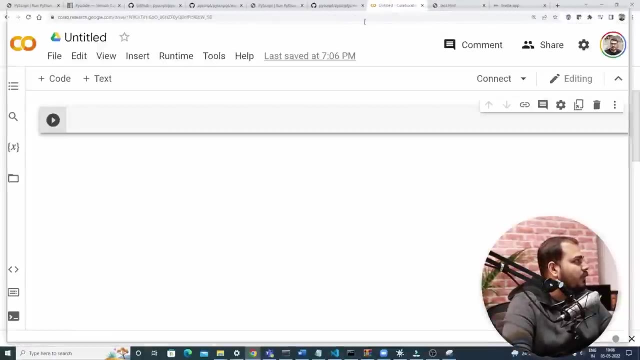 run, you know, while training the deep learning model, so it will be very much important itself. okay, quickly. uh, let's start without wasting any time now. so a notebook file i will be opening over here, okay. so here is the notebook file, uh, that we will basically be working on with, okay, and this is. 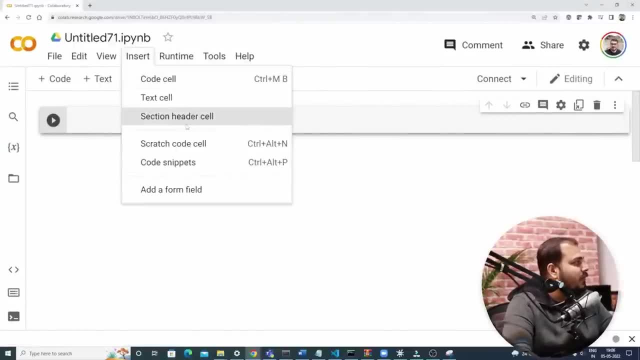 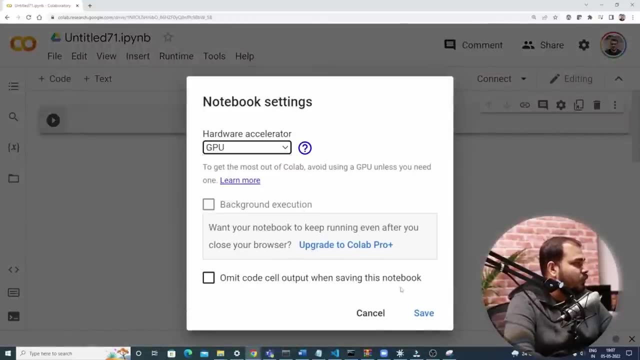 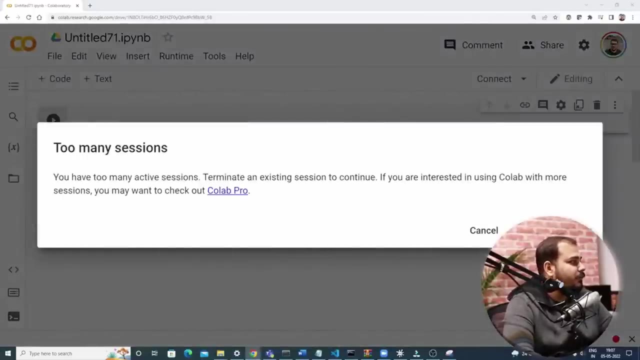 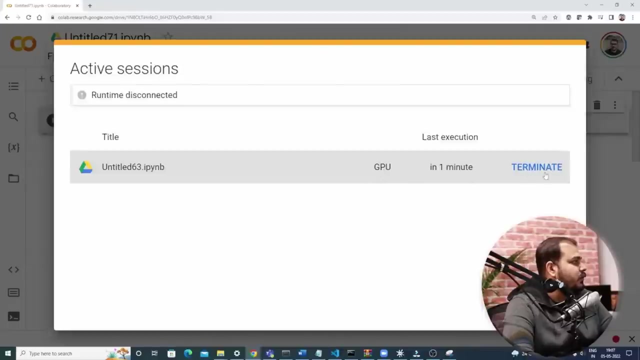 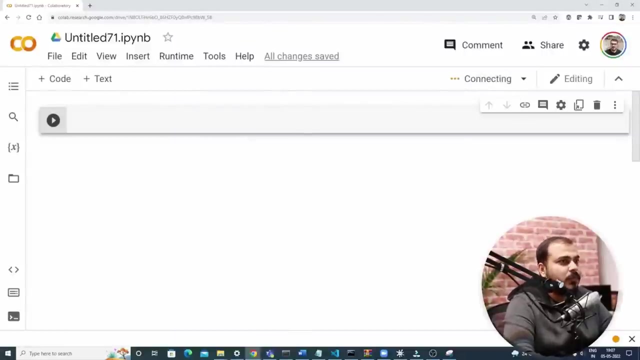 from google collab. you can basically use google collab itself and you do one thing before we start: we will change the runtime to gpu. i hope everybody knows what google collab is. you please make sure that someone in the pin in the message you can actually ping over there and tell. 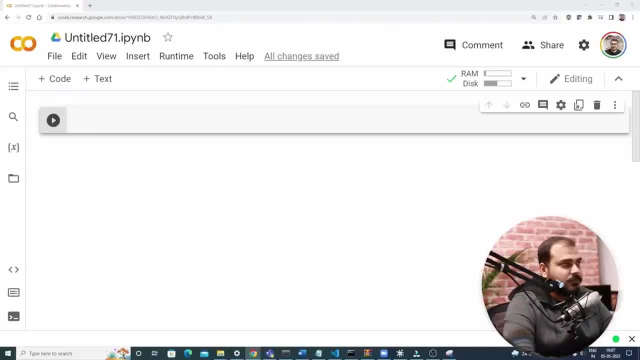 people to download the link. okay, fine, so perfect. uh, after downloading the data set, if you probably open the data set, uh, the google drive link, you will be able to see the csv file. okay, so, churn modelingcsv. we are going to see and we are going to cover this, okay, so here i'm just going to open. 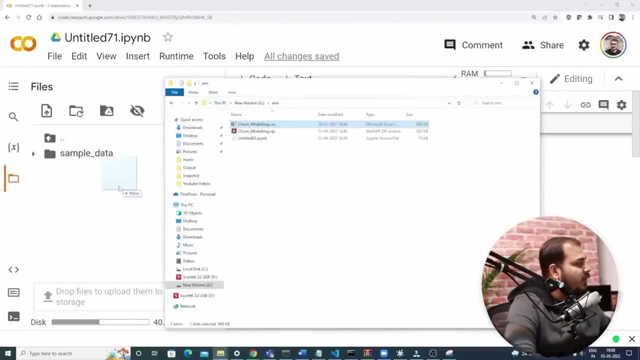 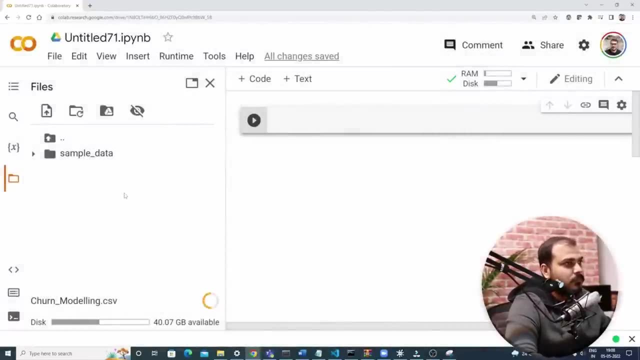 the folder. how do you download this? you just drag and drop it over here and you will see that you can download it over here. that's it, and automatically this churn modelingcsv will get uploaded over here. okay, so once you have this churn modelingcsv, now we can basically start what all things we are. 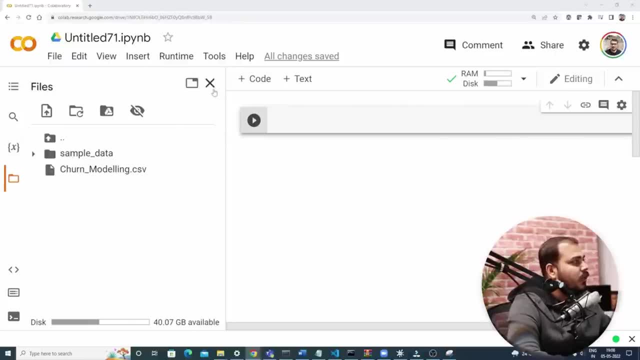 actually going to do with respect to ana? okay, very simple: with the help of google collab, you can do it now. now, the next thing that we are actually going to do is that start writing the code, okay, and here we are specifically going to implement an n, that is, artificial neural network. now let's go ahead and let's start writing the code, okay, so 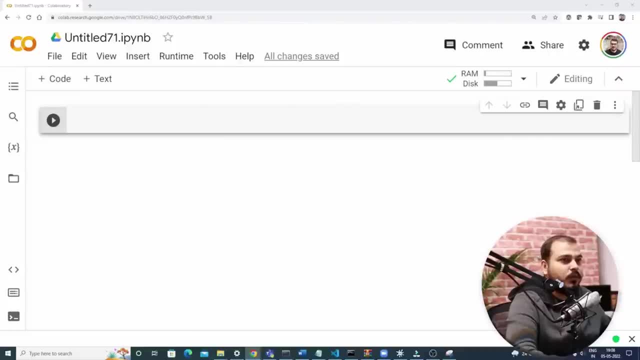 as usual. uh, in the initial stage, what all things we have to do and how we have to do so. first of all, i will start with pip install. pip install tensorflow, because i'm going to use tensorflow gpu, so i'm just going to do this installation and it will. 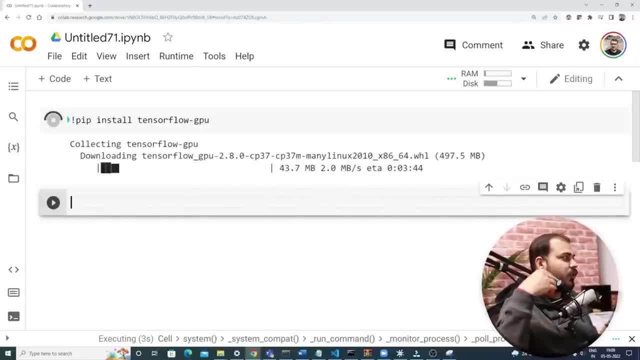 probably take some time to do the installation. it depends on your internet speed and then we will start seeing which version of tensorflow we are going to work. work with right, which is the recent version. with the help of that, we are going to basically work with okay, so we'll wait, uh, till the uh, the entire tensorflow gpu gets. 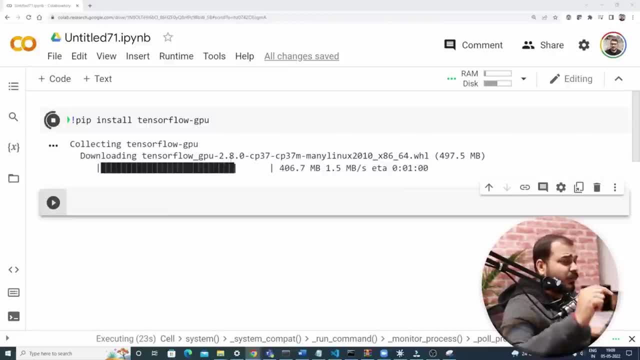 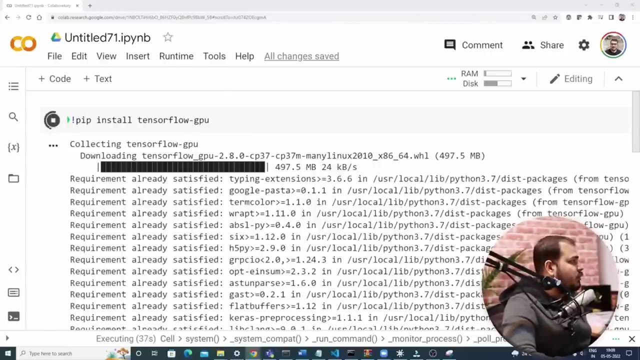 downloaded and right now we'll be working with the version that is greater than 2.0, because the version with 2.0 has, uh- you know uh, the. the version that is greater than 2.0 has, uh- you know uh, the keras also integrated within them. okay, so let the installation happen and you'll be seeing that. 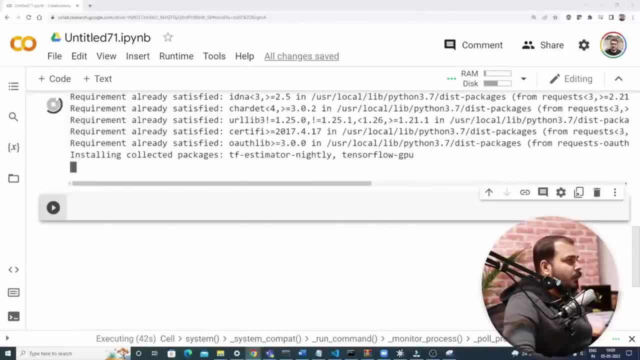 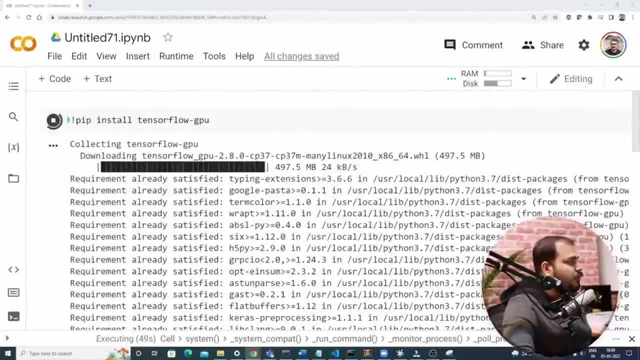 after some time the installation will be done. okay, then, uh, after this installation takes place, i can also go ahead and see which version of the tensorflow we are going to use. okay, so again some time more, and probably everybody is going in that specific speed. okay, so it is 497.5 mb, so the fine. 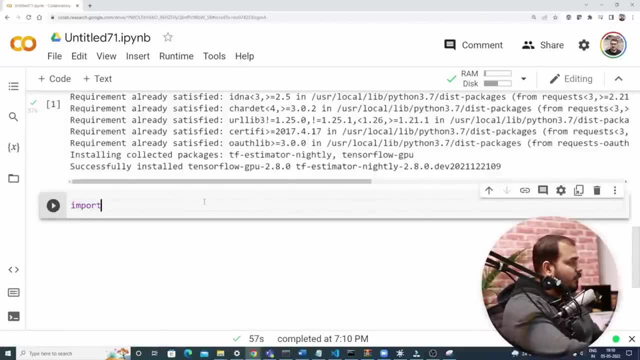 the code has got executed. now what i'm actually going to do? i'm going to import tensorflow- tensorflow- as tf and then i'm also going to print the tf version. okay, so, tf dot- underscore, underscore, version, underscore, underscore. okay, when i execute this here, you'll be able to see what version is there. it is nothing. 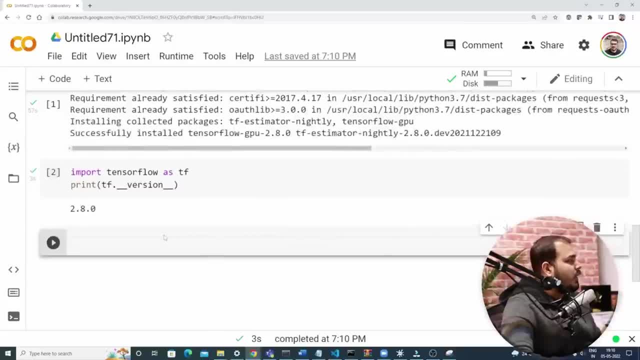 but 2.8.0. okay, now, uh, in this version, we are basically going to work because this version is greater than 2.0 and, uh, this version, uh has keras integrated into it, so we'll continue with this specific version. perfect. now, in the next step, what we are going to do is that we are going to 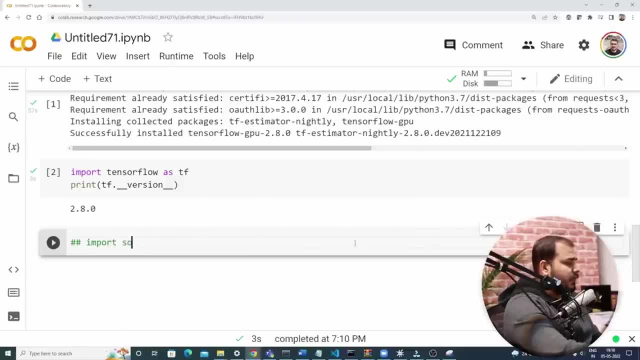 import some basic libraries. import some basic libraries. okay, make sure that you always write the comments so that you'll be able to understand what all things we are actually going to do. so here i'm going to import numpy as np. i'm going to import matplotlib for the plotting purpose i plot as plt. then i'm going to import. 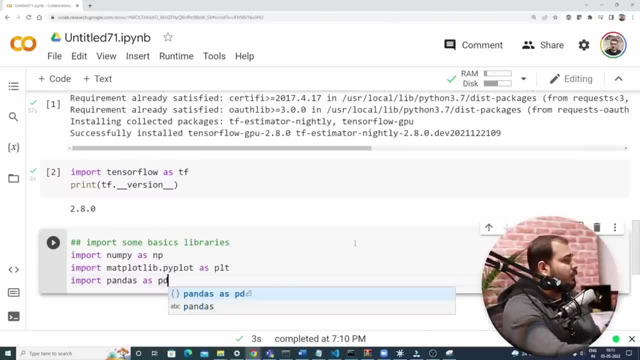 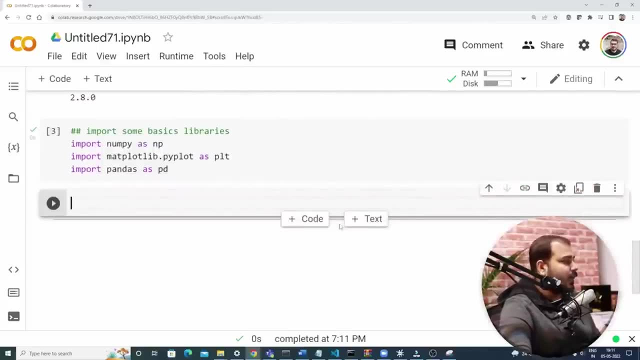 pandas as pd. okay now, uh, this three libraries i'll specifically be importing because i really need to read the data sets and all, so that is the reason why i'm going with this. then, uh, let's go ahead and read my data set, so it will be pdread, underscore, csv and i have this. 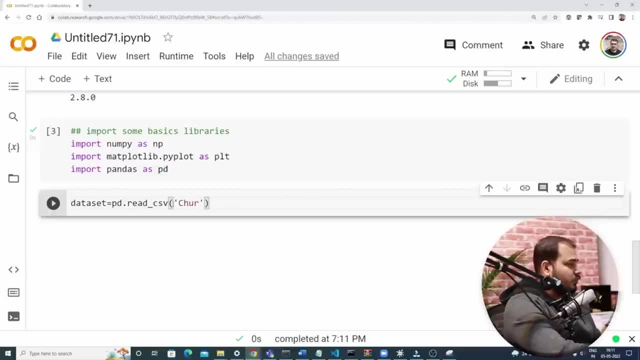 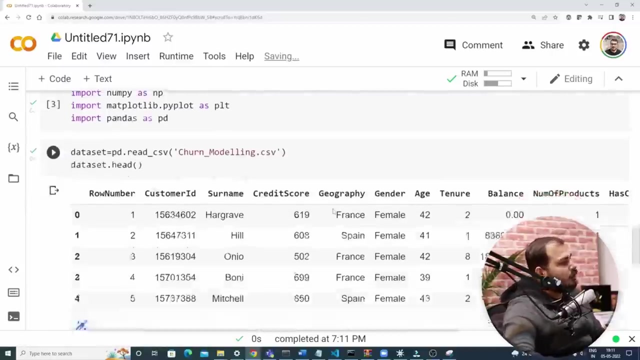 churn modeling data set: churn underscore modeling dot csv. remember, i have actually put this data set over here, so in this folder you can actually see it, okay, and once i will execute this and probably and i'll write data set dot head. so the problem statement is quite simple and here what we are actually trying to do is that. 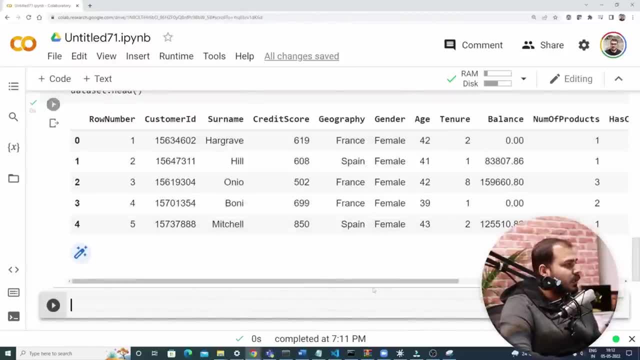 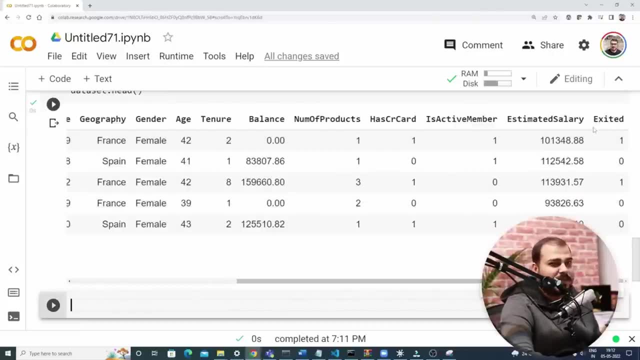 there is specific data set over here, from row number to this, all things, and we need to predict right now. this is a binary classification problem. we need to predict, basically, whether the customer is going to exit that particular bank or any company, whether all these products, that they are being used in the specific bank, whether they are going to just uh, you know uh. 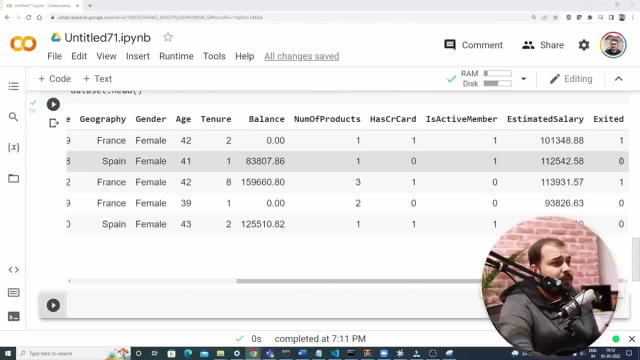 exit it in the future case or not. so if you want to really prevent it- to uh, prevent the execution, like they don't want to quit the bank- so we should definitely provide some more services. so that is the reason we are trying to create aérique table. so that's all and for this video. i hope you liked the video and if you did subscribe to the channel now, don't forget to decided to hit the like button. it means a huge help and i will see you forever in the next policy video. so see you in next video. Bye, Bye Jingle. announce the results of the group as a mentor in tech. introductory audience interview. 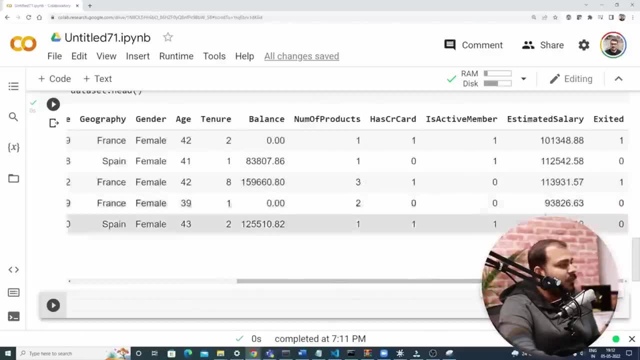 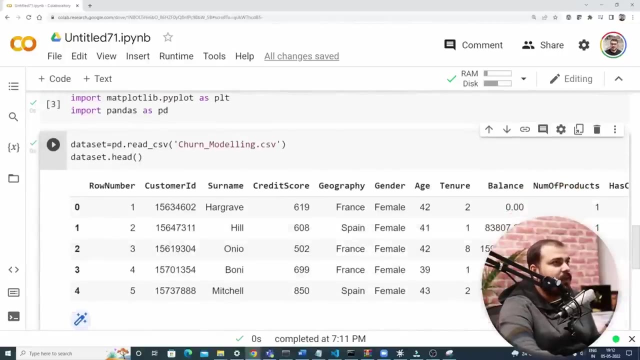 model. uh, by seeing all these details, uh, we will try to see, like, whether the customer is going to exit the bank or not. so here, exited is basically my dependent feature. remaining, all are my independent features. okay, so now the main thing that what we do over here is that, first of all, 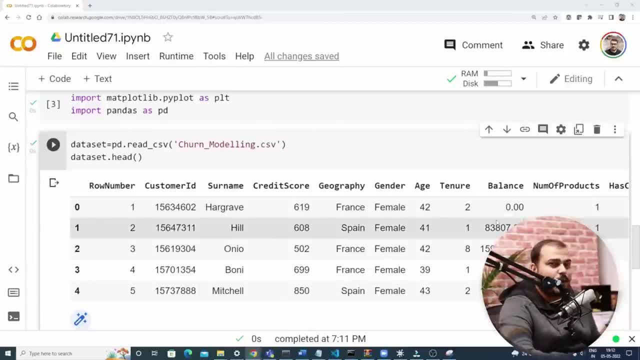 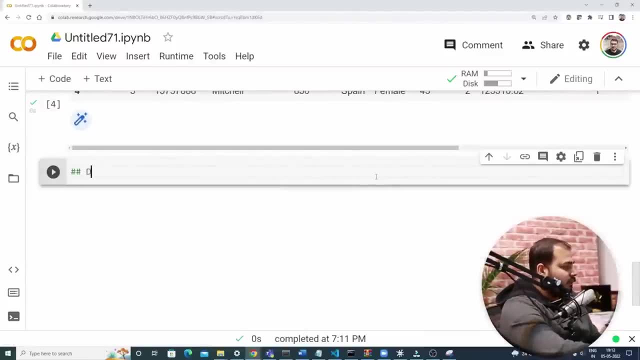 whenever we are doing this, we really need to convert this entire data set into independent and dependent features. so here what i am specifically going to do: i'm going to basically divide the data set- data set into independent and dependent features. right, dependent features. so once you do this, uh, then what i'm actually going to do: independent features. 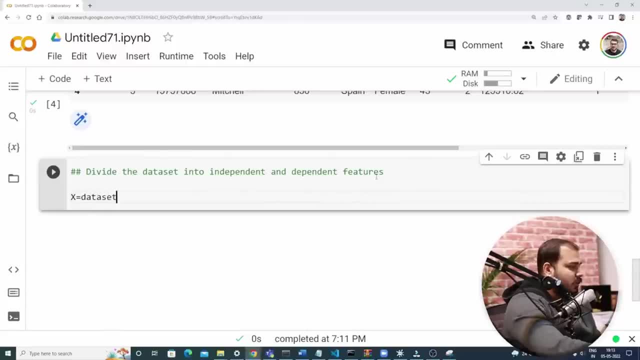 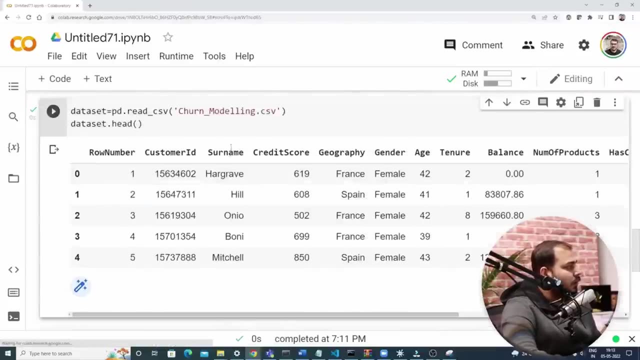 i'll denote it by capital x and i'll write dataset dot. i lock, i log basically means index location. okay, now, index location: here you can basically see from row number, row number two, specific. you know the item here. in this case it's kind of an index location. okay, so i'll write, you know, binates. 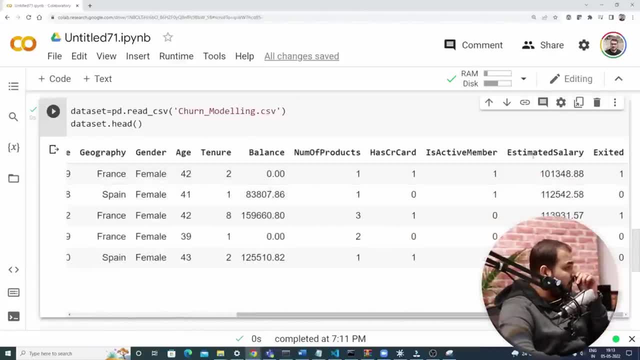 if I probably talk about estimated salary. this should all be my independent features, right? And again, row number is also a continuous number, right? So I would definitely not like to have row number over here. I can remove the row number because it is just a unique value. 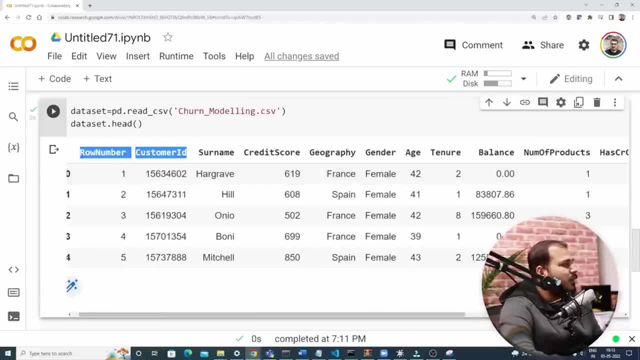 I would also like to remove the customer ID, because customer ID will also not make any sense. So what I will do is that from this surname- okay, name can also not play a very important role, because I definitely don't like to have name and all also. 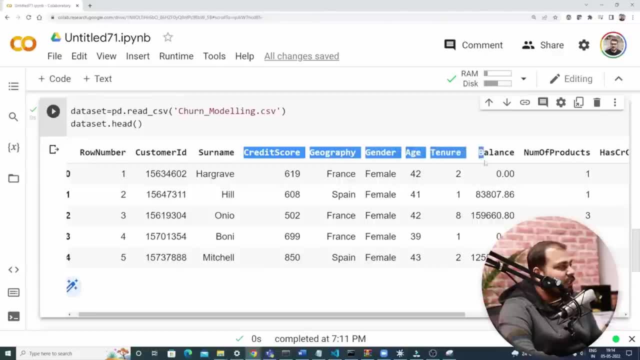 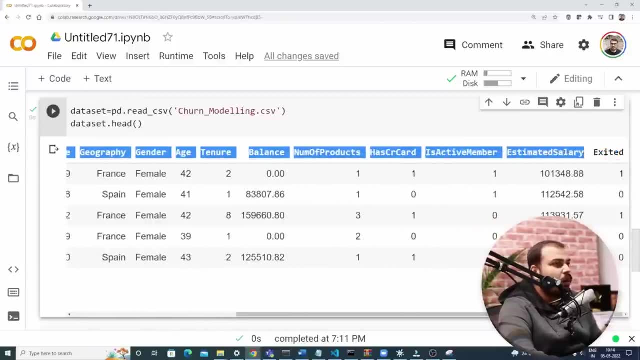 but I will focus more on this features, that is, credit score, geography, gender tenure, balance, number of products as credit is active card and estimated salary and exited. okay, So this till here will all be my independent features and exited will be my dependent feature. 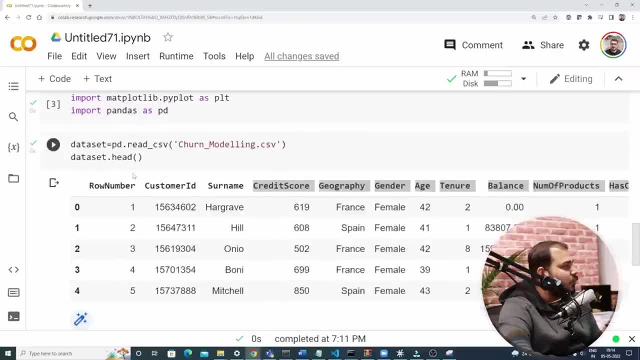 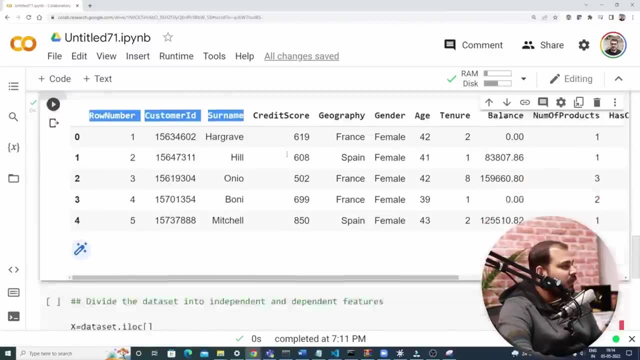 So in order to do this, I need to find out from which index location I want. So if I count like zero, one, two, right. All these features I don't want, right. So I can basically start for the third index. 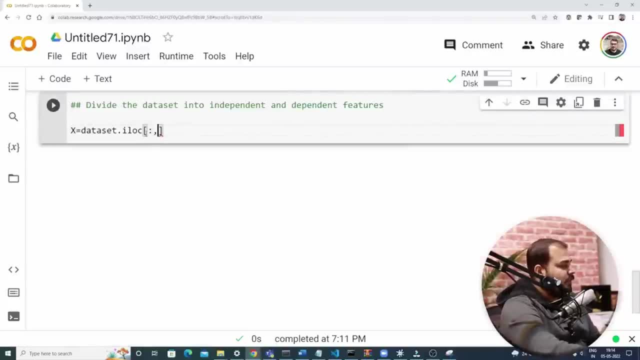 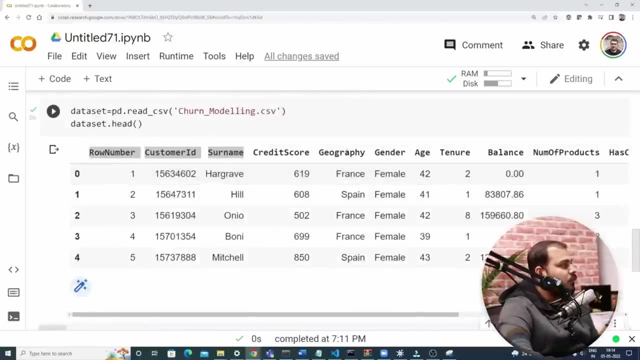 So I definitely want all the row comma I basically want from three to 13th column. 13th column is nothing, but if I start counting zero, one, two, three, four, five, six, seven, eight, 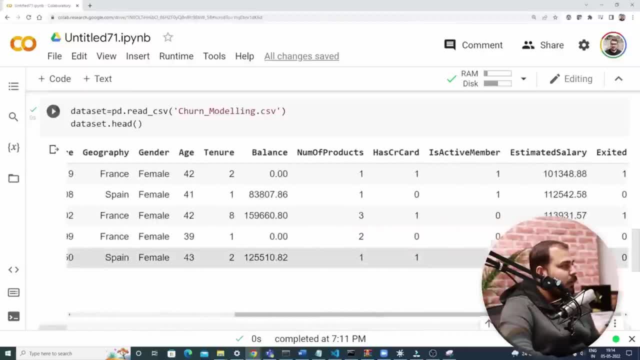 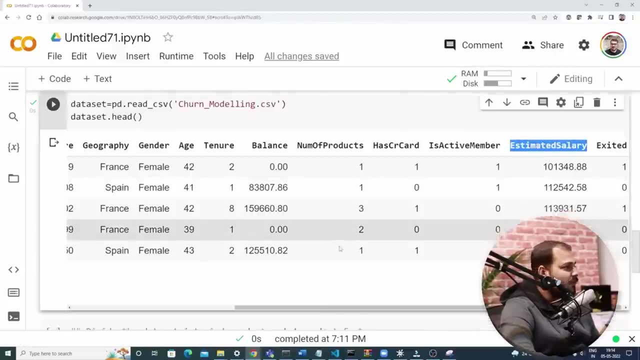 nine, 10,, okay, Nine 10,. 11,, 12,- right, So 11,, 12,, 13.. So till the 12th index. I require all these values in my independent features, So I will basically be writing three colon 13.. 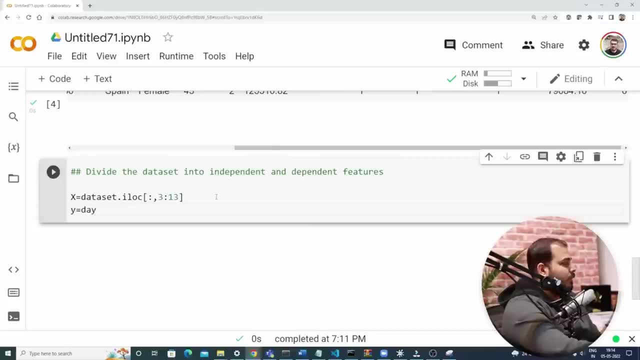 Similarly, when I go to the next line, y is equal to data set, Data set dot iloc. okay, Here I definitely want to write all the rows and my output feature is basically my 13th column. So if I execute this here, you'll be able to see that. 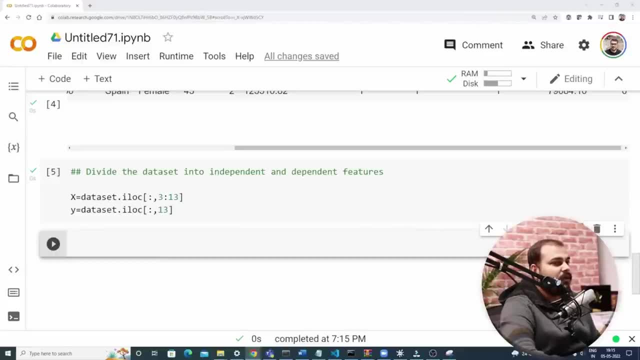 I have actually divided the entire data set into independent and dependent features. okay, And what I will do? I will just go and basically check out xhead and here you'll be able to see the independent features, which is very much easily available, okay. 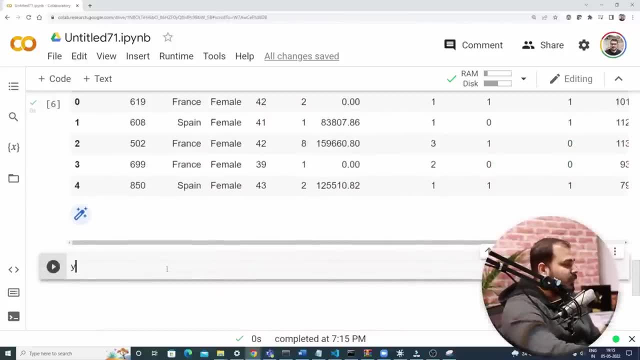 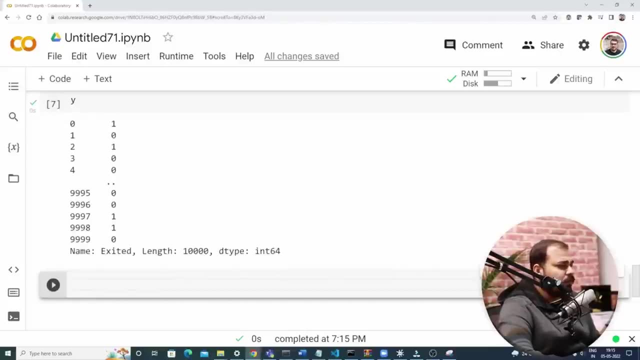 So here you can basically see this, okay, And similarly, if I probably see y and here you'll be able to see my output feature, which is my dependent feature, okay, So I hope everybody's clear with this much and let's go to the next step. 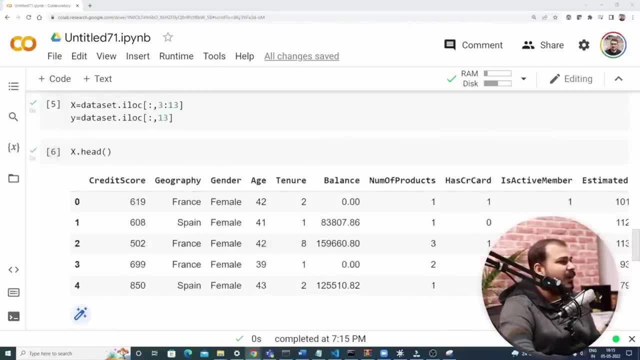 We see over here also. this data set is not that clean. They are independent features. They are in this independent features. they are categorical columns, right, Categorical columns like gender age tenure. sorry, Gender geography is definitely our category features. 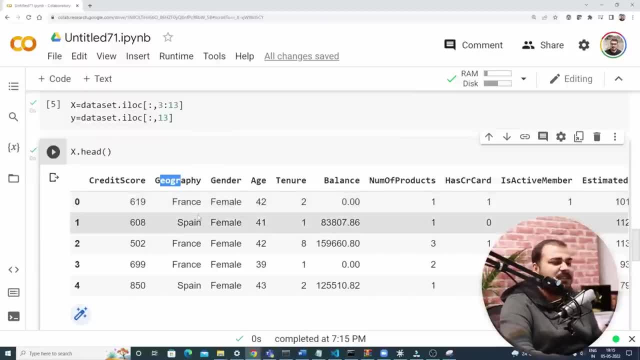 So we really need to fix this category features. The number of categories in this category features are very less. We can basically use one-hot encoding or we can use get dummies in pandas- right, It is up to your choice, okay. 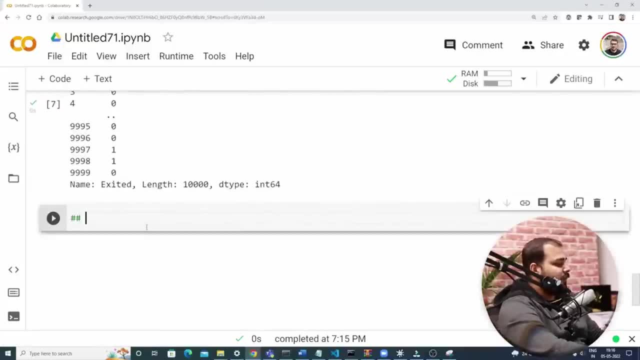 Now what I'm actually going to do, and probably this will basically be my feature engineering part, because in the feature engineering I really need to fix all these problems of, you know, handling the category features or not. So here I have geography. 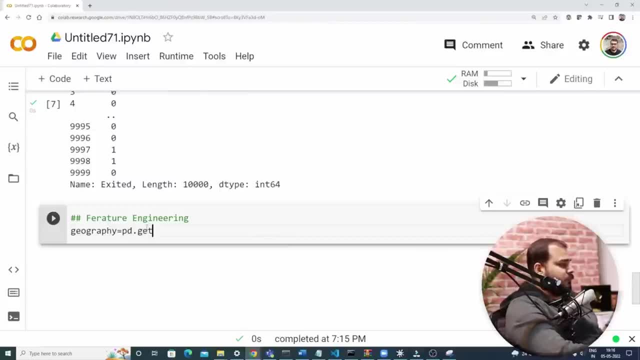 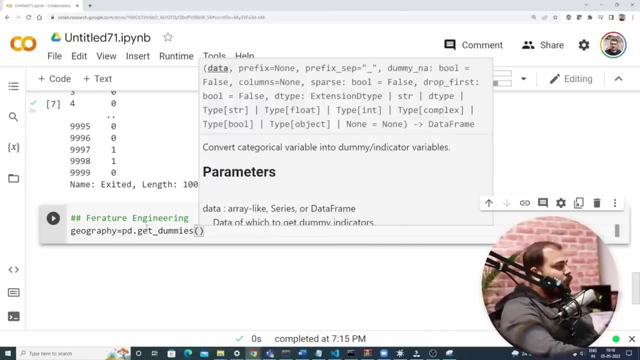 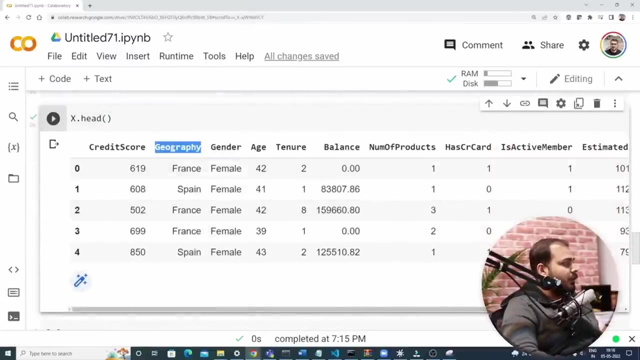 Here I have geography and here I'll basically write pdget underscore dummies, Okay, pdget underscore dummies. And here I'm specifically going to basically say that which column I really want to convert that as in my category feature. So here is my geography column, right? 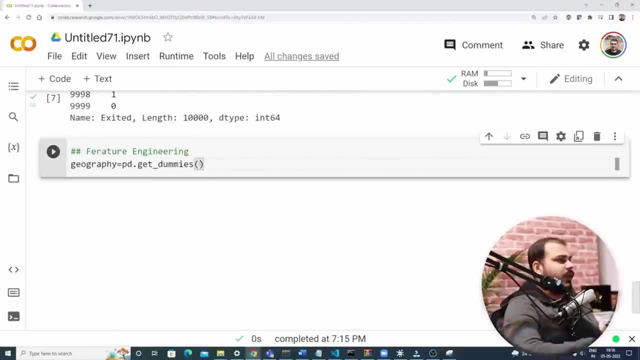 So I'll pick up this value and I'll put it over here And I'll say x of geography. right, When I say pdget dummies with respect to geography. let me just execute this Now: geography, let's say it has three unique columns. 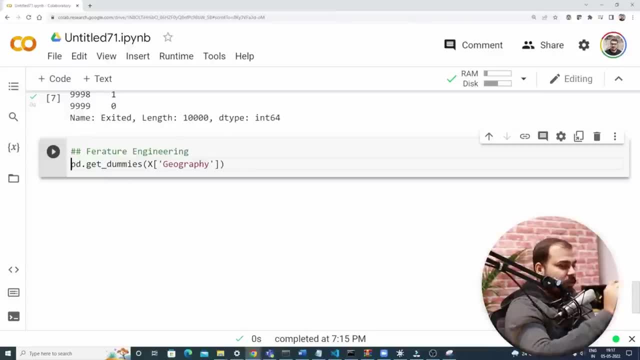 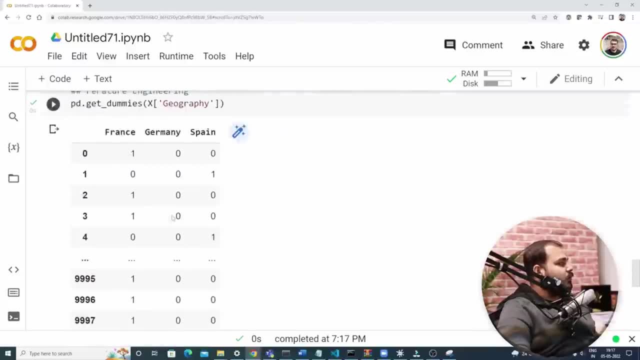 So, as I have to do, I've got three unique features like three unique values right- Different different countries- And if I try to just execute this, I will be able to see that it will get converted into one hot encoded. 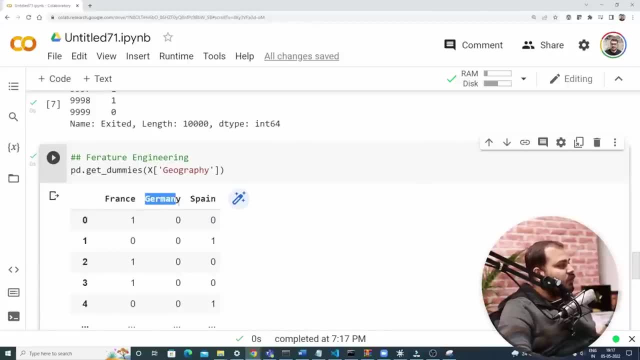 Like: wherever the France value will be there, that will become one. Wherever Germany will be there, that will become zero, Because in this row France was there. wherever that specific value is there, it will become one. remaining all will become zero. 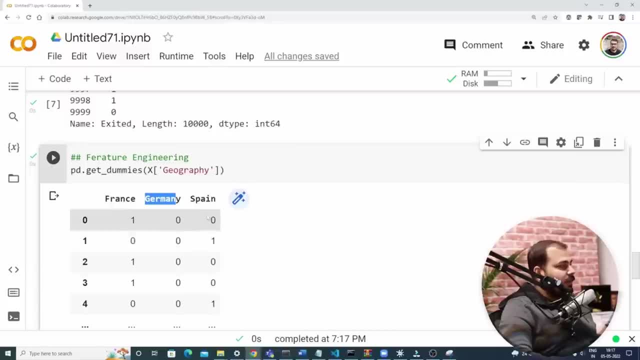 Now suppose in the second record we had one in Spain, right, The Spain record was there, so it became one. So that is the purpose of the get underscore dummies over here. we are specifically trying to do, okay, and the next step, what we are also. 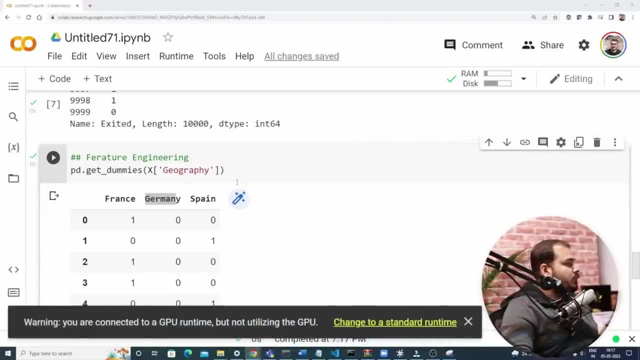 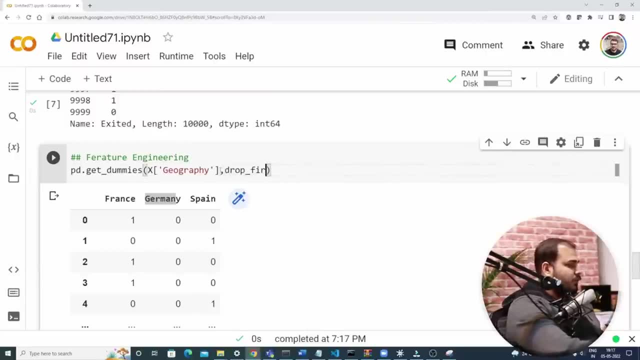 looking at is that we will try to focus on. we will try to focus on one more important parameter, which is called a drop underscore first is equal to true. right, when I use drop underscore first is equal to true. instead of showing all the three columns, it will just show the two columns like Germany and Spain. 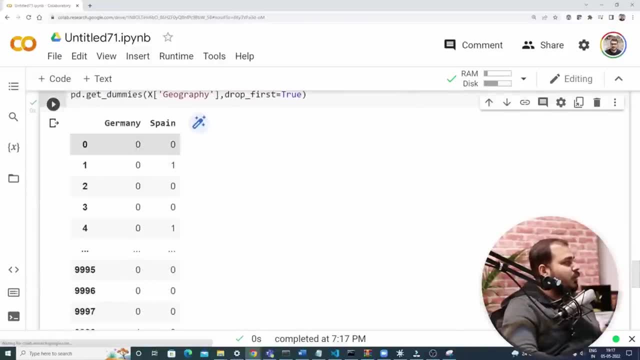 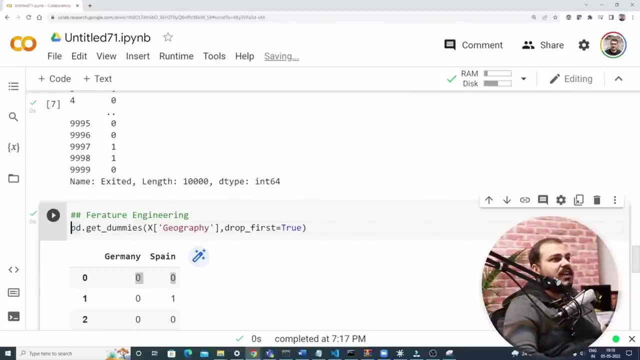 because if France is present this, both will become zero. okay, so we can actually use this two columns to represent all the three columns itself. okay, so this is where we specifically use get underscore dummies. now, what I am actually going to do is that I'm going to create a column for this. okay, so I will say that, okay. 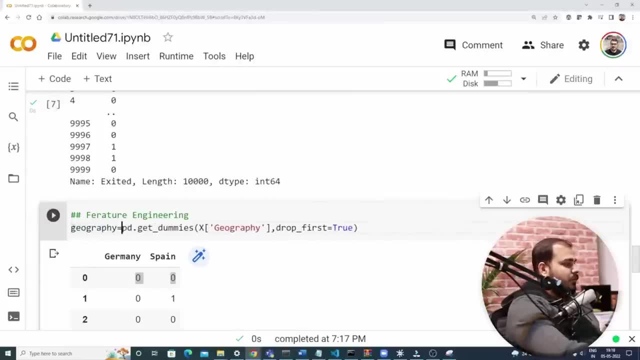 fine, this will be my geography variable and I'm going to basically create this. similarly, if I use gender for gender also, we will specifically write like this: PD dot get underscore dummies. and here I'm just going to say that X of okay gender, and here also I'm going to 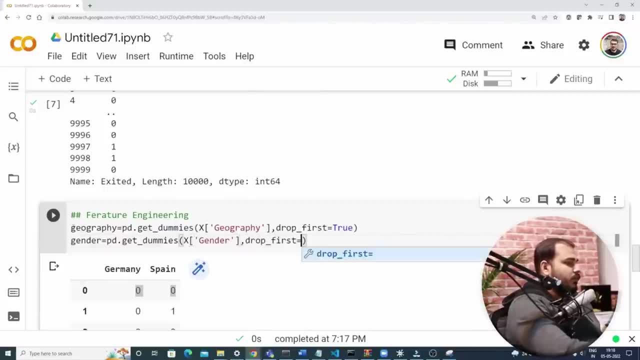 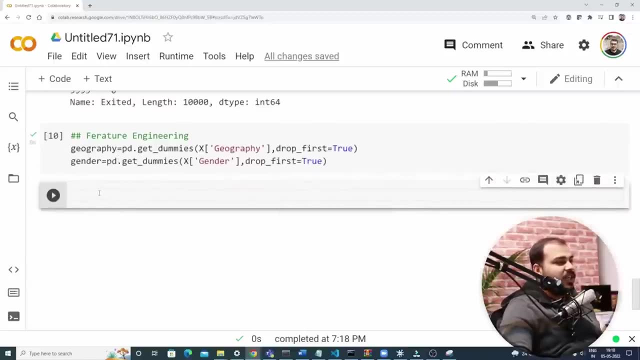 basically apply: drop underscore first is equal to true. okay, so if I execute this two things, it will get executed perfectly. and now I will also have a gender, which will be a one-hot encoded, and I'll also have geography, which is will be one-hot encoder. now what I'm actually going to do is that I'm going 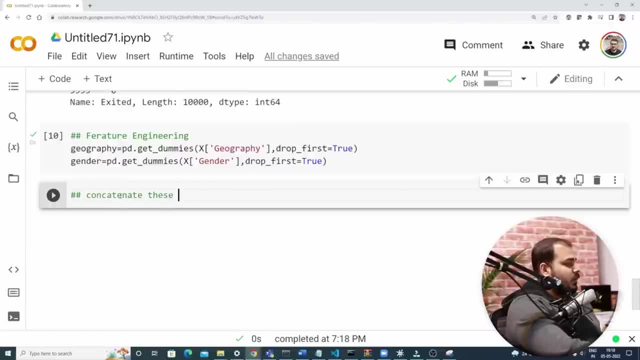 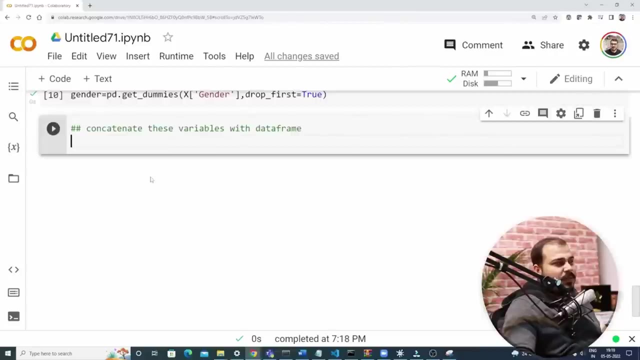 to concatenate. concatenate this variables with the data frame: right, with data frame. now, in order to do this, the first thing is that I will drop geography and gender column, because now I don't want this geography and gender column, so I'm just going to drop it now. in order to drop it, it is very much simple. all you have to 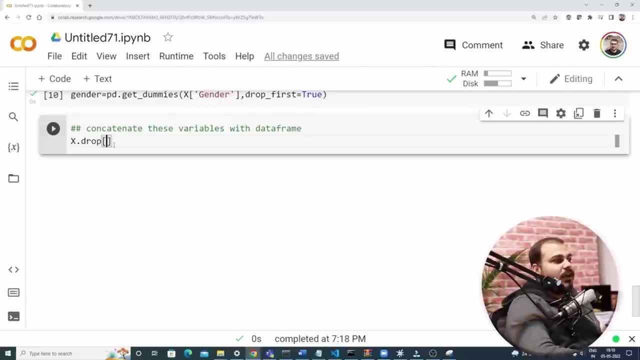 basically say that let's take the independent feature and apply a drop operation and inside this, what I'm actually going to give. I'm just going to give my, so it will be a function. I'm just going to give it a function. I'm just going to give it a function, so it will be a function. I'm just 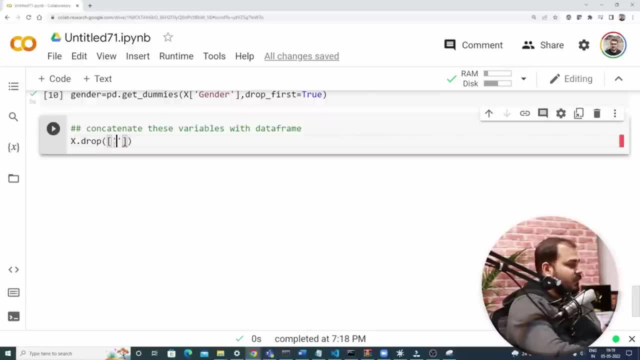 going to give it a function. I'm just going to give it a function. I'm just going to give it a function. I'm just going to give my features right. what all going to give my features right? what all features I have. I have specifically features I have. I have specifically. 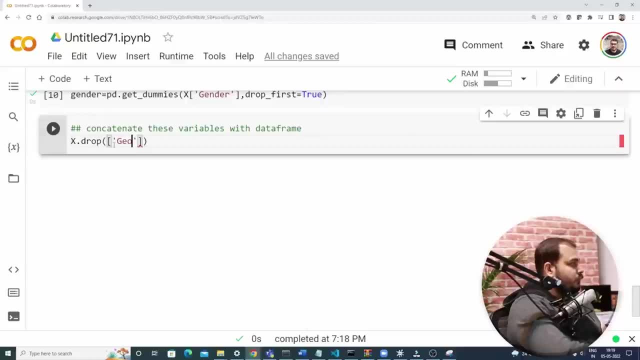 features I have. I have I have specifically geography, geography, and my another geography, geography and my another geography, geography and my another feature, that is my gender right. I'm just feature, that is my gender right. I'm just feature, that is my gender right. I'm just going to say gender. okay, so these two. going to say gender okay. so these two going to say gender okay. so these two features I'm going to have and I'm going features I'm going to have and I'm going features I'm going to have and I'm going to make sure that I have to write axis. 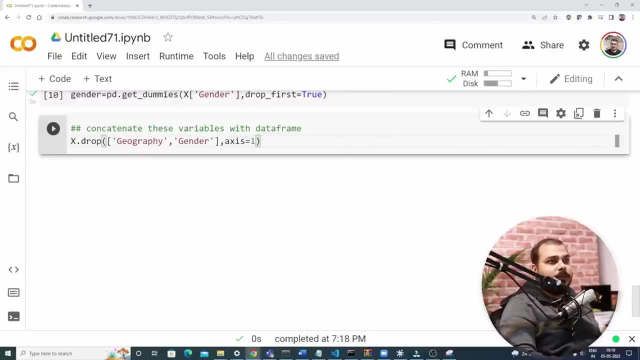 to make sure that I have to write axis. to make sure that I have to write axis equal to 1, because I need to drop the equal to 1, because I need to drop the equal to 1, because I need to drop the columns, I do not need to drop the rows. 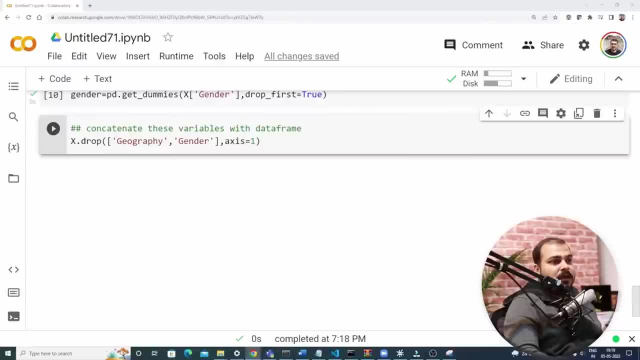 columns, I do not need to drop the rows, columns, I do not need to drop the rows. so that is specifically very much so. that is specifically very much so. that is specifically very much important. okay, and you, I hope important. okay, and you, I hope important, okay, and you, I hope everybody is able to understand till. 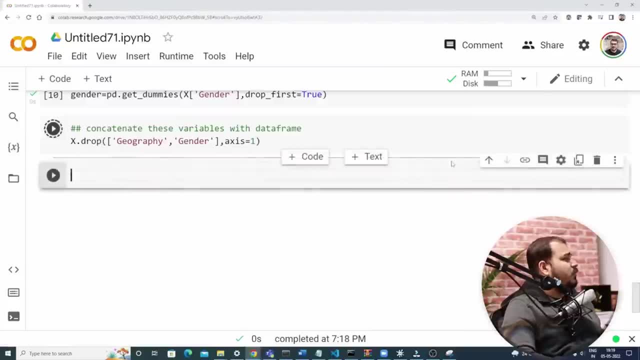 everybody is able to understand till. everybody is able to understand till here, right. so once I execute this, you here, right. so once I execute this, you here, right. so once I execute this, you will be able to see what will happen. so will be able to see what will happen. so. 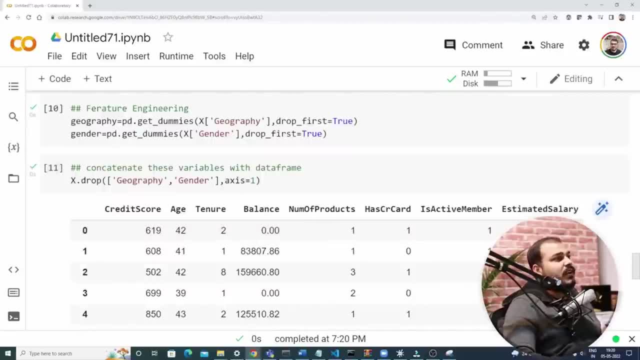 will be able to see what will happen. so this is my value that I'm getting, and this is my value that I'm getting, and this is my value that I'm getting. and now you can see that these two features, now you can see that these two features. 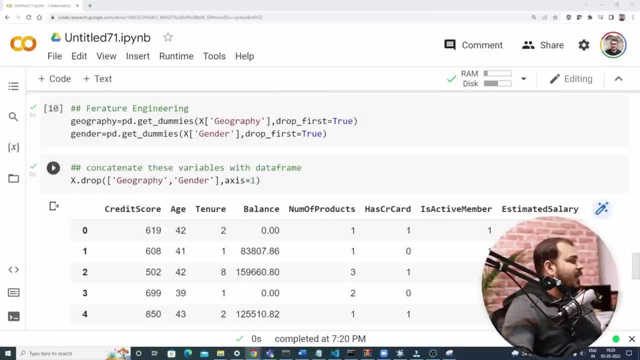 now you can see that these two features are not present. okay, but what I have to are not present. okay, but what I have to are not present. okay, but what I have to do after this is that I have to do after this is that I have to. 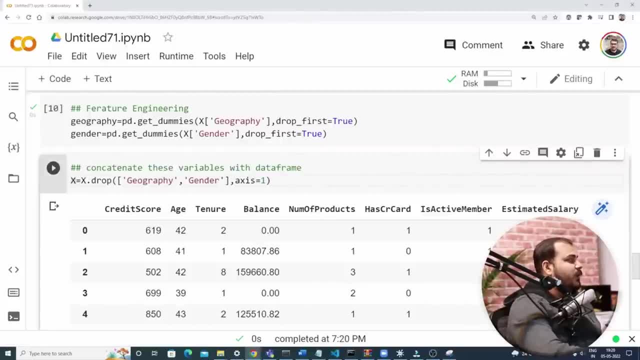 do after this is that I have to basically update my X right right now. X. basically update my X right right now. X. basically update my X right right now. X is not updated, okay, so I'm just going to. is not updated, okay, so I'm just going to. 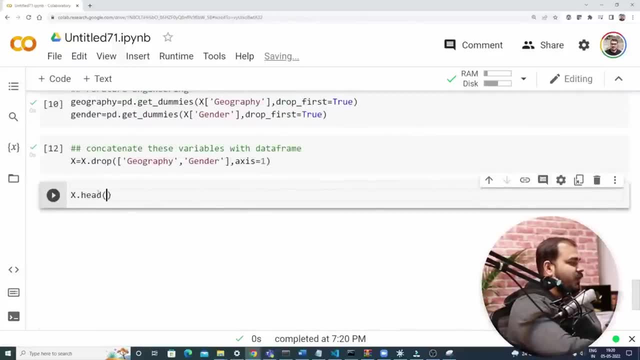 is not updated. okay, so I'm just going to replace this entirely in my X now. if I replace this entirely in my X now, if I replace this entirely in my X now, if I probably go and see X dot head, you'll be. probably go and see X dot head, you'll be. 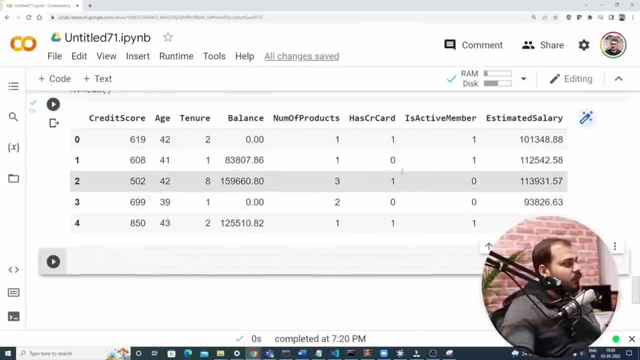 probably go and see X dot head. you'll be able to see that geography and gender. able to see that geography and gender. able to see that geography and gender is not present. okay, geography and gender is not present. okay, geography and gender is not present. okay, geography and gender is not present. so we are able to see. 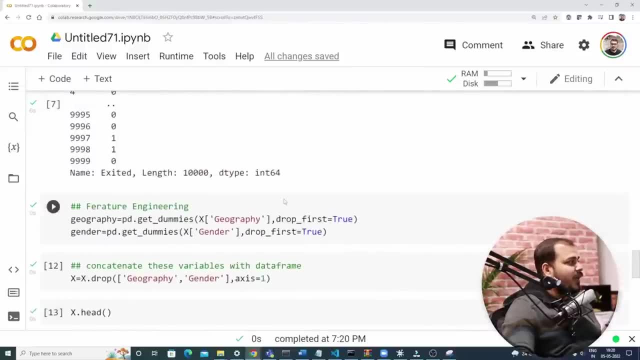 is not present, so we are able to see is not present, so we are able to see that. okay, fine, the category features- we that. okay, fine, the category features- we that, okay, fine, the category features. we have one hot encoded now what we will do. have one hot encoded, now what we will do. 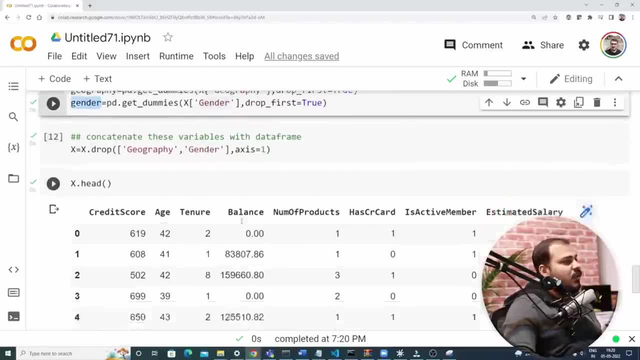 have one hot encoded now, what we will do is that we'll do the concatenation of: is that we'll do the concatenation of, is that we'll do the concatenation of these two variables in this now, these two variables in this now, these two variables in this now, concatenation process is also very much. 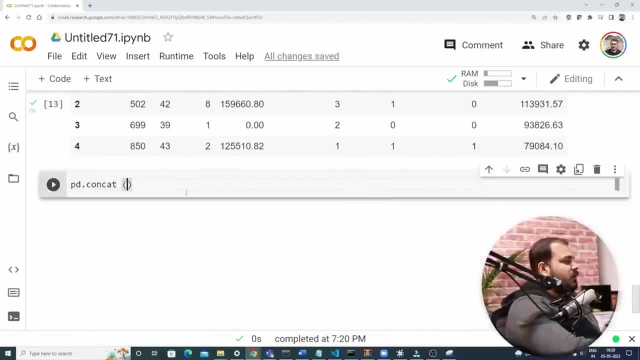 concatenation process is also very much concatenation process is also very much simple. all we have to do is that right simple. all we have to do is that right simple. all we have to do is that right. just PD dot concat, which is a function in, just PD dot concat, which is a function in. 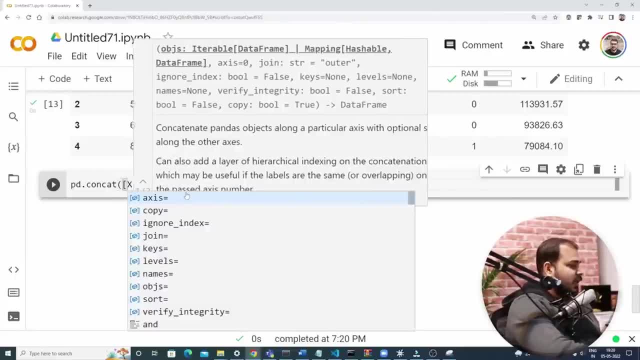 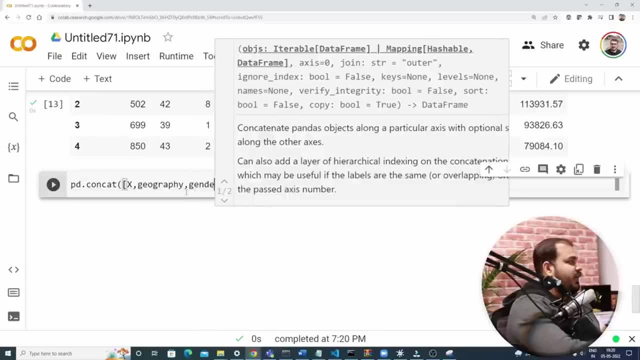 just PD dot concat, which is a function in pandas, and here I'm specifically pandas and here I'm specifically pandas, and here I'm specifically basically saying that X comma geography, basically saying that X comma geography, basically saying that X comma geography, so geography, comma gender, right. so we 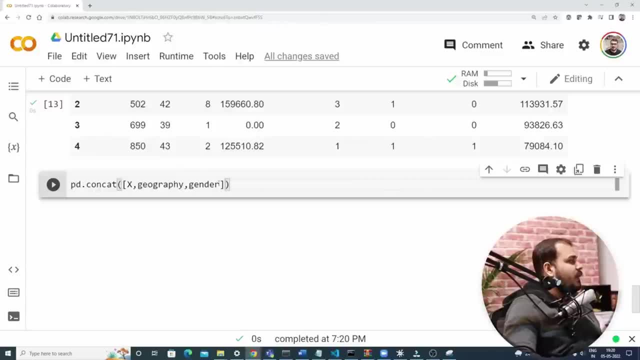 so geography comma, gender right. so we so geography comma, gender right. so we are going to just concatenate this, all are going to just concatenate this, all are going to just concatenate this. all things and this concatenation should things and this concatenation should things and this concatenation should again happen in the column wise right. 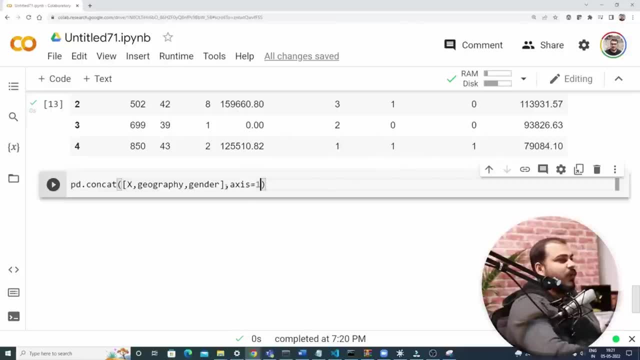 again happen in the column wise right. again happen in the column wise right, not in row wise. so for that I will not in row wise. so for that I will not in row wise. so for that I will basically write: axis is equal to 1, okay, basically write: axis is equal to 1, okay. 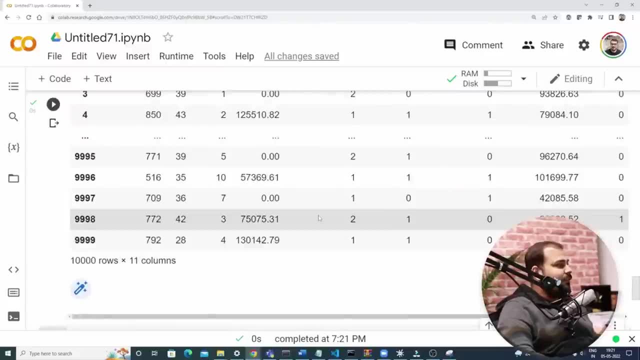 basically write: axis is equal to 1. okay, now, once I execute this here, you will be now. once I execute this here, you will be now. once I execute this here, you will be able to see don't directly replace it for able to see don't directly replace it for. 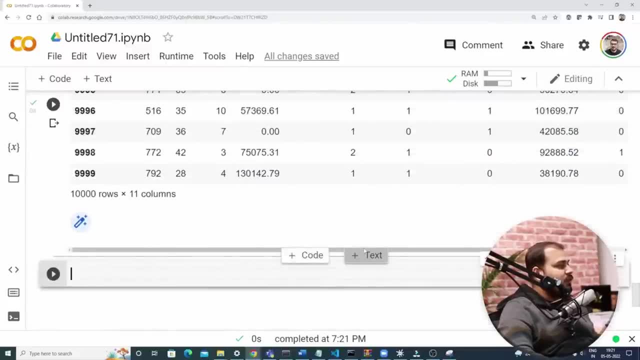 able to see. don't directly replace it for see whether everything is working. see whether everything is working. see whether everything is working properly or not. so if you go and see in properly or not, so if you go and see in properly or not, so if you go and see in the right hand side, here you will be. 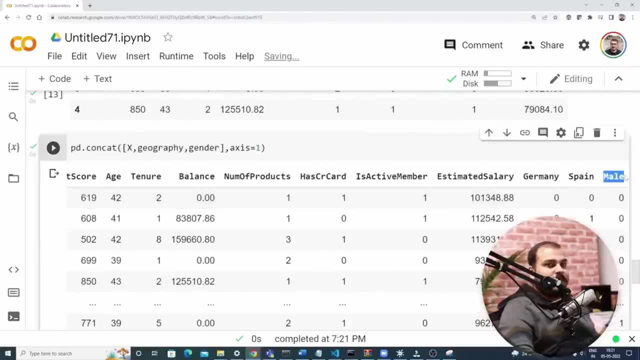 the right hand side here you will be the right hand side here. you will be able to see Germany, Spain and mail has able to see Germany. Spain and mail has able to see Germany. Spain and mail has got added. okay, so one of the column has got added. okay, so one of the column has. 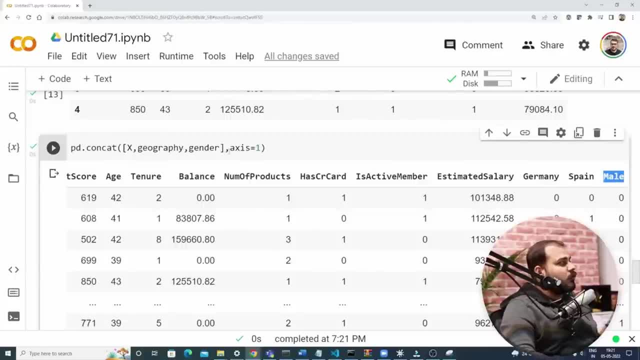 got added. okay, so one of the column has got deleted from here and one of the got deleted from here and one of the got deleted from here, and one of the column has also deleted- got deleted, so column has also deleted. got deleted, so column has also deleted. got deleted. so, in short, why we are doing all these. 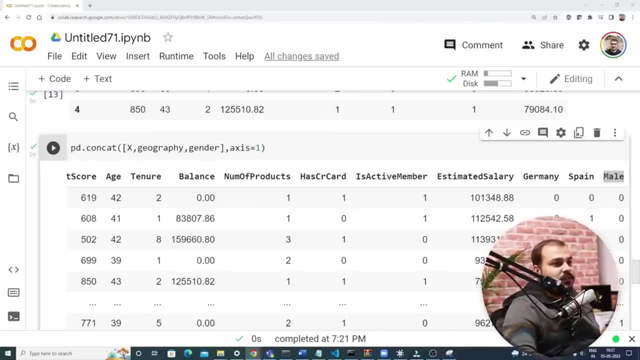 in short, why we are doing all these. in short, why we are doing all these things? because we really need to handle things, because we really need to handle things, because we really need to handle the categorical weight features: okay. the categorical weight features: okay. the categorical weight features: okay. categorical features: we should. 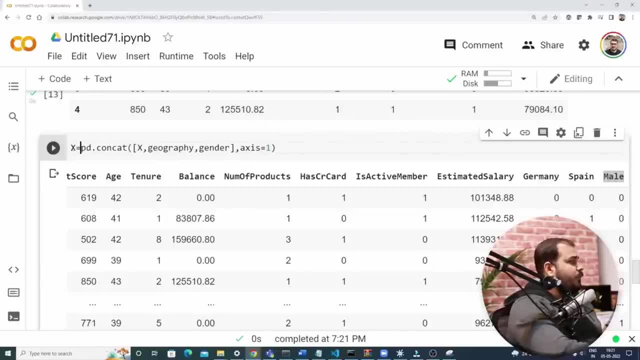 categorical features. we should categorical features. we should definitely handle this. so now I'm just definitely handle this. so now I'm just definitely handle this. so now I'm just going to write X is equal to, and going to write X is equal to, and going to write X is equal to, and probably update this in my X variable. 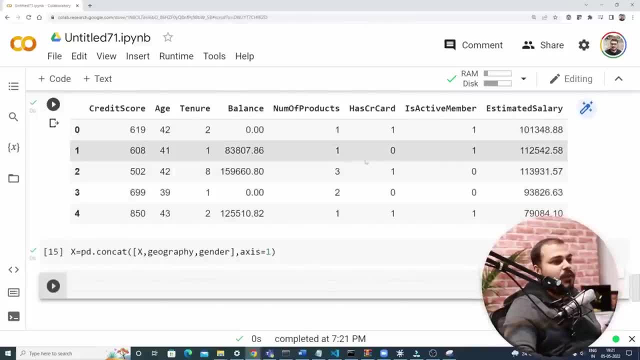 probably update this in my X variable. probably update this in my X variable. perfect, so we have got this and we are perfect. so we have got this and we are perfect. so we have got this and we are able to do till here, which is pretty much able to do till here, which is pretty much. 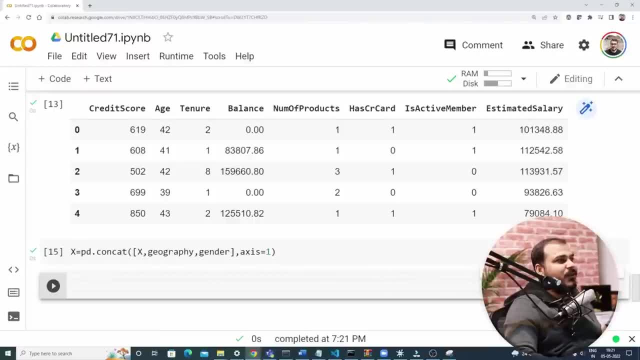 able to do till here, which is pretty much amazing. and now the thing that we amazing, and now the thing that we amazing, and now the thing that we really need to do because we have handle, really need to do because we have handle really need to do because we have handle the category features, we have handled. 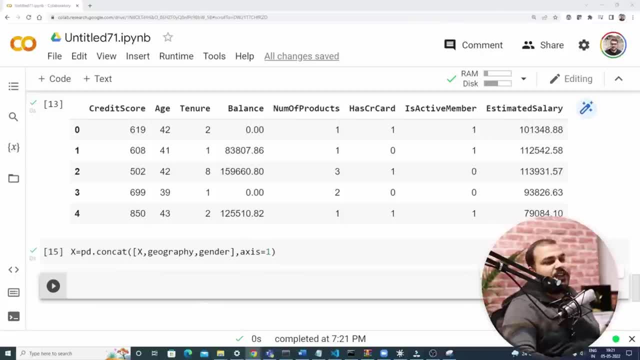 the category features. we have handled the category features. we have handled the other things. now it's time we do a the other things. now it's time we do a the other things. now it's time we do a rain test plate, because train to spit is rain test plate, because train to spit is. 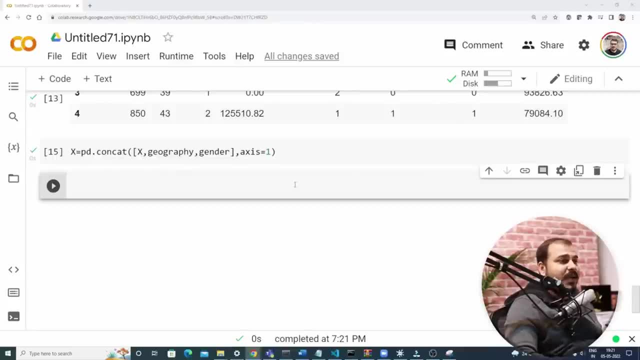 rain test plate, because train to spit is required, because we will be training required, because we will be training required, because we will be training this with the help of a and n right, this with the help of a and n right, this with the help of a and n right artificial neural network. so now, what I 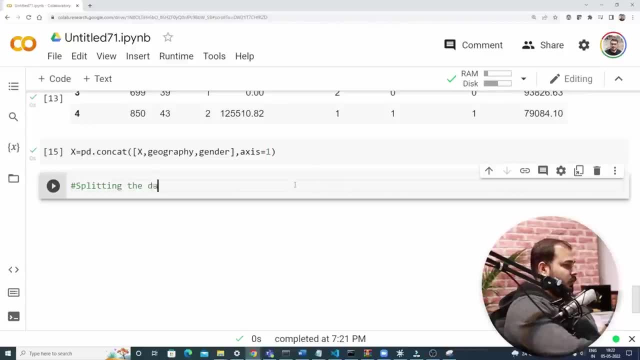 artificial neural network. so now what I artificial neural network. so now what I will do is that I'll say: splitting the will do is that I'll say: splitting the will do is that I'll say: splitting the data set into training set and test set. data set into training set and test set. 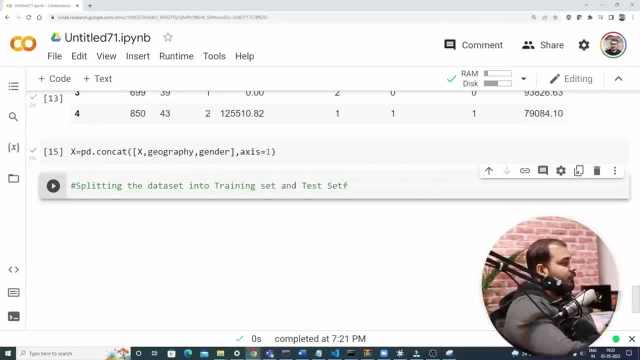 data set into training set and test set. okay, and then I will basically write: okay, and then I will basically write okay, and then I will basically write from a scale on dot model selection and from a scale on dot model selection and from a scale on dot model selection, and then I'm going to import train test. 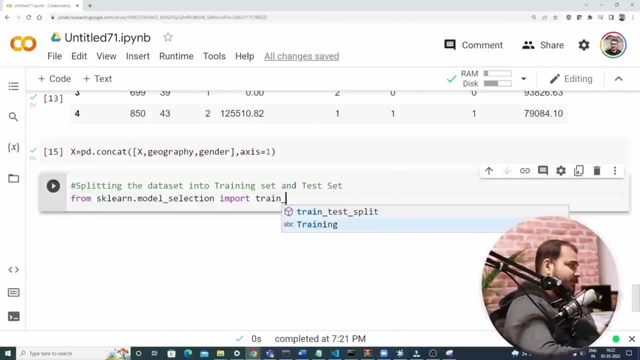 then I'm going to import train test, then I'm going to import train test split. I hope everybody is very much split. I hope everybody is very much split. I hope everybody is very much familiar with this. so train test split. familiar with this. so train test split. 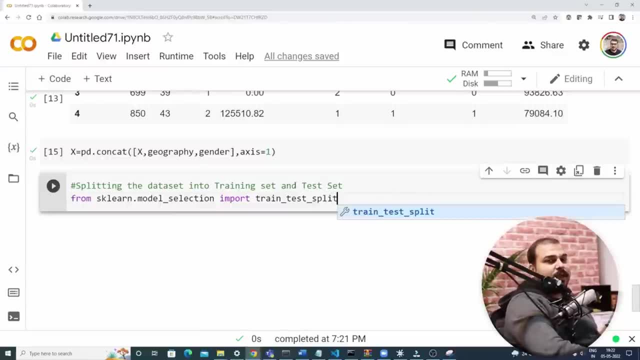 familiar with this. so train test split: okay now with the help of train test. okay now with the help of train test. okay now with the help of train test. plate what all things we can get. we can plate what all things we can get. we can plate what all things we can get we can get, basically, extra nx test, white rain. 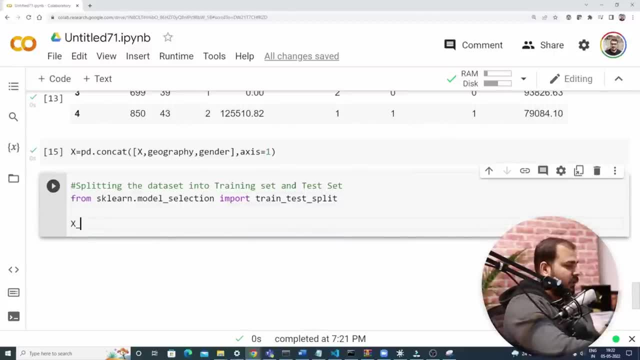 get basically extra nx test, white rain. get basically extra nx test, white rain, white s. so we will just go ahead and white s. so we will just go ahead and white s. so we will just go ahead and write this. I'll say extreme comma X test. write this: I'll say extreme comma X test. 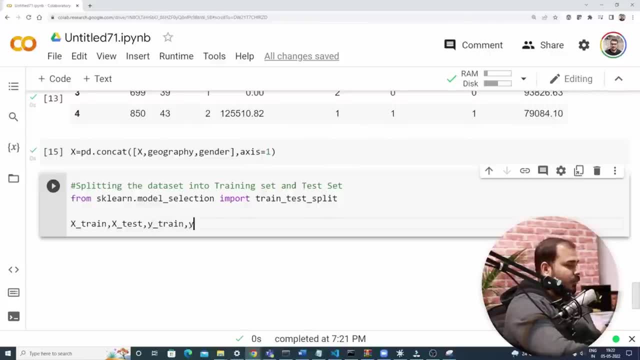 write this. I'll say: extreme comma X test, comma white rain, comma white test and comma white rain, comma white test and comma white rain, comma white test. and here I'm specifically going to use this, here I'm specifically going to use this, here I'm specifically going to use this train test split okay, and then I will be. 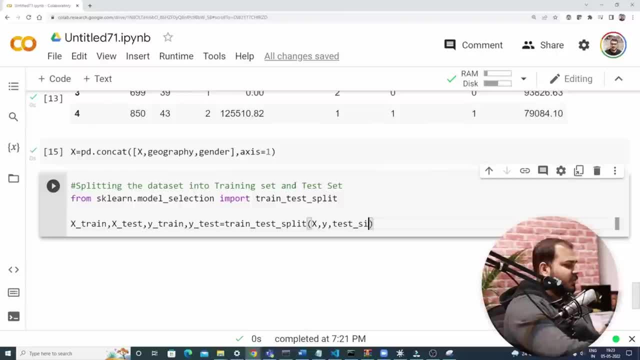 train test split. okay, and then I will be train test split. okay, and then I will be using my X and Y variable. I lets me say using my X and Y variable. I lets me say using my X and Y variable. I lets me say that my test size is just 20%, so I'm 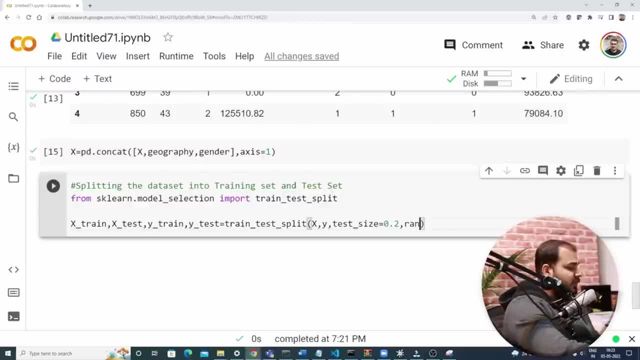 that my test size is just 20%. so I'm that my test size is just 20%, so I'm just going to write 0.2, and then just going to write 0.2, and then just going to write 0.2 and then finally, I'm going to basically say random. 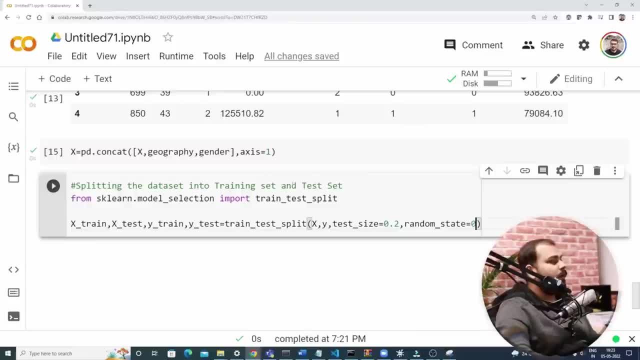 finally, I'm going to basically say random. finally, I'm going to basically say random. underscore state is equal to 0- okay. underscore state is equal to 0- okay, underscore state is equal to 0. okay, so till here, if you probably execute it. so till here, if you probably execute it. 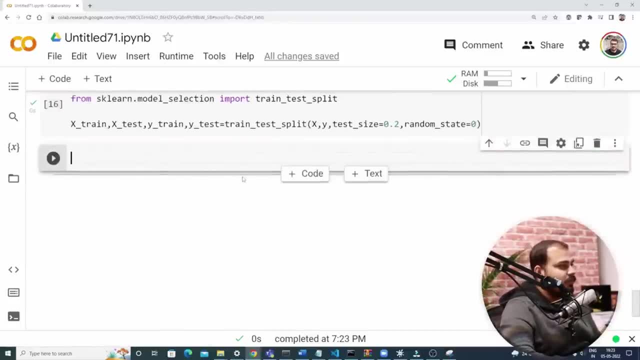 so till here. if you probably execute it now here, you will be able to get your now here. you will be able to get your now here. you will be able to get your train test split, which is perfectly fine. train test split, which is perfectly fine. train test split, which is perfectly fine. now one very important thing, okay one. 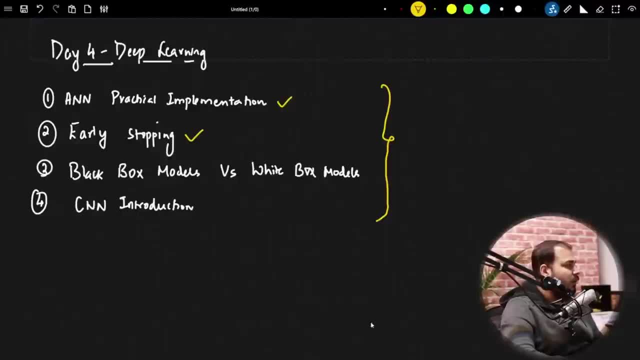 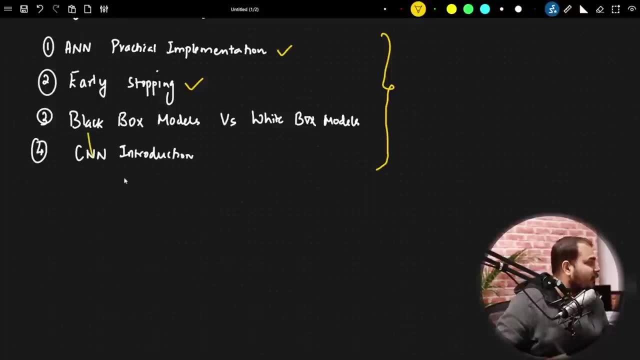 now one very important thing. okay, one now one very important thing. okay, one very, very important thing, which probably very, very important thing, which probably very, very important thing, which probably we have not discussed till now. okay, we have not discussed till now. okay, we have not discussed till now. okay, one thing is that feature scaling. 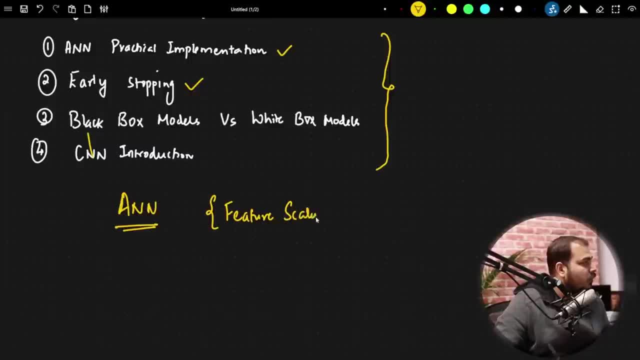 one thing is that feature scaling. one thing is that feature scaling, feature scaling and the main interview: feature scaling and the main interview: feature scaling and the main interview question that you may get right. let's question that you may get right. let's question that you may get right. let's talk about an interview question. they 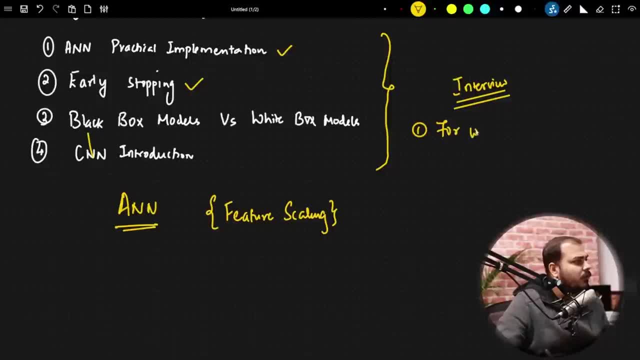 talk about an interview question. they talk about an interview question. they will ask whether features for which all will ask, whether features for which all will ask, whether features for which all machine which all algorithm, let's say machine which all algorithm, let's say machine which all algorithm, let's say for which all algorithms. 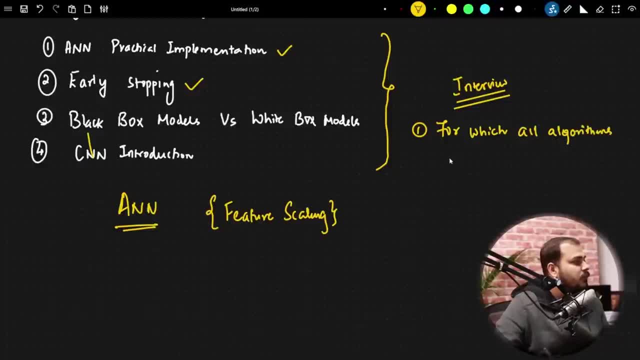 for which all algorithms, for which all algorithms, which all algorithms, which all algorithms feature scaling is which all algorithms feature scaling is which all algorithms feature scaling is required. feature scaling is required. this is a super important interview. this is a super important interview. this is a super important interview question. like many people ask this, I've 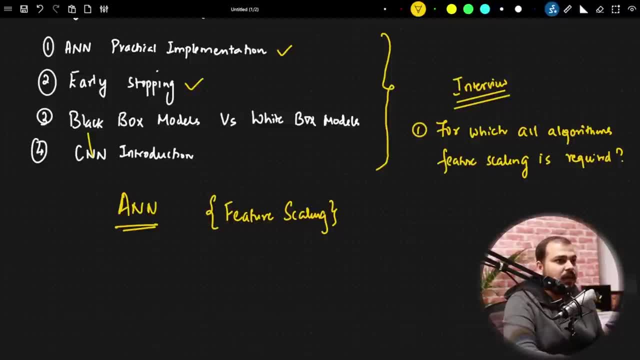 question, like many people ask this. I've question, like many people ask this. I've also seen from the people who have also seen, from the people who have also seen, from the people who have attended interviews: right so, here, you attended interviews. right so, here, you attended interviews. right so here you can basically say that for which? 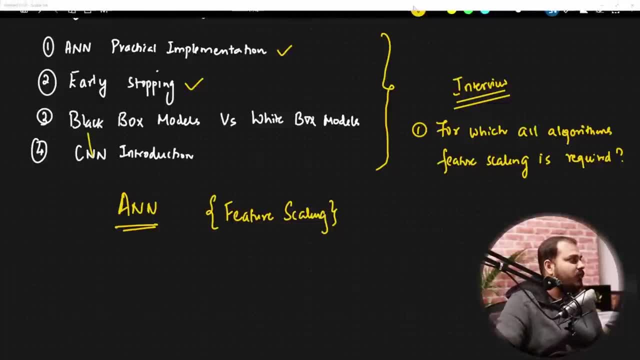 can basically say that, for which? can basically say that for which algorithm feature scaling is required. so algorithm feature scaling is required, so algorithm feature scaling is required. so the next question that probably someone, the next question that probably someone, the next question that probably someone may drop right, whether for ANN is it. 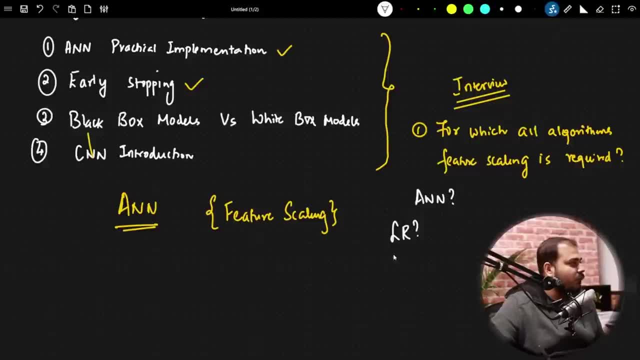 may drop right. whether for ANN is it may drop right. whether for ANN is it required for linear regression. is it required for linear regression? is it required for linear regression? is it required for logistic regression? is it required for logistic regression? is it required for logistic regression? is it required for decision tree? is it? 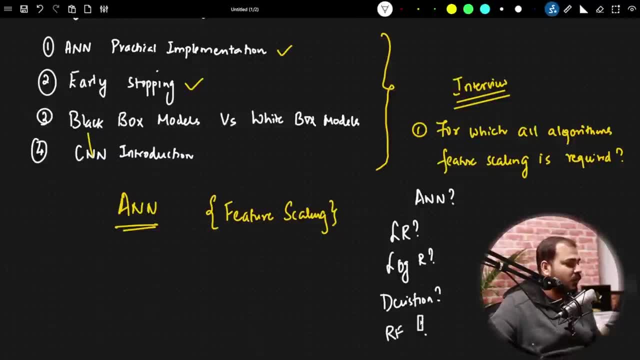 required for decision tree? is it required for decision tree? is it required for random forest? is it required for random forest? is it required for random forest? is it required? so this all kind of questions required, so this, all kind of questions required, so this all kind of questions may come in your mind right for feature. 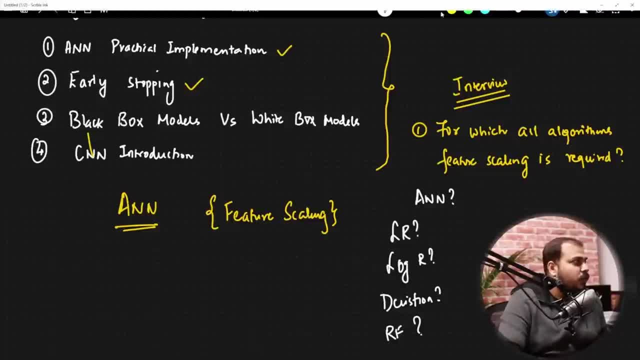 may come in your mind right for feature may come in your mind right for feature. scaling is whether it is required or not. scaling is whether it is required or not. scaling is whether it is required or not. in short, if I really want to talk about, in short, if I really want to talk about, 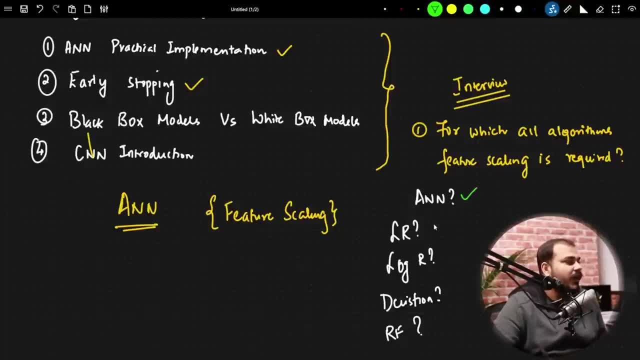 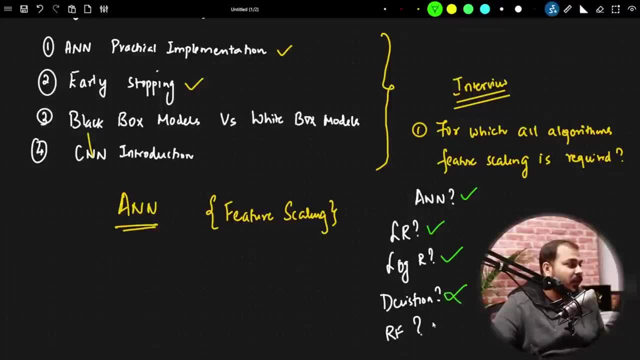 linear regression for logistic. linear regression for logistic regression for decision tree: decision regression for decision tree: decision regression for decision tree: decision tree not necessary. RF random forest, not tree. not necessary. RF random forest, not tree. not necessary. RF random forest not necessary. XG boost not necessary. if I 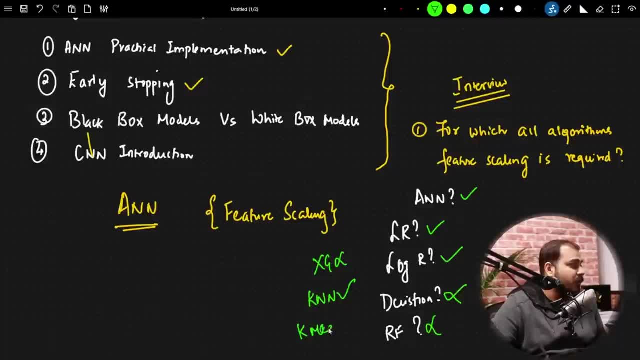 necessary XG boost. not necessary if I necessary XG boost. not necessary if I talk about KNN. yes, it can require for K talk about KNN. yes, it can require for K talk about KNN. yes, it can require, for K means it will be definitely important. 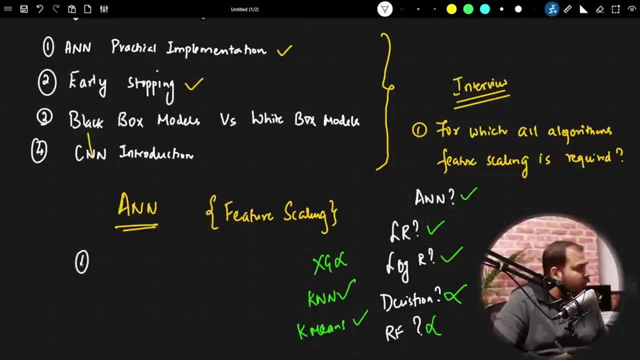 means it will be definitely important, means it will be definitely important where two things are there for which all. where two things are there for which all. where two things are there for which all. algorithm, first of all, anything that is algorithm. first of all anything that is algorithm. first of all, anything that is related to distance based. we really need 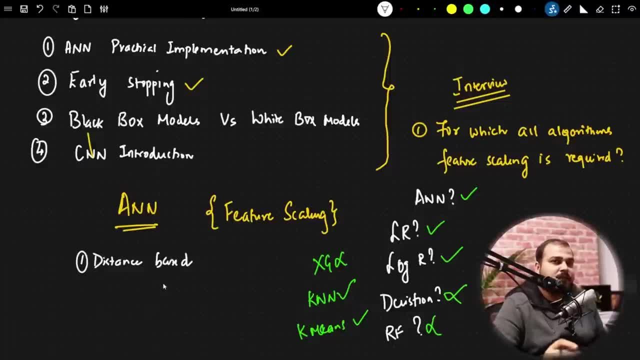 related to distance based. we really need related to distance based, we really need to do feature scaling right. because to do feature scaling right, because to do feature scaling right, because whenever there is some distance based, whenever there is some distance based, whenever there is some distance based problem, you will definitely know that. if 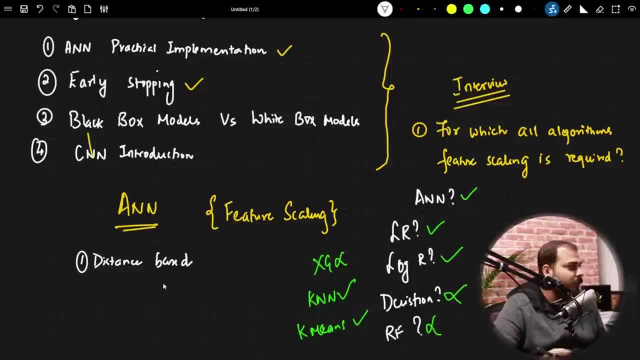 problem, you will definitely know that. if problem, you will definitely know that if the values is bigger, so the calculation, the values is bigger, so the calculation, the values is bigger, so the calculation will definitely take time, right then, the will definitely take time, right then, the will definitely take time, right then. the second thing is that wherever gradient 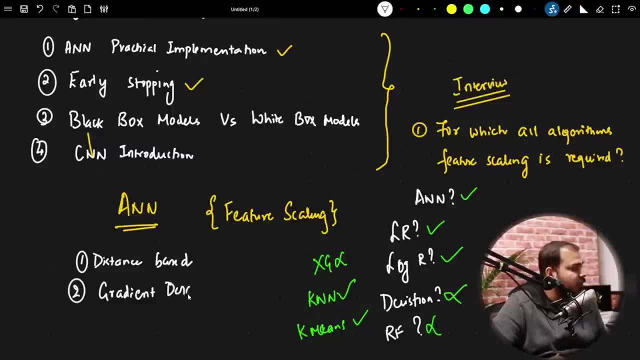 second thing is that wherever gradient- second thing is that wherever gradient descent, or wherever optimizers is descent, or wherever optimizers is descent or wherever optimizers is involved, like gradient descent is involved, like gradient descent is involved, like gradient descent is involved, in linear regression logistic, involved in linear regression logistic. 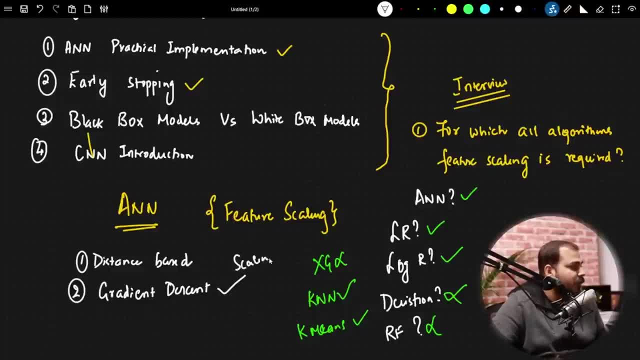 involved in linear regression: logistic regression in this particular case also, regression in this particular case also. regression in this particular case also. scaling will be requiring right, so that scaling will be requiring right, so that scaling will be requiring right, so that our convergence- that usually happens will, our convergence, that usually happens will. 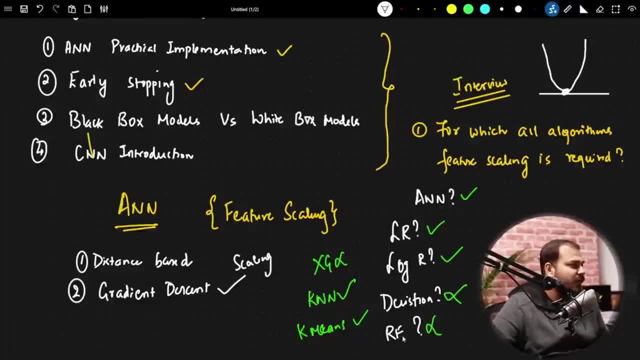 our convergence. that usually happens. will be quicker when compared to the other. be quicker when compared to the other. be quicker when compared to the other things okay, and definitely decision things. okay, and definitely decision things okay and definitely decision trees. does not. does not require XG boost. 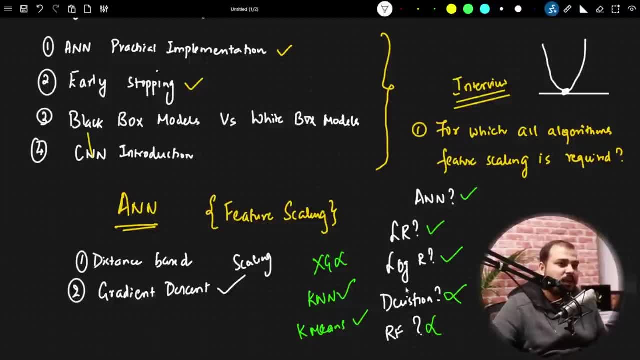 trees does not does not require XG boost. trees does not does not require XG boost, does not require. you know, add our boost does not require. you know, add our boost does not require. you know, add our boost does not require: and all okay, so this does not require and all okay, so this. 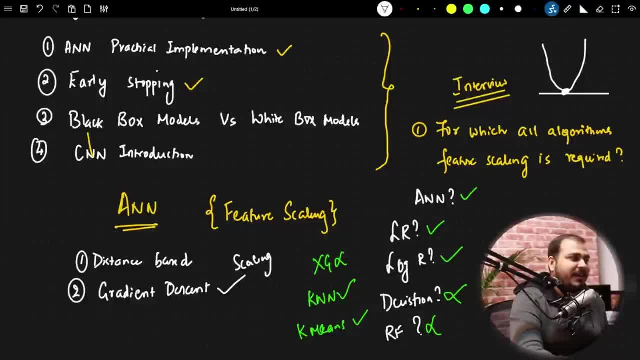 does not require, and all okay. so this specific question, you can actually get specific question. you can actually get specific question. you can actually get it and you'll be later thanking me that it, and you'll be later thanking me that it, and you'll be later thanking me that. Chris, yes, I may probably have got this. 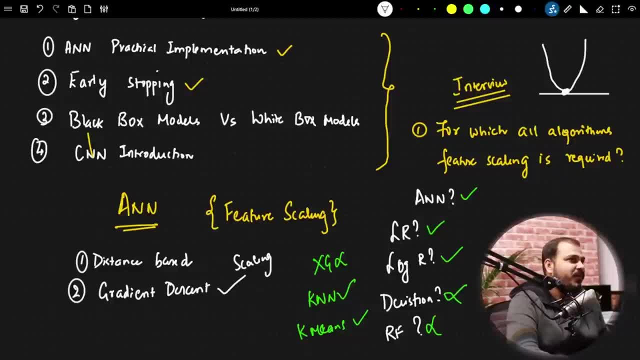 Chris, yes, I may probably have got this, Chris, yes, I may probably have got this question. I hope everybody will be able question. I hope everybody will be able question. I hope everybody will be able to answer. okay, so this is super to answer. okay, so this is super. 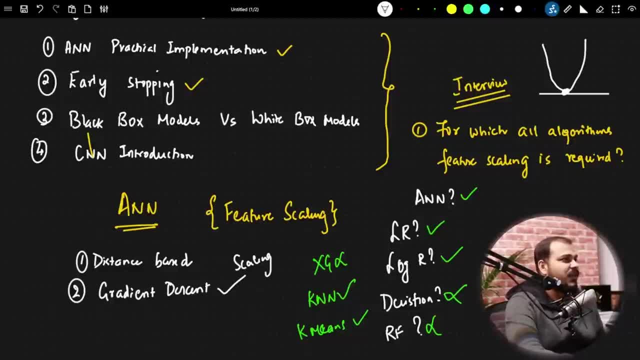 to answer. okay, so this is super important. now let's go to the next thing important. now let's go to the next thing important. now let's go to the next thing. let's, let's continue the coding part. let's, let's continue the coding part. let's, let's continue the coding part. right? so what I am actually going to do? right, so what I am actually going to do, right, so what I am actually going to do now. let's go to the coding part now. we now. let's go to the coding part now. we now. let's go to the coding part now. we have done the train test split. now we. 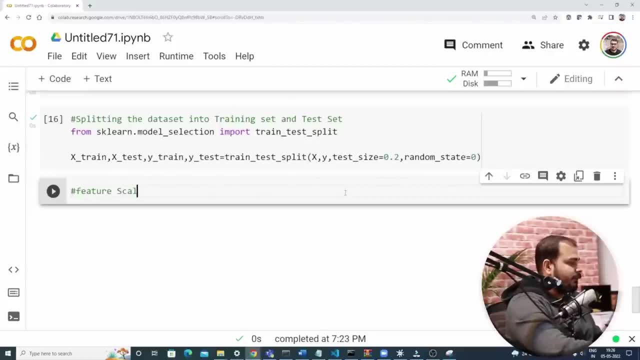 have done the train test split. now we have done the train test split, now we really need to do something called as, really need to do something called as. really need to do something called as feature scaling. okay, now feature scaling. feature scaling- okay, now feature scaling. feature scaling- okay, now feature scaling. I will just say: from SK, learn dot. 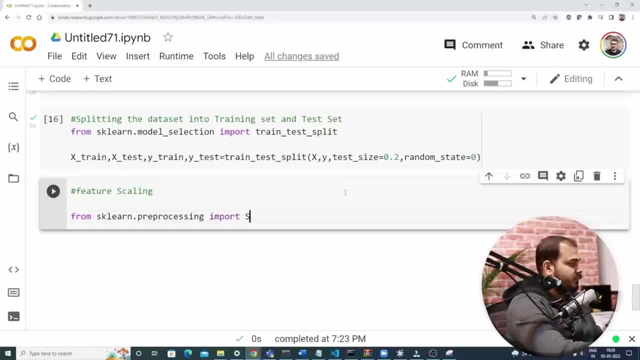 I will just say: from SK, learn dot. I will just say: from SK, learn dot reprocessing. and I'm going to import reprocessing and I'm going to import reprocessing and I'm going to import standard scalar. now there may be standard scalar, now there may be. 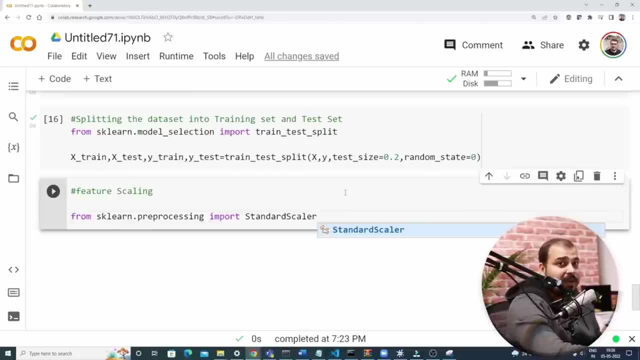 standard scalar. now there may be scenarios where you may be asking Chris, scenarios where you may be asking Chris, scenarios where you may be asking Chris: why standard scalar only, why not min? why standard scalar only, why not min? why standard scalar only? why not min max scalar? see min max scalar. also, you can 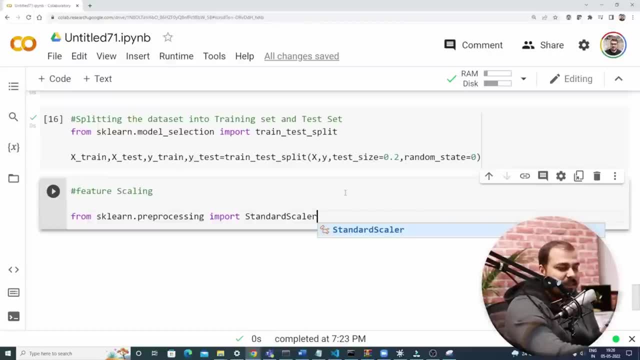 max scalar- see min max scalar also. you can max scalar- see min max scalar also. you can definitely apply. but that will get definitely apply. but that will get definitely apply. but that will get applied to CNN tomorrow. we'll be applied to CNN tomorrow. we'll be applied to CNN tomorrow. we'll be discussing about that today. I'll just 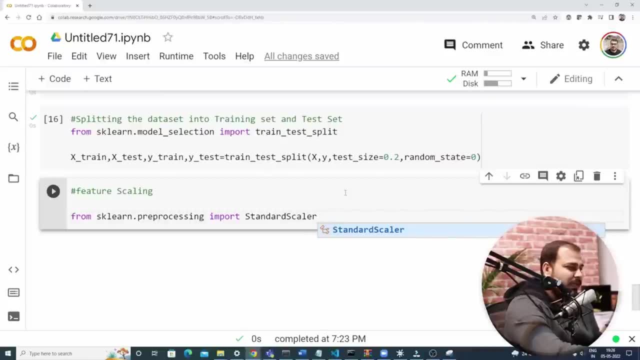 discussing about that today. I'll just discussing about that today. I'll just give you a brief introduction, but mostly give you a brief introduction, but mostly give you a brief introduction, but mostly min max scalar, anything that you want to min max scalar, anything that you want to. 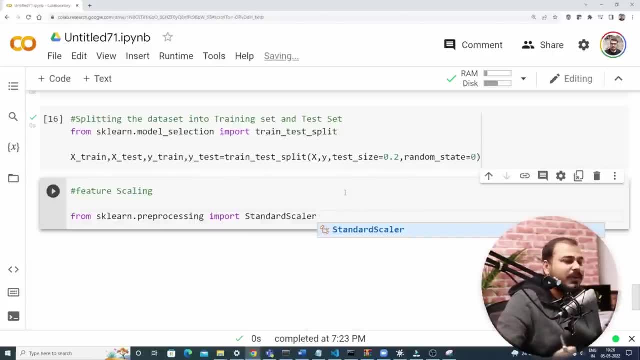 give you a brief introduction, but mostly min, max, scalar, anything that you want to restrict between 0 to 1 or minus 1, to restrict between 0 to 1 or minus 1, to restrict between 0 to 1 or minus 1 to plus 1, and all right, you should. 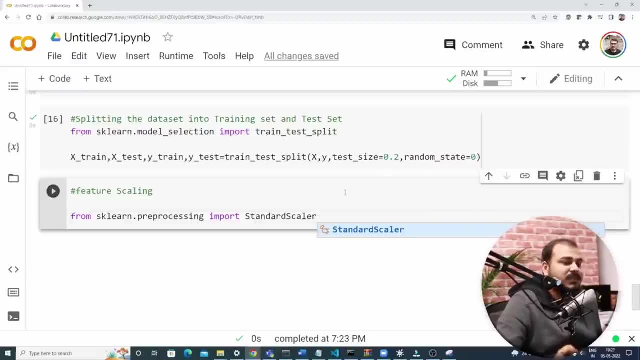 plus 1 and all right, you should plus 1 and all right, you should definitely try it with respect to CNN. definitely try it with respect to CNN. definitely try it with respect to CNN. standard scalar basically means based on standard scalar, basically means based on standard scalar, basically means based on that Z score that you have probably seen. 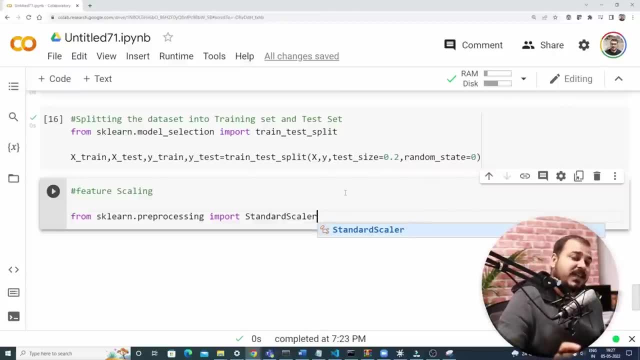 that Z score, that you have probably seen that Z score, that you have probably seen those formulas where I have specifically those formulas, where I have specifically those formulas where I have specifically spoken about in my statistics lessons or spoken about in my statistics lessons or spoken about in my statistics lessons or machine learning lessons. right, so there. 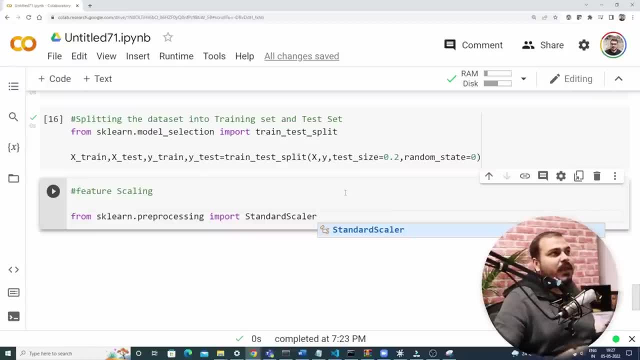 machine learning lessons. right. so there, machine learning lessons, right. so there, we should definitely go ahead and use. we should definitely go ahead and use, we should definitely go ahead and use standard scalar and this way you know standard scalar and this way you know standard scalar and this way you know, suppose, if your data is normalized, you, 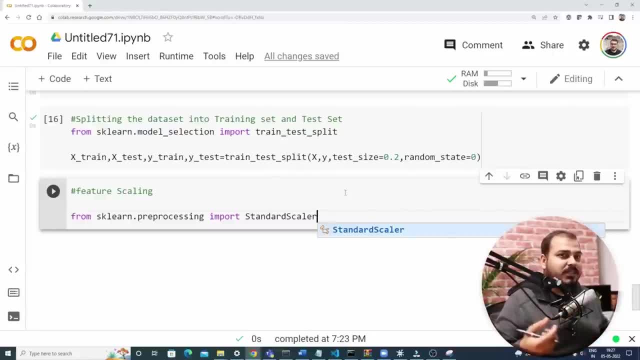 suppose, if your data is normalized. you suppose if your data is normalized, you know it basically rotates around your know. it basically rotates around your know it basically rotates around your mean value with some standard deviation, mean value with some standard deviation, mean value with some standard deviation to the right and the left. okay, so that. 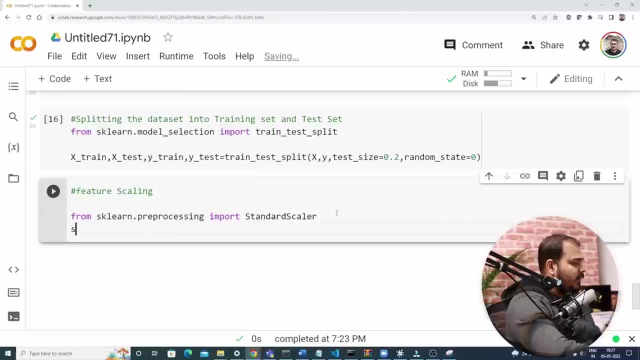 to the right and the left. okay, so that to the right and the left, okay. so that is the reason why we specifically use. is the reason why we specifically use, is the reason why we specifically use standard scalar, and here I'm going to standard scalar, and here I'm going to. 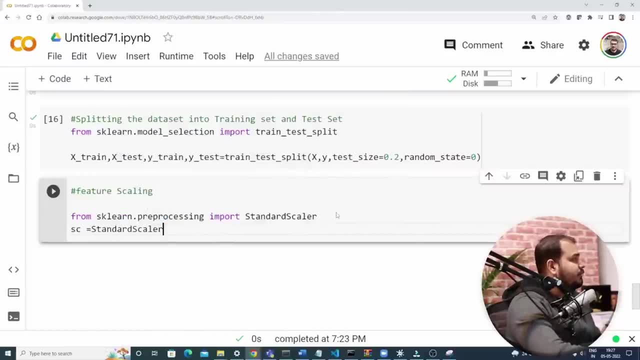 standard scalar. and here I'm going to initialize: SC is equal to standard. initialize SC is equal to standard initialize SC is equal to standard scalar. okay, I'm just going to initialize scalar. okay, I'm just going to initialize scalar. okay, I'm just going to initialize it and finally you'll be able to see. I'm 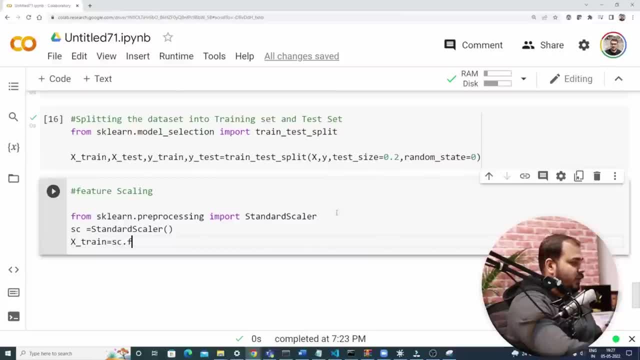 it and finally you'll be able to see I'm it and finally you'll be able to see I'm using extra in, where I'll specifically using extra in, where I'll specifically using extra in, where I'll specifically say SC dot fit underscore transform okay. say SC dot fit underscore transform okay. 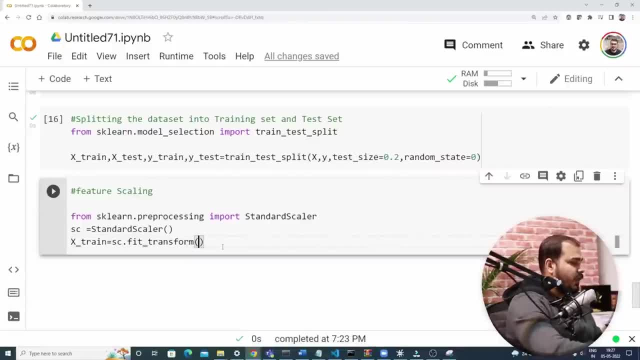 say: SC dot fit underscore transform. okay, fit underscore transform. and here I'm fit underscore transform. and here I'm fit underscore transform. and here I'm going to give my extra main value. okay, going to give my extra main value. okay, going to give my extra main value. okay, and always understand what is the. 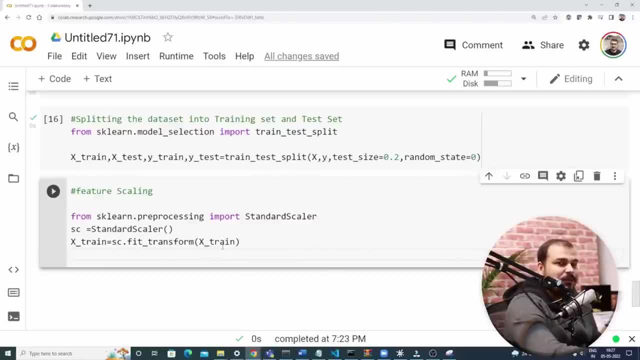 and always understand what is the and always understand what is the difference between fit underscore, difference between fit underscore, difference between fit underscore, transform and transform. I've also made a transform and transform. I've also made a transform and transform. I've also made a detailed video about it. but if any, 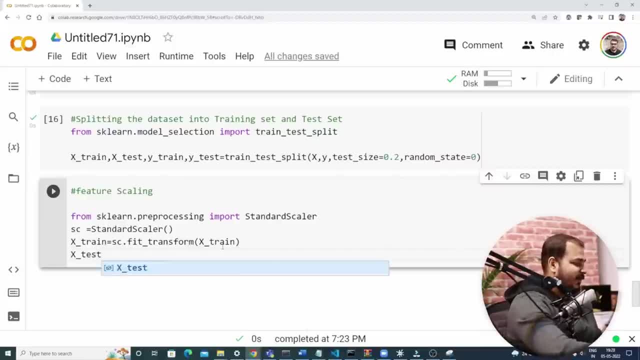 detailed video about it. but if any detailed video about it, but if any, would anybody would like to comment down? would anybody would like to comment down? would anybody would like to comment down in the comment section? you can let me in the comment section. you can let me. 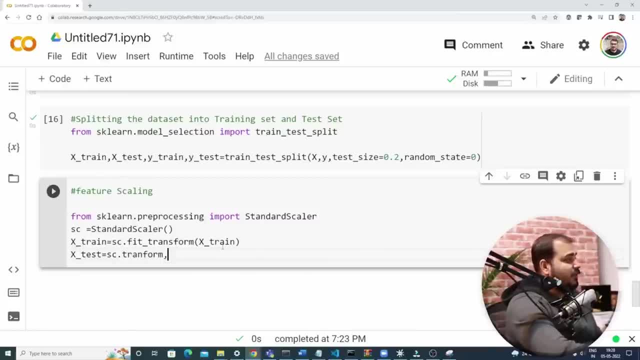 in the comment section you can let me know. okay, so SC dot transform. so this know. okay, so SC dot transform. so this know. okay, so SC dot transform. so this can also be an interview question like: can also be an interview question like can also be an interview question like: why do we apply fit underscore transform? 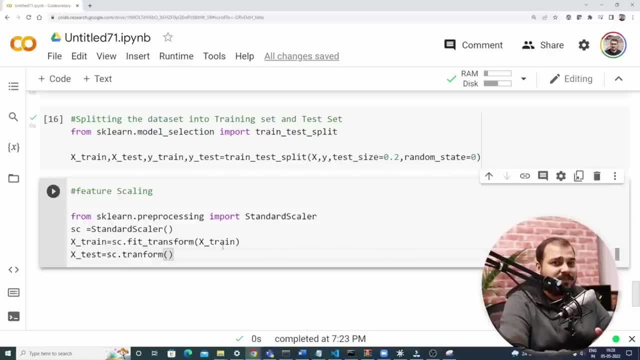 why do we apply fit underscore transform? why do we apply fit underscore transform only to the training data set, not to the only to the training data set, not to the only to the training data set, not to the test data set. you know so this kind of test data set. you know so this kind of? 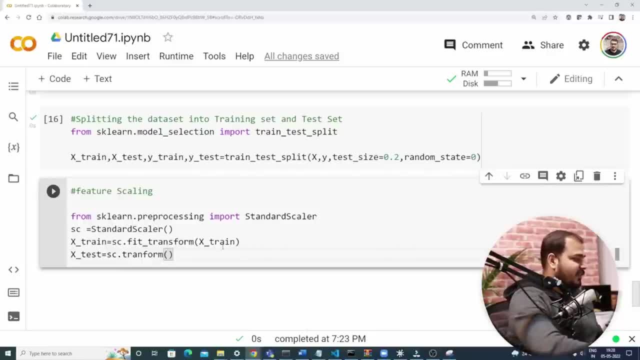 test data set, you know. so this kind of questions may also definitely come to questions, may also definitely come to questions, may also definitely come to you, so be prepared. I've always given you you, so be prepared. I've always given you you, so be prepared. I've always given you all the hints that you want, okay, so. 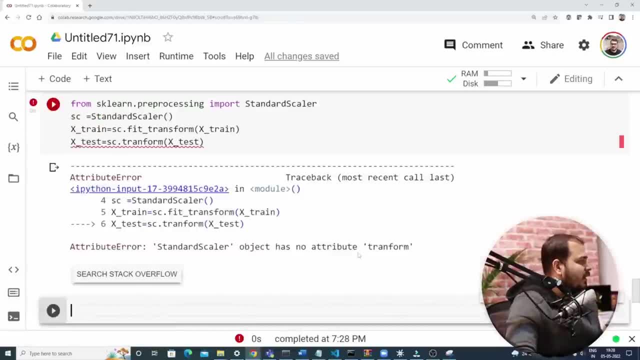 all the hints that you want: okay. so, all the hints that you want, okay. so here it is. we will try to execute it. here it is. we will try to execute it. here it is. we will try to execute it. okay. transform. okay. find there is an. okay, transform, okay, find there is an. 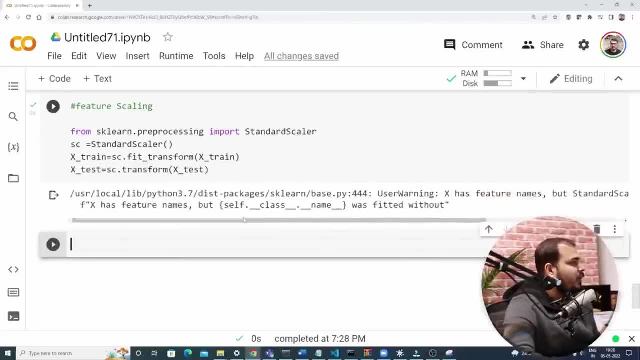 okay, transform. okay, find there is an error, will try to execute it. so now if error, will try to execute it. so now if error will try to execute it. so now, if you probably X has feature names, but you probably X has feature names, but you probably X has feature names but standard, say, was fitted without feature. 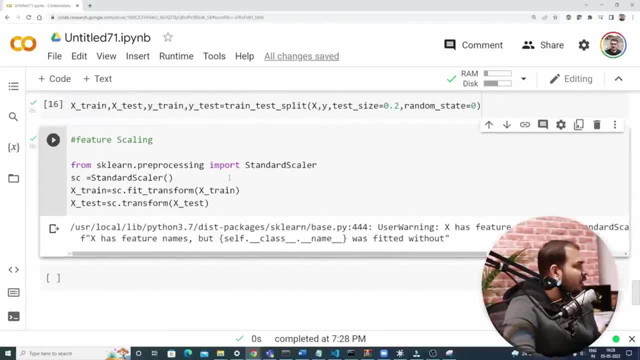 standard say was fitted without feature. standard say was fitted without feature name. okay, let's see what things X train name. okay, let's see what things X train name. okay, let's see what things X train for. I think it is fine. this is a for. I think it is fine, this is a. 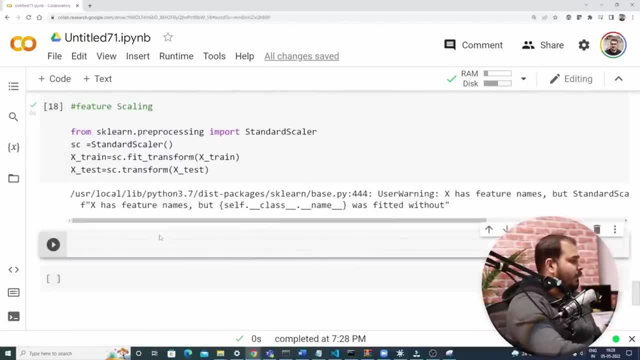 for I think it is fine, this is a warning. I guess so if I go and probably warning, I guess so if I go and probably warning. I guess so if I go and probably see my X underscore plane, and if I see my X underscore plane and if I 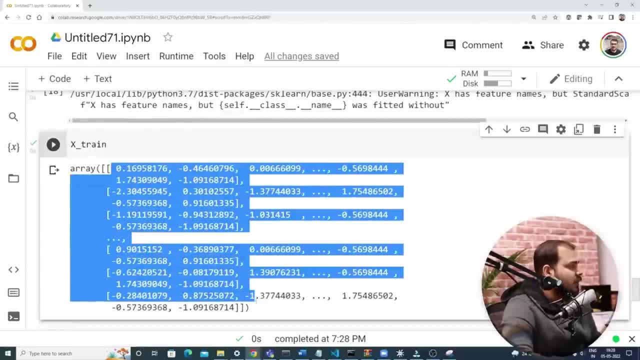 see my X underscore plane and if I execute it, you will be able to see that. execute it. you will be able to see that. execute it, you will be able to see that my data has got transformed okay and my data has got transformed okay and my data has got transformed okay. and similarly, if I go and probably see X, 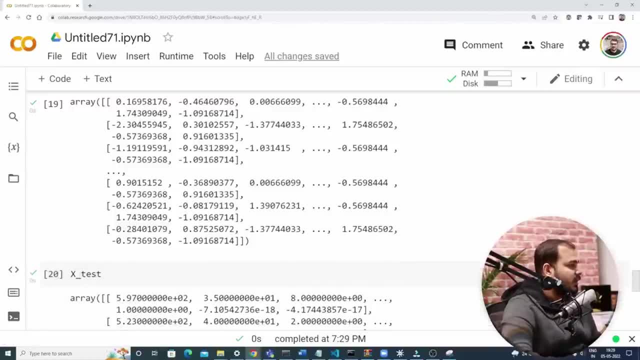 similarly, if I go and probably see X. similarly, if I go and probably see X, underscore test here also, you'll be able underscore test here also. you'll be able underscore test here also. you'll be able to see my data has got transformed. to see my data has got transformed. 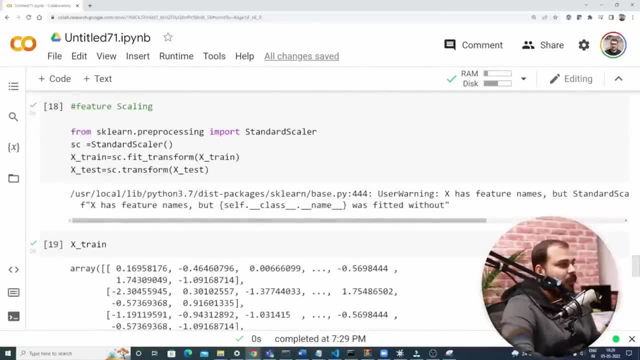 to see my data has got transformed perfect. so train and test has got perfect. so train and test has got perfect. so train and test has got transformed completely, which is quite transformed completely, which is quite transformed completely, which is quite amazing. and now, if you probably also amazing, and now, if you probably also, 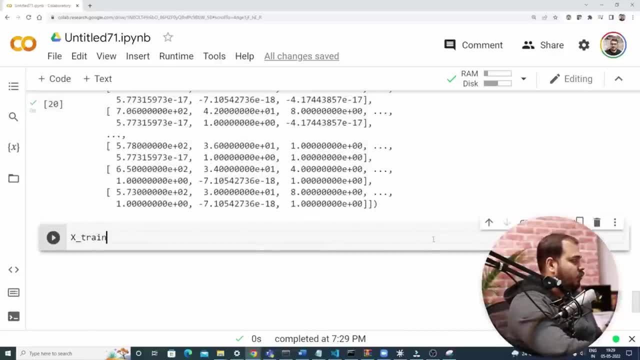 amazing. and now, if you probably also check out the shape of the train right X, check out the shape of the train right X. check out the shape of the train right X: underscore train dot ship. so right now, underscore train dot ship. so right now, underscore train dot ship. so right now you're still in feature engineering it. 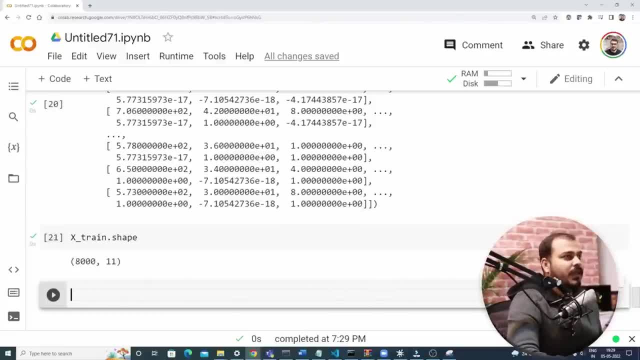 you're still in feature engineering. it you're still in feature engineering. it is not like an ANN you don't require, is not like an ANN you don't require, is not like an ANN. you don't require feature engineering because ANN problem, feature engineering because ANN problem. 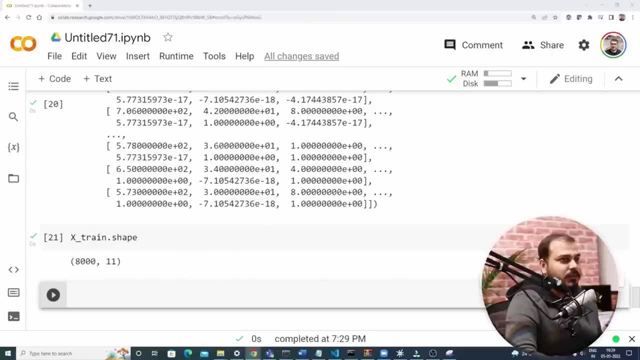 feature engineering, because ANN problem can also be solved with the help of, can also be solved with the help of, can also be solved with the help of machine learning right. so that is the machine learning right, so that is the machine learning right, so that is the reason. okay, an end problem can also be. 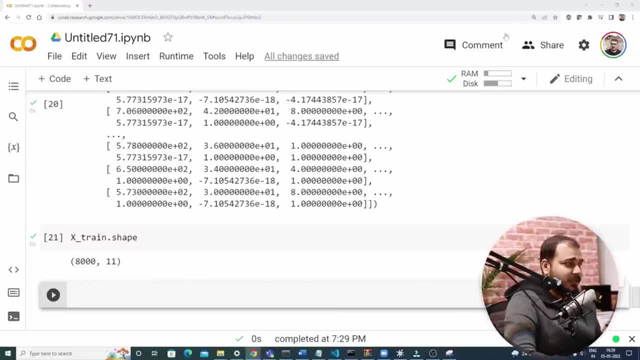 reason. okay, an end problem can also be reason. okay, an end problem can also be sure solved by machine learning part. sure, solved by machine learning part. sure solved by machine learning part also okay, yes, one amazing answers that I also okay. yes, one amazing answers that I also okay. yes, one amazing answers that I can tell you that. why fit underscore? 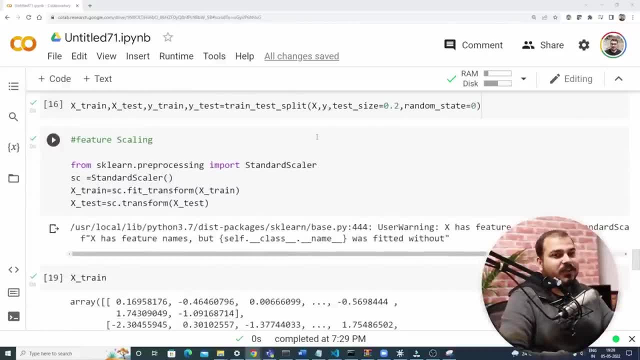 can tell you that? why fit underscore. can tell you that? why fit underscore? transform and transform is used only for transform, and transform is used only for transform, and transform is used only for test data. because of data leakage: okay, test data because of data leakage: okay, test data because of data leakage: okay, avoid data leakage. data leakage, video. 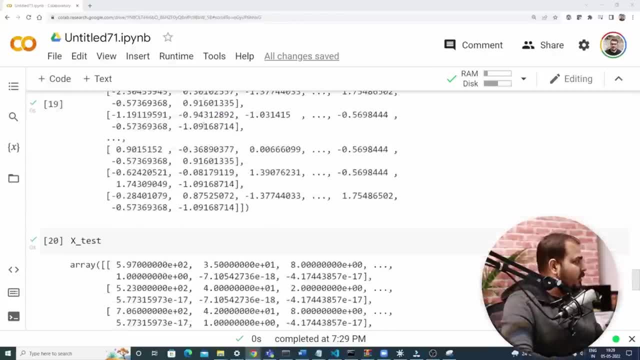 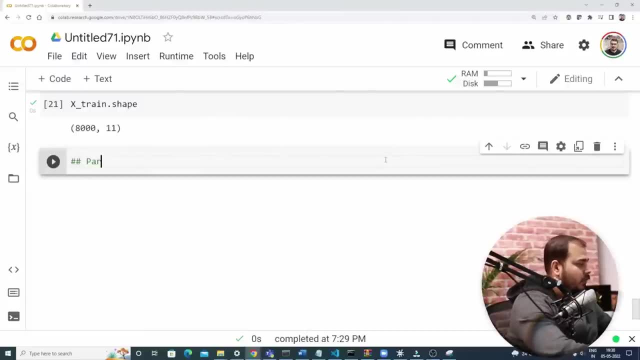 avoid data leakage. data leakage video. avoid data leakage. data leakage video. I've created in a detailed way. okay, I've created in a detailed way. okay, I've created in a detailed way. okay, then, definitely check it out. okay, then, definitely check it out. okay, then definitely check it out. okay, perfect. now the part 2. part 2: here we 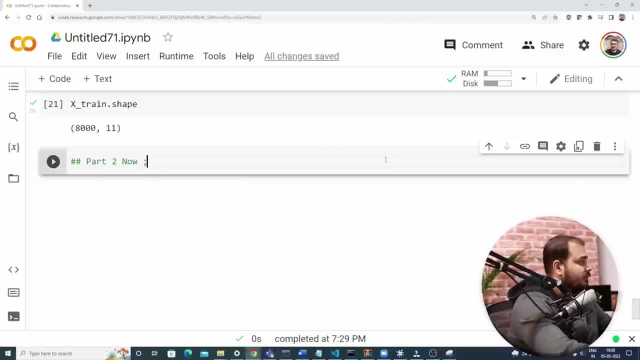 perfect now the part 2, part 2. here we perfect now the part 2, part 2. here we are going to create now let's let's are going to create, now let's let's are going to create. now let's let's create the ANN, the artificial neural. 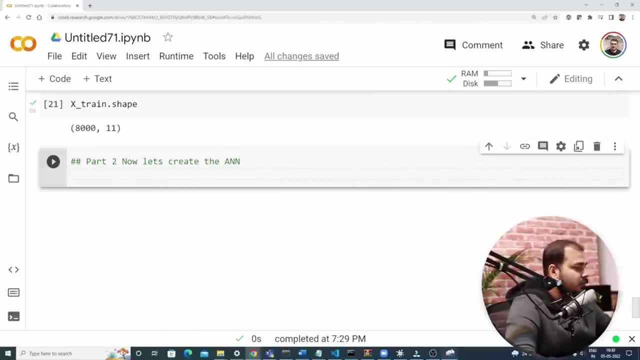 create the ANN, the artificial neural. create the ANN, the artificial neural network, now, before this. you need to network now, before this. you need to network now, before this. you need to understand what is tensorflow, what is understand what is tensorflow, what is understand what is tensorflow, what is Keras? okay here, whenever we talk about 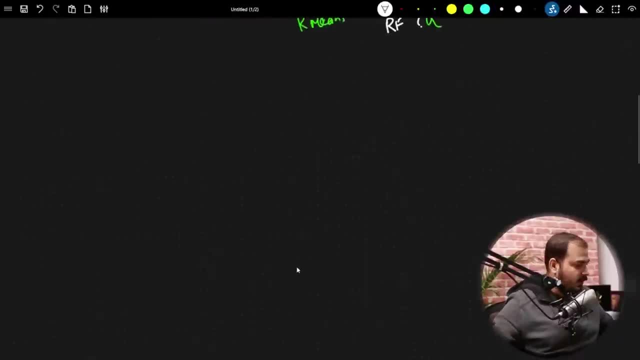 Keras. okay here whenever we talk about Keras. okay here whenever we talk about this. the library that we are going to this, the library that we are going to this, the library that we are going to use, is basically tensorflow right. use is basically tensorflow right. use is basically tensorflow right- tensorflow. a popular library. this was. 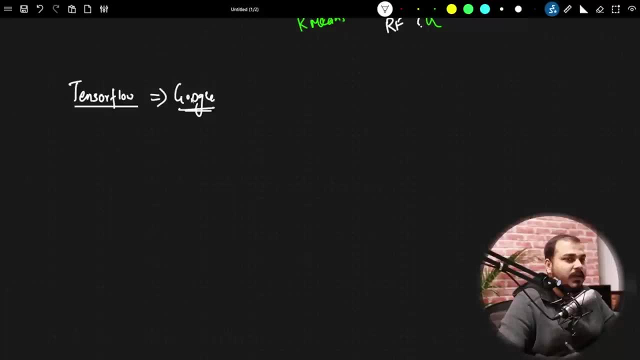 tensorflow, a popular library. this was tensorflow, a popular library. this was open sourced by Google. okay, Google deep open sourced by Google. okay, Google deep open sourced by Google. okay, Google deep. minds is a minds is a minds is a team. who have actually created this? okay, team who have actually created this? okay. 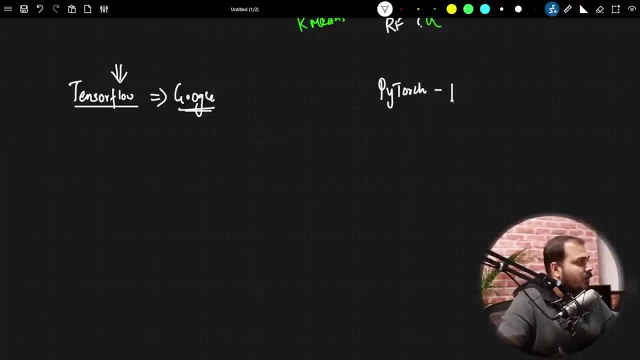 team who have actually created this. okay. and again, you know about PyTorch also. and again, you know about PyTorch also. and again, you know about PyTorch also: PyTorch is from Facebook overall- same. PyTorch is from Facebook overall- same. PyTorch is from Facebook overall- same things. you can do with both of them, okay. 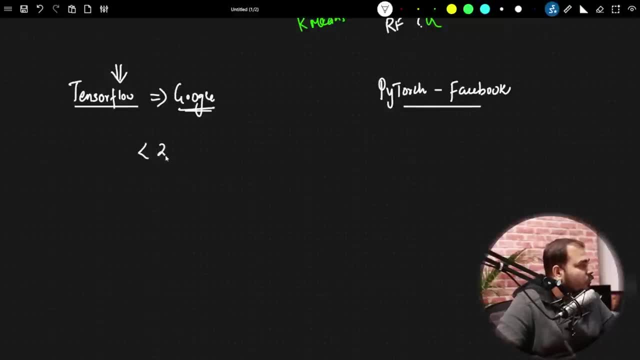 things you can do with both of them: okay, things you can do with both of them. okay, now initially, when before tensorflow 2.0. now, initially, when before tensorflow 2.0. now initially, when before tensorflow 2.0: okay, tensorflow was separate. okay, tensorflow was separate. 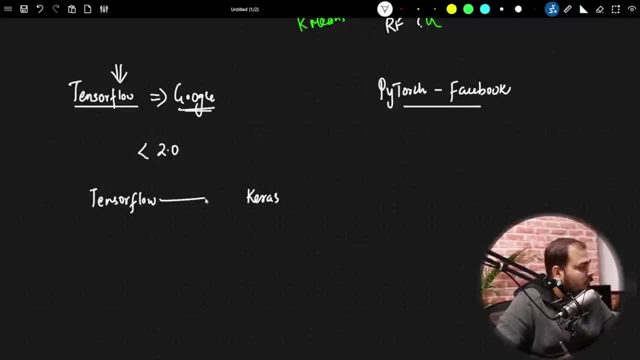 okay, tensorflow was separate. Keras is a wrapper- okay. so if you talk, Keras is a wrapper, okay. so if you talk, Keras is a wrapper, okay. so if you talk about tensorflow, Keras is basically a about tensorflow. Keras is basically a about tensorflow. Keras is basically a wrapper. wrapper basically means it uses. 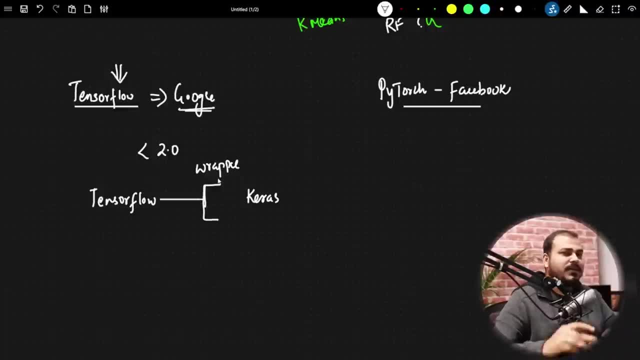 wrapper wrapper basically means it uses wrapper wrapper basically means it uses. this tensorflow API is only but over. this tensorflow API is only but over. this tensorflow API is only but over here you will find a simple function. you, here, you will find a simple function. you, here, you will find a simple function. you can just call the function and you can. 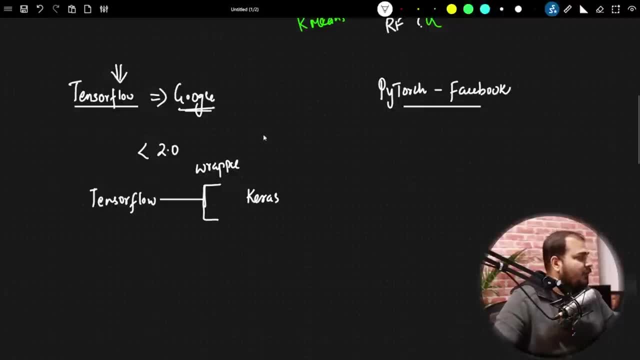 can just call the function and you can can just call the function and you can basically use the tensorflow in depth. basically use the tensorflow in depth. basically use the tensorflow in depth. inside this: okay, so after 2.0: greater. inside this: okay, so after 2.0: greater. 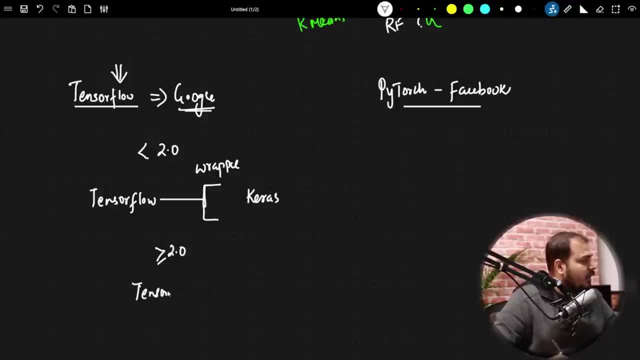 inside this. okay, so, after 2.0, greater than 2.0, what happened Keras and than 2.0? what happened Keras and than 2.0? what happened Keras? and basically in use again. it is a wrapper. basically in use- again, it is a wrapper. 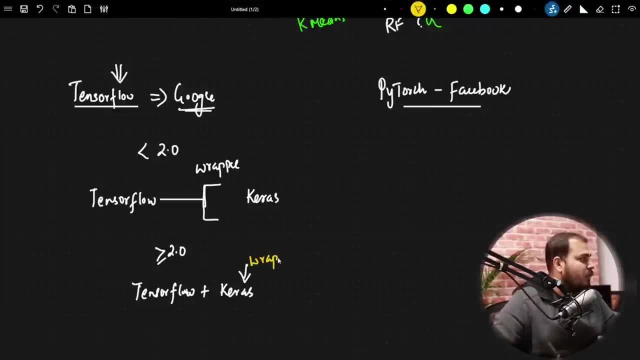 basically in use. again, it is a wrapper. obviously this Keras is a wrapper over. obviously this Keras is a wrapper over. obviously this Keras is a wrapper over here. okay, and you can actually use here. okay, and you can actually use here. okay, and you can actually use tensorflow in a much more better way. 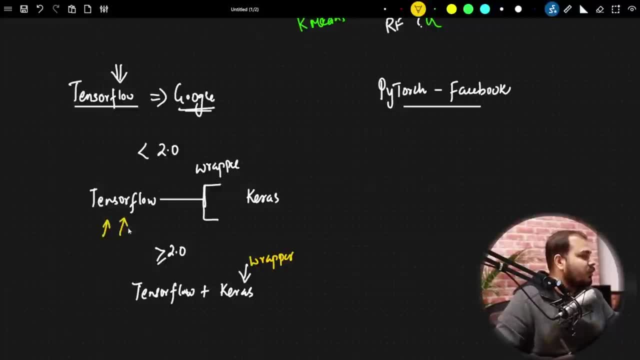 tensorflow in a much more better way. tensorflow in a much more better way before the installation used to be, before the installation used to be, before the installation used to be working like this first of all. we need working like this first of all. we need working like this: first of all, we need to install tensorflow, and separately, we. 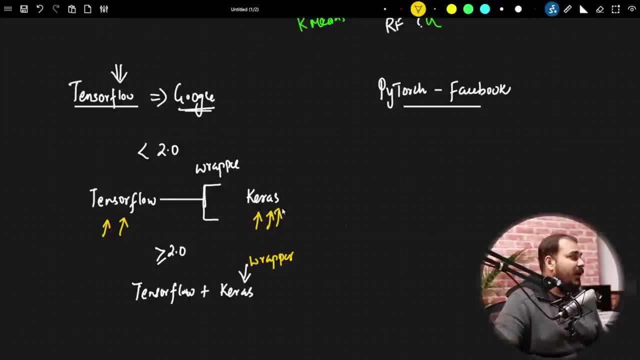 to install tensorflow and separately we to install tensorflow and separately we need to install Keras and then probably need to install Keras and then probably need to install Keras and then probably we'll be able to work right and there we'll be able to work right and there. 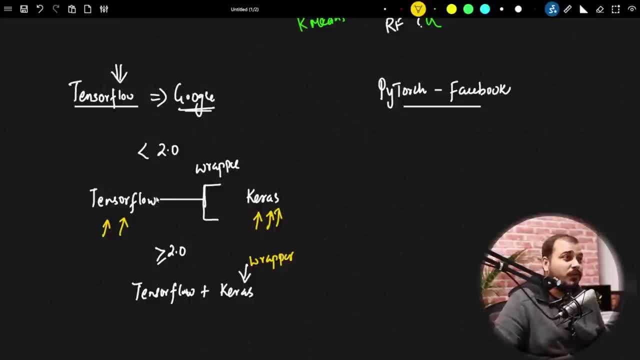 we'll be able to work right. and there was also definition of. there was also a was also definition of. there was also a was also definition of. there was also a dependency on the version that we are, dependency on the version that we are, dependency on the version that we are trying to use. okay, so right now it has. 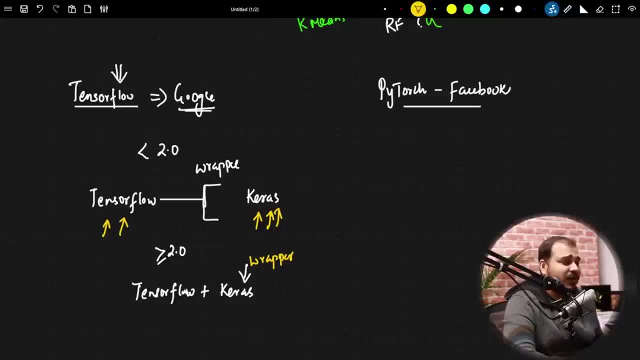 trying to use okay, so right now it has trying to use okay, so right now it has been made simple, when probably been made simple, when probably been made simple, when probably but tensorflow greater than 2.0 had, but tensorflow greater than 2.0 had. 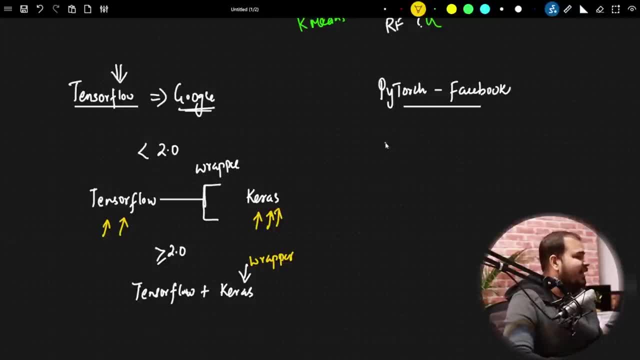 but tensorflow greater than 2.0 had actually come. okay, so let's go ahead and actually come. okay. so let's go ahead and actually come. okay. so let's go ahead and let's try to now start coding. and let's try to now start coding, and. 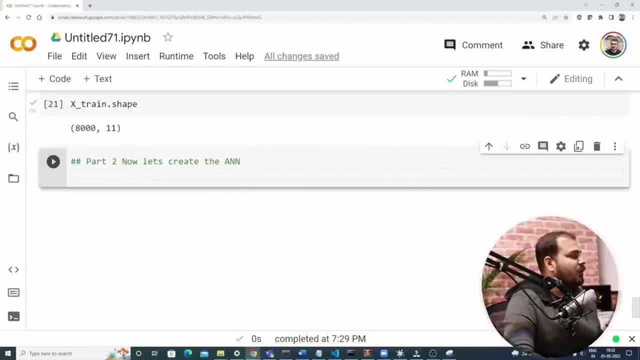 let's try to now start coding and tensorflow and Keras. so here it is here: tensorflow and Keras. so here it is here: tensorflow and Keras. so here it is here. what I am actually going to do is that. what I am actually going to do is that. 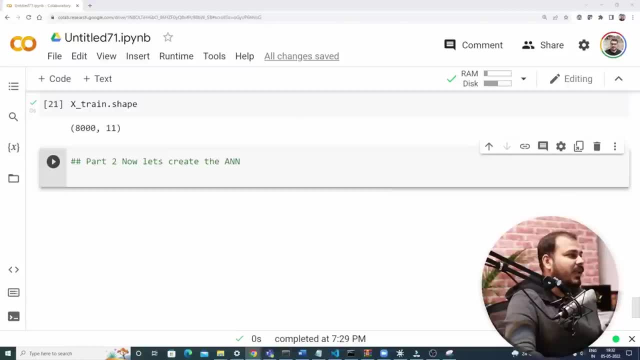 what I am actually going to do is that we are going to create the ANN to create. we are going to create the ANN to create. we are going to create the ANN to create the ANN. all we have to do is that import the ANN. all we have to do is that import. 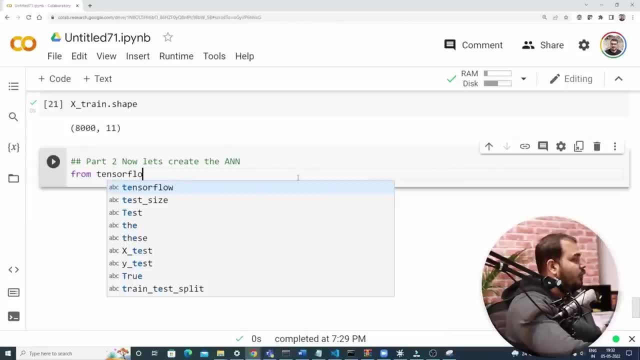 the ANN. all we have to do is that import some very important things. so, right now, some very important things. so right now, some very important things. so right now, first thing that I'm going to import, I'm first thing that I'm going to import, I'm. 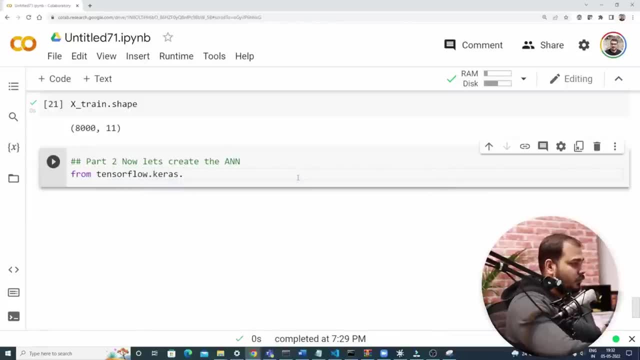 first thing that I'm going to import. I'm going to say from tensorflow dot Keras. going to say from tensorflow dot Keras. going to say from tensorflow dot Keras, I'm going to dot models. I'm going to, I'm going to dot models. I'm going to. 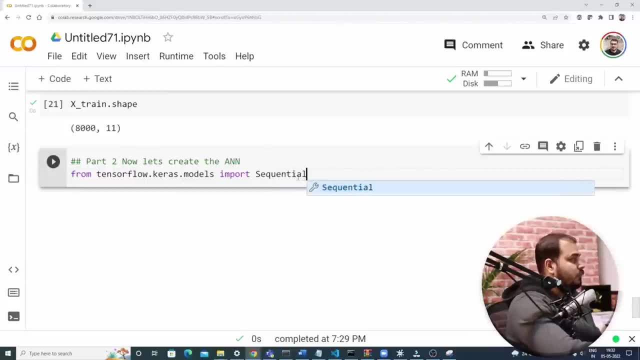 I'm going to dot models. I'm going to import sequential. okay then from import sequential. okay, then from import sequential. okay then from tensorflow dot. Keras dot layers. I'm going tensorflow dot. Keras dot layers. I'm going tensorflow dot. Keras dot layers. I'm going to import dense. okay, I'll talk about. 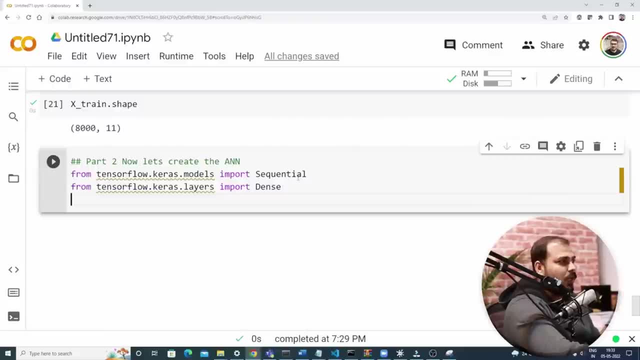 to import dense. okay, I'll talk about to import dense. okay, I'll talk about each and everything. what is sequential, each and everything, what is sequential, each and everything. what is sequential, what is dense and all, what is dense and all, what is dense and all you know from tensorflow dot Keras you. 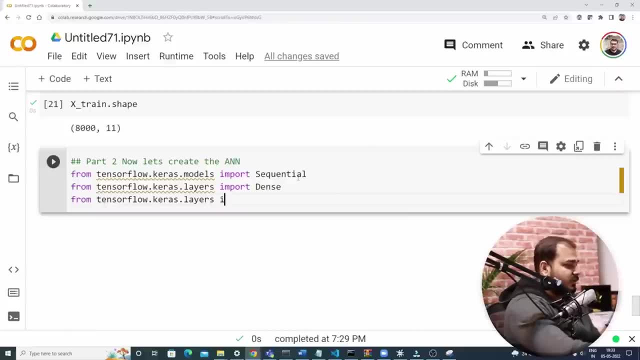 you know, from tensorflow dot Keras. you, you know, from tensorflow dot Keras. you can also import different, different can also import different, different can also import different. different layers- now what kind of layers this is. layers- now, what kind of layers this is layers- now, what kind of layers this is. these are specifically related to: 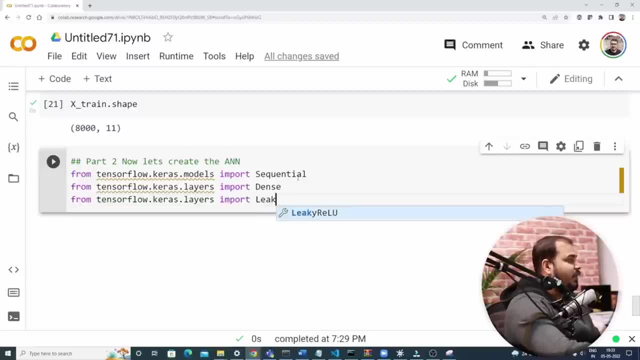 these are specifically related to. these are specifically related to activation function like this: I can activation function like this: I can activation function like this: I can basically say leaky delu. okay. I can basically say leaky delu. okay. I can basically say leaky delu. okay. I can basically say pre-relu: okay. so suppose, 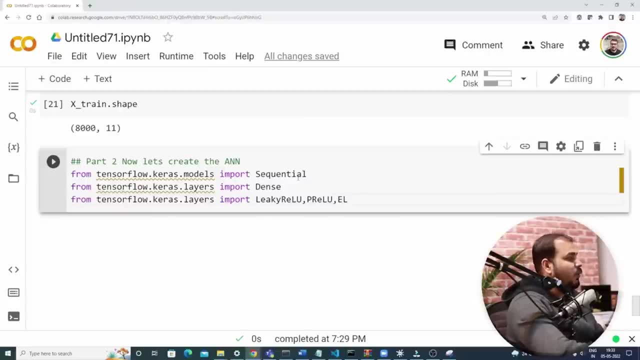 basically say pre-relu okay. so suppose, basically say pre-relu okay. so suppose: pre-lu right, this is also there. I can pre-lu right, this is also there. I can pre-lu right, this is also there. I can also say elu okay, if you see, elu is also. 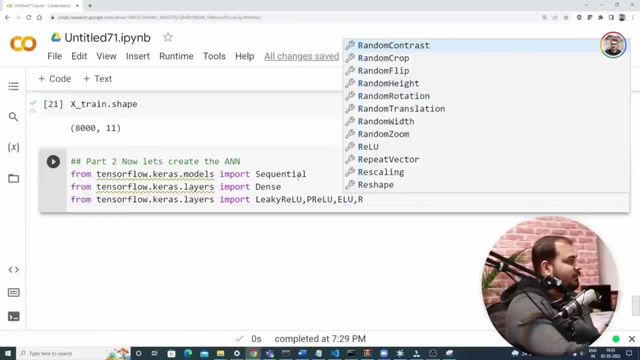 also say elu. okay, if you see elu is also also say elu. okay, if you see elu is also there. right. if I probably say relu, I can there right. if I probably say relu, I can there right. if I probably say relu, I can also add up relu. okay, so all these. 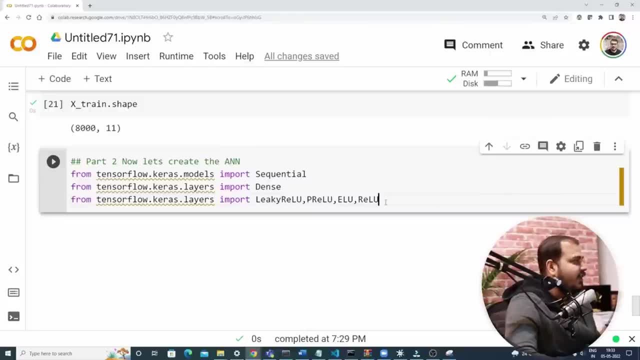 also add up relu, okay. so all these also add up relu, okay. so all these things right, the activation function, things right, the activation function, things right. the activation function that we have basically discussed right, that we have basically discussed right, that we have basically discussed right, all those things we can basically import. 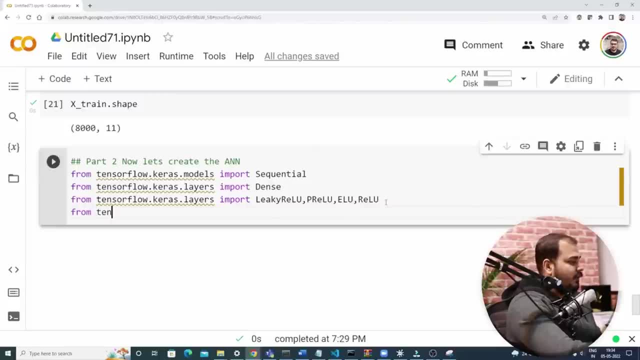 all those things we can basically import, all those things we can basically import, okay, and then up on top of it, I will okay, and then up on top of it, I will okay, and then up on top of it, I will also be importing one very important, also be importing one very important. 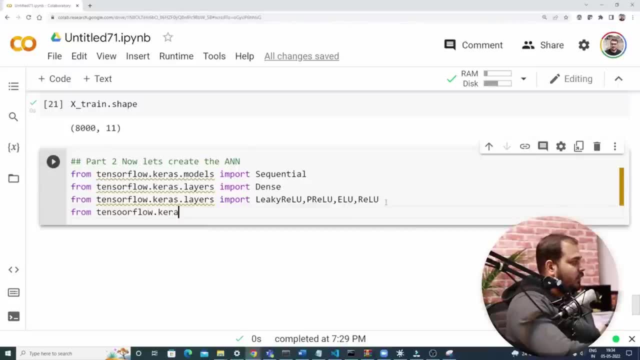 also be importing one very important thing which is called as dropout. okay, so thing which is called as dropout, okay, so thing which is called as dropout, okay. so I'll say: from tensorflow dot, keras dot. I'll say from tensorflow dot, keras dot, I'll say from tensorflow dot, keras dot layers, I'm going to import, import dropout. 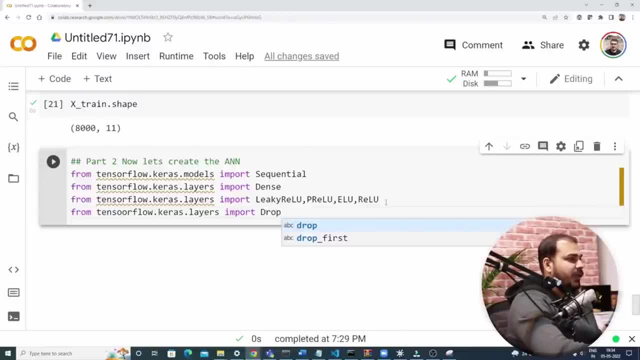 layers. I'm going to import import dropout layers. I'm going to import import dropout. okay, so what is dropout dropout layer? okay, so what is dropout dropout layer? okay, so what is dropout dropout layer? I'll just discuss about this theoretical. I'll just discuss about this theoretical. 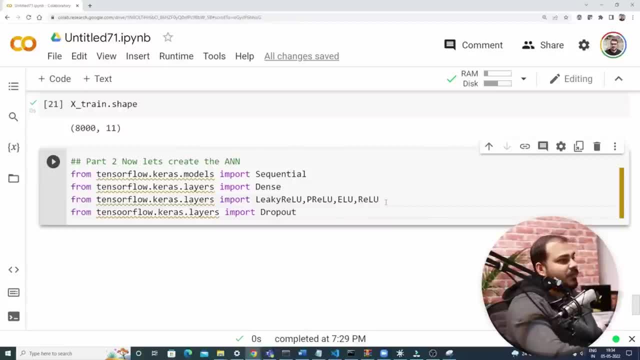 I'll just discuss about this, theoretical, okay, and to make everybody understand okay, and to make everybody understand okay, and to make everybody understand okay. so from tensorflow dot keras dot. okay. so from tensorflow dot- keras dot. okay. so from tensorflow dot- keras dot layers. I'm just going to input dropout. 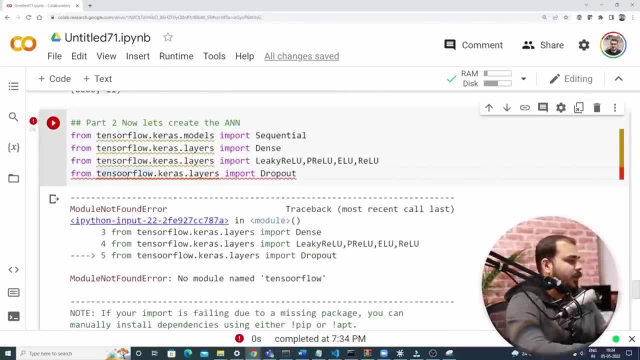 layers. I'm just going to input dropout layers. I'm just going to input dropout now. oh okay, tensorflow, okay, fine now now. oh okay, tensorflow, okay, fine now now. oh okay, tensorflow, okay, fine now. let's discuss about all these things. let's discuss about all these things. 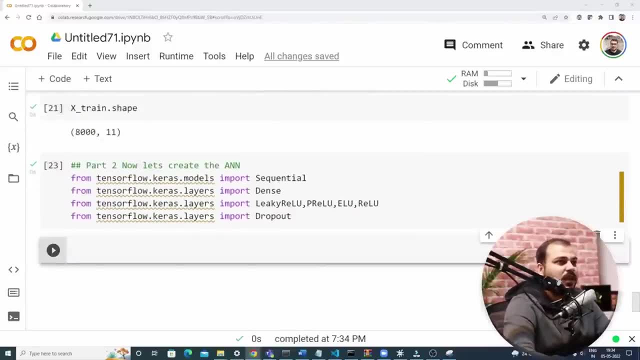 let's discuss about all these things. what is sequential? why dense library? what is sequential? why dense library? what is sequential? why dense library specifically used? you know why all these specifically used. you know why all these specifically used. you know why all these things are there, why we have to use so. 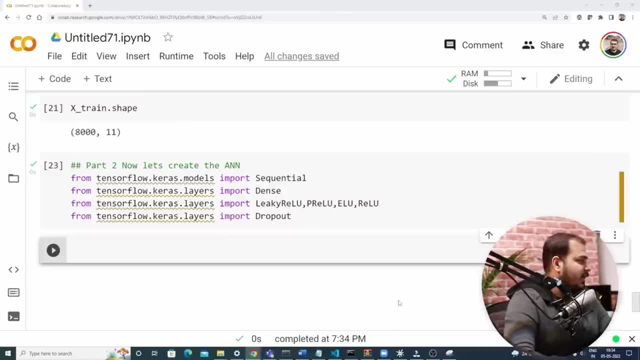 things are there, why we have to use so things are there, why we have to use so many things, and all everything will try many things and all everything will try many things, and all everything will try to see so quickly, let's go ahead. and to see so quickly, let's go ahead. and 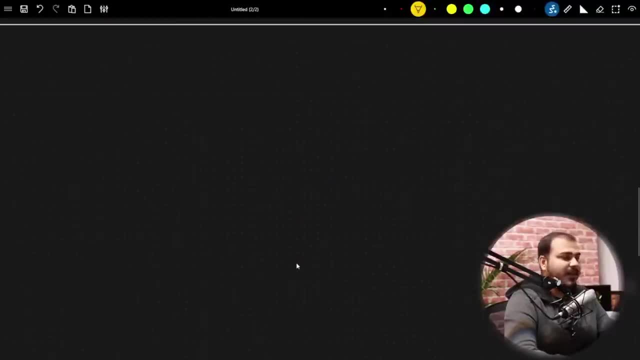 to see so quickly. let's go ahead and let's try to understand so first thing. let's try to understand so first thing. let's try to understand so first thing. first, as usual, we will go from basics first. as usual, we will go from basics first. as usual, we will go from basics first thing. we imported something called. 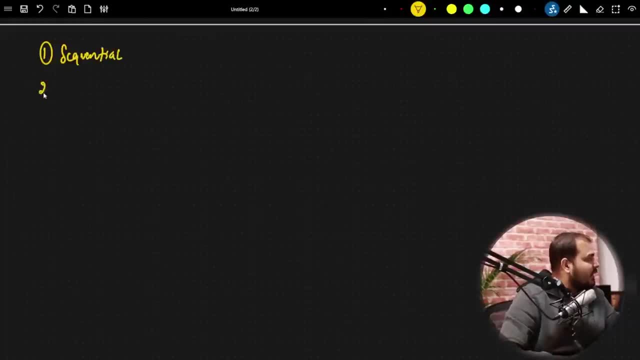 first thing: we imported something called. first thing: we imported something called a sequential okay. second thing: we a sequential okay. second thing: we a sequential okay. second thing: we basically discussed about dense. third, basically discussed about dense. third, basically discussed about dense. third thing: that relu and all that is. 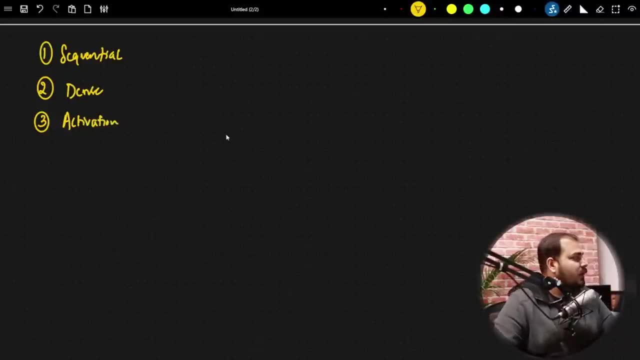 thing that relu and all that is thing that relu and all that is basically the activation function. right, basically the activation function. right, basically the activation function right now. understand if I probably draw now, understand if I probably draw now, understand if I probably draw quickly a neural network. right, let's say: 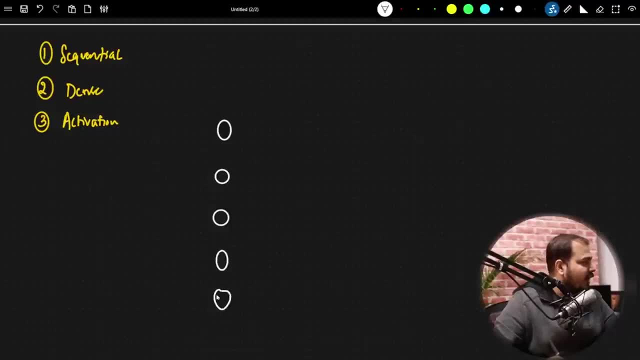 quickly a neural network right. let's say: quickly a neural network right. let's say: this is my basic neural network right. this is my basic neural network right. this is my basic neural network right now. the number of inputs that I have: 11. now the number of inputs that I have: 11. 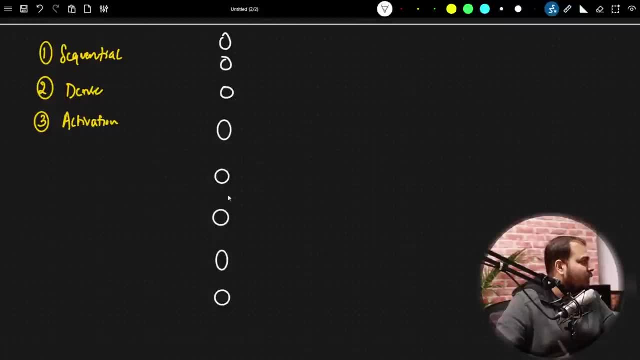 now the number of inputs that I have: 11. let's say this is my 11 inputs: 1, 2, 3, 4, 5. let's say this is my 11 inputs: 1, 2, 3, 4, 5. let's say this is my 11 inputs: 1, 2, 3, 4, 5, 6, 7, 8, 9, 10. one more we can insert over: 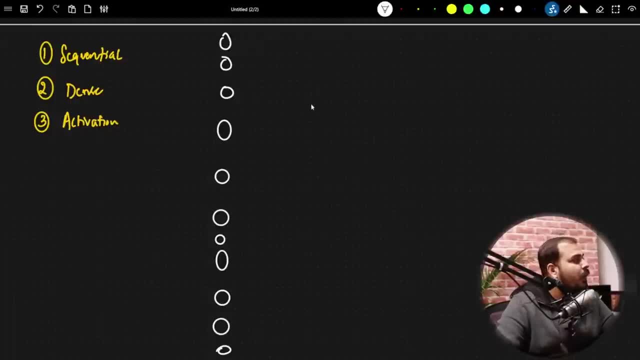 6, 7, 8, 9, 10, one more we can insert over: 6, 7, 8, 9, 10. one more we can insert over here: okay, 11 inputs will be there, okay here. okay, 11 inputs will be there, okay here. okay, 11 inputs will be there, okay. and then let's say in my hidden layer: and then let's say: in my hidden layer, and then let's say: in my hidden layer there are some neurons. I'm not just there are some neurons, I'm not just there are some neurons. I'm not just going to count how many hidden levels, going to count how many hidden levels. 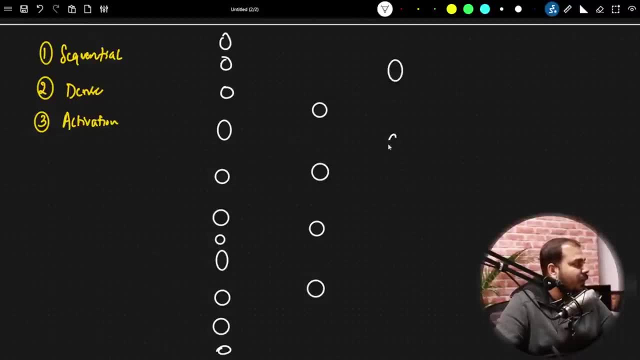 going to count how many hidden levels. are there okay? and then I may have. are there okay? and then I may have. are there okay? and then I may have another hidden layer. okay, I may have another hidden layer. okay, I may have another hidden layer. okay, I may have another hidden layer. and remember this: 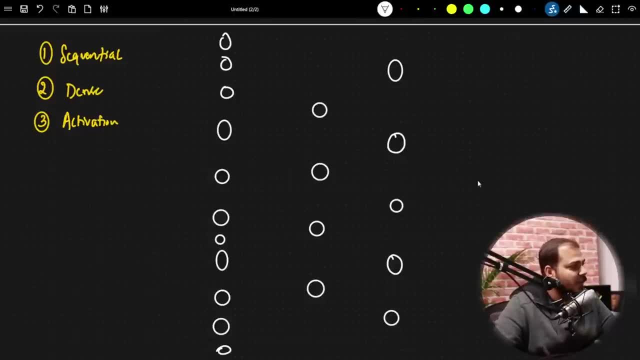 another hidden layer. and remember this. another hidden layer and remember this: all will get interconnected. and since all will get interconnected, and since all will get interconnected, and since this is a binary classification problem- I, this is a binary classification problem. I, this is a binary classification problem- I can have one single output which will: 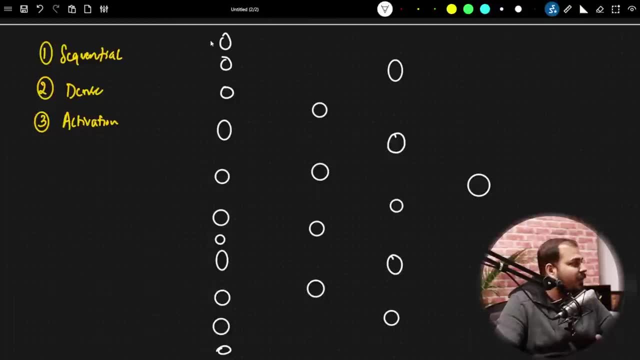 can have one single output which will can have one single output which will basically be able to tell you, whether basically be able to tell you, whether basically be able to tell you whether the output is 1 or 0. okay, and remember, the output is 1 or 0. okay, and remember. 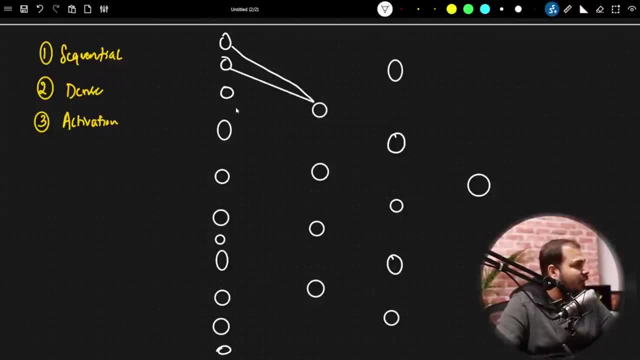 the output is 1 or 0. okay, and remember this: all will be interconnected. right? this: all will be interconnected. right? this: all will be interconnected. right? this will be interconnected, interconnected. this will be interconnected. interconnected. this will be interconnected, interconnected, interconnected. interconnected like this: interconnected, interconnected. interconnected like this. 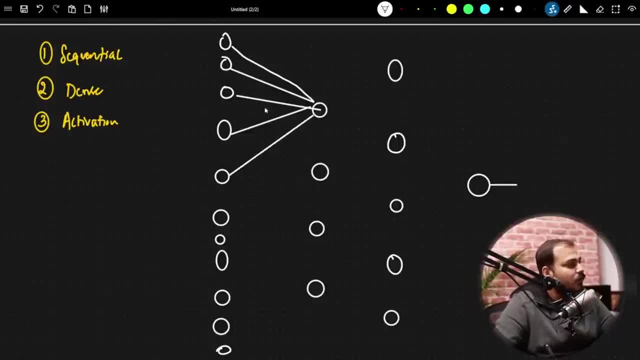 interconnected, interconnected, interconnected, interconnected. like this, all will be interconnected right and all will be interconnected right and all will be interconnected right and similarly. finally we get the output similarly, finally we get the output similarly. finally we get the output layer. this is all my input. right input layer. this is all my input. right input. 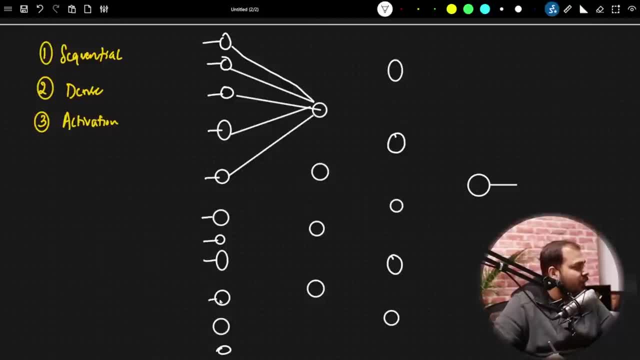 layer. this is all my input, right input. now let's understand why we have imported now. let's understand why we have imported now. let's understand why we have imported sequential and all everything okay when sequential and all everything okay when sequential and all everything okay when I take this entire neural network at once. 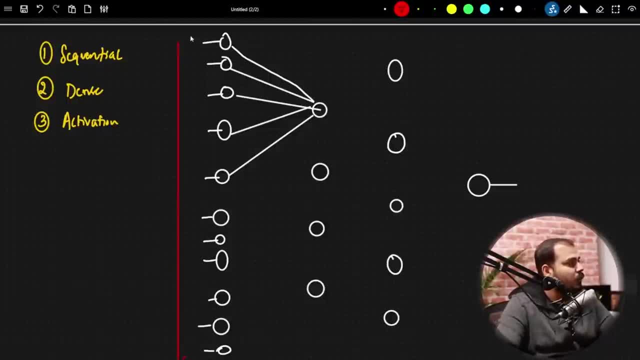 I take this entire neural network at once. I take this entire neural network at once, if I probably take this entire neutral, if I probably take this entire neutral, if I probably take this entire neutral neural network together right as a block, neural network together right as a block. 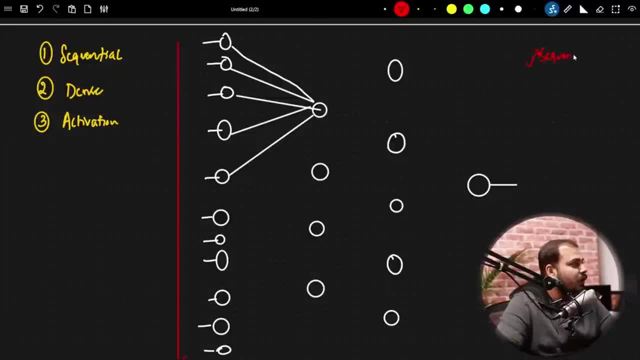 neural network together, right as a block. okay, I will basically say that as okay. I will basically say that as okay. I will basically say that as sequential, sequential okay. this sequential, sequential okay, this sequential, sequential okay. this sequential basically indicates that we. sequential basically indicates that we. sequential basically indicates that we will definitely be able to do forward. 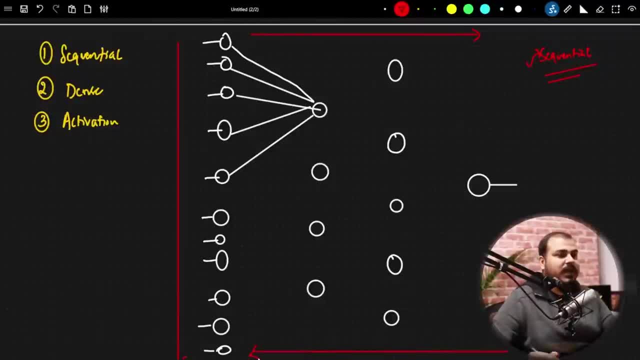 will definitely be able to do forward, will definitely be able to do forward propagation and backward propagation- okay. propagation and backward propagation. okay, propagation and backward propagation- okay. so I just think as a huge block that has so, I just think as a huge block that has, so I just think as a huge block that has a neural network inside this and that can. 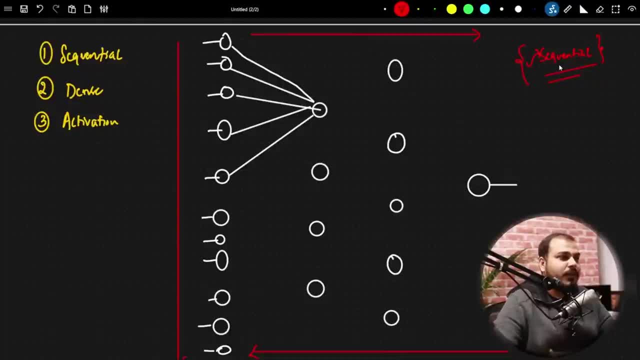 a neural network inside this and that can a neural network inside this, and that can be basically done with the sequential. be basically done with the sequential, be basically done with the sequential- okay, and this sequential whenever we okay and this sequential whenever we okay and this sequential whenever we write. we will definitely be able to do. 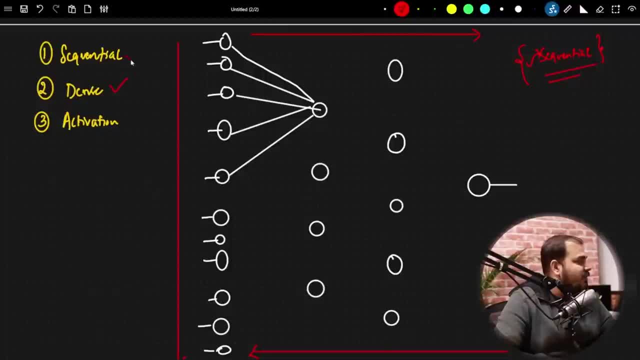 write, we will definitely be able to do write, we will definitely be able to do the forward and backward propagation now. the forward and backward propagation now, the forward and backward propagation now, whenever we use dense- okay, whenever we. whenever we use dense- okay, whenever we. whenever we use dense- okay, whenever we use dense. that basically means we'll be. 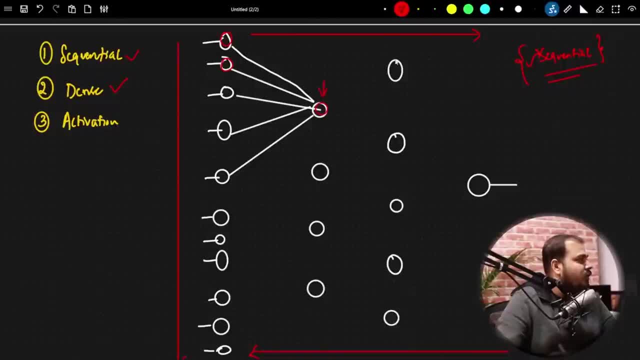 use dense. that basically means we'll be use dense. that basically means we'll be able to create the circles in the hidden. able to create the circles in the hidden. able to create the circles in the hidden layer. we will be able to create neurons layer. we will be able to create neurons. 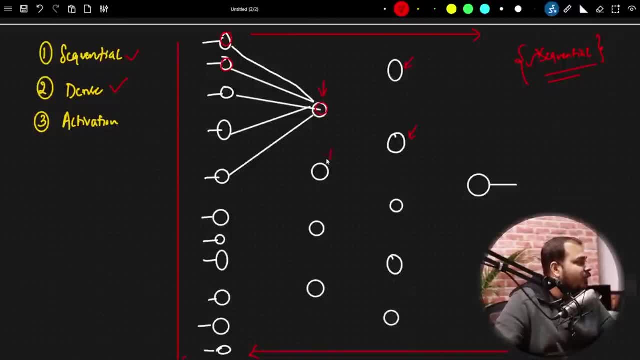 layer. we will be able to create neurons in in the hidden layer. we will be able to in in the hidden layer. we will be able to. in in the hidden layer. we will be able to create all the different neurons, create all the different neurons, create all the different neurons. whenever we need to create neurons or 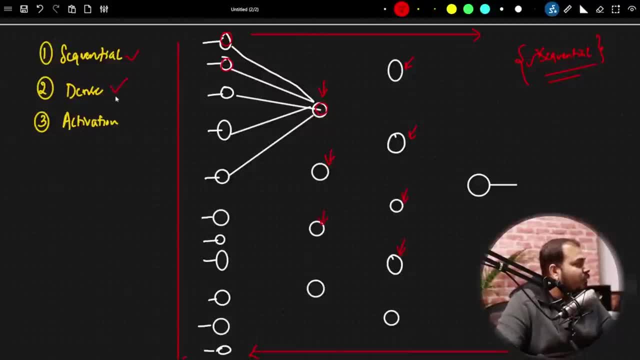 whenever we need to create neurons, or whenever we need to create neurons or input layer, or this the circles, then at input layer, or this the circles, then at input layer, or this the circles, then at that point of time we will be using the. that point of time we will be using the. 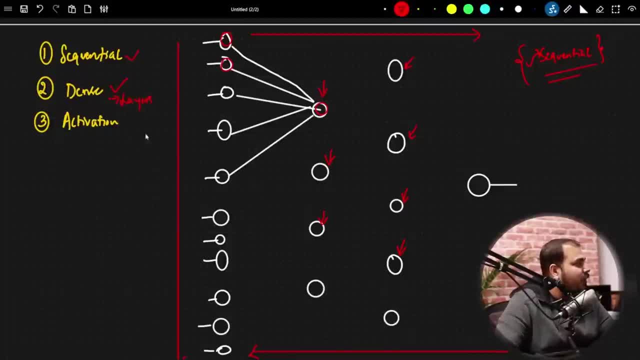 that point of time, we will be using the dense layer. okay, so this is specifically dense layer. okay, so, this is specifically dense layer. okay, so this is specifically dense layer. with the help of dense layer, dense layer, with the help of dense layer, dense layer, with the help of dense layer, we will be able to create the hidden. 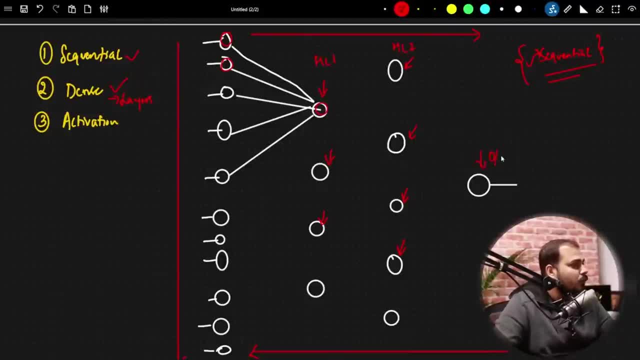 we will be able to create the hidden. we will be able to create the hidden layers. will be able to create the input layers. will be able to create the input layers. will be able to create the input layers. will be able to create the output layers. will be able to create the output. 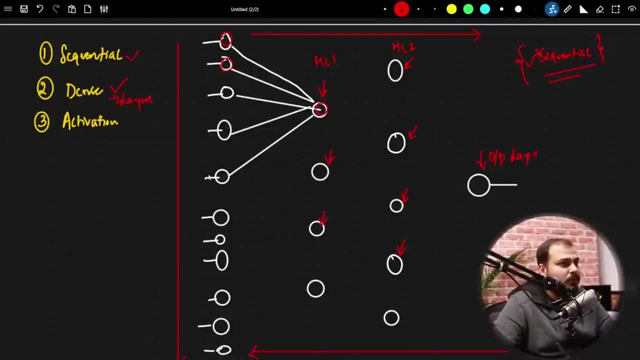 layers will be able to create the output layer: okay. input layer- output layer- okay. layer okay. input layer- output layer: okay. layer okay. input layer- output layer: okay. so that is the reason we use dense now. so that is the reason we use dense now. so that is the reason we use dense now when we come to the activation function. 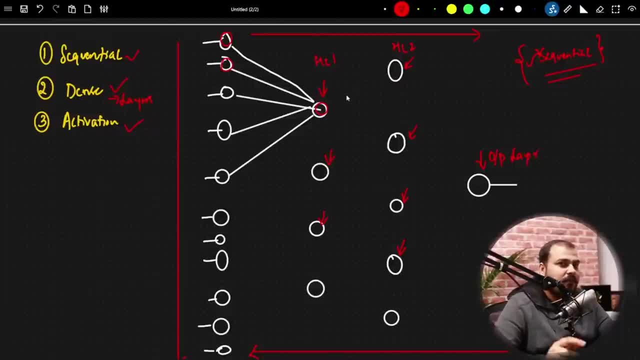 when we come to the activation function, when we come to the activation function, I hope everybody knows that. what all? I hope everybody knows that, what all I hope everybody knows that, what all activation function we have. we have activation function we have. we have activation function we have. we have learned it in depth pre-relu, elu, relu. 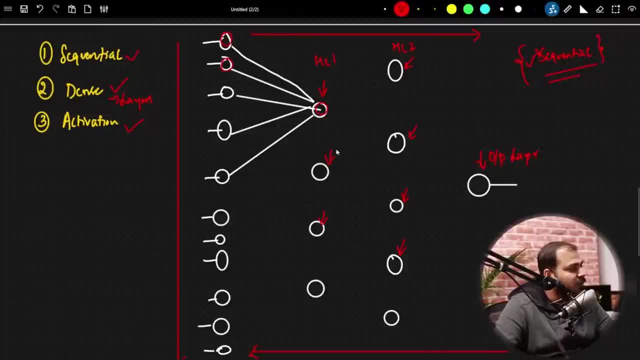 learned it in depth pre-relu. elu relu learned it in depth pre-relu. elu relu. sigmoid right tanh and all where we'll sigmoid right tanh and all where we'll sigmoid right tanh and all where we'll be using we'll be using in the hidden. 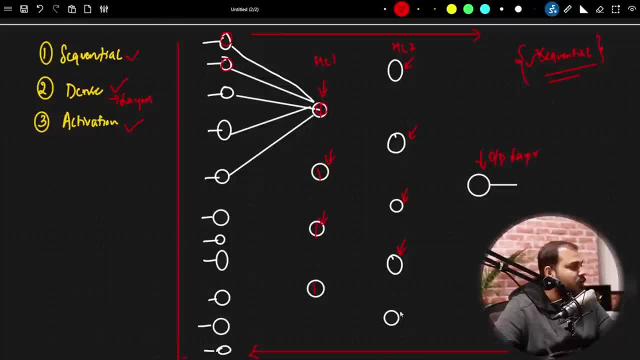 be using, we'll be using in the hidden be using, we'll be using in the hidden layer itself inside this, whatever layer itself inside this, whatever layer itself inside this, whatever activation function we want, we will be activation function we want. we will be activation function we want. we will be able to use it right, we will be able to. 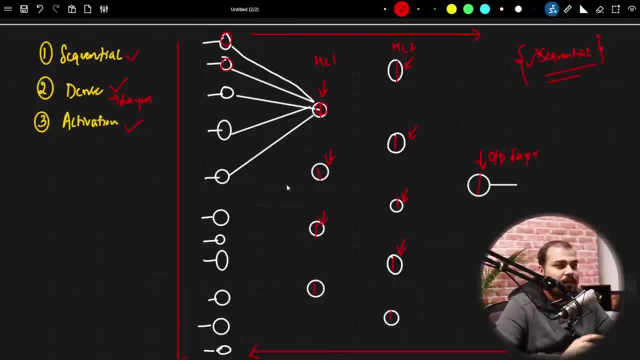 able to use it right, we will be able to able to use it right. we will be able to use it over here, here, here, here, right. use it over here, here, here, here, right. use it over here, here, here, right, here, here, right, we'll be able to use it in a. 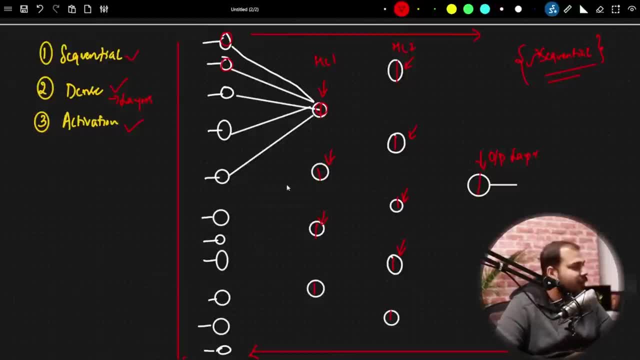 we'll be able to use it in a. we'll be able to use it in a better way. okay, now, mostly we have covered better way. okay, now, mostly we have covered better way. okay, now, mostly we have covered this. there is also one more layer. this: there is also one more layer. 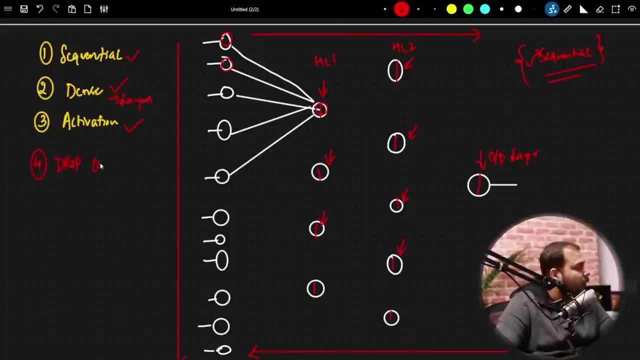 this. there is also one more layer, which is called as dropout layer, now let, which is called as dropout layer, now let, which is called as dropout layer. now let me talk about this dropout. okay, now me talk about this dropout. okay, now me talk about this dropout. okay, now, what does dropout basically say: let's. 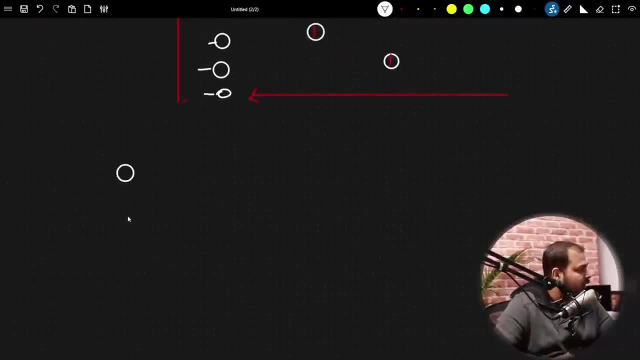 what does dropout basically say: let's. what does dropout basically say: let's say I have a simple neural network like say: I have a simple neural network. like say: I have a simple neural network like this: let's say I have a three input. this: let's say I have a three input. 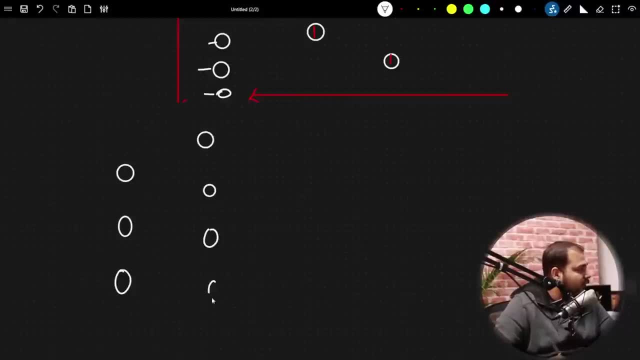 this: let's say I have a three input layer and I may have many hidden neurons layer and I may have many hidden neurons layer and I may have many hidden neurons, let's say, and I may have another set of. let's say, and I may have another set of. 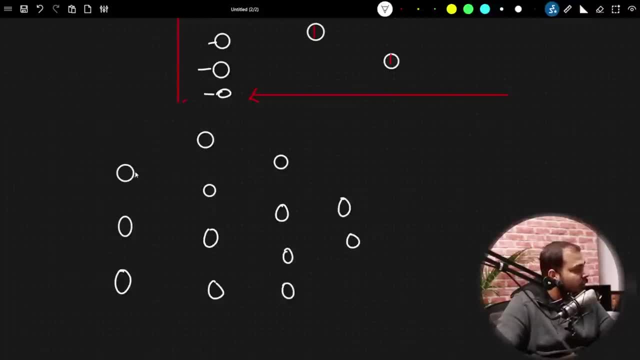 let's say, and I may have another set of hidden neurons, and finally I may have hidden neurons, and finally I may have hidden neurons, and finally I may have output layer. okay now, when I have this output layer. okay now, when I have this output layer. okay now, when I have this interconnected multi-layered neural. 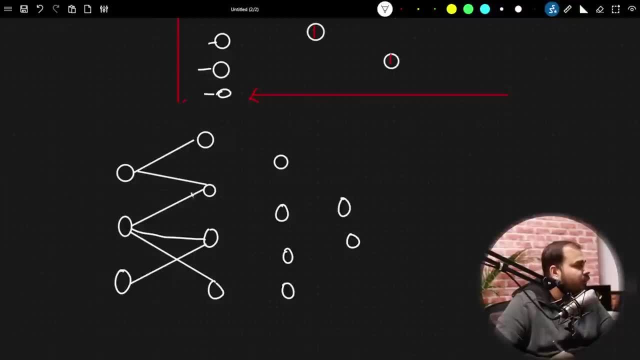 interconnected, multi-layered neural, interconnected, multi-layered neural network. and you know that because of network, and you know that because of network, and you know that because of this, neurons neurons, right it it it, this neurons, neurons, right it it it. this neurons neurons, right it it. it actually helps us to solve complex. 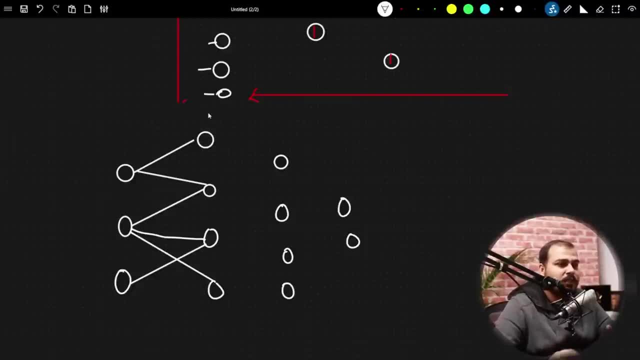 actually helps us to solve complex problems. also because we will be doing problems. also because we will be doing problems also because we will be doing forward and backward propagation, will- forward and backward propagation will- forward and backward propagation will always be continuously monitoring the, always be continuously monitoring the. 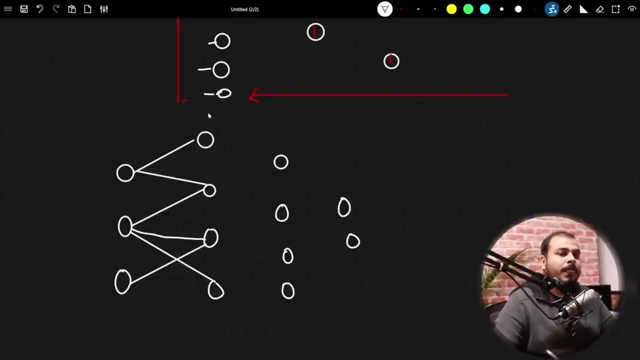 always be continuously monitoring the loss function and, with the help of loss function, and with the help of loss function, and with the help of optimizers, will always try to come to a. optimizers will always try to come to a. optimizers will always try to come to a. you know the global minima in some time. 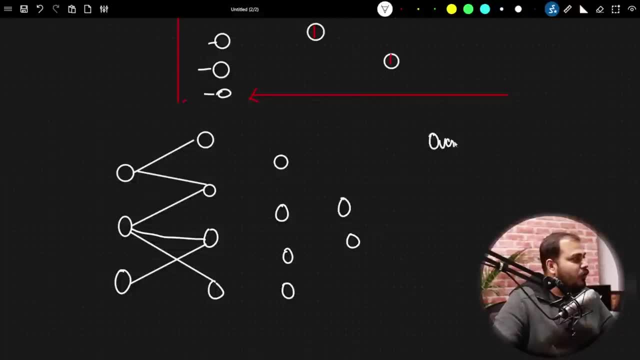 you know the global minima in some time. you know the global minima in some time, right, sometime this, this entire lead right. sometime this, this entire lead, right sometime this, this entire lead, this entire neural network leads to this entire neural network, leads to this entire neural network, leads to overfitting. now what is overfitting? 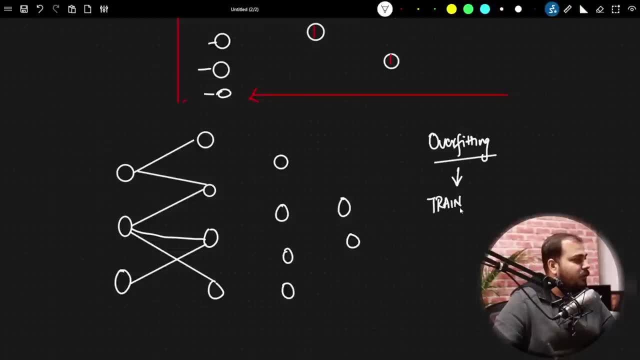 overfitting, now what is overfitting. overfitting, now what is overfitting. accuracy goes down. okay, my accuracy goes. accuracy goes down. okay, my accuracy goes. accuracy goes down. okay, my accuracy goes down. now this kind of to reduce the down. now this kind of to reduce the. 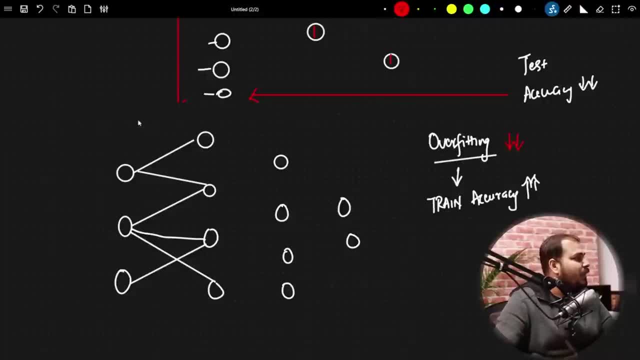 down now this kind of to reduce the overfitting. what we do specifically is overfitting. what we do specifically is overfitting. what we do specifically is that we basically introduce something, that we basically introduce something, that we basically introduce something called a dropout layer. now this dropout. called a dropout layer. now this dropout called a dropout layer, now this dropout layer. what it does, it is just like a layer. what it does, it is just like a layer. what it does, it is just like a regularization parameter which we learned. regularization parameter which we learned. 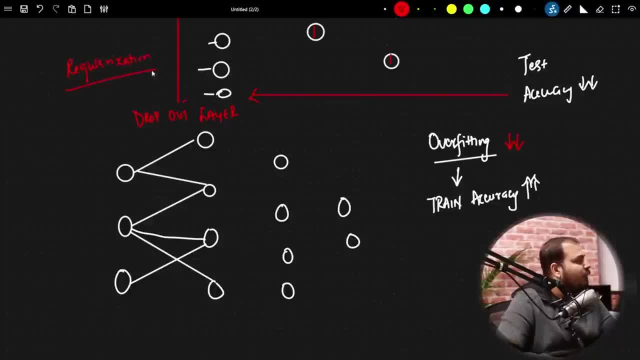 regularization parameter which we learned in machine learning regularization, in machine learning regularization, in machine learning regularization parameter. i hope everybody knows about parameter. i hope everybody knows about parameter. i hope everybody knows about l1 norm, l1 norm, l1 norm- right, we have discussed this. l2 norm and 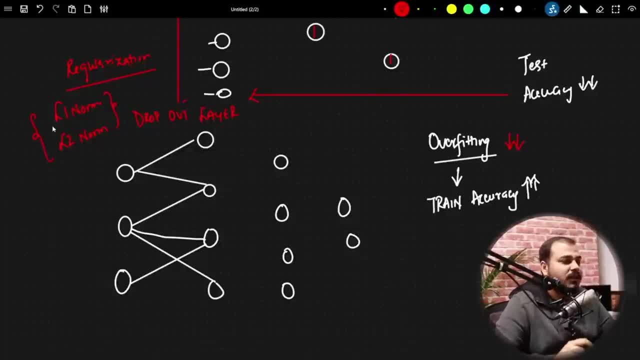 right, we have discussed this l2 norm. right, we have discussed this l2 norm. all we have discussed in depth, all we have discussed in depth, all we have discussed in depth, right, all these things we have discussed, right, all these things we have discussed, right, all these things we have discussed in completely depth, right in my machine. 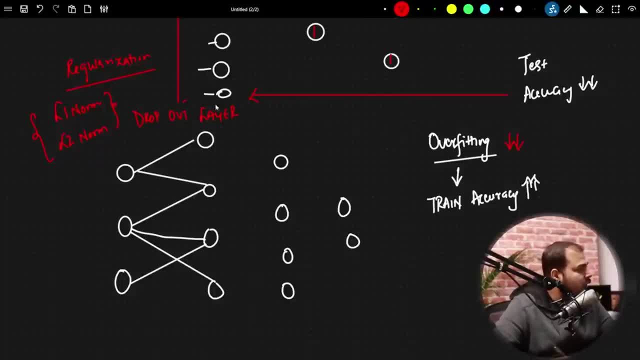 in completely depth, right in my machine, in completely depth, right in my machine learning, learning, learning sessions, right now, in this dropout sessions, right now in this dropout sessions, right now in this dropout layer. what it does is that layer, what it does is that layer, what it does is that every layer suppose, if i say my dropout? 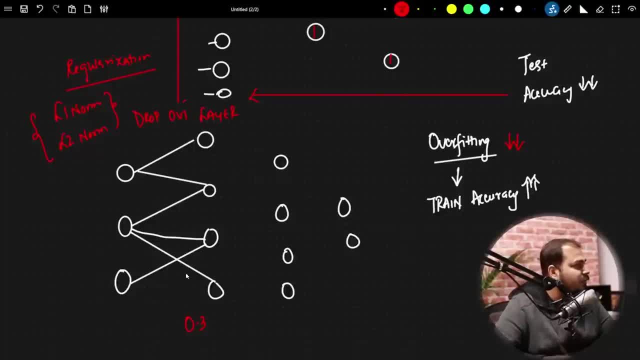 every layer. suppose if i say my dropout layer, suppose if i say my dropout over here ratio is 0.3, this basically over here ratio is 0.3. this basically over here ratio is 0.3. this basically indicates that 30 percentage of the 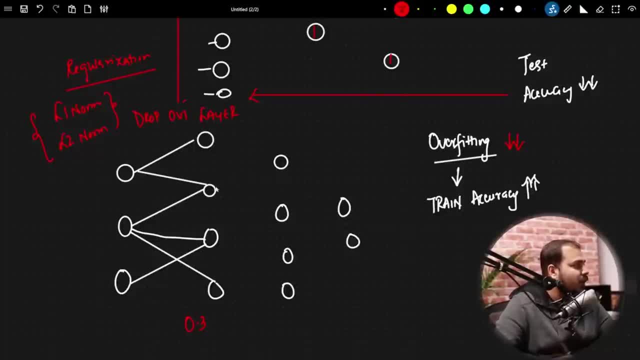 indicates that 30 percentage of the indicates that 30 percentage of the entire neurons that are present in this entire neurons that are present in this entire neurons that are present in this layer will get deactivated while layer will get deactivated. while layer will get deactivated while training okay- will get deactivated, like 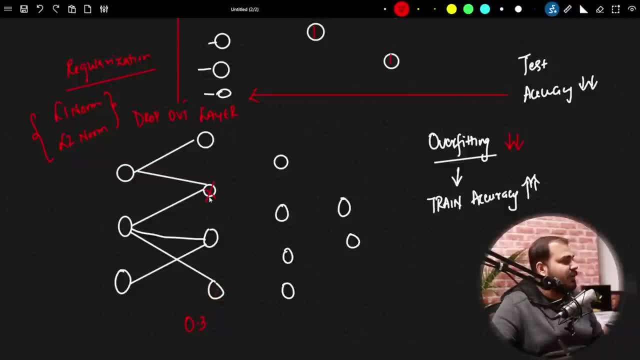 training okay will get deactivated like training okay, will get deactivated like while training. let's say the 30 is one while training. let's say the 30 is one while training. let's say the 30 is one neuron out of all this right, this will neuron out of all this right, this will. 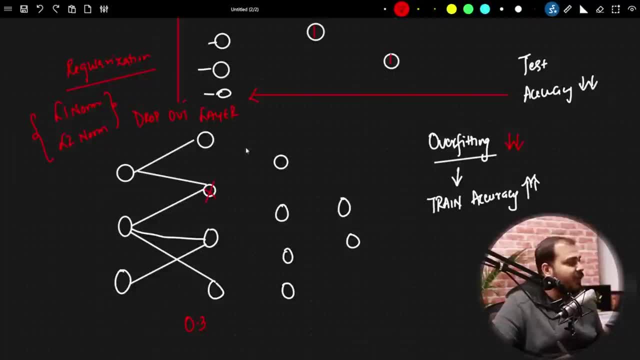 neuron out of all this right. this will get deactivated during the training, get deactivated during the training, get deactivated during the training purpose. so when it is when the training purpose. so when it is when the training purpose, so when it is when the training is basically happening, when the forward. 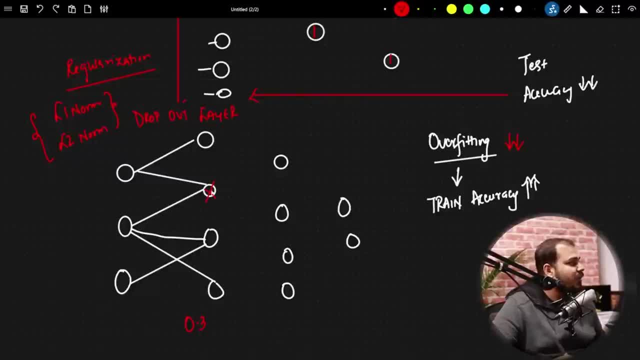 is basically happening, when the forward is basically happening, when the forward propagation and backward propagation is propagation and backward propagation is propagation and backward propagation is actually happening, you will basically be actually happening. you will basically be actually happening. you will basically be seeing that this will get deactivated. seeing that this will get deactivated. seeing that this will get deactivated right similarly over here, i can right, similarly over here, i can right similarly over here. i can basically say 0.5, 50 percentage of the. basically say 0.5, 50 percentage of the. 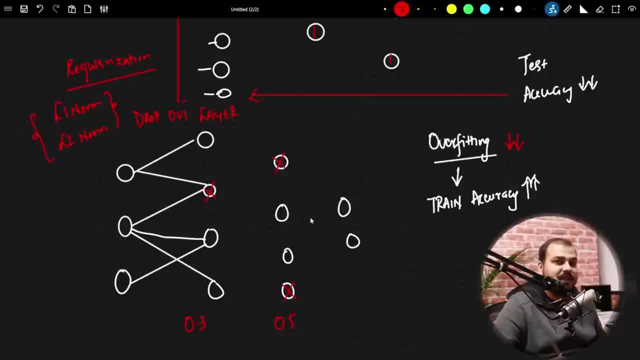 basically say 0.5, 50 percentage of the neurons will get deactivated. so suppose neurons will get deactivated. so suppose neurons will get deactivated. so suppose this and this will get randomly selected, this and this will get randomly selected, this and this will get randomly selected and this will get deactivated. remaining: 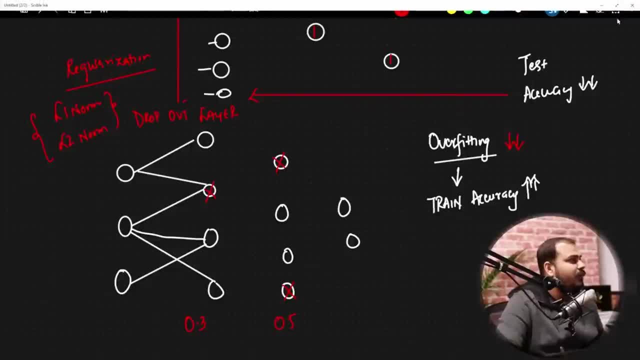 and this will get deactivated. remaining, and this will get deactivated. remaining. all the connections will be there. all the connections will be there. all the connections will be there whenever the neurons are deactivated. we, whenever the neurons are deactivated, we, whenever the neurons are deactivated, we will basically cut off the layer. okay. 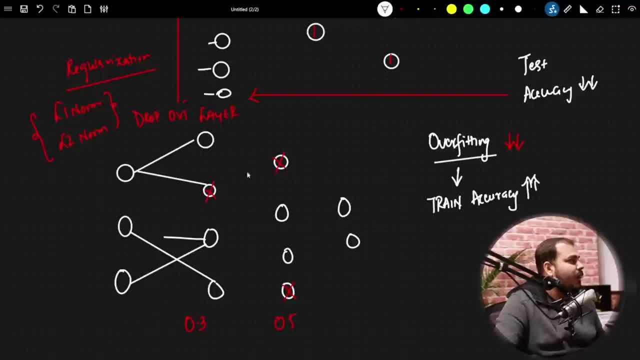 will basically cut off the layer. okay, will basically cut off the layer. okay, because it will be of no use, right it because it will be of no use, right it, because it will be of no use, right, it will just be like a dead neuron, right, will just be like a dead neuron, right. 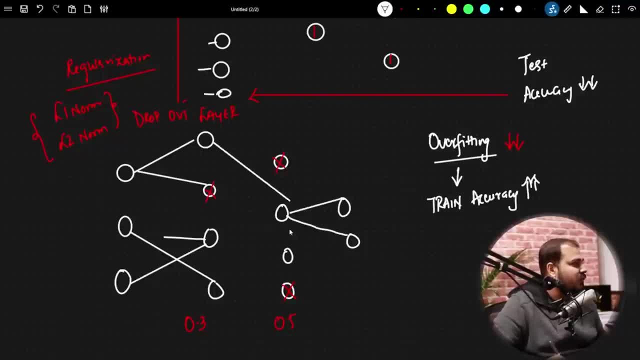 will just be like a dead neuron right and this will get this, this will get and this will get this, this will get and this will get this, this will get connected to this, this, this, this, like connected to this, this, this, this, like connected to this, this, this, this, like this, and through this way, what happens? 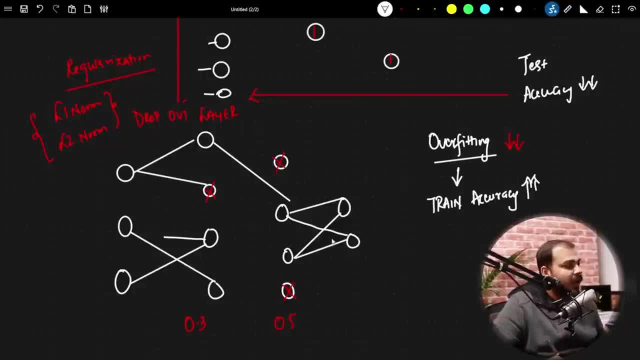 this and through this way. what happens, this and through this way, what happens is that my entire training process will, is that my entire training process will, is that my entire training process will actually go ahead. you know, and the this actually go ahead. you know, and the this. 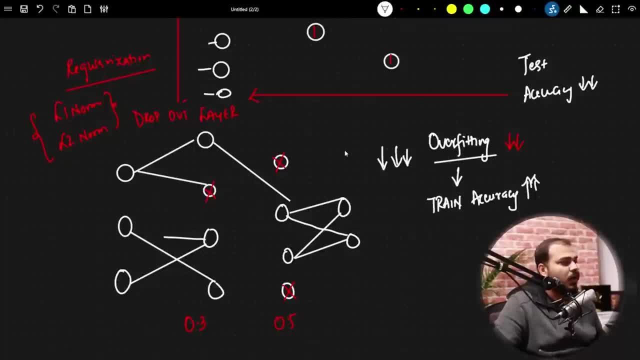 actually go ahead. you know, and the- this is in short: whenever we use dropout layer is in short: whenever we use dropout layer is in short: whenever we use dropout layer, we are basically trying to, we are basically trying to, we are basically trying to reduce the overfitting and work in an 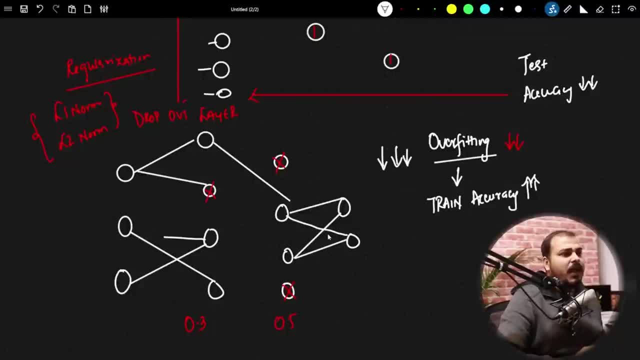 reduce the overfitting and work in an reduce the overfitting and work in an efficient way. so this is an idea about efficient way. so this is an idea about efficient way. so this is an idea about dropout layer and the same thing we'll- dropout layer, and the same thing we'll. 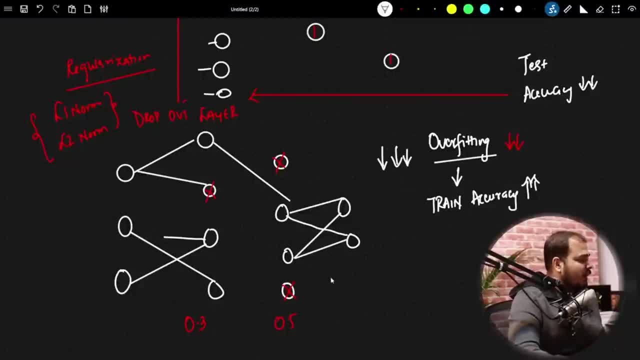 dropout layer. and the same thing we'll also try to do in today's thing, right. so also try to do in today's thing, right. so also try to do in today's thing, right. so let's go ahead and let's go back to the. let's go ahead and let's go back to the. 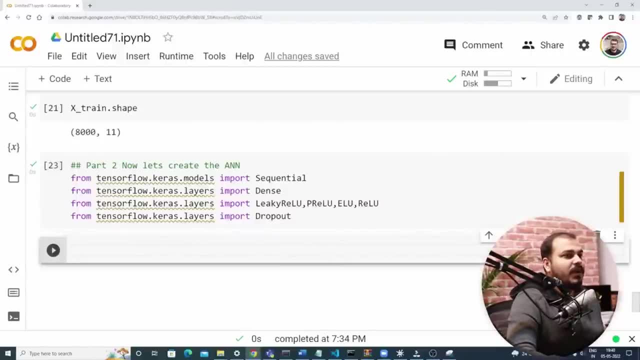 let's go ahead and let's go back to the code now, now, over here. we have imported code now. now over here. we have imported code now, now over here. we have imported everything that is required. so let's everything that is required. so let's everything that is required. so let's continue and let's try to do the things. 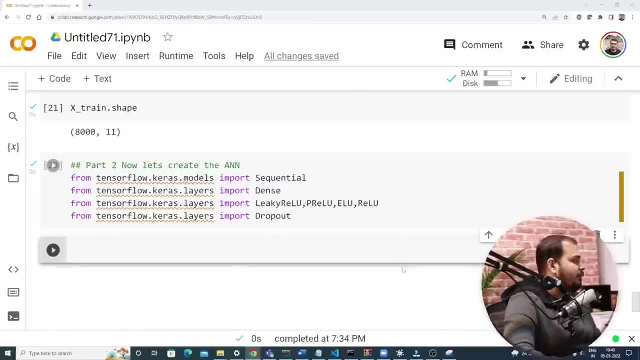 continue and let's try to do the things continue and let's try to do the things okay, now, first thing first. we will okay, now, first thing first. we will okay, now, first thing first. we will initialize the ANN. okay, we have just initialize the ANN. okay, we have just. 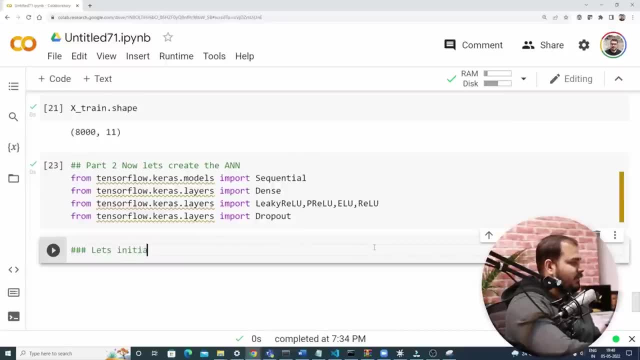 initialize the ANN: okay, we have just imported the library, so I'm just going, imported the library, so I'm just going, imported the library. so I'm just going to: let's initialize the ANN: okay, ANN. and to let's initialize the ANN: okay, ANN. and to let's initialize the ANN: okay, ANN. and then I'm going to basically write: 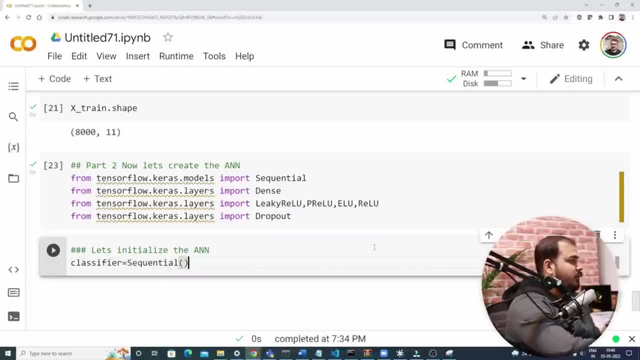 then I'm going to basically write. then I'm going to basically write: classifier is equal to sequential. classifier is equal to sequential. classifier is equal to sequential- sequential. so this is the classifier sequential. so this is the classifier sequential. so this is the classifier that I'm specifically going to use. let's 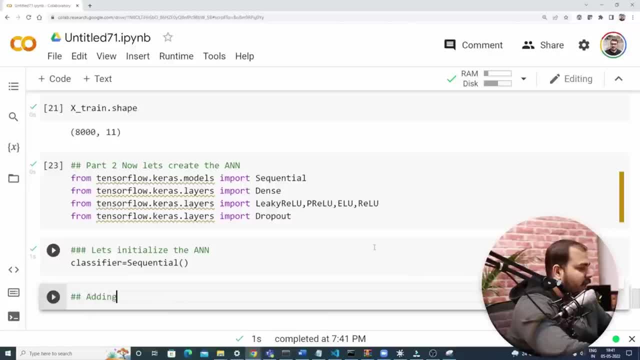 that I'm specifically going to use. let's that I'm specifically going to use. let's initialize the ANN itself and then I'm initialize the ANN itself, and then I'm initialize the ANN itself and then I'm going to basically add, add the input, going to basically add, add the input. 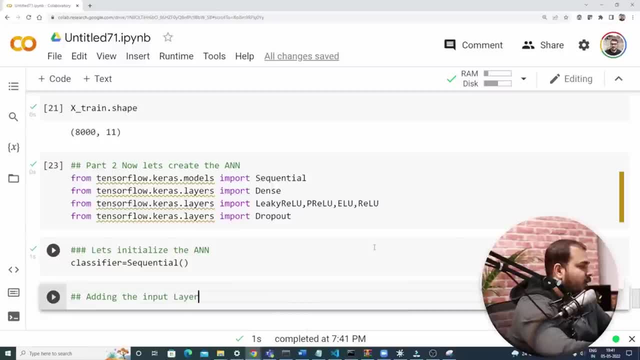 going to basically add: add the input layer, adding the input layer. okay, now, layer adding the input layer. okay, now, layer adding the input layer. okay, now, when we decide that, okay, we initialize. when we decide that, okay, we initialize. when we decide that, okay, we initialize this ANN, this entire in by the. 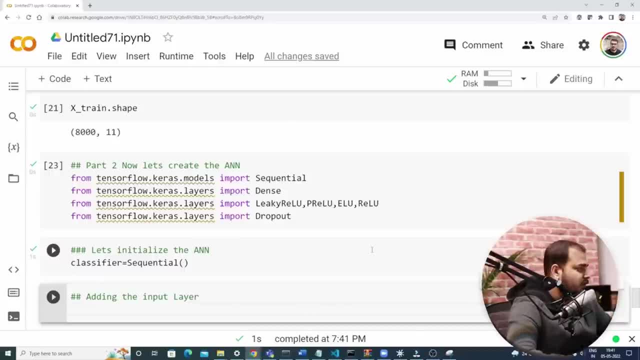 this ANN, this entire in by the this ANN, this entire in by the sequential part. now I need to add the sequential part, now I need to add the sequential part. now I need to add the input layer, because see from this what input layer, because see from this what. 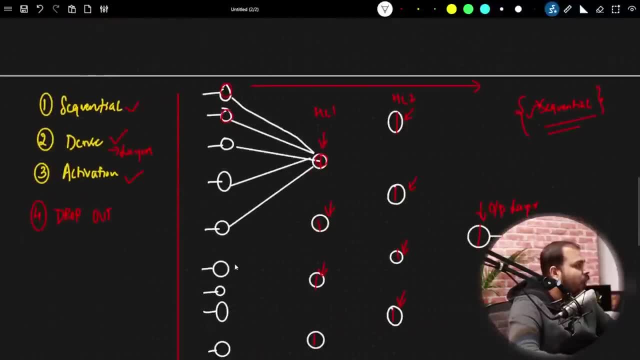 input layer, because see from this what we are doing first of all, we need to add. we are doing first of all, we need to add. we are doing first of all, we need to add this input layer right and we know how, this input layer right and we know how. 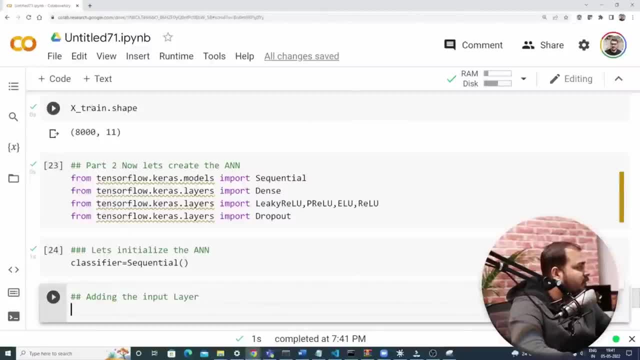 this input layer right and we know how many inputs are there. see if we probably many inputs are there. see if we probably many inputs are there. see if we probably go and see my X train shape: they are 11. go and see my X train shape: they are 11. 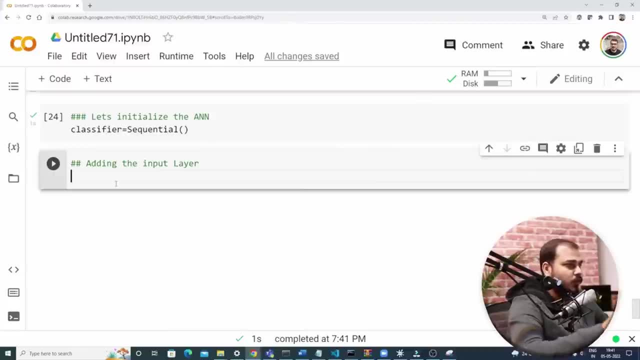 go and see my X train shape. they are 11 inputs. so definitely in the input layer inputs. so definitely in the input layer inputs. so definitely in the input layer. I need to have 11 nodes, so what I will do. I need to have 11 nodes, so what I will do. 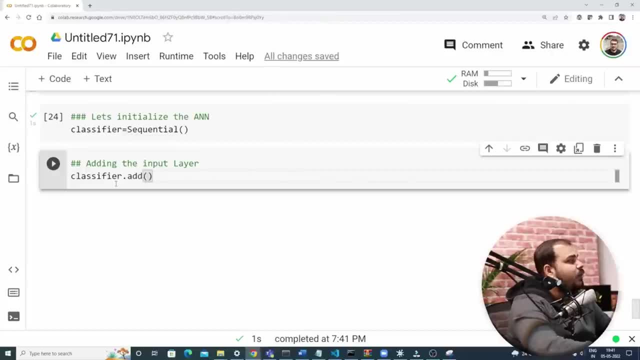 I need to have 11 nodes. so what I will do is that I will say classifier dot add. is that I will say classifier dot add? is that I will say classifier dot add. now what I need to add, as I said you. now what I need to add, as I said you. 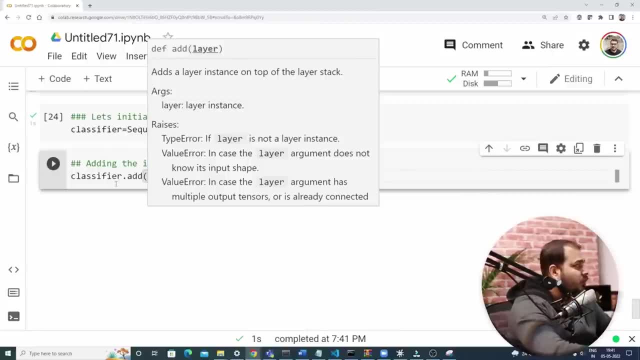 now what I need to add. as I said you that I have to use dense layer to add that I have to use dense layer to add that I have to use dense layer to add the input hidden layer and everything so the input hidden layer and everything so. 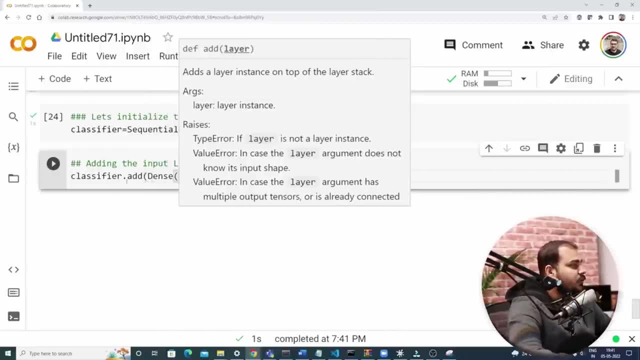 the input hidden layer and everything. so here I'm specifically going to use dense. here I'm specifically going to use dense. here I'm specifically going to use dense. and this dense- see you internally, I'm. and this dense see you internally, I'm, and this dense see you internally. I'm going to basically use dense now inside. 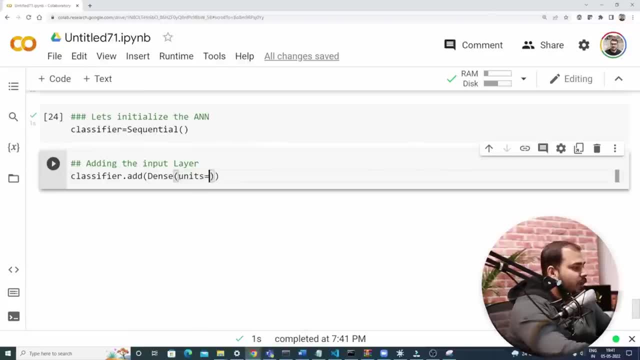 going to basically use dense now inside. going to basically use dense now inside this dense. I will be seeing parameters. this dense, I will be seeing parameters- this dense. I will be seeing parameters like units. okay, so, how many units I need like units? okay, so, how many units I need. 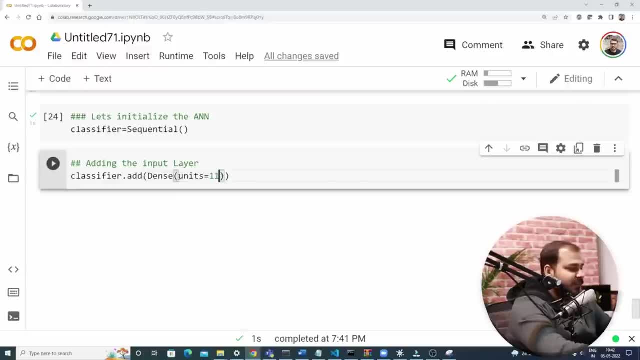 like units. okay, so how many units I need to add over 11? okay, so, 11 units we to add over 11. okay, so, 11 units we to add over 11. okay, so, 11 units we specifically need to add, and then I will specifically need to add and then I will. 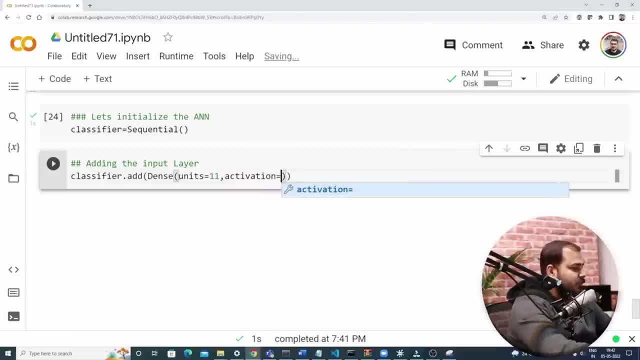 specifically need to add, and then I will also be trying to add the activation. also be trying to add the activation, also be trying to add the activation function: activation function, which is function, activation function, which is function. activation function, which is called as the relu. okay, this will get. 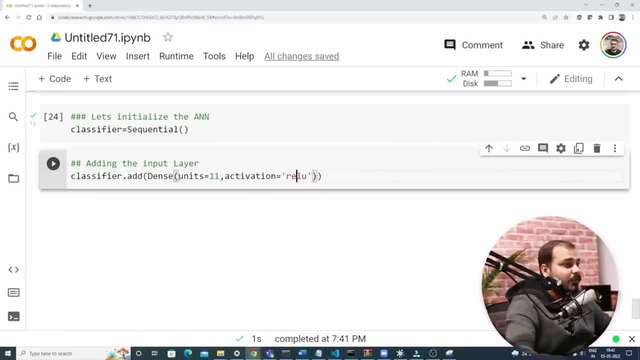 called as the relu. okay, this will get called as the relu. okay, this will get applied to the next layer. relu will get applied to the next layer. relu will get applied to the next layer. relu will get applied to the next upcoming layer. okay, applied to the next upcoming layer. okay. 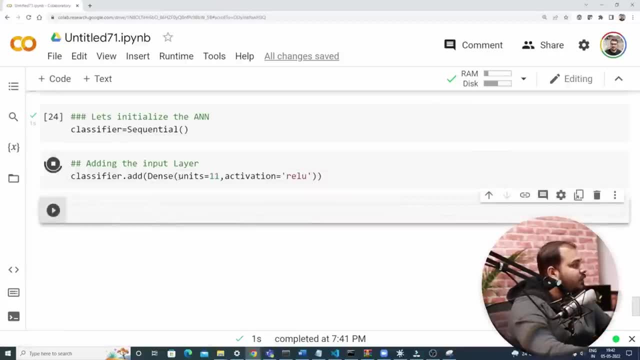 applied to the next upcoming layer. okay, so here only we need to specify with. so here only we need to specify with. so here only we need to specify with respect to that. so here is my classifier: respect to that. so here is my classifier: respect to that. so here is my classifier. I have actually created the input layer. 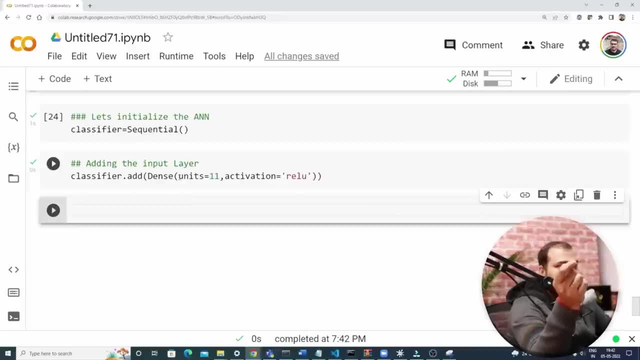 I have actually created the input layer. I have actually created the input layer. the number of input nodes have actually the number of input nodes. have actually the number of input nodes have actually told until the next layer? what told until the next layer? what told until the next layer? what activation function will get applied? I? 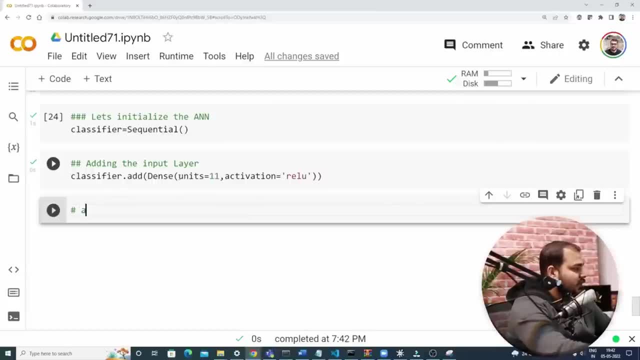 activation function will get applied. I activation function will get applied. I have actually told okay now coming to the. have actually told okay now coming to the. have actually told okay now coming to the second one: adding the second input. second one: adding the second input. second one: adding the second input layer of first hidden layer. sorry, first 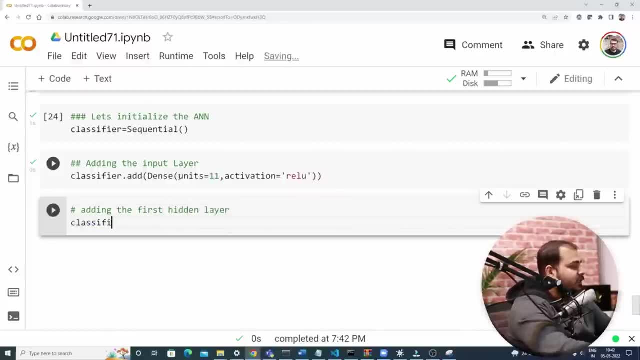 layer of first hidden layer. sorry, first layer of first hidden layer. sorry, first hidden layer. now to add it again. what I hidden layer now. to add it again. what I hidden layer now. to add it again. what I will say: I will say classifier dot add. will say I will say classifier dot add. 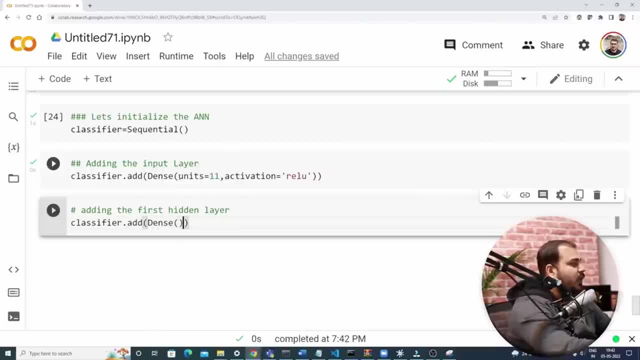 will say I will say classifier, dot, add, and here I'm basically going to again, and here I'm basically going to again, and here I'm basically going to again, take dance. and let's say that in my take dance, and let's say that in my take dance, and let's say that in my first hidden layer I'm just going to. 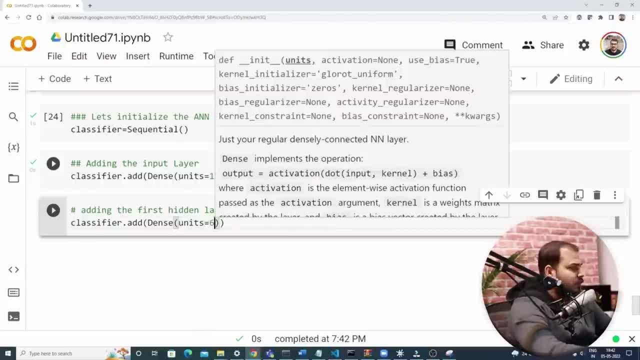 first hidden layer. I'm just going to first hidden layer. I'm just going to consider six units: okay. six, six neurons. consider six units, okay. six, six neurons. consider six units. okay, six, six neurons. or seven neurons, whatever you want. okay. or seven neurons, whatever you want okay. 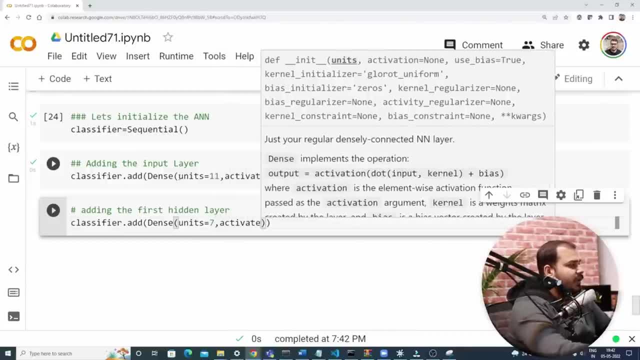 or seven neurons, whatever you want. okay, seven neurons, so seven neurons. I'm going seven neurons, so seven neurons. I'm going seven neurons, so seven neurons I'm going to basically use, and then I'm going to to basically use, and then I'm going to basically use, and then I'm going to basically say that activation function. 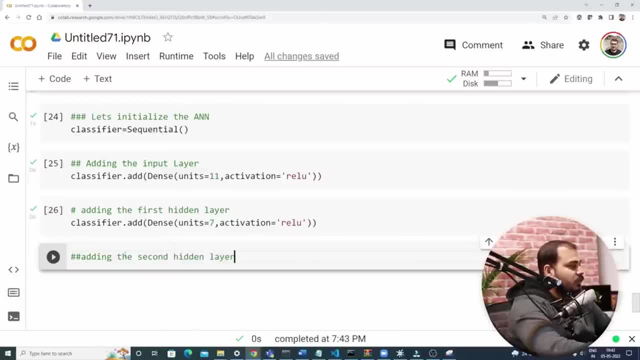 to basically say that activation function. to basically say that activation function, let's say I'm going to just add seven. let's say I'm going to just add seven. let's say I'm going to just add seven neurons. so six neurons, whatever you want. neurons. so six neurons, whatever you want. 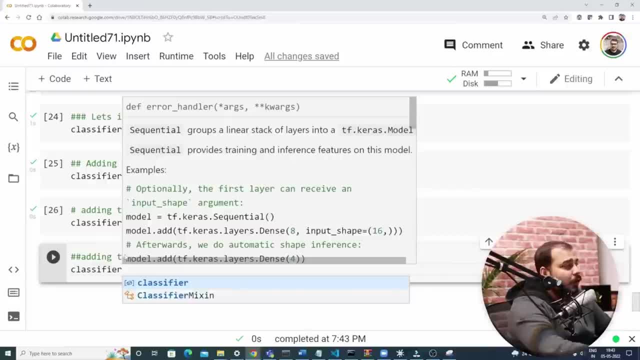 neurons, so six neurons, whatever you want. okay, there are techniques. how to find. okay, there are techniques how to find. okay, there are techniques how to find out that, how many number of hidden out that, how many number of hidden out that, how many number of hidden neurons needs to be added. but here will 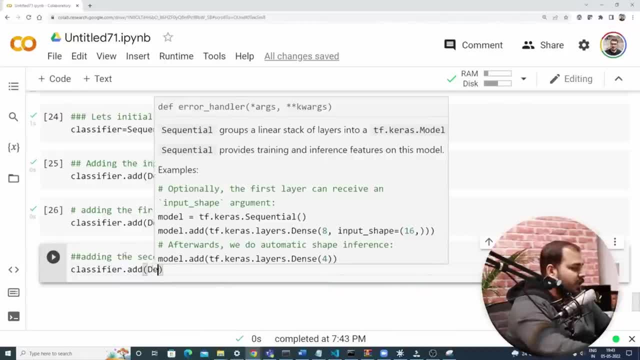 neurons needs to be added, but here will neurons needs to be added, but here will not focus on much on that, because later not focus on much on that, because later not focus on much on that, because later on we'll try to see that. so here I'm. 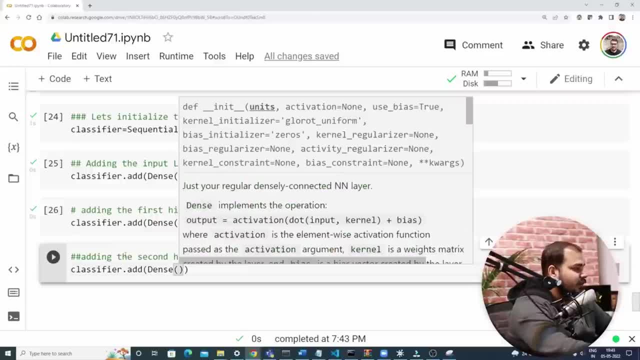 on, we'll try to see that. so here I'm on, we'll try to see that. so here I'm again going to use dense and dense will again going to use dense and dense will again going to use dense and dense will basically have different different. basically have different different. 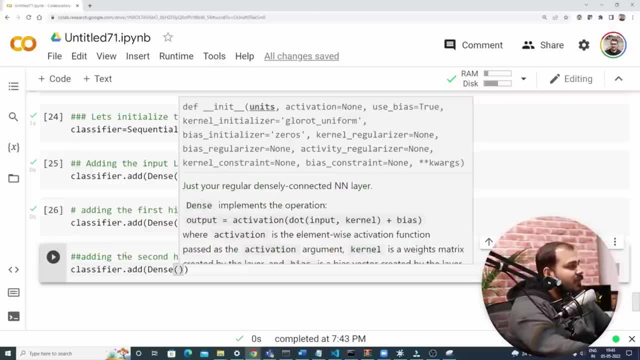 basically have different, different parameters like units activation function, parameters like units activation function, parameters like units activation function, bias and all we can basically add it up, bias and all we can basically add it up, bias and all we can basically add it up. okay, so here I'm basically going to say: 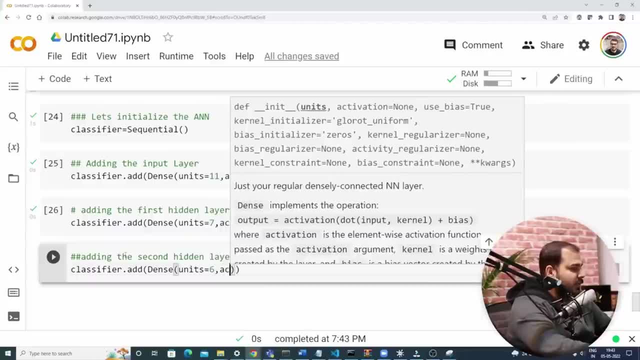 okay. so here I'm basically going to say okay. so here I'm basically going to say: units is equal to six and let's say my units is equal to six. and let's say my units is equal to six. and let's say my activation function is value, okay, value. 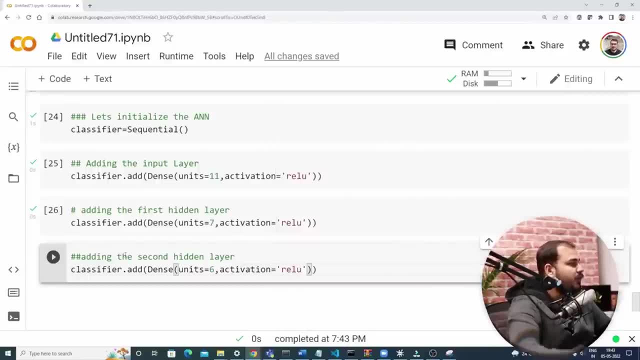 activation function is value okay, value activation function is value okay, value okay. so I'll be basically giving in the okay. so I'll be basically giving in the okay. so I'll be basically giving in the codes. if you don't want to give in the codes, if you don't want to give in the 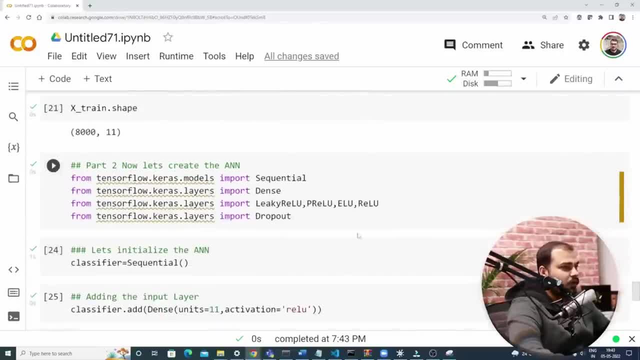 codes. if you don't want to give in the codes, you can directly name this value codes. you can directly name this value codes. you can directly name this value itself wherever you want. okay, so that is itself wherever you want. okay, so that is itself. wherever you want. okay, so that is also available. so here I've added my. 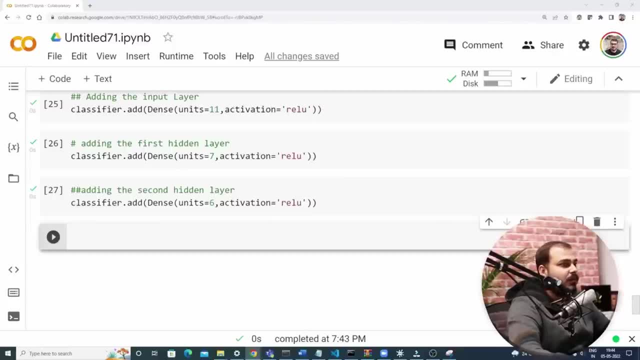 also available. so here I've added my also available. so here I've added my second hidden layer again okay, and we second hidden layer again okay, and we second hidden layer again okay, and we are basically going to do this okay, and are basically going to do this, okay, and 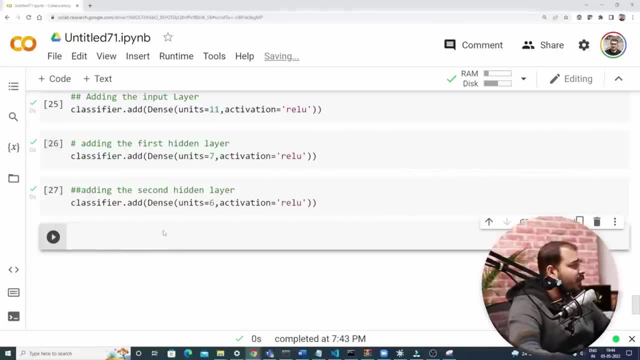 are basically going to do this, okay, and I think we are going in the right stage. I think we are going in the right stage. I think we are going in the right stage. okay, and finally we will add our output. okay, and finally we will add our output. 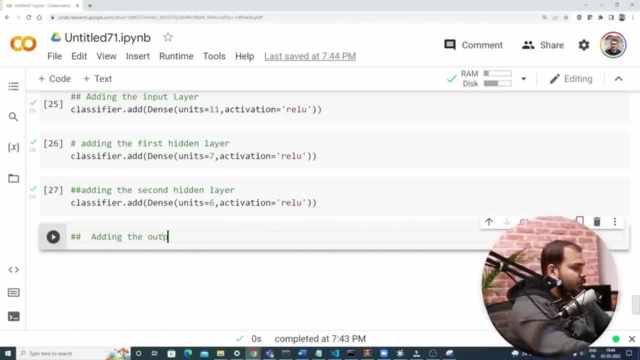 okay, and finally, we will add our output layer. so adding the output layer. okay, layer, so adding the output layer. okay, layer, so adding the output layer. okay, now adding the output layer again. I'll now adding the output layer again. I'll now adding the output layer again. I'll say classifier dot add and then I'll be. 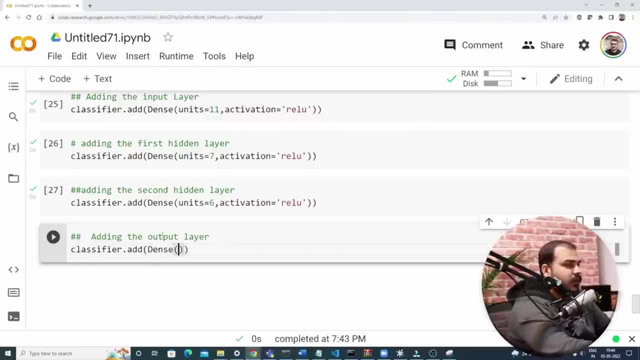 say classifier dot add, and then I'll be say classifier dot add, and then I'll be using a dense and dense and I'll be using a dense and dense and I'll be using a dense and dense and I'll be saying that, okay, fine, I, what I will do is: 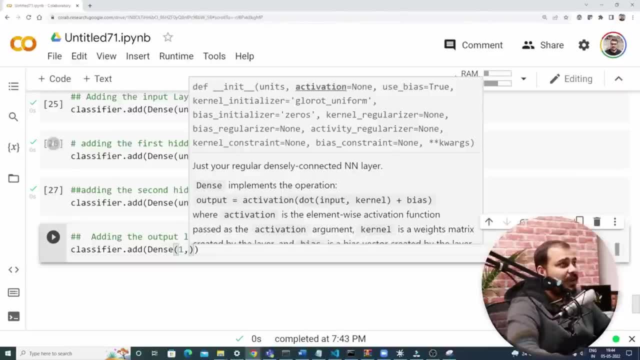 saying that, okay, fine, I. what I will do is saying that, okay, fine, I. what I will do is that I'll just say one neuron. because that I'll just say one neuron, because that I'll just say one neuron, because I actually need to focus on that also. 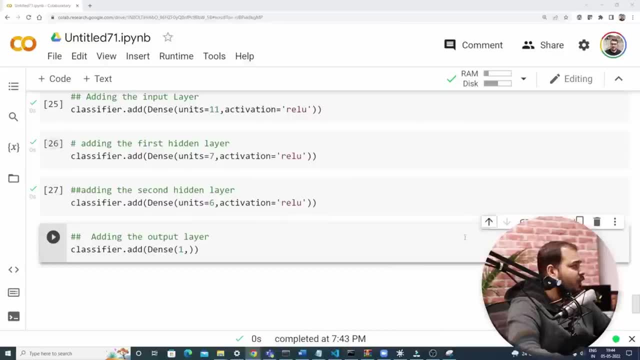 I actually need to focus on that also. I actually need to focus on that also, because now this is a binary, because now this is a binary, because now this is a binary classification, I just require one neuron classification. I just require one neuron classification. I just require one neuron. and here, tell me any guesses, just pause. 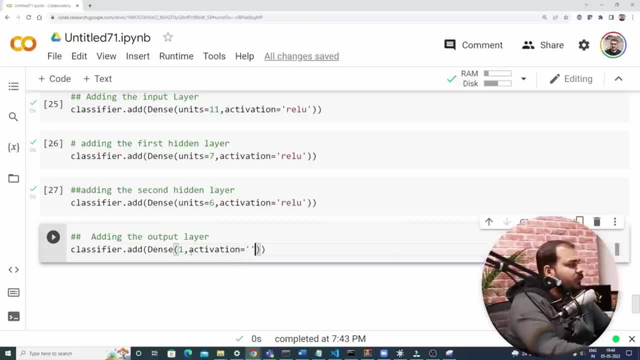 and here tell me any guesses. just pause. and here tell me any guesses. just pause the video and let me know what is the the video. and let me know what is the the video. and let me know what is the activation function. the activation. activation function, the activation. 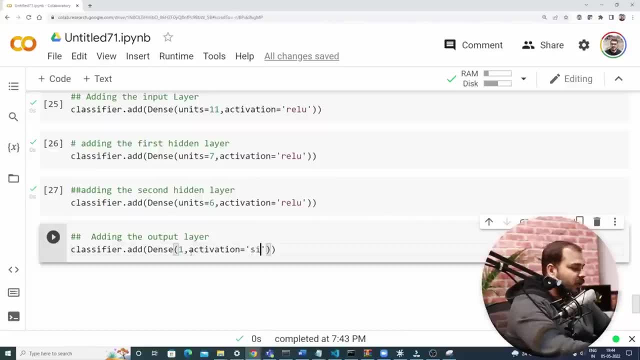 activation function. the activation function over here, since this is a binary function over here, since this is a binary function over here, since this is a binary classification problem which we have classification problem, which we have classification problem which we have learned it, that is basically Sigma okay. learned it, that is basically Sigma, okay. 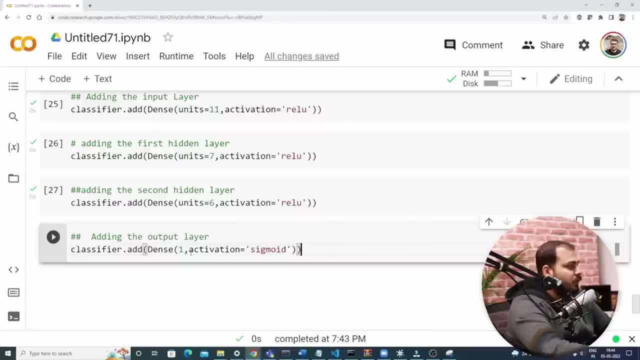 learned it. that is basically Sigma. okay, so Sigma, we are basically going to add. so Sigma, we are basically going to add. so Sigma, we are basically going to add over here: perfect, so, let's execute this over here. perfect, so, let's execute this over here. perfect, so, let's execute this. let's execute this now. perfect, this is. 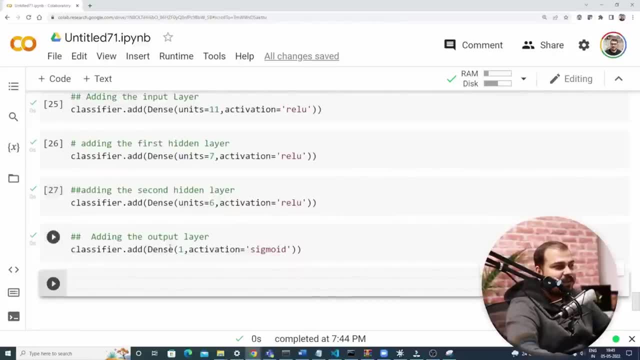 let's execute this now. perfect. this is: let's execute this now- perfect. this is got executed. my classifier neuron, the, got executed. my classifier neuron, the, got executed. my classifier neuron- the entire neural network is ready now. all I entire neural network is ready now. all I entire neural network is ready now. all I have to do is that quickly, quickly. 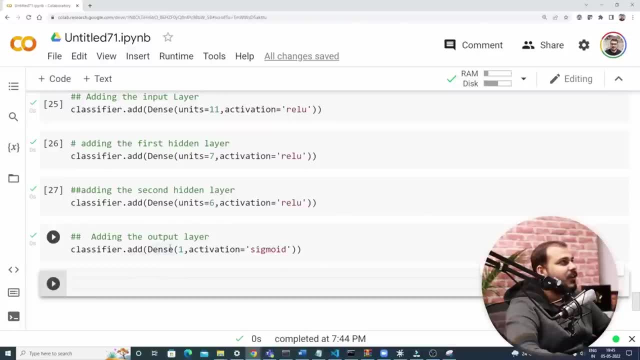 have to do? is that quickly, quickly have to do? is that quickly, quickly, quickly, train train my entire? you know quickly, train train my entire, you know quickly, train train my entire. you know the neural network and let's see how do the neural network and let's see how do. 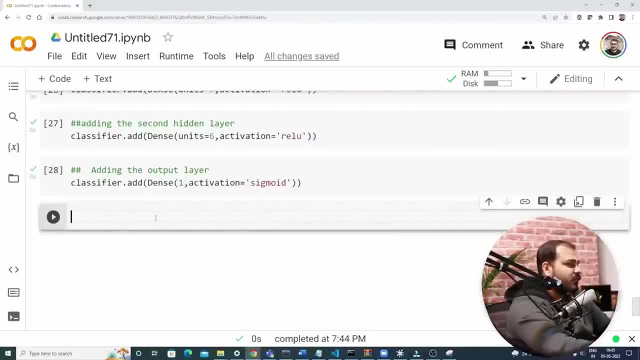 the neural network. and let's see, how do we train our entire neural network? okay, we train our entire neural network. okay, we train our entire neural network. okay, so here what I'm actually going to sue. so here what I'm actually going to sue. so here what I'm actually going to sue. I'm going to say: classifier, dot, compile. 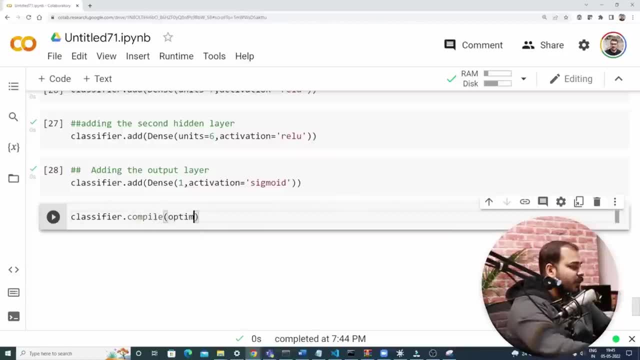 I'm going to say classifier dot compile. I'm going to say classifier dot compile. okay, we have to bustable compile the okay, we have to bustable compile the okay, we have to bustable compile the entire neural network. and here the first entire neural network. and here the first. 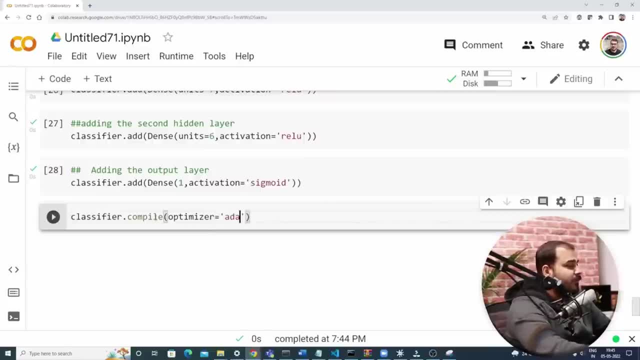 entire neural network. and here, the first thing that we are going to give is thing that we are going to give is thing that we are going to give is optimizer. what optimizer do we give we optimizer? what optimizer do we give we optimizer? what optimizer do we give we give Adam optimizer, because it is a best. 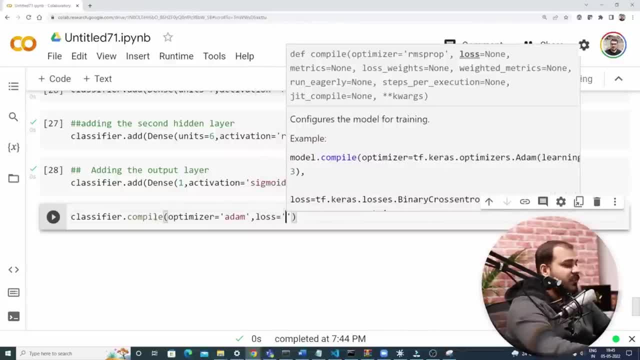 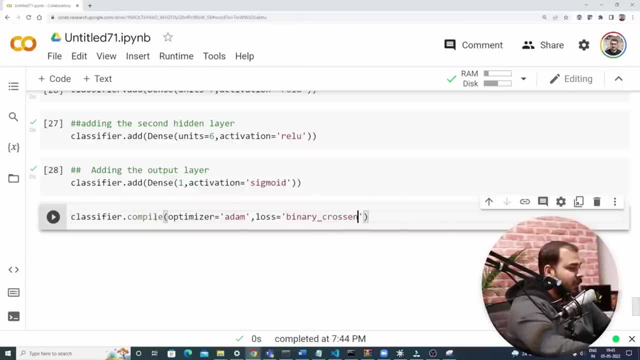 give Adam optimizer because it is a best. give Adam optimizer because it is a best optimizer and apart from that, I also optimizer and apart from that, I also optimizer and apart from that, I also the type of metrics that I'm actually going, the type of metrics that I'm actually going. 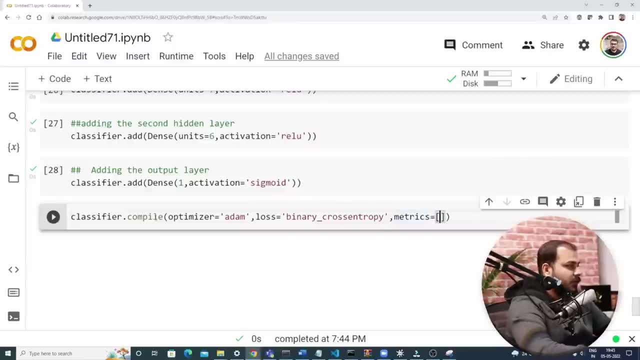 the type of metrics that I'm actually going to focus on. is my accuracy okay? so to focus on? is my accuracy okay? so to focus on? is my accuracy okay? so accuracy, I'm actually going to focus on accuracy. I'm actually going to focus on accuracy. I'm actually going to focus on which will be my metric? okay, so this is. 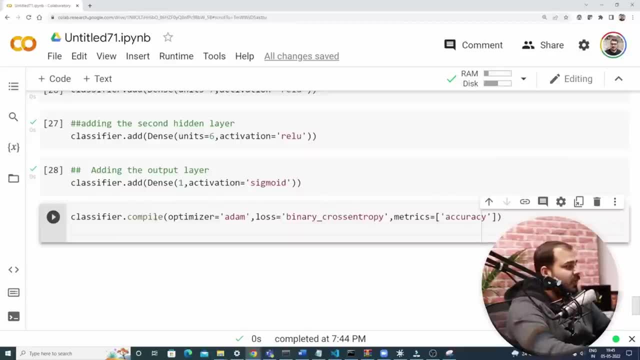 which will be my metric. okay, so this is which will be my metric. okay, so this is it. I think we have done successfully till it. I think we have done successfully till it. I think we have done successfully till here. it's amazing, it's beautiful till here. it's amazing, it's beautiful till. 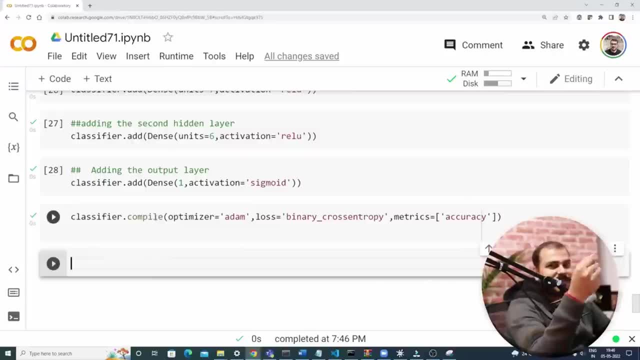 here. it's amazing, it's beautiful till here. we are able to do it, but still you here, we are able to do it, but still you here, we are able to do it, but still you may be thinking, Chris, where is the? may be thinking Chris, where is the? 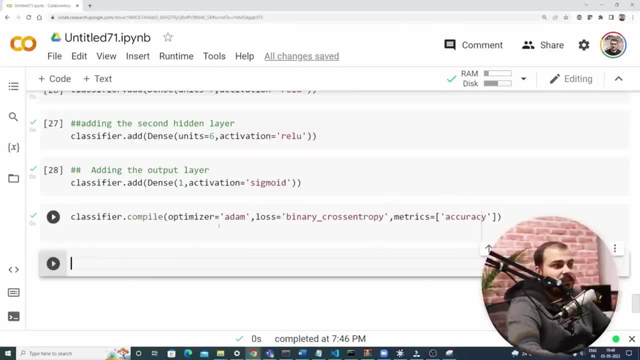 may be thinking: Chris, where is the learning rate right? by default, Adam uses learning rate right. by default, Adam uses learning rate right. by default, Adam uses a learning rate of 0.01. if you really a learning rate of 0.01, if you really a learning rate of 0.01, if you really want to provide your own learning rate. 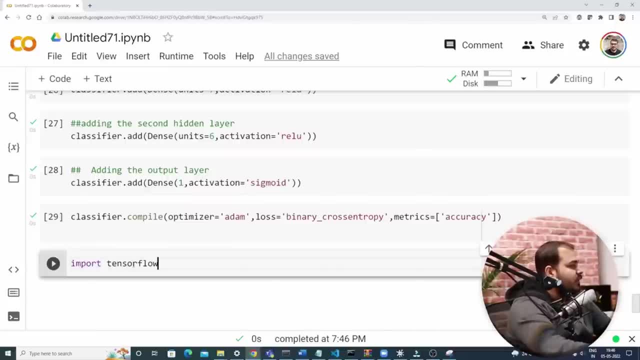 want to provide your own learning rate? want to provide your own learning rate? just say that: import tensorflow. let's just say that import tensorflow. let's just say that import tensorflow. let's say I'm going to import tensorflow and say I'm going to import tensorflow. and 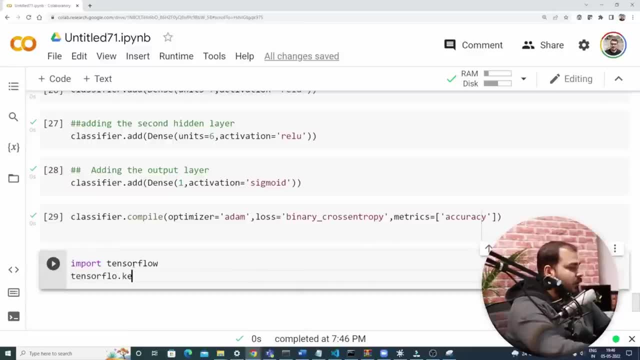 say I'm going to import tensorflow and here I'm just going to say tensorflow, here I'm just going to say tensorflow, here I'm just going to say tensorflow dot keras, dot. optimizers- right dot keras dot. optimizers, right dot keras dot. optimizers: right optimizes dot Adam. okay, we initialize. 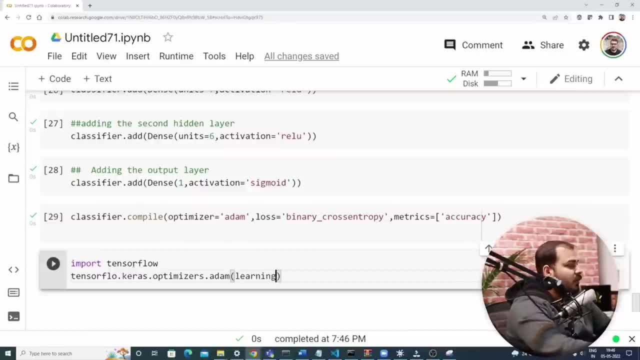 optimizes, dot Adam. okay, we initialize. optimizes, dot Adam. okay, we initialize: Adam like this Adam. and here I can: Adam like this Adam. and here I can Adam like this Adam. and here I can specify my learning rate, learning rate. specify my learning rate, learning rate, specify my learning rate, learning rate. I'll make this as capital, Adam and this. 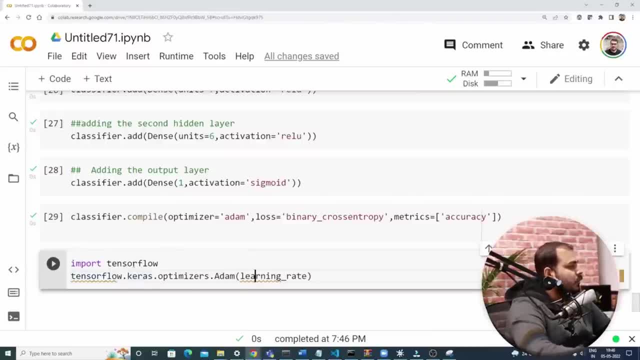 I'll make this as capital Adam and this: I'll make this as capital Adam and this will basically be my tensor flow. okay, will basically be my tensor flow. okay, will basically be my tensor flow. okay, and here I can initialize my learning and here I can initialize my learning. 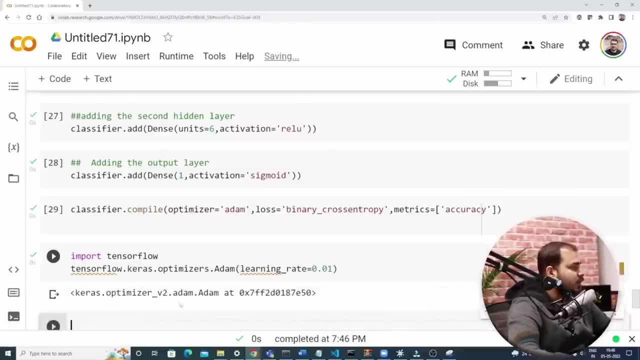 and here I can initialize my learning rate with respect to whatever value I rate. with respect to whatever value I rate with respect to whatever value I want. so if I execute this okay, so here want so. if I execute this okay, so here want so. if I execute this okay, so here you can see that it is a Adam object. I. 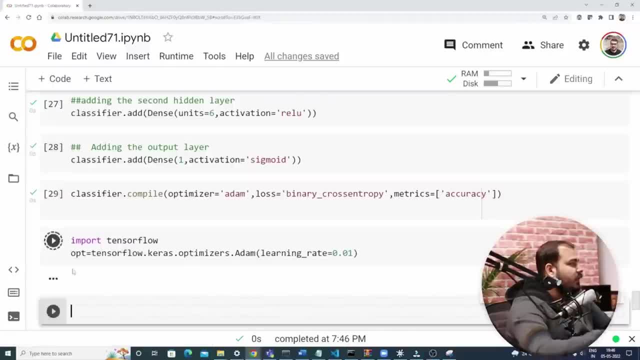 you can see that it is a Adam object. I- you can see that it is a Adam object. I will probably say this, as my optimizer will probably say this, as my optimizer will probably say this as my optimizer: and execute this and this same opt can. and execute this and this same opt can. 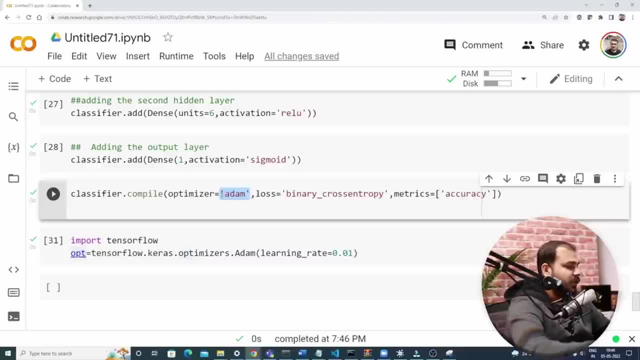 and execute this, and this same opt can basically be put up over here. okay, basically be put up over here. okay, basically be put up over here. okay, instead of using Adam, you can also use. instead of using Adam, you can also use. instead of using Adam, you can also use anything that you want. so, over here. 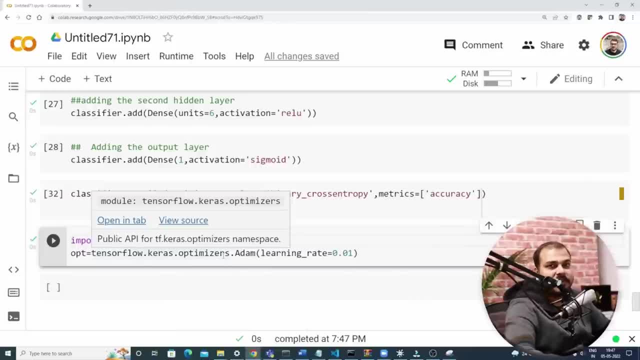 anything that you want so over here, anything that you want so over here inside the optimizers. you have all the inside the optimizers, you have all the inside the optimizers. you have all the options with respect to all the options, with respect to all the options, with respect to all the optimizers that we have discussed, like 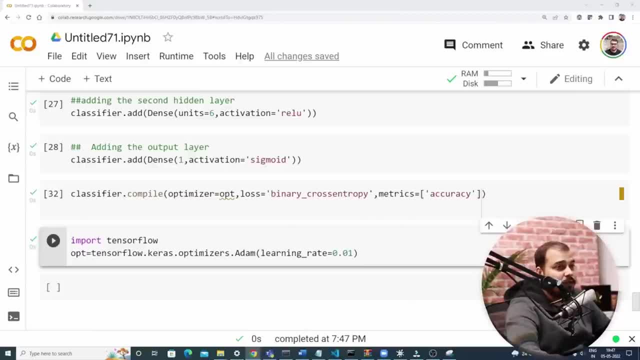 optimizers that we have discussed, like optimizers that we have discussed, like gradient descent and all and all and all gradient descent and all and all and all gradient descent and all and all and all. okay. whatever you want, you can basically okay. whatever you want, you can basically. 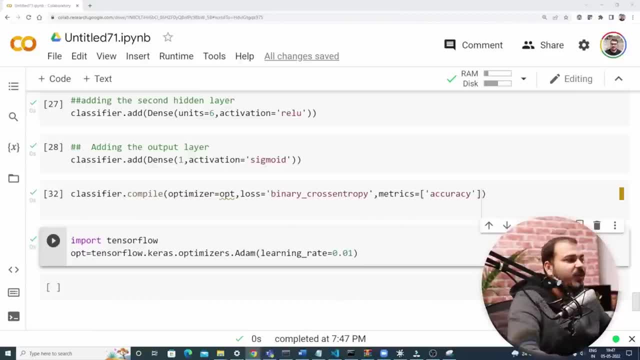 okay, whatever you want, you can basically use it. it is up to you, but I have use it. it is up to you, but I have use it. it is up to you. but I have already told you that Adam optimizers already told you that Adam optimizers. 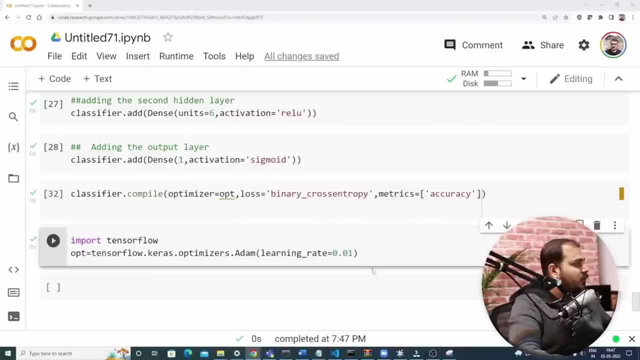 already told you that Adam optimizers are very good when compared to the other, are very good when compared to the other, are very good when compared to the other. optimizes right, so here it is done. optimizes right, so here it is done. optimizes right, so here it is done. everything is done. now is the main thing. everything is done now is the main thing. everything is done now is the main thing- is that we have to really train our. is that we have to really train our. is that we have to really train our neural network right now in order to neural network right now in order to 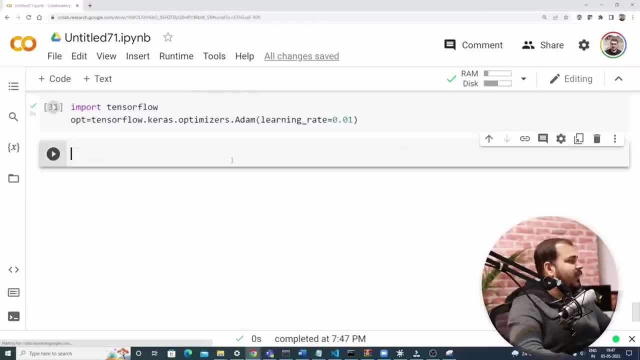 neural network right now, in order to train our neural network. all I will train our neural network, all I will train our neural network. all I will basically be doing is that I will say, basically be doing. is that I will say basically be doing is that I will say, okay, find my model history, okay, model. 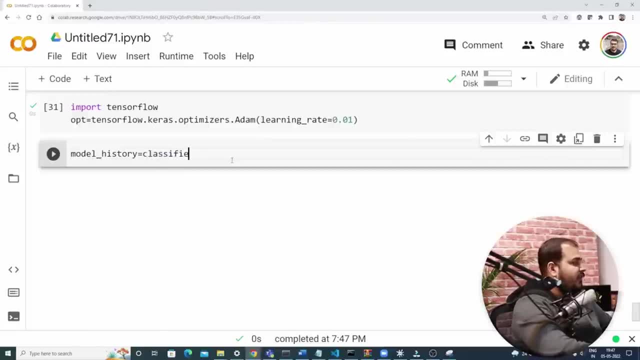 okay, find my model history- okay, model okay, find my model history- okay, model history- okay, will basically be nothing history- okay, will basically be nothing history. okay, will basically be nothing but classifier dot fit. and here I'm but classifier dot fit, and here I'm but classifier dot fit, and here I'm going to give my extreme comma white. 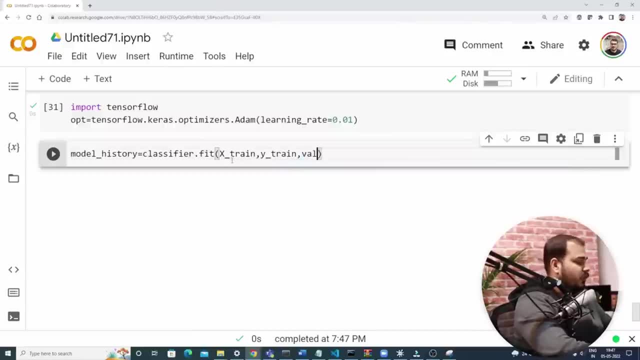 going to give my extreme comma white, going to give my extreme comma white, train okay. and then I'm going to give train okay, and then I'm going to give train okay, and then I'm going to give something called as validation split and something called as validation split, and 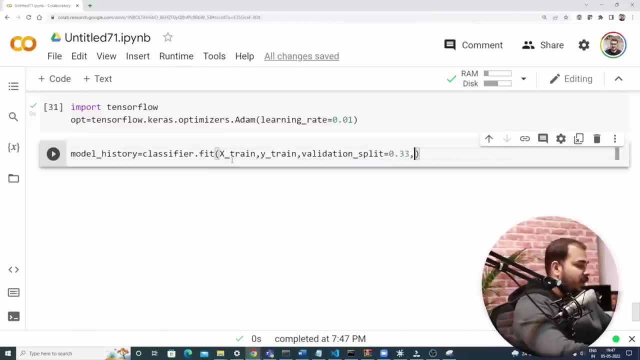 something called as validation split, and apart from that, I'll say 0.33, and there, apart from that, I'll say 0.33, and there, apart from that, I'll say 0.33, and there I can also specify my size right. so by. 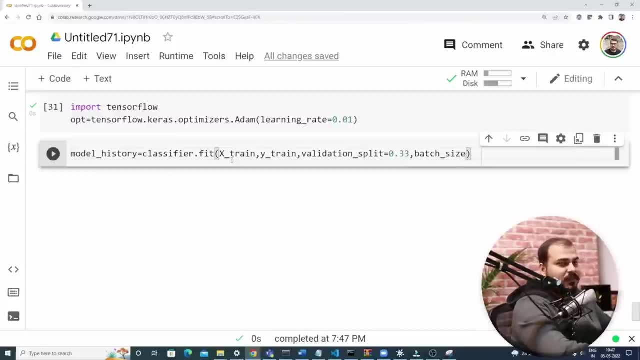 I can also specify my size right. so by: I can also specify my size right. so by size. we have to give it because we know size. we have to give it because we know size. we have to give it because we know that in this also, Ram size will be less. 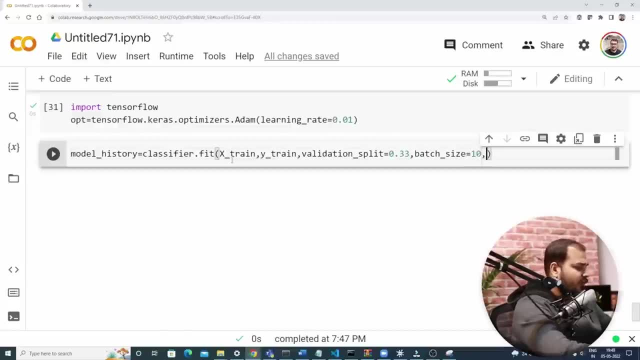 that in this also, Ram size will be less. that in this also, Ram size will be less. so bass size is equal to 10. let's me. so bass size is equal to 10. let's me. so bass size is equal to 10. let's me give a bass size. I'm going to give it. 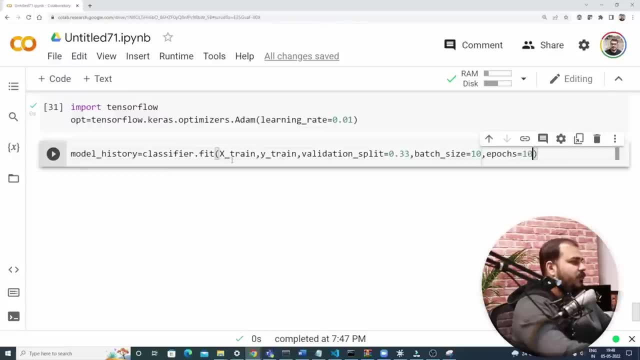 give a bass size, I'm going to give it. give a bass size. I'm going to give it as 10 and epochs. let's say that I'm going as 10 and epochs. let's say that I'm going as 10 and epochs. let's say that I'm going to give it thousand. okay, let's, let's. 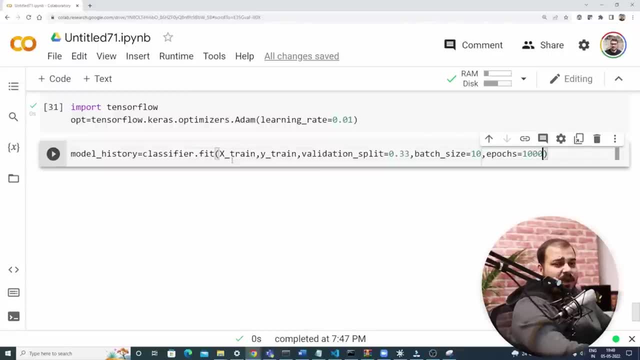 to give it thousand. okay, let's. let's. to give it thousand. okay, let's, let's. let's consider I'm giving thousand epochs. let's consider I'm giving thousand epochs. let's consider I'm giving thousand epochs. you may be saying Krish, are you mad? you may be saying Krish, are you mad? 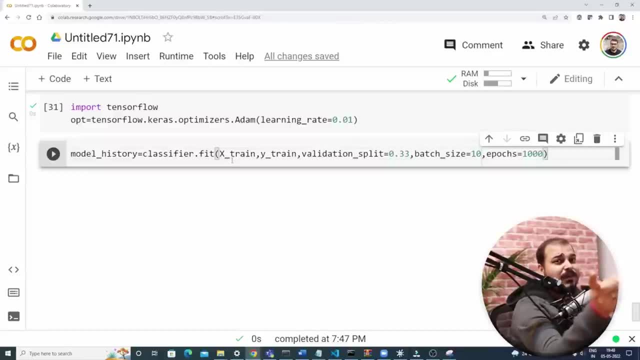 you may be saying: Krish, are you mad? thousand epochs, what will happen this thousand epochs? what will happen this thousand epochs? what will happen? this will keep on running, and that is where will keep on running, and that is where will keep on running, and that is where I'll be talking about early shopping. okay. 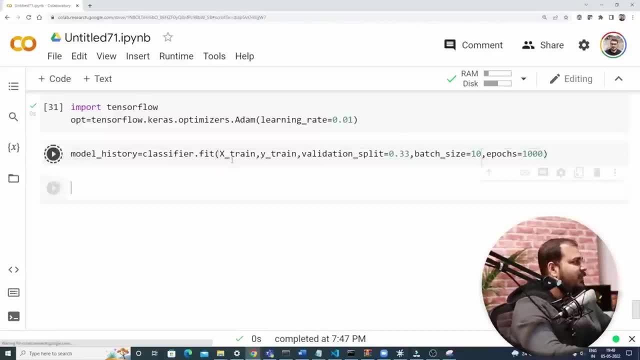 I'll be talking about early shopping. okay, I'll be talking about early shopping, okay. so right now, let's give epochs 1000. so right now, let's give epochs 1000. so right now, let's give epochs 1000 and just execute it, and how smoothly it. 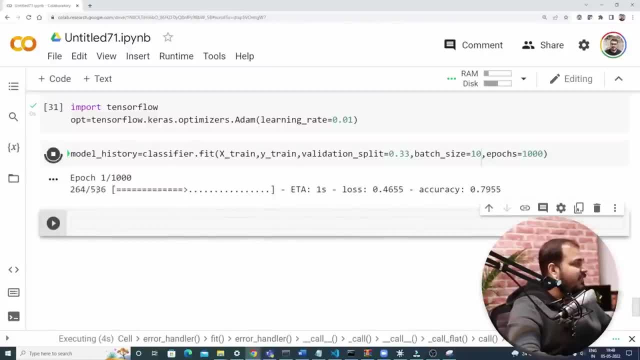 and just execute it and how smoothly it and just execute it and how smoothly it will start executing. and here you will be, will start executing, and here you will be, will start executing and here you will be able to see that 560 536 iterations, able to see that 560 536 iterations. 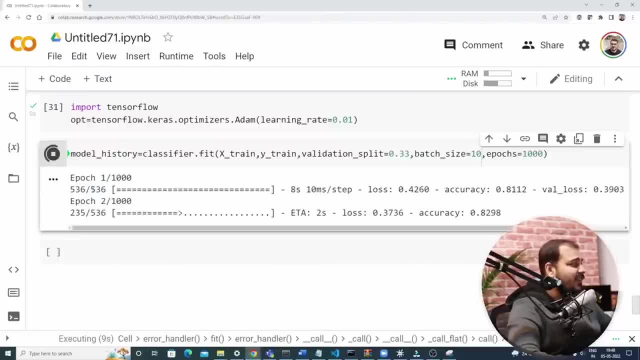 able to see that 560, 536 iterations are there now. you calculate based on the. are there now? you calculate based on the. are there now? you calculate based on the data set size: why 536 is there and here. data set size why 536 is there and here. 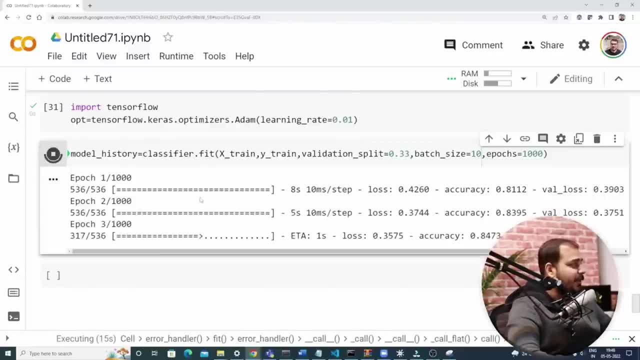 data set size. why 536 is there? and here we have also applied validation split. we have also applied validation split. we have also applied validation split. right cross validation. we basically say right cross validation. we basically say right cross validation. we basically say why 536 iteration is there? just do the. 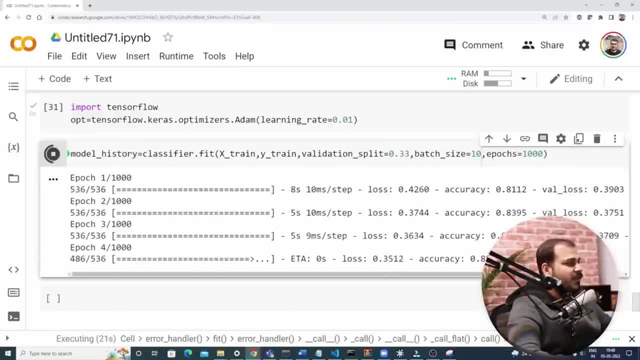 why 536 iteration is there? just do the. why 536 iteration is there? just do the calculation. you know, based on the number calculation. you know, based on the number calculation, you know, based on the number of epochs and bass size right now here of epochs and bass size right now here. 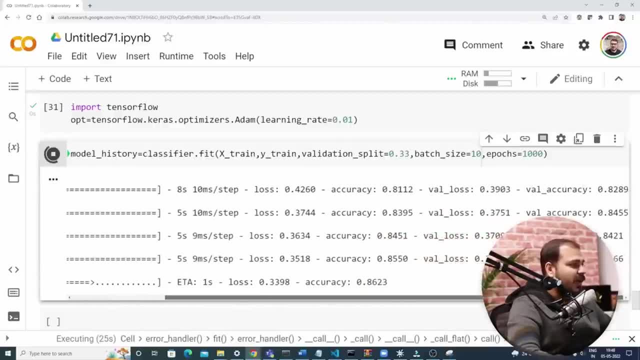 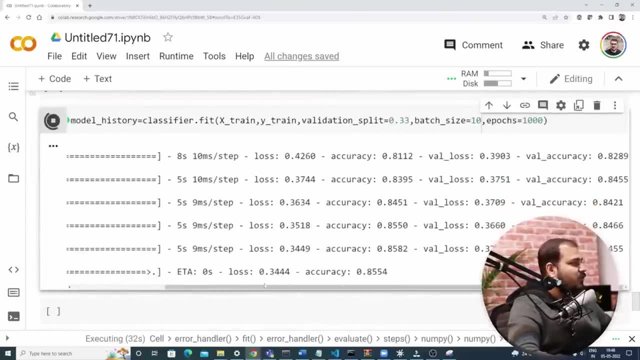 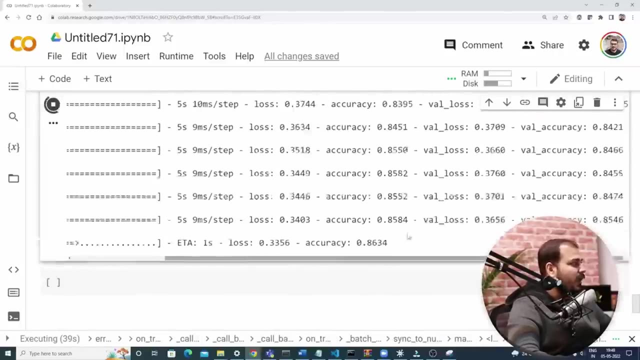 of epochs and bass size right now. here you'll be able to see that my accuracy, you'll be able to see that my accuracy, you'll be able to see that my accuracy is increasing. my validation loss is going is increasing. my validation loss is going is increasing. my validation loss is going little decrease as we go ahead. so we little decrease as we go ahead. so we little decrease as we go ahead. so we will wait, wait, wait, and we'll see that will wait, wait, wait and we'll see that will wait, wait, wait and we'll see that after some point of time. you know my. 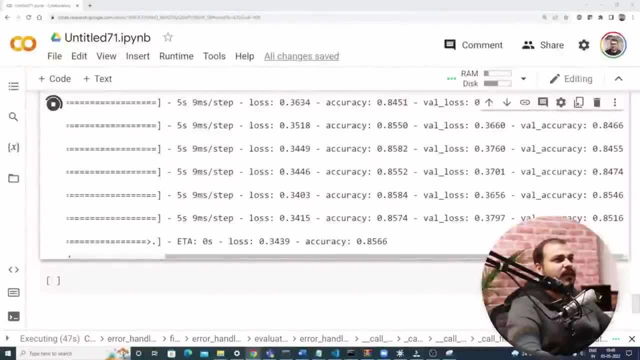 after some point of time, you know my, after some point of time, you know my accuracy will be almost stagnant. so at accuracy will be almost stagnant. so at accuracy will be almost stagnant. so at that point of time, what should I do we? that point of time? what should I do we? 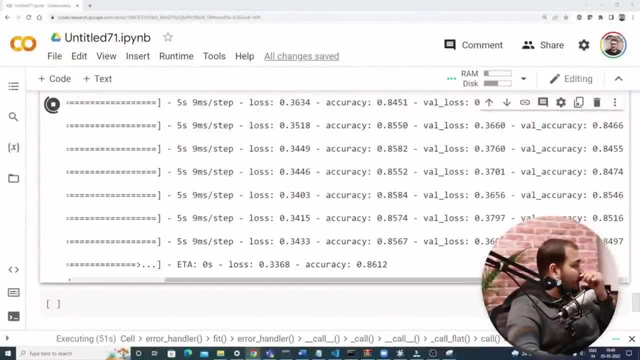 that point of time. what should I do? we will discuss about it, okay, okay, so here will discuss about it. okay, okay, so here will discuss about it, okay, okay, so here it is. so here you can see the accuracy. it is so here you can see the accuracy. 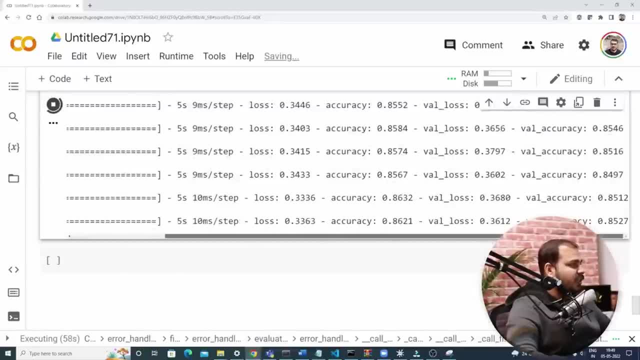 it is. so here you can see: the accuracy is going going up: now it is an 86%. is going going up: now it is an 86%. is going going up: now it is an 86%. validation accuracy is in 85%, which is: 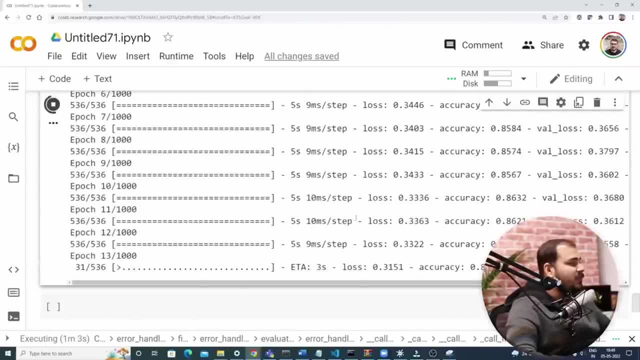 validation accuracy is in 85%, which is validation accuracy is in 85%, which is going amazing right, but we have. we are going amazing right, but we have. we are going amazing right, but we have. we are running this for thousand epochs, just running this for thousand epochs, just. 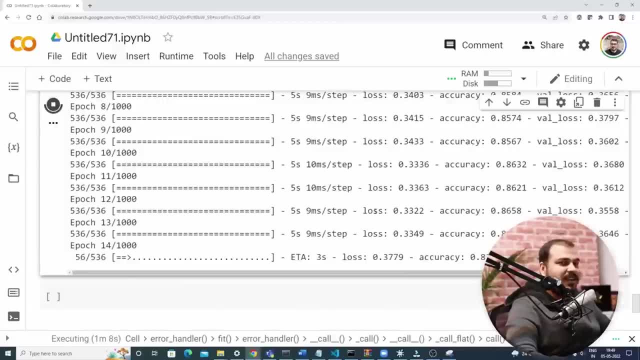 running this for thousand epochs, just imagine thousand epochs. okay, so we are imagine thousand epochs. okay, so we are imagine thousand epochs. okay. so we are definitely going to put early stopping, definitely going to put early stopping, definitely going to put early stopping, because the thing, the idea that you will 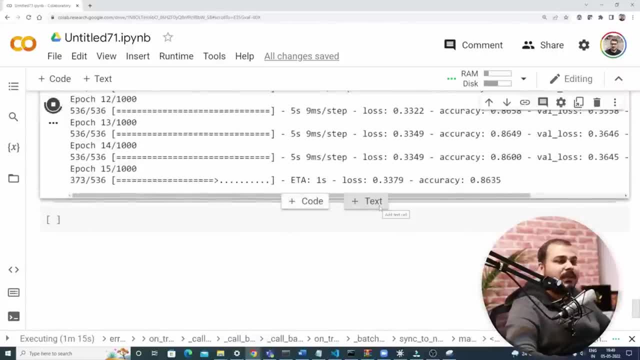 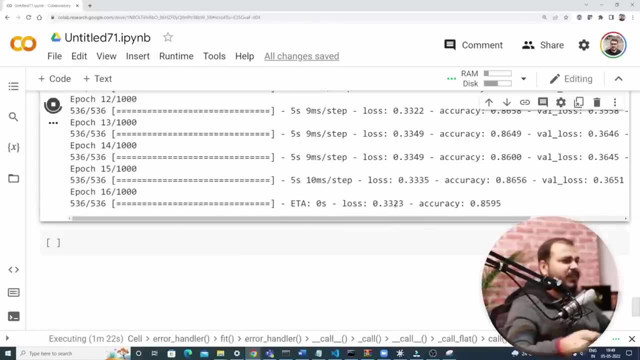 because the thing, the idea that you will, because the thing, the idea that you will be thinking, is that what should be my be thinking, is that what should be my be thinking, is that what should be my epochs, and then you will probably see a epochs, and then you will probably see a. 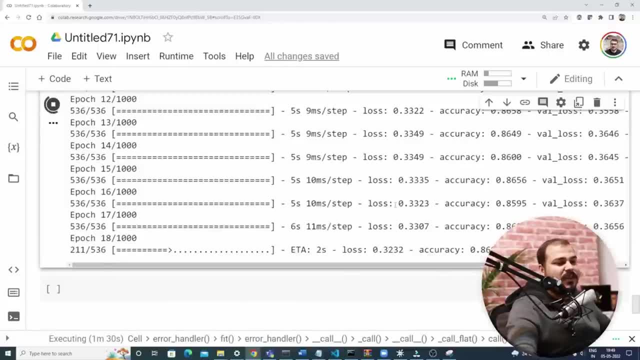 epochs. and then you will probably see a kind of observation that the accuracy kind of observation, that the accuracy kind of observation that the accuracy will not be increasing at all, so the will not be increasing at all, so the will not be increasing at all. so the main question is that: how do we decide? 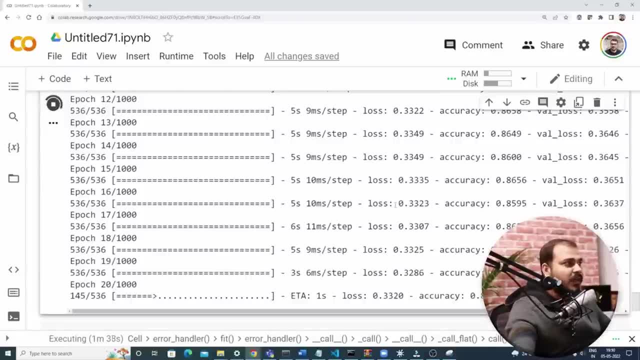 main question is that: how do we decide? main question is that: how do we decide that when the accuracy should how many, that when the accuracy should how many, that when the accuracy should how many number of epochs, we should basically number of epochs, we should basically number of epochs, we should basically stop right. so here you can see that it. 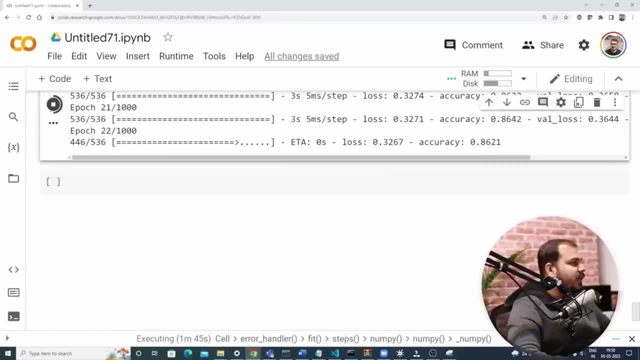 stop right. so here you can see that it stop right. so here you can see that it is going on quickly in an efficient way. is going on quickly in an efficient way. is going on quickly in an efficient way, or 86 percent now, here you can see right. 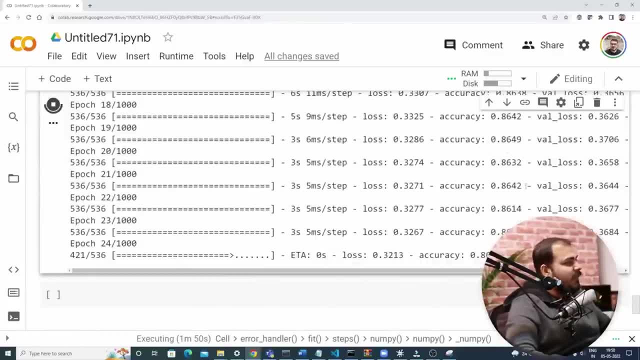 or 86 percent. now here you can see right- or 86 percent. now here you can see right: 86.42, 86.49, 86.32. it is 6.42, 86.14. it is 86.42, 86.49, 86.32. it is 6.42, 86.14 it is. 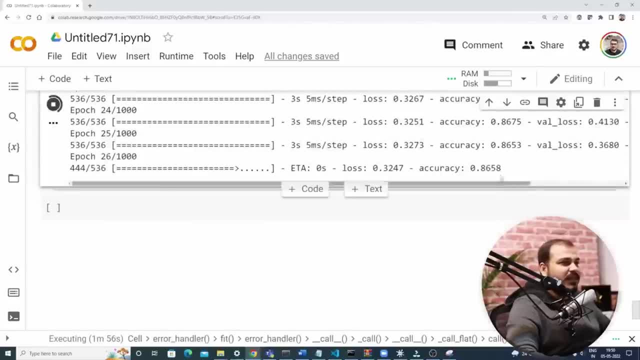 86.42, 86.49, 86.32. it is 6.42, 86.14. it is rotating there right. it is rotating, rotating there right. it is rotating, rotating there right. it is rotating there itself, right it is not increasing. or there itself, right, it is not increasing, or. 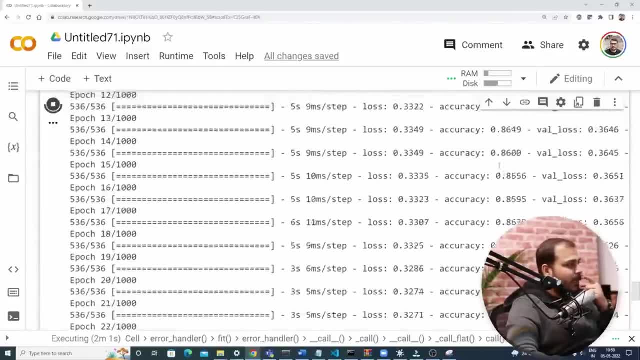 there itself. right, it is not increasing or it is not reducing okay, so that is the. it is not reducing okay, so that is the. it is not reducing okay. so that is the thing over here, that is happening, okay. thing over here, that is happening, okay. thing over here, that is happening, okay. validation split basically says that and 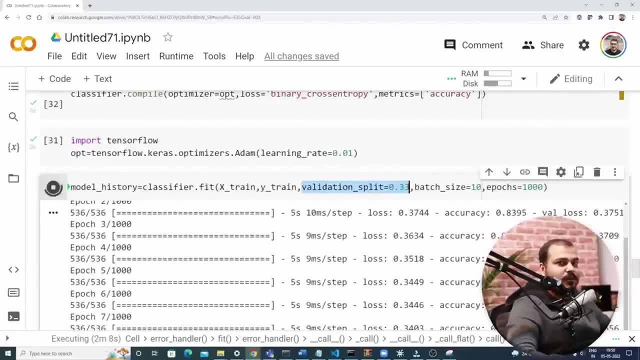 validation split basically says that, and validation split basically says that and that training data set is there. you, that training data set is there. you, that training data set is there. you are just taking somewhere around 66, are just taking somewhere around 66, are just taking somewhere around 66 percentage of the data and you are. 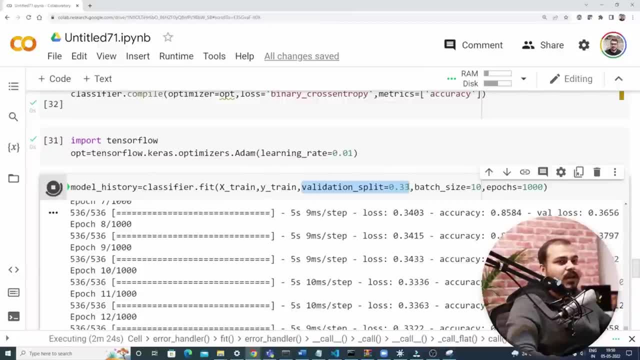 percentage of the data and you are percentage of the data and you are basically using it and you are dividing, basically using it, and you are dividing, basically using it, and you are dividing the data set with respect to every epoch, the data set with respect to every epoch. 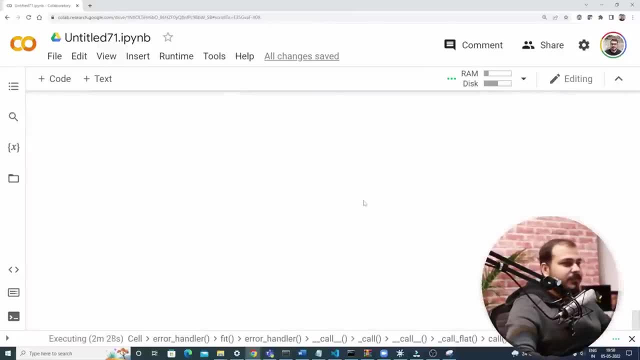 the data set with respect to every epoch, so that it takes up for the training, so that it takes up for the training, so that it takes up for the training purpose. okay, uh, okay. now, here you can see 86, 86, 86, so. uh, okay, now, here you can see 86, 86, 86, so. 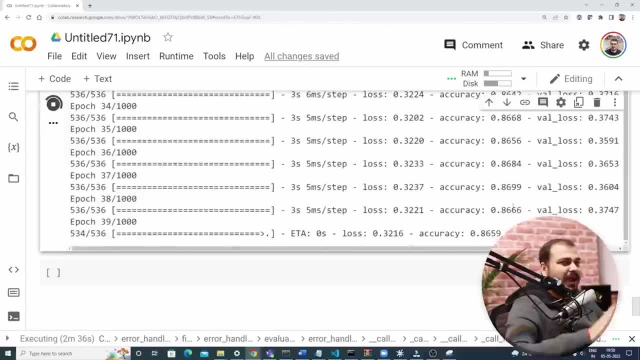 uh, okay, now here you can see 86 86, 86. so what i am actually going to do over what i am actually going to do, over what i am actually going to do over here, it is going to here, it is going to here, it is going to, you know, iterate in that same accuracy. so you know, iterate in that same accuracy. so you know, iterate in that same accuracy. so what i am going to do, i'm just going to what i am going to do. i'm just going to what i am going to do. i'm just going to do the stop part. 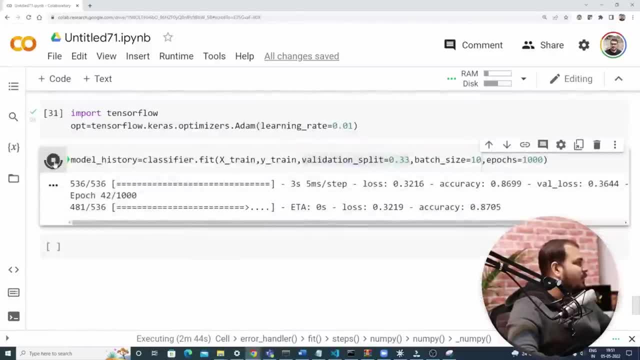 do the stop part. do the stop part. let's see whether i can do the stop part. let's see whether i can do the stop part. let's see whether i can do the stop part. so, so, so, oh okay, oh okay, oh okay. uh, i'm just going to stop it, let's see. 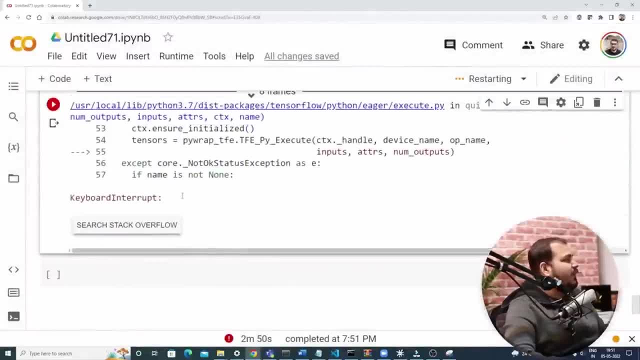 uh, i'm just going to stop it. let's see, uh, i'm just going to stop it, let's see whether it will stop, whether it will stop, whether it will stop. so, yes, i've stopped it over here, okay, key. so yes, i've stopped it over here, okay, key. 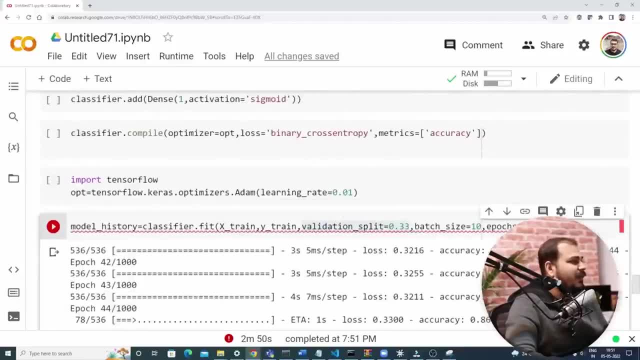 so, yes, i've stopped it over here. okay, key and keyboard interrupt because i don't, and keyboard interrupt because i don't. and keyboard interrupt because i don't want to go with 3500, want to go with 3500, want to go with 3500 thousand epochs, because i know that at 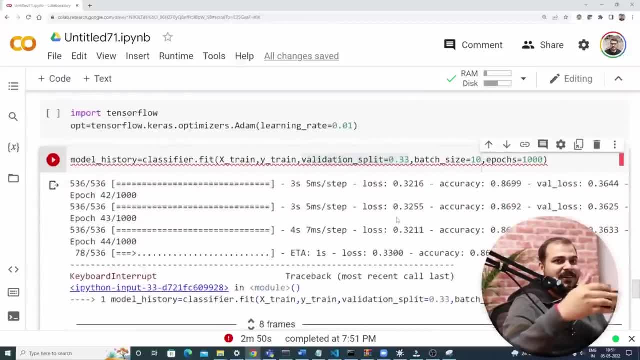 thousand epochs, because i know that, at thousand epochs, because i know that at one point of time, one point of time, one point of time, this is really uh, you know, uh, this is really, uh, you know, uh, this is really uh, you know, uh, what, what, what is happening over here? 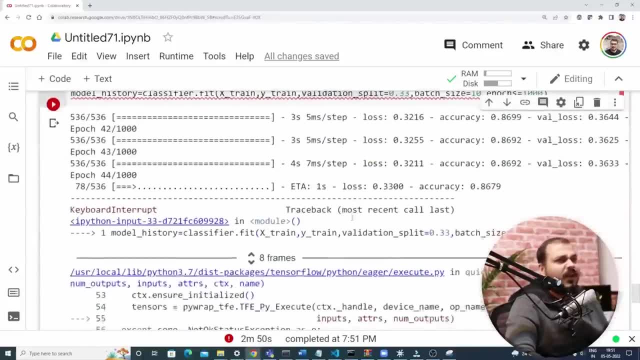 what, what? what is happening over here? what, what? what is happening over here? the accuracy is becoming almost same. the accuracy is becoming almost same. the accuracy is becoming almost same. right, so what do i do? where do i stop? right, so what do i do? where do i stop? 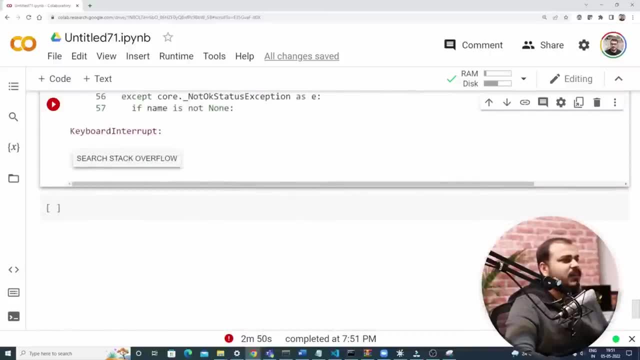 right. so what do i do? where do i stop? exactly okay. or let me just say that: exactly okay. or let me just say that exactly okay. or let me just say that: let's, let's consider, over here, i'm just, let's, let's consider, over here, i'm just. 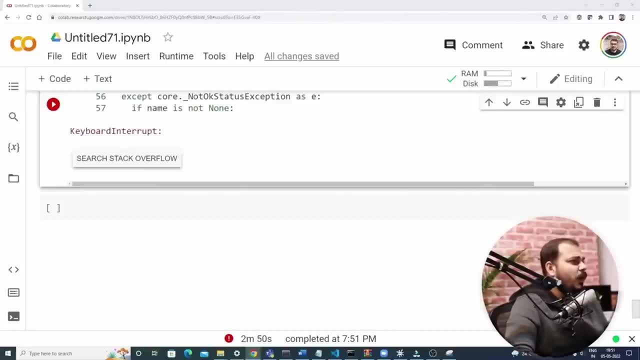 let's, let's consider over here. i'm just going to copy and paste some code, okay, going to copy and paste some code. okay, going to copy and paste some code, okay, and probably we'll try to plot it. okay, and probably we'll try to plot it okay. 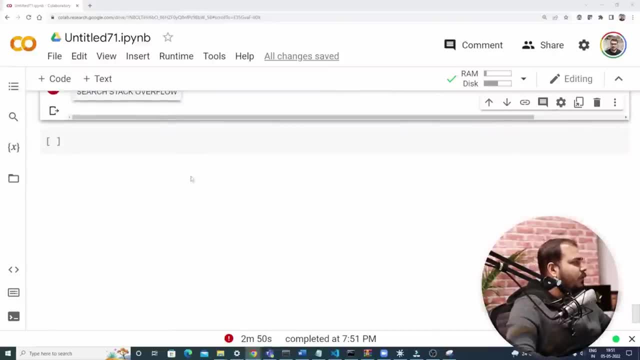 and probably we'll try to plot it. okay, let's say whatever it has been trained. let's say whatever it has been trained. let's say whatever it has been trained. till how many epochs? like till 44 epochs. till how many epochs like till 44 epochs. 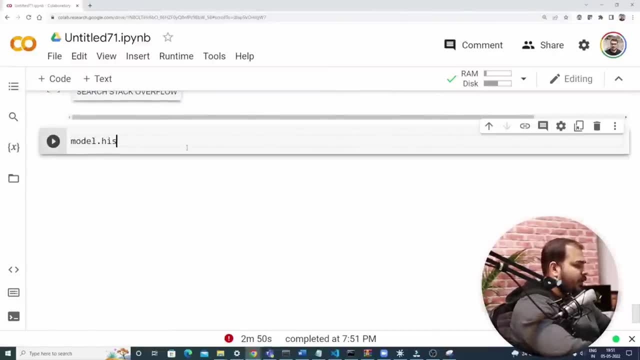 till how many epochs? like till 44 epochs. right, i'll just say that. right, i'll just say that. right, i'll just say that model dot history, because this entire model dot history, because this entire model dot history, because this entire information will get captured over here. 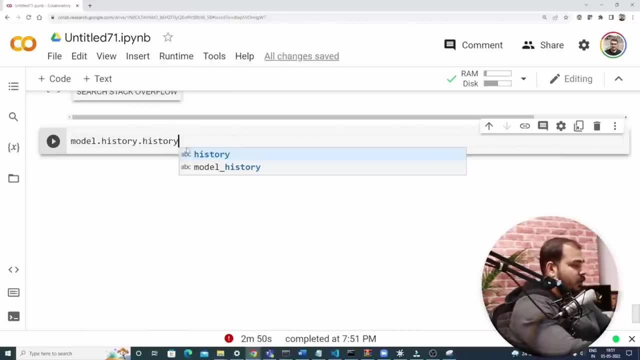 information will get captured over here. information will get captured over here. so i'm going to say history, so i'm going to say history, so i'm going to say history, dot history, dot keys. so there are some dot history dot keys. so there are some dot history dot keys. so there are some something called as keys, right and when i 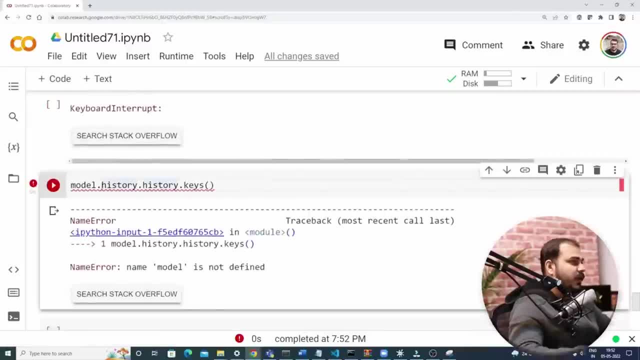 something called as keys right, and when i something called as keys right and when i execute this, execute this, execute this sorry model underscore history. that's sorry model. underscore history. that's sorry model. underscore history. that's right model. underscore history, right so right model. underscore history, right so. 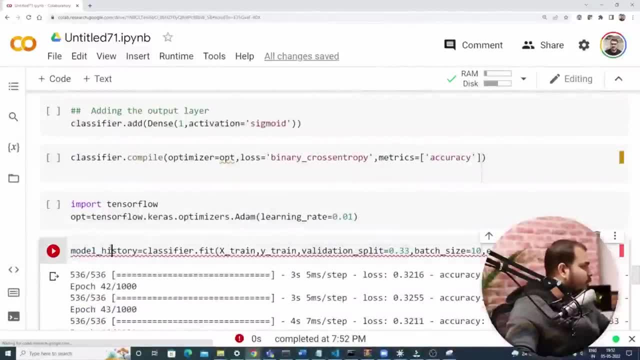 right, model underscore history, right. so here you can see, here you can see, here you can see: model underscore history is not defined. model underscore history is not defined. model underscore history is not defined. why no model underscore history? the. why no model underscore history? the. why no model underscore history? the spelling is wrong. 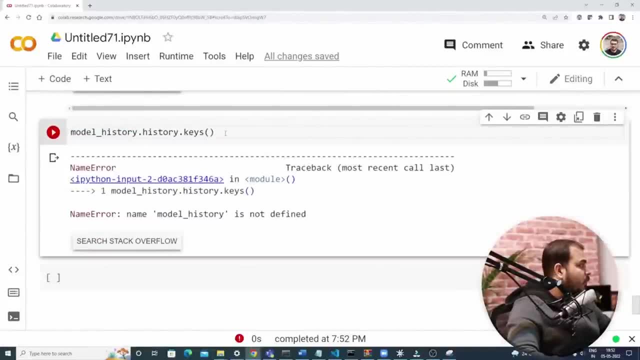 spelling is wrong. spelling is wrong or what or what or what? not history dot keys, not history dot keys. not history dot keys. okay, i think we have not trained it. okay, i think we have not trained it. okay, i think we have not trained it entirely. so i think that 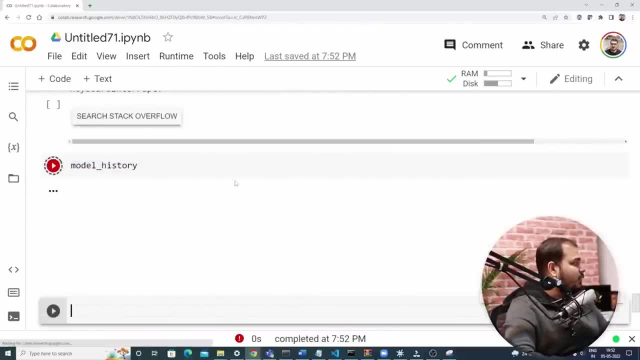 entirely. so i think that entirely. so i think that value is there or not. or let me just value is there or not, or let me just value is there or not, or let me just print model: underscore history. print model: underscore history. print model: underscore history: okay model. and this case is not there. 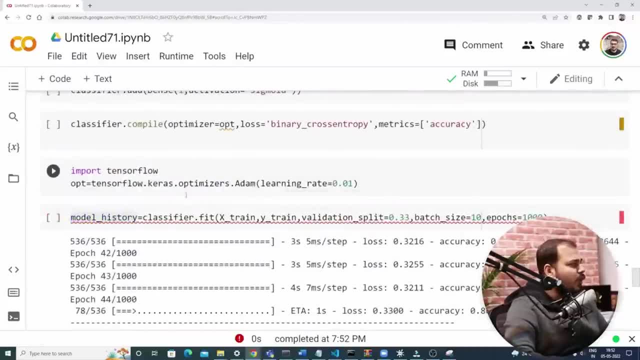 okay model and this case is not there. okay model and this case is not there because we have interrupted it right, because we have interrupted it right, because we have interrupted it right. so we cannot definitely plot. so what i? so we cannot definitely plot. so what i? so we cannot definitely plot. so what i will do is that i will add something. 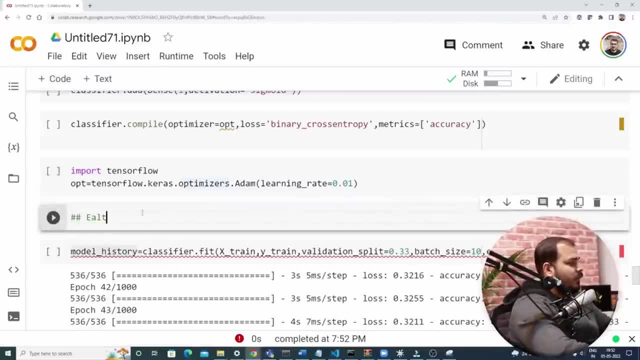 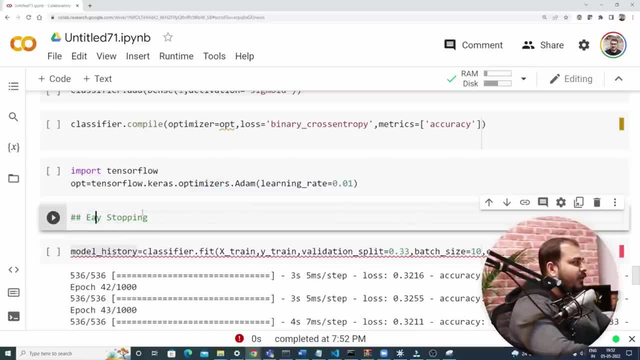 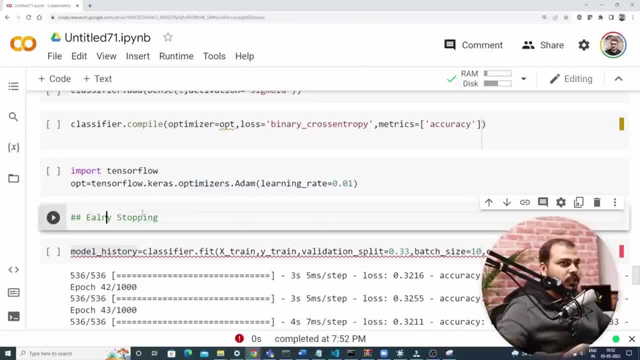 makes sure that when, when the accuracy is not at all increasing automatically, is not at all increasing automatically, is not at all increasing automatically, the training of the model will stop, the training of the model will stop, the training of the model will stop. okay, and that is what we are actually. 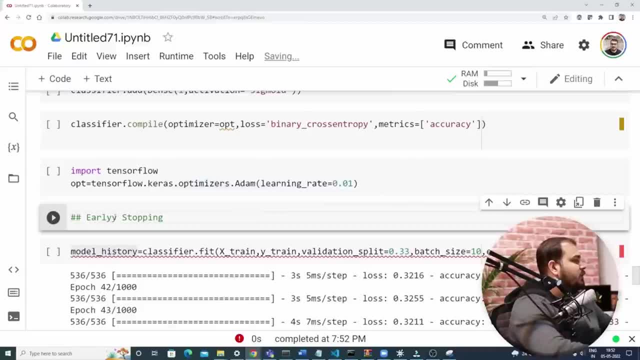 okay, and that is what we are actually okay, and that is what we are actually going to do with the help of early going to do with the help of early going to do with the help of early shopping. now early stopping is uh. shopping now early stopping is uh. 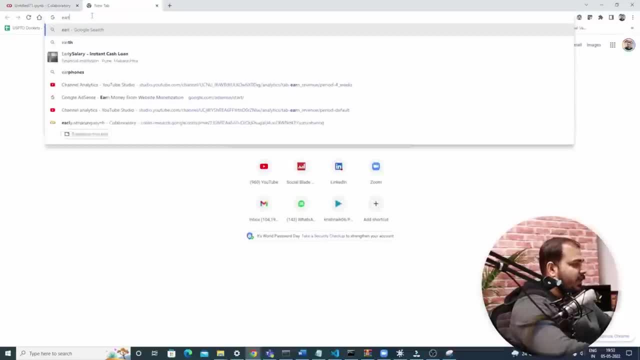 shopping. now, early stopping is uh, i'll just go to my garage documentation. i'll just go to my garage documentation. i'll just go to my garage documentation, okay, and i'll write early stopping. okay, and i'll write early stopping. okay, and i'll write early stopping, garage okay. 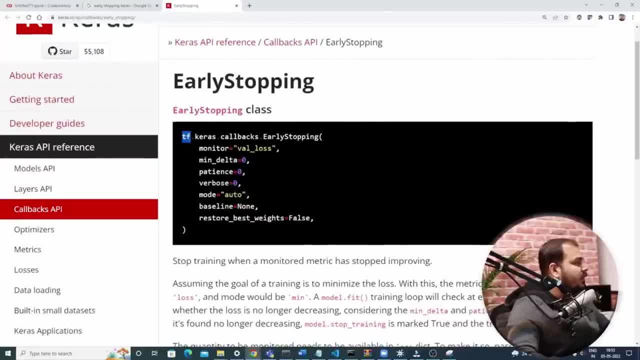 garage, okay, garage, okay now. here you can basically see early now. here you can basically see early now. here you can basically see early stopping keras and just copy this entire stopping keras and just copy this entire stopping keras and just copy this entire thing see, copy this entire thing with. 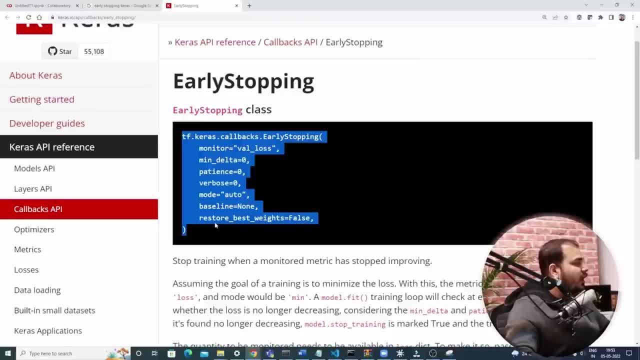 thing- see, copy this entire thing. with thing- see, copy this entire thing. with respect to minimum delta patience. respect to minimum delta patience. respect to minimum delta patience. verbose mode, verbose mode, verbose mode. uh, restore best weights, and all are there. uh, restore best weights and all are there. 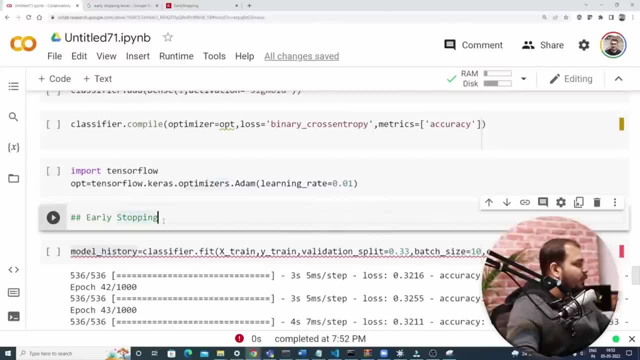 uh, restore best weights and all are there. so what i am actually going to do, i'm so what i am actually going to do. i'm so what i am actually going to do. i'm just going to copy this, just going to copy this, just going to copy this, i'm going to paste it over here and i'm i'm going to paste it over here and i'm i'm going to paste it over here and i'm going to play with some values, going to play with some values, going to play with some values. so, before that, i'm just going to say so, before that i'm just going to say 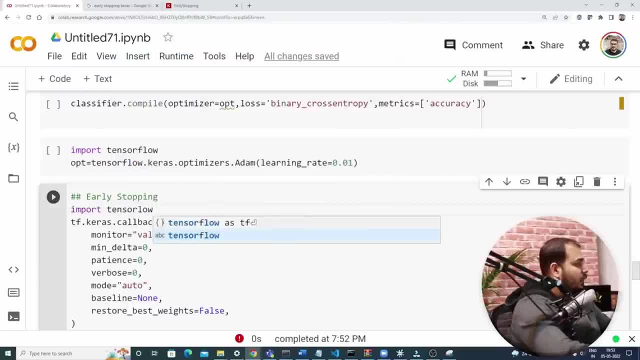 so before that, i'm just going to say import tensor flow, import tensor flow, import tensor flow or tensor flow as tf- okay and basically. or tensor flow as tf- okay and basically. or tensor flow as tf- okay and basically. this will basically be my, this will basically be my. 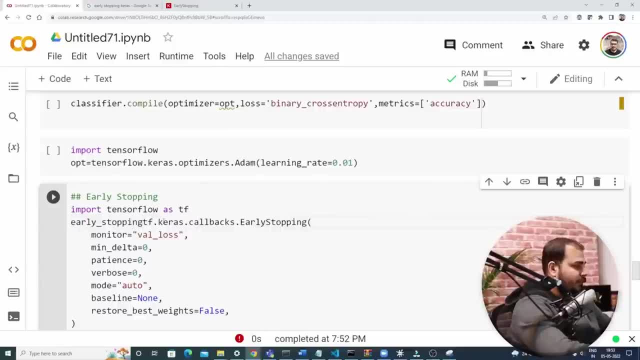 this will basically be my early stopping, early stopping variable, early stopping, early stopping variable. early stopping, early stopping variable. okay, okay, okay, and let me play with some of the values and let me play with some of the values. and let me play with some of the values. what does this early stopping say? 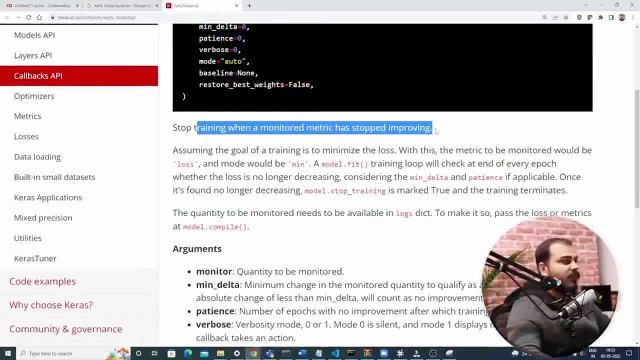 what does this early stopping say? what does this early stopping say: stop training when the monitored method. stop training when the monitored method stop training when the monitored method, metric has stopped improving. okay when metric has stopped improving. okay when metric has stopped improving. okay when it stops getting improved. it is. 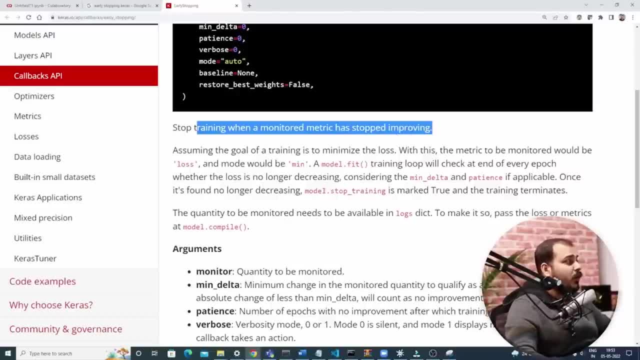 it stops getting improved. it is. it stops getting improved, it is automatically going to stop and it will automatically going to stop. and it will automatically going to stop and it will be able to understand that at what epoch, be able to understand that at what epoch, be able to understand that at what epoch it basically stopped. okay, and we are. 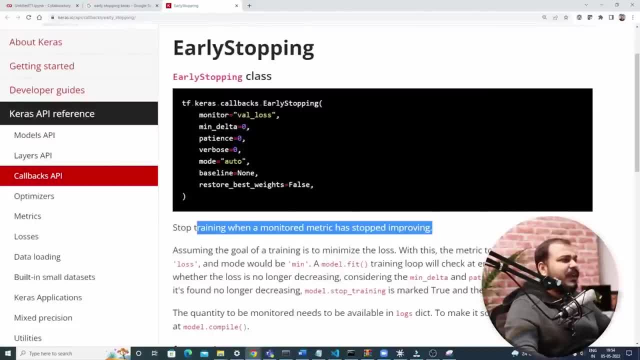 it basically stopped, okay, and we are. it basically stopped okay, and we are going to play with this, going to play with this, going to play with this specific values like what should be my specific values, like what should be my specific values, like what should be my delta value, what should be my other. 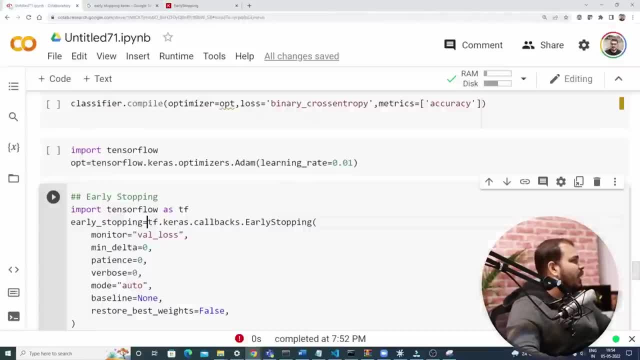 delta value. what should be my other delta value? what should be my other value? that we can definitely play value. that we can definitely play value that we can definitely play okay. so let's say i'm just going to put okay. so let's say i'm just going to put. 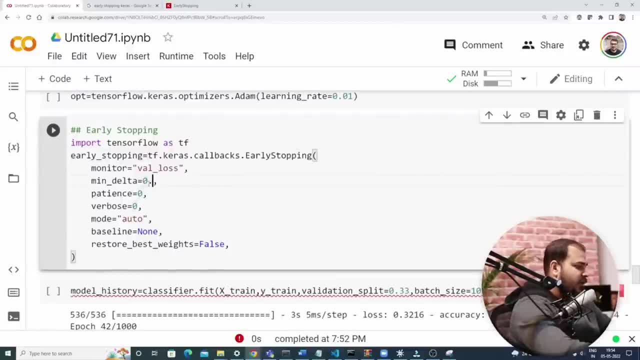 okay. so let's say, i'm just going to put some values over here, some values over here, some values over here- minimum delta- let's see, i'm just saying minimum delta. let's see, i'm just saying minimum delta. let's see, i'm just saying that, okay, this much should be my minimum. 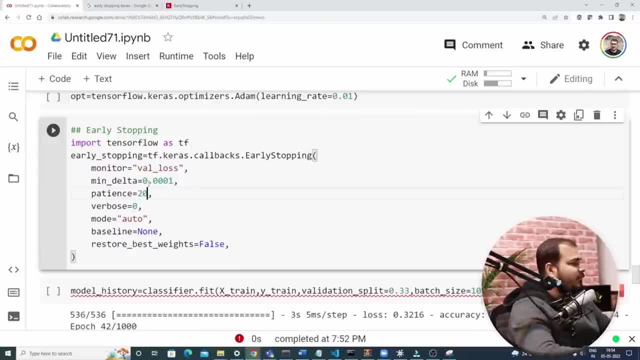 that, okay, this much should be my minimum. that, okay, this much should be my minimum. delta the patience- uh, you can check out. delta the patience- uh, you can check out. delta the patience- uh, you can check out each and every variable- okay, verbose i. each and every variable- okay, verbose i. 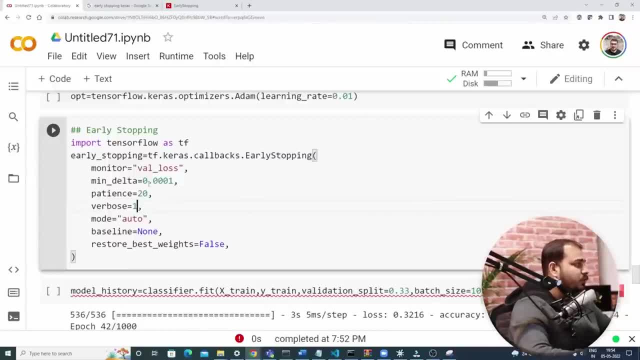 each and every variable. okay, verbose, i require one because i need to see all require one. because i need to see all require one, because i need to see all the details, and probably i'm just going the details, and probably i'm just going the details and probably i'm just going to execute in this way all i do execute. 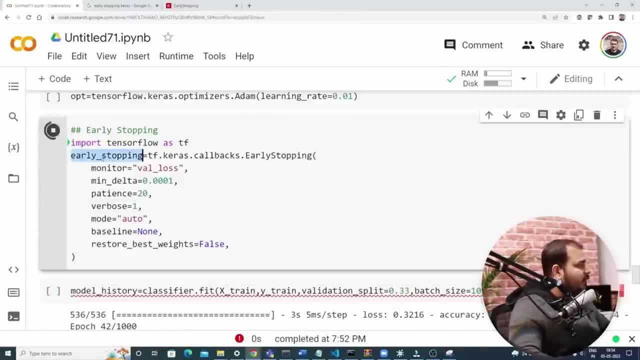 to execute in this way, all i do execute. to execute in this way, all i do execute this: okay, the early stopping has got this. okay, the early stopping has got this. okay, the early stopping has got executed. the variable will get created. executed, the variable will get created. 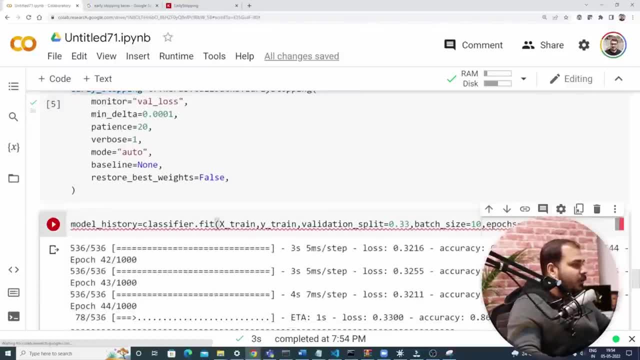 executed, the variable will get created. this variable i want and i will just this variable i want and i will just this variable i want and i will just paste this variable over here. where i paste this variable over here, where i paste this variable over here, where i can use one more parameter, where i can, 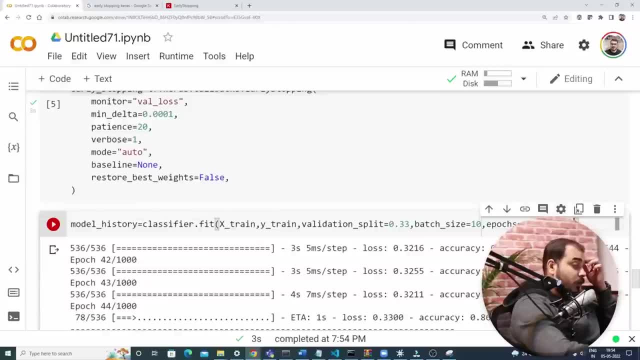 can use one more parameter where i can. can use one more parameter where i can say: early stopping, early underscore stopping- okay, sorry, early underscore stopping, okay, sorry, early underscore stopping, okay, sorry. here what i'll say, i'll say: call back. here what i'll say, i'll say: call back. 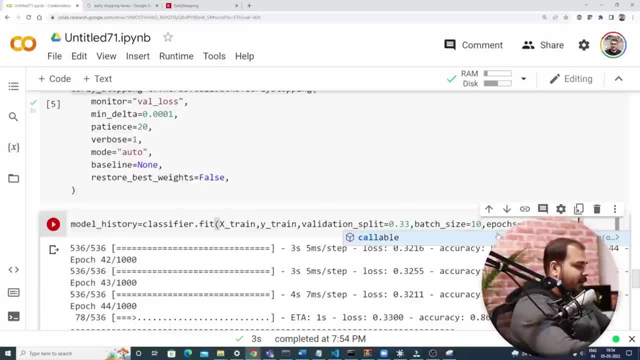 here what i'll say. i'll say: call back, okay, so call back is a function. uh call, okay, so call back is a function. uh call, okay, so call back is a function. uh, call back, back, back, okay, call backs is a function. okay, where i okay, where i can assign this early, stopping. 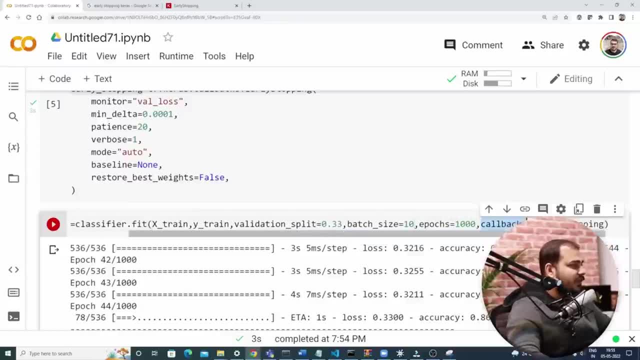 can assign this early stopping, can assign this early stopping. okay, okay, okay, when i assign this, that basically means when i assign this, that basically means when i assign this. that basically means we are basically assigning, or we are, we are basically assigning, or we are, we are basically assigning, or we are telling that you have to stop and you. telling that you have to stop and you telling that you have to stop and you have to monitor this validation loss and have to monitor this validation loss and have to monitor this validation loss and you have to make sure that if it does, you have to make sure that if it does. 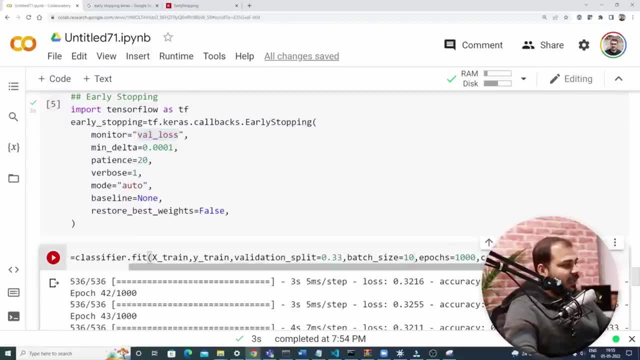 you have to make sure that if it does not improve, i'm just going to stop it, not improve, i'm just going to stop it, not improve. i'm just going to stop it over there. so once i just update this over there. so once i just update this. 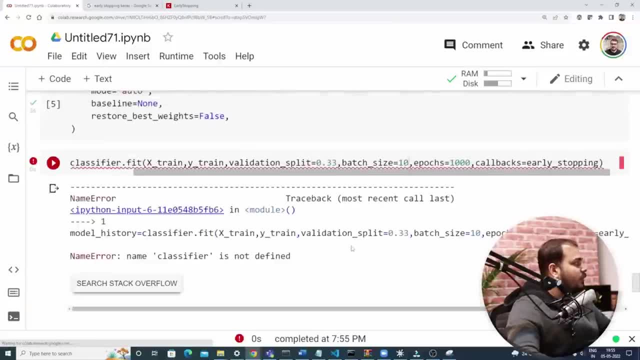 over there. so once i just update this callbacks and stopping, and once i callbacks and stopping, and once i callbacks and stopping, and once i execute it, execute it. execute it now. here you'll be able to see. now here you'll be able to see. now here you'll be able to see: classifier is not defined, okay. 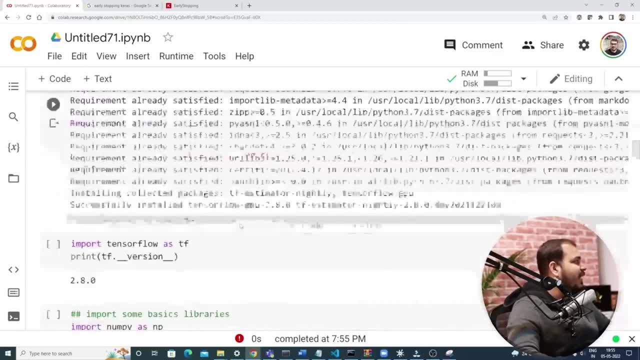 classifier is not defined. okay, classifier is not defined. okay, let me do one thing quickly. okay, this. let me do one thing quickly, okay, this. let me do one thing quickly. okay, this is entirely uh. i think uh is entirely uh. i think uh is entirely uh. i think uh, this has got uh. 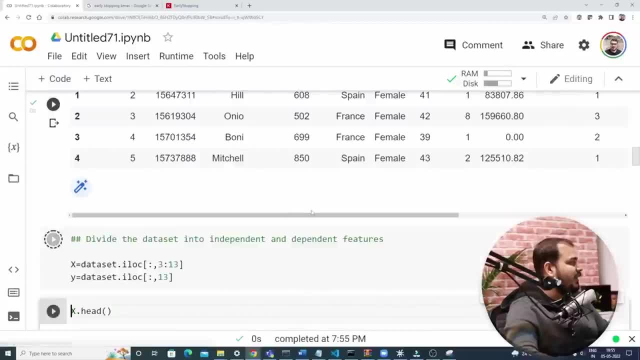 this has got, uh, this has got, uh, entirely this. you know the kernel has got entirely this. you know the kernel has got entirely this. you know the kernel has got restarted, so i'm just going to execute restarted. so i'm just going to execute restarted. so i'm just going to execute it totally. 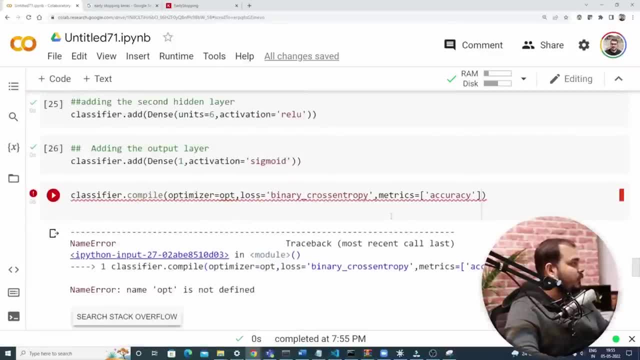 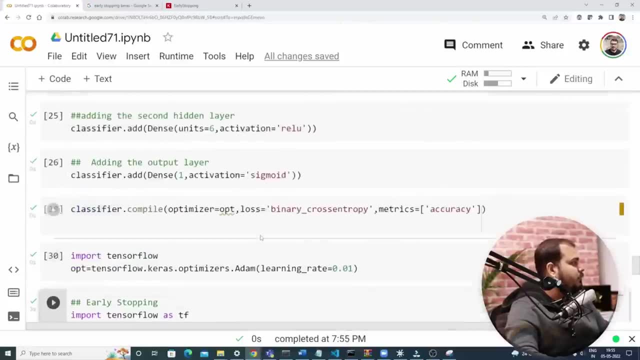 it totally. it totally. okay. fine, this has got executed. okay, fine, this has got executed. okay, fine, this has got executed. um, um, um, perfect, perfect, perfect. this has also got executed. then i'm: this has also got executed. then i'm: this has also got executed, then i'm going to apply this tensorflow. 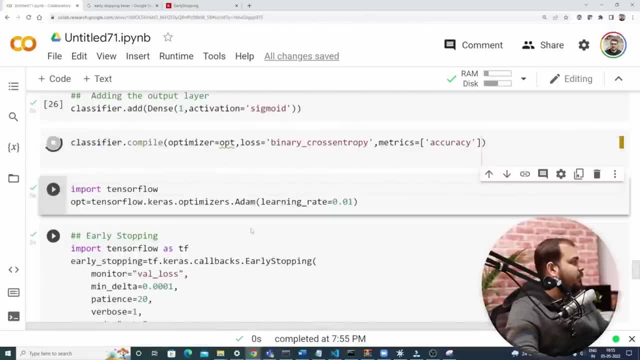 okay, perfect, i'm just going to execute. okay, perfect, i'm just going to execute. okay, perfect, i'm just going to execute this, this, this opt compile, and finally, uh, let's go opt compile. and finally, uh, let's go opt compile. and finally, uh, let's go ahead and execute this. 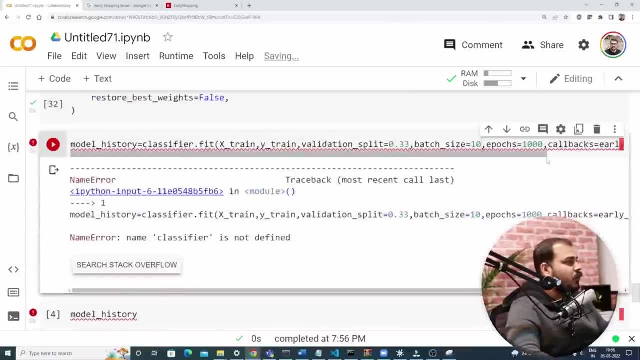 ahead and execute this ahead and execute this code early stopping, and then wherever i'm code early stopping, and then wherever i'm code early stopping, and then wherever i'm using callbacks, i'm going to use this using callbacks. i'm going to use this using callbacks. i'm going to use this early stopping. okay. 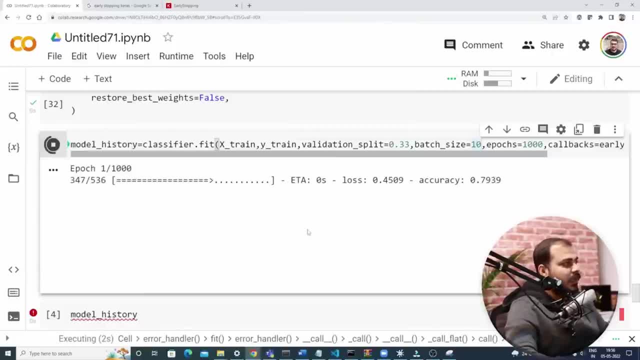 early stopping, okay. so once i execute this now my model, so once i execute this now my model, so once i execute this now my model, training will start happening, training will start happening. training will start happening now. here you can see that i have applied. now, here you can see that i have applied. 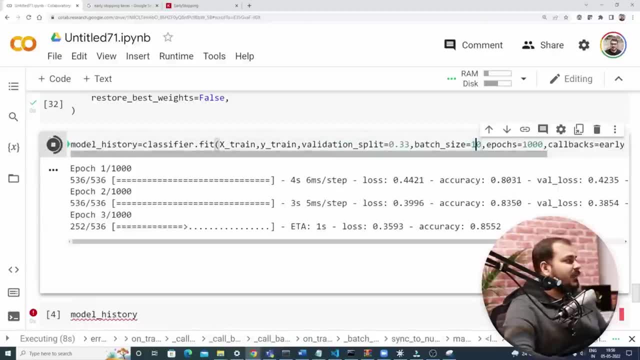 now, here you can see that i have applied early stopping, early stopping, early stopping now. let's focus on at what epoch? now, let's focus on at what epoch? now, let's focus on at what epoch it will just stop. you know at what epoch it will just stop. you know at what epoch. 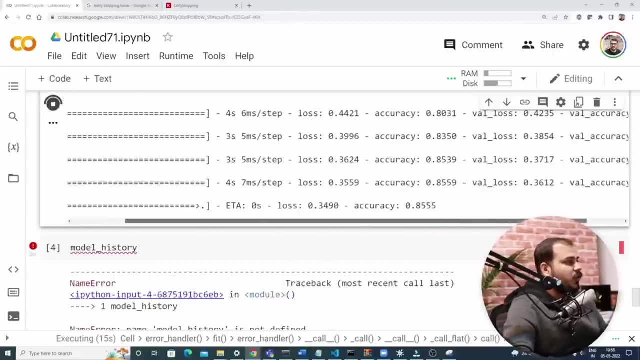 it will just stop. you know at what epoch it will basically stop. okay, it will basically stop okay, it will basically stop okay, now. here you can see we have focused on now. here you can see we have focused on now. here you can see we have focused on the. 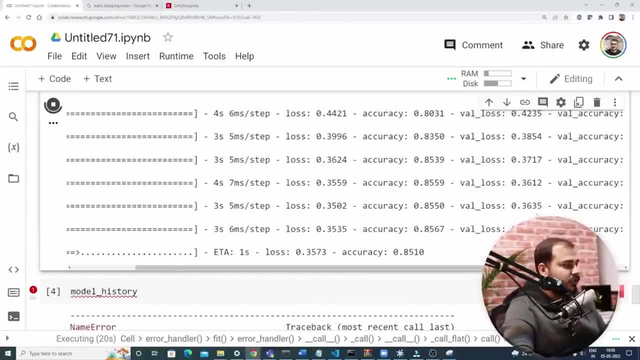 the the validation loss right now, validation, validation loss right now. validation, validation loss, right now, validation loss. if it does not improve much loss, if it does not improve much loss, if it does not improve much, then it is automatically going to stop. then it is automatically going to stop. 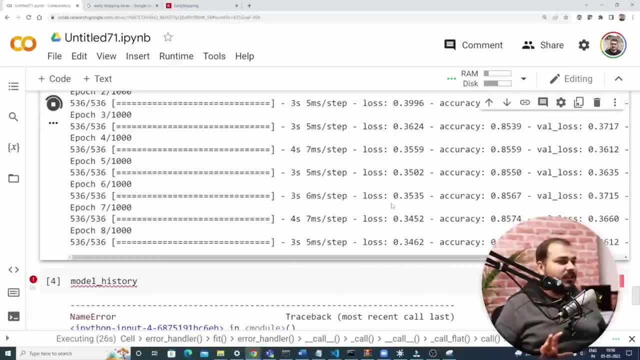 then it is automatically going to stop. let's see at when it will stop. okay, i'm let's see at when it will stop. okay, i'm let's see at when it will stop. okay, i'm not stopping it, not stopping it, not stopping it already. this will make sure that it will. 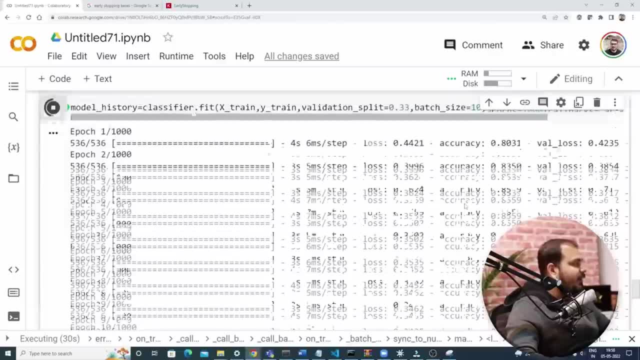 already. this will make sure that it will already. this will make sure that it will get stopped okay. get stopped okay. get stopped, okay. so let's see how much time it will take, let's see, let's see how much time it will. let's see, let's see how much time it will. 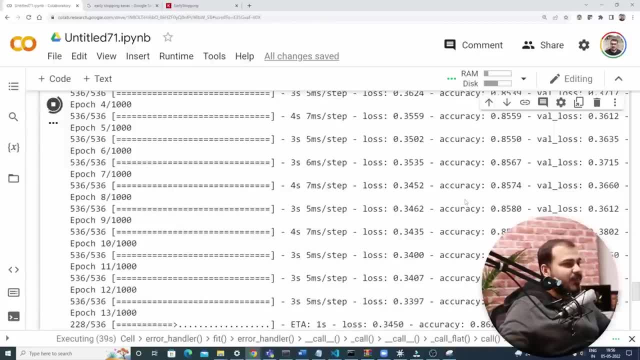 let's see. let's see how much time it will take and probably this will take some take and probably this will take some take and probably this will take some time, at least for some number of epochs time, at least for some number of epochs time, at least for some number of epochs, it is going to definitely get improved. 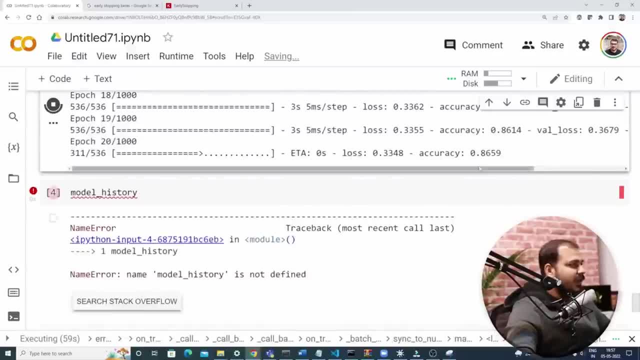 it is going to definitely get improved. it is going to definitely get improved. so here now still the accuracy is. so here now still the accuracy is. so here now still the accuracy is increasing in a better way, increasing in a better way, increasing in a better way, and then it will stop automatically. you. 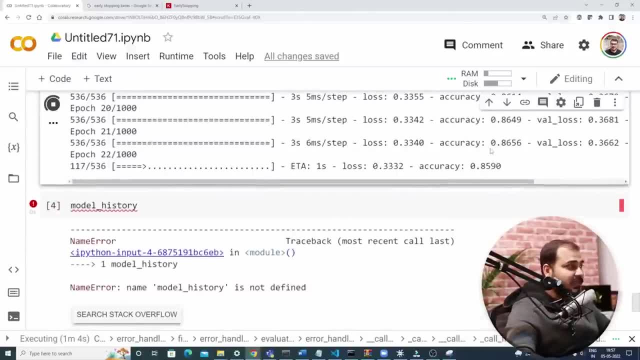 and then it will stop automatically. you, and then it will stop automatically. you see this now. i know that it. this see this now. i know that it. this see this now. i know that it- this accuracy is not going to go. accuracy is not going to go. accuracy is not going to go more than 87 percent. so whether it will, 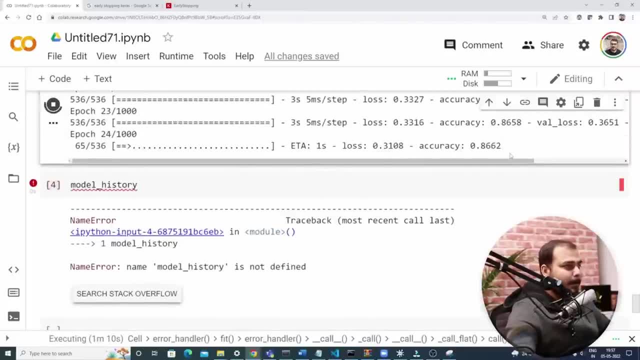 more than 87 percent. so whether it will more than 87 percent, so whether it will be able to go or not be able to go or not be able to go or not, we'll try to see. okay, so here you can see validation loss it. so here you can see validation loss it. 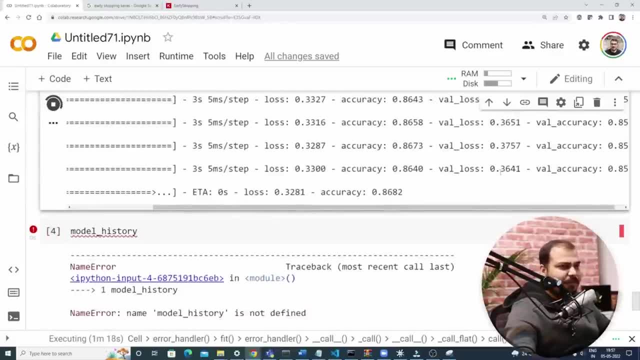 so here you can see validation loss: it is increasing, is increasing, is increasing and probably i think very we are very and probably i think very we are very and probably i think very we are very much near, much near, much near, you know, to stop the training itself. 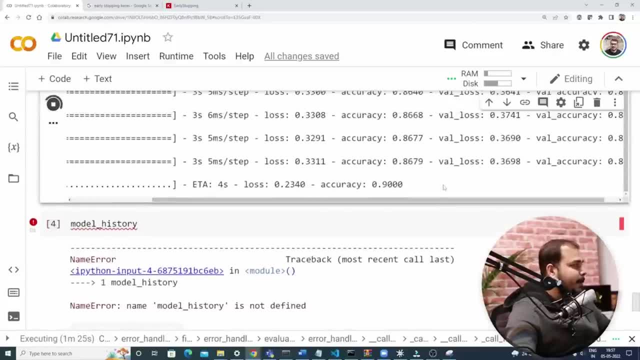 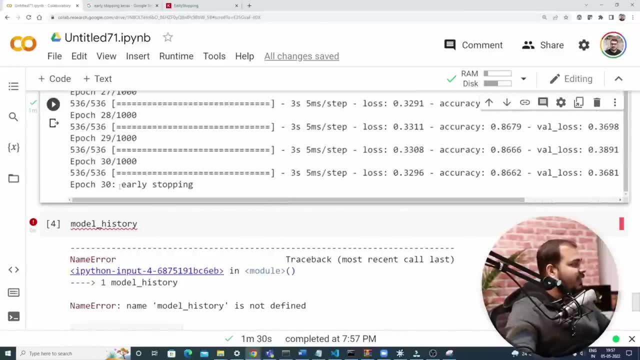 you know to stop the training itself. you know to stop the training itself. let's see, okay, automatically, the let's see, okay, automatically, the let's see, okay, automatically, the training will get stopped. so we are in 30 epochs, now you can see. so we are in 30 epochs, now you can see. 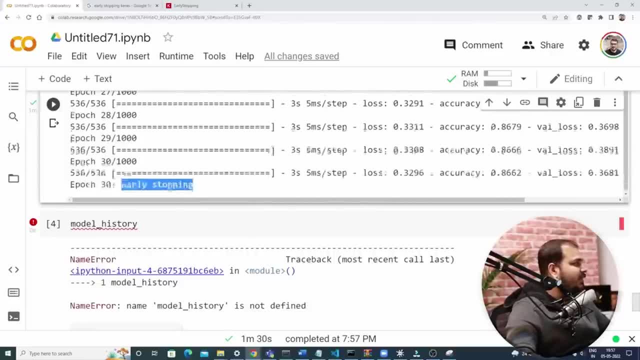 so we are in 30 epochs. now you can see epoch 30 early stopping right. so epoch 30 early stopping right. so epoch 30 early stopping right. so automatically, this stop, automatically, this stop, automatically, this stop the epoch 30. it has got stopped. and now 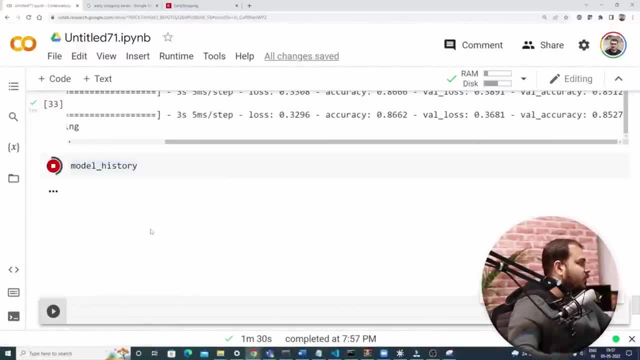 the epoch 30, it has got stopped. and now the epoch 30, it has got stopped, and now we are basically having 85. we are basically having 85, we are basically having 85. now, what i can do, i can basically execute. now, what i can do, i can basically execute. 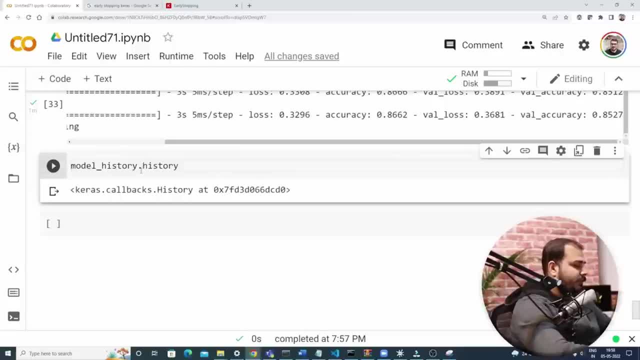 now what i can do. i can basically execute model history, model history, model history, and i can basically say dot history and i can basically say dot history and i can basically say dot history, dot, dot, dot. geez right, if i execute this, you will be. geez right, if i execute this, you will be. 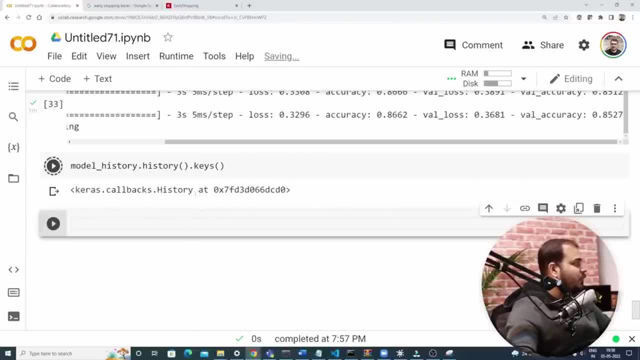 geez right, if i execute this, you will be able to see what all able to see what. all able to see what all parameters. we have specifically focused parameters. we have specifically focused parameters we have specifically focused on: okay, okay, okay, what all parameters we are specifically what all parameters we are specifically focused on. okay, sorry, this is something. 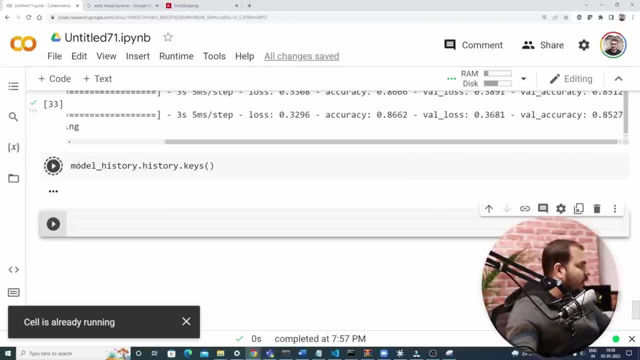 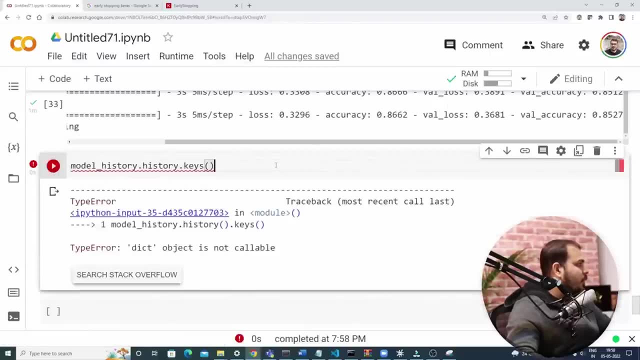 focused on: okay, sorry, this is something focused on. okay, sorry, this is something wrong, okay, okay, fine. so here it is model dot history. fine, so here it is model dot history. fine, so here it is model dot history, dot keys, dot keys, dot keys, and here you can see loss, accuracy. 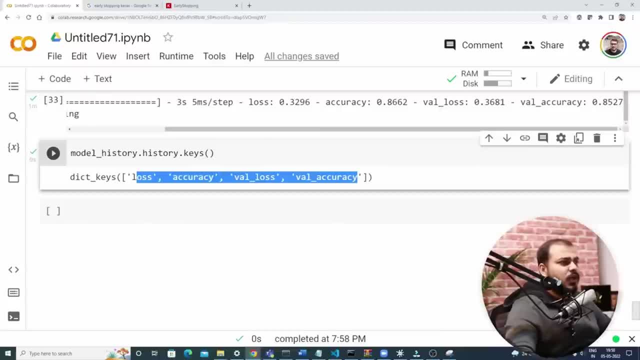 and here you can see loss accuracy. and here you can see loss accuracy, validation loss and validation accuracy. validation loss and validation accuracy. validation loss and validation accuracy. now what i'm actually going to do. uh, i'm now what i'm actually going to do. uh, i'm. 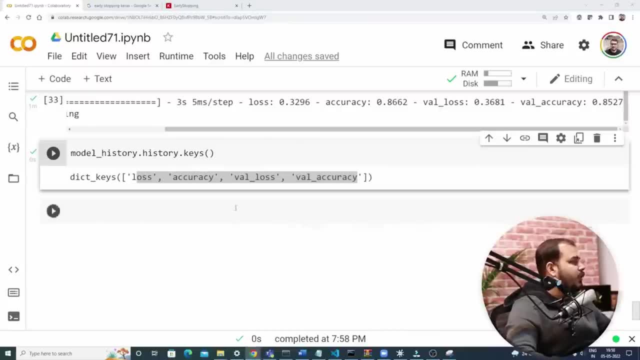 now what i'm actually going to do. uh, i'm basically going to just plot, basically going to just plot, basically going to just plot the summary for the history, for the summary for the history, for the summary for the history, for accuracy, accuracy, accuracy. so here you can see, this is how. 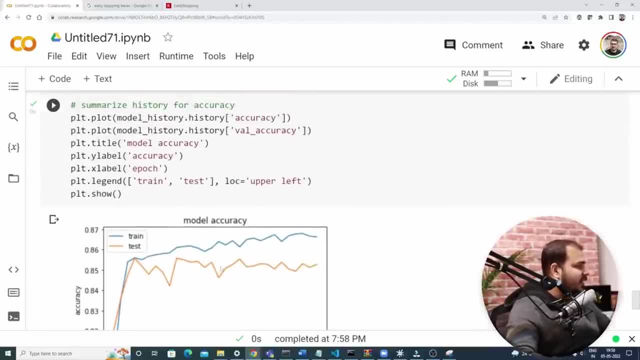 so here you can see, this is how. so here you can see, this is how my accuracy looks like. my accuracy looks like my accuracy looks like and it looks good. you know because this and it looks good, you know because this and it looks good, you know, because this is the test accuracy that is increasing. 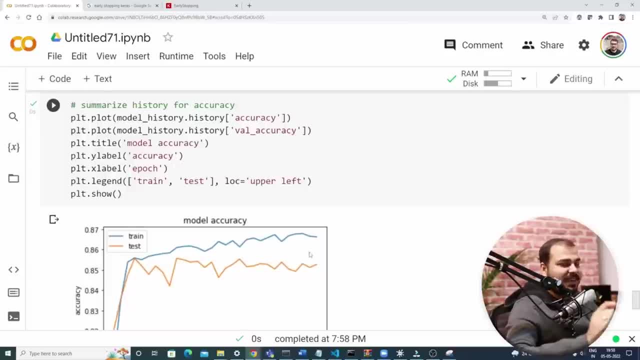 is the test accuracy that is increasing, is the test accuracy that is increasing and that is maintaining train accuracy and that is maintaining train accuracy and that is maintaining train accuracy. so this size is almost very less so, this size is almost very less so, this size is almost very less so. this is the power of this. uh, early. 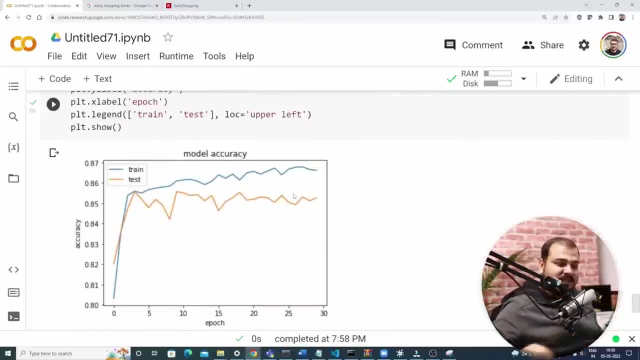 so this is the power of this uh early. so this is the power of this uh early. stopping you know, stopping you know, stopping, you know, before this size increases, you know, before this size increases, you know, before this size increases, you know, before this, this entire size increases it. 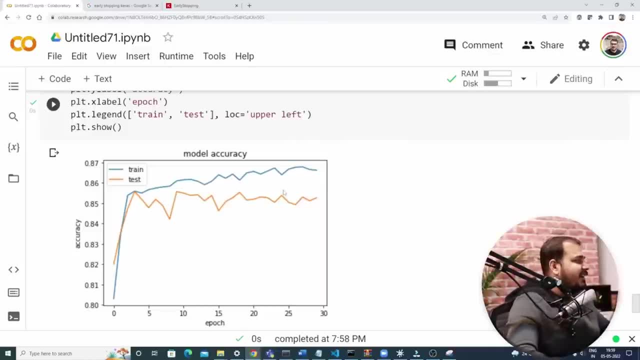 before this, this entire size increases, it. before this, this entire size increases, it is going to stop. and it is going to say: is going to stop. and it is going to say: is going to stop. and it is going to say that yes, that yes, that yes. now your model is basically ready, right. 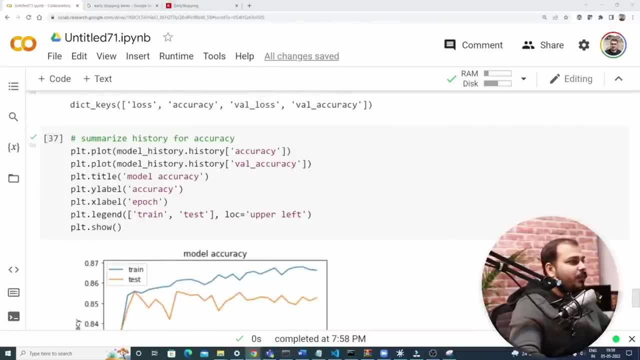 now, your model is basically ready. right now, your model is basically ready, right, and similarly, what i can do is that i, and similarly, what i can do is that i, and similarly, what i can do is that i can, basically, can, basically, can, basically, uh, plot it for the loss itself. 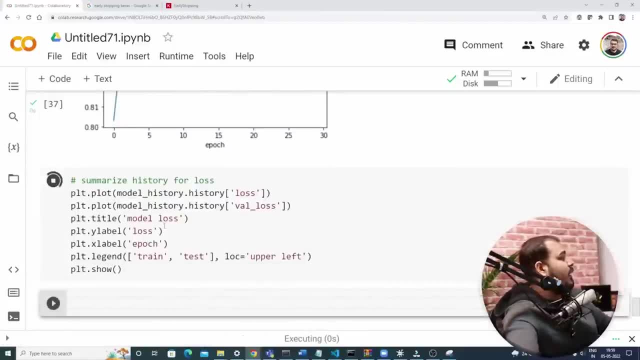 uh, plot it for the loss itself. uh, plot it for the loss itself. and we will go ahead and plot it for, and we will go ahead and plot it for, and we will go ahead and plot it for the loss, the loss, the loss, okay, and for the loss also, you will be. 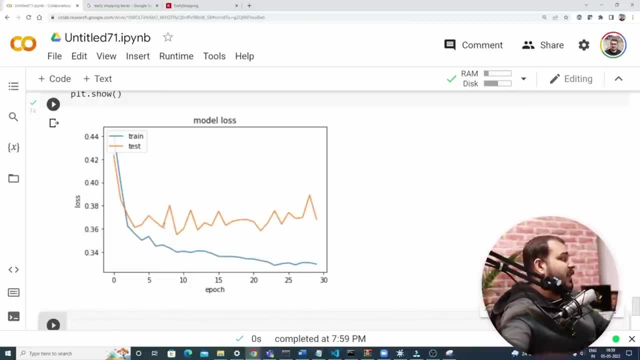 okay, and for the loss also, you will be okay and for the loss also, you will be able to see that now we are able to get able to see that now we are able to get able to see that now we are able to get this training and test accuracy in a 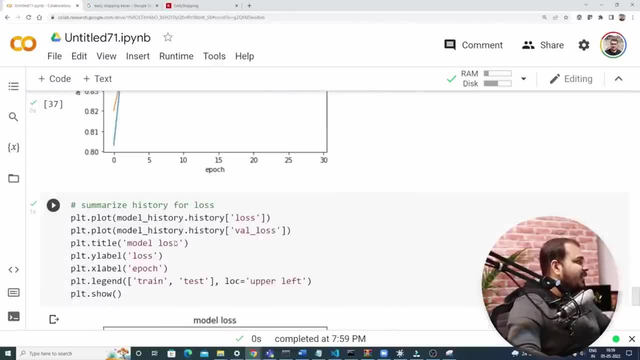 this training and test accuracy in a. this training and test accuracy in a better way, right. so here you can better way, right. so here you can better way, right. so here you can definitely see everything, uh, and this definitely see everything, uh, and this definitely see everything, uh, and this gap you can see from 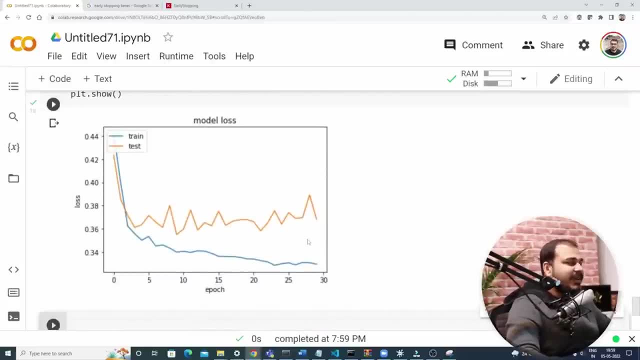 gap. you can see from gap. you can see from down to bottom, down to up. it has down to bottom, down to up. it has down to bottom, down to up. it has actually come so and it has basically actually come so and it has basically actually come so and it has basically stopped over there. so, through this way, 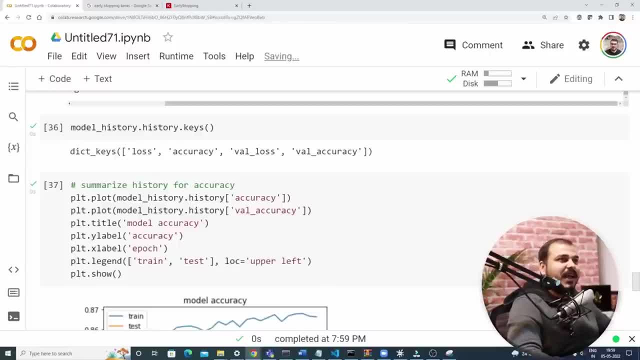 stopped over there. so through this way, stopped over there, so through this way- you can basically understand that. how you can basically understand that, how you can basically understand that how early stopping is actually done and how early stopping is actually done, and how early stopping is actually done and how, with the help of 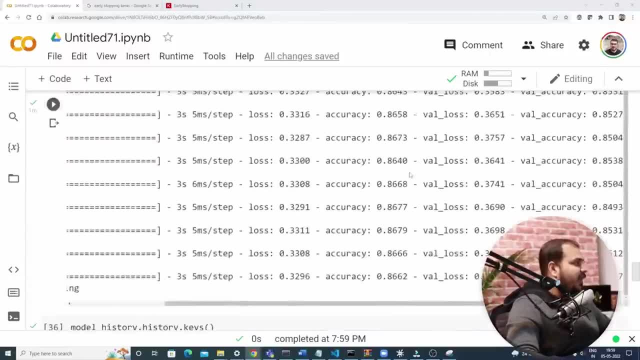 with the help of, with the help of uh this codes. you know we can basically uh this codes. you know we can basically uh this codes. you know we can basically do these things right, do these things right, do these things right and uh the next step. obviously we'll try. 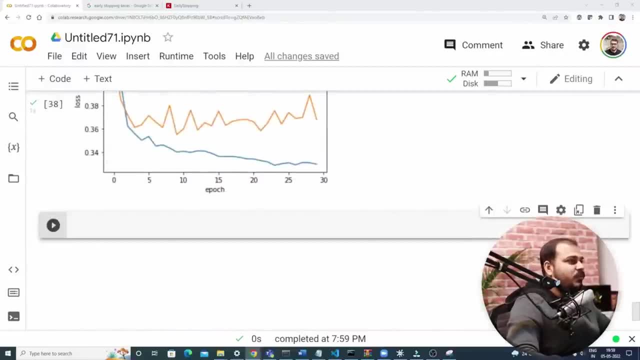 and uh the next step. obviously we'll try and uh the next step. obviously we'll try to do the prediction for the test data, to do the prediction for the test data, to do the prediction for the test data. so let's go ahead and do the prediction. 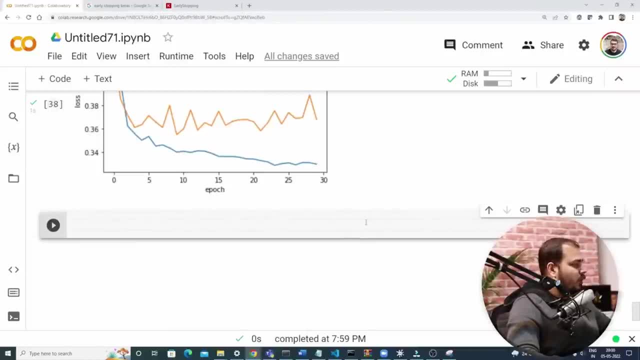 so let's go ahead and do the prediction. so let's go ahead and do the prediction for the test data, for the test data, for the test data for making the prediction. i'm just going for the test data for making the prediction. i'm just going for the test data for making the prediction. i'm just going to copy some code and paste it over. 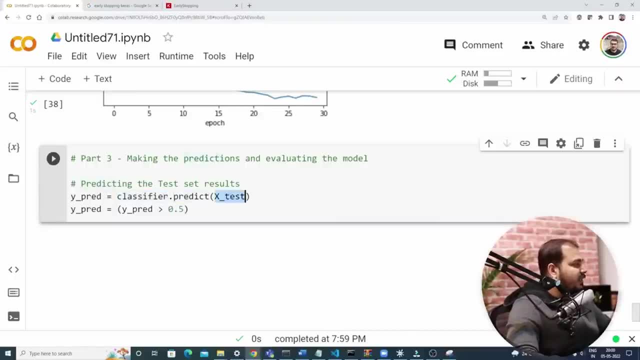 to copy some code and paste it over. to copy some code and paste it over here. right, i'm just going to use this here. right, i'm just going to use this here. right, i'm just going to use this. classifierpredict on x test and classifierpredict on x test, and. 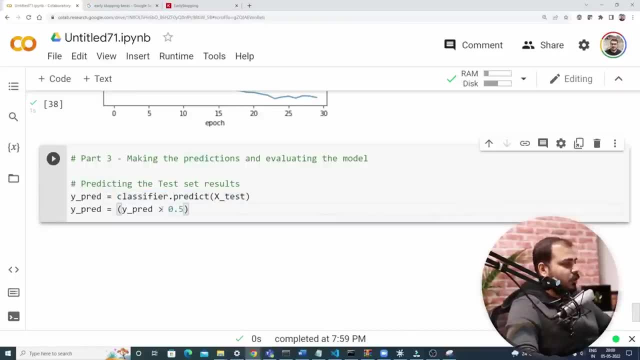 classifierpredict on x test. and whenever the value is greater than. whenever the value is greater than. whenever the value is greater than 0.5 right. greater than or equal to 0.5. 0.5 right greater than or equal to 0.5. 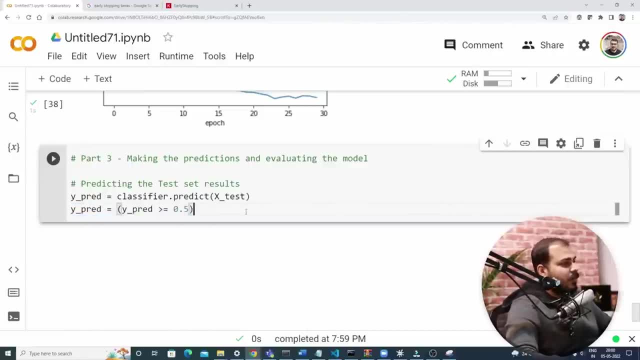 0.5 right greater than or equal to 0.5. i'm going to take it as 1, else i'm going. i'm going to take it as 1, else i'm going. i'm going to take it as 1, else i'm going to take it as 0. okay, and once i execute, 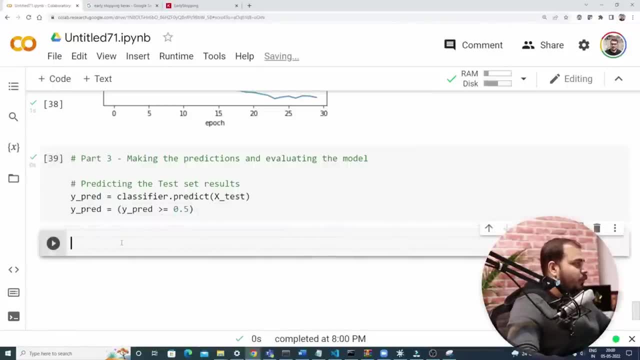 to take it as 0- okay. and once i execute, to take it as 0- okay. and once i execute, this, this, this i'm going to get true or false with. i'm going to get true or false with. i'm going to get true or false with respect to white red. all now that i have 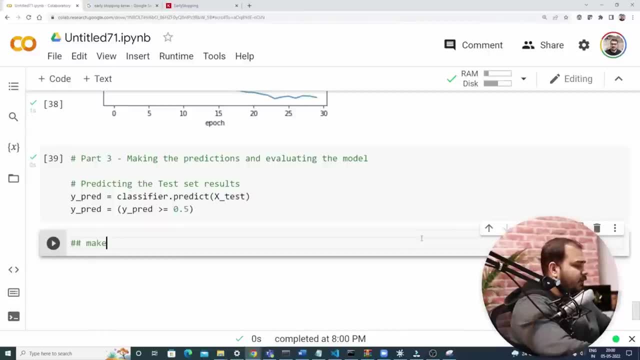 respect to white red. all now that i have respect to white red, all now that i have to do is that to do. is that to do? is that construct or make the confusion? matrix- construct or make the confusion? matrix- construct or make the confusion. matrix- make the confusion. 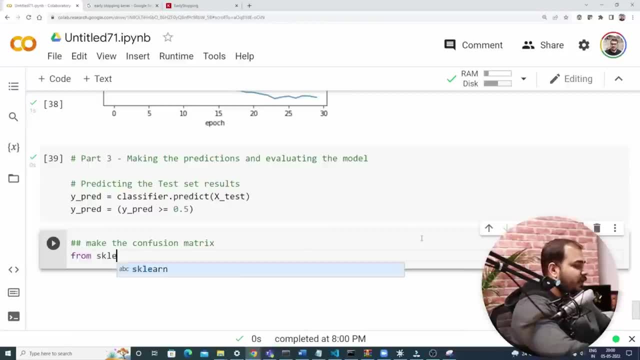 make the confusion, make the confusion matrix. now, when i say make the confusion matrix, now, when i say make the confusion matrix, now, when i say make the confusion matrix, i can say from sklearn dot matrix. i can say from sklearn dot matrix, i can say from sklearn dot matrix i'm going to import. 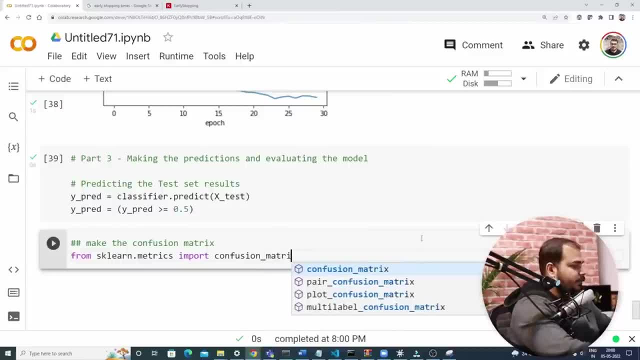 matrix. i'm going to import matrix. i'm going to import confusion, confusion, confusion, matrix, right, matrix, right, matrix, right, and then, finally, you will be able to see, and then finally you will be able to see, and then finally you will be able to see that i have cm. 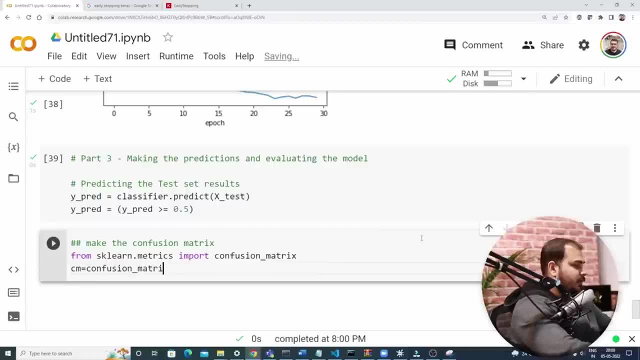 that i have cm, that i have cm is equal to nothing, but confusion is equal to nothing, but confusion is equal to nothing but confusion. matrix, matrix, matrix. and i'm going to basically say y and i'm going to basically say y and i'm going to basically say y underscore: test comma: y underscore. 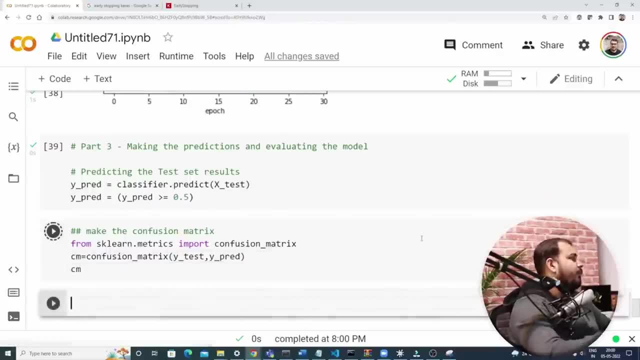 underscore: test comma y. underscore: underscore test comma y. underscore: spread right, spread right, spread right. and finally you will be able to see cm and finally you will be able to see cm and finally you will be able to see cm. now, here you can see, this is what is my. 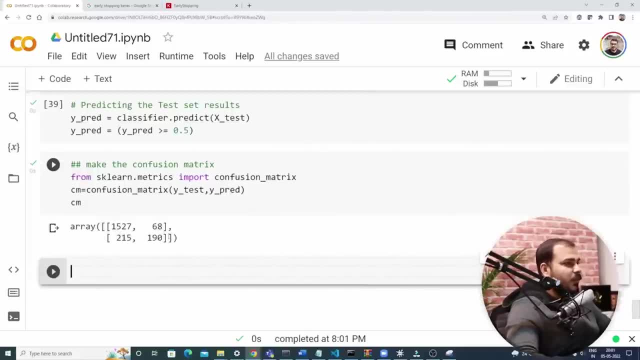 now here you can see. this is what is my now here you can see. this is what is my confusion matrix now. if i confusion matrix now, if i confusion matrix now, if i probably want to quickly, probably want to quickly, probably want to quickly calculate the accuracy, so what i have to 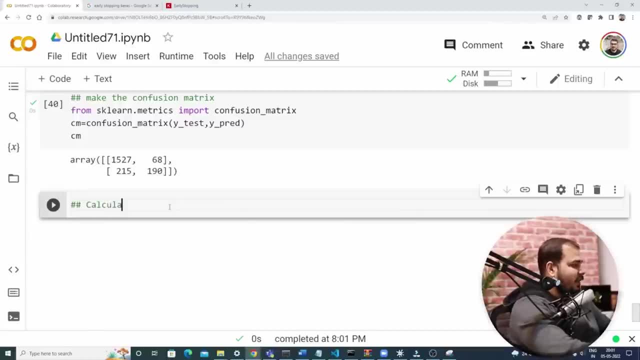 calculate the accuracy. so what i have to calculate the accuracy, so what i have to do. so i will just say do so. i will just say do so. i will just say: calculate the, calculate, the, calculate the accuracy, accuracy, accuracy. i will say from sklearn dot, i will say from sklearn dot. 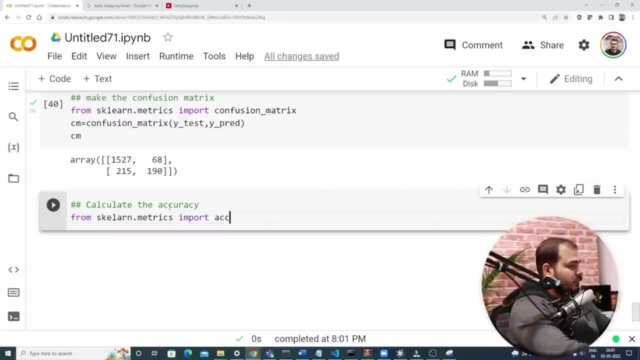 i will say: from sklearn dot matrix, matrix, matrix, i'm going to import, i'm going to import, i'm going to import the accuracy score, and then i'm basically going to say score, and then i'm basically going to say score, and then i'm basically going to say score is equal to. 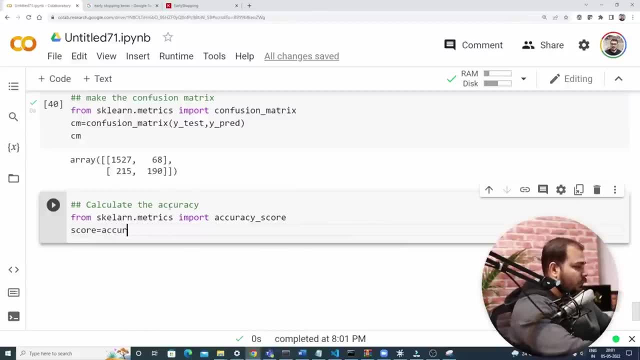 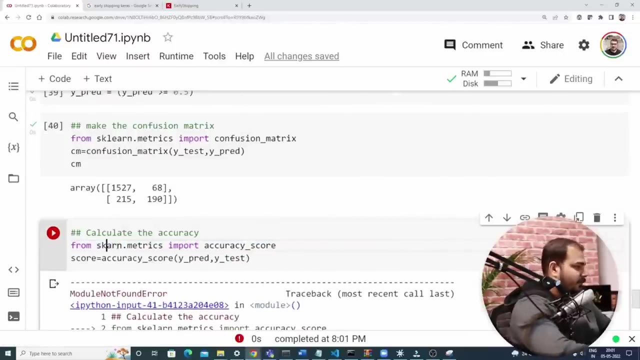 is equal to, is equal to accuracy, accuracy, accuracy, accuracy, score, score, score. and here i'm going to basically say y and here i'm going to basically say y and here i'm going to basically say y, pred, pred, pred, comma, y test, so so, so okay, sk learn, sk, learn okay. 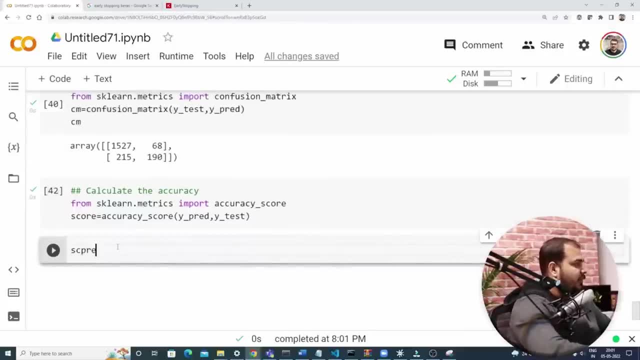 oops- okay, perfect, uh. so if i go and probably oops, okay, perfect, uh. so if i go and probably oops, okay, perfect, uh. so if i go and probably see my score, see my score, see my score- i will be able to get some good. i will be able to get some good. 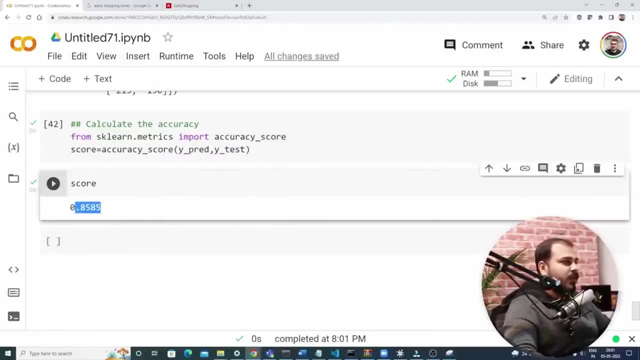 i will be able to get some good accuracy. let's see the 85 percent accuracy. let's see the 85 percent accuracy. let's see the 85 percent accuracy accuracy. let's see the 85 percent. accuracy is basically here, okay, accuracy is basically here, okay. 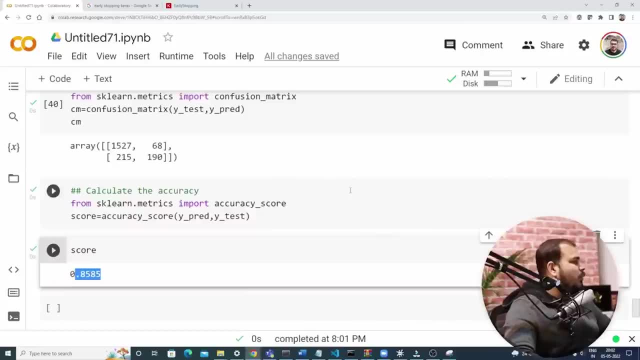 accuracy is basically here. okay, you may get somewhere around 86- 87, and you may get somewhere around 86- 87, and you may get somewhere around 86- 87 and all, all, all, now the one thing that i really wanted to, now, the one thing that i really wanted to. 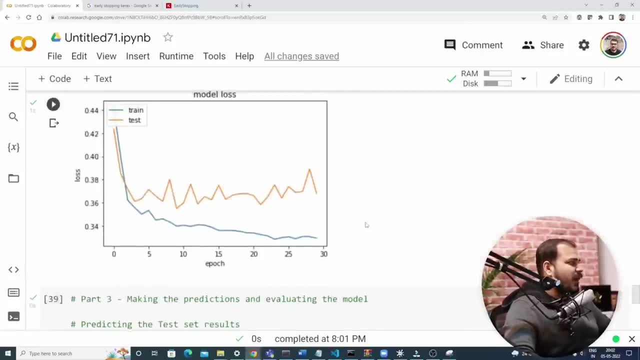 now, the one thing that i really wanted to talk about is that- okay, fine, crash. talk about. is that okay, fine, crash. talk about. is that okay, fine, crash. you have basically constructed such a, you have basically constructed such a, you have basically constructed such a big neural network, and all where i can. 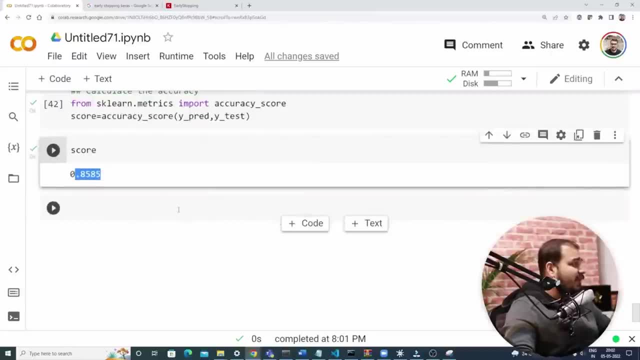 big neural network and all where i can big neural network and all where i can see the weights that is assigned with. see the weights that is assigned with, see the weights that is assigned with respect to each and every layer, so that, respect to each and every layer, so that 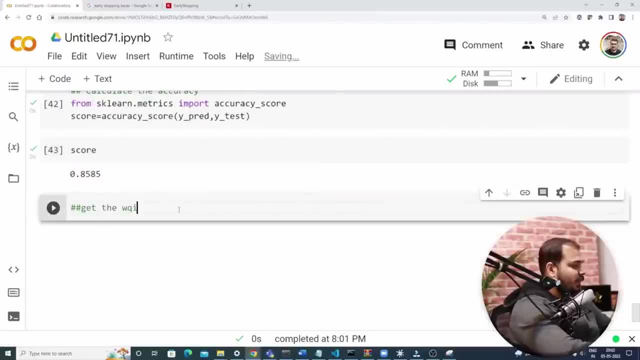 respect to each and every layer. so that information also, you can get information also. you can get information also. you can get get the weights okay and you can also get the weights okay and you can also get the weights okay and you can also store the weights. store the weights. 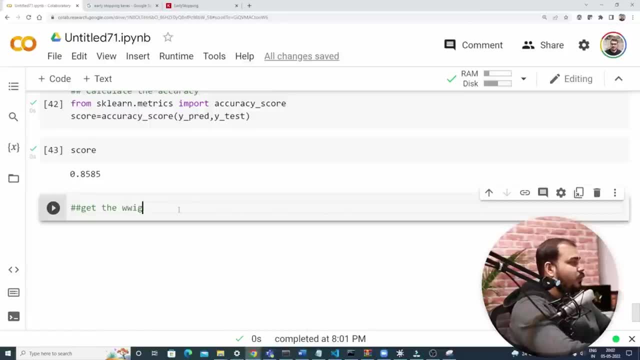 store the weights as a pickle file, you know, and probably you as a pickle file, you know, and probably you as a pickle file, you know, and probably you can use it wherever you want, can use it wherever you want, can use it wherever you want to get the weights you want to store. to get the weights you want to store. to get the weights. you want to store the weights, you can also get it. so what the weights? you can also get it. so what the weights? you can also get it. so what you can write is that you can just write. 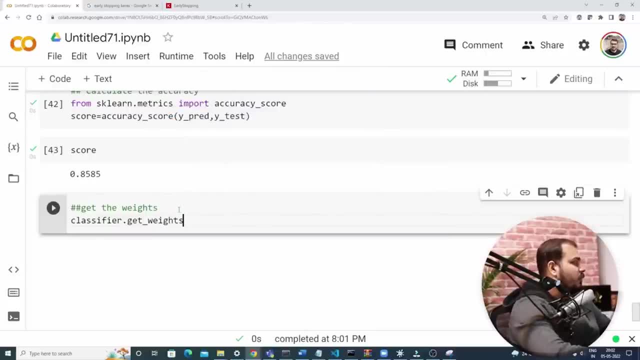 you can write, is that you can just write you can write, is that you can just write: classifier dot. classifier dot. classifier dot. get weights right. so, if you execute this, get weights right. so, if you execute this, get weights right. so, if you execute this, these are your weights value. 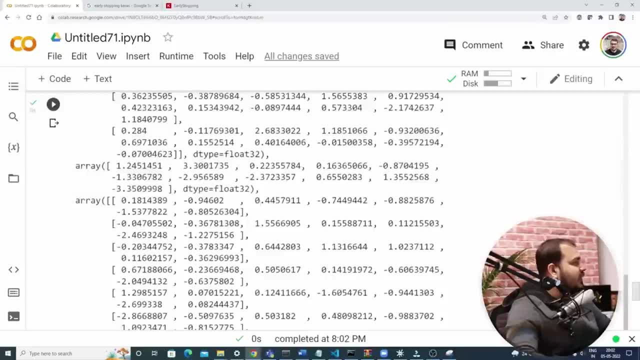 these are your weights value. these are your weights value. i'll use it as a function and these are: i'll use it as a function and these are: i'll use it as a function and these are all basically your weights. value that: all basically your weights. value that. 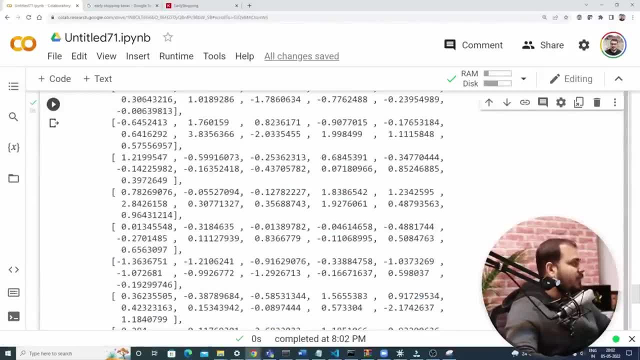 all, basically your weights value that you can basically get right and it will. you can basically get right and it will. you can basically get right and it will always be in the array format. because always be in the array format? because always be in the array format because there are so many layers and all right. 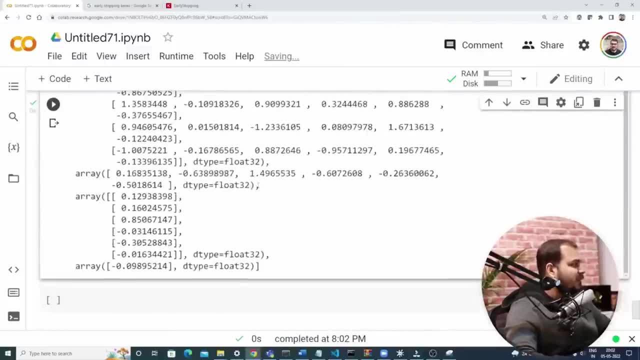 there are so many layers, and all right. there are so many layers, and all right. so, based on that, arrays will be there. so, based on that, arrays will be there. so, based on that, arrays will be there. and this many weights, just imagine. and this many weights, just imagine. 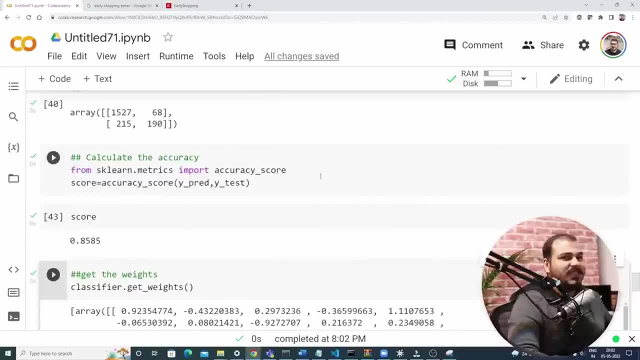 and this many weights. just imagine parallelly how you are able to train this parallelly, how you are able to train this parallelly, how you are able to train this many weights, right? so, just by seeing many weights, right. so, just by seeing many weights right. so just by seeing this. that will not be sufficient, you may. 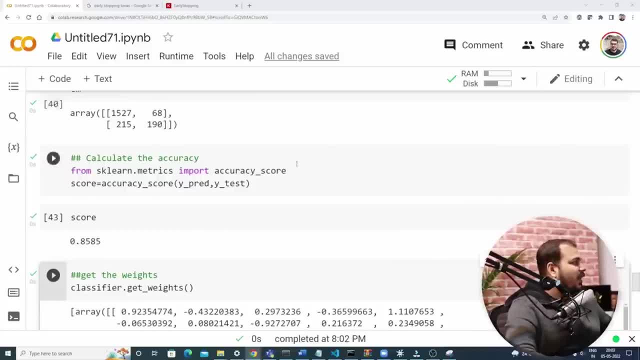 this? that will not be sufficient. you may this? that will not be sufficient. you may not, not not exactly get, and all okay. so, uh, this was exactly get, and all okay. so, uh, this was exactly get, and all okay. so, uh, this was it. uh, now, one thing that you can do is 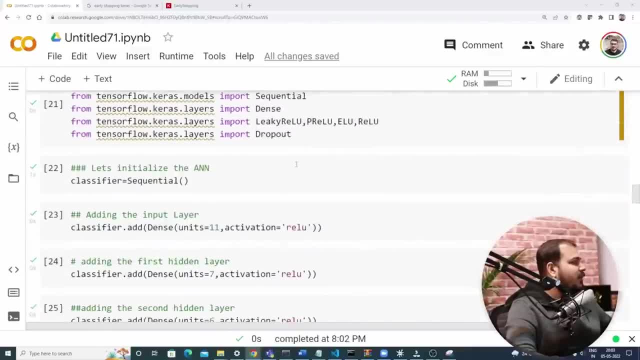 it? uh, now, one thing that you can do is it? uh, now, one thing that you can do is that i've also spoken about the dropout, that i've also spoken about the dropout, that i've also spoken about the dropout layer, right layer, right now, inside the dropout layer. how do i? 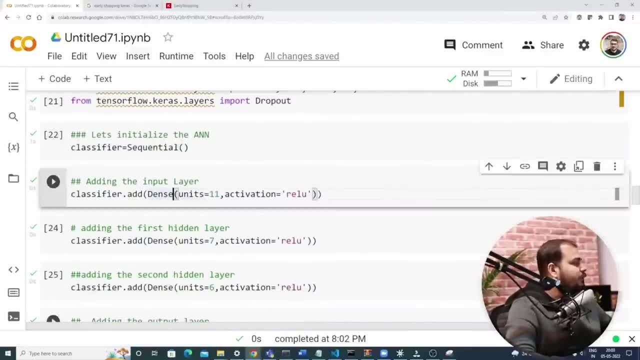 now inside the dropout layer? how do i now inside the dropout layer? how do i add a dropout layer? so here you can add a dropout layer. so here you can add a dropout layer. so here you can basically see that. when you basically see that, when you basically see that when you pinpoint over here, right, 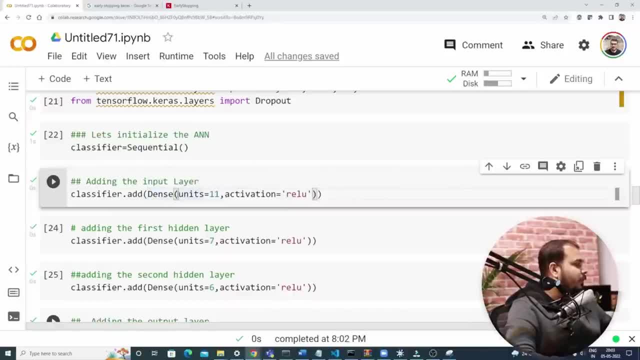 pinpoint over here, right. pinpoint over here. right, let's say where i'm pinpointing over. let's say where i'm pinpointing over. let's say where i'm pinpointing over here: right, import dense here. right. import dense here. right, import dense. let's see whether we'll get an option. or 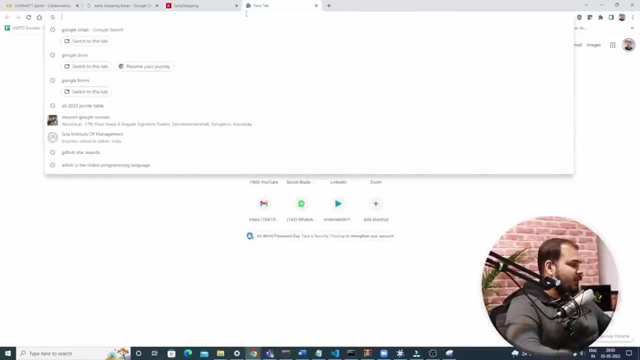 let's see whether we'll get an option. or let's see whether we'll get an option or not, because i really wanted to show you, not because i really wanted to show you, not because i really wanted to show you this, this, this. or let me open dense layer in keras. 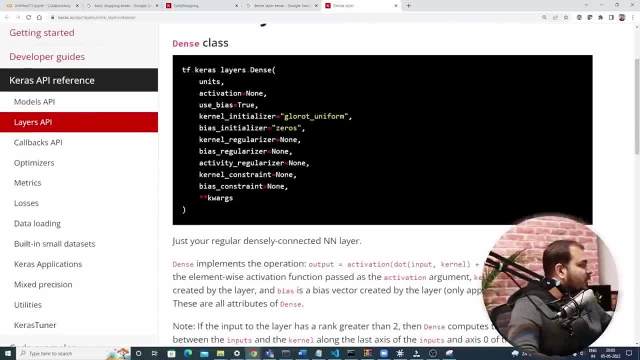 okay, dense layer in keras in keras. uh i okay dense layer in keras in keras. uh, i okay dense layer in keras in keras. uh, i think somewhere you will be able to see. think somewhere you will be able to see. think somewhere you will be able to see dropout layer. 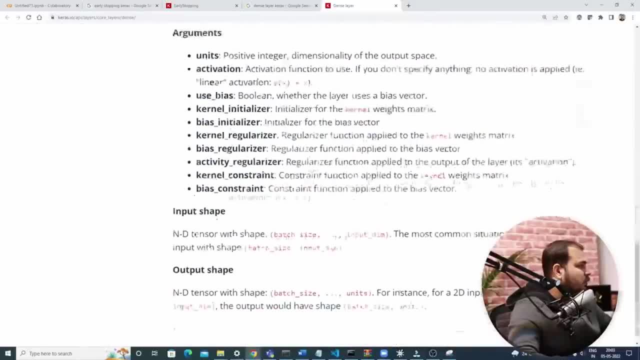 dropout layer, dropout, layer, dropout, dropout, dropout- somewhere. you can basically write it as somewhere. you can basically write it as somewhere. you can basically write it as dropout. it's okay if you're not getting dropout. it's okay if you're not getting dropout. it's okay if you're not getting over here. 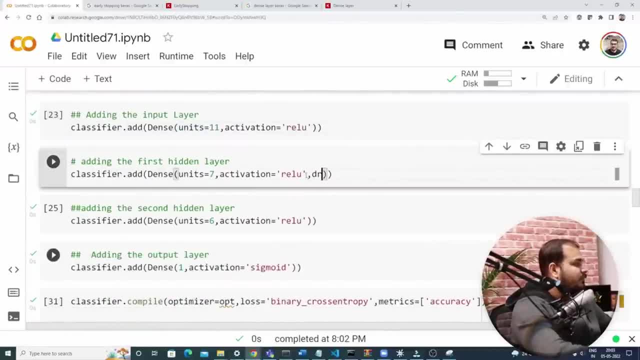 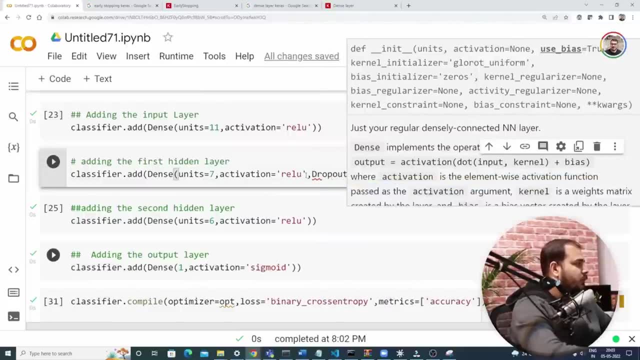 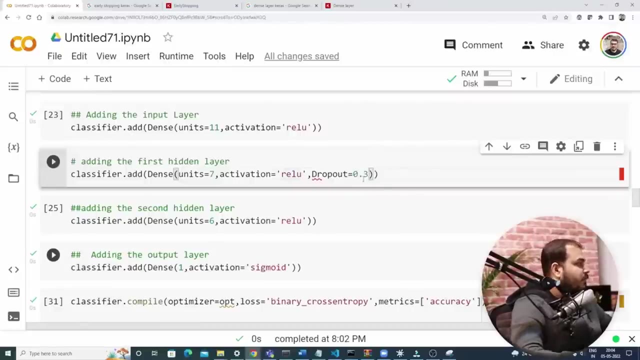 over here. over here, let's see, over here, can i write it. let's see, over here, can i write it. let's see, over here can i write it down: drop, dropout. if i say is equal to dropout. if i say is equal to dropout, if i say is equal to point three, right point three. 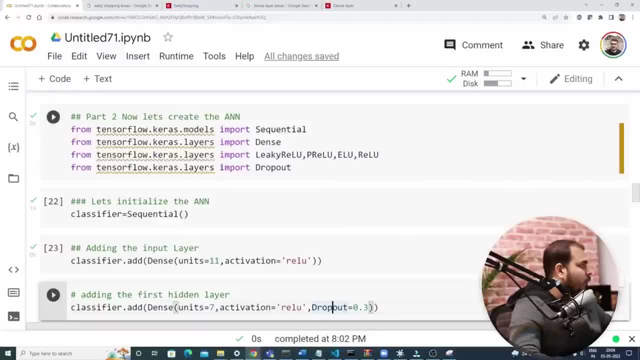 point three, right point three. point three, right point three. something like this: i think this should something like this, i think this should something like this. i think this should work, work, work. or let me just execute it from starting, or let me just execute it from starting, or let me just execute it from starting, so this gets executed, this gets. 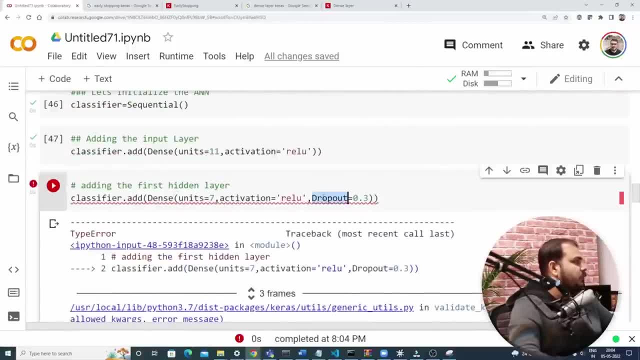 so this gets executed. this gets, so this gets executed. this gets executed, executed, executed. no keyword understood. no dropout fine. no keyword understood. no dropout fine. no keyword understood. no dropout, fine. let me just find out whether there is. let me just find out whether there is. let me just find out whether there is any dropout or not. 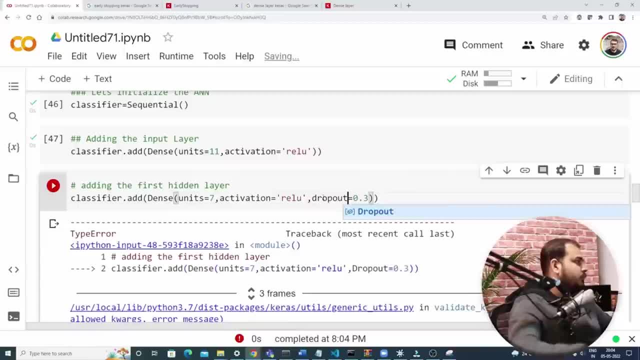 any dropout or not, any dropout or not. well, i can see you some examples. let's well, i can see you some examples. let's well, i can see you some examples. let's see, see see, um drop out, um drop out, um drop out. i think i did this. it's been very many. 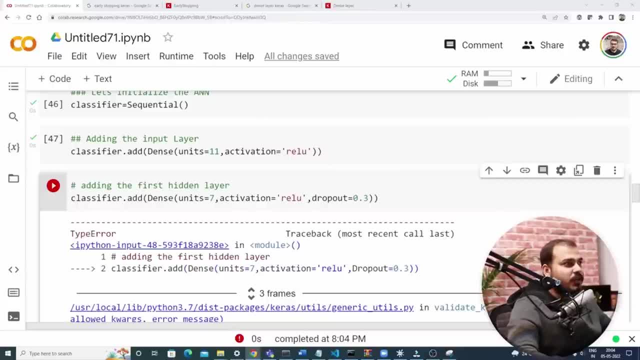 i think i did this. it's been very many. i think i did this. it's been very many days, i guess days. i guess days. i guess i'm just going to see the documentation. i'm just going to see the documentation. i'm just going to see the documentation of uh. 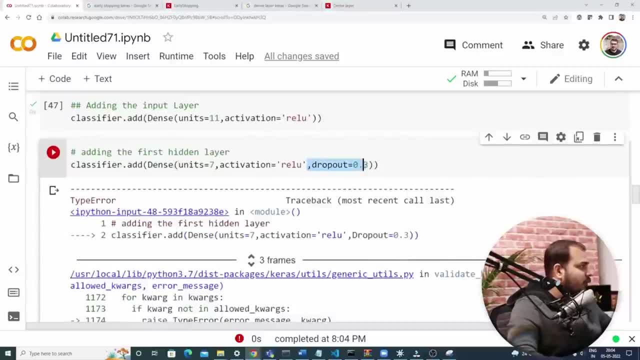 of uh, of uh, okay, okay, okay, okay, okay, got it, got it. got okay. okay, okay, okay, got it, got it. got okay. okay, okay, okay, got it, got it, got it. i think i don't have to add it over it. i think i don't have to add it over. 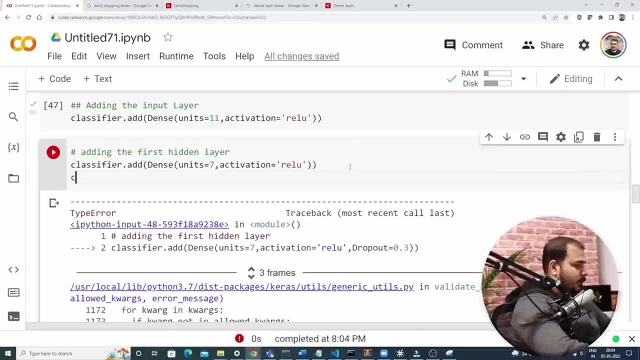 it. i think i don't have to add it over here here. here i can basically say: classifier dot, add dot, add dot, add something like this: dropout, something like this dropout, something like this: dropout. okay, okay, okay, drop out, drop out, drop out, because this is a layer. 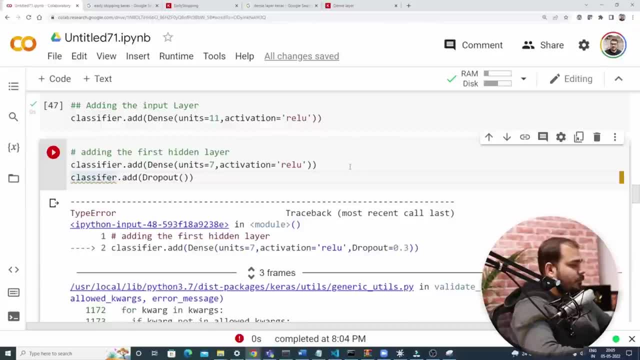 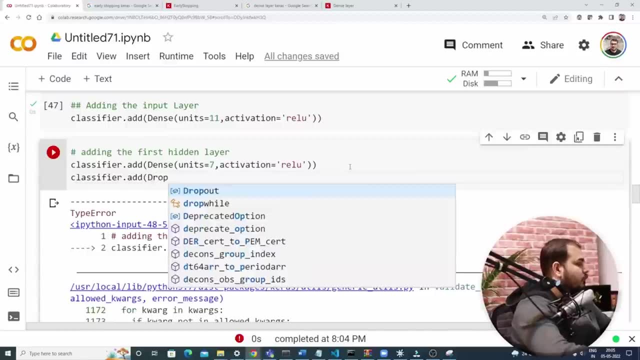 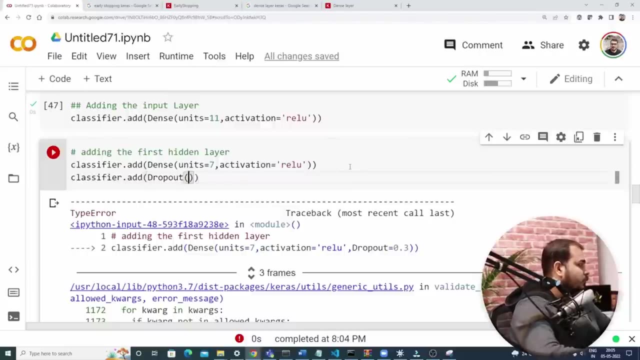 because this is a layer, because this is a layer, oops, oops, oops. classifier, classifier, classifier, dot, add, dot, add, dot, add. with respect to, with respect to, with respect to drop out, with respect to drop out, is equal to 0.3. let's see whether this: 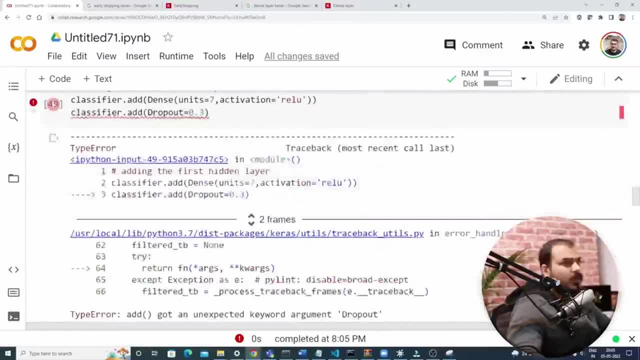 is equal to 0.3. let's see whether this is equal to 0.3. let's see whether this will get executed or not. will get executed or not. will get executed or not? no, still it is getting an error, but i. no, still it is getting an error, but i. 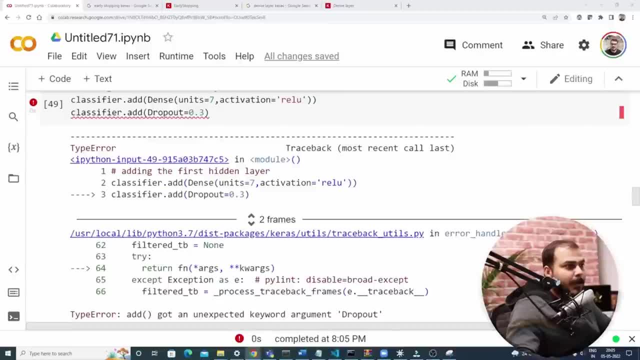 no, still it is getting an error, but i think this is what think, this is what think, this is what is the documentation saying: okay, perfect, okay, perfect, okay, perfect. i have to use this as a function. i have to use this as a function. i have to use this as a function. dropout. 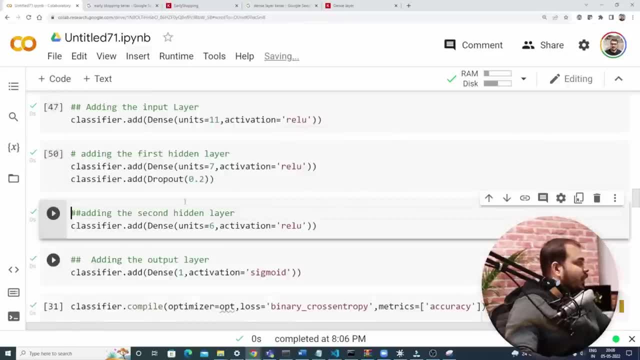 dropout. dropout like 0.2, something like this, like 0.2, something like this, like 0.2, something like this. okay, it is working. see so after every. okay, it is working. see so after every. okay, it is working. see so after every layer. 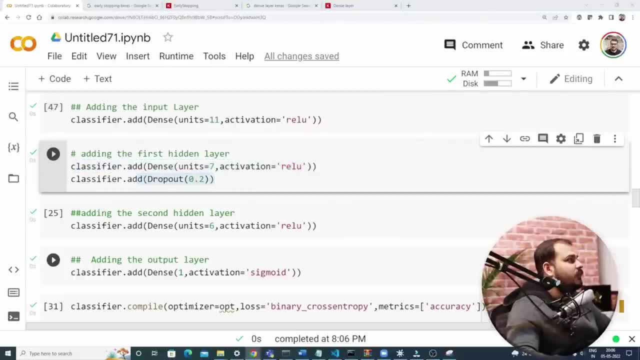 layer, layer. suppose if you write like this, see um. i suppose if you write like this, see um. i suppose if you write like this, see um. i actually got this entire information from, actually got this entire information from, actually got this entire information from the documentation, the documentation. 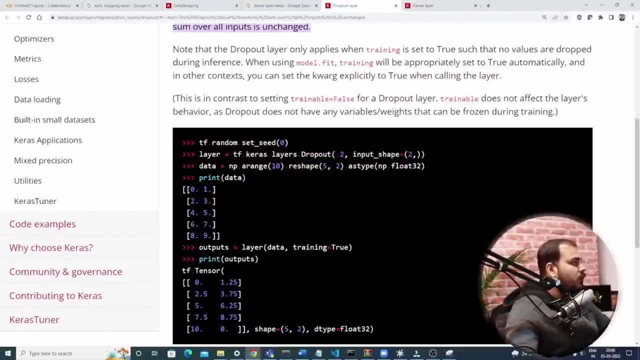 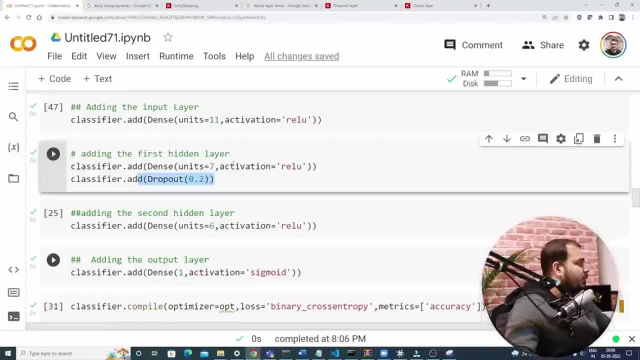 so when you write tf dot chaos, dot layer, so when you write tf dot chaos, dot layer, dot dropout as point two, you will be able dot dropout as point two, you will be able dot dropout as point two, you will be able to see this. okay, so here you can. 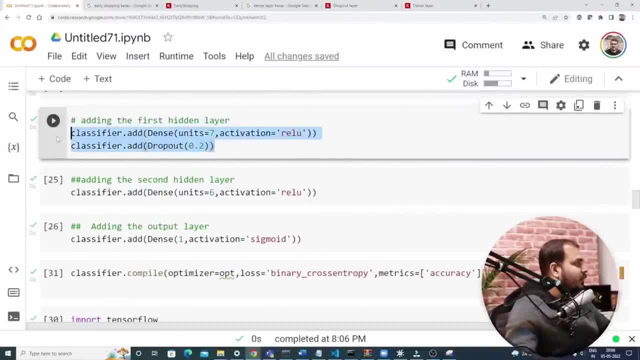 to see this. okay, so here you can. to see this. okay. so here you can basically use dropout in every layer. basically use dropout in every layer. basically use dropout in every layer, after every layer, let's say over here at. after every layer, let's say over here at. 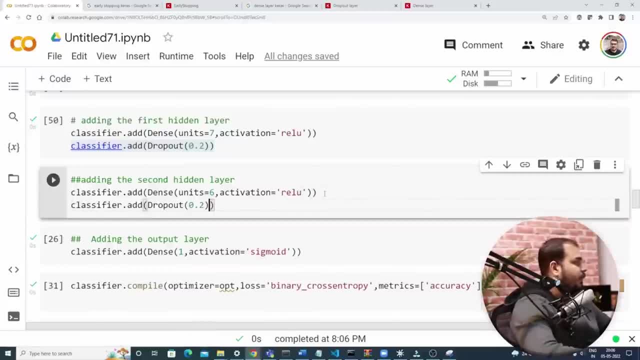 after every layer, let's say, over here at 20: 20, 20 over here, 30 right over here, 0.3 over here, 30, right over here, 0.3 over here, 30 right over here, 0.3 over here. everything as such you will be. 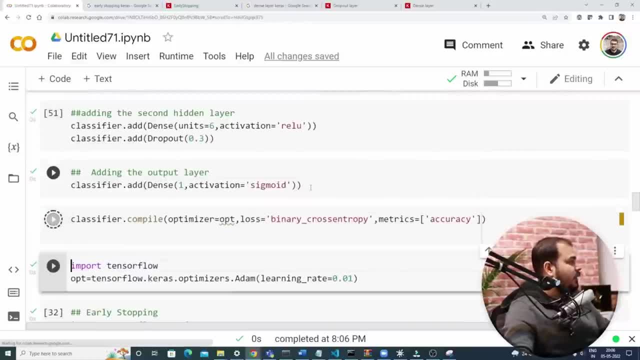 over here, everything as such. you will be over here, everything as such. you will be able to write it down, able to write it down, able to write it down and then create it and then execute it, and then create it and then execute it, and then create it and then execute it, then execute it, then execute it. 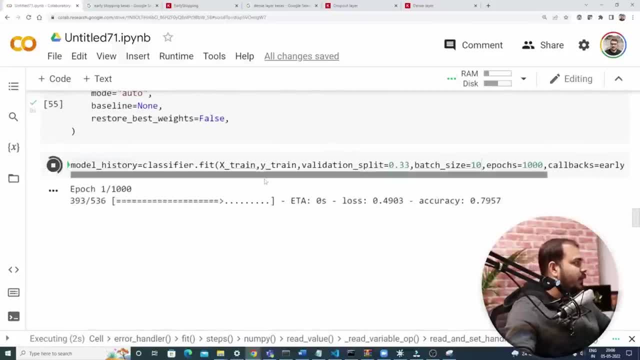 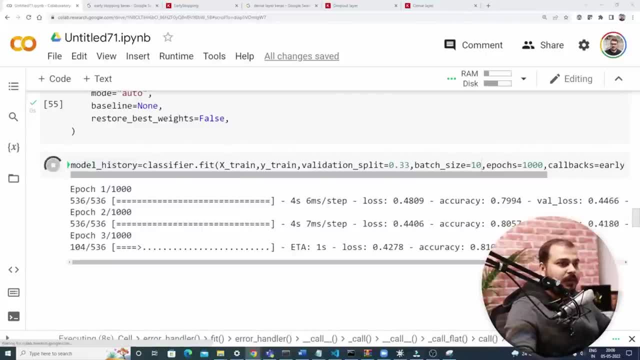 run and you will be able to get the run, and you will be able to get the early stopping and, based on that, it will early stopping and based on that, it will early stopping and based on that, it will be working fine. be working fine, be working fine, right, okay, perfect. 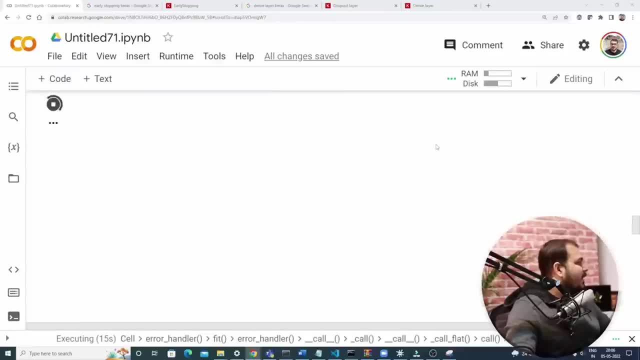 right, okay, perfect, right, okay, perfect. you all are amazing, you all are amazing. you all are amazing, okay, uh, so i hope you have got an idea. okay, uh, so i hope you have got an idea. okay, uh, so i hope you have got an idea till here. uh, you can also save the model. 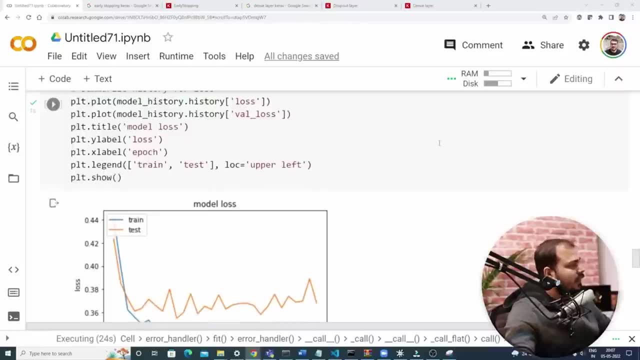 till here. uh, you can also save the model till here. uh, you can also save the model by using pickling or the h5 format by using pickling or the h5 format, by using pickling or the h5 format, and many things you can actually do do. 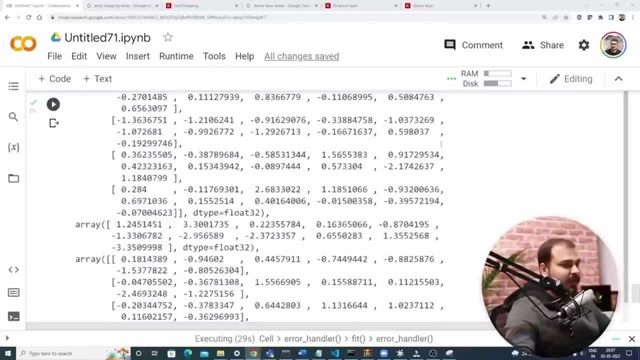 and many things you can actually do do and many things you can actually do: do the prediction, you do the scoring, the prediction, you do the scoring, the prediction, you do the scoring. everything i've actually explained you everything. i've actually explained you everything. i've actually explained you okay. 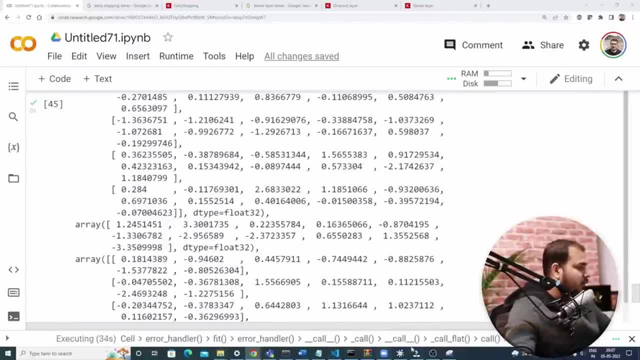 okay, okay, now, uh, the one thing that you can now uh, the one thing that you can now uh, the one thing that you can basically do, is that basically do, is that basically do, is that i'll just open one more thing, and let's i'll just open one more thing, and let's. 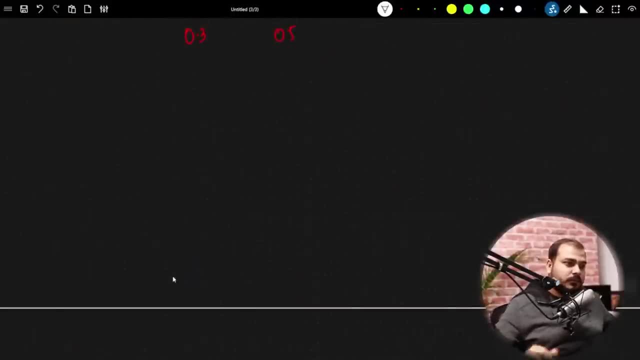 i'll just open one more thing, and let's talk about one, two important things. one: talk about one, two important things. one talk about one, two important things. one is: black blocks model. black black box model, black box model, black box model versus white box. now, guys, this black box versus white box. 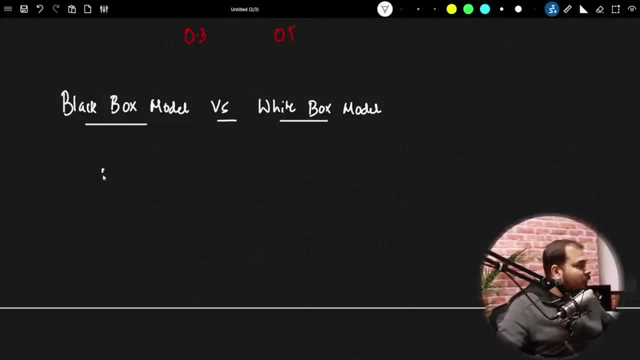 now, guys, this black box versus white box. now, guys, this black box versus white box. model right, it is quite important to model right. it is quite important to model right. it is quite important to understand. if i say complex algorithm, understand if i say complex algorithm, understand if i say complex algorithm like random forest, can anybody 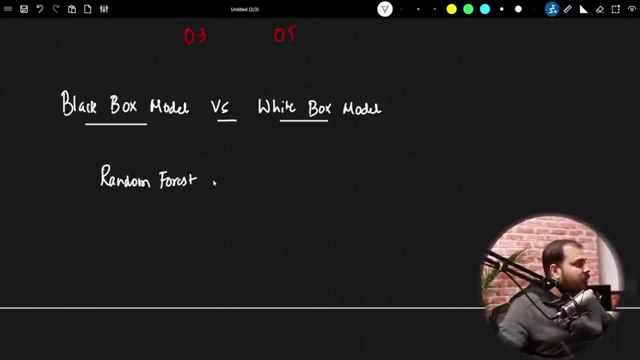 like random forest. can anybody like random forest? can anybody tell me or write down in the comment: tell me or write down in the comment. tell me or write down in the comment: saying that, which, saying that, which, saying that, which model this will be, whether this is a. 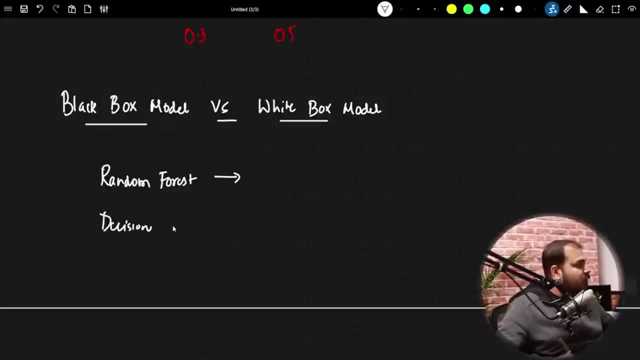 model. this will be whether this is a model. this will be whether this is a black box or a white box, black box or a white box, black box or a white box, if it is decision tree, whether this is a. if it is decision tree, whether this is a. 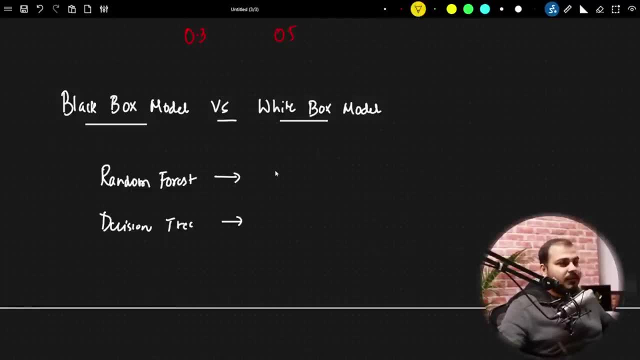 if it is decision tree, whether this is a black box or white box, right black box or white box, right black box or white box, right? so just tell me, write down in the comment. so just tell me write down in the comment. so just tell me write down in the comment and basically, 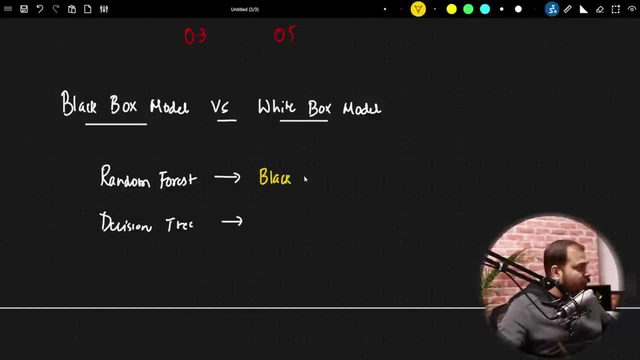 and basically, and basically see it what it is. so this is basically see it what it is. so this is basically see it what it is. so this is basically a black box model, a black box model, a black box model. this is actually a white box model, right? 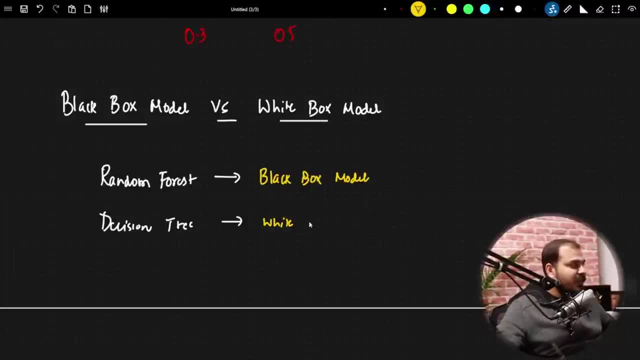 this is actually a white box model, right? this is actually a white box model, right? because here in decision tree whenever, because here in decision tree whenever, because here in decision tree whenever, use this kind of algorithm, we can use this kind of algorithm. we can use this kind of algorithm. we can definitely see it. 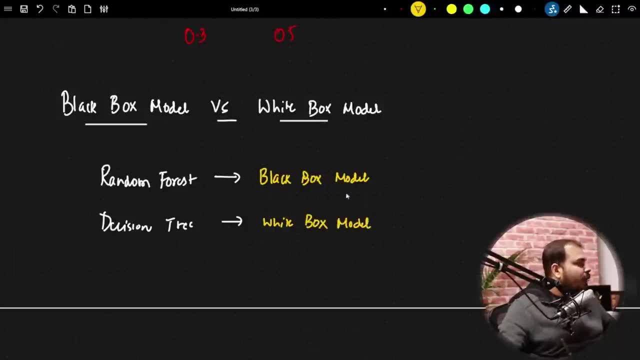 definitely see it, definitely see it. so here i will say that: okay, this is my. so here i will say that: okay, this is my. so here i will say that: okay, this is my white box model, white box model, white box model. okay. and suppose, if i say that, okay, let's. okay, and suppose, if i say that okay, let's okay. and suppose, if i say that okay, let's, let's discuss about what about? let's discuss about what about? let's discuss about what about? a and n, whether this is white box or a and n, whether this is white box or. 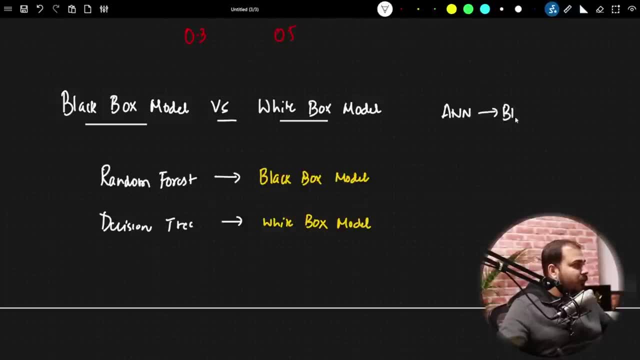 a and n, whether this is white box or black box, this will also be black box, this will also be black box. this will also be a black box model right. because a black box model right? because a black box model right? because obviously we cannot monitor and see all. 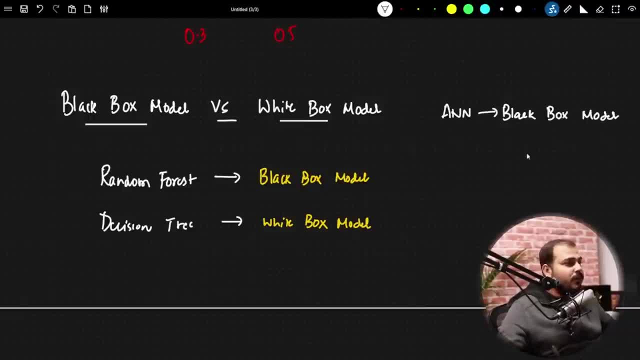 obviously we cannot monitor and see all. obviously we cannot monitor and see all the weights. it is very difficult, the weights, it is very difficult, the weights. it is very difficult. uh, it is very, very difficult because we uh, it is very, very difficult because we uh, it is very, very difficult because we cannot just directly see. 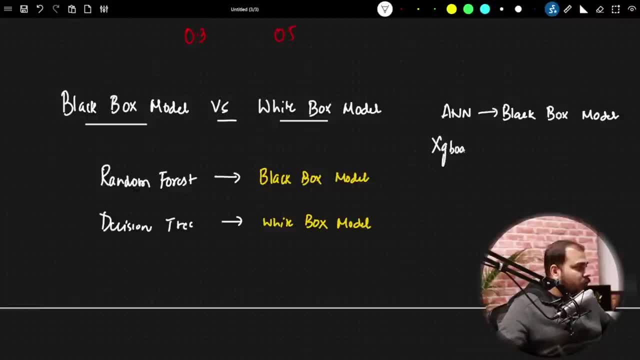 cannot just directly see. cannot just directly see how it is working internally right. if i how it is working internally right. if i how it is working internally right. if i probably talk about xg boost, how many probably talk about xg boost? how many how it is working internally right. if i probably talk about xg boost, how many decision trees are used? 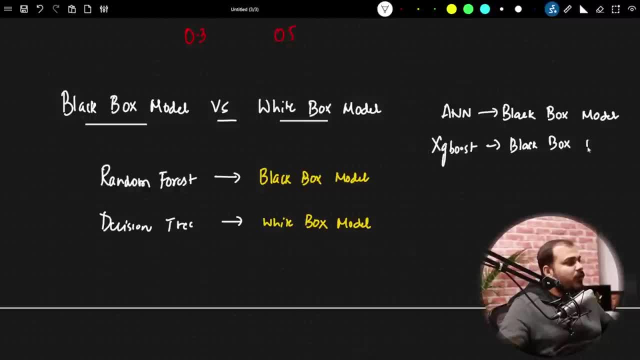 decision trees are used. decision trees are used. this is also a kind of black box model. this is also a kind of black box model. this is also a kind of black box model, right, if i probably talk about linear, right, if i probably talk about linear, right, if i probably talk about linear regression, that is fine, linear regression. 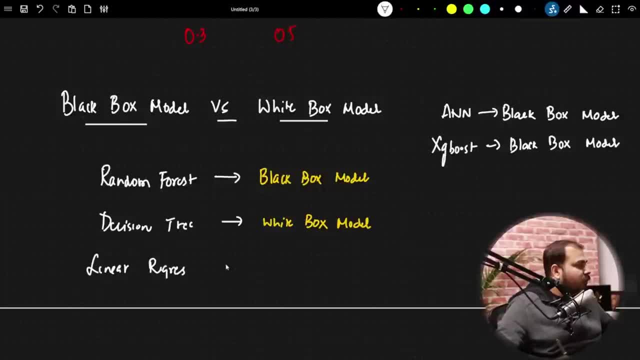 regression- that is fine linear regression. regression- that is fine linear regression. we can definitely see many things. we can definitely see many things. we can definitely see many things. uh, and this becomes a white box model. uh, and this becomes a white box model. uh, and this becomes a white box model. right, so this becomes a white box model. 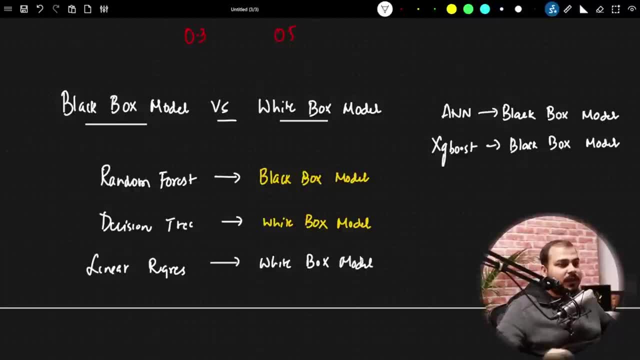 right, so this becomes a white box model. right, so this becomes a white box model. so internal working and all it is very so internal working and all it is very so internal working and all. it is very difficult to check out in some of the difficult to check out in some of the 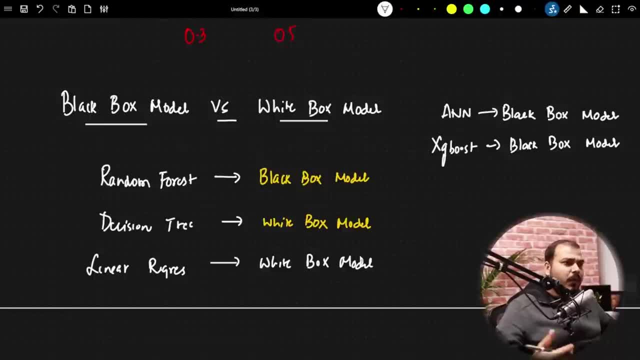 difficult to check out in some of the algorithms because it is quite huge algorithms, because it is quite huge algorithms, because it is quite huge, quite big you know, and how internally quite big you know, and how internally quite big you know and how internally how much it works, because in random 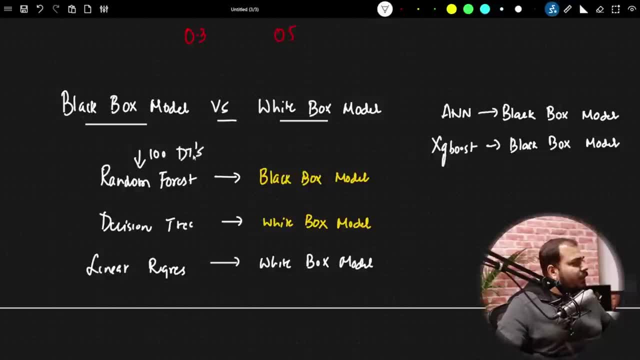 how much it works because in random. how much it works because in random forest. let's say we are taking forest. let's say we are taking forest. let's say we are taking hundred decision trees. right, it is very hundred decision trees, right, it is very hundred decision trees, right. it is very difficult to monitor each and. 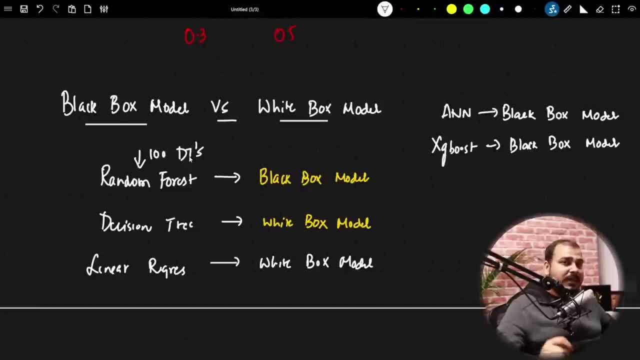 difficult to monitor each and difficult to monitor each and everything, and we cannot do that we everything. and we cannot do that we everything. and we cannot do that. we cannot see each and everything, cannot see each and everything clearly right, whereas in the case of a clearly right, whereas in the case of a. 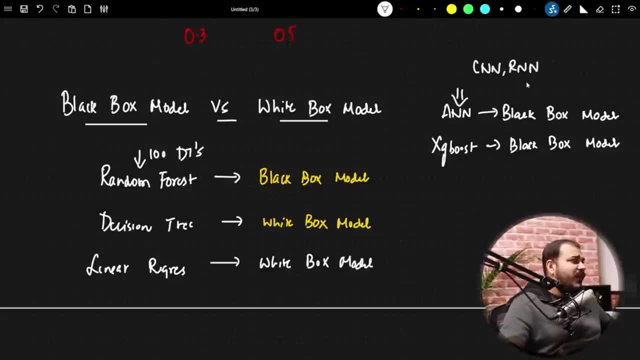 clearly right, whereas in the case of a and n, let's say cnn and n, let's say cnn and n let's say cnn. rnn right, these all are very difficult. rnn right, these all are very difficult, rnn right, these all are very difficult. so we, we can see up to some level, but 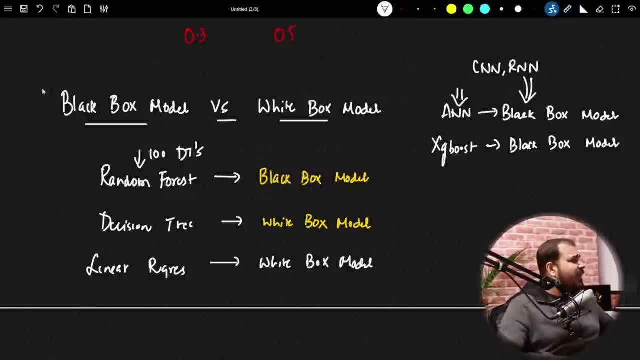 so we, we can see up to some level, but so we, we can see up to some level, but definitely we can't see everything right. definitely we can't see everything right. definitely we can't see everything right. so this is again another important, and so this is again another important, and 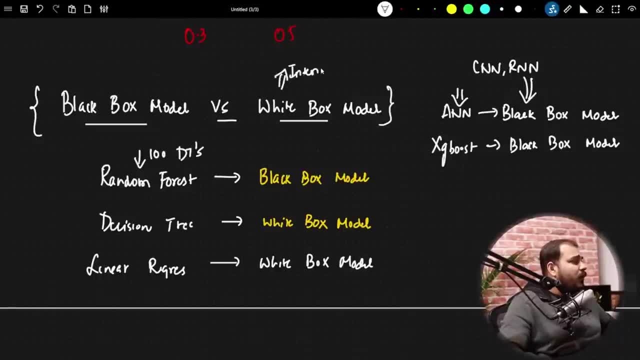 so this is again another important and interview question that everybody should interview, question that everybody should interview, question that everybody should know, uh, you know, and because of that, know, uh, you know, and because of that, know, uh, you know, and because of that, there is one amazing thing which is: 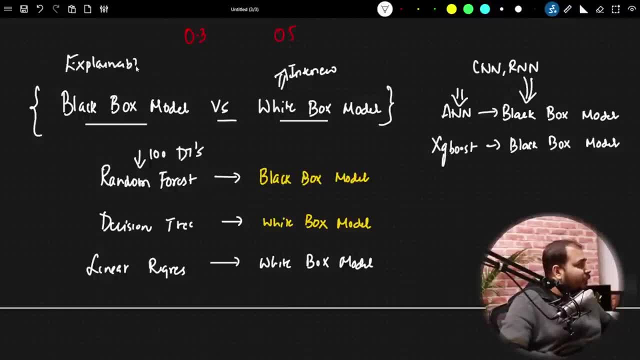 there is one amazing thing which is: there is one amazing thing which is called as explainable ai, called as explainable ai. called as explainable ai. this is also becoming very, very popular. this is also becoming very, very popular. this is also becoming very, very popular because people want to come up with some. because people want to come up with some, because people want to come up with some kind of tool which will be able to kind of tool which will be able to kind of tool which will be able to monitor the model how the model is, monitor the model, how the model is. 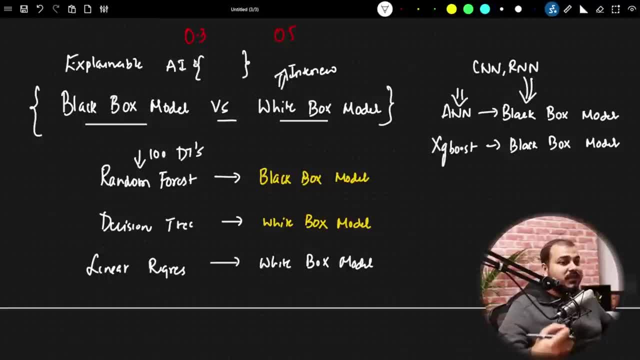 monitor the model, how the model is basically performing with respect to each basically performing with respect to each basically performing with respect to each and every input feature. this thing is, and every input feature. this thing is, and every input feature. this thing is going on as a research, okay, and that is. 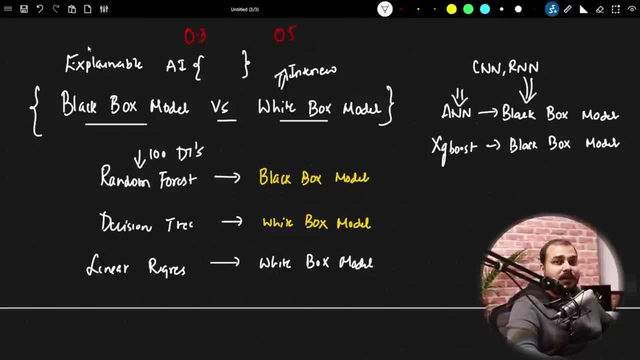 going on as a research, okay, and that is going on as a research okay, and that is what we are going to see in the upcoming, what we are going to see in the upcoming, what we are going to see in the upcoming days, like people are able to create some. 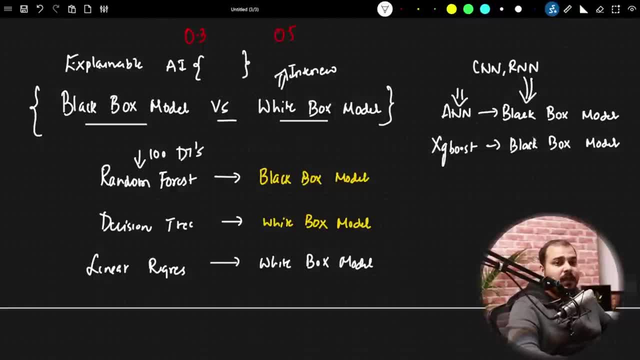 days like people are able to create some days like people are able to create some amazing explainable algorithm. which will amazing explainable algorithm, which will amazing explainable algorithm which will be able to monitor the algorithms, be able to monitor the algorithms, be able to monitor the algorithms properly, right? so i hope you like this. 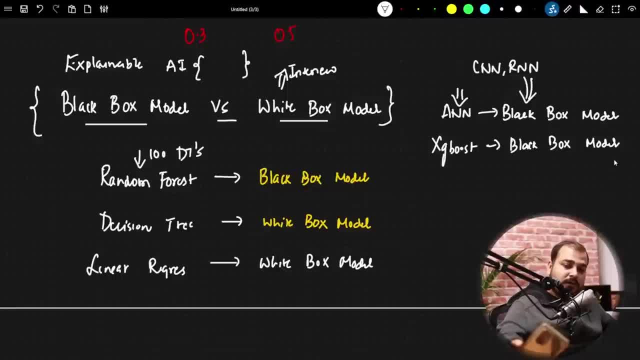 properly, right, so i hope you like this properly, right. so i hope you like this particular video. i hope you like this particular video. i hope you like this particular video. i hope you like this. session tomorrow we are going to cover. session tomorrow we are going to cover. 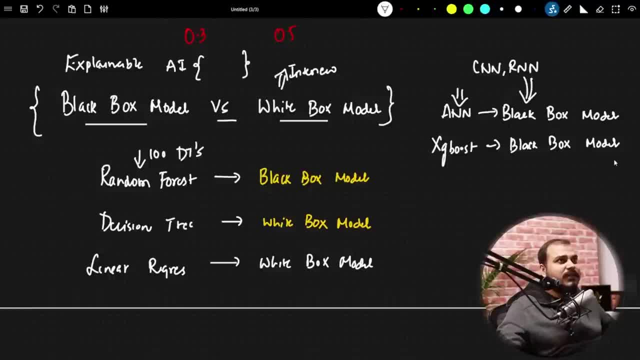 session tomorrow we are going to cover cnn guys and cnn guys and cnn guys and after that, uh, let's conduct on the after that. uh, let's conduct on the after that, uh, let's conduct on the second or the third week. we will try to. second or the third week, we will try to. 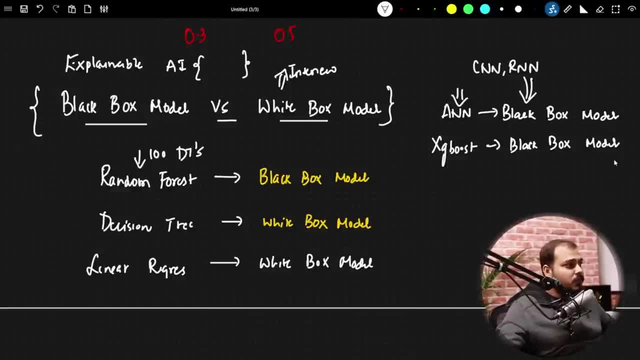 second or the third week, we will try to cover nlp. where will i'll be covering cover nlp? where will i'll be covering cover nlp? where will i'll be covering rnn? okay, so tomorrow i my main plan is rnn. okay, so tomorrow i my main plan is: 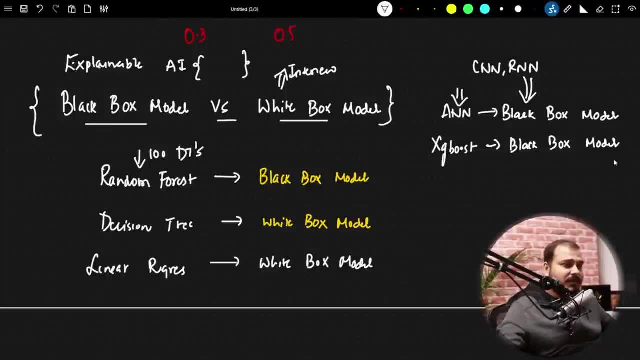 rnn. okay, so tomorrow i my main plan is to cover uh, to cover uh, to cover uh cnn and see one practical example: uh, cnn. and see one practical example. uh, cnn, and see one practical example. uh, and yes, in the next session we will be. and yes, in the next session we will be. 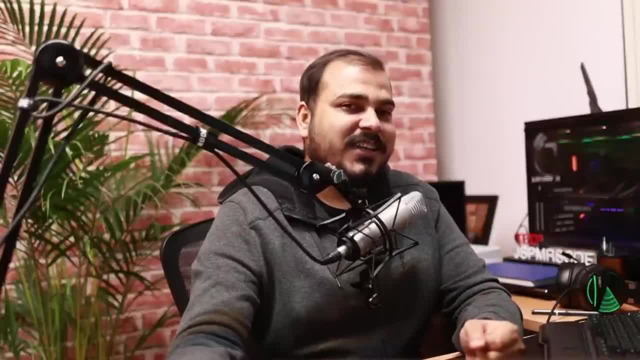 and yes, in the next session we will be discussing about rnn and all discussing about rnn and all discussing about rnn and all. and uh, yes, i'll see you all in the next. and uh, yes, i'll see you all in the next. and uh, yes, i'll see you all in the next session. have a great day. 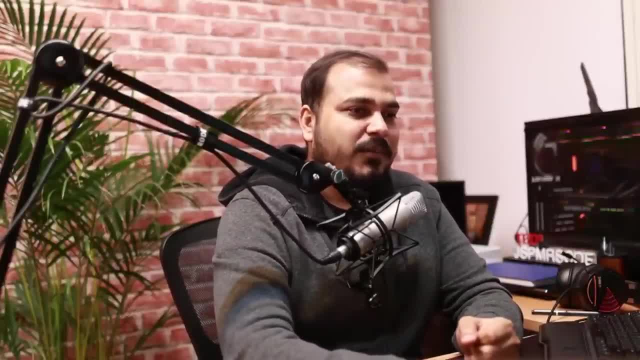 session. have a great day session. have a great day. i'll see you tomorrow where we'll be. i'll see you tomorrow where we'll be. i'll see you tomorrow where we'll be discussing about cnn, discussing about cnn, discussing about cnn. uh, keep on rocking, keep on learning and 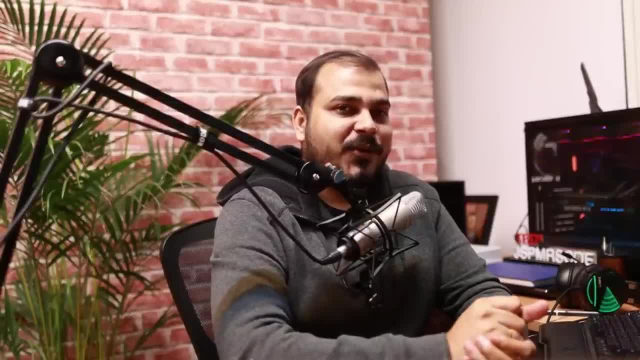 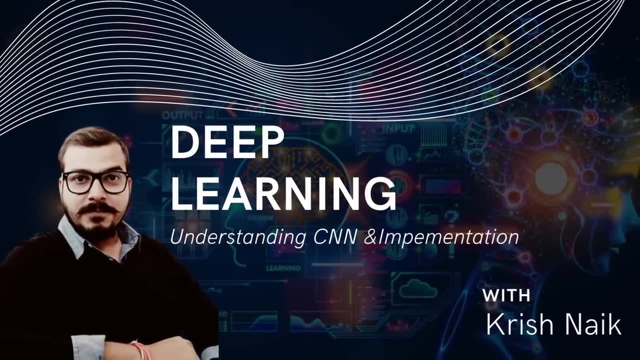 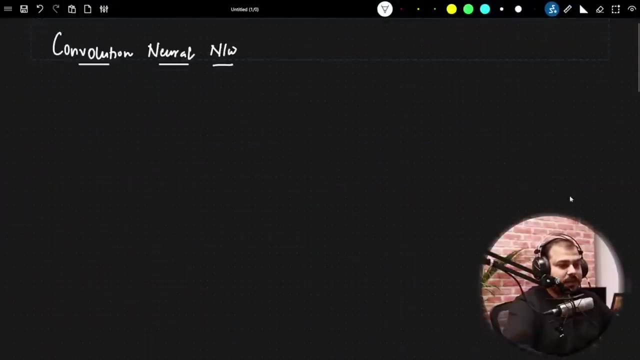 uh, keep on rocking, keep on learning. and uh, keep on rocking, keep on learning. and yes, yes, yes, have a great day ahead. thank you on it. have a great day ahead. thank you on it. have a great day ahead. thank you on it all. bye-bye today. uh, we are going to discuss about it. 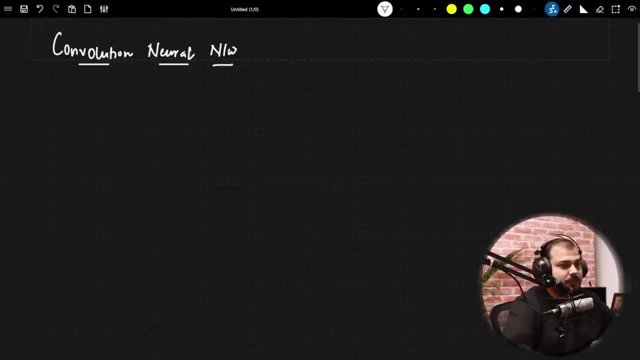 today. uh, we are going to discuss about it today. uh, we are going to discuss about it and yes, uh and yes, uh. how does CNN work? and then we'll try to do the implementation. as you all know, we have already discussed about ANN. now we have seen the theoretical explanation. 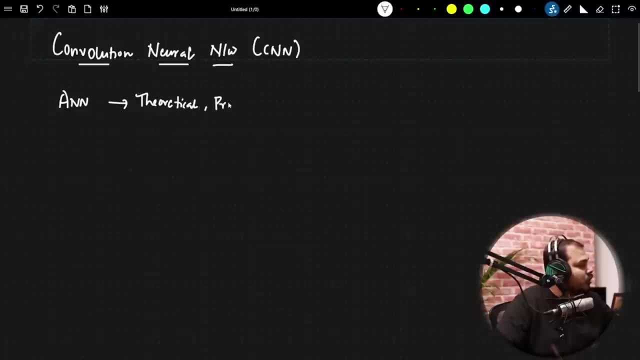 right. and then we also saw the practical part and when we were discussing about optimizers, loss functions and all the things in this. but in today's session, in this session we are going to discuss about CNN. CNN will focus on understanding what exactly is convolution- neural network convolution. 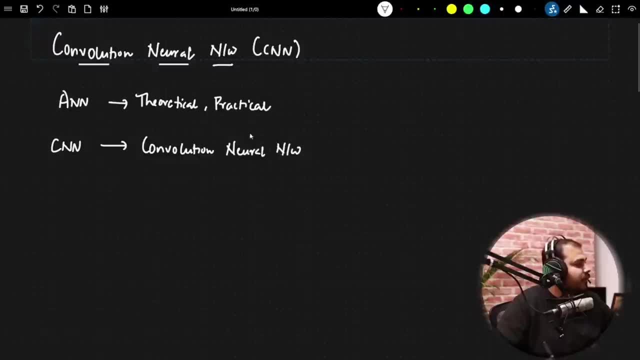 neural network and how specifically it works. whenever we talk about convolution neural network, we are basically going to mostly discuss about images and, let's say, video frames, right? so whenever we have images- and probably we want to work with that, you know, you know we want to work with that, you know. 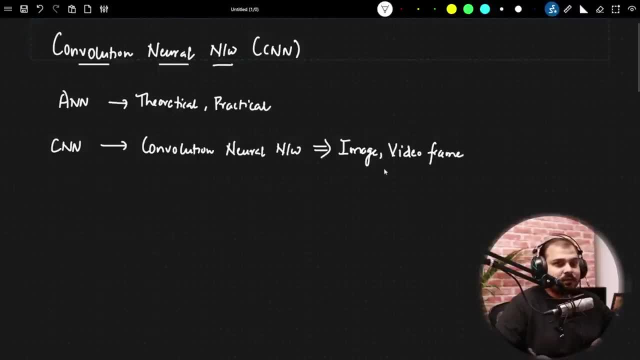 specifically related to, you know, different kind of images itself, some of the tasks like image classification, object detection, which we specifically used, a different kind of CNN networks which are focused more on detecting objects in a specific images or videos itself. right, so, as as usual, the agenda will be that we will try to divide this entire topics in understanding, first of, 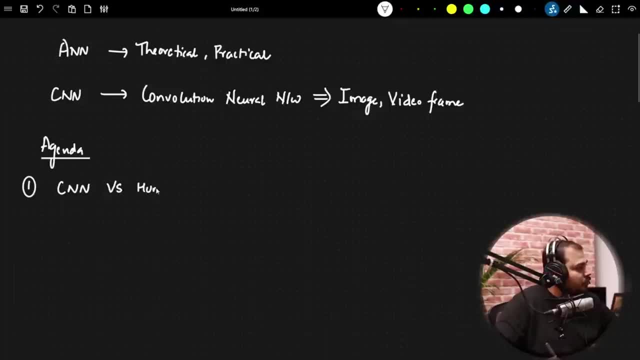 all we'll try to understand about CNN versus human brain. okay, because this is really in sync, like how human brain works. this entirely mimics that specific part and based on that, we will be learning some internal amazing techniques that are included in CNN. if I talk about second topic, first of all we'll be 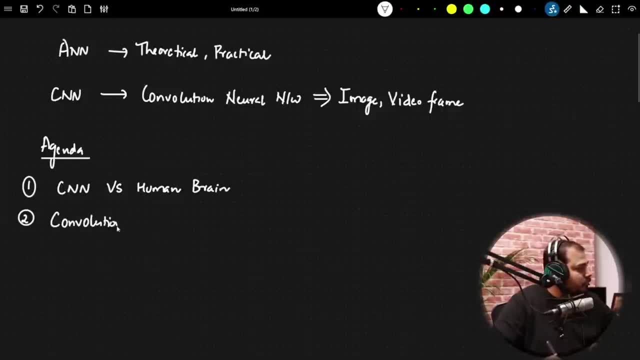 discussing about convolution operation, convolution operation. in this convolution operation, we are going to discuss about various, various words that I'm going to bring up over here, like: what is convolution? okay, what is padding? what is strides? right, we will be discussing this, you know, and how do we? 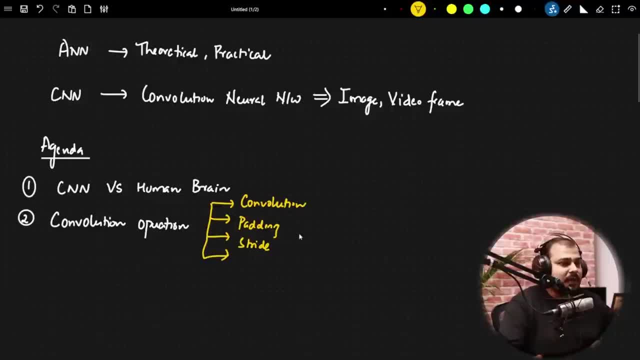 determine that how the output of a specific image will look like after we pass through this filters. filters are also called something called as kernels. okay, so we'll also be discussing about this specific thing as we go ahead. once we complete this two, then we will be discussing. 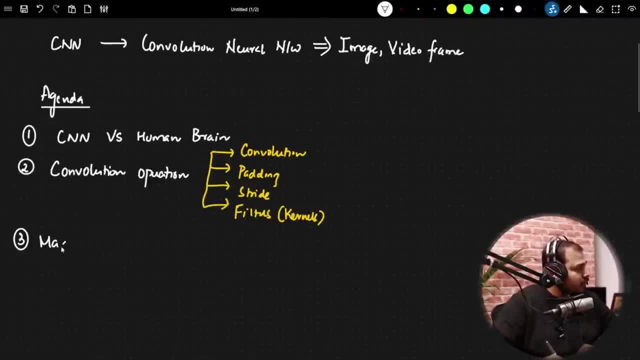 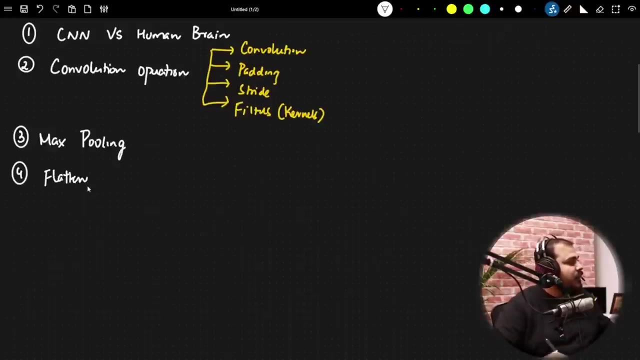 about the third part, which is called as max pooling, and in max pooling we will try to understand what is the importance of max pooling itself. in the fourth topic, we'll understand about the flattened layer, which is again one amazing thing that happens in the final layer of the cnn. 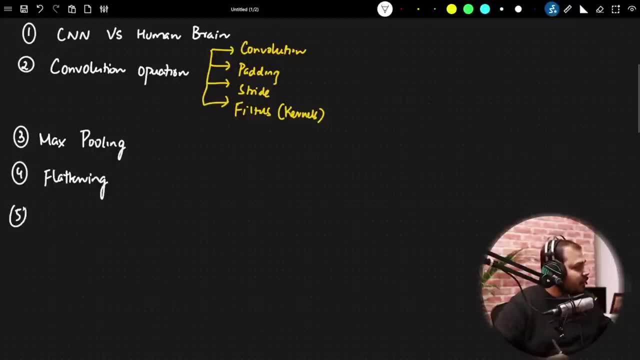 itself, so we specifically call it as flattening. and in the fifth part we are going to see the practical implementation. okay, how do we implement the cnn? okay, practical implementation. so these all things we are going to cover, and we are going to cover and make sure that we understand each and. 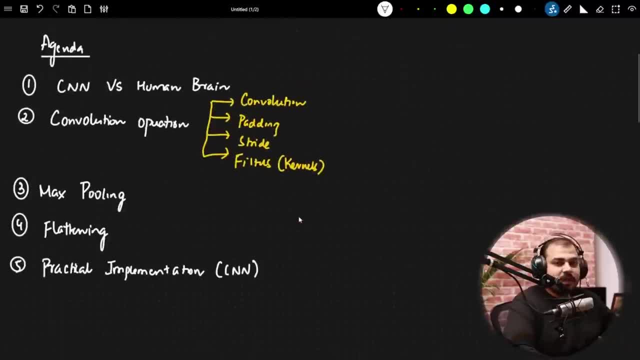 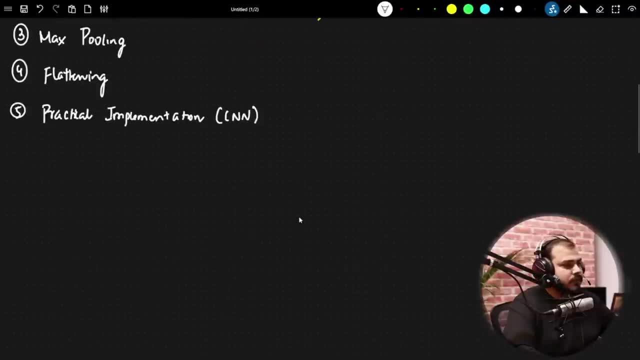 everything. okay now, this is the entire agenda of this session and we'll try to cover up all of these things. okay, and again, let's start with understanding cnn versus human brain, right versus human brain, now human brain always understand. how does it work, you know, like, suppose i am seeing a specific object. okay, suppose let's say that i'm 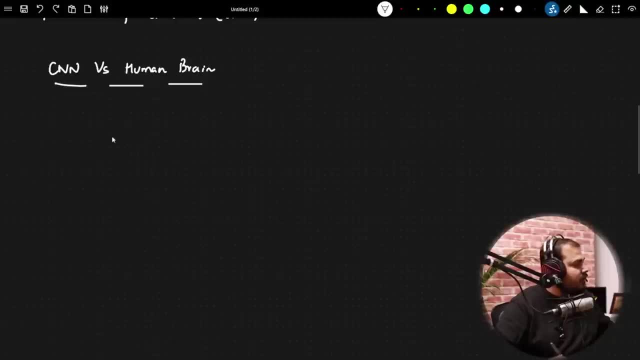 seeing a cat, okay, i'm seeing a cat. or let's say, in a specific image: right, i may have various objects, i may have cat, i may have dog- okay, i may have a bicycle- okay, i may bicycle. i may have a car and i may have a human being- okay. now, in this specific 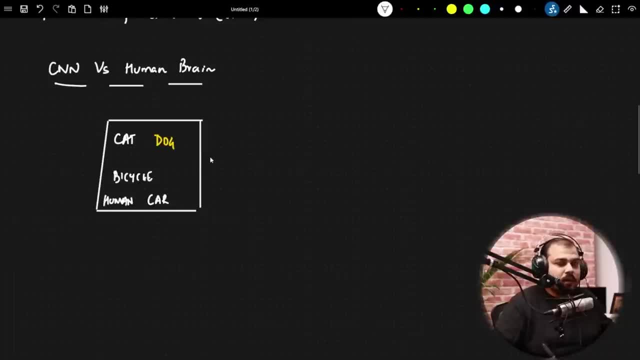 image. let's say that we have so many things over here right now, specifically as a human being, right, when i am specifically seeing an object, right, i may find out many things. right, i may see a person moving, i may see an animal over there, i may see a bird flying. so many details is getting processed in my brain itself, right. 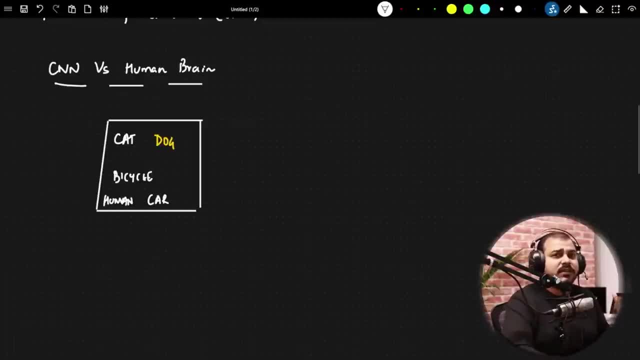 and because of that, because of that crossing, i'm able to understand a lot of things: the major part of the brain which we specifically call as cerebral cortex right, the cerebral cortex which is in the back side of this brain, in this back side, you know, and in this part, only you know. 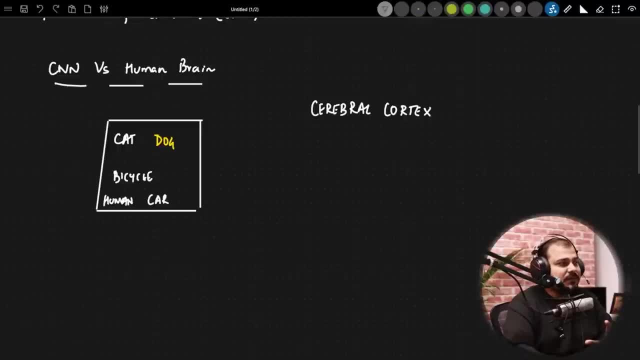 there is a place, what there is a part of this specific brain which we call it as visual cortex. okay, visual cortex, which is specifically responsible for seeing any items that are there, any objects that are there in a specific image or in a video. okay, now, this is a specific place in the brain and we call it the cerebral cortex in this particular 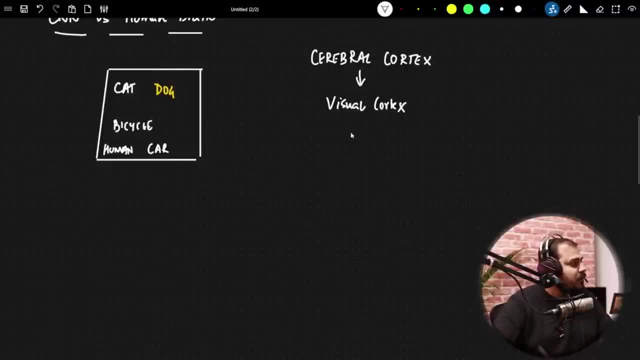 visual cortex may it may have many layers. okay, suppose let's say that if i probably talk about this visual cortex, it may have layers like let me name this layer at v1, v2, v3, v4, v5, v6 and let's say v7. i'm just, i'm just creating some layers. you know, like this, there may be many layers, but i'm just 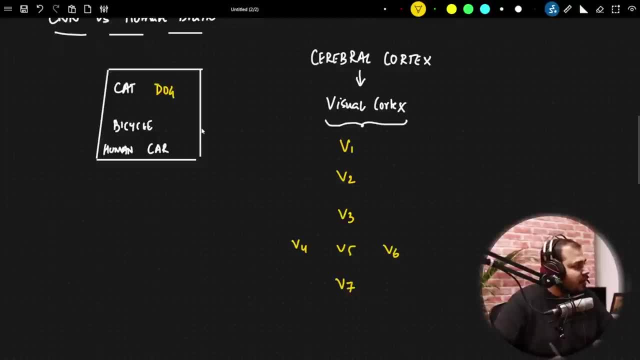 going to define some of the layers like this now, as soon as this input passes through each and every layer you know, let's say, this layer is responsible in understanding or in in basically seeing the moving objects. so when it passes through this layer, we will be able to determine that. okay, fine. 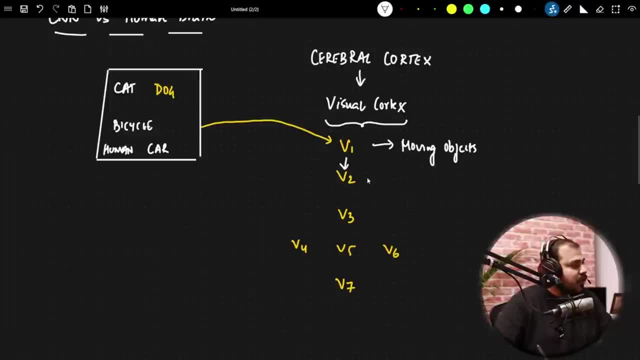 there is some moving object that is going on, then when we go to the next layer- over here- right, let's say over here we are able to, we are able to understand some of the animals, right, like cat, dog or something right. so over here will be able to understand some of the animals you know- when then, as it passes through this layer and 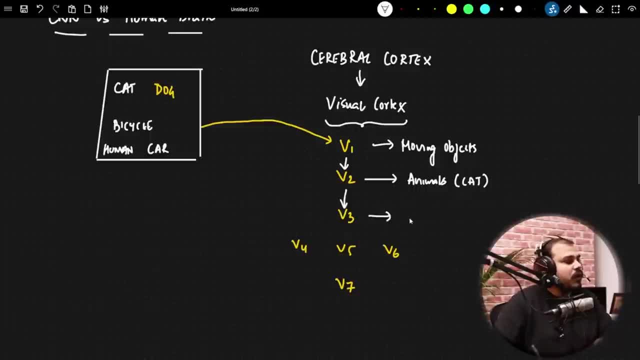 goes to the v3 layer. let's say, and this is responsible for doing some other task, you know, here we are able to map the environment. let's say some functionalities, map the environment, right, you are able to visualize the entire environment. so something is happening in each and every layer. 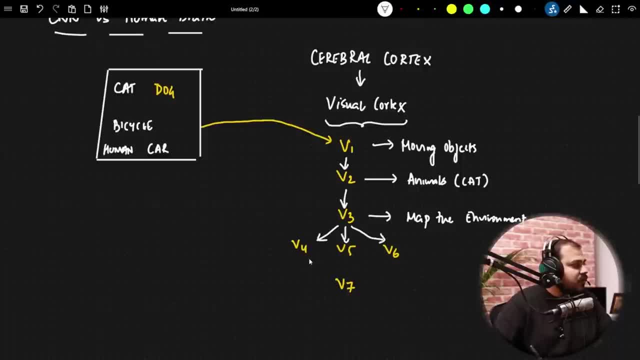 you know, and finally, all this information, when it is passed, we will be able to visualize this specific image over here, and then we are able to understand some of the animals. you know when, then, this v7 layer, which is the part of visual cortex. okay, so by this you are able to finally find out. 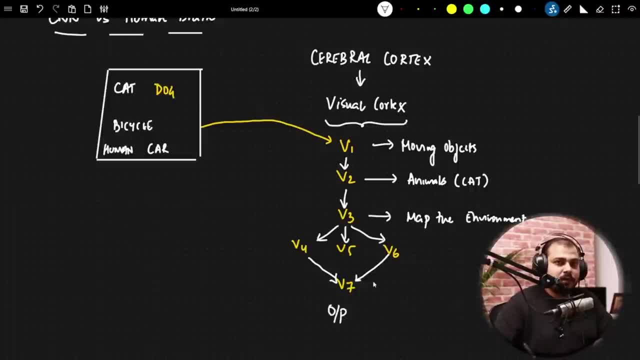 the output over here after so many processing, right? similarly, if i talk about convolution, neural network, right, it should be also able to do this many number of different kind of processing. but now the thing rises: is that how we can make sure that probably whatever cnn we are trying? 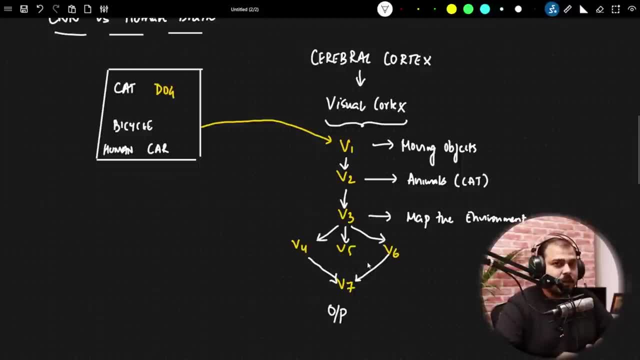 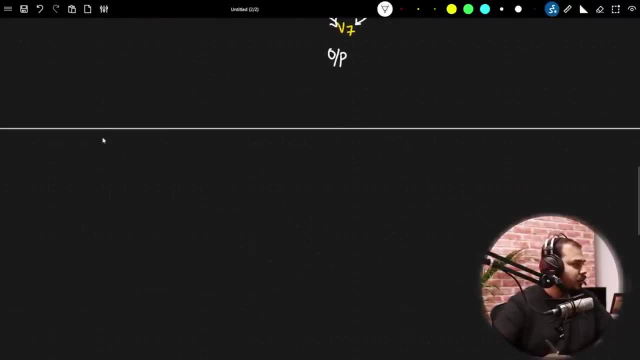 to develop, it should also be able to do all this kind of task. okay, so let's go ahead and understand. so the first thing with respect to cnn: when, when i probably discuss about cnn, you know we will divide this into multiple steps. the first step of operation, which is called as convolution. 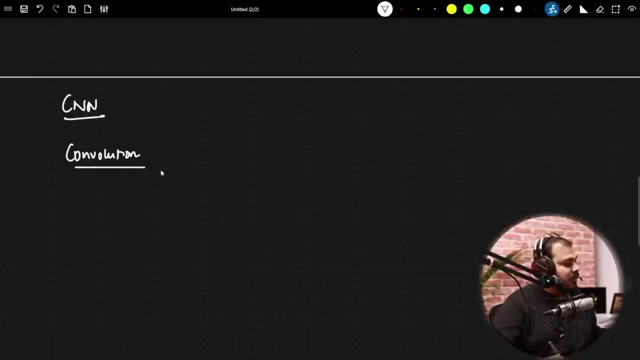 now, what exactly is convolution? before we go ahead and understand about convolution, we need to understand some of the basic information about the images, right? so what are specifically images? right, what are images? suppose you click your photo, right? so let's say: this is your photo, okay, and it has specific, some kind of pixels. let's say so, let's. 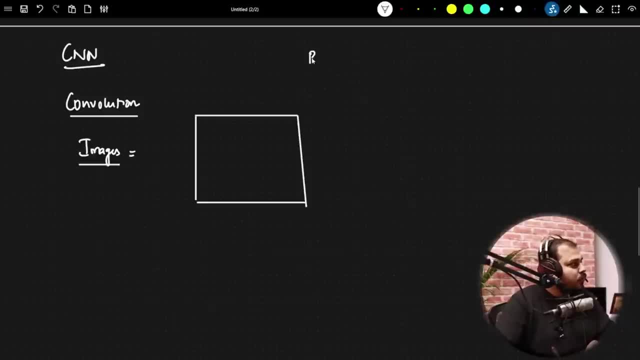 say that this is a photo, and whenever you have a photo, there are two types of focus. one is black and white and one is rgb type and the other one is something called as rgb type. in black and white, you just have a single channel. okay, that basically means your, your entire photo will either be: 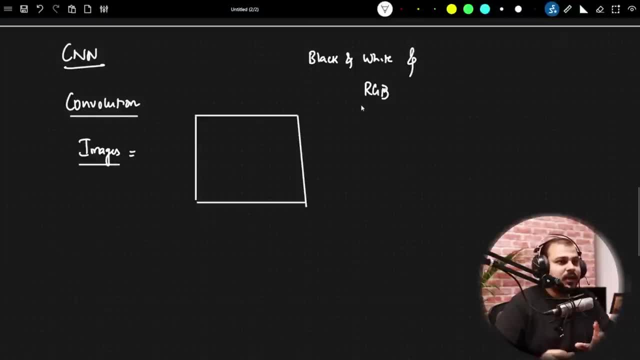 mostly the component of a black color or white color, something like that. okay, so here in, in black and white, in this right, you just have a single channel, one channel, okay, and whenever we divide these images, we divide by some kind of pixels, let's say, if i probably 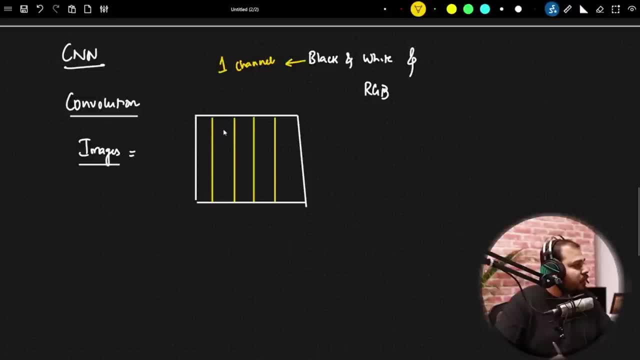 create this kind of line right. so over here let's say one, two, three, four, five. so in the width and height let's say there are five different different pixels. okay, so let's say, if i want to probably call this image, it will be five cross five pixel image. 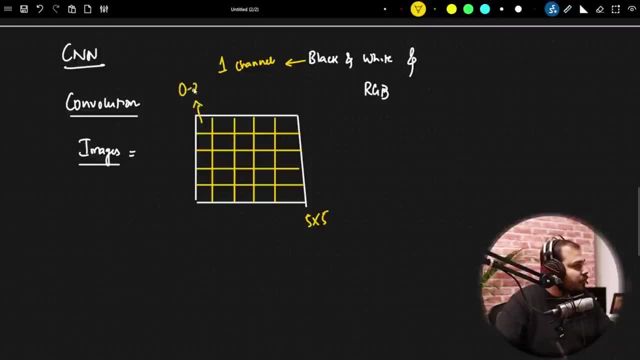 okay, and here each and every pixel will be ranging between zero to 255. right, if i specifically talk about mostly, zero is nothing, but it is a black color. okay, so let's say 0 is a black color and 255 is actually a white color. let's say: 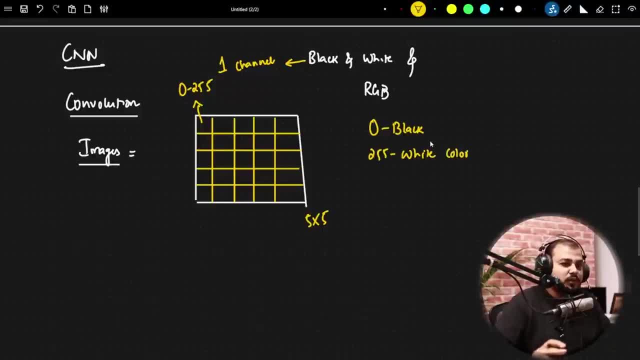 white color. all these values if your value is ranging between 0 to 255, so every pixel may have different, different values based on the image composition. right over here you you may probably have 40,. over here you may have 0,. here you may have 255,. here you may. 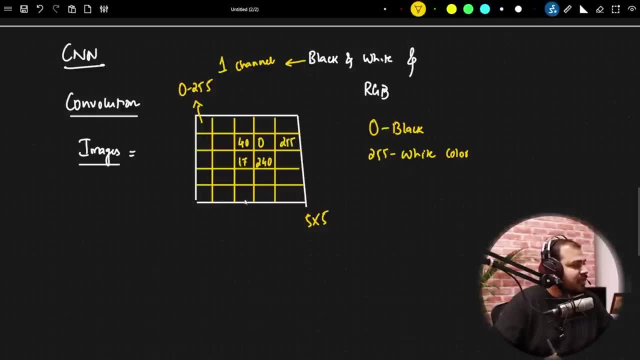 have 240, here you may have 17,. like this, each and every values are there, So this is basically called as a 5x5 pixel image, and in each pixel your value will be ranging between 0 to 255 in a single channel. 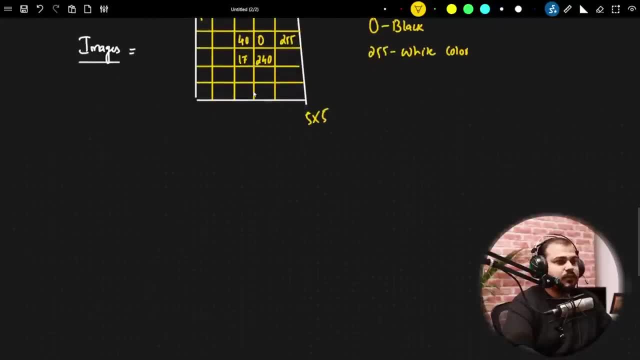 Now with respect to a RGB image, which is a colored image. so suppose, if I probably consider an RGB image Now, how does an RGB image look like Here? let's say we will be having 3 channels: one is the R channel, the R channel and this. 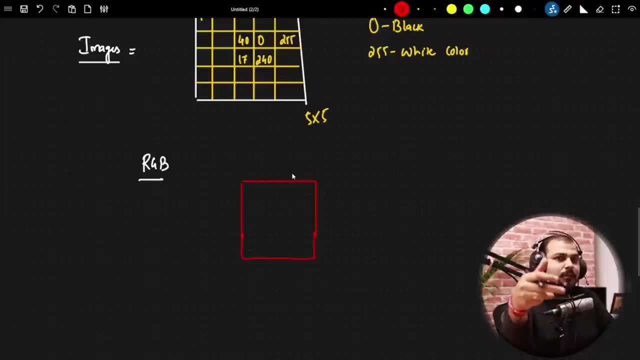 is basically the colored image. you know, whenever probably you click from your mobile phone or from some DSLR camera, you know you always get that specific image in the form of RGB format, because every color combination can be created with the help of this RGB image. that is red, green, blue, right? So suppose let's say this is a 4x4 pixel image. So suppose let's say this is a 4x4 pixel image. So suppose let's say this is a 4x4 pixel image. 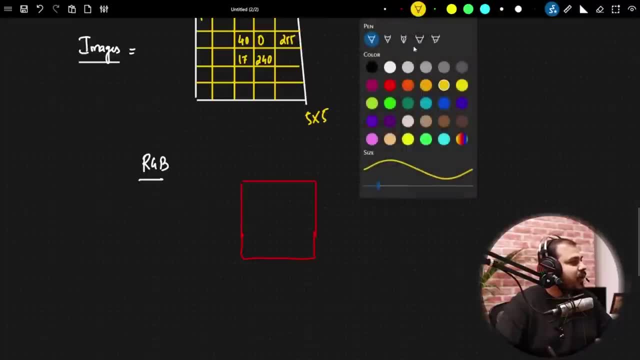 So suppose let's say this is my R channel and with respect to the other thing, I may also have a green channel. so suppose this is my green channel. So I may create something like this: this is my green channel. okay, This is my green channel, okay. 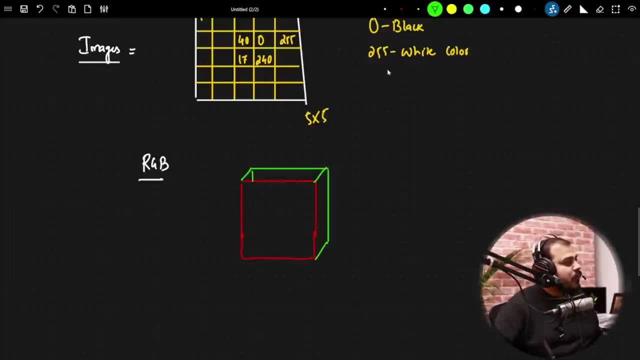 So this is my green channel, let's say okay, And on top of it you may also have another channel which is like a blue channel. So suppose I go and pick a blue color. let's see where is blue color. 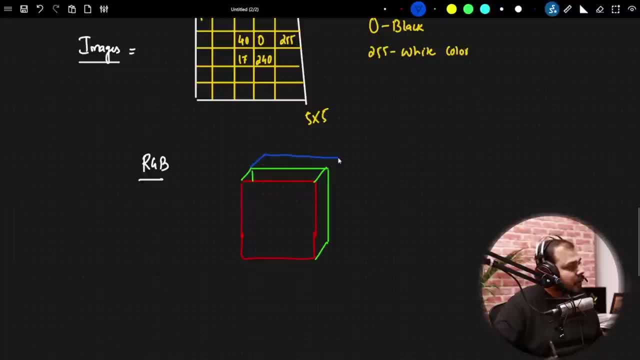 Somewhere like this, right? So this is my blue color, So this blue will be another channel, right? So whenever I have this kind of combination, then what will happen Over here? let's say this is 5x5,. let's say this is 5x5, 1,, 2,, 3,, 4,, 5, right. 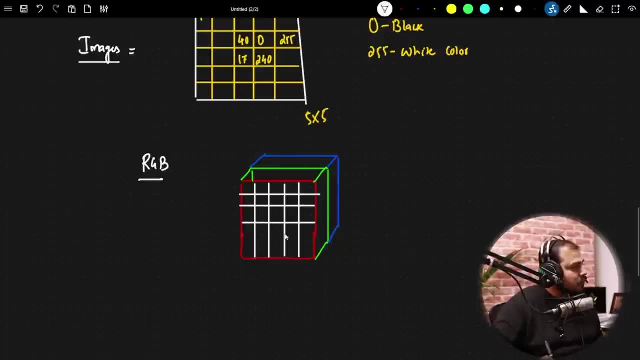 And similarly, I have 1,, 2,, 3, 4, 5, right. So whenever you have this 5x5 pixels, here also, it will be 5x5, right. So any image that you're going to take is that you're going to combine this RGB right. 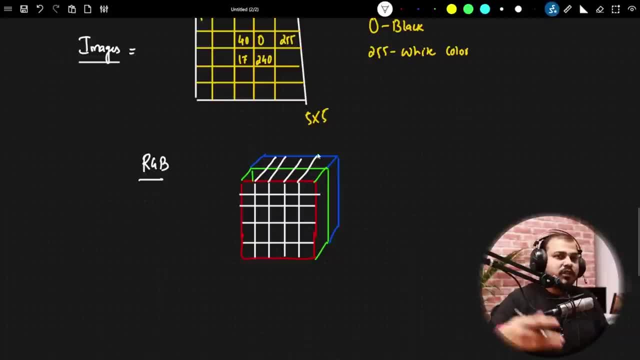 This will be R channel, that is, red channel, this will be a green channel, this will be a blue channel, And when it combines, it can basically come up with some kind of format. okay, And here also, your values will again be ranging between 0 to 255 with respect to each, and. 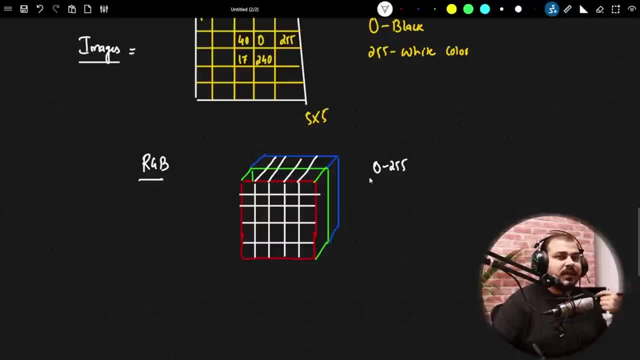 every channel And when you combine them, then the combination that you're actually going to get, you'll be getting it in different colors, okay, So this is with respect to RGB format And suppose, if I want to represent this in the form of pixel format, I will basically. 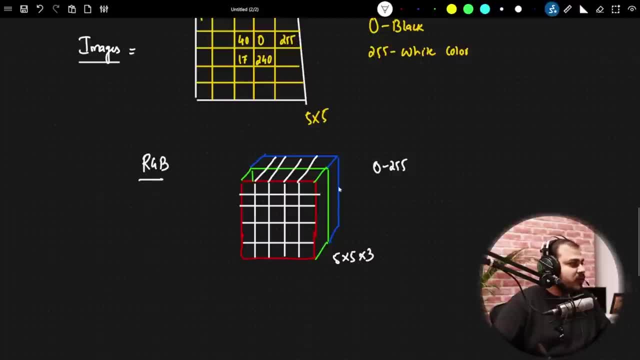 write 5x5 x 3 channel. okay, Because they are 3 channel. This is my R channel, this is my green channel and this is my blue channel, right? So red, green blue, Red green, green blue. 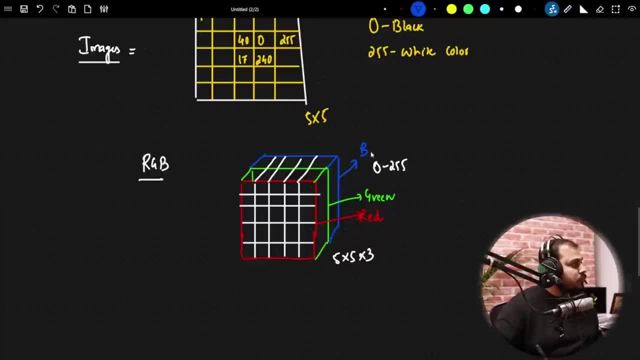 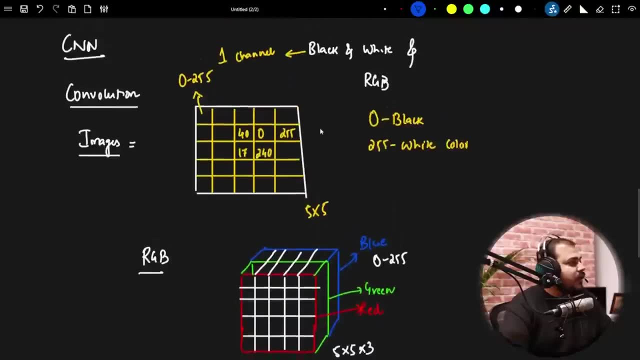 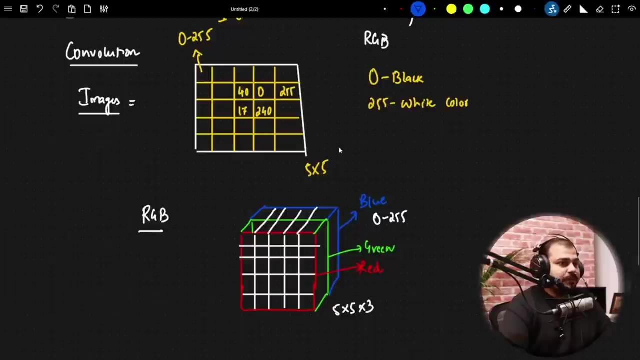 Green and blue channel. okay, So these are my red, green, blue channel, So I hope you got the difference in understanding the black and white image versus the RGB image, okay, So this is the basic information you really need to understand, okay. 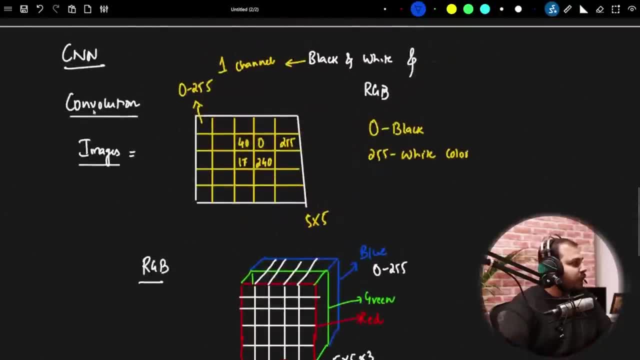 Now, if I go to the next step, let's talk about this convolution layer. So what exactly happens in a convolution layer? And later on I'll show you an example with respect to a single black and white image and also with respect to a RGB image. 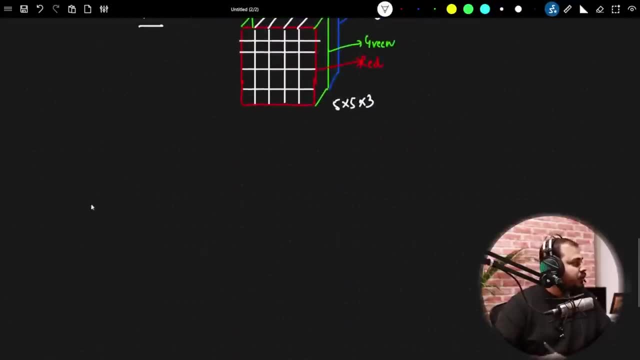 So if I go over here and probably take up this convolution operation Now, in convolution operation what happens is that- and this is the first step with respect to a convolution neural network, Let's say you have an image, and this is my specific image. 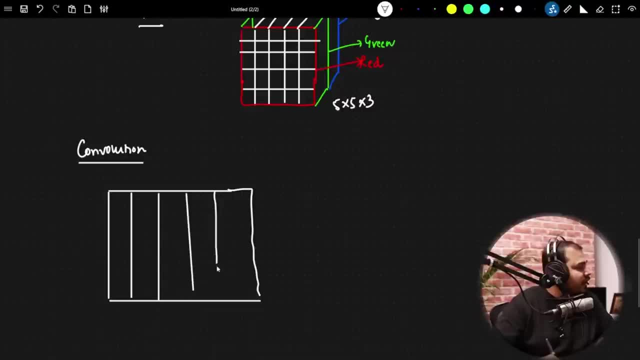 And here I have values, let's say how many number of channels I have. Okay, So let me just create this: 3,, 4, 5.. Okay, Okay, 1,, 2,, 3,, 4,, 5,, 6, right. 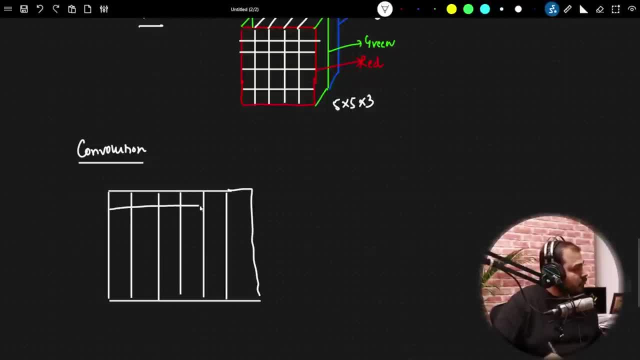 So here also, you have 1,, 2,, 3,, 4,, 5, 6, right? So this is my 6 x 6 image. okay, 6 x 6 image. Now, when this is basically a 6 x 6 image, what we are actually going to do is that we 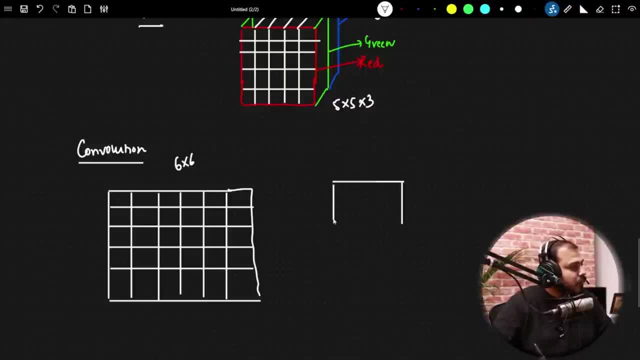 are going to pass it through a filter. okay, We are going to pass it through a filter And this filter will be 3 x 3.. Let's say 1,, 2,, 3, right, Let's say that this is my 3 x 3 filter. 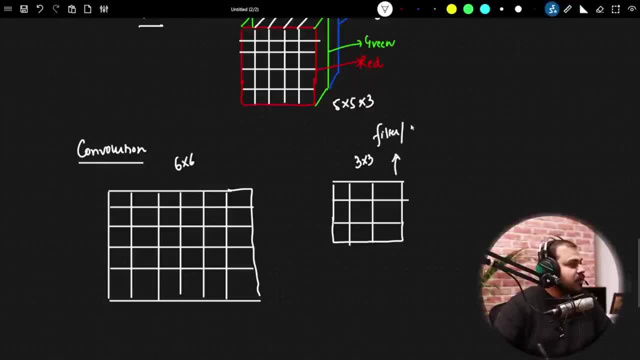 Here you can say this as filter also, or this as kernel also. Okay, This as filter, or this as kernel also, And finally you get some kind of output, And let's say that this is a 4 x 4 output. 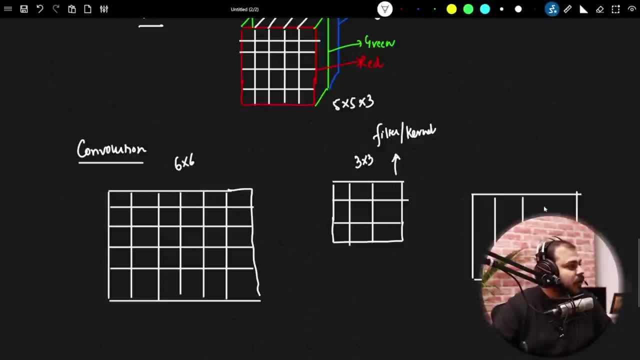 I'll tell you why we are getting a 4 x 4 output, Why you are getting a 6 x 6 output. Okay, Because we are getting a 6 x 6 output and all 2,, 3,, 4, okay. 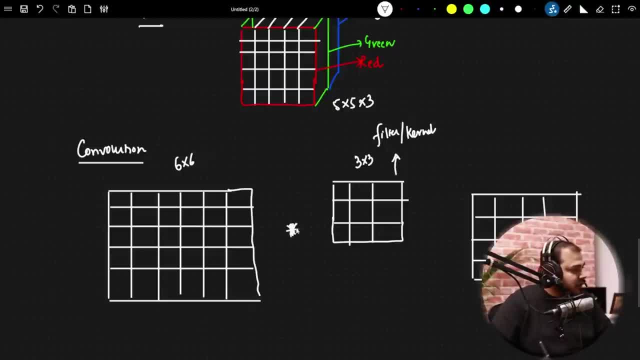 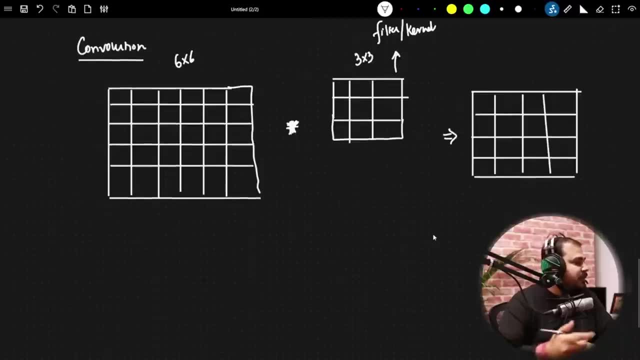 Now, whenever you do this convolution operation, convolution, let's say we are doing this kind of symbol, we are getting and we are getting this specific as an output. okay, Now let's say this is my 6 x 6 image and let me put some values. 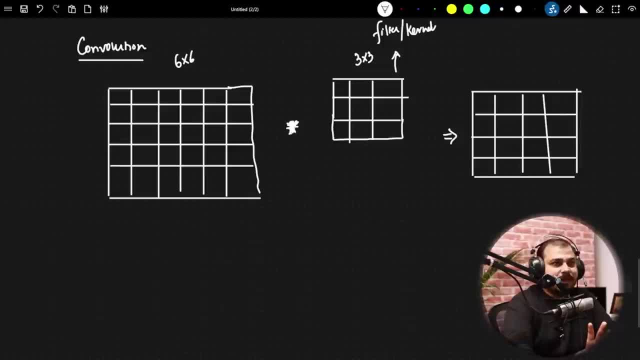 You know that whenever we try to put some values with respect to the image pixels, you know that it will be ranging between 0 to 255,. right Now, in convolution, what we do is that if I really want to convert this into 0 to let's. 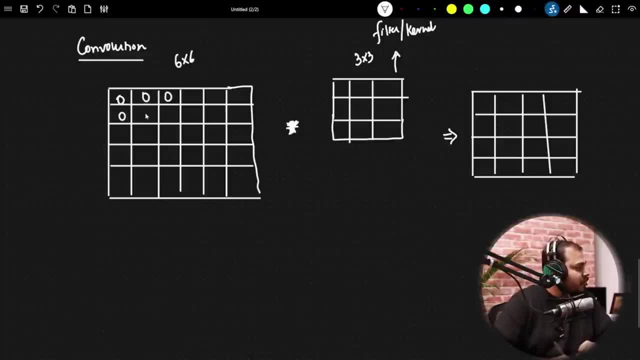 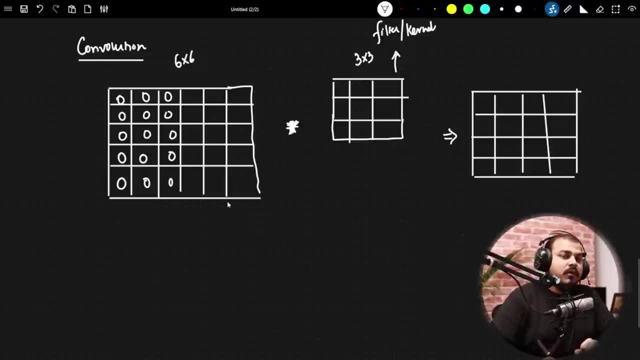 So these are my values. Let's say, and these all are 255,. okay, Always remember, the first step that we do in a convolution is that we try to bring this all values between 0 to 1,. okay, If I am trying to bring these values between 0 to 1,, then what will happen? 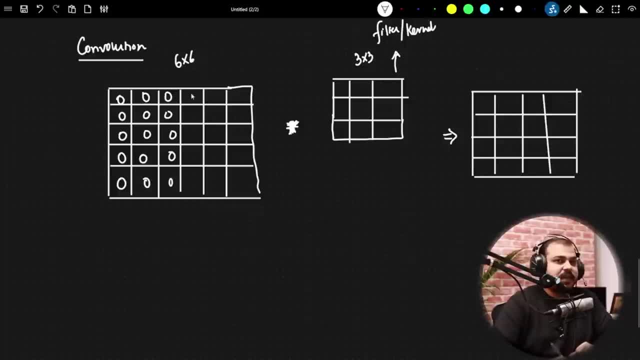 I will divide each number by 255. So over here, if 255 is there, I will make sure that this all will get converted to 1.. This we basically say it as min max scaling. okay, Min max scaling. So this process is actually called as min max scaling, okay. 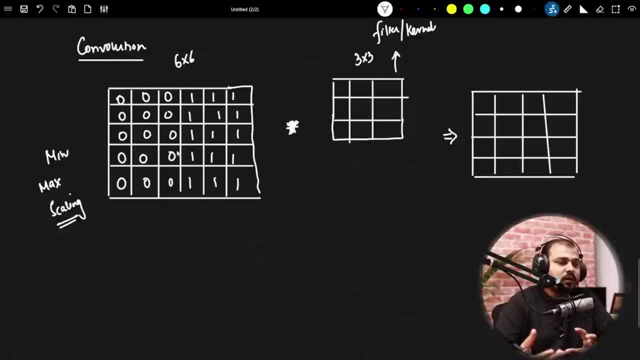 Min max scaling. Now, in min max scaling, what we are doing is that we are just trying to convert all the values of the pixels between 0 to 1, okay, Super important, and this is the step that we are also going to see. 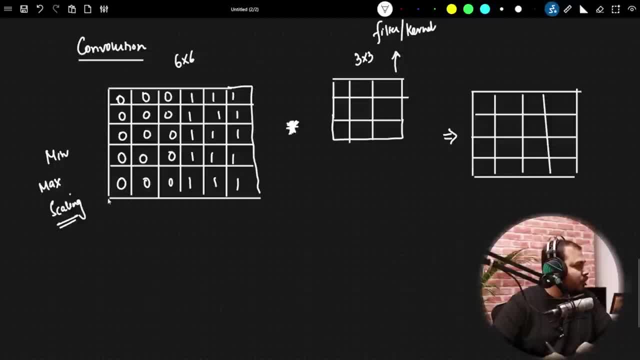 Okay, So here you can see: 1,, 2,, 3,, 4,, 5,. okay, One more value. I will just one more row. I will just try to put it over here, So this will be my lines, okay. 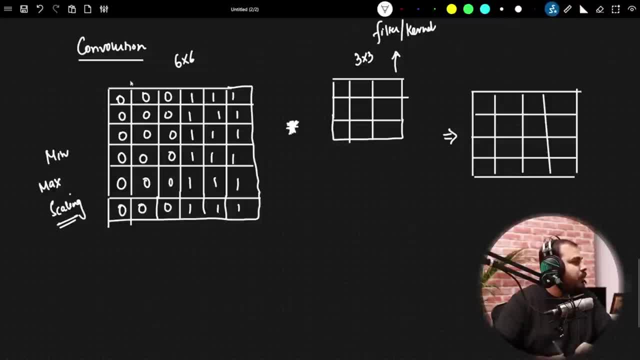 0, 0,, 0,, 1,, 1, so 1,, 2,, 3,, 4,, 5,, 6,. okay, And so you have actually got this much idea that what I have done is that my first step. 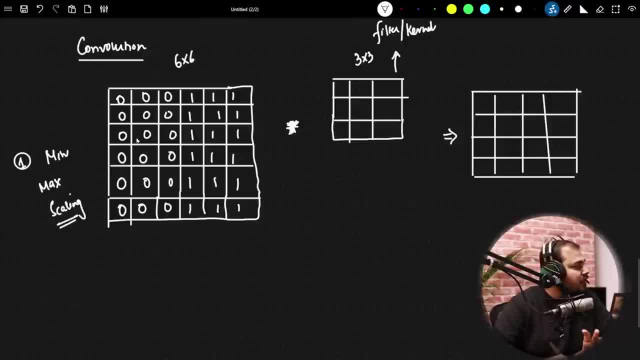 I've done a min max scaling, so whatever pixels are there, I'm going to basically convert this into 0 to 1,. okay, Let's say that I have a specific filter over here and this filter what I'm actually going to put the values like is that I will just write 1, 2, 1, I'll talk about it why I'm 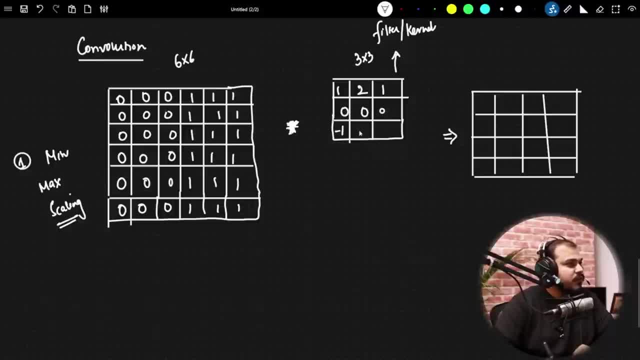 putting this specific filter like this: 0, 0, 0, minus 1, minus 2, minus 1.. Let's say that I put this specific filter. This filter is actually called as something called as horizontal edge detector or horizontal. 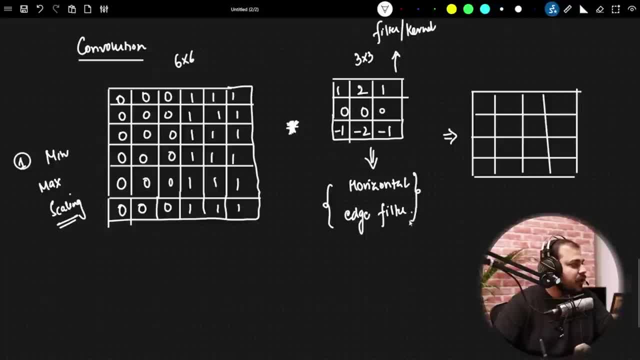 edge filter. Let's say I'm just saying this as horizontal edge filter. Now I hope you have got an idea with respect to this. So what I have done is that I've given 6 cross 6 image. I've passed it through a convolution. 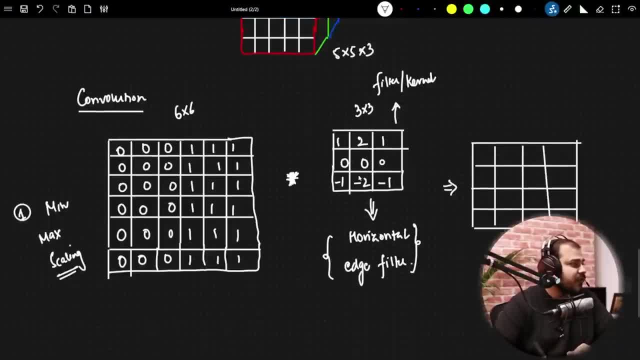 filter. Sorry, I've passed it through a filter which is 3 cross 3 with these values, which I specifically say this as my horizontal edge filter And finally the output that I'm actually getting. I'm getting it over here and this is actually. 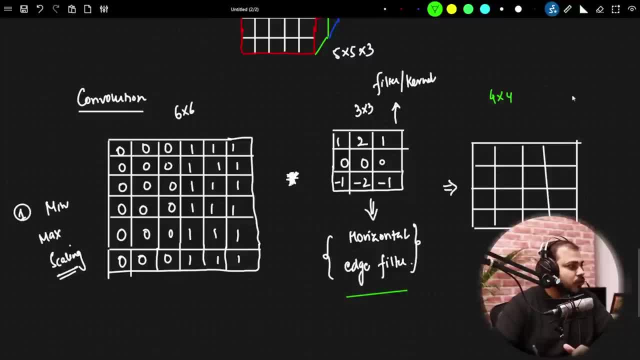 4 cross 4, okay, And this is specifically my output, okay. Okay, And what kind of output we will get, that I'll try to discuss. okay, Now let's try to understand how this convolution operation happens. Convolution operation: what it says is that I will take this filter and I will just place. 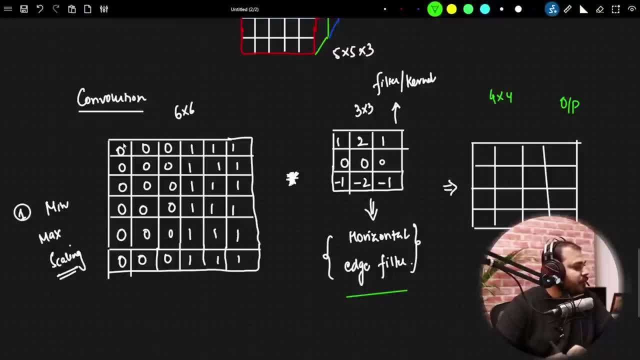 it in top of top of this specific image from left. from the starting, Let's say that I've taken this filter and I'm placing it over here, So I'm placing it like this. I'm placing it like this on top of it. 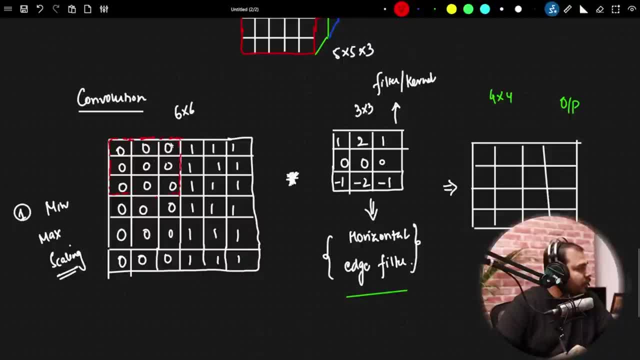 I'm placing it over here, in top of it. Now, when I place it over here, when I place it over here, what will happen? What will happen? The first operation that I'm actually going to do- I will take this value and, wherever, 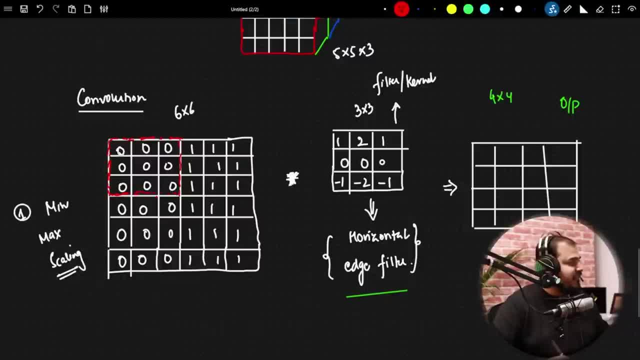 it is placed to that same same row or same cell. right, Suppose, this cell is there and I've actually put this 3 cross 3 filter over here. So over here this value and this value will get multiplied. So if it gets multiplied it is like 1 multiplied by 2.. 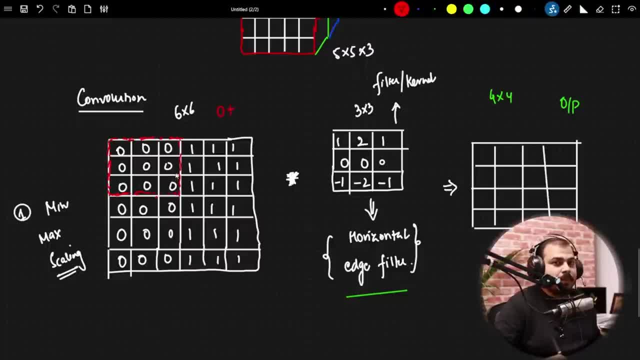 Okay, This is multiplied by 0. So I'm going to get 0.. Okay, Then I'm going to add the next value, So this value will get multiplied with this, So this will also become 0. And similarly, 1 will also become 0. 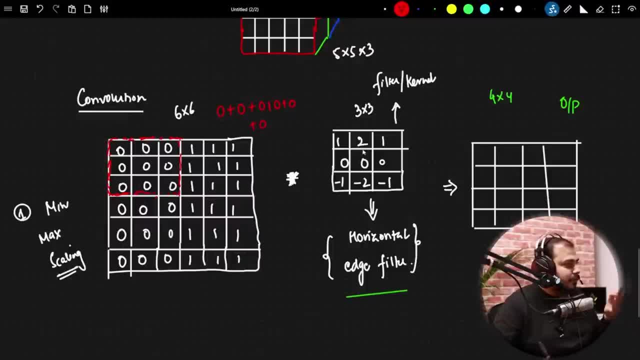 And, like this, all the values will become 0 in the first instance when I'm placing this specific filter, And whenever we add up this value, whatever is the final output, we will place it over here. Okay, So this is the first operation. 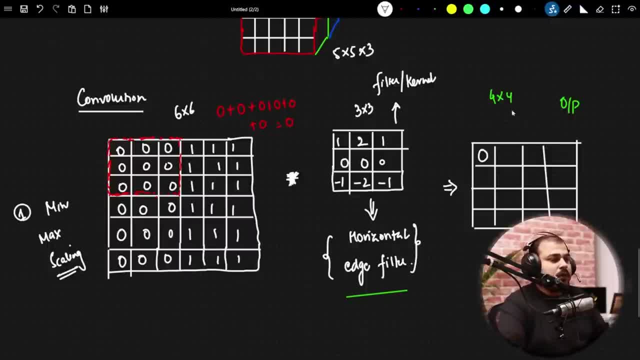 So I hope you are getting a clear idea about it. Okay, So what we are doing over here? we just place this convolution filter, this filter or kernel, on top of it, We are multiplying each cell with that cell and then we are adding up all the values. 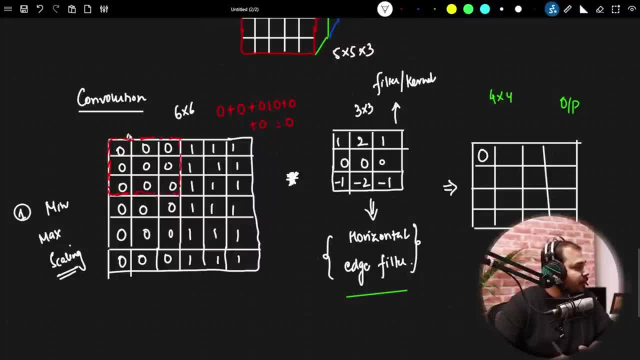 Right Now, after this, what we do is that we move one step to the right. We move one step to the right. Whenever we move one step to the right, there is a variable which is called a stride. We specify the stride variable as 1.. 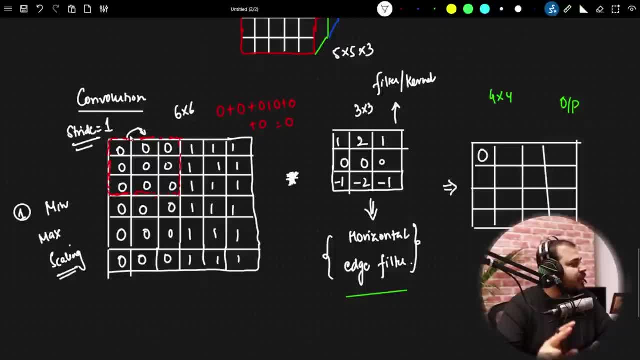 If you are jumping two steps to the right, then we will basically make stride is equal to 2.. So here we are jumping, just one position to the right. So one position to the right, the stride will be 1.. Now what will happen? 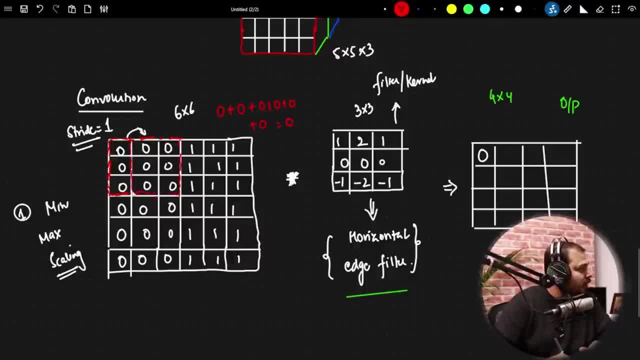 My filter. this filter will start moving from here to here Right Now. when it moves from here to here, then what will happen? Again, do the calculation. My calculation will start 1 multiplied by, let's say, my calculation will start for the. 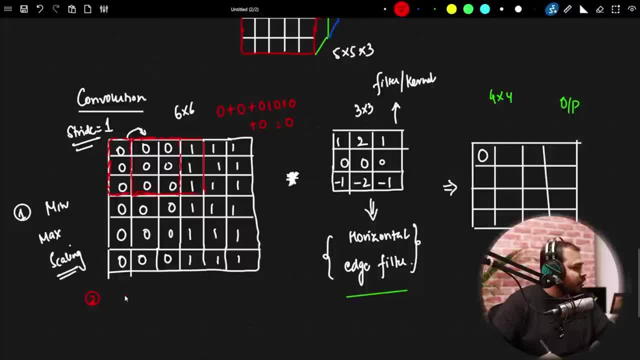 second instance: Okay, 1 multiplied by 0.. So it will be 0.. Plus 2 multiplied by 0.. It will be 0.. 1 multiplied by 1.. So it will be 1.. Plus 0 multiplied by 0.. 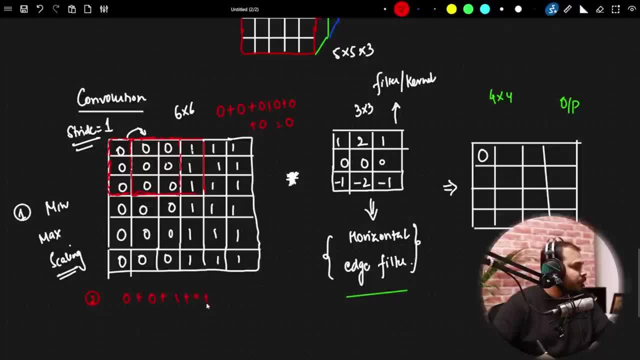 It will be 0. Then again 0, 0. Then over here. if we go over here, it will be minus 1, minus 2. This both will get multiplied and to this also it will be 0, 0.. 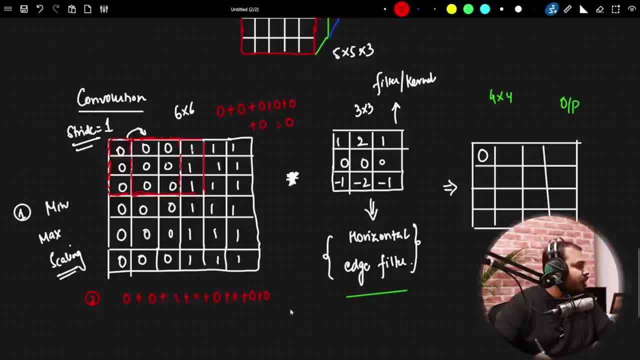 And finally, I will have minus 1 multiplied by 1. It will be minus 1.. Right, So here also what I will be getting. My total value will actually be 0.. Okay, So I hope you are getting an idea about it. 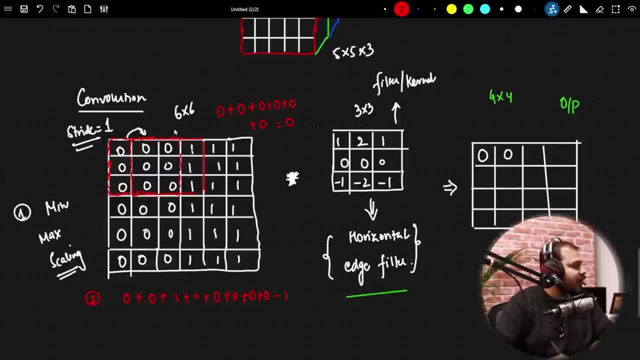 Then what we will do. We will again jump one step to the right after this, because I have to go and take the next pixel of the information over here. and here we go with respect to this. Now, when I jump one step to the right, then what will happen over here? 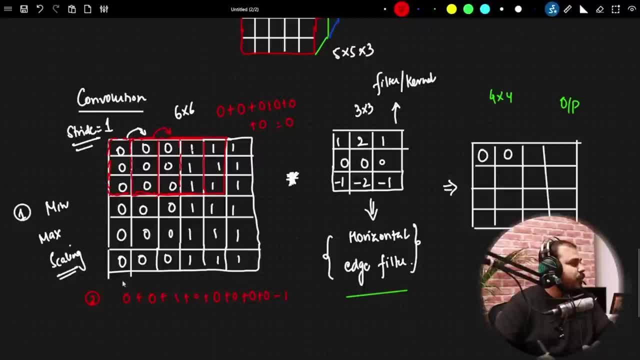 Like I will be jumping at this position to this position and again the same operation will happen. The third operation: again, if you try to see, everything should be equal to 0, most probably because, see, if I multiply this so 0, then this will be 2, then this will be 1, then all. 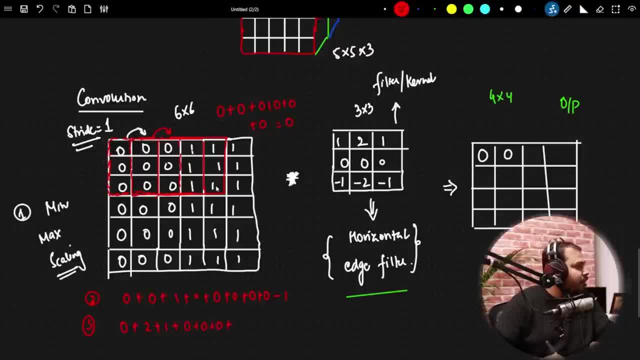 will be 0 over here, and then over here you have minus 2 and minus 1.. So if I try to calculate it, it will be minus 2 and minus 1.. So this will entirely become 0. So the next operation will also become 0 and finally, when you continue, you will be getting. 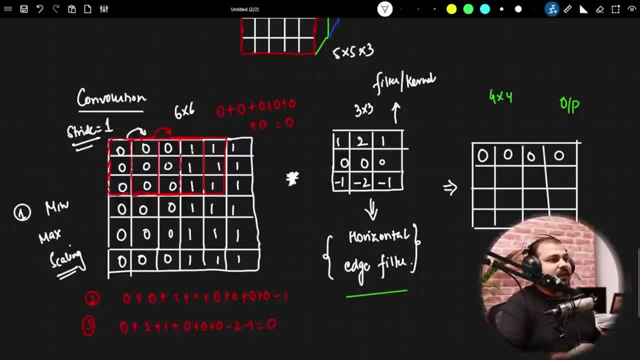 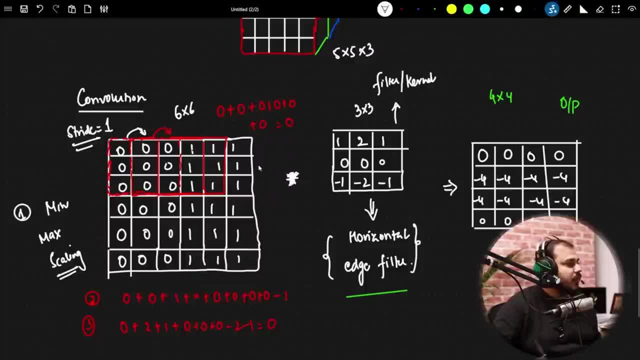 4. You can do the calculation, guys, and this will be 0, 0.. That basically means, after we finally go to the next step, then my next stride will move towards this position and again it will do the calculation, again I will get jump, it will become 0 over here. and after this, what we do? we go one step. 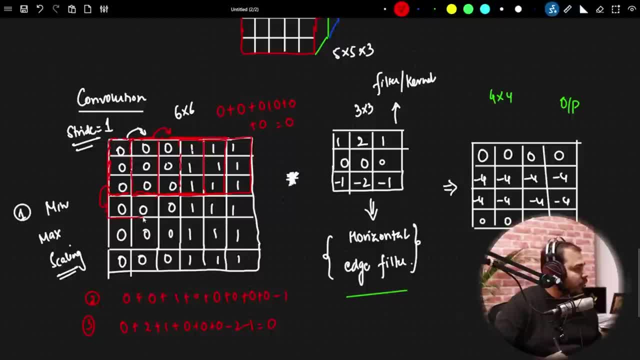 towards downwards. So from here to here will be my next step, and we will continue this particular step, This particular step from here, and then we will do the calculation Here. you will be able to see that I will be able to get minus 4 for the same thing. 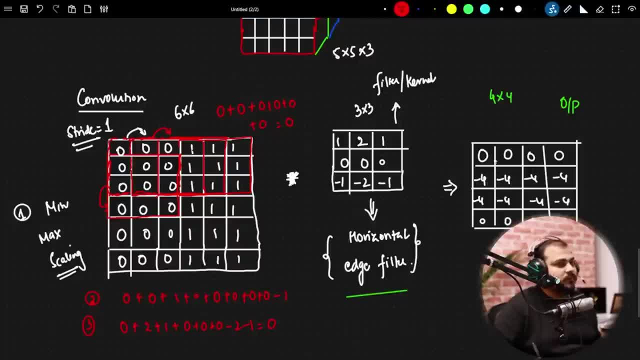 So I hope you are getting an idea about it and you are able to understand some kind of calculation that we have actually done over here. So this is very much clear till here, I guess, and you are able to understand things And definitely you can do this entire calculation and you can try to find out. 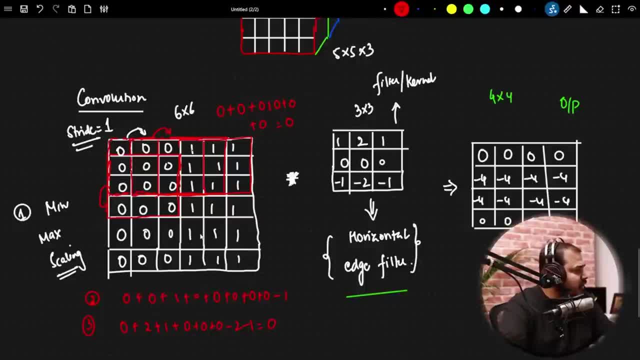 So if you move one step towards down, Then again one more step. if you move towards down and if you do the calculation, you will be getting some values like this. Let's say that I have got the output, which looks like this. So I hope everybody is clear with respect to this specific output and you are able to 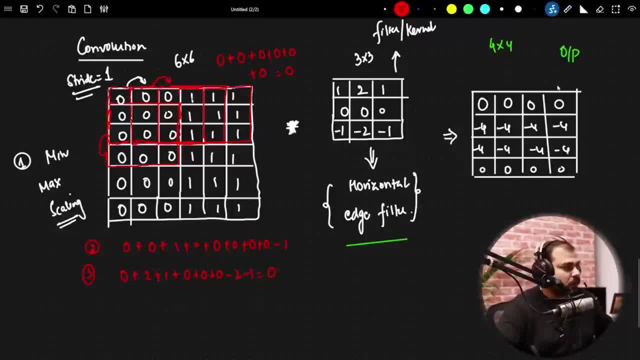 understand it. Let's say that I have got this specific output Now. this operation is specifically called as convolution. This operation is specifically called as convolution Now, whenever we are giving Okay, Filter can be one more thing. guys, filter, we will talk about it, right? 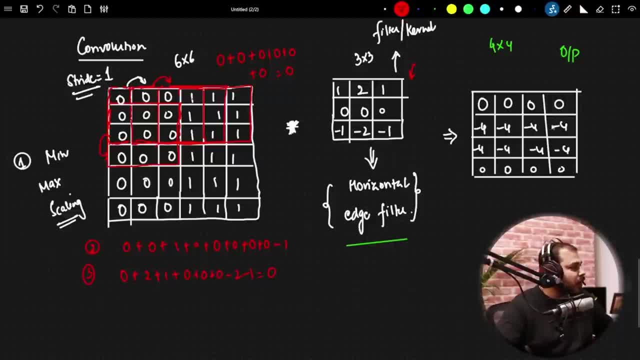 I have just initialized a horizontal edge filter. Okay, Now let's say that when we got this specific output- one thing that you see over here, I am just going to rub this now. One thing you see over here- when I pass a 6 cross 6 filter, 2 or 3 cross 3 filter, I 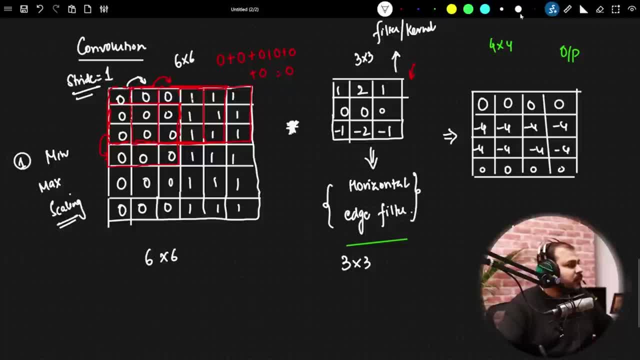 am getting a 4 cross, 4 filter. Okay, Yes, guys, I think this will also be 0.. Okay, Let's say this also: I am getting it as 0.. Let's say that I am getting these values, as if I do this operation, then automatically. 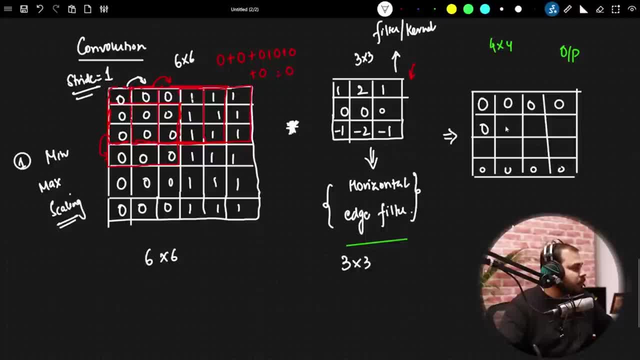 this will become 0.. This will also become 0.. This will also become 0.. See, do the calculation. Whatever value you get, Okay, Let's consider, I am just saying that. Okay, Let's say here that I am getting these values. 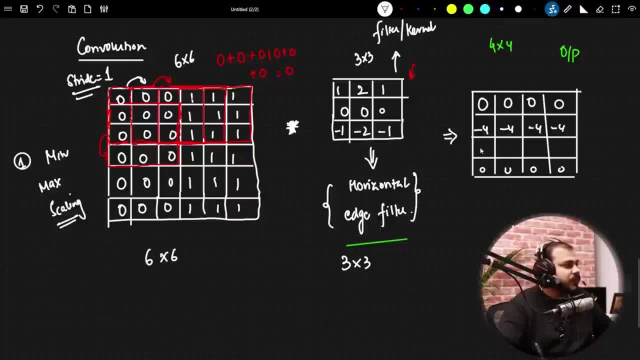 Let's just imagine: Okay, I am getting these values. Okay, I am getting these values by passing through this. Let's just consider: Okay, I know this value will become 0 or it can be anything else. You know, I am just saying that. 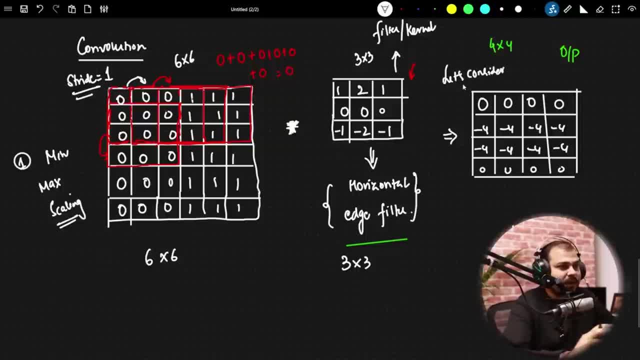 Let's consider Okay, Because I want to give you a very important point by putting this: Okay, How we will be getting minus 4 or whatever values you may be getting. Okay, Or do one thing If you don't want to go ahead with this. 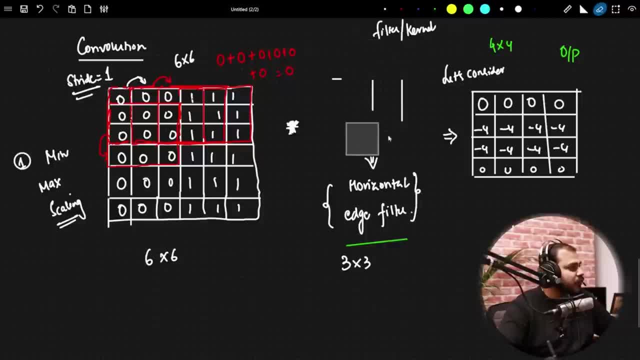 You know, Change the filter. Okay, What I will do is that I will try to make a new filter over here. Okay, Let's say that I have got this new filter. Okay, And let's say this is my 3x3 matrix. 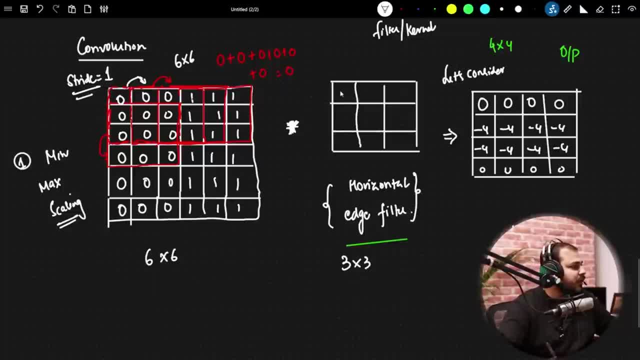 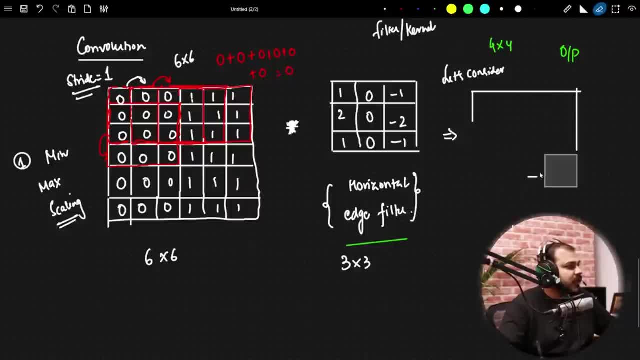 Minus 1.. Minus, 1.. Okay, So let's say, I have this specific filter And let's start the operation from again. Okay, Let's say: And this filter is basically called as vertical edge detector, Let me just drop it. 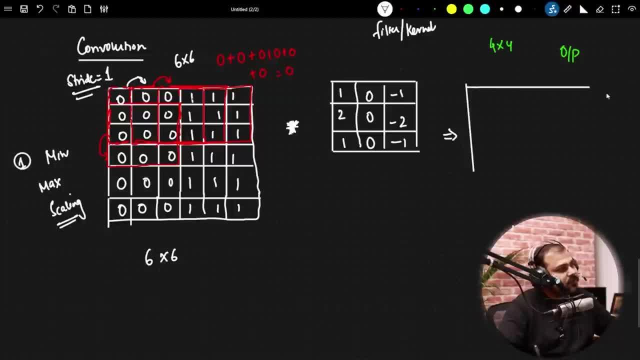 Okay, Now let me pass this filter. Now, when I pass this specific filter, And I will be getting a 4x4 output. okay, one, two, three, four. okay, now do the calculation. everyone. what will happen? first time, everything will become zero, right. second time. uh, if i go one step to the right, 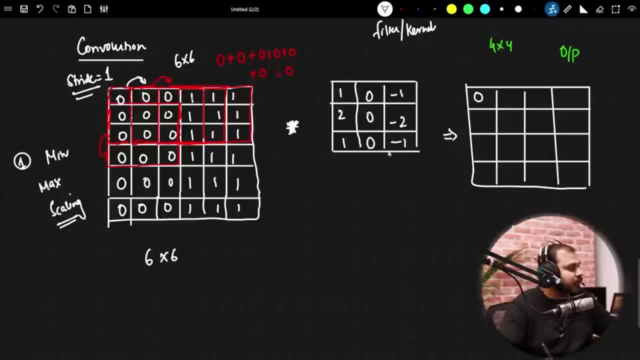 then it will become minus four minus one, minus two minus one. when i add this up, it will become minus four. then again, when we go to the one step to the right, okay, then then again i'll be getting minus four, and then this will become zero. and similarly, this will happen for every row. just do: 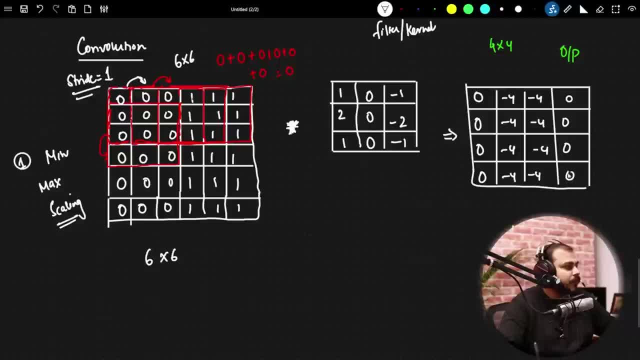 the calculation and let me know whether you are able to get it or not. okay, so this kind of values we are actually getting. okay, very simple. when i place from here, i go one step towards the right. similarly, i go one step towards the right and i do the convolution operation, you will be able to. 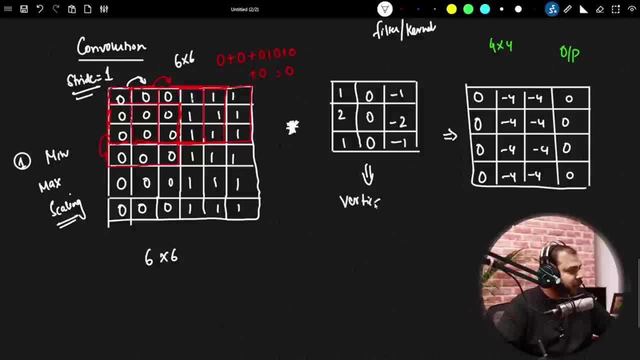 get this. okay, so this is basically called as vertical edge filter, edge filter or curve. okay, so this is my vertical edge filter occur. okay, so i hope everybody is able to get this. okay, how to choose the filter values and all. i'll just explain. let's say that there is this specific: 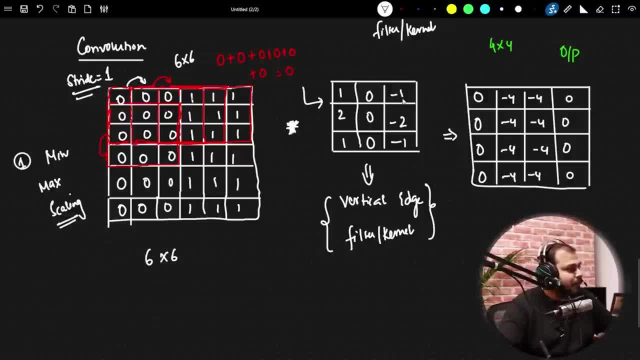 filter which is already defined, and whenever i pass this filter to this, i'm going to get vertical edges some or the other way. now one very important thing with respect to the output. you know that if i again re-change these values because you know that we had done feature scaling over here- right, if i do, 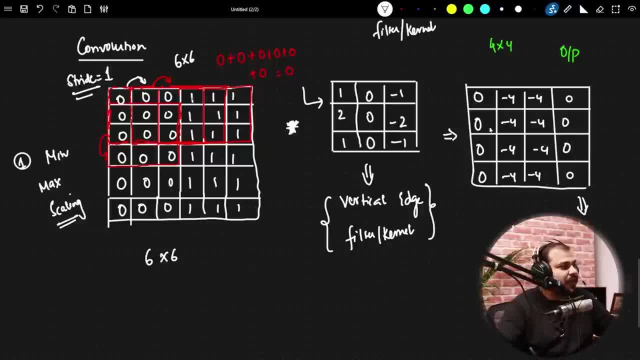 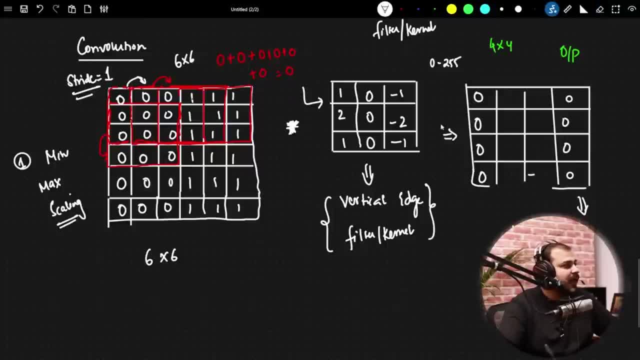 four will actually become. okay, will actually become 255. i hope everybody is able to get this. everybody agrees that. right, this will become 255. sorry, this will become zero. right, this will become zero. why? because this was minus four. the lowest value will get converted to zero and the highest 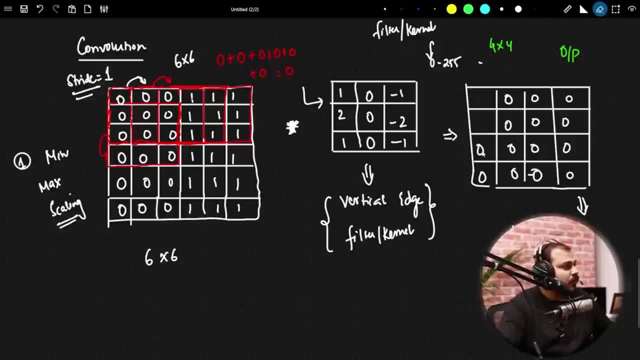 value will get converted to 255. i hope everybody remembers this. how we do it: feature scaling- right, so this will entirely become. this will entirely become 255. okay, so if i do back the feature scaling, this all will become zero and this will become 255, because 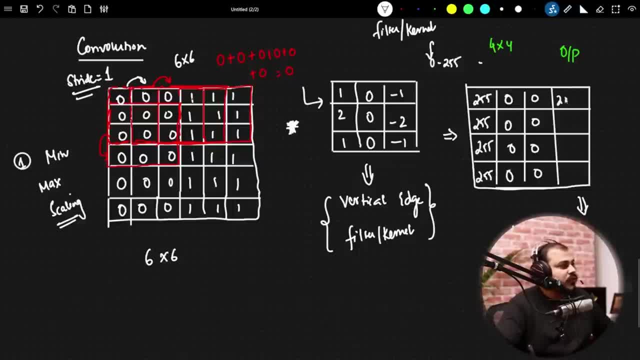 the highest value was zero and the lowest value was minus four. so if we bring back the min max scalar, if we apply the min max scalar again, what is going to happen? the smaller value will become zero and the larger value will become 255. now, 255 is nothing, but it is a white color. 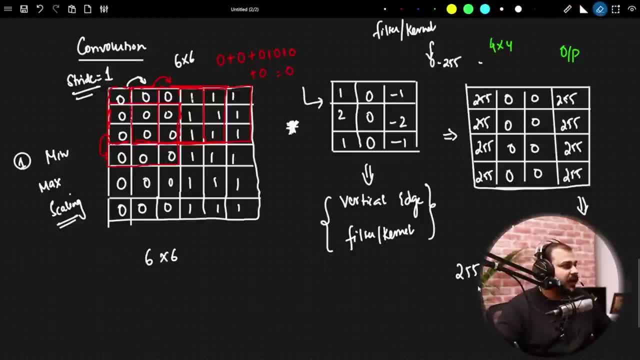 255 is nothing, but it is a white color, right? so i hope everybody knows about it. so 255 is nothing but white color, right, and zero is nothing but black color. now, when i have this, that basically means this entire thing is black color, right, zero, and 255 is white color. so how do i get this? 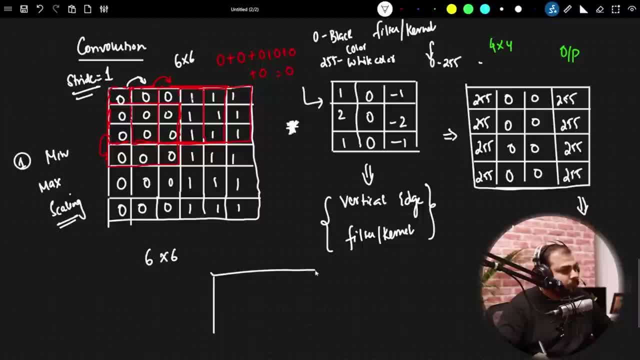 if i probably try to draw this in the form of a diagram, right? it will look something like this: so this will be my white color and this remaining all will be my black color. so this will be my white color and this will all be my black color, right? so this? 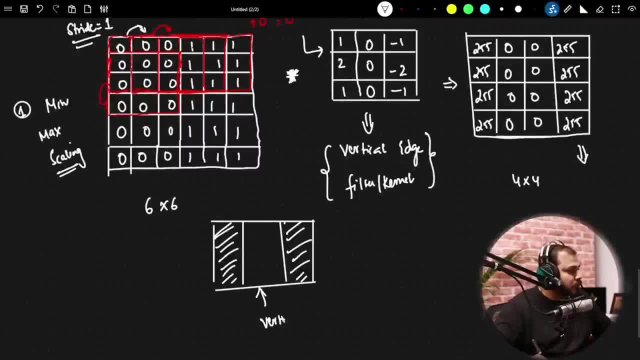 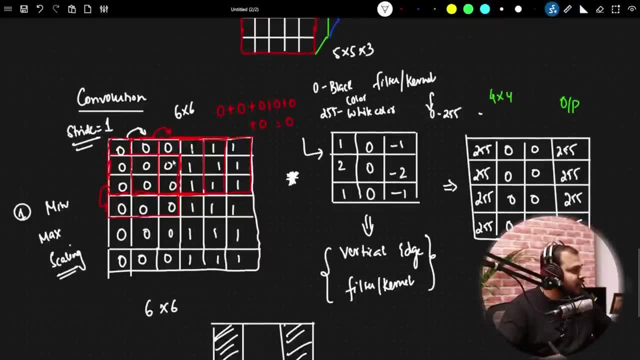 is nothing. but this is my vertical edge, vertical edge. so in this specific image, so in this specific image, you know that zeros and ones are there. obviously i should be getting a vertical, i should be getting a vertical edge. in between that and after passing this filter, i am able to get a. 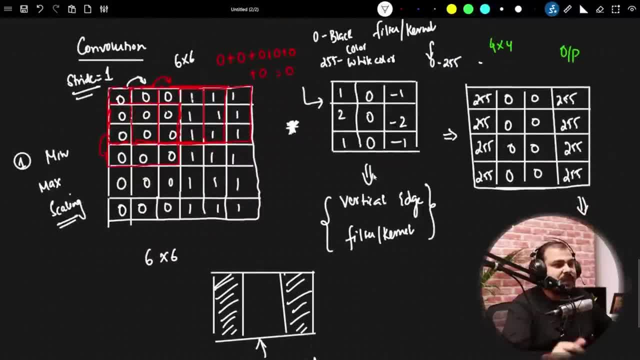 vertical edge that you can see from here, right from this specific example, and this filter is responsible for doing that. it is responsible for getting the vertical edges right. so from here you can see, as soon as i pass this filter, i am able to get the vertical edges. so what does this basically? 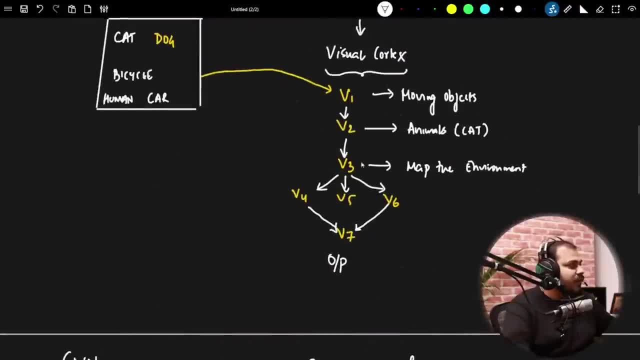 mean here. i discussed about my various layers right: v1, v2, v3, v4, v5, v6, v7. similarly, we have created a layer over here and we have created a layer over here and we have created a layer over here which is able to extract some information now in this particular case, with the help of this. 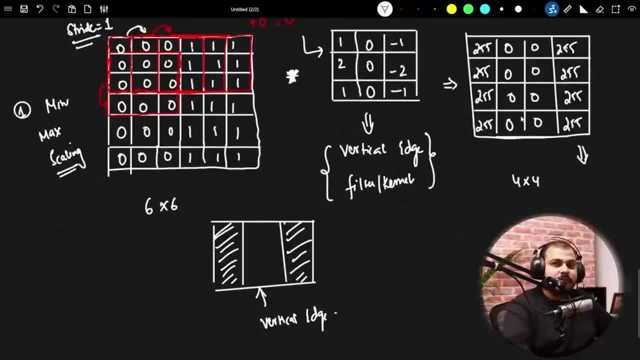 filter i am able to extract where are my vertical edges right. so this process is basically called as a convolution operation. similarly, i may have various different kind of filters. i may have a horizontal filter, i may have a. i may have another filter like this with, and this filter will be also. 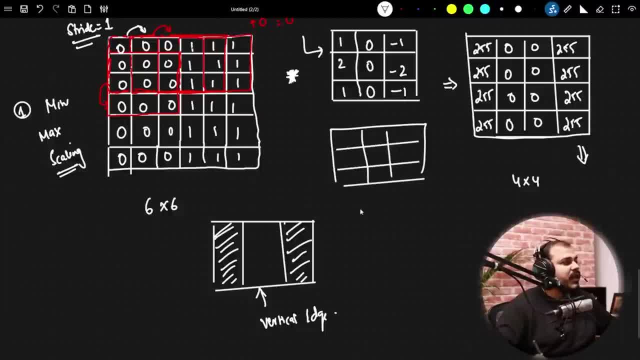 three cross three, let's say, and this will be able to determine my horizontal edge. there will be one more filter, let's say, which will be able to determine my round objects, let's say: okay, so i may have multiple kind of filters over here. you know this. filters is basically like what? 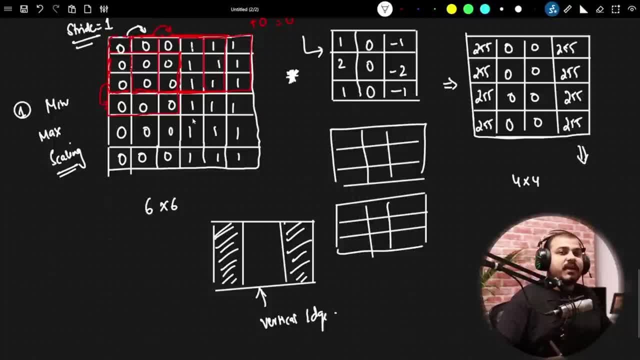 what we are doing. it's just like this information. we are trying to extract it from the image with the help of this filters. we are just trying to extract the information of this specific image, right. so i hope you are able to understand till here, right now, in a specific image, whenever we are. 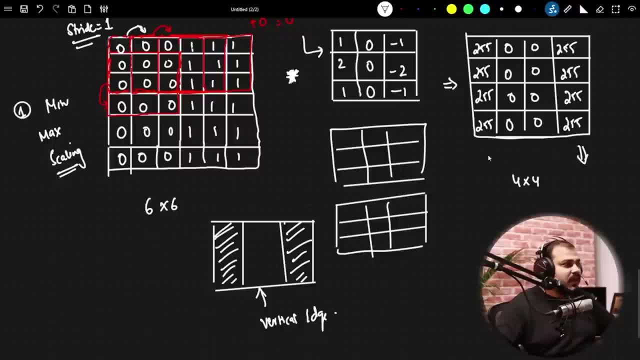 forming, convolution, neural network. we can have multiple filters like this and we will also be getting multiple outputs like this. okay. so like this, multiple outputs we will be getting. okay, like how we got over here: for horizontal filter, we may get a different output. we. for round shape filter, we may get a different outputs from a specific image. 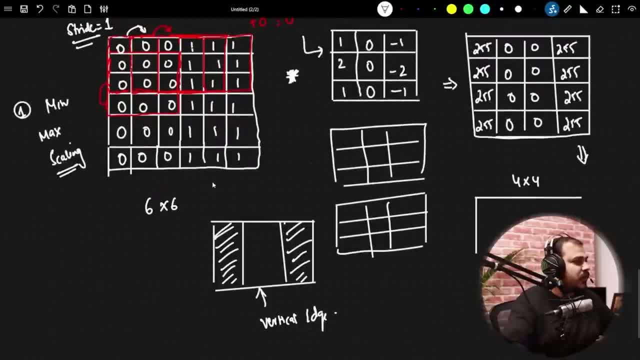 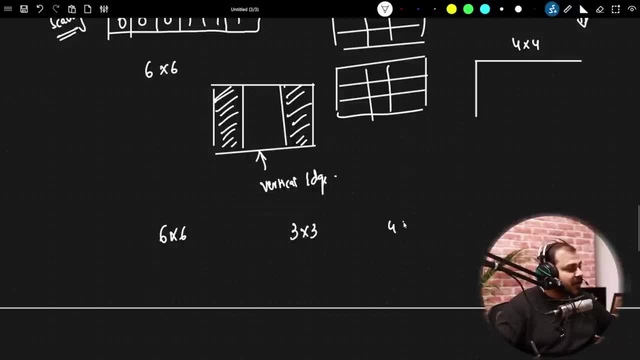 okay, now you need to understand some very important things. whenever i pass a 6 cross 6 image in a 3 cross 3 filter, i'm getting a output as 4 cross 4, right. whenever i take a 6 cross 6 image, i pass it through a 3 cross 3 filter. 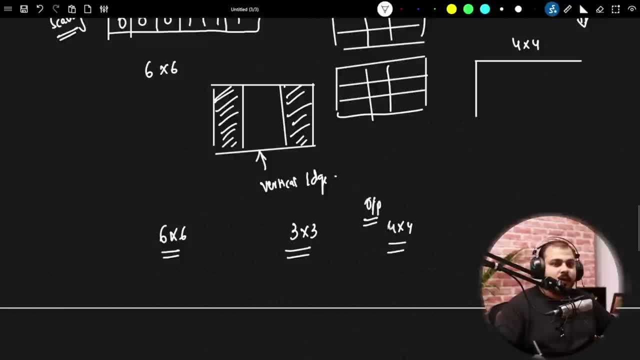 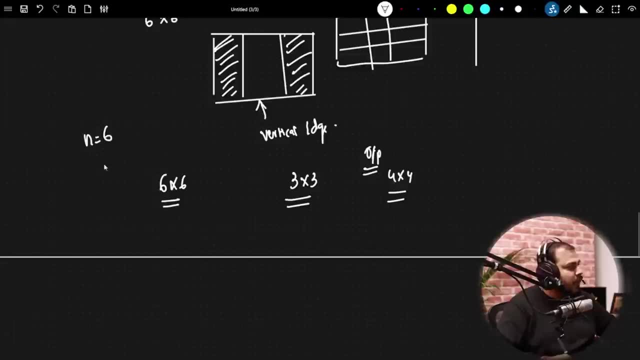 i get an output as 4 cross 4, right? how this is basically happening, right? so over here. let's say the size of the image is given by n, so n is equal to 6. okay, n is equal to 6. let's say the filter is nothing but 3, right? so if my n size is 6 and filter is 3, 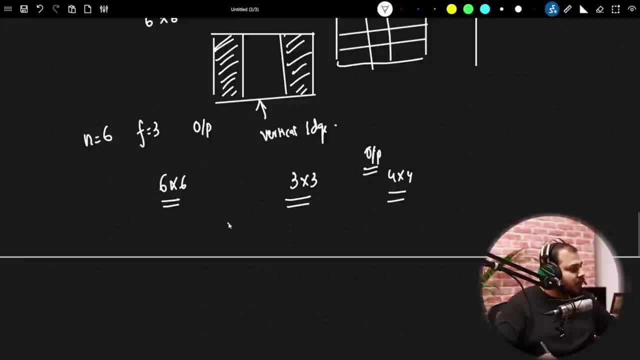 what will be my output image. so here you can use a mathematical formula. the mathematical formula will be n minus f plus 1.. so when you use this n minus f plus 1, it is nothing but 6 minus 3 plus 1, which is nothing but 6 minus 4, which is nothing but sorry. 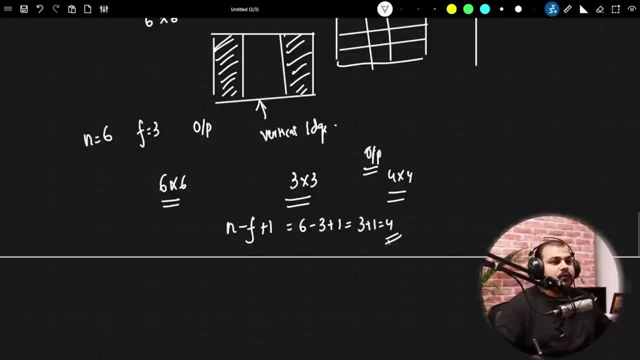 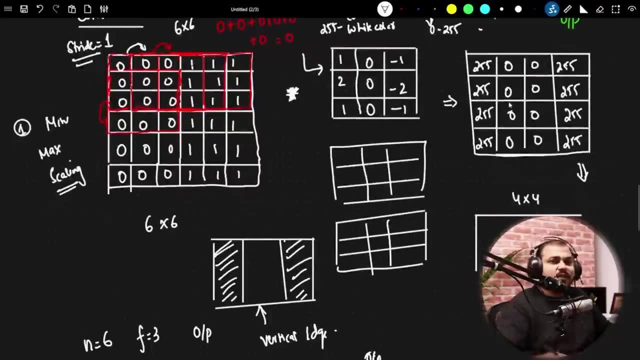 which is nothing but 3 plus 1, which is nothing but 4.. so finally, you are getting a 4 cross 4 output. okay, you may be having a confusion, krish. how do we define these filters? you don't have to define it, guys. i'll talk about it just in some time here. you don't have to even do any kind of hard coding, or 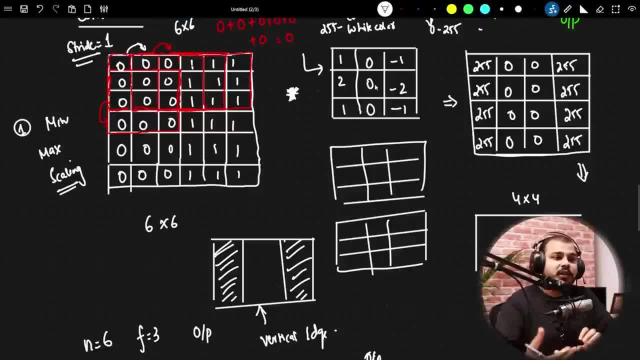 you- and here i'm just giving an example- what filters can actually do. filters can actually take out the information from the specific image. okay, how do we define this filter? i'll just say you in some time. okay, but here you understand that you have applied this formula and i have. 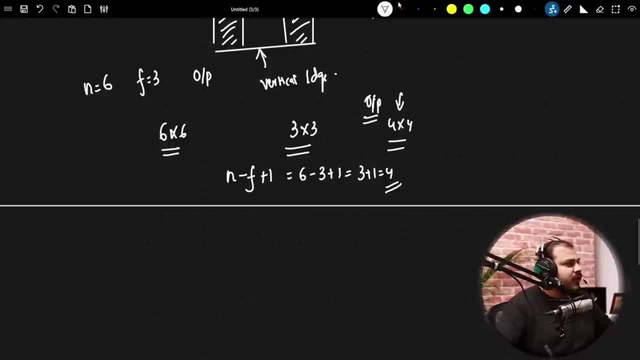 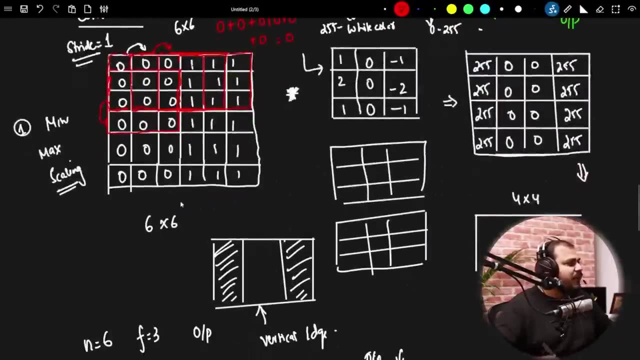 got three plus one is equal to four and that that is what my output is. right. that is what my output is right now. a very important question: what is happening? see, if i give a 6 cross 6 image to a convolution operation, i'm getting a 4 cross over value output. 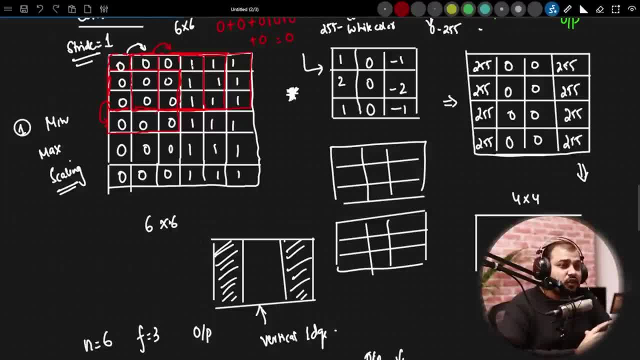 here. my image size is decreasing, and this should not happen. if my image size decreases, that basically means we are losing some kind of information. now, in order to prevent this loss, what we can actually do, we can come up with something called as padding. what we want to do is we want to do is that by происходит- some kind of on the edge of this- 3- create three Fur teaches- we can take a feed from osります without losing order, and that's exactly what we are creasing. see, if the size decreases, that basically means we are losing some kind of information. now, in order to prevent this loss, what we can actually do, we can come up with something called a padding. now, what's this process like? okay, you can solve this. 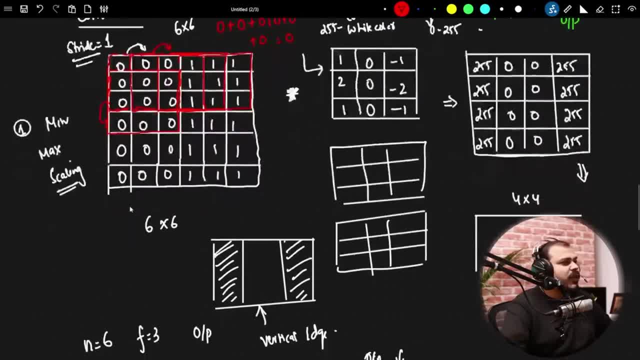 what exactly is padding? Padding says that do not do anything. If my image size is 6x6, I want to get the same output over here like 6x6. All you have to do is that apply padding on top of it. 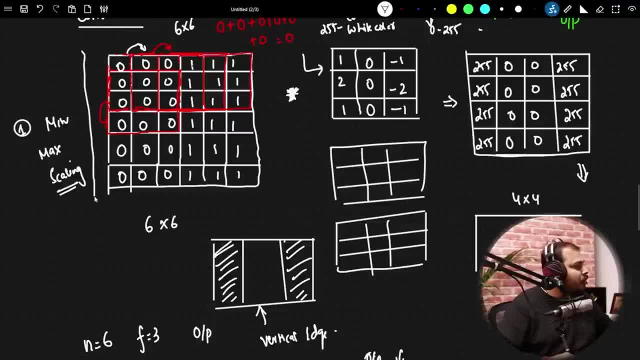 So how do I apply padding? Padding is just like building a compound, building a compound around the images. Let's say, I'm building one more additional compound on this specific image, on this specific image, on this specific image, like this: Now, when I build this compound, 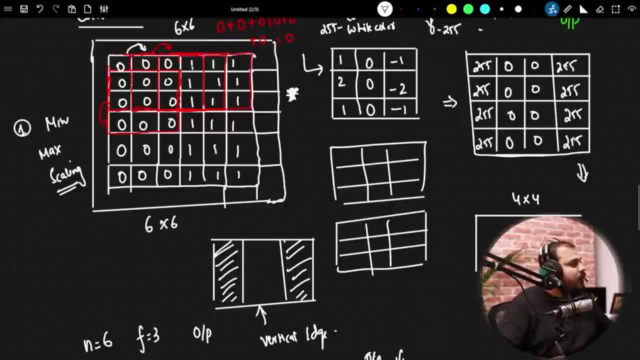 when I build this specific compound, then what will happen When I build this specific compound? what will happen? So if I build this compound here, you'll be able to see that I'm actually getting a 8x8 image. My image size is 6x6 only. 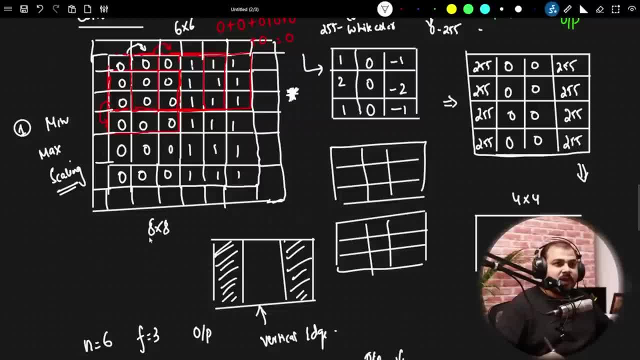 But now it becomes an 8x8 image. Now it becomes an 8x8 image, But my image size is anyhow 6x6.. But since I'm applying padding, this concept of applying a layer on top of the image is called as padding. Padding basically means that I am protecting the image by adding another. 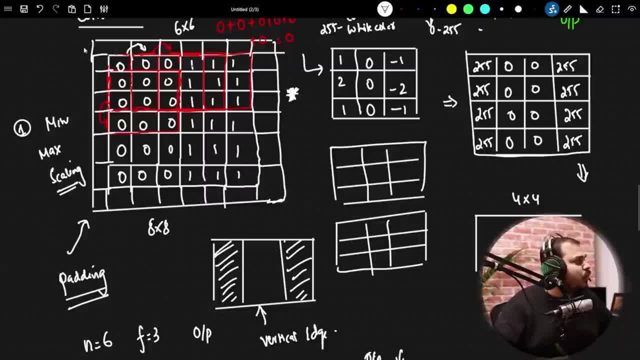 layer on top of it. Now you may be thinking what values can come inside this specific cell. This is a question that many people don't know, So I'm going to show you how to do that. So I'm going to show you how to do that. So I'm going to show you how to do that. 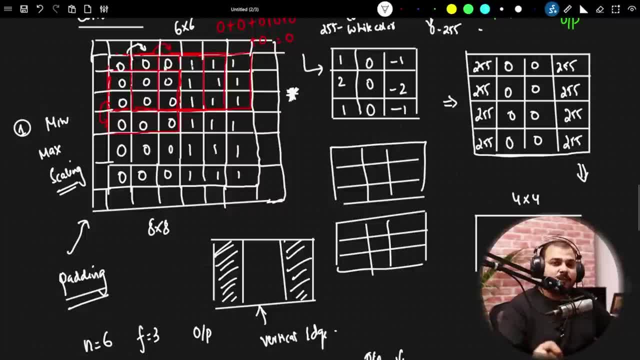 This is a question that many people may have. For this, you can have different kind of paddings. One kind of padding is that zero padding- Just go ahead and fill this cell by zeros. Just go ahead and fill this cell by zeros. The other kind of padding is that whatever is the 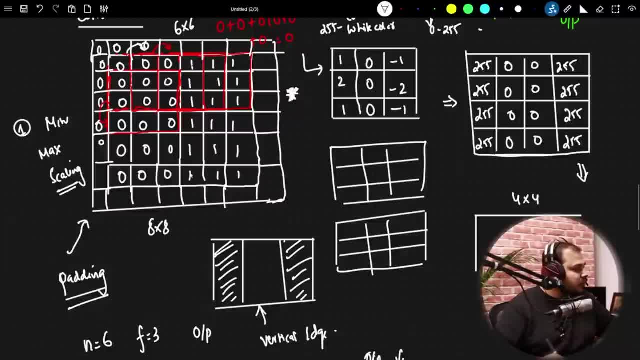 nearest value. you try to put that Like suppose I'm trying to pad or put some values over here. the nearest value is 1, so I'll try to put 1 over here. I may put also 1 over here. 1 over here. 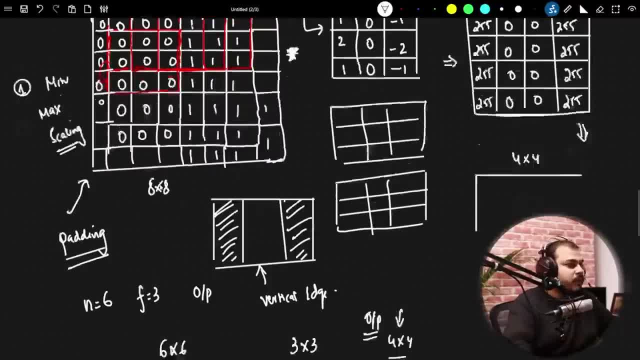 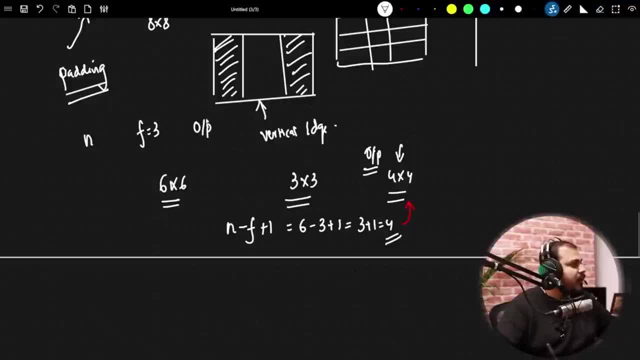 now, if I apply the same operation, what will happen? see my image size initially was six, but after applying padding it became eight. right, it became eight now. so eight minus. this is after padding. eight minus three plus one is equal to what is this value? this is nothing but. 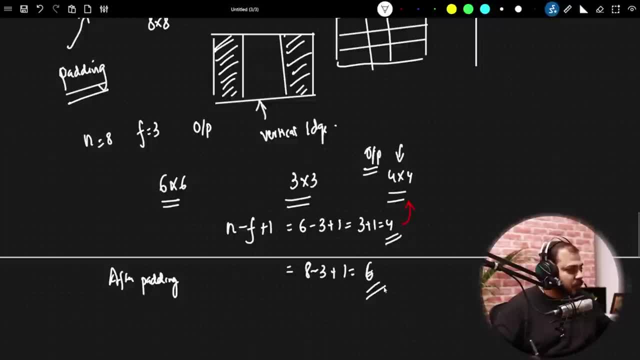 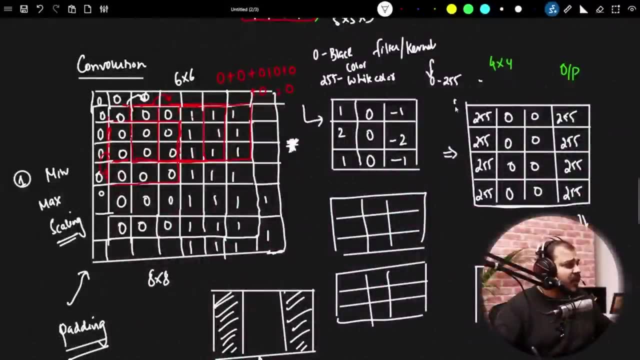 eight minus three is nothing but five. five is nothing, but output will be six. so, finally, you will be seeing that I will be able to get one more additional layer and this additional layer will actually create a six cross six image. it will create a six cross six image. 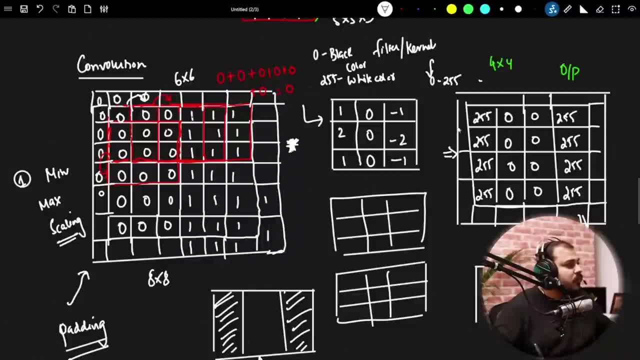 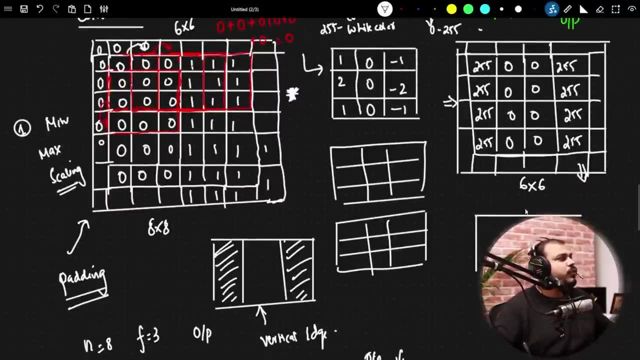 it will create a six cross six image. okay, so this will actually now become a six cross six image. this is what we wanted, right? this is what we wanted and what will be this? values that will be coming up based on the calculation. whatever we get through this filters we. 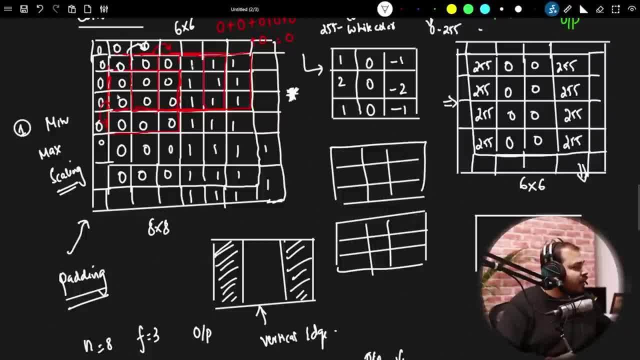 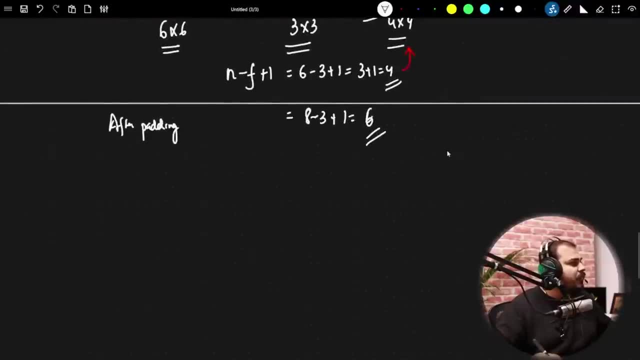 are going to get that and remember, we will be starting our again filtering operation from here, convolution operation from here, and then we will be crossing this entirely and finally I'll be getting at six cross, six output. okay, so what will be now my updated formula? my updated formula will be now like this: and plus two p, minus s. 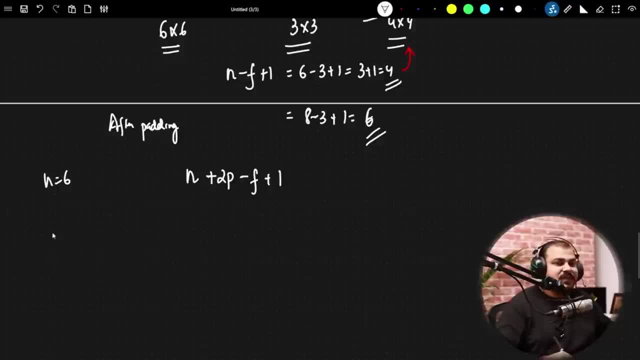 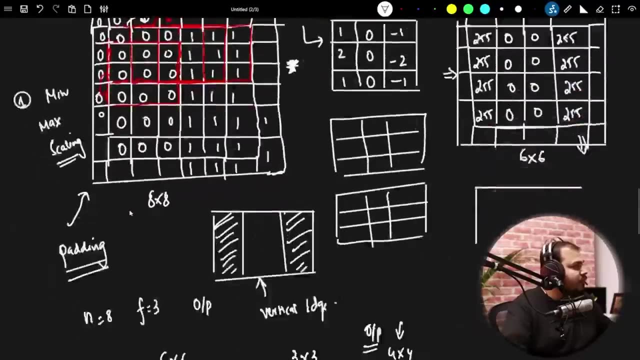 plus one. so what will be my initial size of the image? six, right, how much later, of padding I'm actually doing one padding, right? I did one padding for this, one padding for this. so I i'm writing p is equal to 1. what is my filter size? it is. 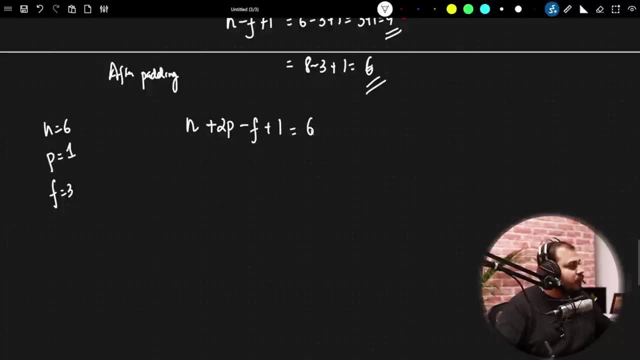 nothing but three, and here if i try to put all these values so it will become six plus two. 3 plus 1, it is nothing but 6 plus 2 is 8. 8 minus 3 is 5. 5 plus 1 is nothing but 6. 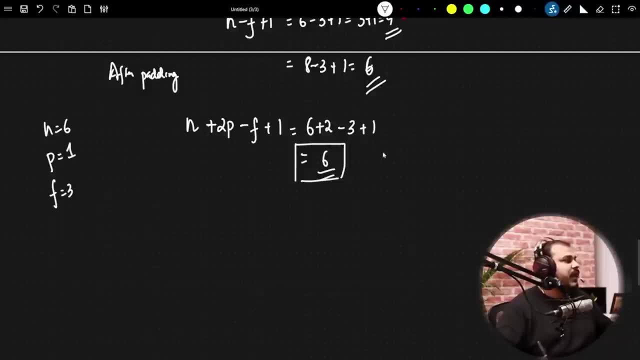 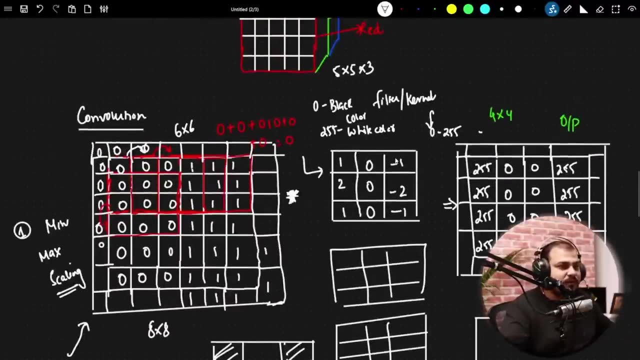 so finally, i'm actually getting 6 as my output, and this will be the output of the specific image. okay, so a very important interview question: what is the importance of padding to prevent the information loss of the image? we basically apply different kind of padding techniques. okay, so this. 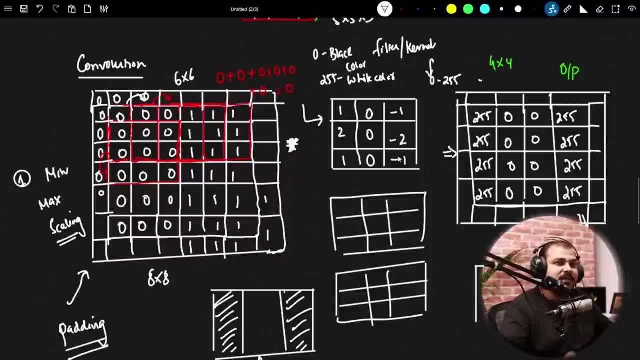 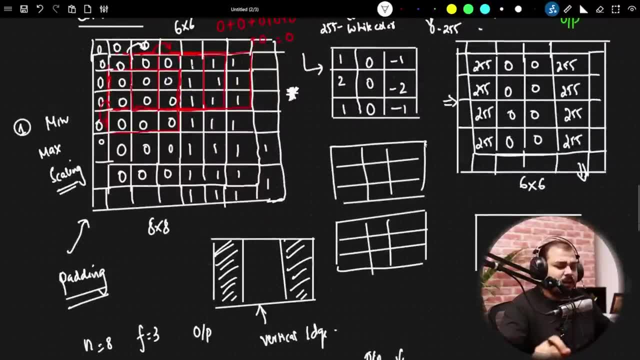 is with respect to convolution operation. i hope everybody's clear. the main thing is that i'm just trying to extract some information now. a very important thing again, very, very, very important. as many people said- or many people may have a confusion saying that, krish, why did you hard code these values and in a real world problem statement, do we need to? 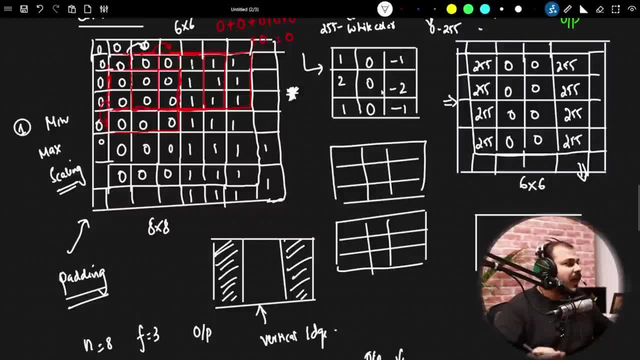 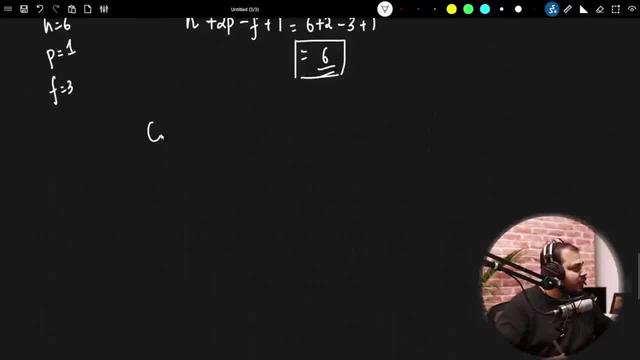 hard code this: specific values. okay, the answer is no. you don't need to hard code this like how in ann, how in ann. let's say, how in ann. we create a neural network like this: i have my hidden layer and i have my output layer right, i have my output layer right in this. we. 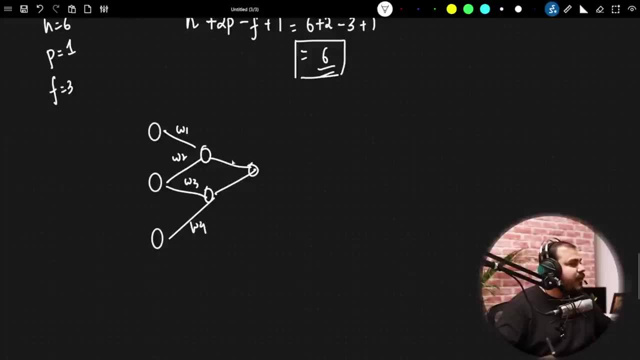 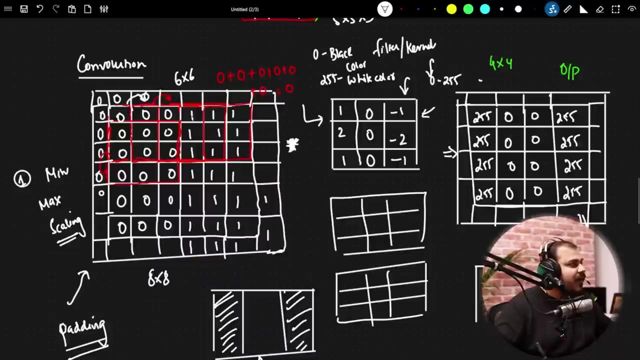 assign weights right and in the back propagation we we update this weights. so in cnn also, you also have to make sure that you update the filters based on the input. so we need to update this filter values. okay, initially let's say that we have initialized some filter randomly. 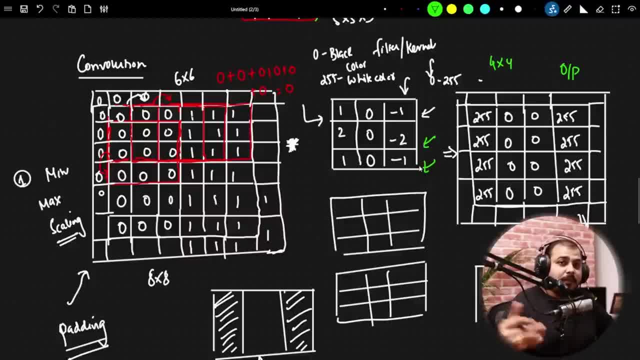 okay, initially we have initialized some filter randomly, but through back propagation again, like how we did in the case of ann. we also have to update these filters based on the input image, because every image will be different. right, every image can be a black and white, it can be rgb, it can. 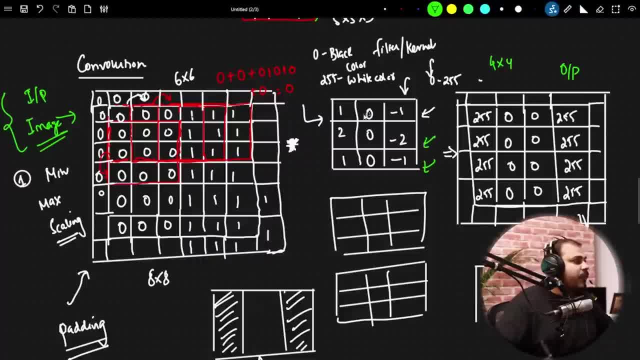 be of different, different types, right. so, with the help of back propagation, i need to update these filters. but now still the question comes that how does the backpropagation of filters work? but now still the question comes that how does the backpropagation of filters work? 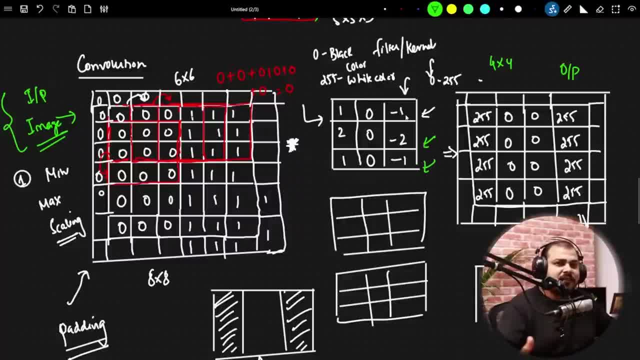 backpropagation will actually happen. we have still not used any kind of activation function, so where do we specifically use the activation function after this convolution operation? guys, whenever we get the output, on top of this, for each and every value, we apply a ReLU activation function. I hope. 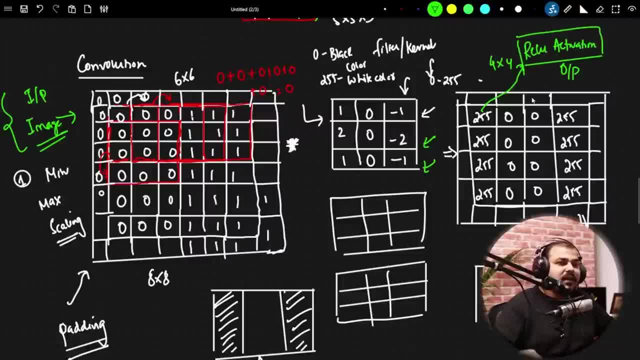 everybody knows the importance of ReLU activation function. ReLU activation function is nothing but max comma, 0, comma X, right? so I hope everybody remembers this. so, on each and every value, we apply a ReLU activation function. now the question is that: why do we, why are we applying ReLU activation? 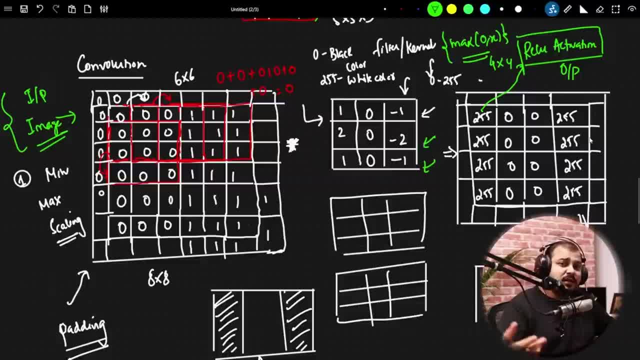 function because you know that ReLU activation function during the back propagation that derivative can be found out. right, the derivative can be found out now. since we can find out the derivative, ReLU activation function or other activation function like PreReLU can definitely get applied over here because in the back propagation we will be updating this, all kind of filter. 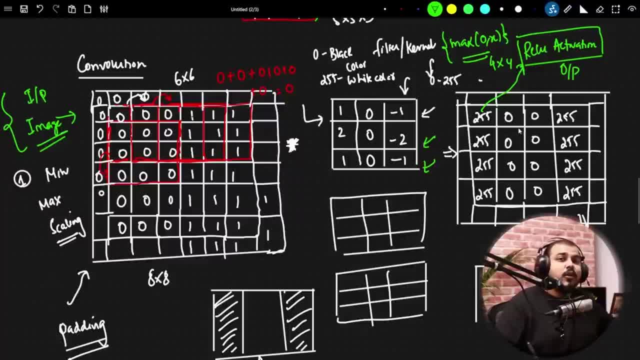 values. When we have all the values over here and we apply ReLU activation function on top of it, you will be able to do the back propagation and you will be able to find out the derivative and, similarly, you will be able to update this filter values. 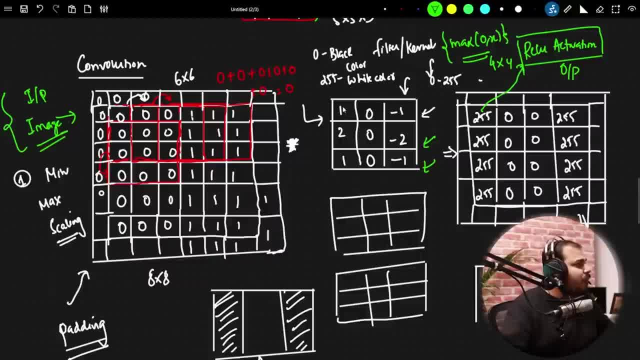 So I hope I am super clear with respect to this. One important thing: I told you about stride. Now what if my stride becomes 2, your stride can also become 2, I can jump 2 steps. I can also jump 2 steps while doing the convolution operation. will this create an impact in my 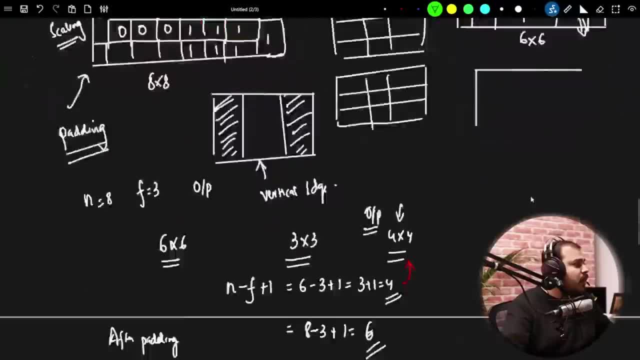 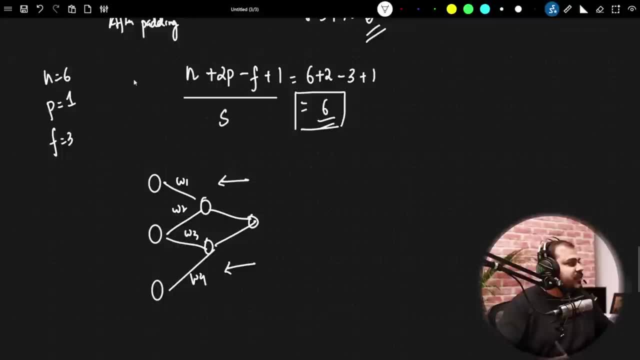 output. Yes, definitely, it can create an impact in your output. So now my updated formula. it will not be just like this, but it will be divided by S. S basically means stride, So if my S is 1,, I need not write this, but if my S is 2,, this will definitely create. 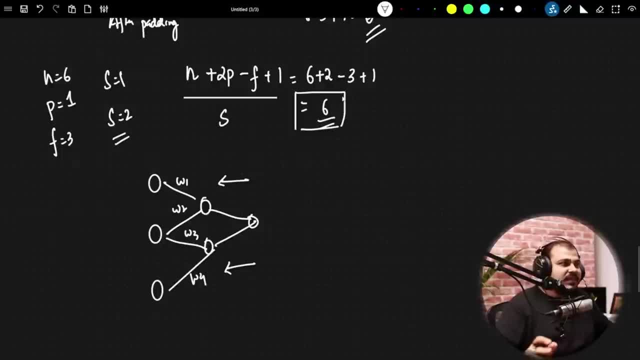 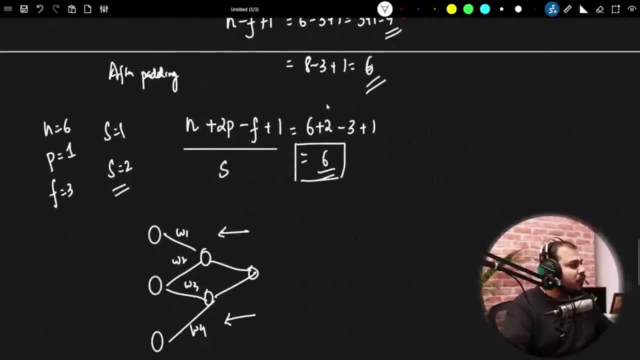 an impact with respect to my output. So is it clear guys, with respect to convolution operation, I have covered convolution, padding, stride, everything and the formula, what is the use of this? ReLU activation function, everything. So this was with respect to convolution operation. 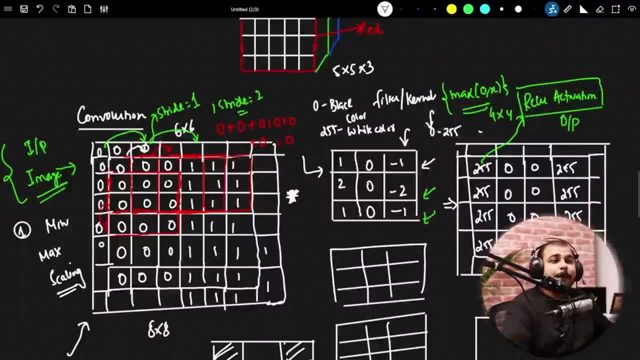 Now let's go ahead and understand the next operation, which is called as max pooling. So like this, This convolution we can have horizontally stacked right. So what all things we have in the convolution neural network? quickly, let me just write it down. 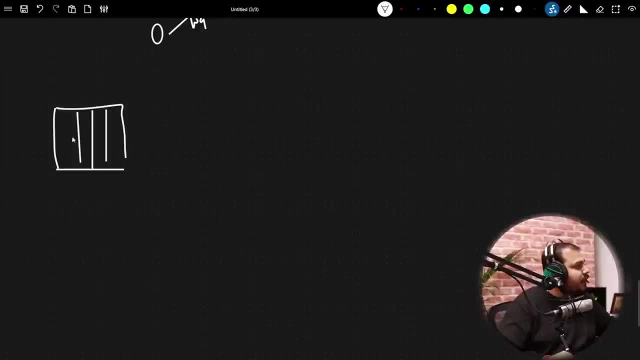 So I have a specific image, let's say some image over here: 4 cross 4, 1, 2,, 3, 4, this will also be 4 cross 4, this will get passed. this will get passed to another filter. okay. 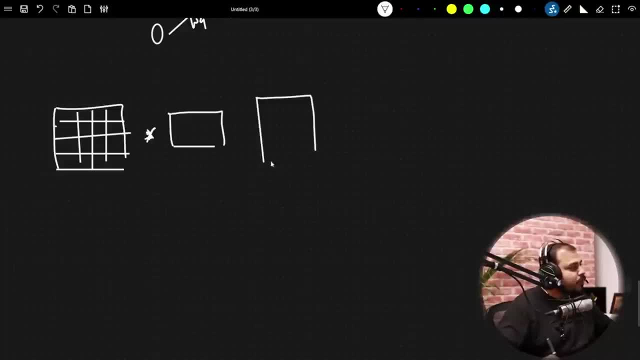 And based on this, any filter it can be, I will be getting an output right. So this entire thing, along with the ReLU activation function, is basically my convolution operation. Convolution operation And this entire thing can be stacked together. So this will be my one convolution operation and after that in my CNN, I may have another. 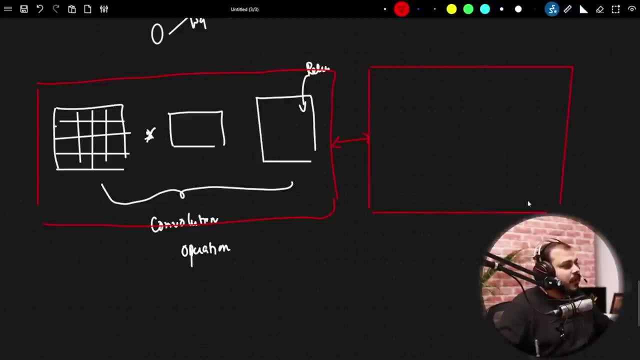 convolution operation similarly like this right And over here, I can have any number of filters. I can have any number of filters I like. Okay, This you need to understand, And our main aim in the convolution operation is that we need to learn from these filters. 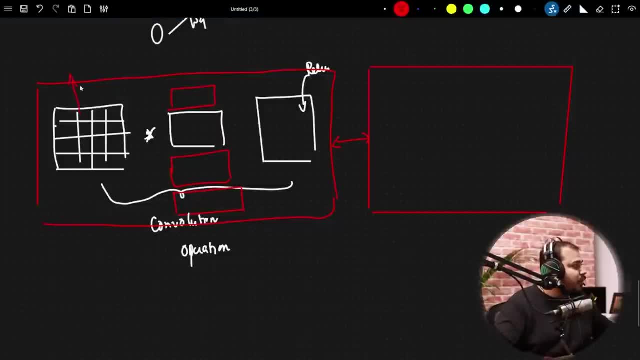 We need to learn and update based on the input images. Based on the input images, we need to learn from it. Okay, So I hope you are able to get the idea about it and you are able to understand over here, Okay, Okay. 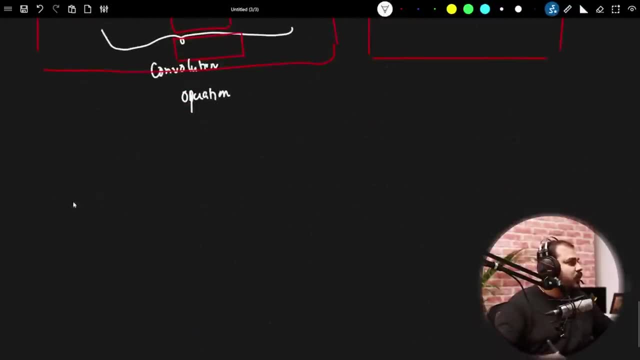 Now let's go to the second one, which is called as max pooling. Now, what exactly is max pooling? Max pooling, Max pooling- Okay, After a convolution operation, there is something called as max pooling layer. Okay, And I will show you in images also how it will look like over here. 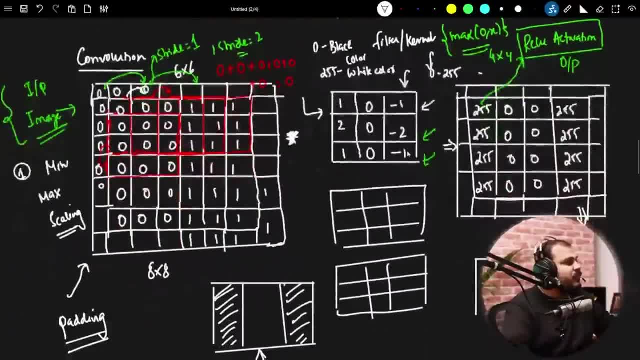 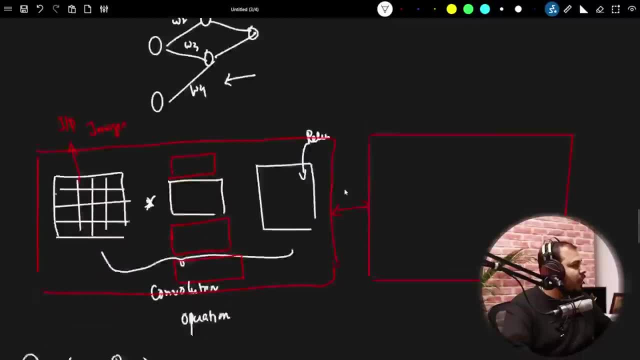 Just try to understand the crux. Understand the keywords that I am specifically using, Right? This will all actually help you to understand in a better way. Okay, Now filters can be selected in different, different ways. You can have a 5 cross 5 filter. 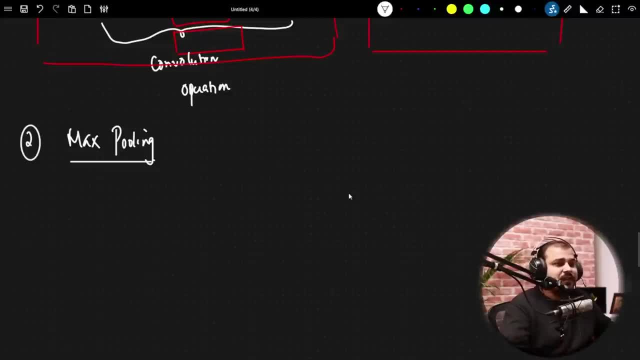 You can have a 7 cross 7 filter. You know you can have a 3 cross 3 filter. This is all like kind of hyper parameter tuning. Later on in the upcoming classes I will probably take one more live session There. I will discuss about transfer learning. 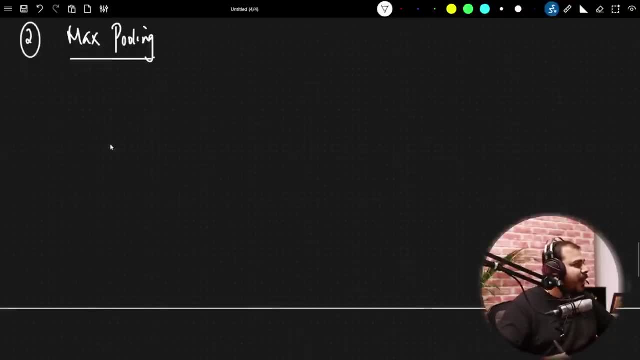 Okay, Now in the max pooling layer. What happens in a specific max pooling layer? Let's say this is my input. Let's say I have 3 cats. Okay, So this is my cat 1.. This is my cat 2.. 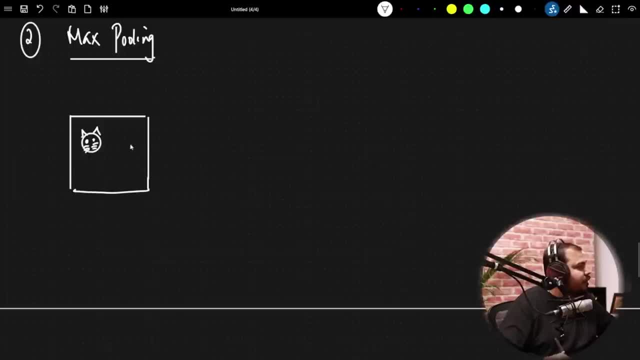 Okay, I hope you like my diagram, And this is my cat 3.. Okay, Let's say this is my image With respect to a cat, And then my first operation is basically my convolution operation, where I start, pass through a filter or kernel. 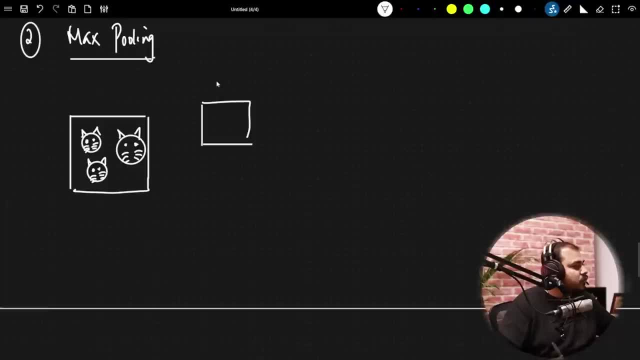 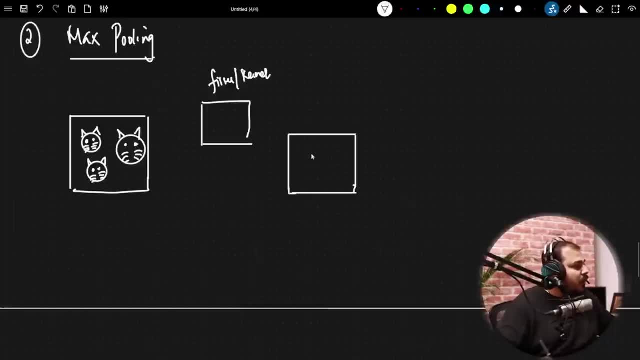 Okay, This output and after the output, we apply a relu activation function. So this entire operation is my convolution. So that basically means I'm applying this And I am getting this. So this is my convolution operation. Okay, Now, Now, after this, what can we have? 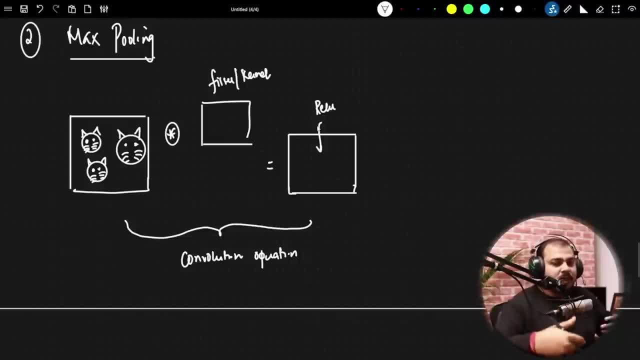 We can have multiple convolution layer also, But again, I've seen a lot of transfer learning techniques where they have used another layer which is called as max pooling. So here I'm just going to define something like this: Okay, And this layer is basically called as max pooling layer. 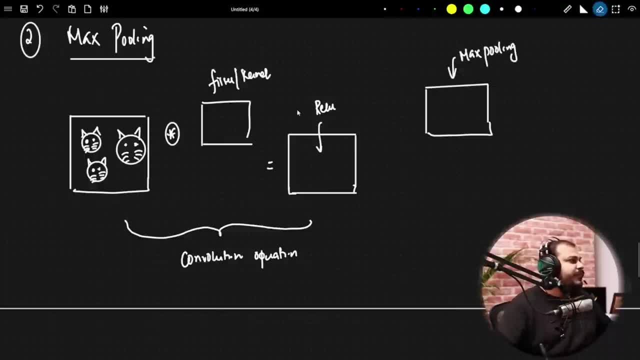 I'll talk about max pooling layer And let's say, after this convolution operation, I applied the ReLU and I probably got a 3x3 output with some values. I'm just going to initialize values, So don't worry that. how did I take up? 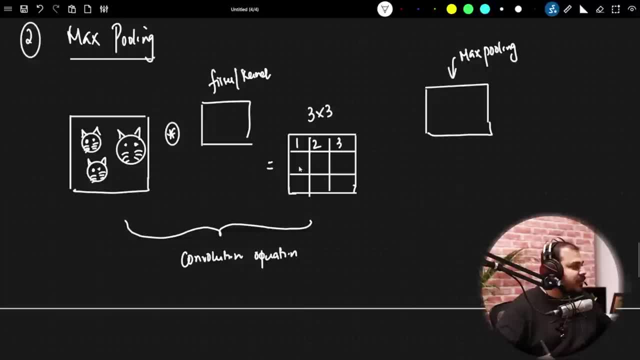 Let's say that this is a 3x3 and I've got some pixel values like this: 1, 2, 3, 4, 5, 7, 0, 3, 5.. So let's say this is my this. 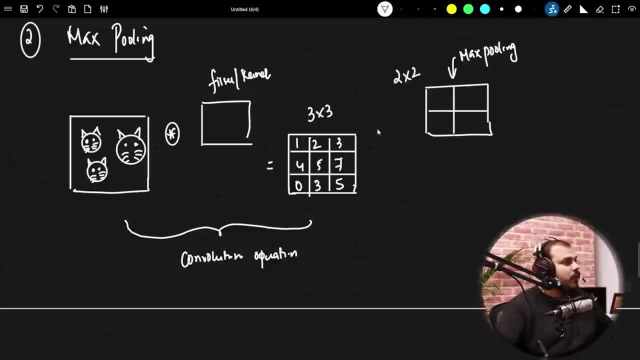 Let's say I'm using a max pooling of 2x3.. Now why exactly max pooling is used? Now see guys, here I have three cats. right Here I have three cats. Okay, And when I apply a filter operation, let's say, from these images I'm able to see the rounded eyes and probably I'll be having another filters also for vertical edges, horizontal edges and all. 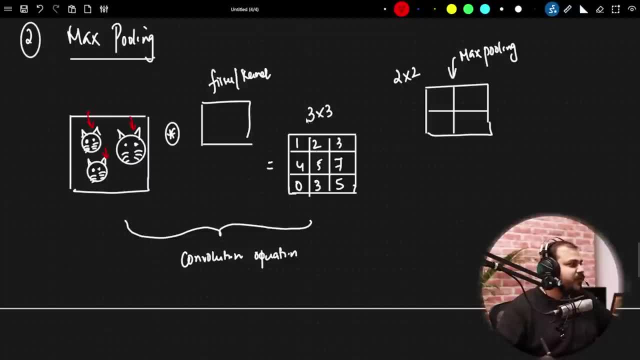 Now some information I'm able to extract from this particular filter. Let's say, I may have any number of filters as we go ahead, Okay, And I'm just focusing over here. Okay, Now there is a concept which is called as location invariant. 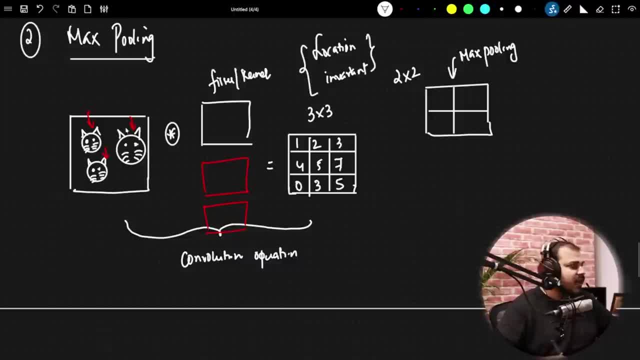 Now, what does location invariant say? is that Location invariant says that, let's say there are multiple objects in the images. My convolution neural network. till it goes ahead towards the next layer itself, it should be able to extract more and more clear information. 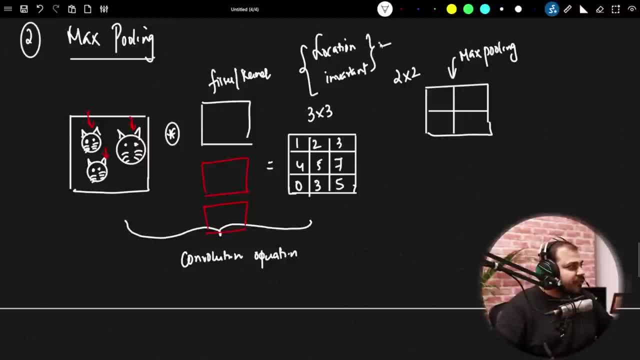 Okay, More and more clear information. So location invariant basically says that my objects may be present anywhere, but as we pass from many convolution layers, I should be able to extract the information more in a better, in a clear way, right? 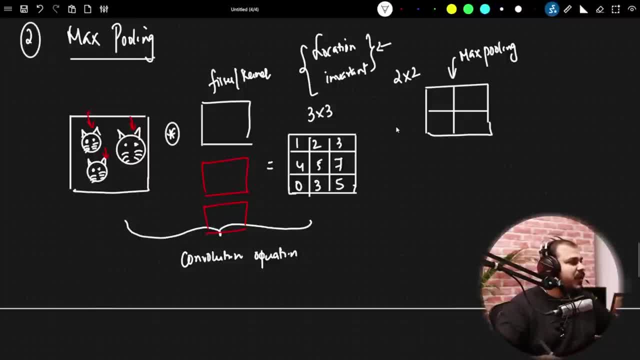 And for that we specifically use something called as max pooling. Now, in max pooling, what it does is that let's say, how do I extract much more clear information? Now, how does this information look like When I apply max pooling? max pooling says that. okay. 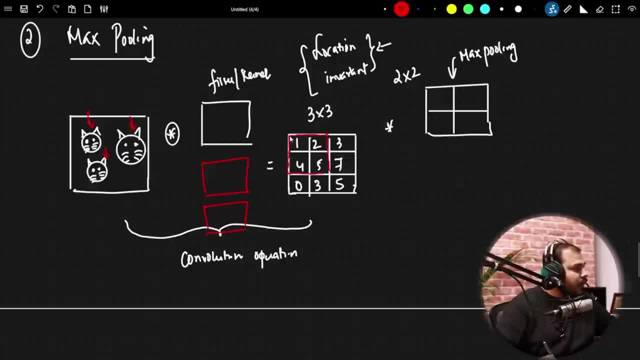 Okay, So I'm just going to place on top of it and let's say what? and there are different types of max pooling layer. There is something called as average max pooling. Let's say there is something called as average pooling. 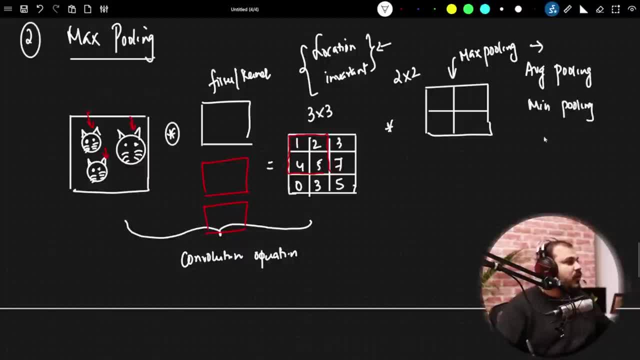 There is something called as min pooling And this is my third type, which is called as max pooling. Okay, Let's say, in this particular scenario, I'm using this max pooling. Now, max pooling. what it says is that I'm just going to place this on top of the output over here. 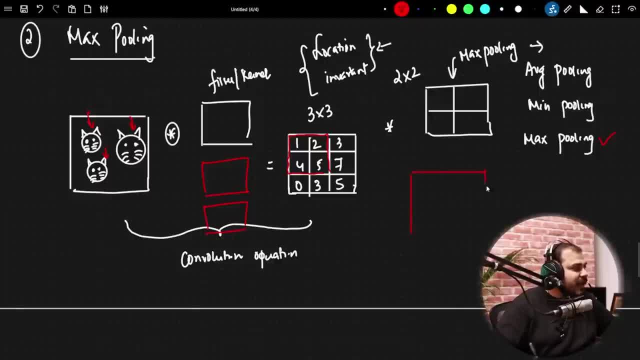 And what I'm actually going to do. I'm going to basically get an output, And this output will only be focusing on the biggest number, the most clear or the highest number over here. Which is the highest number over here? Clearly, you can see that five is the highest number. 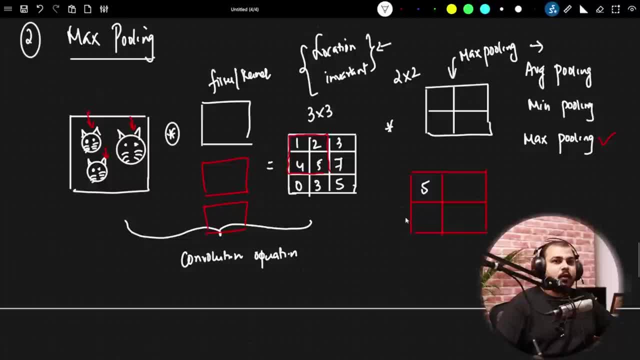 So I'm going to take this information only and update it over here. That basically means one of the cat eyes is clearly visible, So I'm just going to pick up that information and put it over here. Okay, Then I'm just going to jump to the next stride. 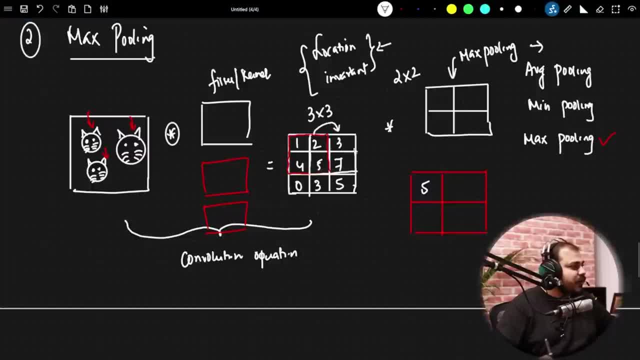 Right In the next stride. what I'm actually going to do? I'm going to basically jump like this and basically take up the next one From this. the highest value that I'm actually going to get is seven. let's say: 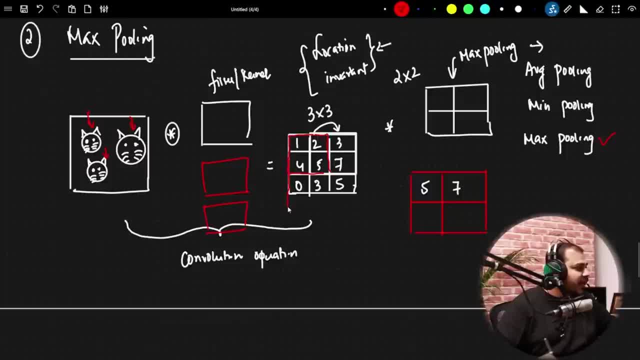 Then I'm going to jump next downwards in this direction, Let's say in this direction and this direction, And I'm going to basically see that which is the highest value. So over here also, I'm going to get Probably three, and over here I'm going to get five. 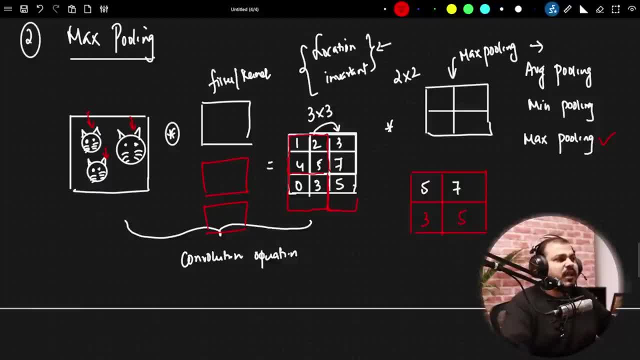 So the most specific and the clear information. I definitely want it from this. Okay, So what I'm actually specifically doing? and over here, guys, one more thing that you need to really understand is that here I'll make a stride of jump two. 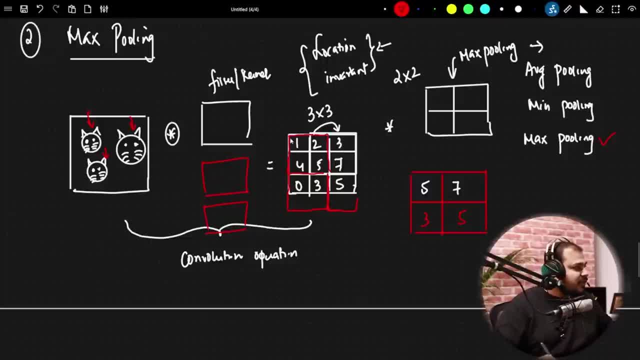 Okay, Stride of jump two, not stride of jump one. Let's say, initially stride was here, I got the value as five. My next jump will be a two step jump, So my next one will be starting from here and it will be ending like this: 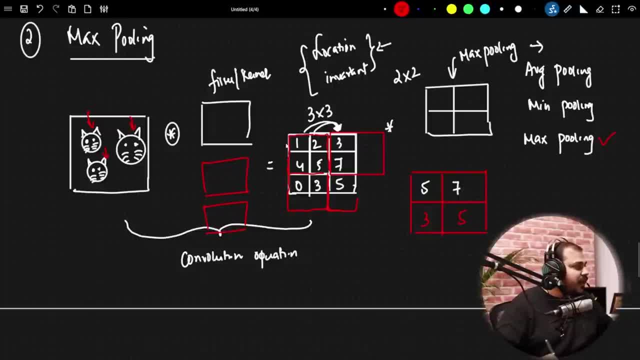 And out of this I have my highest value as seven. Then, similarly, I will make a stride two jump downwards. So this will be my next one From this, I know, which is my highest value: three, And then I will again make a stride jump of two. 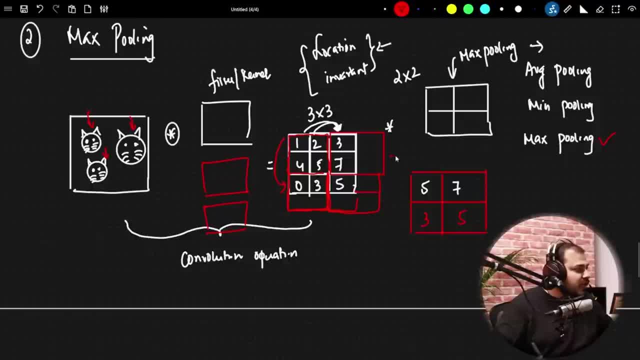 And when it comes over here, whatever value is highest, I'll be getting it. So here I'm actually trying to specifically take up the most important information out of the output that I'm I've got for this specific filter. Okay, 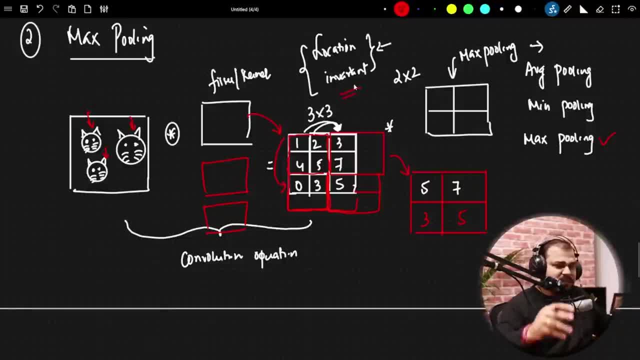 And this basically solves the problem of location invariance. That basically means if I have multiple objects also and if one of my filter is able to determine that particular object, it will be able to clearly pick up from there. Okay, So I hope everybody's able to understand till here and I hope everybody's understood about the max pooling right. 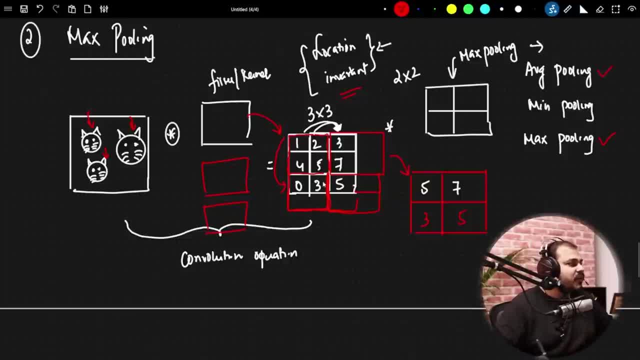 Now suppose I want to use some other pooling, Let's say average pooling. In average pooling, nothing will happen. We will just try to find out What's the average of all these values And similarly, in min pooling, what we are going to find out. 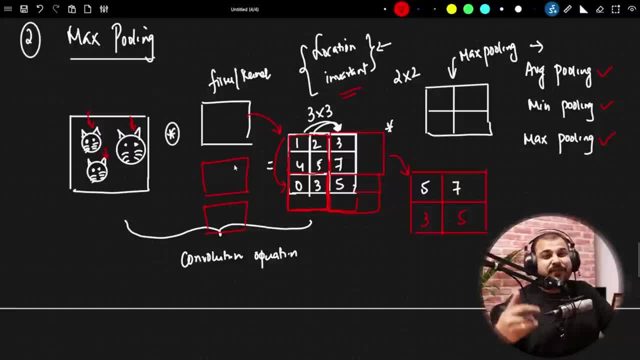 We are going to find out the minimum values Now, based on different, different problem statement. we can play with either of this pooling layer. Okay, We can either use max pooling, We can either use min pooling. We can either use average pooling. 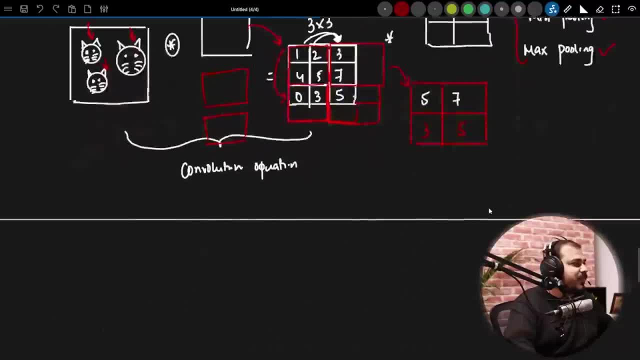 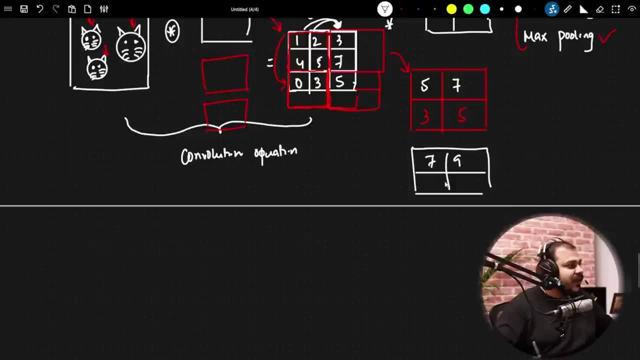 Okay, So finally you get this. And with respect to different, different filter operation, again I may get another two cross, two over here with some values, let's say like seven, nine, two, one. Then another filter will actually able to give me some other values like six, five, three, one, right. 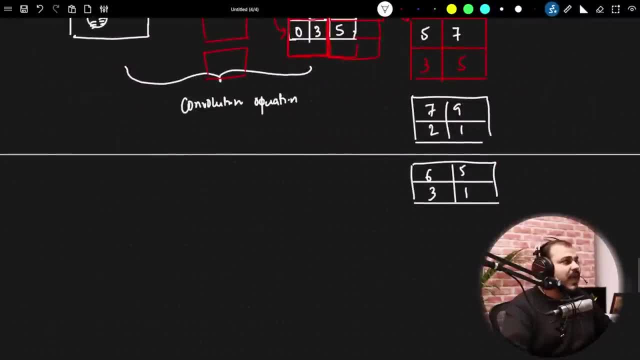 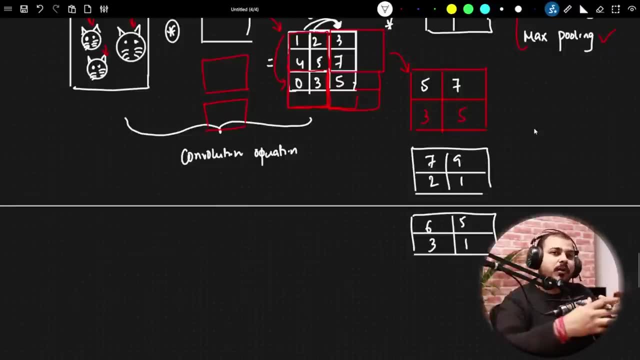 So all these values that I'm actually getting, like this, okay, what I'm actually going to do now. this is the end of the max pooling layer And again, convolution and max pooling layer is used as a combination. We can stack it horizontally any number of times based on different, different neural neural net. 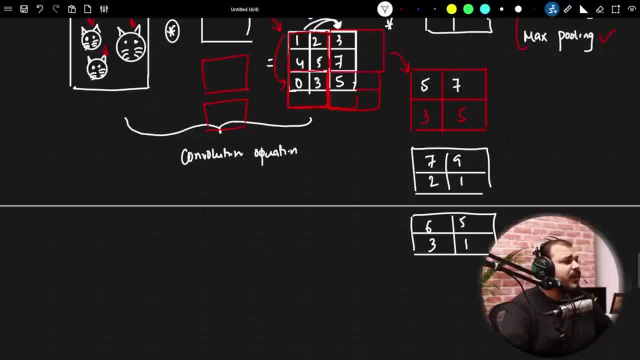 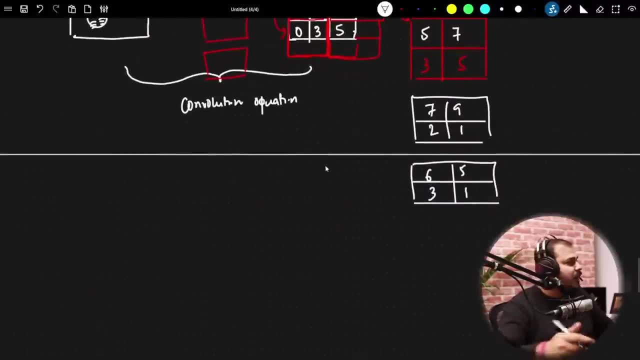 Okay, Different, different neural net. Now, what will happen after this? After this, there is an Amazing layer, because finally we get this output right, Everyone. then after this, we have something called as flattening layer. Now, flattening layer is pretty much simple, because this will actually look like an ANN dense layer, only ANN dense layer. 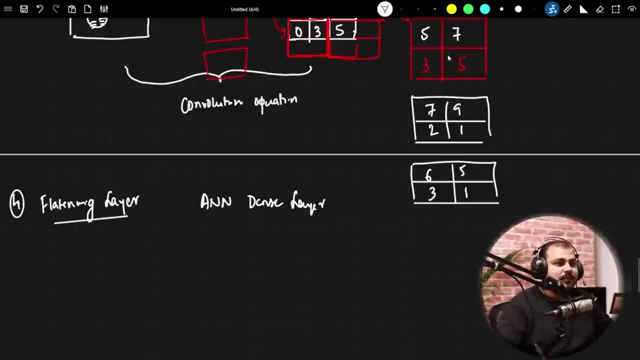 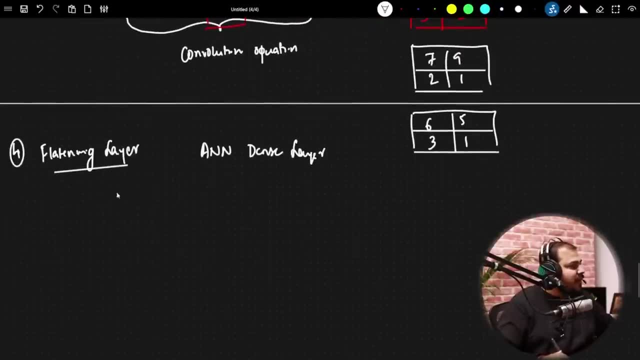 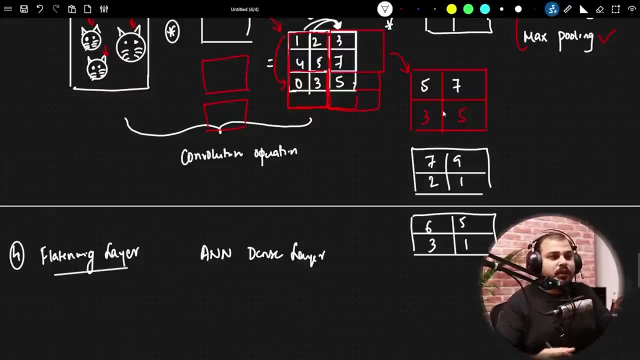 Now, whatever inputs, whatever outputs I get from this max pooling, I am just going to make it straight forward: flattened. flattened basically means I will just go. I'll just pick up this entire filter and I'm just going to elongate it like an input, like how we give input to a ANN right. 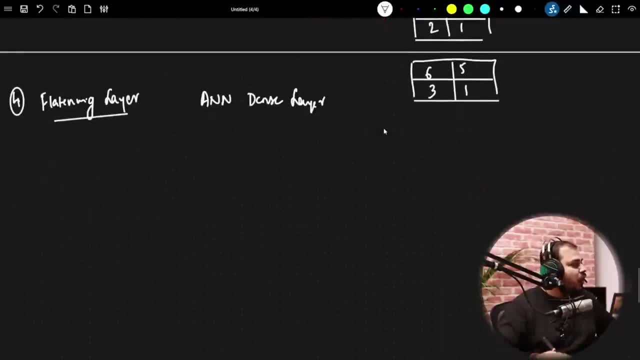 Like that. we are going to flatten it. So my five, seven, three five will get elongated to something like this: It'll become five, seven, three five, and this will basically get elongated, which looks like this: 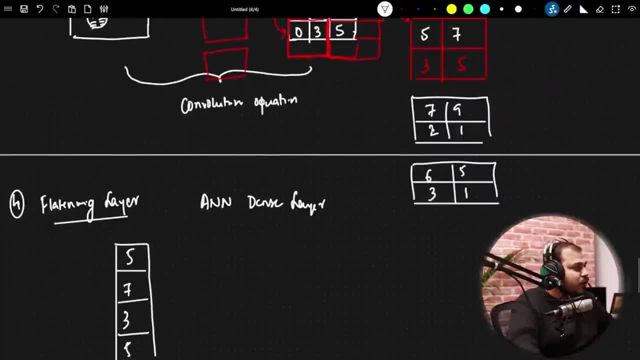 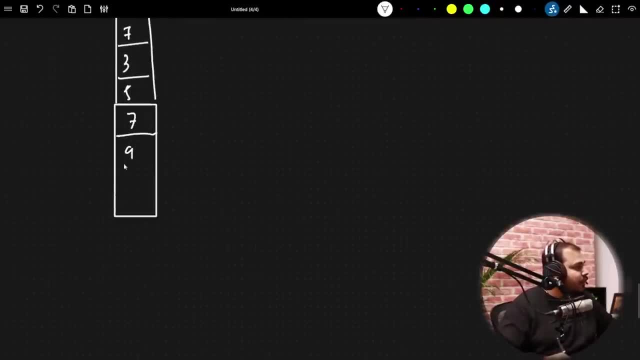 Okay, Then the next filter value that I'm going to get: seven nine two, one that will also get attached to this. So now my seven nine two, one We'll also get attached over here, Right? Similarly, I'm going to flatten this entire, all the filter outputs, and I'm going to combine it over here. 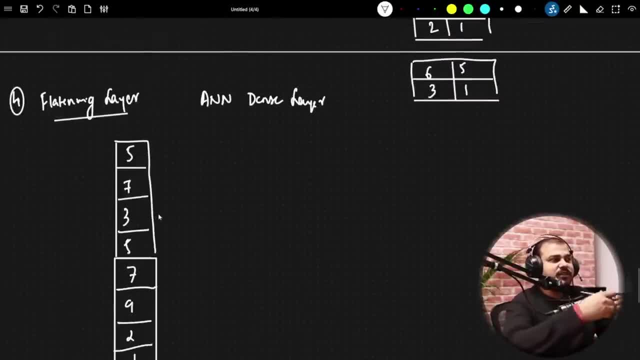 Okay, This is basically called as a flattening layer. I'm just flattening it, I'm just elongating it, And now this becomes an input to my dense layer. Then you go and create a fully neural network connected layer, and how many number of outputs you have. 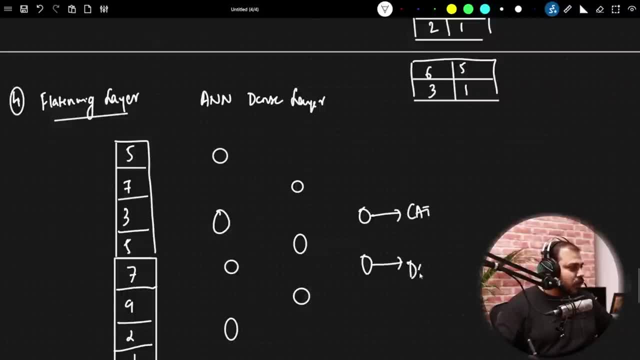 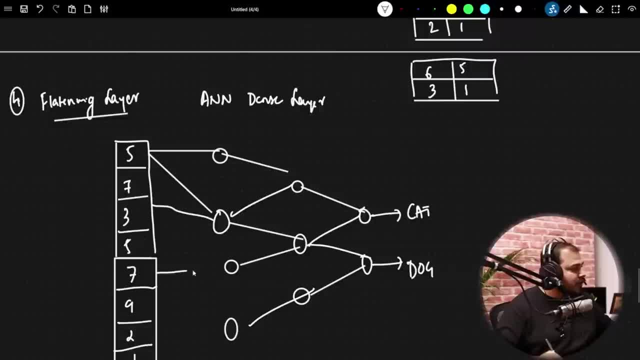 This will, this will all the information will be going to this, all the neural networks, Okay, And finally, I will be able to do this image classification in this specific way. In short, what all things we did, let's say, this is my convolution operation. 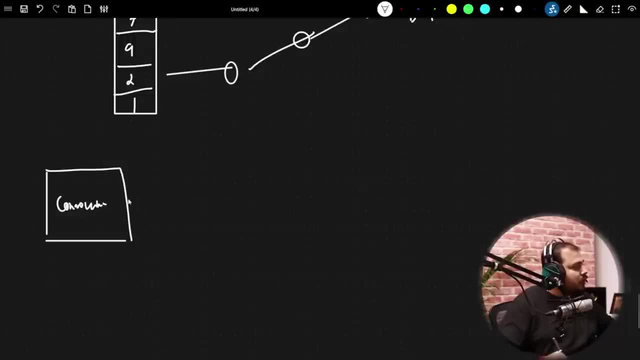 Okay, Convolution operation. Then I went to my max pooling layer. Max pooling. This convolution operation has what all things? Convolution padding, applying filters, everything happens inside this. Then, after the max pooling layer, what we specifically do? we provide it to the next stage, which is called as flattening layer. 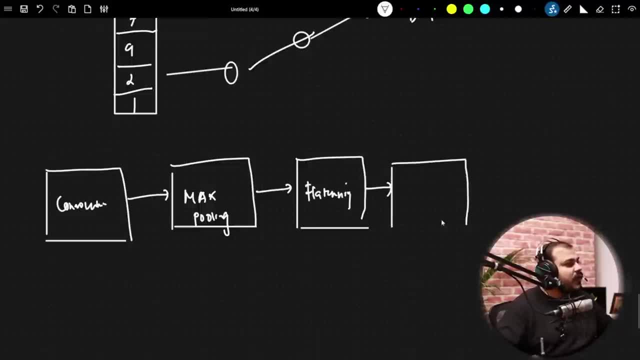 And then we create a ANN or fully connected neural network, And finally I get my output Right. So these are my entire steps. So I'm just going to open this browser. Everyone see over here If I probably try to go and click on images. 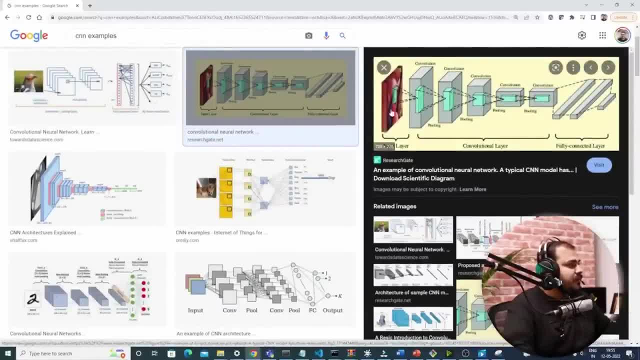 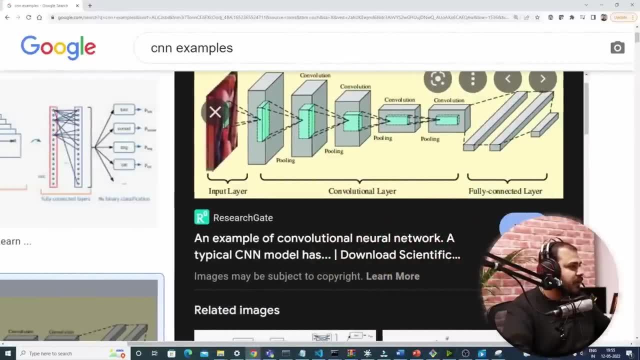 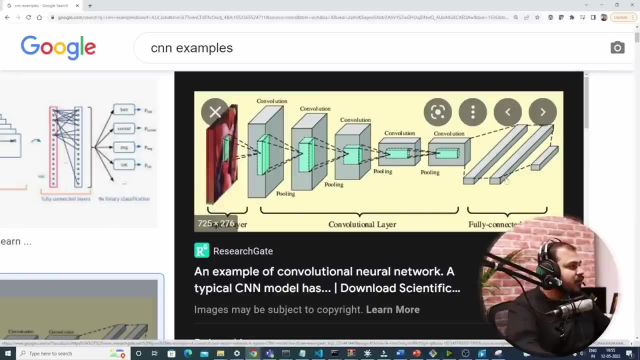 Now you see over here. Right, This is my image. Okay, Probably you'll be able to see over here very clearly. Let's say Again this I've taken from Google. See this: convolution, pooling, convolution, pooling, convolution, pooling, then flattening, then fully connected layer. 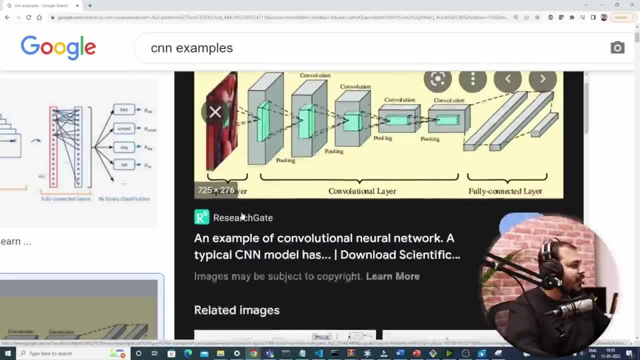 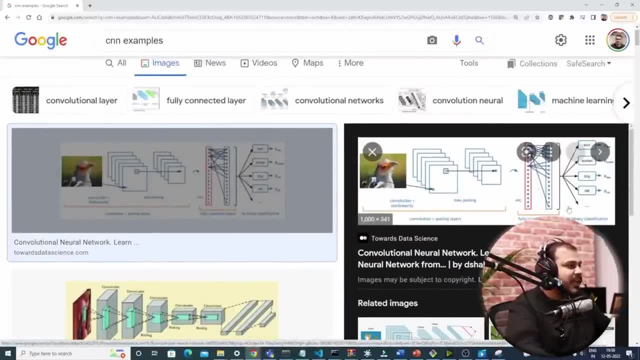 Right, So this way you will be able to see. you can also see other other examples: Convolution, nonlinearity, max pooling, fully connected layer and classification. Right, So we give this image. each and every pixels gets passed. All the information is basically getting extracted. 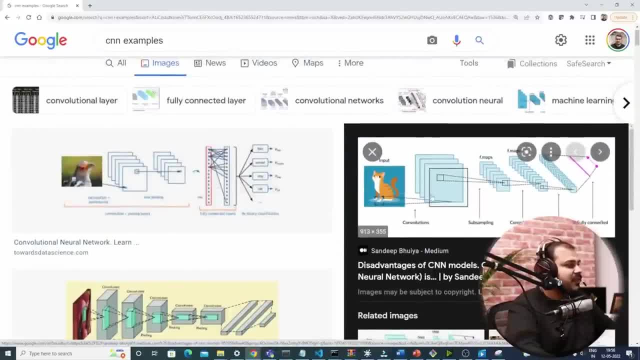 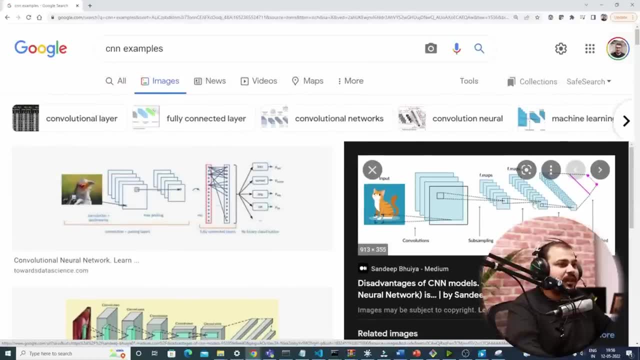 Similarly. here also you can see, this is my input image. I pass it through a convolution, Then I basically got the filters output. Then what we did we did applied another convolution layer, Then we got a fully connected layer, you know, and then finally we got an output. 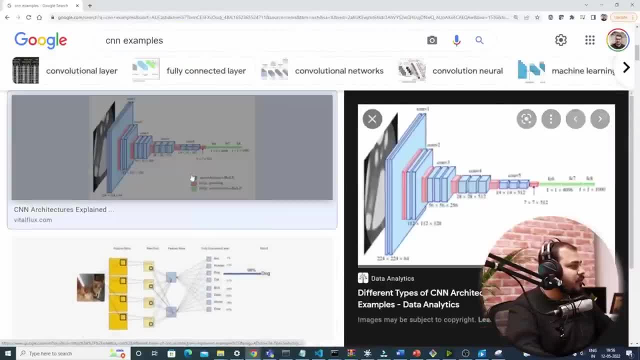 So, like this kind of operations you will be able to see- See here also this image- we applied to convolution layer, Then we applied a max pooling- Red color is max pooling layer. Then you can see that we have got another convolution layer. Then again, we applied a max pooling. 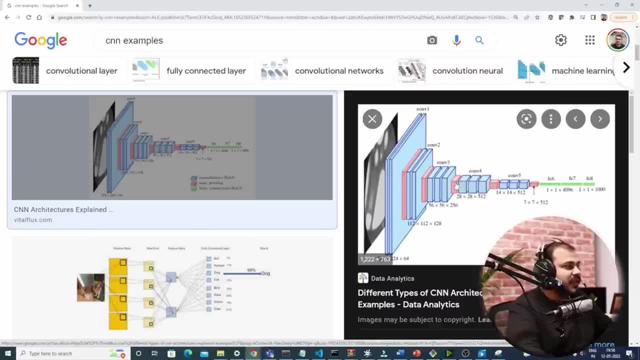 Then we applied convolution layer Three, three times convolution layer. Then we got a max pooling, Then convolution, max pooling, convolution, Then finally fully connected layer. fully connected layer and fully connected layer Right By default. max pooling layer through the code is basically taking two. 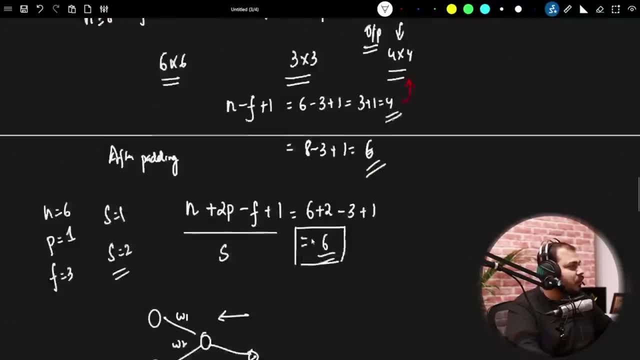 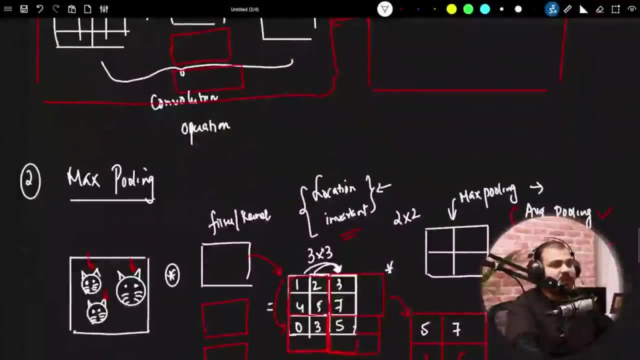 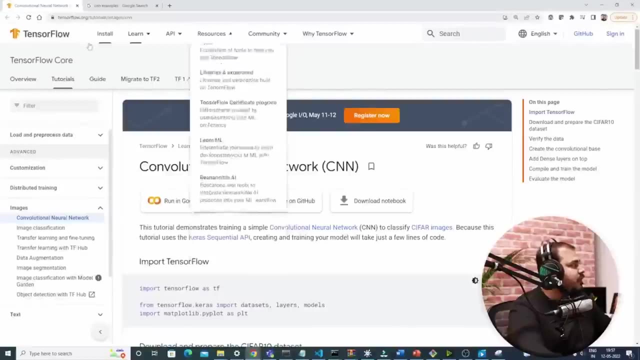 So, guys, did you understand whatever I explained with respect to all the CNN neural network? Can I get a quick yes, if you are able to understand, Now we will try to do one practical example: Yes, So what I want you all to do is that. 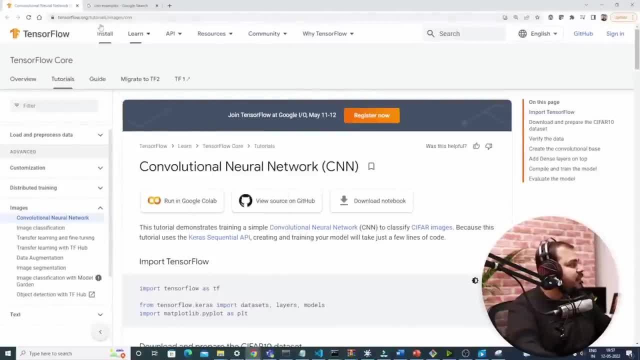 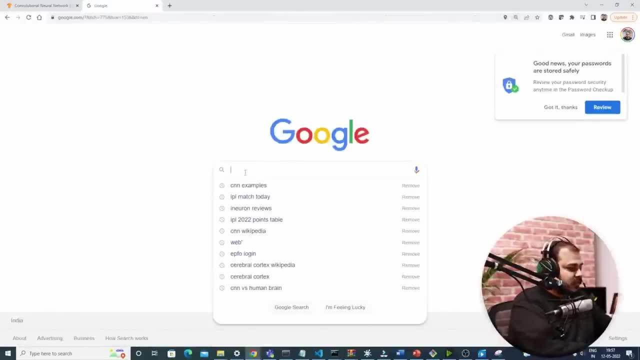 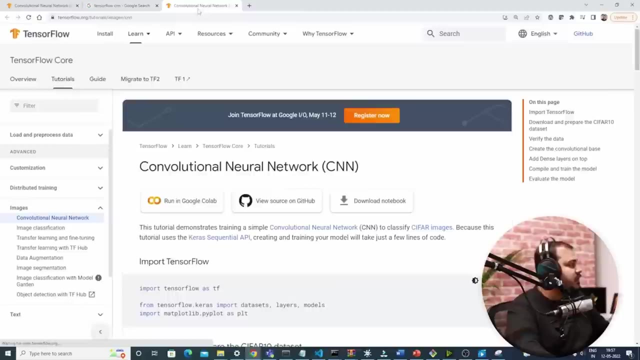 just go and search for TensorFlow images, CNN. Just search for TensorFlow CNN like this: Just go and search for TensorFlow CNN And here you will be able to see the first over here. an example over here. Okay, Okay, Now you cannot determine. 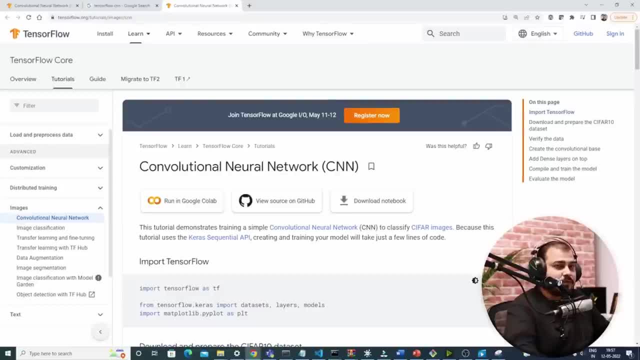 One thing is that how many layers you can actually use. Okay, So there you need to understand from the transfer learning. People play with different kind of layers. There is an ImageNet competition where people focus on understanding that how many layers needs to be used. 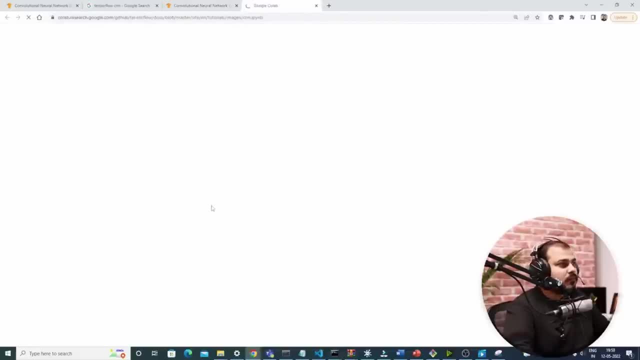 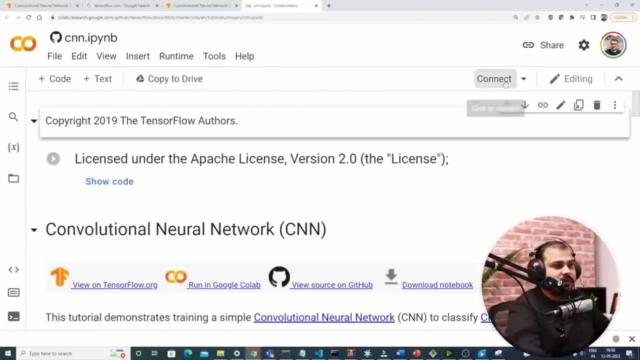 Now just go and click on run in Google Colab Once you search this convolution neural network, go and click on run in Google Colab And here use your specific output Automatically. when the traversing of the entire images will complete, you will get the image. traversing will get complete. 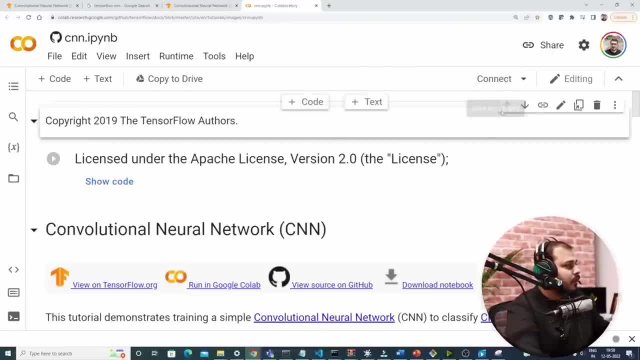 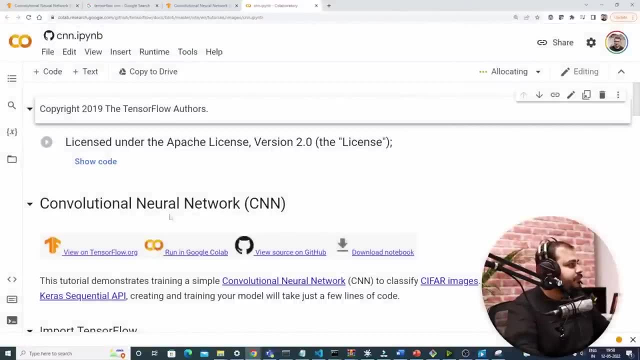 That time the stride will stop moving. Okay, So here is my TensorFlow connected and I'm going to change the runtime to GPU Save, Connect it. Okay, So here you can see that what all things we have actually done. Okay For this. 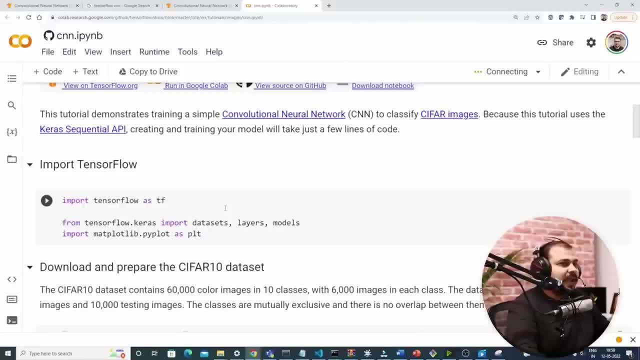 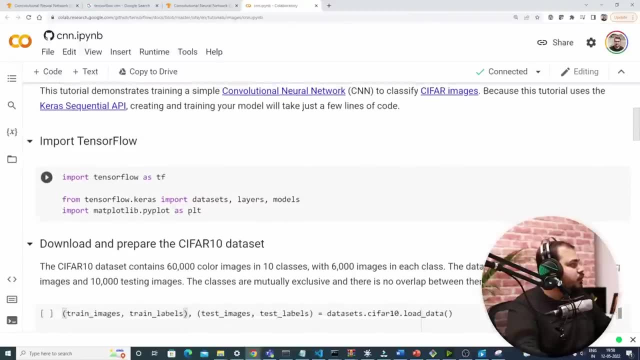 Max pooling is specifically related to extracting more information from a specific image. Okay, So, as usual, I'm going to import TensorFlow, TensorFlow- Keras. I'm going to use data set layers and models. What kind of data set we are going to use? 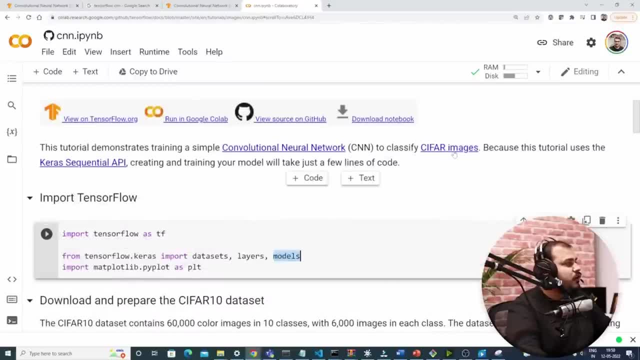 We are going to use CIFAR images data set. So if you click on this, CIFAR images has what all things? It has this: all kind of images like airplane, automobile, bird, cat, deer, dog. So we are going to classify. 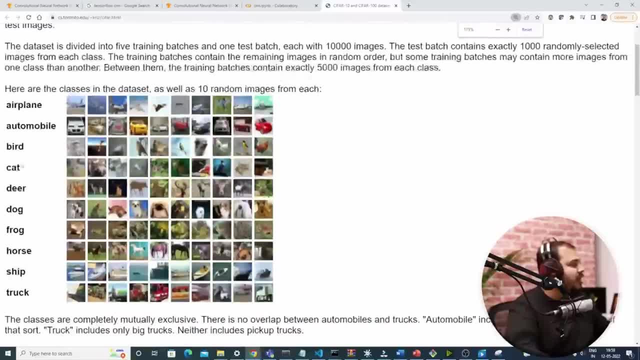 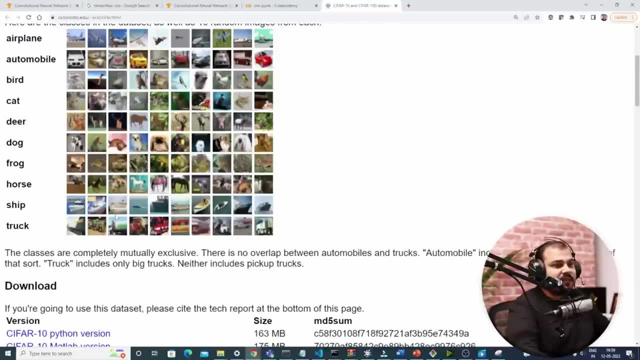 Whenever we get this kind of images, we are going to classify them. Okay, Now let's go ahead. We are going to classify these images. Okay, Now let's go ahead. We are going to classify these images. We are going to classify these images. 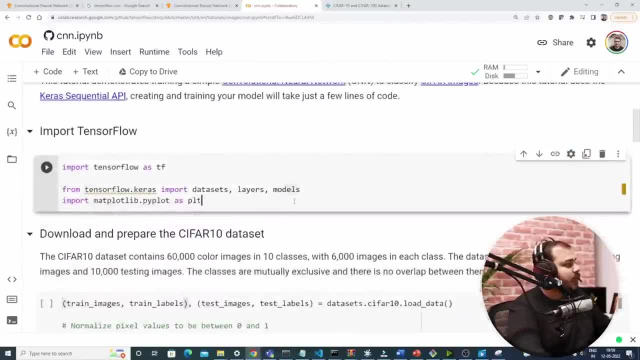 Okay, Now let's go ahead and let's quickly execute. So here, first step, I'm just going to execute the TensorFlow part. It will get executed. Let's see how much time. Yes, it has got executed Now. 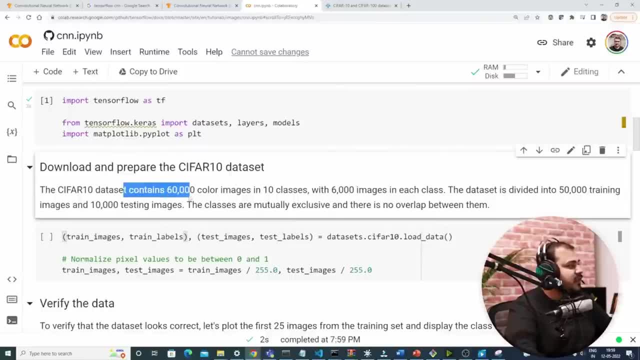 let's download and prepare the CIFAR 10 data set. This data set contains 60,000 color image in 10 classes, with 6,000 images in each class. The data set is dividing into 50,000 training and 10,000 as test image. 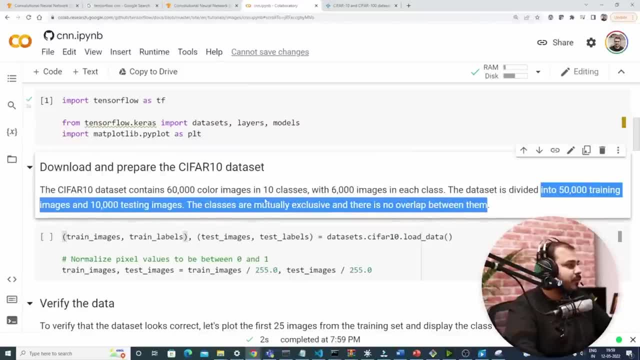 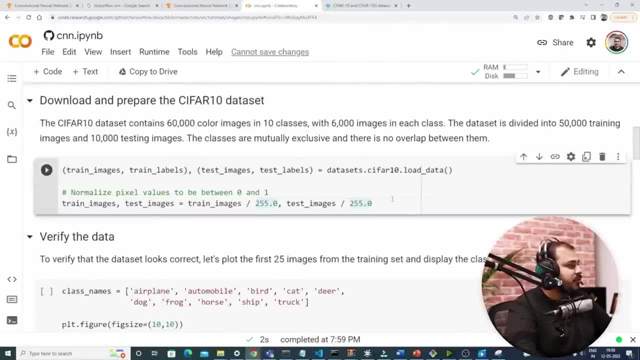 These classes are mutually exclusive and there is no overmatch, There is no overlap between them. Fine, We know all these things, And then we are going to basically say: training images, training label, training test images and labels. Okay, As I said, 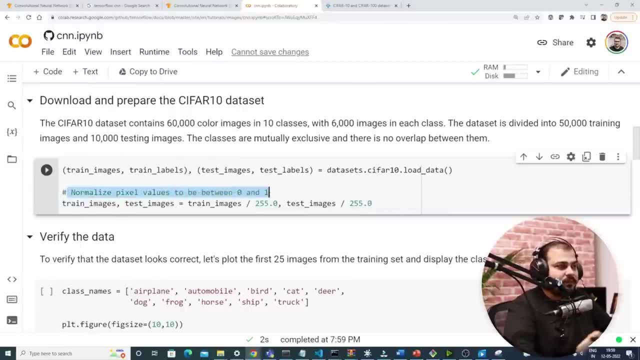 we need to normalize the values to between 0 to 1.. In the first stage- we have already discussed this while explaining the theoretical part- We will normalize it and we will always make it between 0 to 1.. So all we are doing is that- the training and the test image. 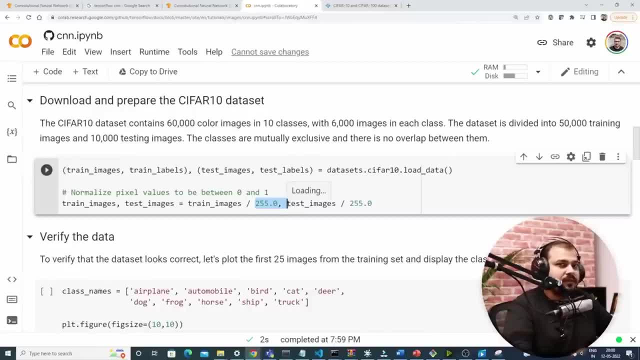 we are dividing it by 255.0.. If the pixels are 255, it will become 0,, sorry, 1.. Otherwise, it will become 0 if the values are 0 pixels. Okay, So I am just going to execute this and automatically. 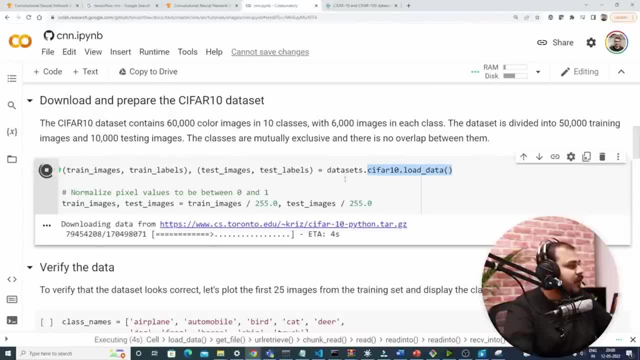 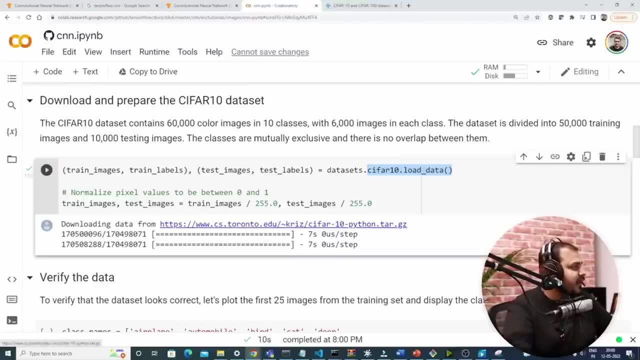 this data set will get downloaded from this particular library: datasetscifar10.loaddata. Okay, So you can just execute this quickly, get it. And here you can see that I have downloaded all the data set from using this specific example. 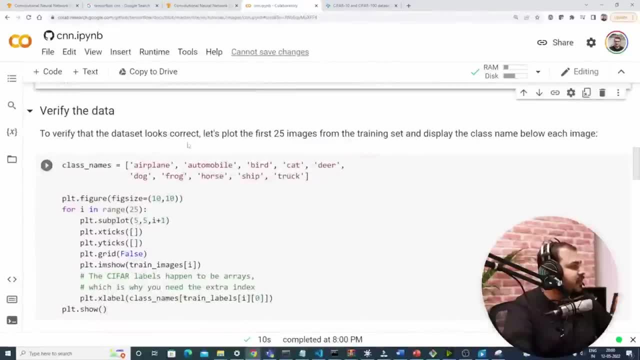 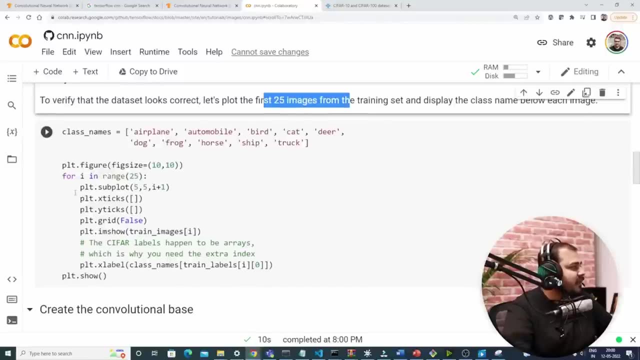 Okay, Now verifying the data set. To verify the data set, let's plot the first 25 image from the training set. So we are just plotting it. That is the reason we use matplotlib. I don't think I need to explain you this, because you already may be knowing matplotlib. 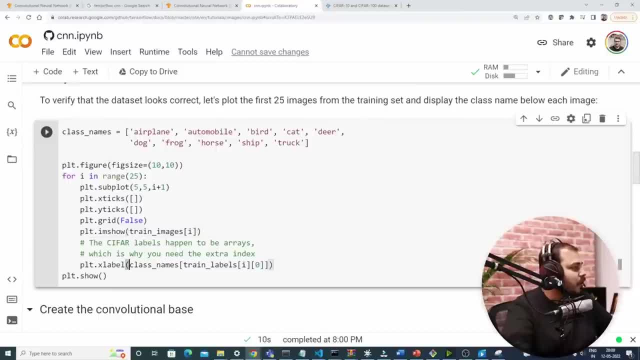 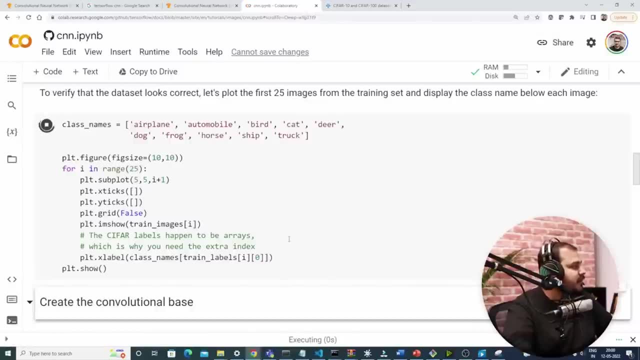 Okay, So here what we are doing based on the class names. we are plotting it And I am taking the training labels and first 25 image. whatever I get, I am just plotting it over here. So once I execute this, 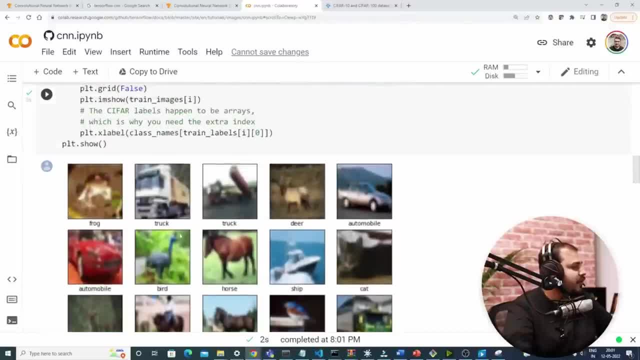 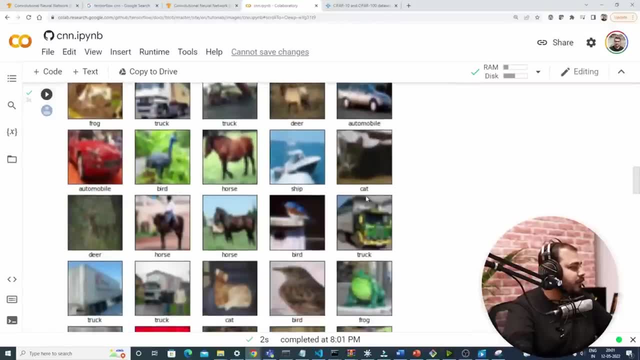 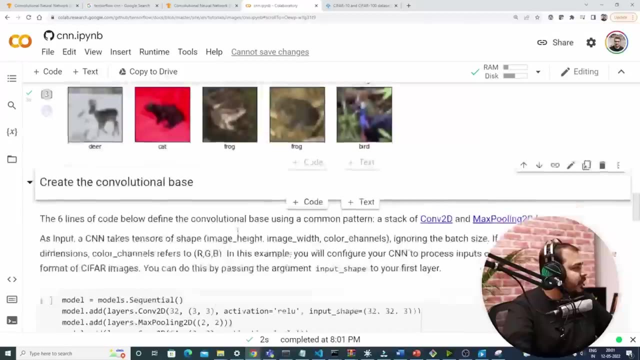 you will be able to see that I am able to get the first 25 images, which looks like frog truck, truck, deer, automobile, automobile, bird, horse, ship, cat, deer horse, horse, horse, everything I am actually being able to get. 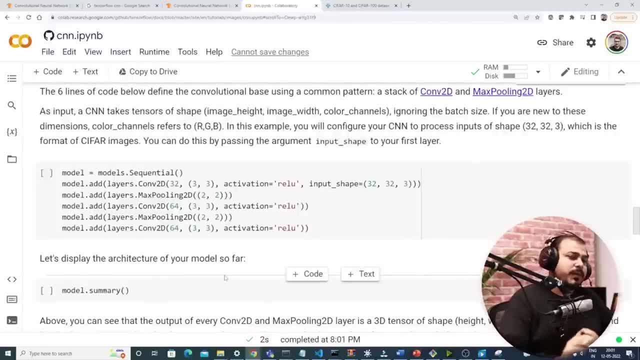 Okay, Then let's go ahead and create a convolution neural network. Now see this, guys. This is super important, super easy. If you are focusing away, you will be able to understand. In the ANN also, we first of all initialize our models with sequential 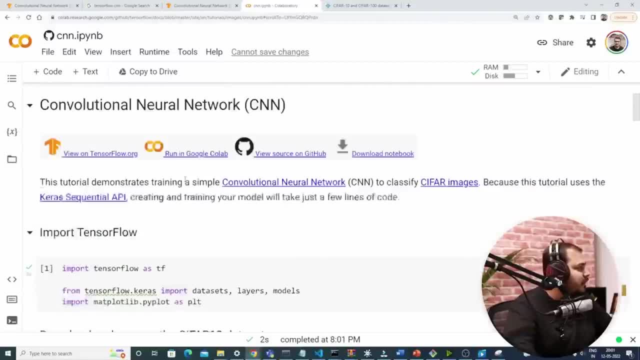 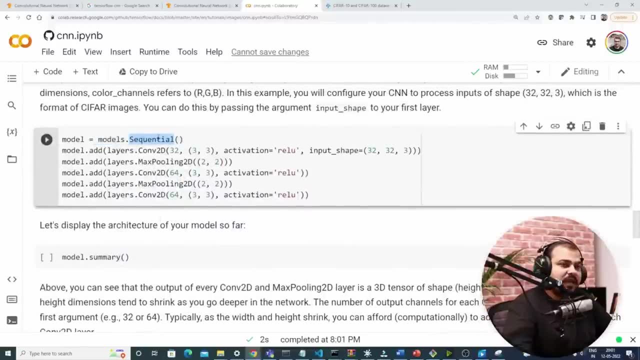 Right, So in this also, we will definitely first let me see that whether I have okay, how many of these models has been imported. Fine, So we have to again initialize with a sequential layer And then we will be using modeladd layerscon2d convolution layer. 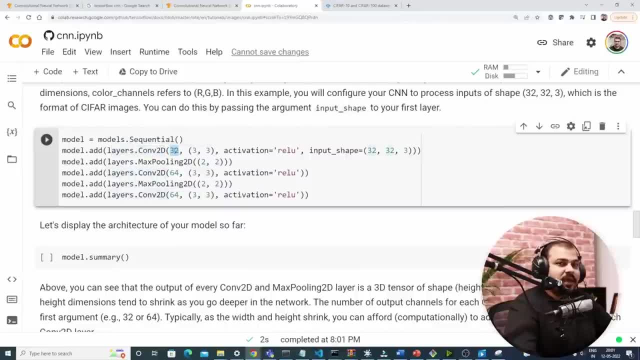 Right Now, in convolution layer, this 32, okay, this 32 will basically be my number of filters. Okay, 32. over here, the first parameter that you see Right, It will be number of filters. So I will use 32 filters. 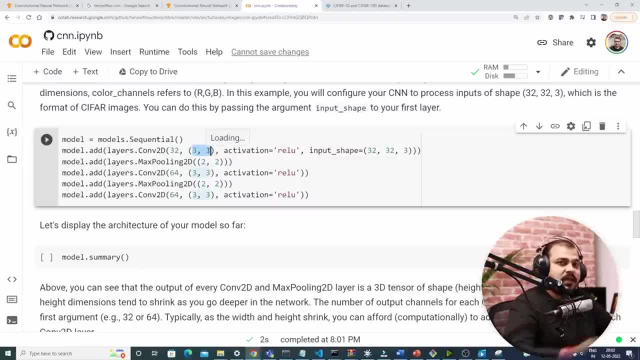 And these filters are nothing but 3x3 size. Okay, Each and every filter will be 3x3 size, But how many total number of filters that we are actually going to use? It is nothing but 32.. Okay, And you know that. 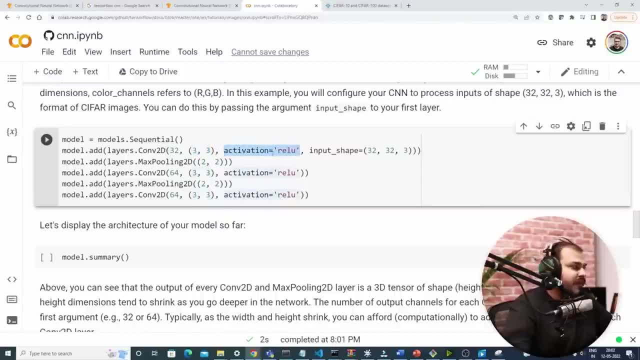 after the convolution operation, I need to apply my activation function as relu. So I have applied my activation function as relu And this is super important, Like what kind of input image we are giving. As I said, that, my input image. 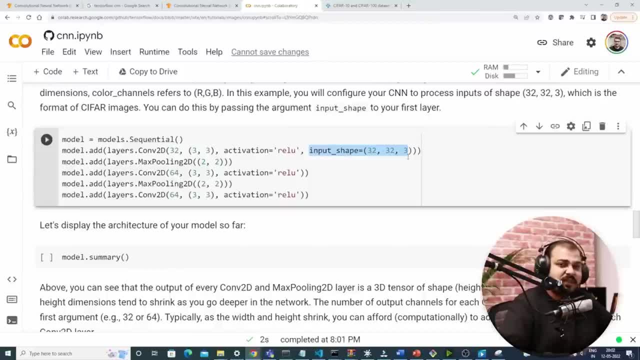 okay, will be basically in a RGB function. If it is in a RGB format, this basically indicates that my input image is 32x32 pixels multiplied by 3 channel. Okay, So here you can basically see the 3 channel. 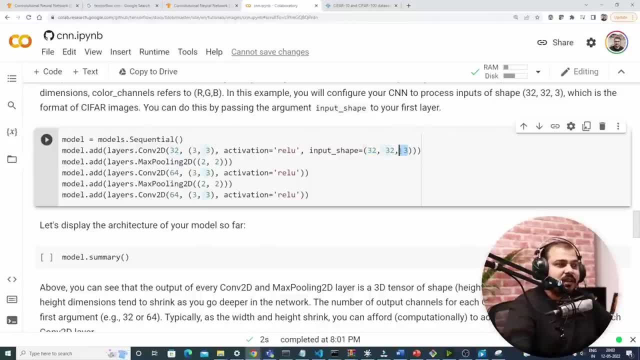 So it is nothing but 32x32x3 based on the 3 channels itself, And then I am going to basically add max pooling layer. So after the convolution layer, I am going to add some max pooling, max pooling layer. 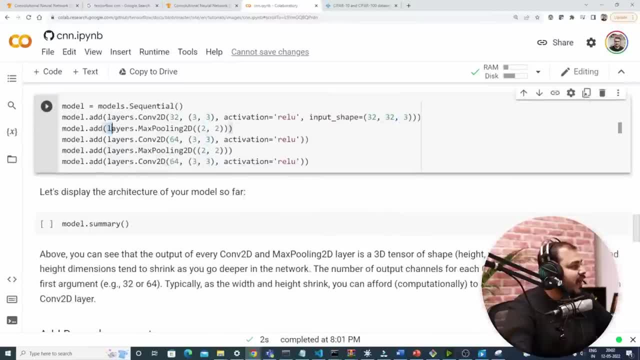 2D layer, Basically like 2x2 matrix. Okay, So it will be a filter of 3. So I am going to basically add max pooling layer. So after the convolution layer, I am going to add some max pooling. 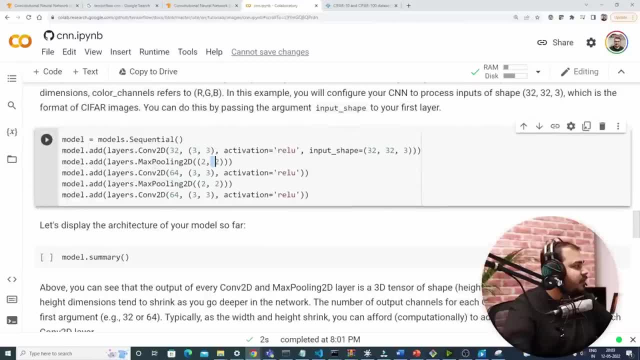 max pooling layer, 2x2 matrix. Okay, So it will be a filter of 2x2.. And similarly I will go and add my another convolution, Then again apply an activation function. Then again I can apply a max pooling layer with 2x2.. 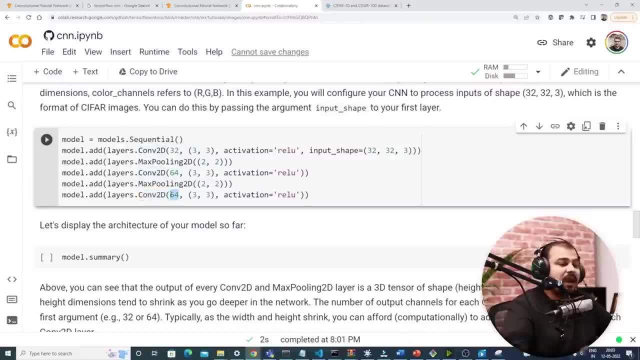 Then again, I am applying a convolution layer Over here, I am specifically using 64 as filters. Now you may be thinking: Krish, how do you decide this number of filters? Okay, See, guys, there is no such thing that you can decide or you can do. 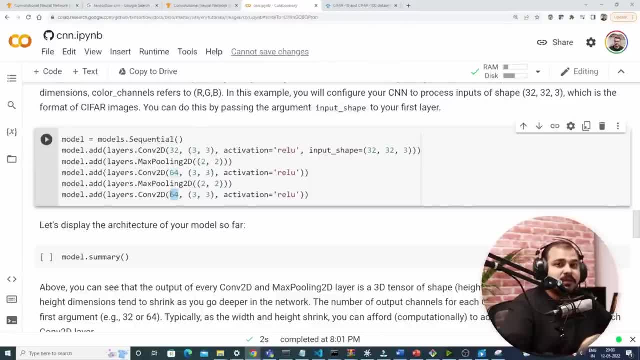 You can write any filters over here, But it is a proper research. that usually happens with filters. Filters are just like a kind of hyperparameter, like how many filters you want to basically solve a specific problem. If you try to see in some of the state of art algorithms, 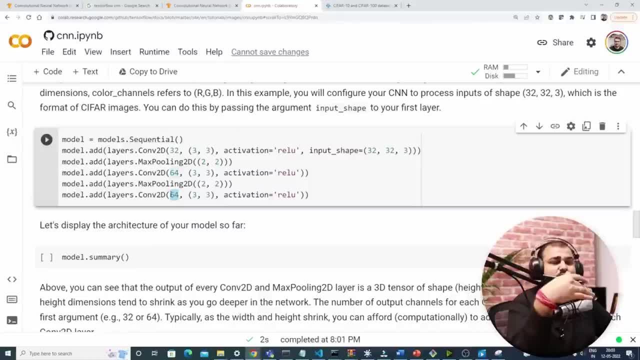 right in convolution neural network. there you will be seeing different, different number of filters, So no such specific thing. Yes, you can try with different, different hyperparameter. You can use 32, 64. You can use the combination of different. 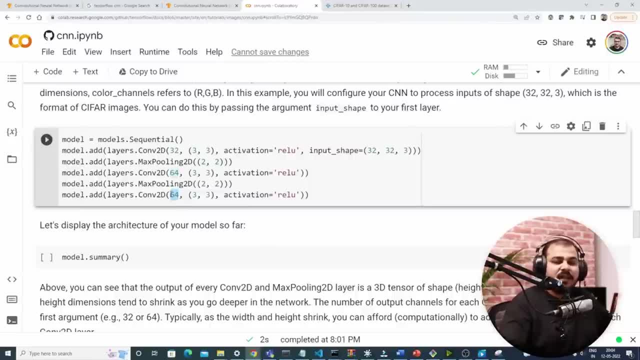 different filter and see how the performance is increasing Right? Other than that, most of the time for different kind of tasks like image classification, object detection, we basically use the state of art algorithm. Okay, So I am just going to execute this. 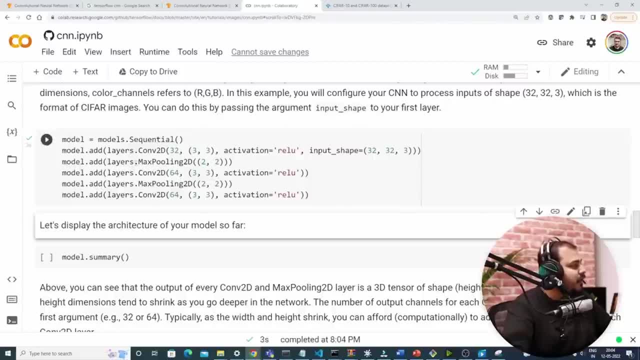 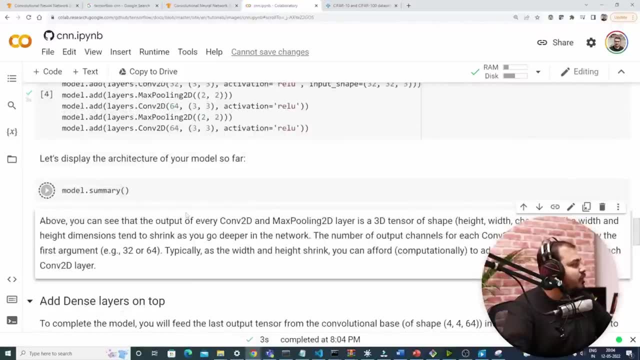 So that is basically means that I have three convolution layer and one two max pooling layer, just stacked horizontally. Finally, if you go and click on modelsummary, you will be able to see the entire summary. See, it starts with convolution 2D layer. 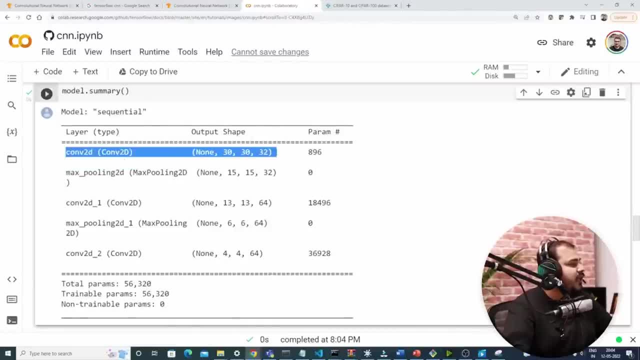 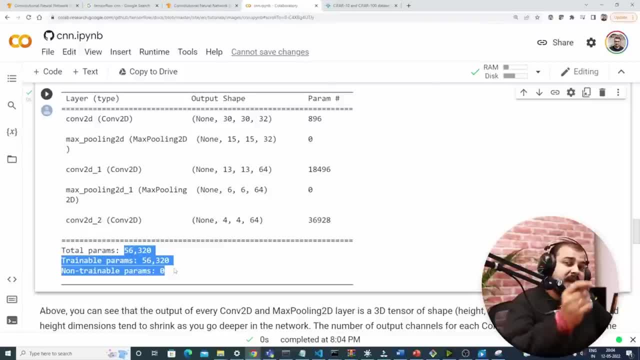 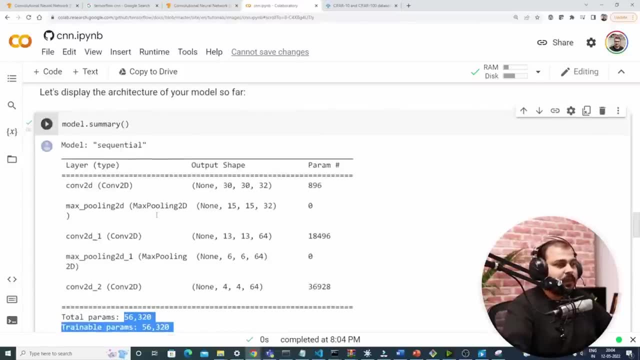 and total number of parameters. this is basically defining, And this parameters even counts the parameter inside the filters. Okay, So by this specific way, you are able to see the entire summary of the model, Like how the model is actually created. 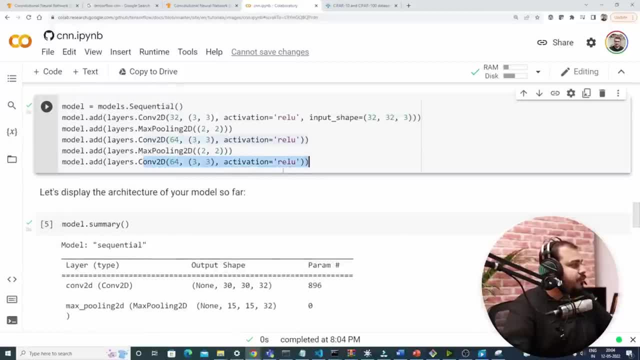 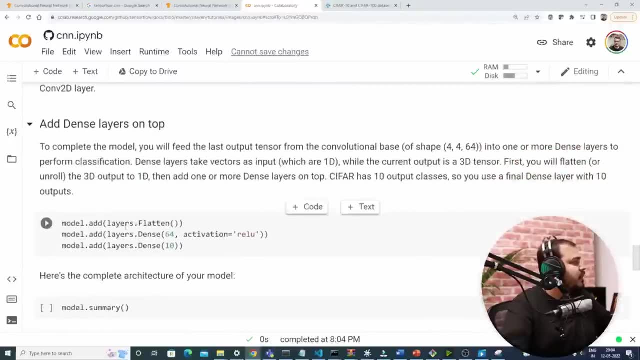 Now till after this. I told you right After we finish of this. you know we can have a flattening layer. Now is the flattening layer defined Here. you can see that modellayer layerflatten. So whatever we had over here. 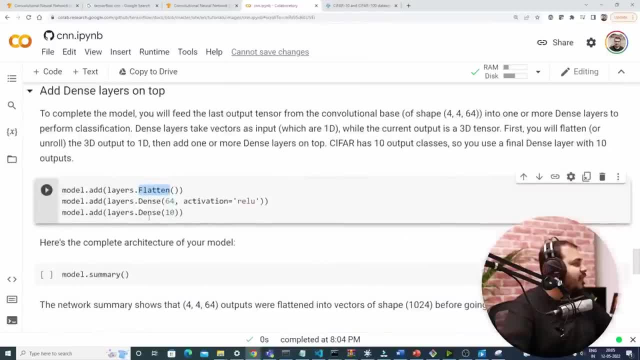 now We are just going to flatten this entire layer and we are going to add it over here, And then I'm going to add a fully connected neuron network with 64 dense neurons, And the total number of output in my data set is 10.. 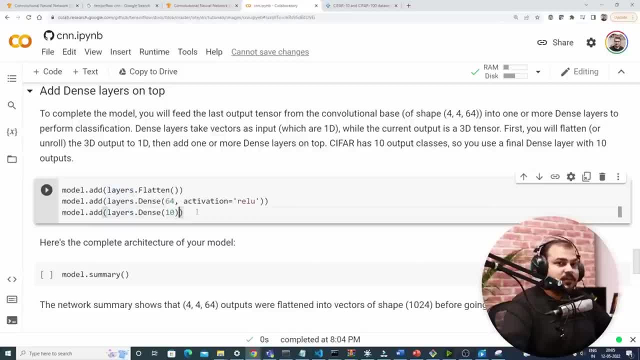 So I'm specifically writing layerdense of 10.. So this is my output layer and this is my hidden layer, right, The ANN layer, which has 64 neurons, And this is basically my flattening process And I've just written layersflatten. 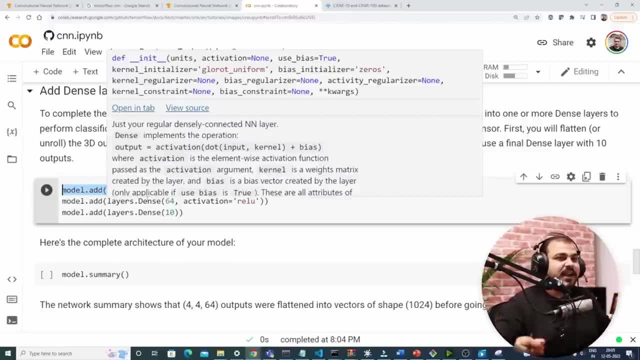 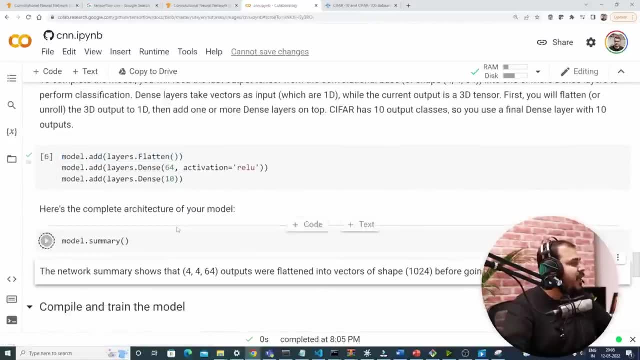 That's it. Whatever is coming after the convolution layer, we are just going to flatten it and we are going to use it. Okay, So once we execute this, you'll be able to see that my model will be ready, And if I probably now go and see modelsummary, here you can see my dense layer, which is my final layer. 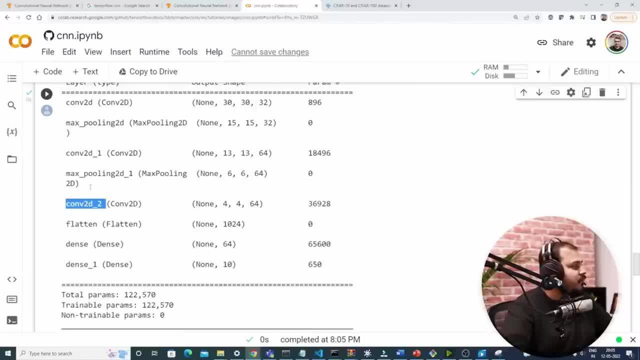 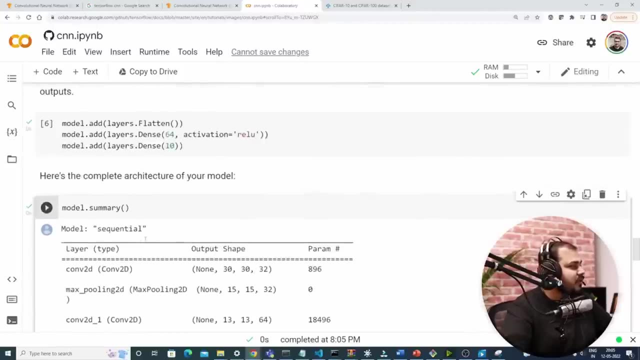 I have my 10 output. Then I have my dense layer, I have my flattened layer, con2d max pooling 2d, 2d, 2d, right. So here I'm specifically getting all the layers that I specifically want. 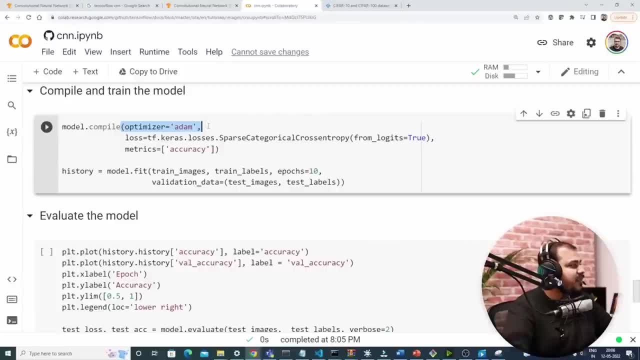 Finally, for the compiler, We'll use the same optimizer, which is called as Adam optimizer, And since we have many, many, many many output, that is, 10 outputs, we are going to use something called a sparse categorical cross entropy. 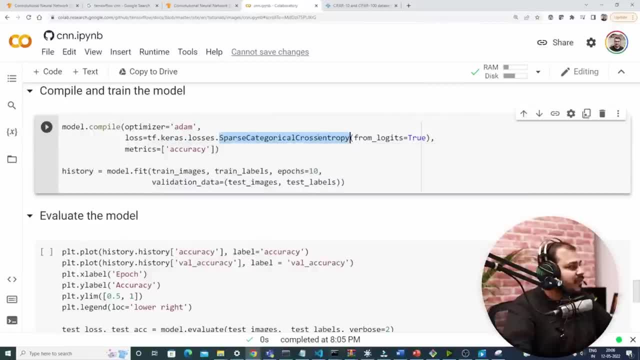 I hope I have discussed about categorical cross entropy, And this is what it is all about. You know we can directly use that in the loss function. And then, finally, you can see my metrics, accuracy, and I'm going to do the fit on train images, train labels, epochs. 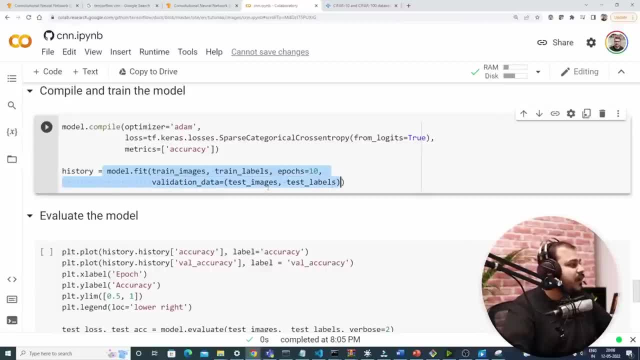 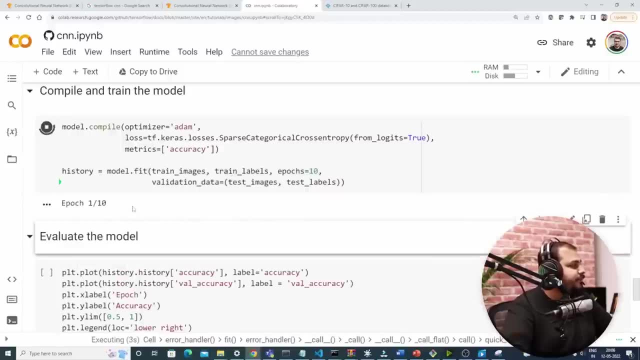 I'm basically Using 10 and the validation data. also, I'm giving my test images and test label. So finally, I execute this and you will be able to see. my epoch will probably start, and let's see how much time it may take. 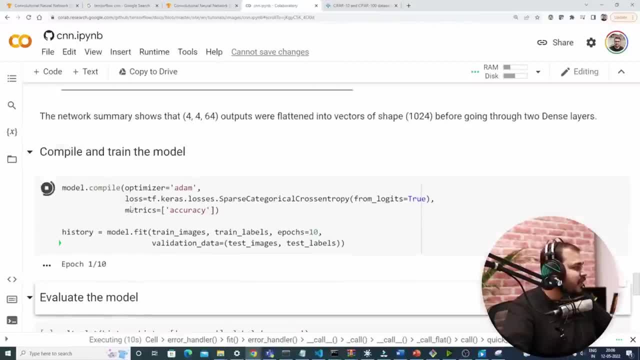 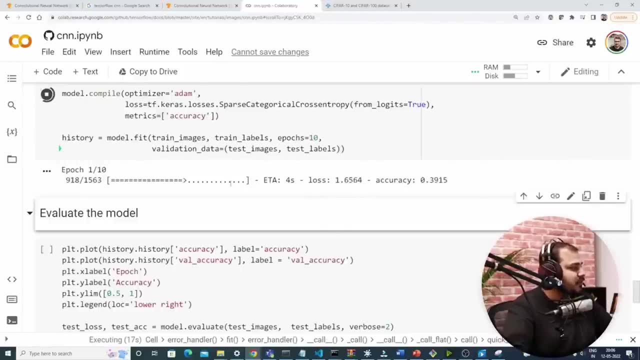 Uh, it depends on the GPU that we are trying to use, but I think this should get completed and started here You can basically say that I'm basically using this one, and here you can see that my Chris is increasing, My loss is decreasing. 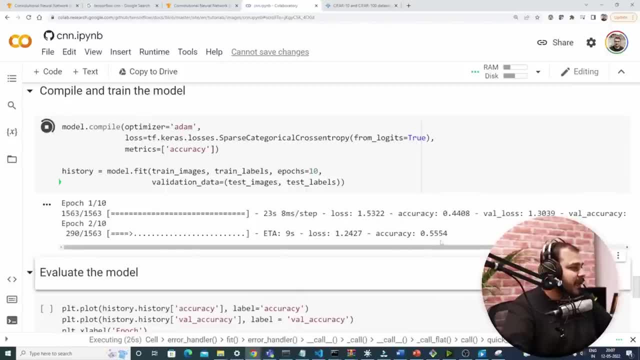 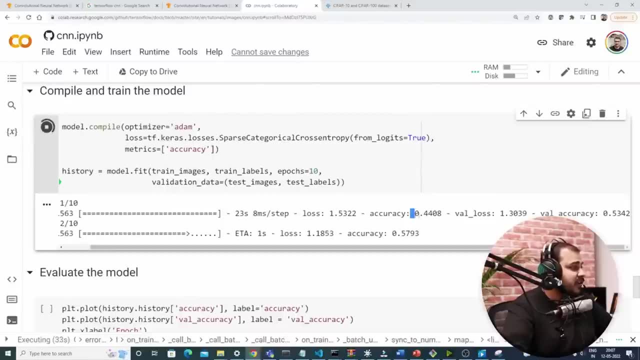 That basically means My neural network is getting trained Well. my accuracy has gone more than 56%. Let's see: the validation accuracy is also 53%. test training Accuracy is 0.44, when my validation increase is much more better. 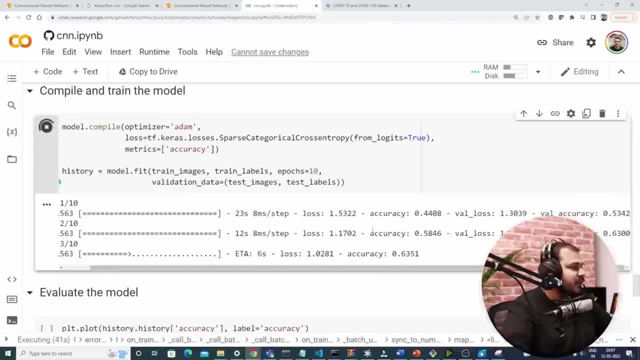 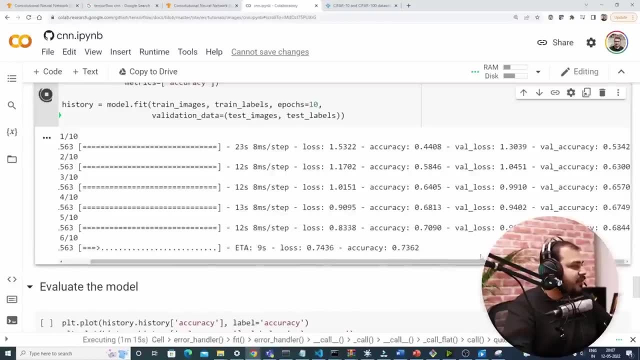 And here you can see, my validation accuracy is much more better than my training accuracy, And this will keep on going right. So we are in the fifth epoch. uh, right now the accuracy is 70%, validation increases 68.. We are going on good. 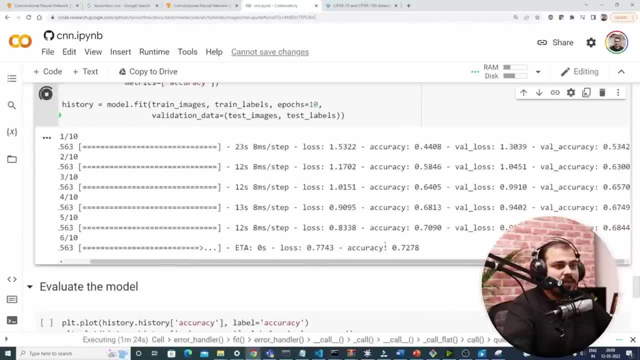 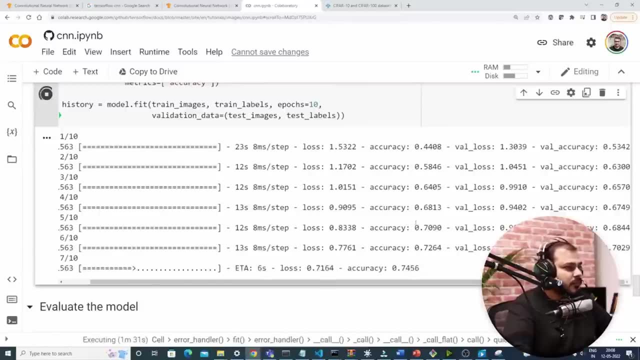 And on this also, You can apply early stop, you know. so early stop can also be applied onto this. That I'll give you as a task. Okay, so here it is. Your accuracy has got to 74% optimizes. 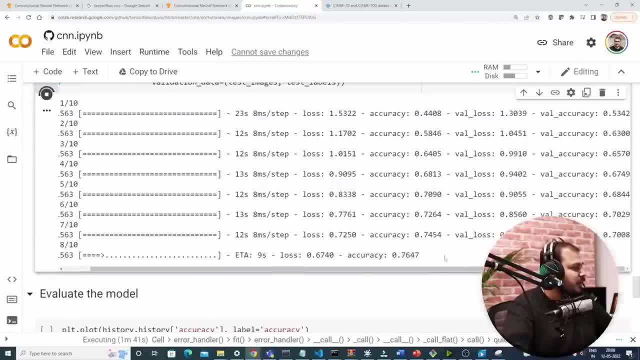 You definitely use Adam optimizer because it is the currently the best one. Okay, Two more epochs and then we'll stop over here just to see that how things are going on. Right? So 76%, 70%, 70%, 70%. 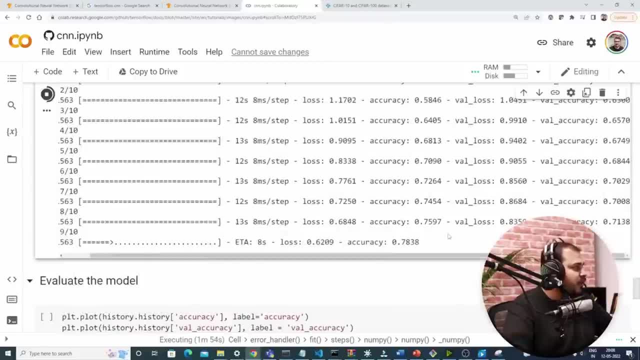 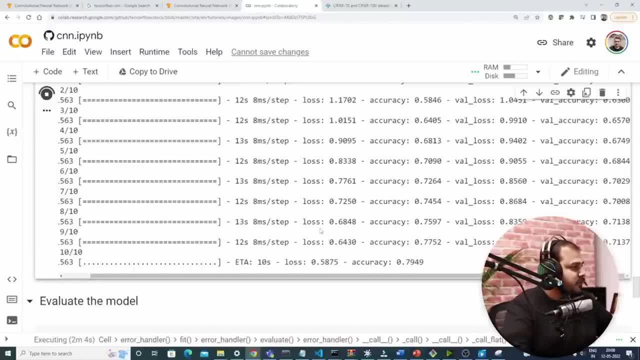 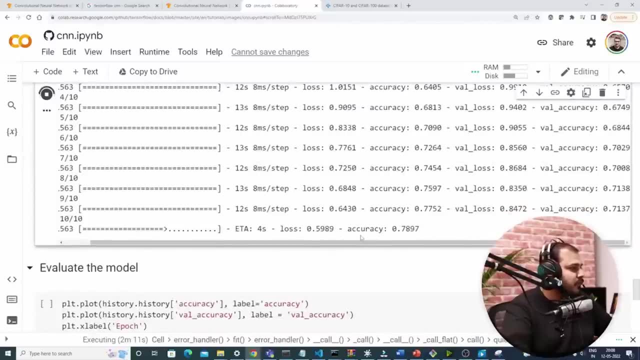 Okay, Perfect Perfectos. Now I'm into my 79% accuracy: 77.. Validation is 71,, which is good. I think it will be more than sufficient if we complete the 10 epochs, And I think you can also do it. 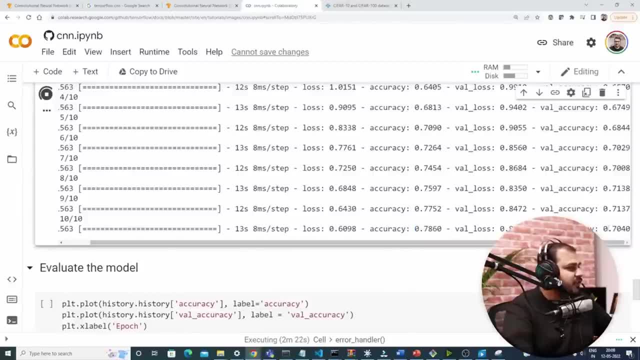 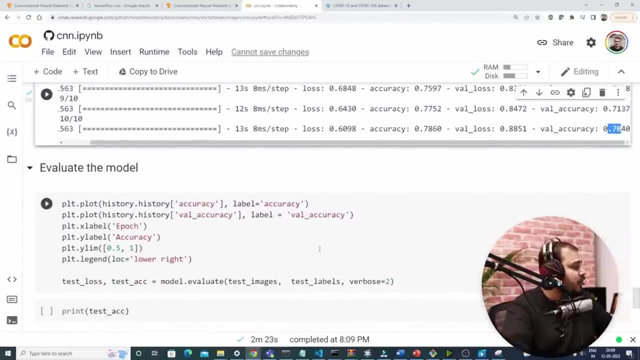 So, finally, I'm getting able to get 78% And my validation accuracy is 70%. I have stopped over here. Okay, You can continue the training, however, how many epochs you want. And finally, I will just plot the history: accuracy, label accuracy, and all with respect. 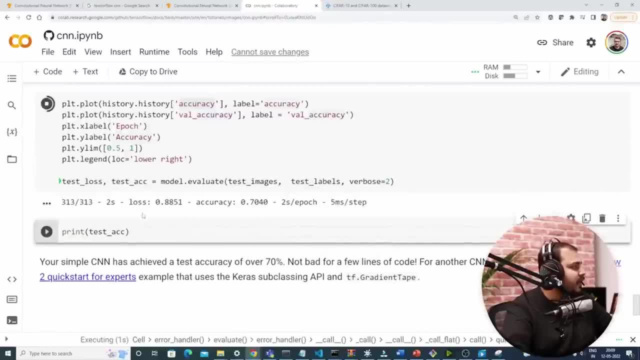 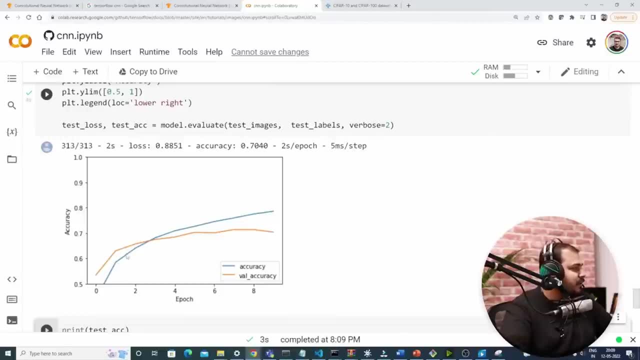 to this particular plotting And we'll also evaluate to this thing, Right. So here it is. This is my graph. This looks good, Right? The accuracy went up. The test accuracy, or validation accuracy was going down, So we stopped over there.